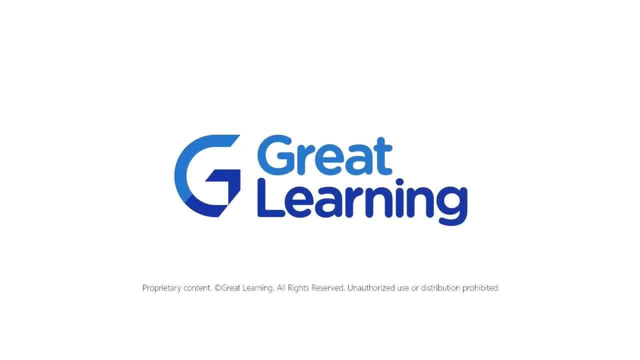 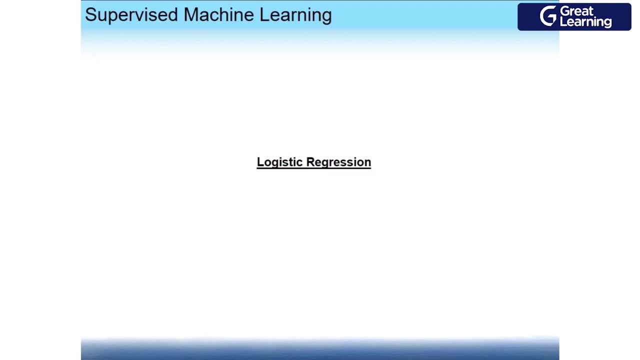 So let us see what this logistic is. The name logistic regression is slightly a misnomer. It is used for classification. it cannot be used for regression. ok, So the name says regression, but there is a reason why it is called regression, not logistic classifier. 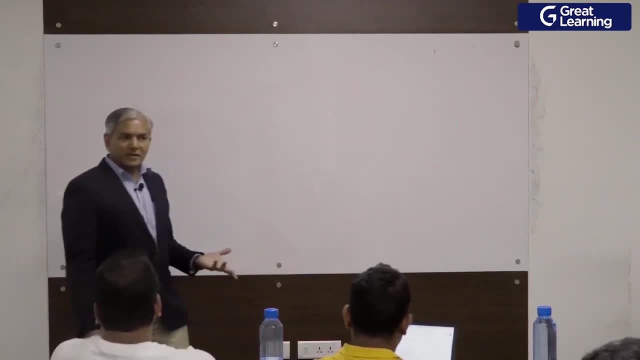 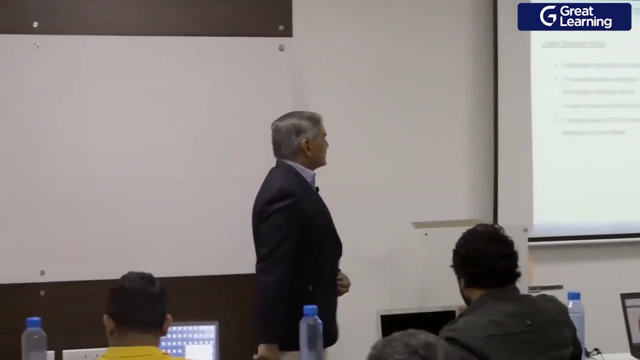 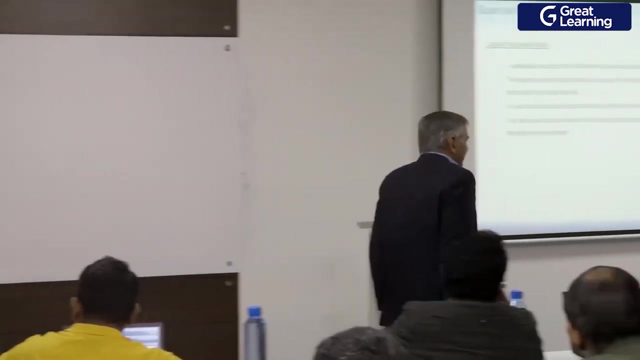 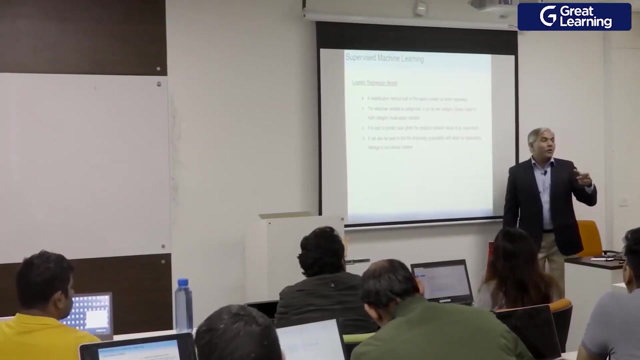 The reason is under the hood: logistic regression uses linear models, linear regression. that is the reason. It is a classification method based on linear regression. The response variable, that is, the target variable, can be binary class, default or non-default, or diabetic, non-diabetic, or it can be multi-class classification. also, I can use logistic regression to find: 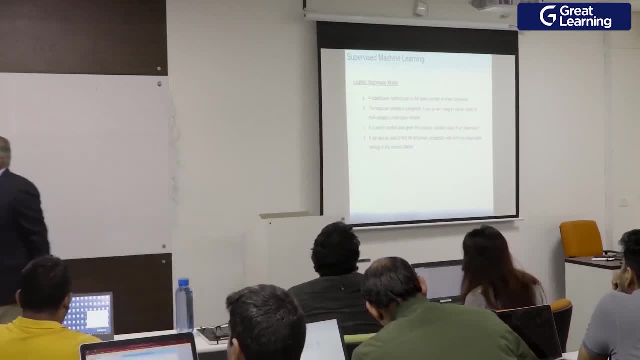 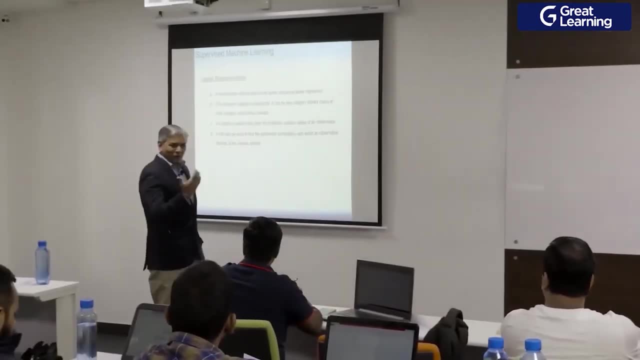 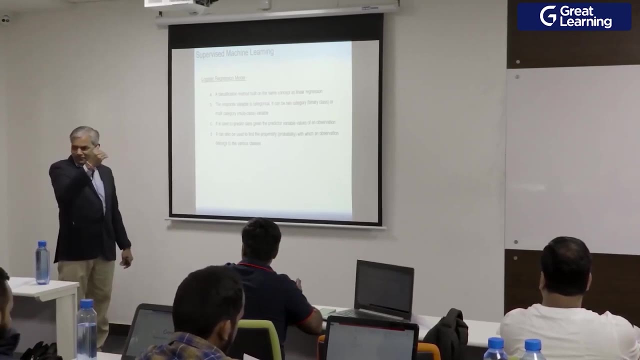 out Charlie Kernel for optical character recognition. I can do that And in my personal experience I have seen and I have also read some papers about it. when you compare models, often logistic regression comes out on the top, If not exactly on the top, at least top few top two or three. 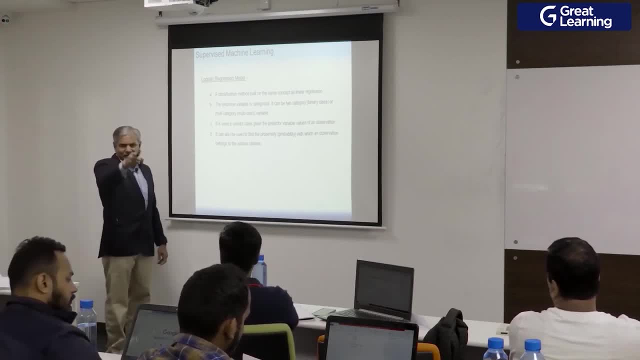 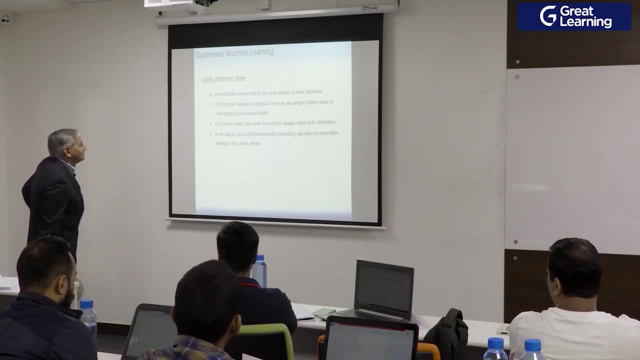 ok for classifications. So I am going to start by showing you binary classification, class classification also, Given your independent variables, what is the class likely to be? that is the objective of this model. I can also use a function available in scikit-learn. 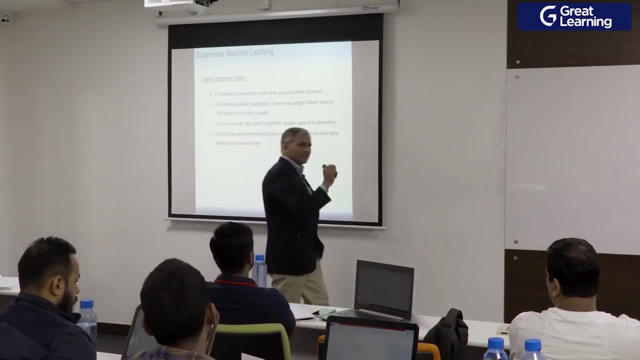 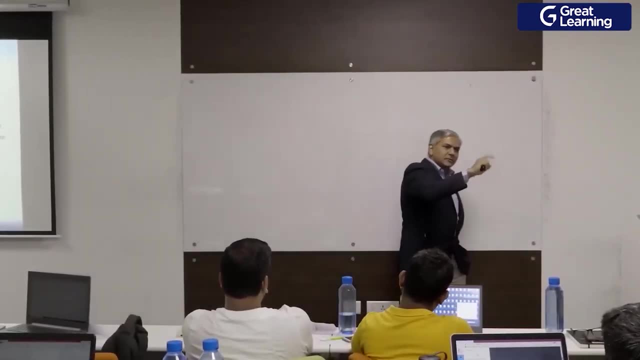 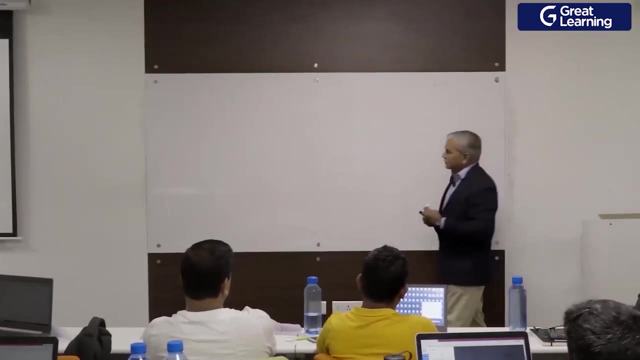 where, instead of defining which class an observation belongs to or test record belongs to, I can print out what is the probability that this record belongs to this class versus this class. I can even print probabilities. This particular function is nothing unique to this. it is. 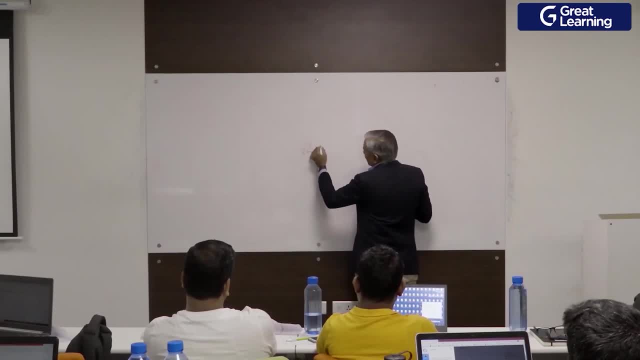 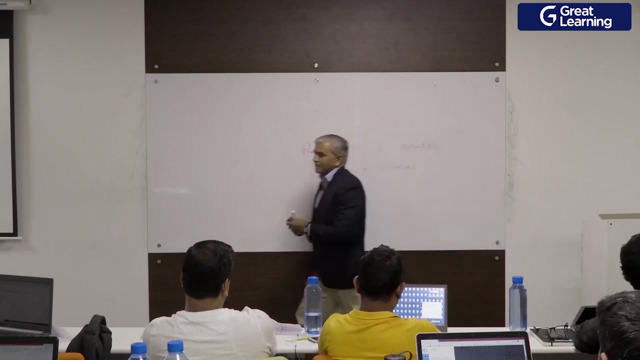 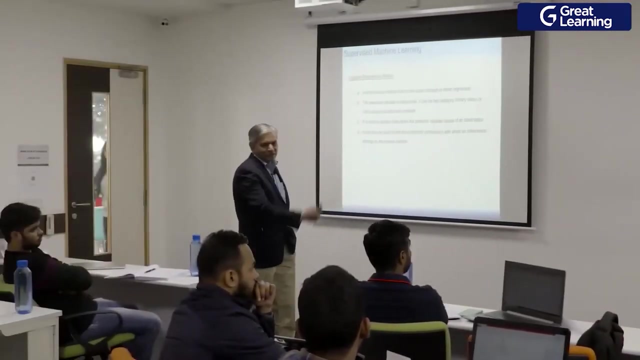 available in all probability based models: Predict. you remember we used predict. we just add underscore proba. This function will print out probability values. If you go for just predict, this will print out. the classes Decision tree also has this Naive Bayes algorithm also has this logistic, also has this Predict. 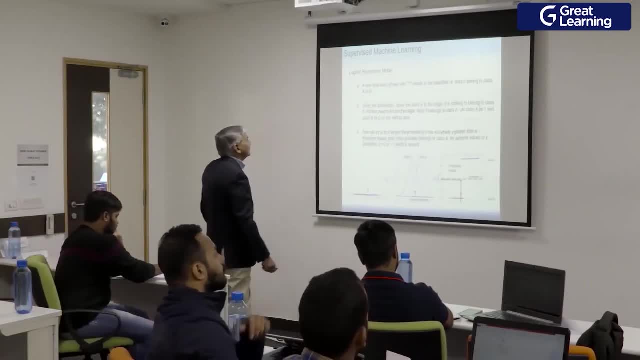 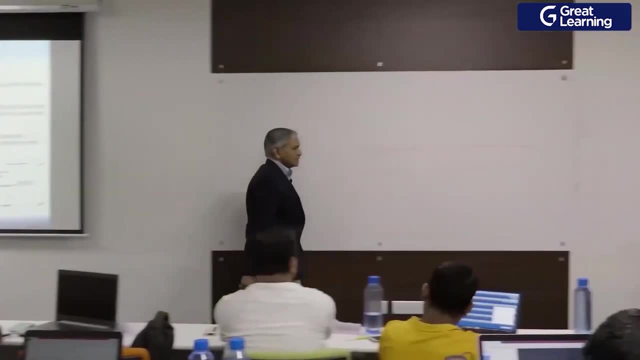 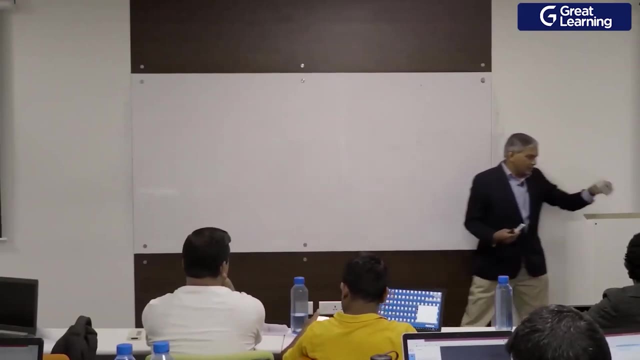 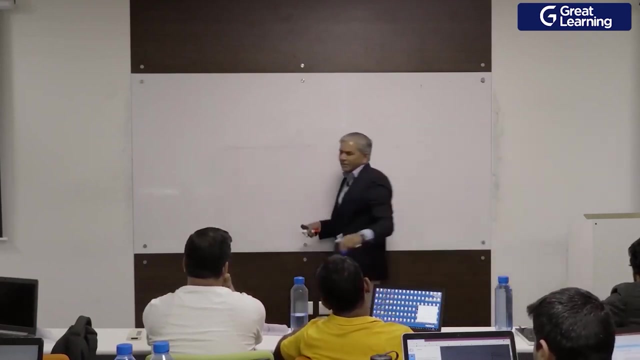 underscore proba. Let us take a hypothetical situation. do not worry about the PVT. Let us take a situation and discuss this concept, And for that we are going to use three colors. You are a data scientist. you are working in a bank. 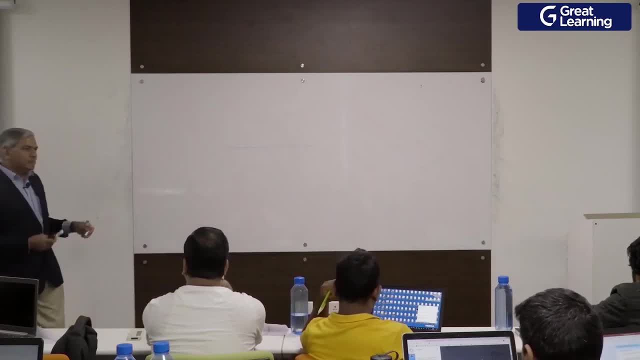 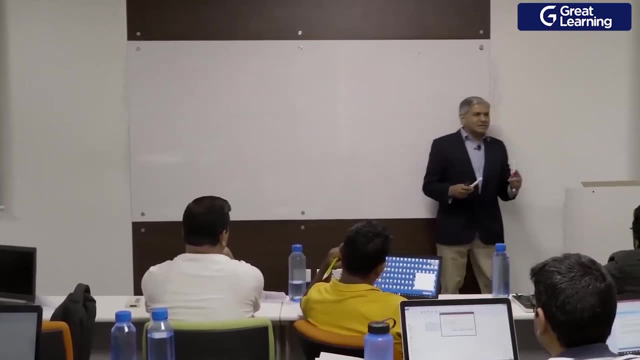 and you have been tasked with. you have been given a responsibility to build a model where the model will take certain inputs and the output of the model will be: is this person likely to default If I give him loan? is this person likely to be a defaulter or a? 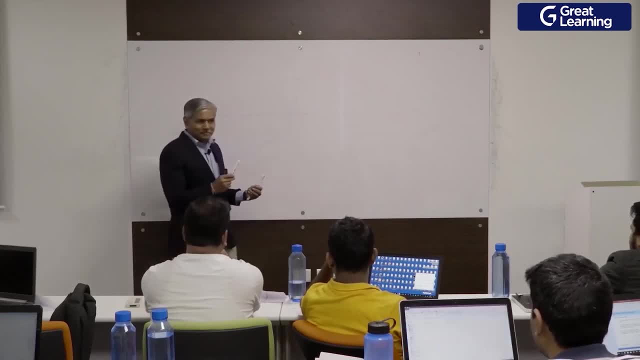 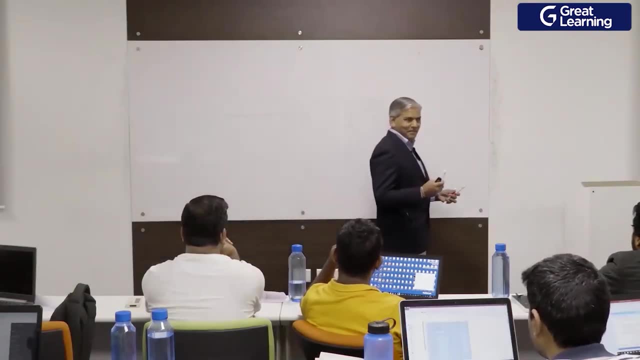 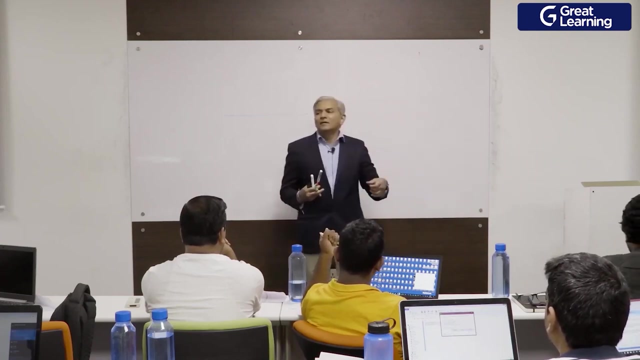 non-defaulter, You have to build that model. Okay, So what kind of data will you need to build such models? So, past history in terms of Sibyl score: okay, Sibyl score is an output of a model. 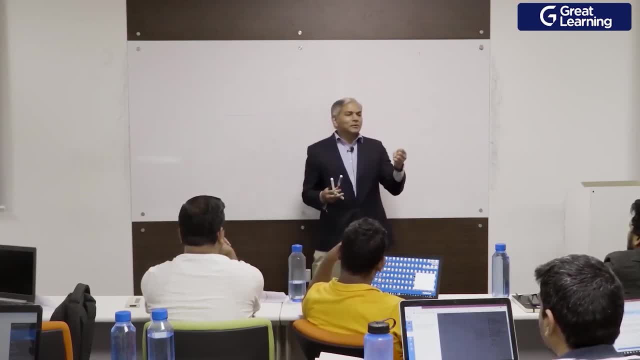 actually So let us keep Sibyl score aside. You need his age, gender, income, any past loans he has taken, any property he has, so on and so forth. so many things. Now let us assume that he is a non-defaulter or a non-defaulter. Now, let us assume that he is a non-defaulter or a non-defaulter. 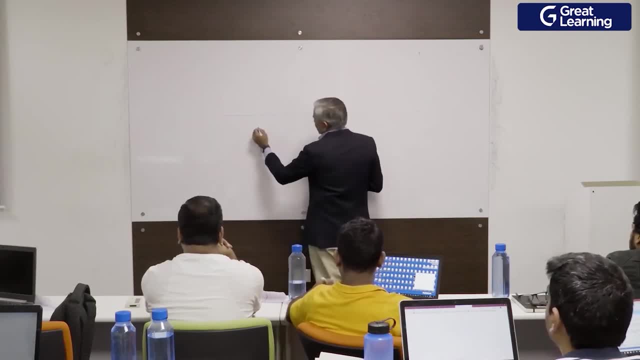 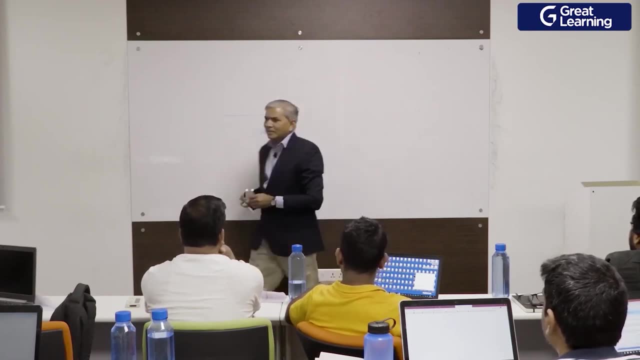 Now, let us assume that he is a non-defaulter or a non-defaulter. Now, let us assume that one of the things given to you is his income. Forget it. This is a touchy subject, So let us call it age. Okay, One of the inputs given to you is the age of the people. So you have. 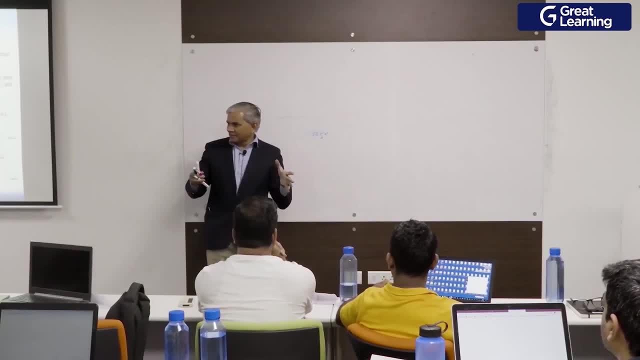 the past data with you. The bank has given you a past data set. In the data set you have both defaulters, non-defaulters, and one of the columns in the data set is age. You notice that. you notice a pattern here. The pattern. 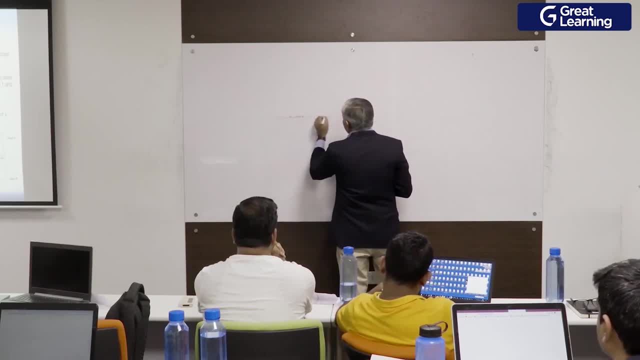 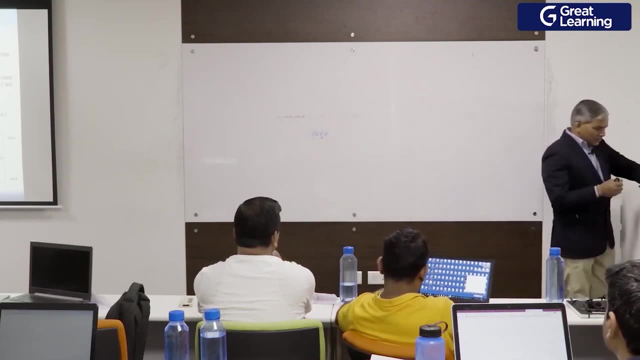 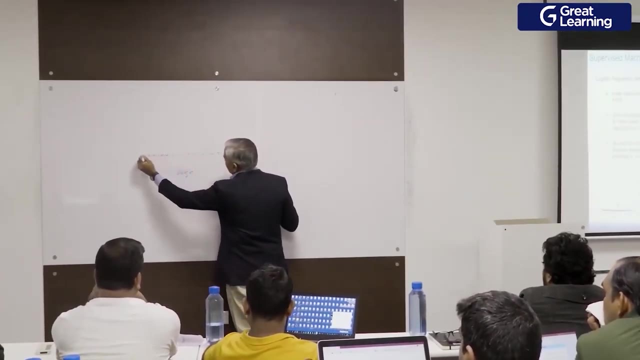 is most of the defaulters. most, not all. most of the defaulters are in the lower age bracket. Okay, And you also notice most of the non-defaulters are concentrated in higher age bracket, But that does not mean there are no non-defaulters in lower age, Okay. 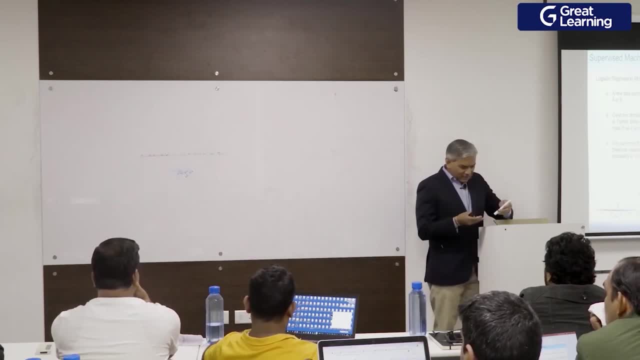 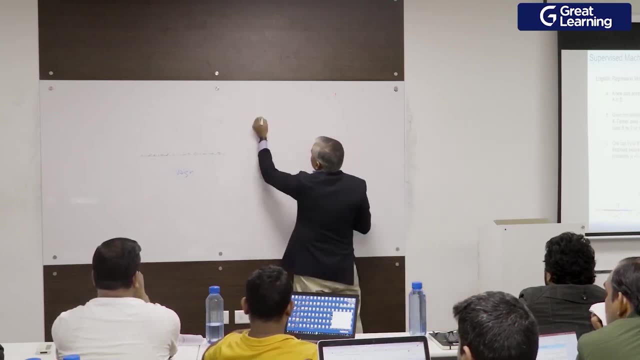 You observe this pattern. Now, since there are two classes here, what we are going to do is we are going to say: green class, we are going to assign a numerical value 1, red class: numerical value 0. Remember, 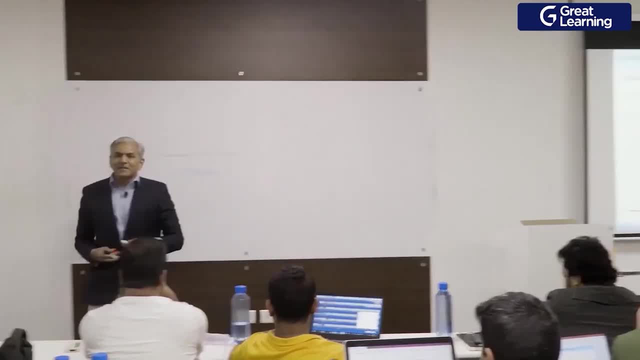 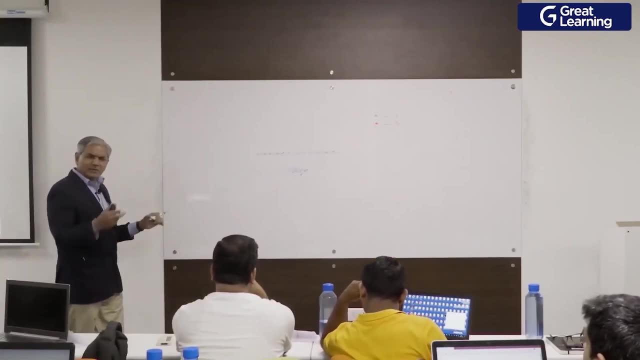 we cannot work on string data types, So the target columns will be assigned numerical types. Okay, Why 1 to this, Why 0 to that? No reason, You can flip it also if you wish, But we assign a value: 0 and 1.. We do not assign any other value, We assign only 0 and 1.. There, 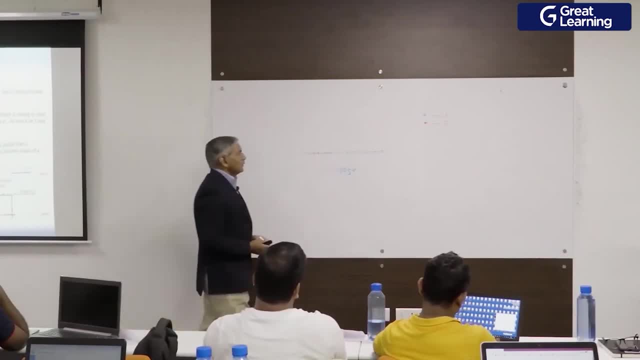 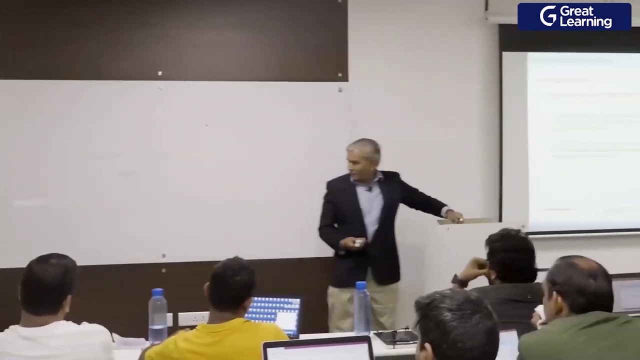 is a reason for that. Okay, Now your objective. yeah, Now you find that the pattern over here: as income increases, you find more greens, As income decreases, you find more reds. You have done a linear model already. So what you do is you try to build a linear model here. So you say: 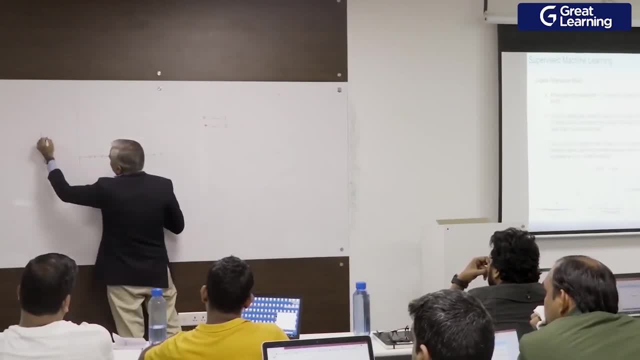 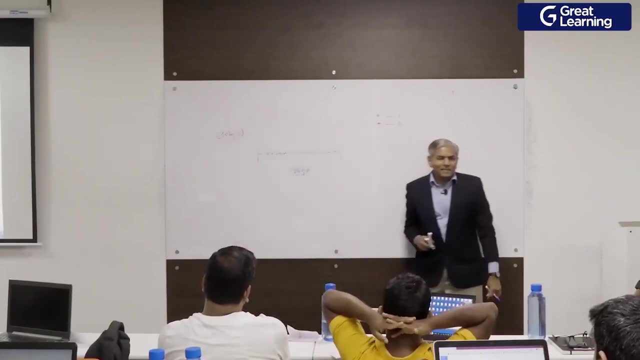 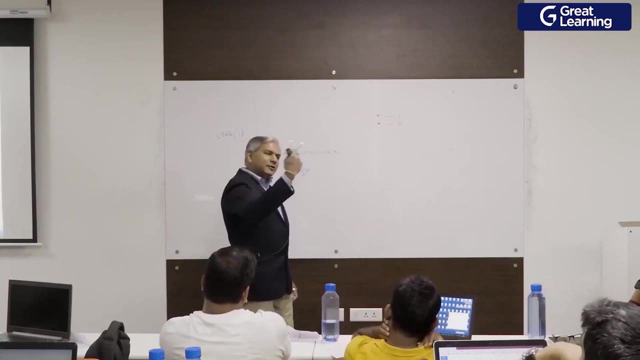 let the y-axis be probability of belonging to Any one of the classes. let us call it 1.. The y-axis is probability of belonging to class 1.. You can actually take it as probability of belonging to class 0 also, if you like. 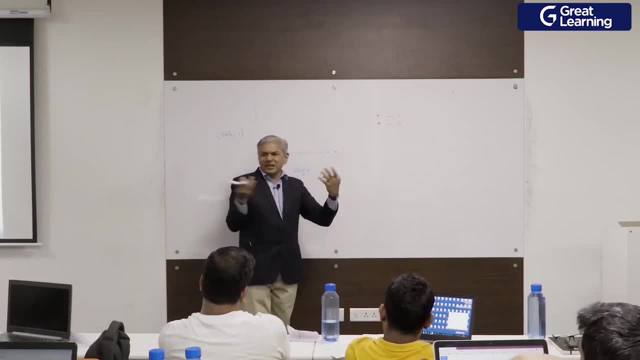 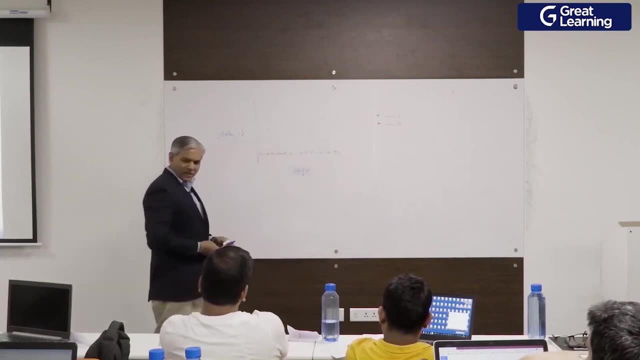 The two probabilities will be inverse of each other, So you can take any one you like. Alright. So when you build a linear model, the linear model, anybody has a black pen here. black black, No, no, this pen, Oh, okay. 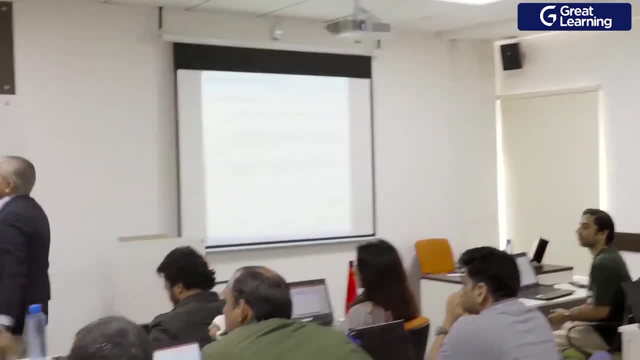 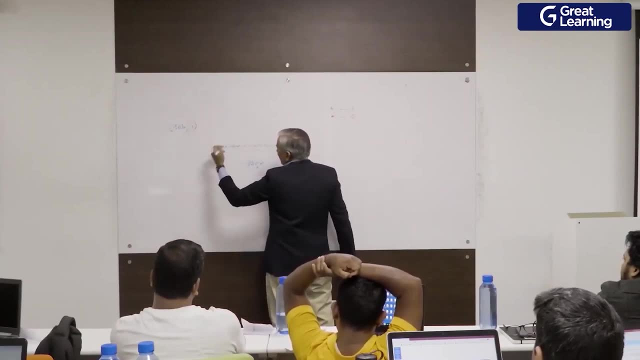 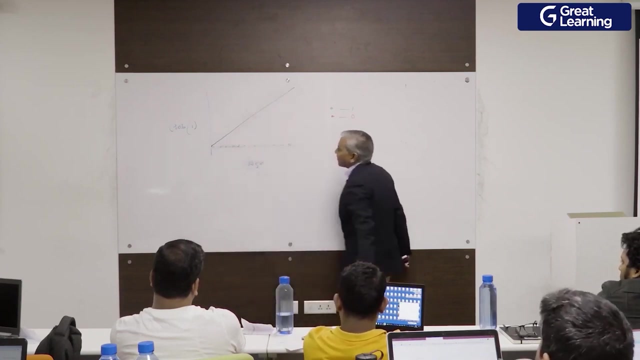 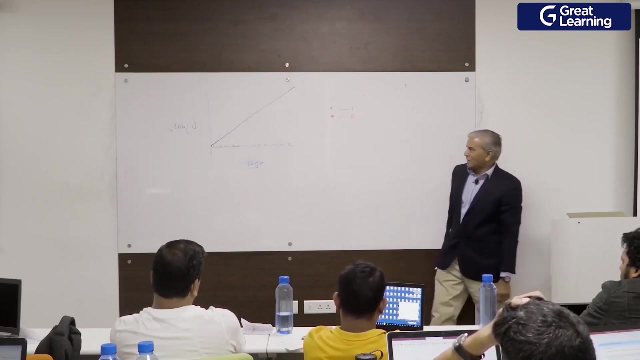 Now you will notice that as the age increases, if this is the probability, the probability of somebody being belonging to green- the probability increases linearly. Probability increases. I can representable linear models If I had taken this as 0,. if this was 0, then 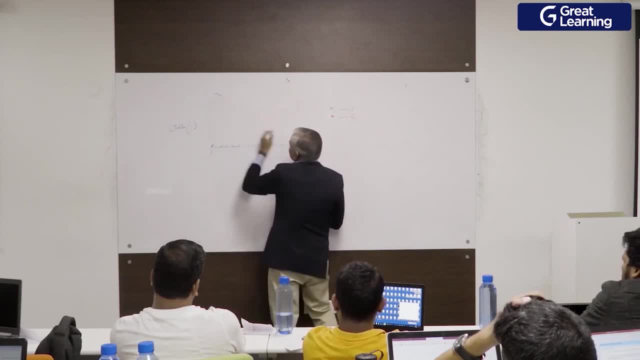 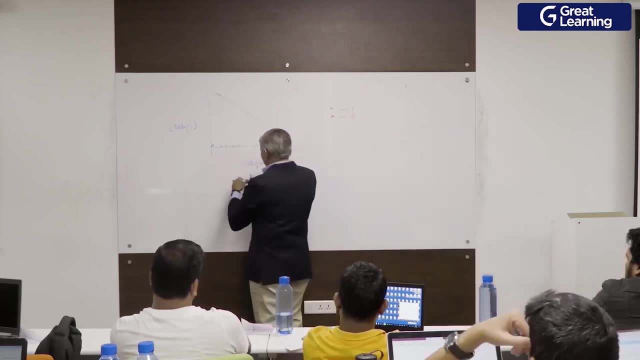 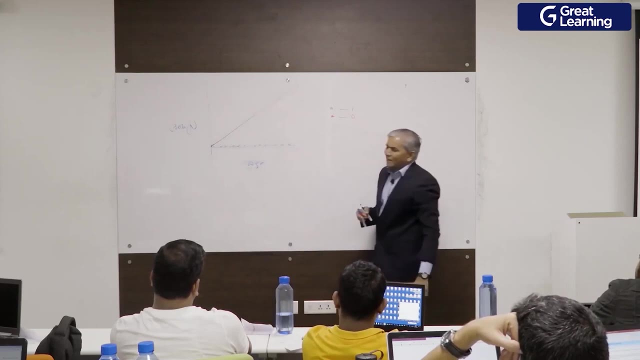 this line. how would it look? It will be reverse. That is the difference. So you can use any line. Okay, So I am taking this as 1, for ease of explanation, because you will be able to connect to what we did yesterday. So the line will look something like this. So this: 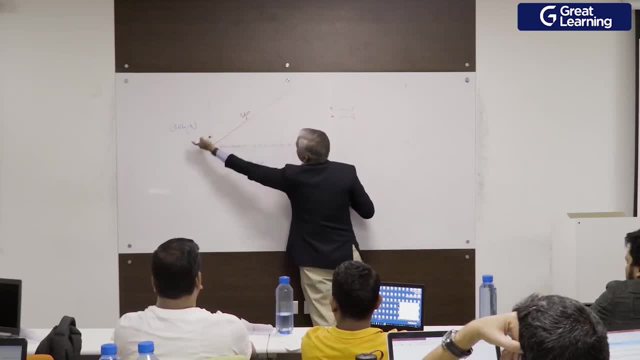 line y equal to y is probability of belonging to blue class. is related to m, x, x. is this variable plus c, c. So this is the probability of belonging to blue class. So this is the probability of belonging to blue class. So this is the probability of belonging to blue. 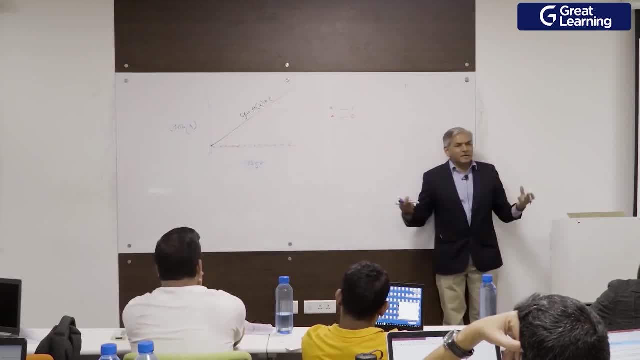 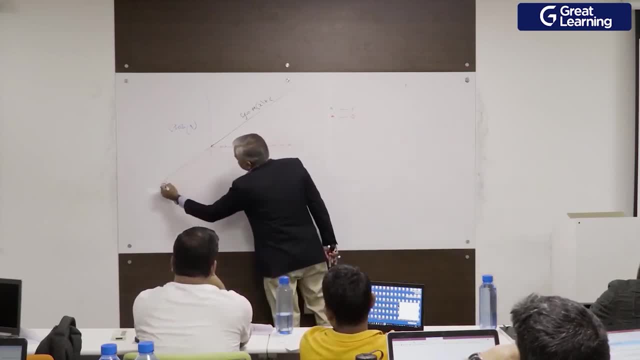 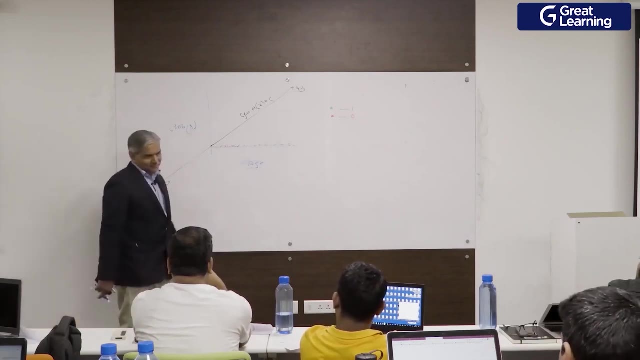 the linear model is. linear models go to infinity. minus plus. Probabilities have to be within 0 and 1.. It cannot be below 0 or above 1.. So we cannot use a linear model. We use another technique where we transform over and so on. 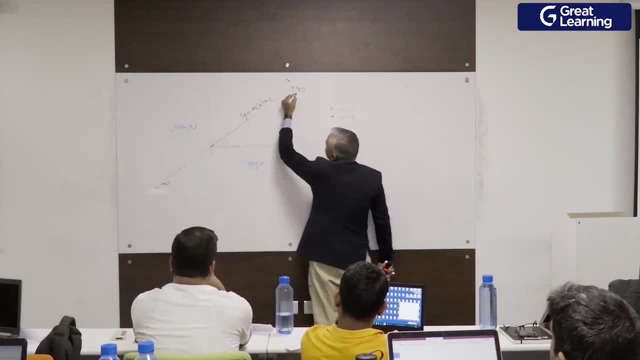 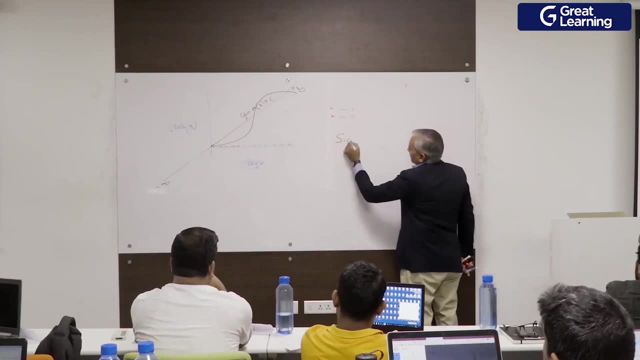 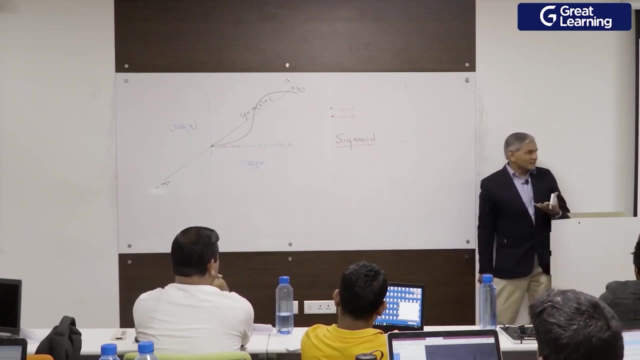 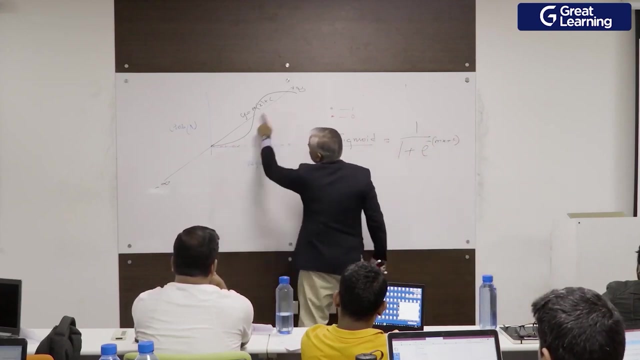 where we transform this line into an S curve. This S curve is called a sigmoid and it is very easy to achieve this. The sigmoid is nothing but 1 by 1 plus e e is Euler constant we use in mathematics- minus mx plus c. So this best fit line, the best fit line which, 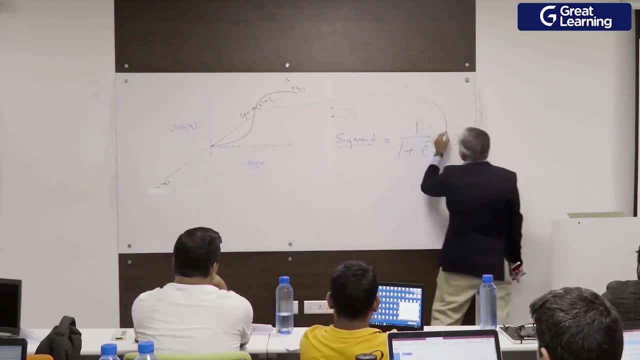 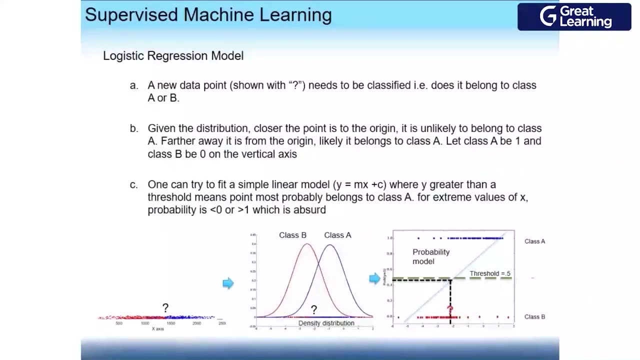 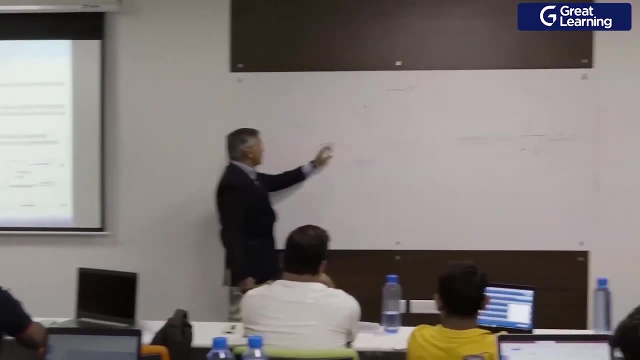 is found for you, this best fit line, is fed into this transformation, this mathematical formula. The result of this transformation is this curve, yeah, sigmoid curve. the property is: it will reach 0 at infinity. it will reach 1 at infinity. 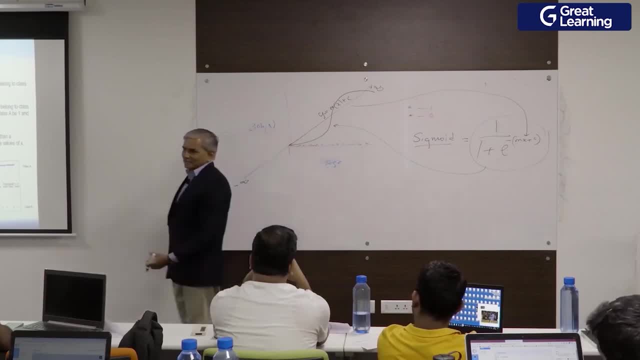 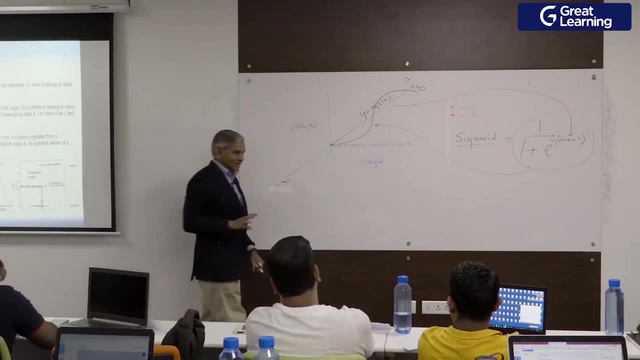 That is exactly the property of a probability distribution. Now let us interpret what this formula is saying. Keep in mind, we are building the model, so which means we are in training set. So in training set, we already know the labels of every record right, The algorithm. 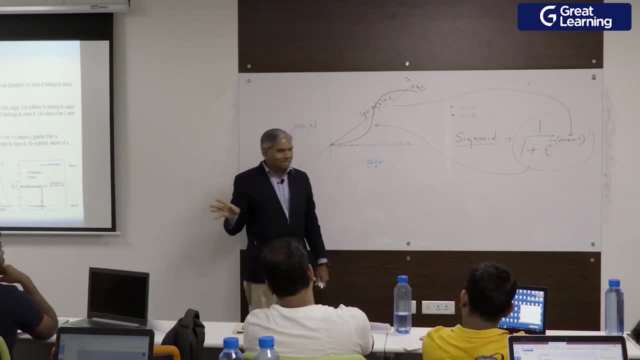 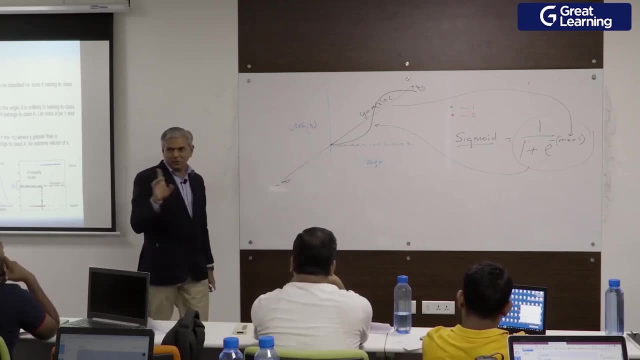 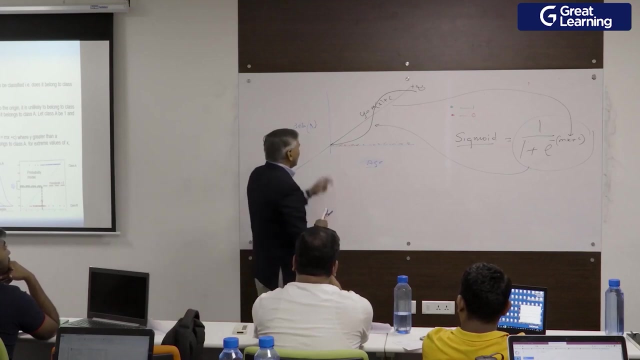 gets both the input variables and the output variable, x and y. So all the labels are already known and the labels are shown in the color over here. Are you all ok? Shall we proceed Now? what the models? now that I got sigmoid, I will remove this this. 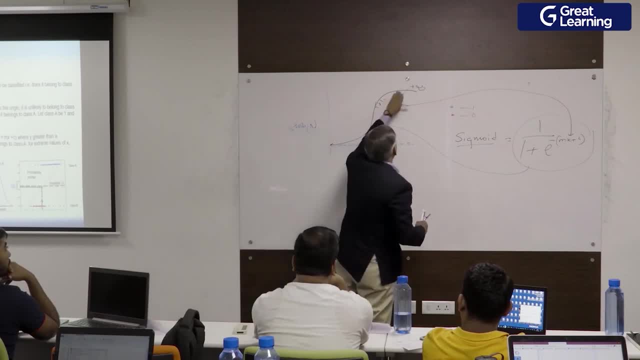 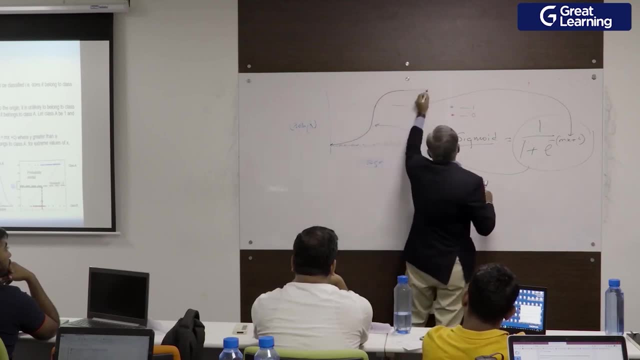 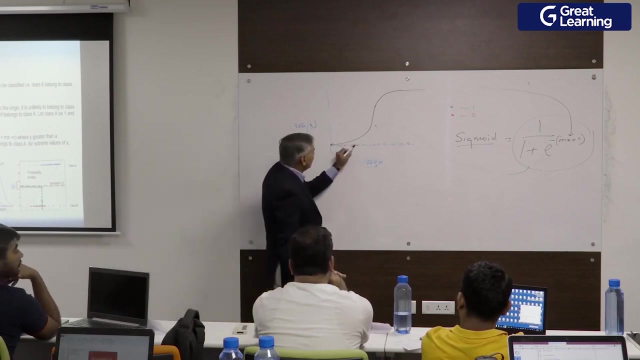 line. I will remove this line. ok, This is going to infinity. We do not even need this, we do not even need this. Now, what this model is telling you. let us look at that, If you take this red point. look at this, if you take this red point, what the model is saying. 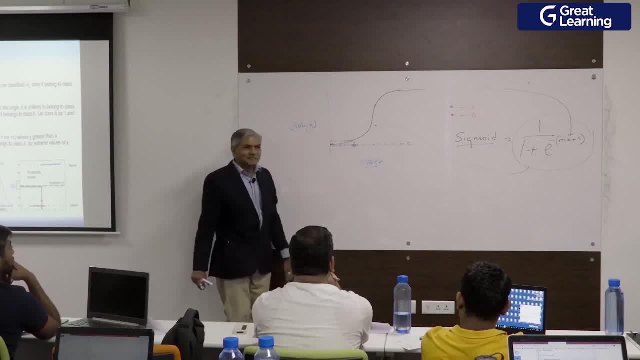 is the probability of belonging to blue class? What is the probability of this guy, Suppose we do not know the color? What is the probability of this point belonging to blue class? It is very low, which means it belongs to the red class. So the model, prediction and actuals. 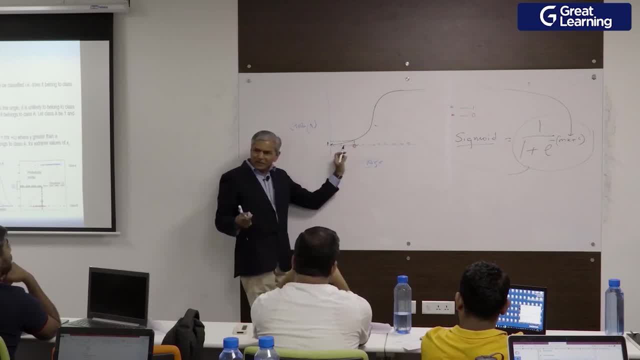 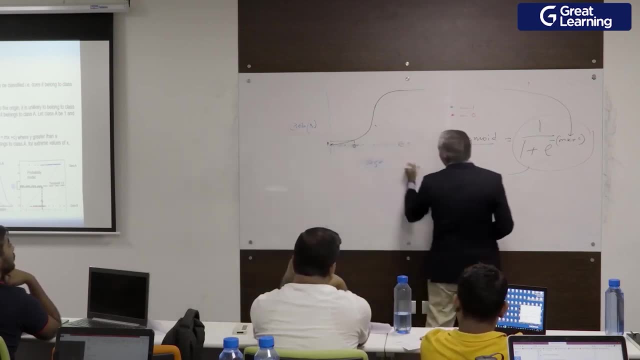 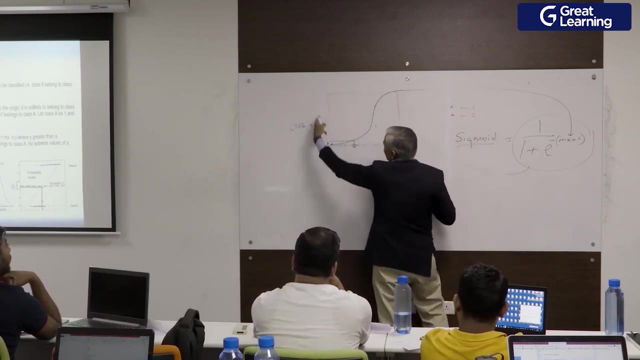 are matching here, The model prediction and the actual label. both of them are matching. Take this green one. What the model is saying is: what is the probability that this green point belongs to blue class? This is probability of blue class. right, The probability is very high. 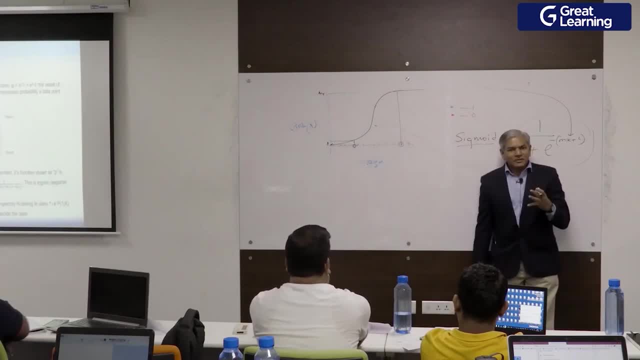 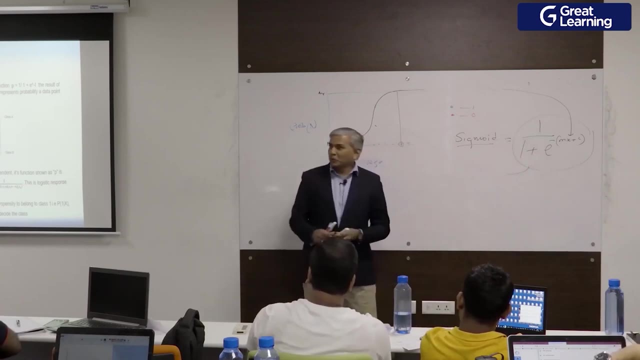 and he is actually green. So both prediction and actuals match right. Hey lady, are you with me? Sure, 100 percent. Ok, Do not get left behind your expressions. tell me a lot of stories. I have content more. 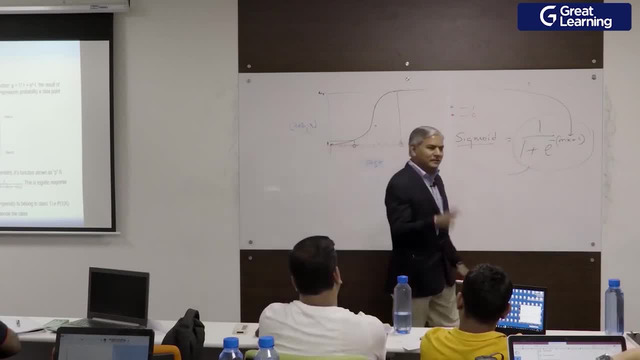 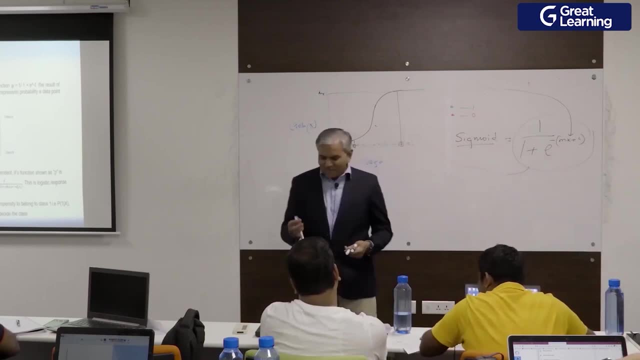 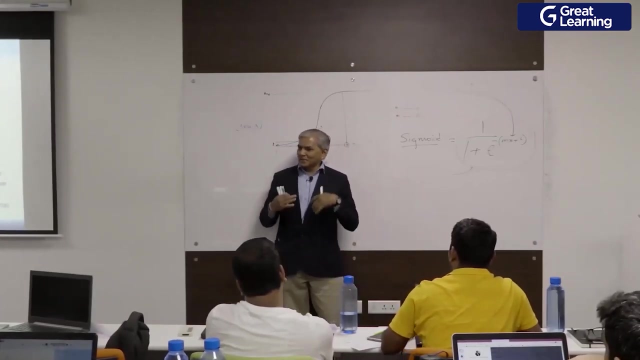 than I lost count- more than 250 sessions now in data science. So I built a model. You know what is coming right. So looking at the place, the position people occupy in the class, I can guess a lot of things about the person. Believe me, we all follow patterns. 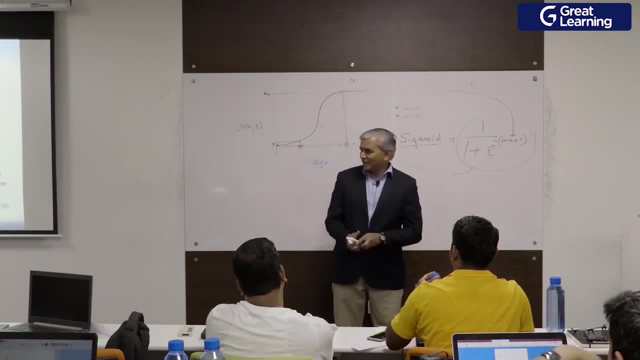 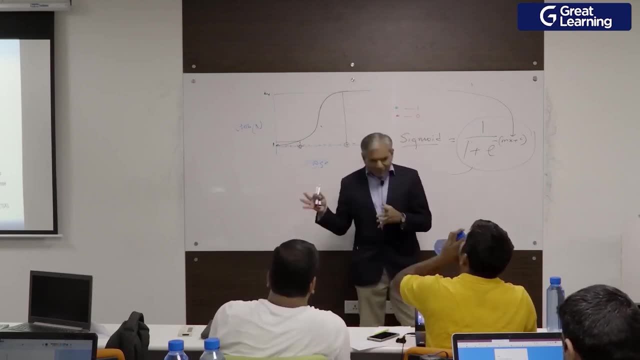 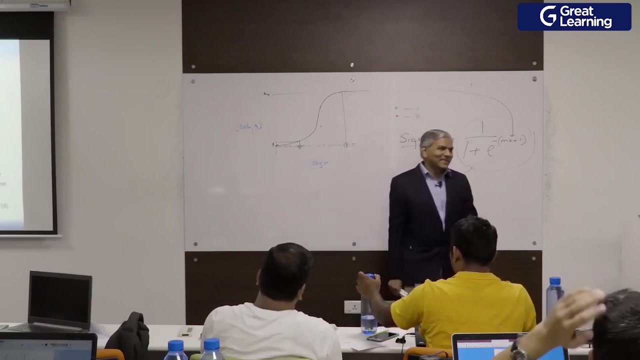 and you will be surprised. what is this pattern without fail, Based on the position people occupy in the class? of course, late comers. they don't have a choice, but people who come early based on the positions they occupy. I can draw lot of conclusions, inferences, from there. So people who are feeling 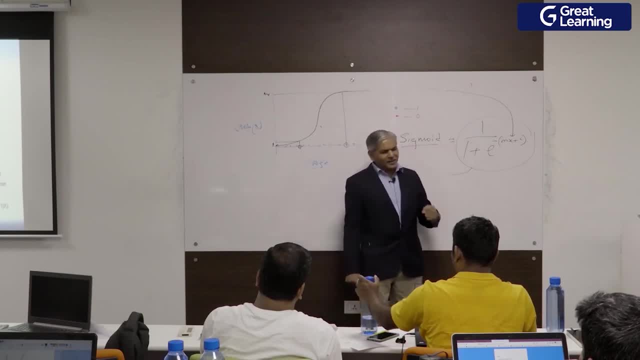 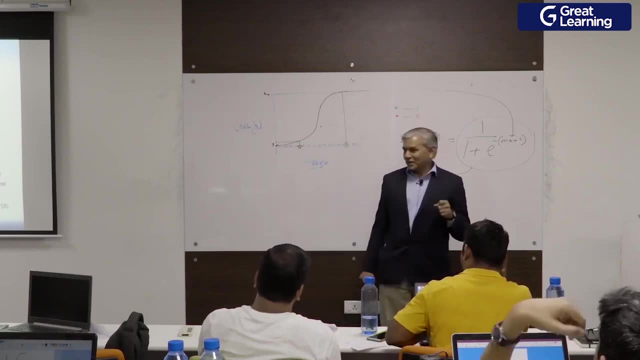 doubtful, but are able to ask. they are not asking. I know I can identify such people, So feel free to ask. ok, all of you, please feel free to ask. don't get left behind. I was always a backbencher. I was always a member of the backbench society. I am not. 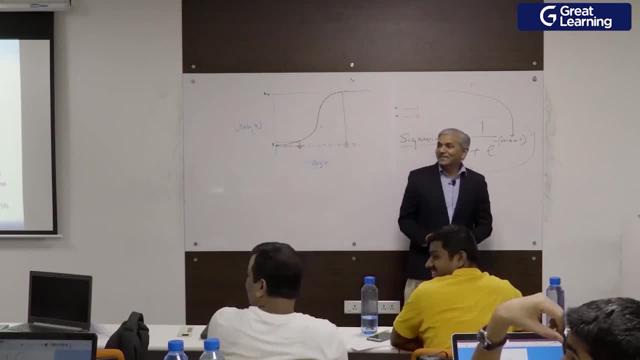 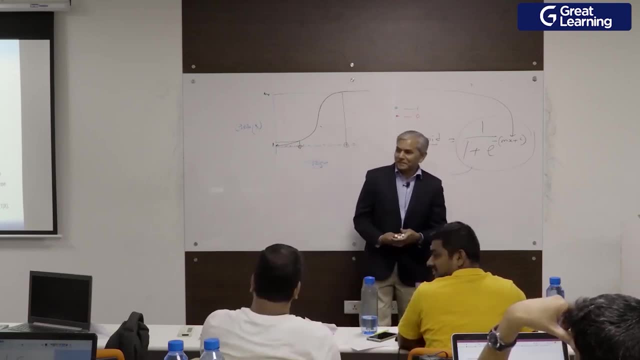 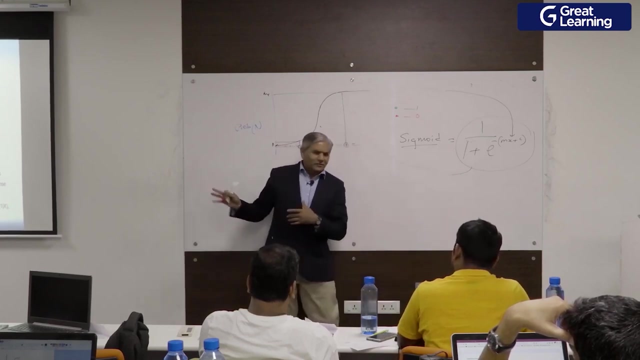 saying anything to you. don't look at me. If you sit in all places means I was always a backbencher, so I know more over the backbench than the frontbench. but other patterns which I observed was during During the sessions. right, so deviation from our main topic of discussion, bottom line. 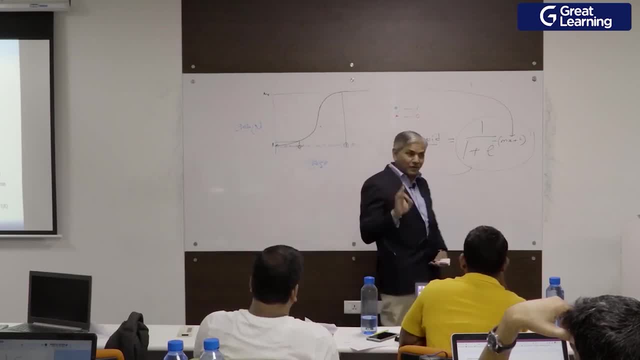 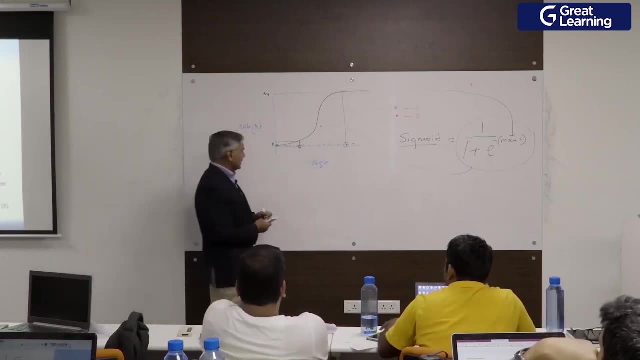 is: don't hesitate to ask. ok, feel free to ask, don't hesitate. Coming back to this, are you all with me on these two discussions? Ok, now look at this point. you see a red point here, this one. what the model is saying is: as per his income, he belongs to probability. 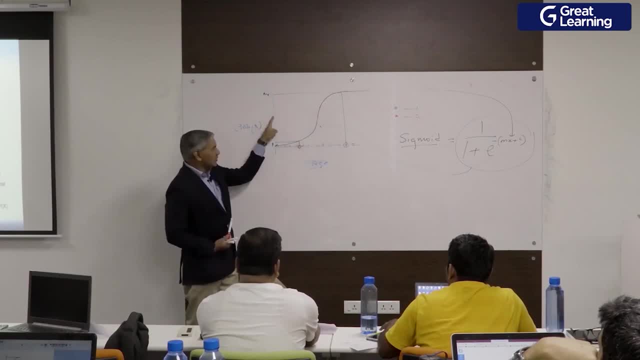 of he belonging to blue class. Blue class is very high, So the model will pass him as blue- sorry, in this case green. green in this case green. So what the model surface is telling you is predicting the probability of belonging to the green class. 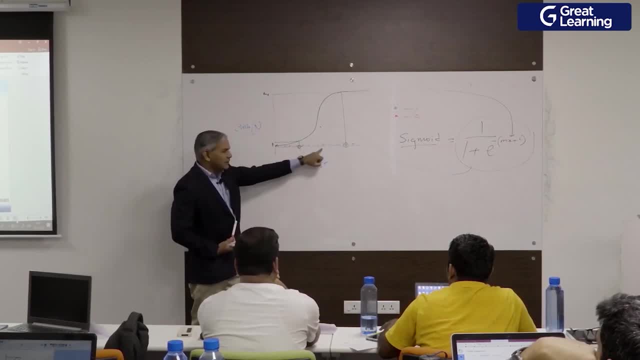 It is very high. So the model will classify him as green, but he is actually red. So model has done an error over here. mistake. Similarly, if you look at this one, this side, the green point here, can you tell me why? 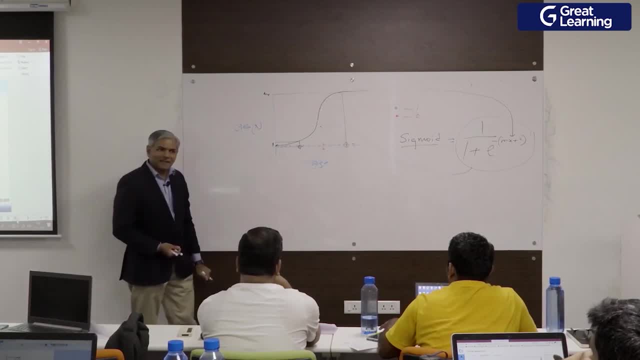 Ok, What the model is telling you. The model is telling you the probability of him belonging to green class is very low, so he is likely to be red, but actually he is green. So the model has done an error here, a mistake, ok. 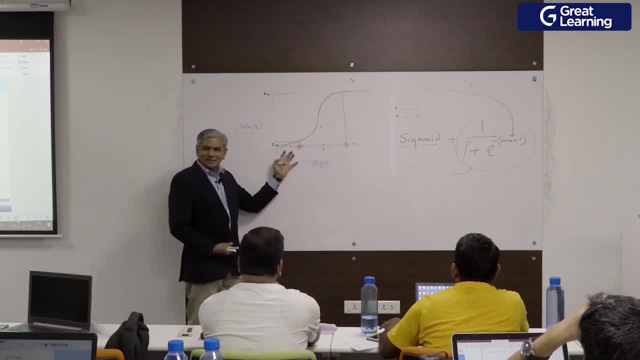 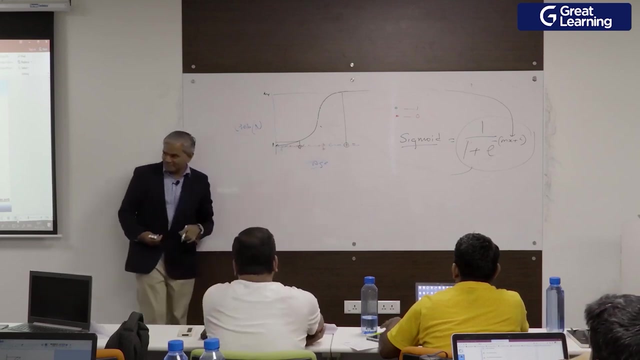 So whenever you have overlapping data sets, as in this case, in spite of the best fit line, Ok, In the classification you will find some errors. They will always be errors. These errors are called training errors- Errors in the training data. 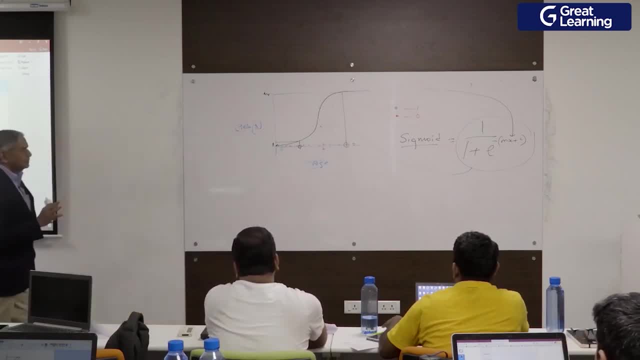 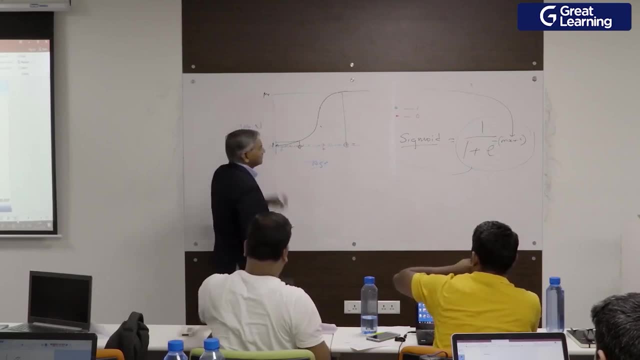 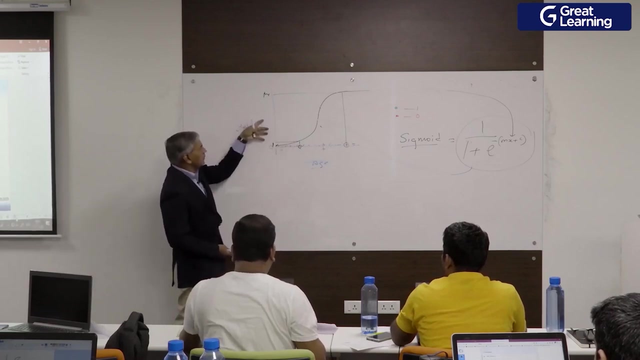 Ok, Alright, No problem. Which one is minus 1?? This is 0,. this is 0,. this is 1.. And this axis in this particular picture, this axis is probability of belonging to class 1.. Ok, That is why your S-curve is coming like this: 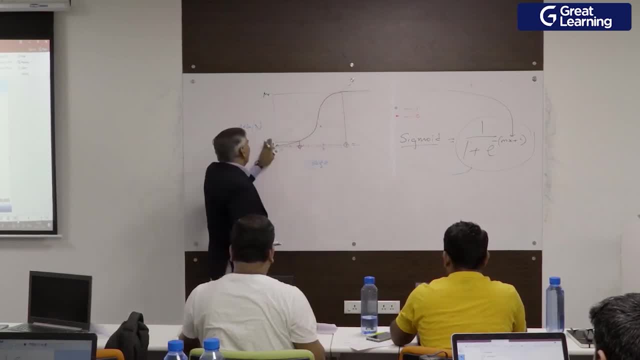 This S-curve has been built out of a linear model. If you had taken this- sorry, if you had taken this as probability of belonging to class 0, then it would be reverse S-curve, Because your curve would be like this. the line would be like that: 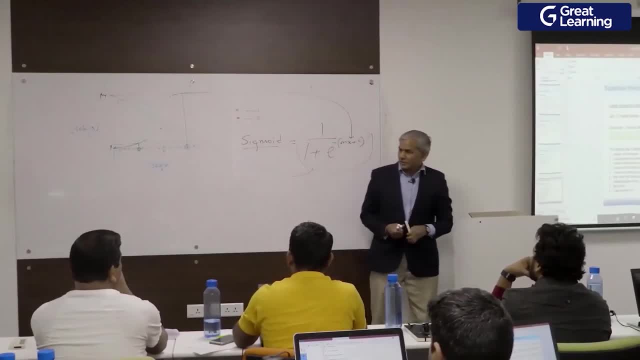 Oh yeah, all models have problem with outliers. Sir, can you explain what is the problem with outliers? Sir, can you explain what is the problem with outliers? Ok, What is the reason you have taken S-curve rather than the linear model? 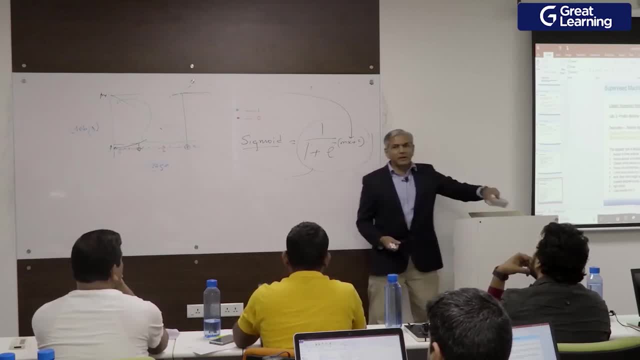 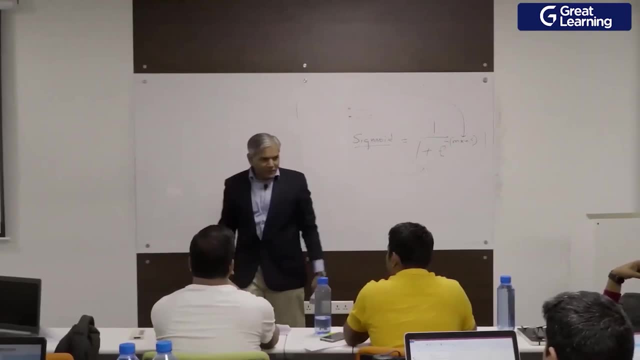 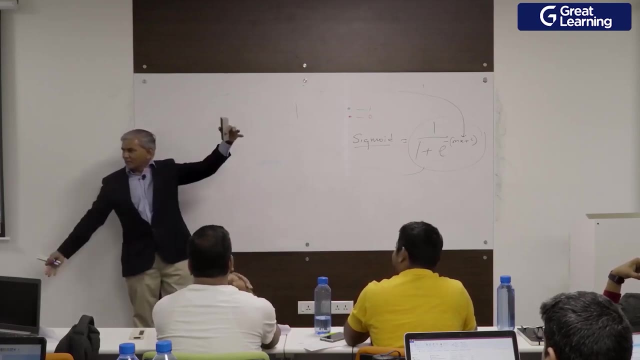 Can somebody answer that question? Why S-curve? Because the linear model is going to be. it will go to plus infinity. It will go to plus infinity. Linear will be over fit. Who said that? What did they say? In linear models, we do not have any boundary. 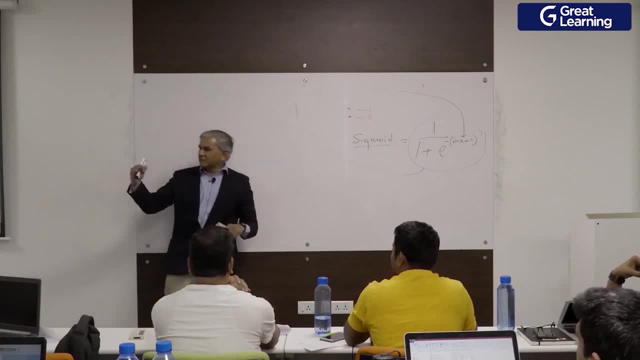 They go to plus infinity, minus infinity. We do not want that. Probabilities have to be between 0 and 1.. That is why they will convert into sigmoid. Sigmoid curve has that property that will always remain between 0 and 1.. 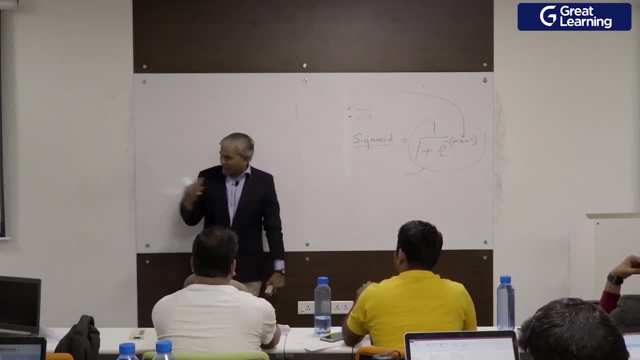 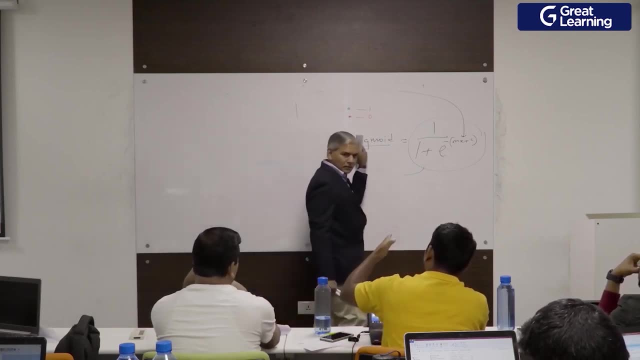 So we are able to map the numerical values to probability function. So, coming back to the same question, now you are explaining the binary, So same thing is applicable for the multi-class classification. Yes, In multi-class classification it will be 1 versus rest. 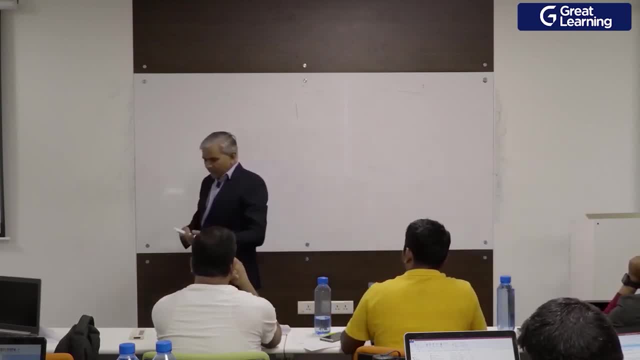 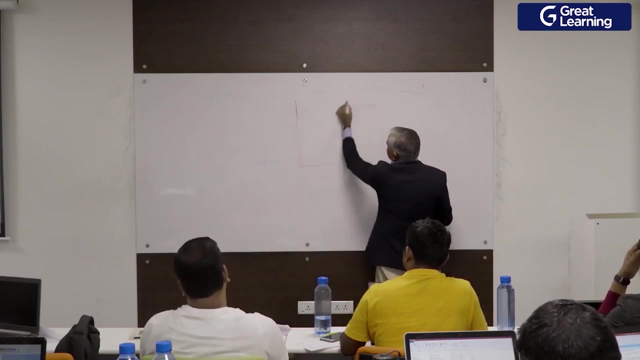 Suppose I used sigma, this logistic regression, for OCR, optical character recognition. So you will have one S-curve for A versus others, One S-curve for B versus others, So on and so forth. So in your mathematical space you will have multiple S-curves cutting each other. 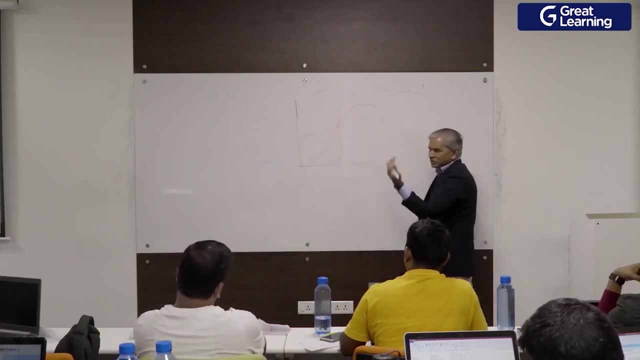 One is for A versus others, the other one is B versus others, C versus others, so on and so forth. All these algorithms, decision tree, Naive Bayes, support vector machines, neural networks, logistic, they all break your mathematical space into compartments. 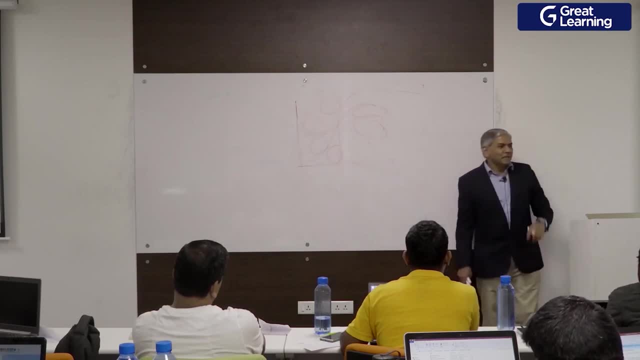 They break them into compartments pockets. Where one pocket belongs to this object, the other pocket belongs to that object. All of them do that. You have done. decision tree yesterday. Yes, Which data set did you use? Diabetes Pima diabetes data set. 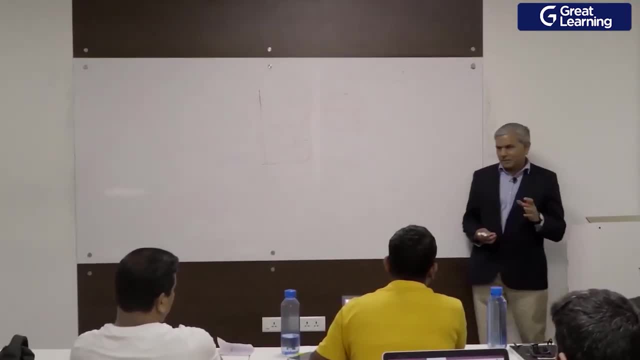 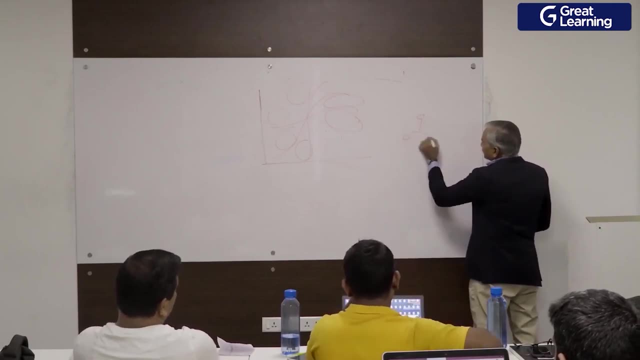 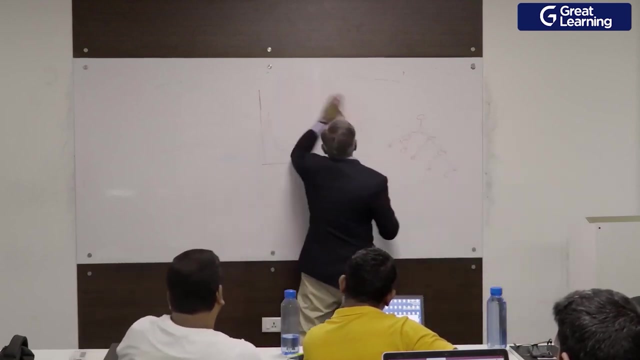 Diabetes: Pima diabetes data set: Okay, That is a binary classification actually. So when you make decision trees, okay, this is the structure you have of decision trees. What you are doing here is This entire mathematical space is your root node. 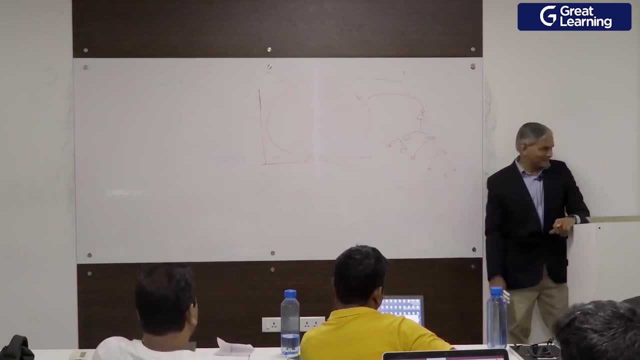 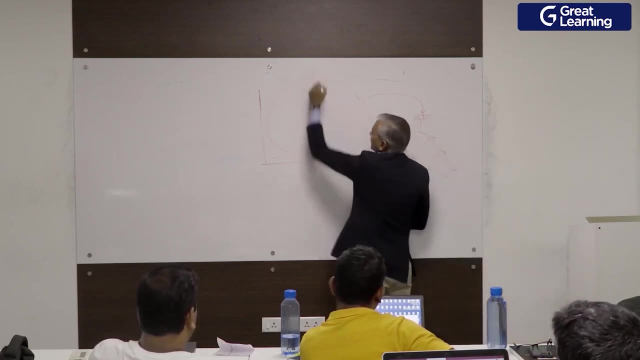 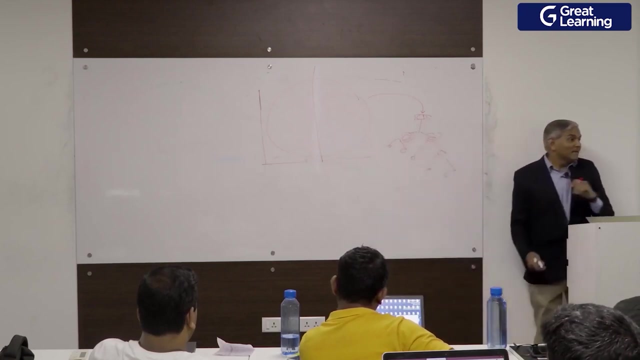 The entire data set, all data points put together, is your root node. Then you find out one particular column on which you break the data into two. That is like putting a vertical boundary here. So these two now are these child nodes, But you have not achieved your what you call homogeneity. 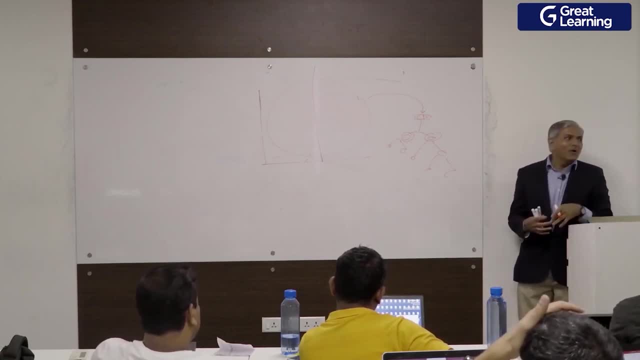 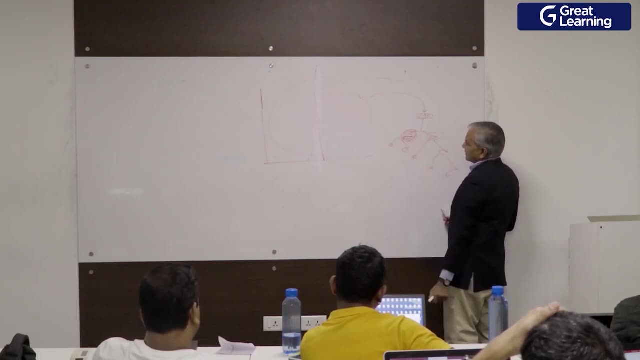 Your, your Gini index. Okay, Your Gini index is still very high, Or entropy is very high, It is still not pure leaf. So what you do is you again find a column here in this data set and break this into. 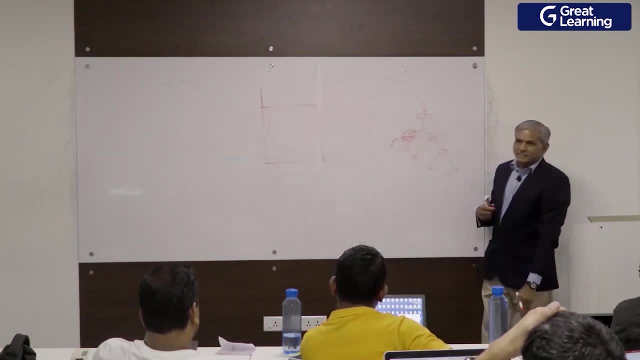 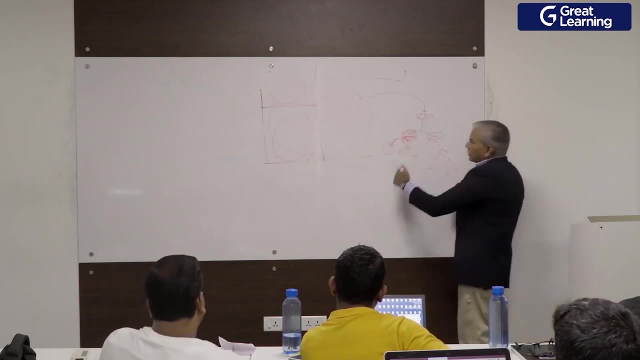 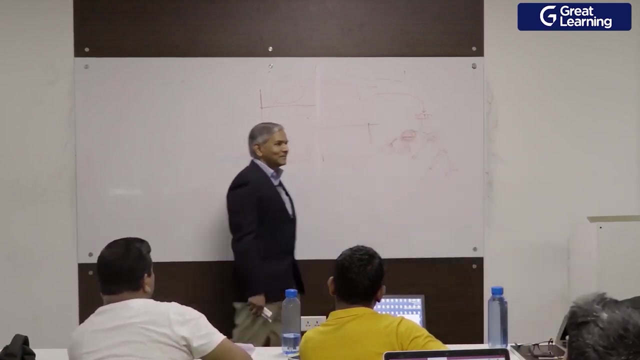 two. That means you are drawing a vertical boundary. So this and this is a child node here and here. So decision tree also breaks your mathematical space into pockets, such that each pocket becomes homogeneous at leaf level. So right now I have reached the leaf level. 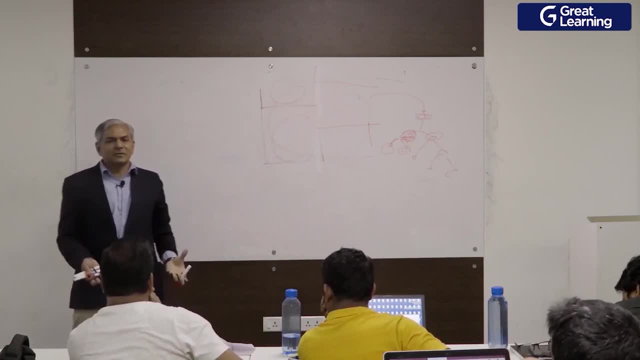 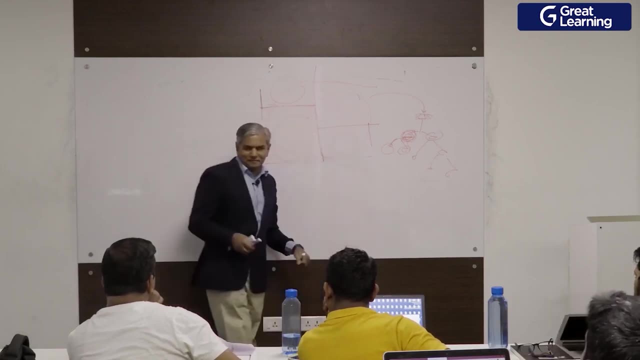 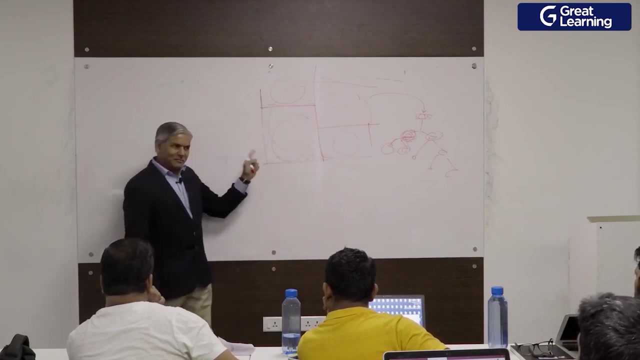 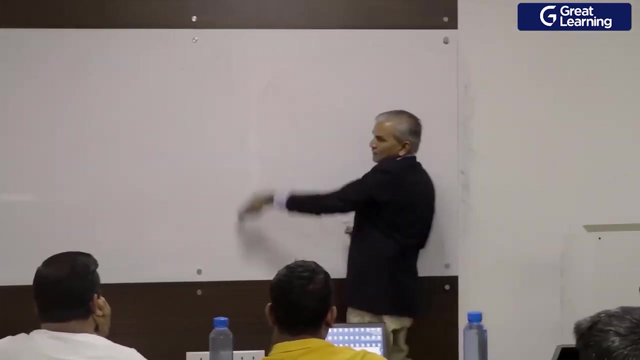 Hopefully, at leaf level each pocket has become homogeneous. Now I know what are the conditions under which somebody belongs to this pocket. That is called the rules of the decision tree. All algorithms break your mathematical space into pockets, including logistic regression. You treat A as class 1.. 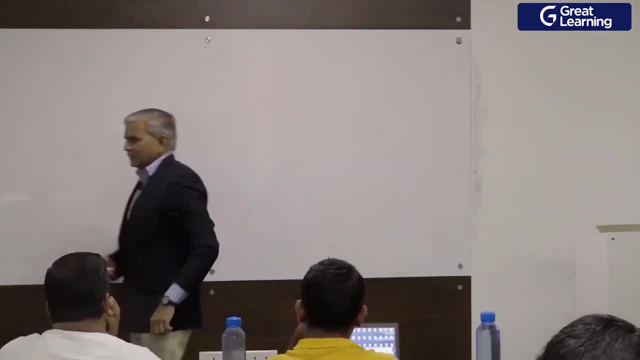 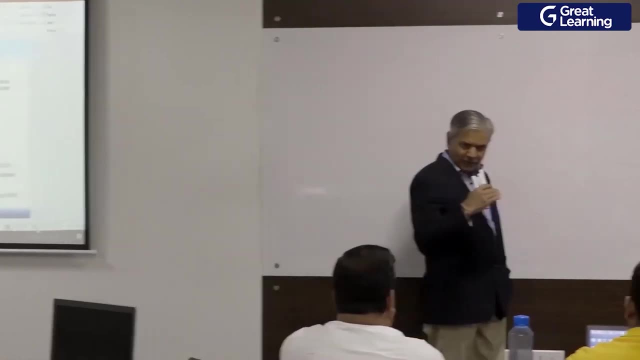 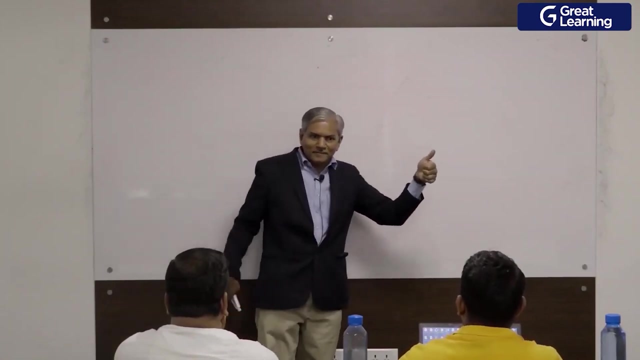 Why class 1?? Why class 2?? So binary class classification. if you are in multi-class classification- optical character recognition- then you treat at one point in time A. all data belong to class A, alphabet A as 1 and rest of them are 0s. see what is the boundary. 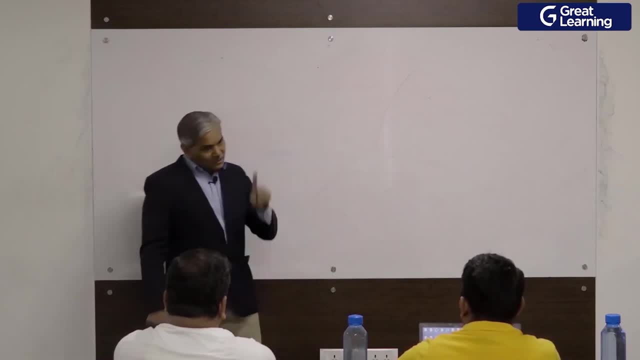 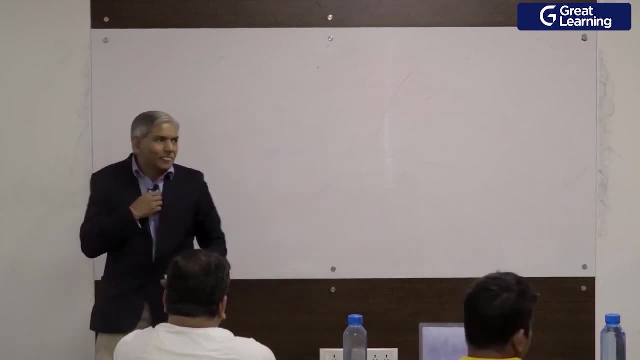 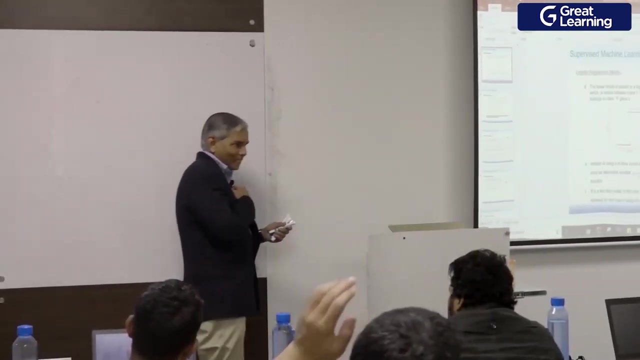 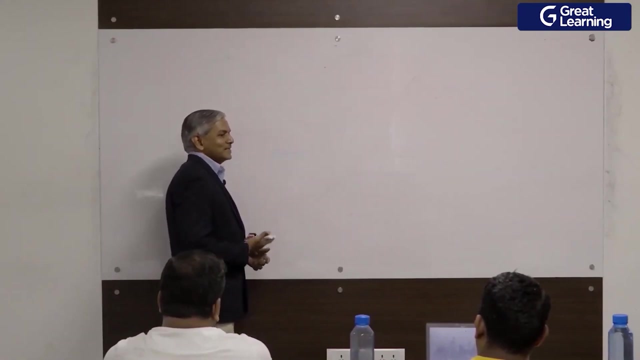 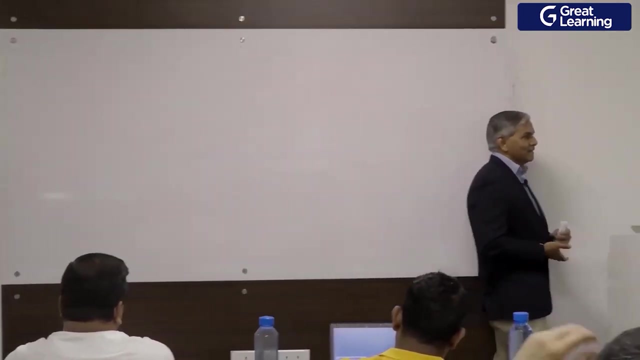 Then treat all the records belonging to class B as 1 and rest of them 0s, then read out the boundary, So you will have multiple boundaries cutting each other. yeah, that will be hypersurface, but multiple hypersurfaces for A, for B, for C, right, yes, 100 percent. yes, the whole. 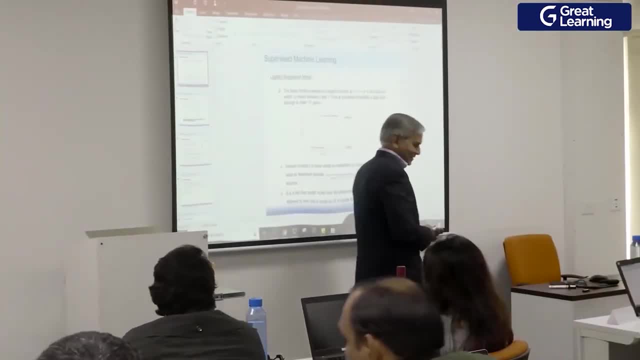 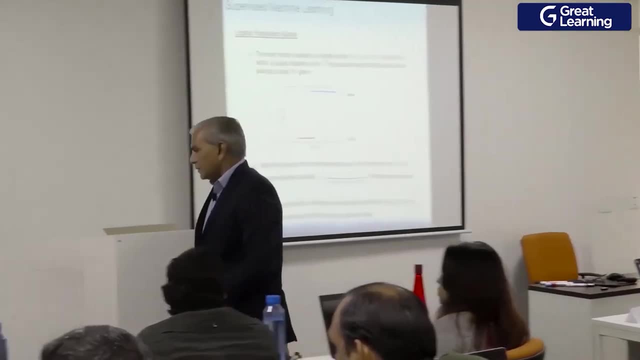 model will be composite of all that. All these surfaces. ok, Let us move on. So multi-class is always 1 versus rest. Multi-class classification: most of the algorithms give you OVR. OVR means 1 versus rest. 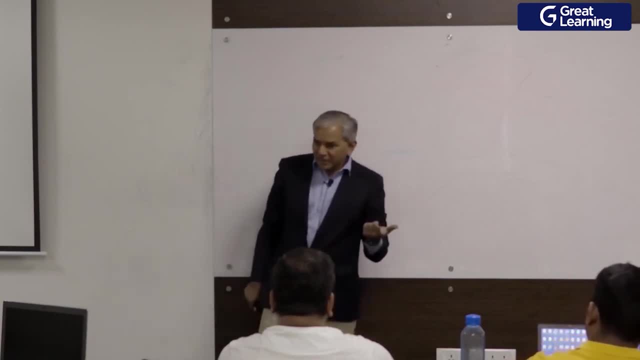 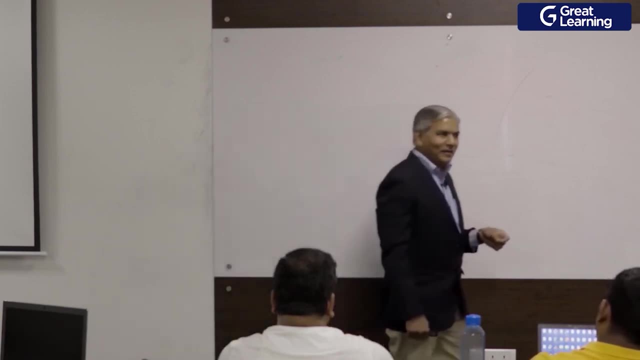 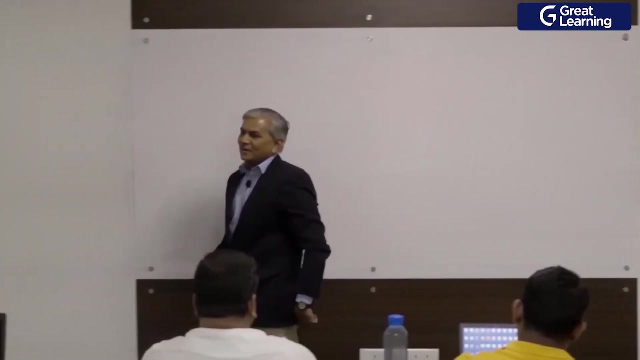 Some algorithms give you a facility of replacing the OVR with Bayesian probabilities. ok, You can actually go and modify that in your hyper parameters, But most of the algorithm by default will give you OVR right. Some algorithms like support victim machines. OVR is not very efficient, so they give you. 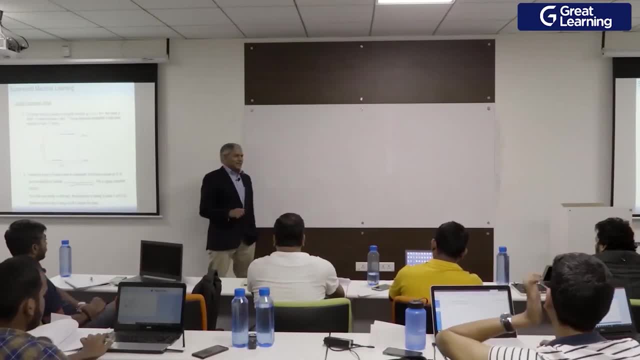 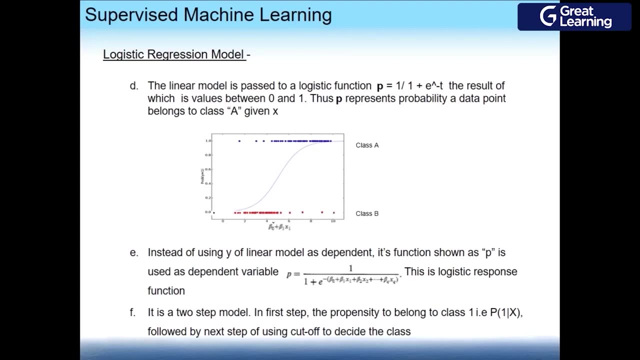 another technique called Bayesian probability based, Shall move on. ok, It has a gradient descent algorithm, one working under the hood to find out the best fit line right. The linear model uses gradient descent algorithm. do you remember gradient descent discussion we had yesterday? 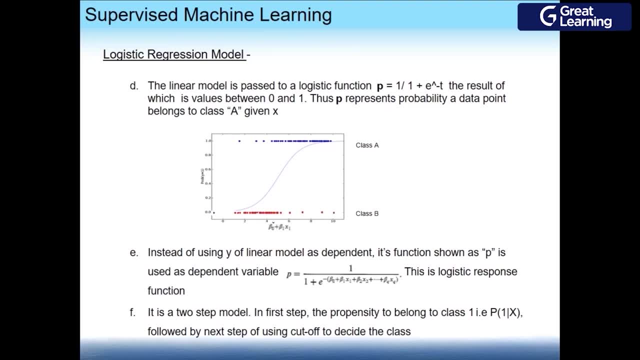 See the gradient. descent is to find best fit line. I will quit. I will quickly summarize this. I know it was too much in one day to cover Your error. function will always have this form. not very difficult, guys. If I give you equation y equal to x square, for any value of x, y will always be positive. 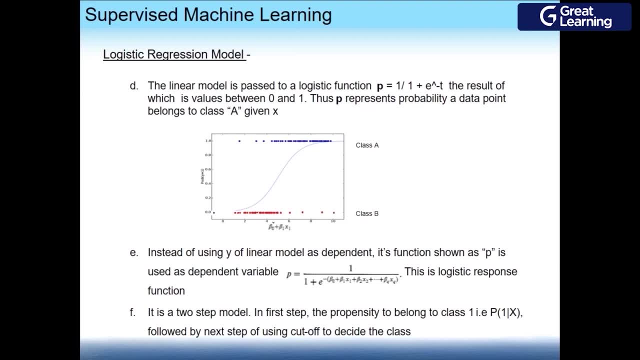 It is a squared term. If x is minus 1, minus 1 into minus 1 becomes plus 1.. This is called the convex function. So whenever you have any function raised to power 2, it will always be convex. Right now, this is single dimension. 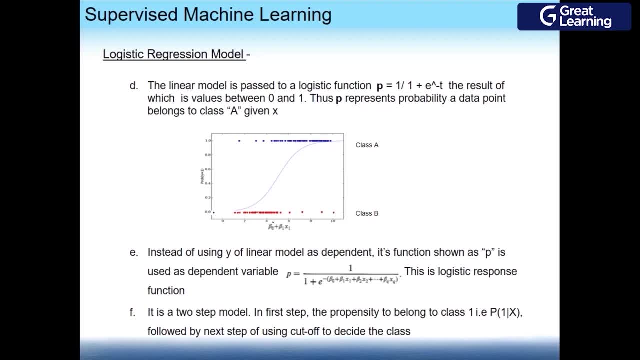 This x can be multiple dimensions. So if I take two dimensions, m and c, and plot the error, this will be a bowl shape. right Now, in this bowl shape, we have reached the global minima. It is guaranteed you will have only one global minima. 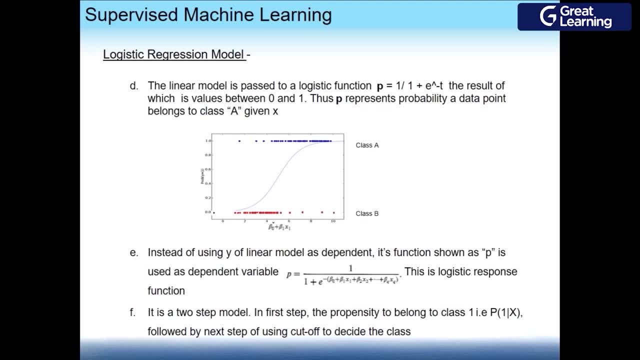 You will not have any other. For quadratic error expressions, you will always have one global minima guaranteed. ok, So we start with some random m and c. That random m and c gives us some error. The same concept applies in logistic, because logistic is also linear model, right? 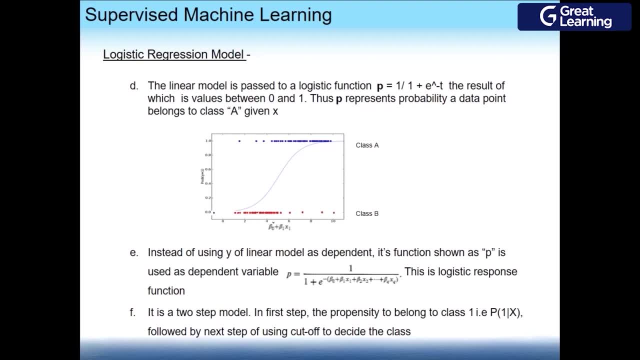 From that m and c. it will come down to this, using your partial derivatives concept. ok, There is lot to discuss in this. I am not going to discuss all these things at this point, but you will need this if you are going to do deep learning. 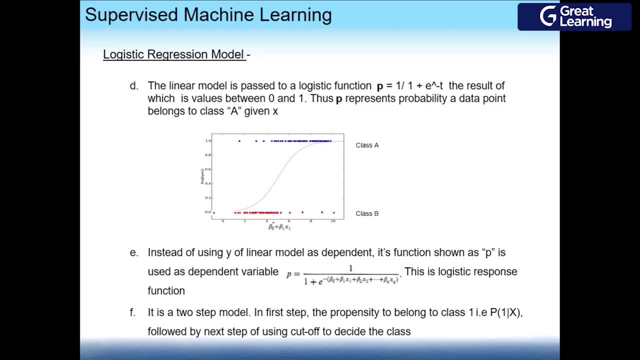 Neural networks and all these things right. At that time we will take it up in detail. Same concept will apply today in logistic, because logistic uses linear model under the hood, So it finds for you the best fit line, given the spread of the data points in mathematic. 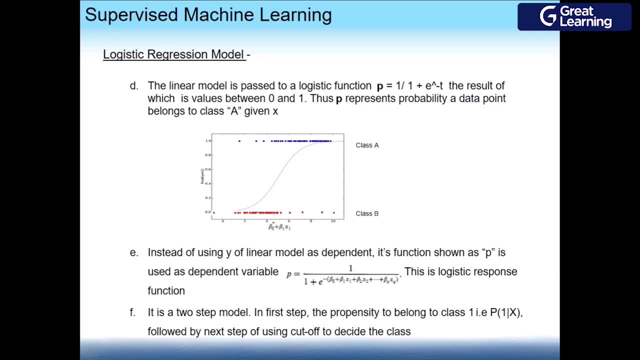 space, or best fit plane, or a hyperplane. Once that plane is found, that plane is sent through the sigmoid transformation and it is converted to S curve. Right Now, the driving force behind this here, in this case it was quadratic. In this case, the S curve which is formed. the S curve can be shifted forward, backward. 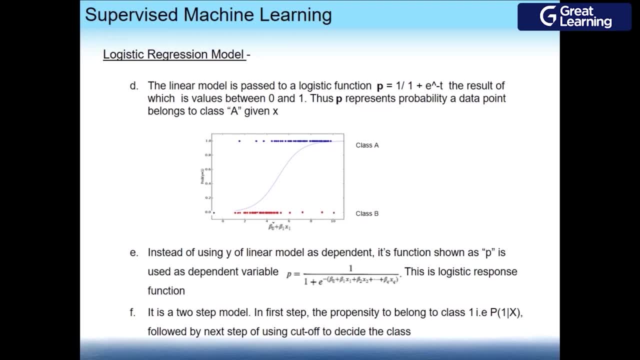 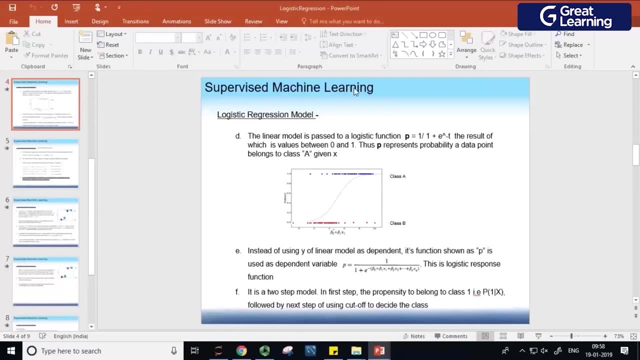 upward, downwards. Let me see if I can show this to you. ok, What happens is insert, Insert, Insert. If I take this S curve, I hope it works. It works. Ok, Now this S curve. you can move it up by changing the c in y, equal to mx plus c, or you can move. 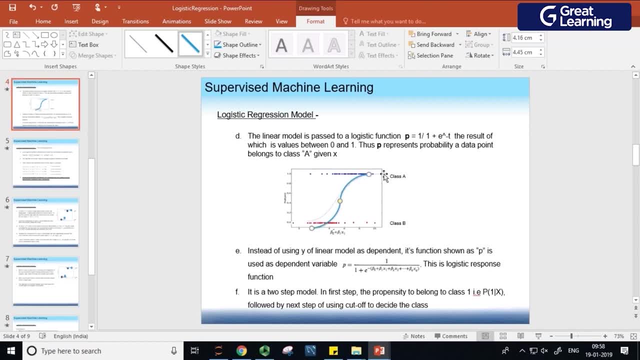 it down. You can flatten it. To flatten it, what do you think we will use? The slope m m of the line By changing the slope m m of the line. By changing the slope m m of the line. 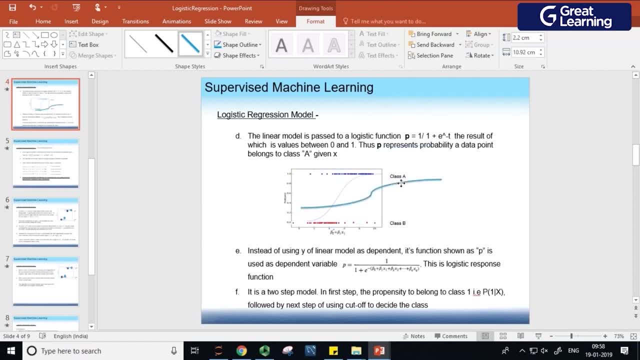 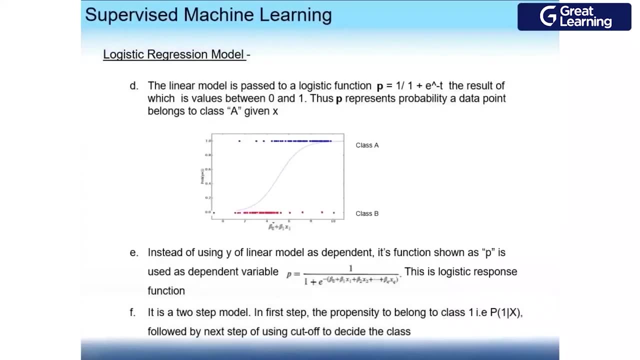 Ok. Ok, By changing the slope I can make it vertical or flatten or move it up and down using c. So by using these two parameters, m and c, I will find out which sigmoid surface I get is the best surface. And to find out which is the best sigmoid surface of all the infinite possibilities. 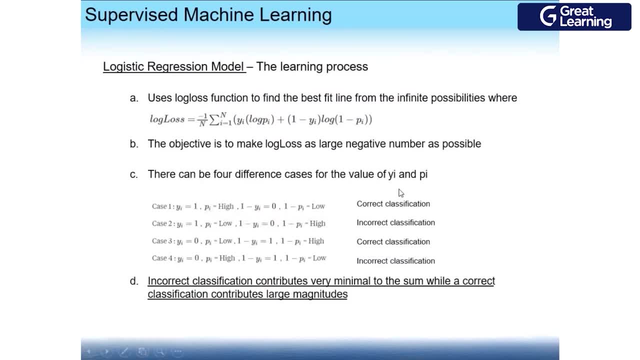 it uses a function. That function is called log loss. This is just like a graph, Ok. Ok, Just like a gradient descent. Ok, Do not worry about this function, It is actually very easy. It looks dangerous, but actually it is very easy. 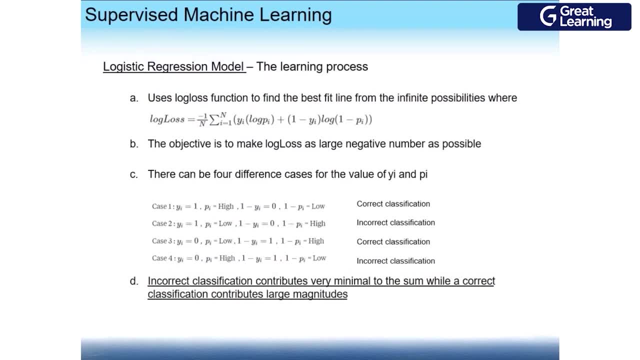 Now let us look at the log loss function. Looks very dangerous, but it is actually simple, very simple, Ok, So forget the sigma and all these things. Just take the expression yi into log of pi. ok, plus, then 1, minus yi into log of pi. 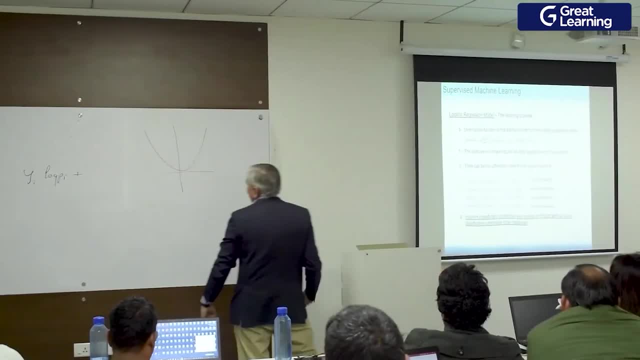 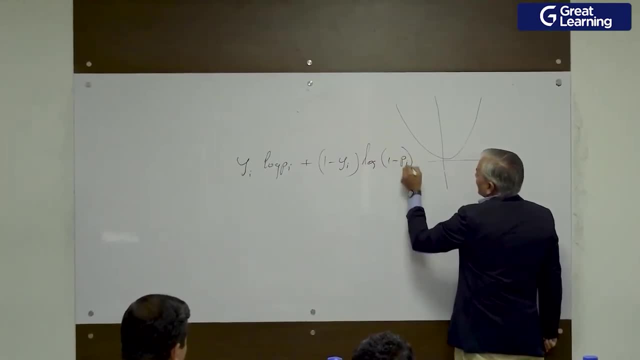 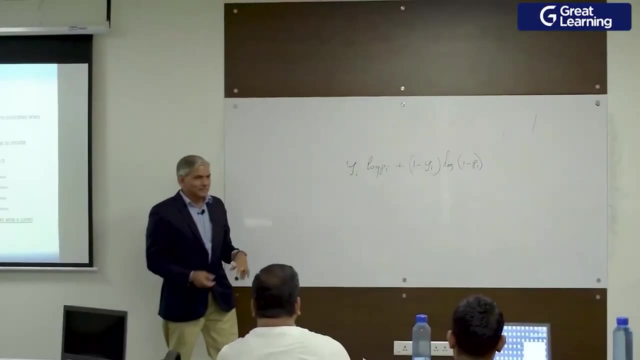 Ok, Ok, Ok, Ok, Ok, Ok, Ok. 1 minus yi into log of 1 minus pi, correct? Just look at this expression. What is this? y? Y is the target variable. Target variable. We know the target variable ranges from 0 and 1 only. 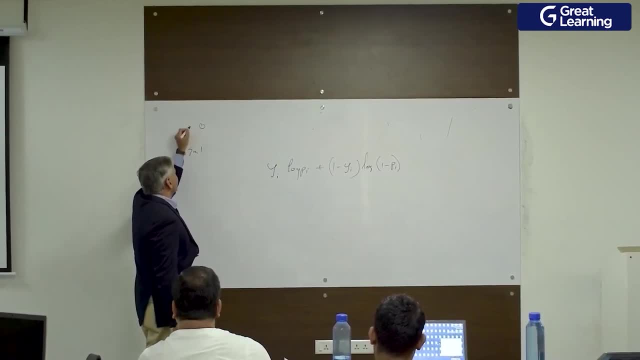 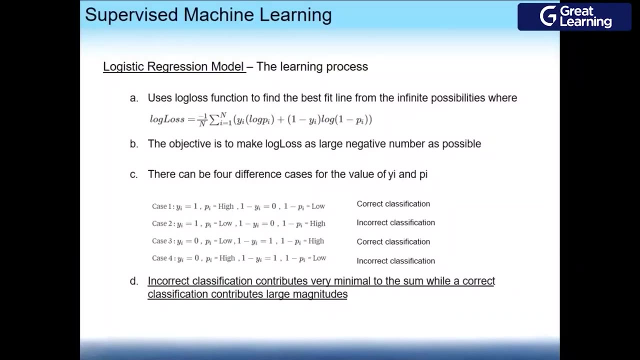 1 is for green and 0 is for red, So this yi can take value of 0 or 1.. Ok, Now let us look at four situations. I am going to show you four cases and the four cases we are going to discuss here. 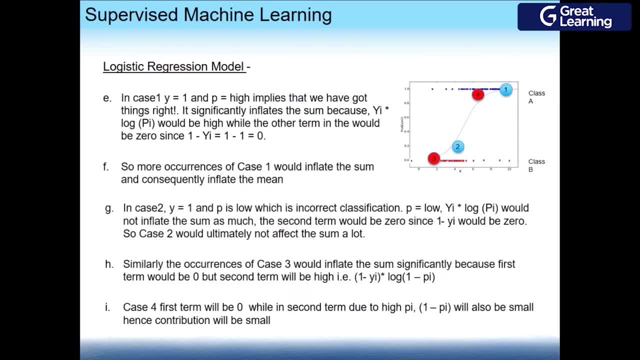 Where is the four cases? Where are these? are the four cases? Look at the first case In your data, the first test case. these are four test records. ok, The first test record has this income. The model is saying that probability belongs to blue class, is very high and is actually. 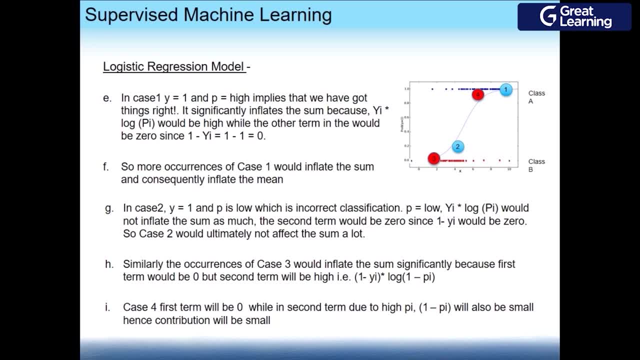 blue class: no error, zero error. right, zero error. Come to this: What is the y value for blue class? One into what is the probability? very high, almost close to one Log of a very high number. when log comes close to one, this is zero. 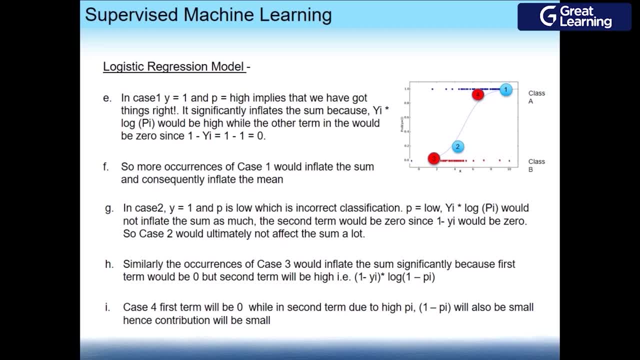 Log of a very high number is zero. Close to zero, Two raised to power zero is one. this is log to the base two. ok, So log to the base two of a very high number. high number means close to one will always. 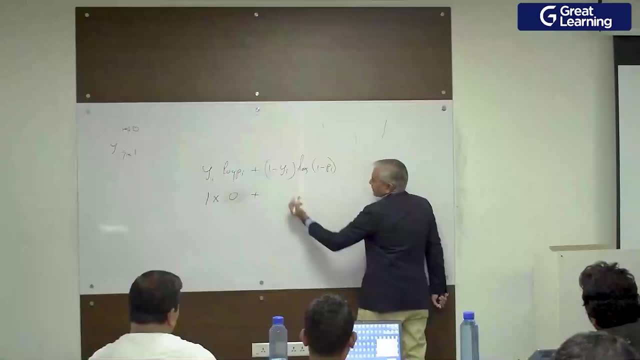 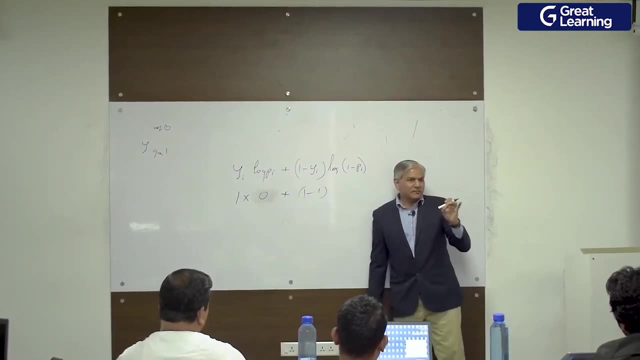 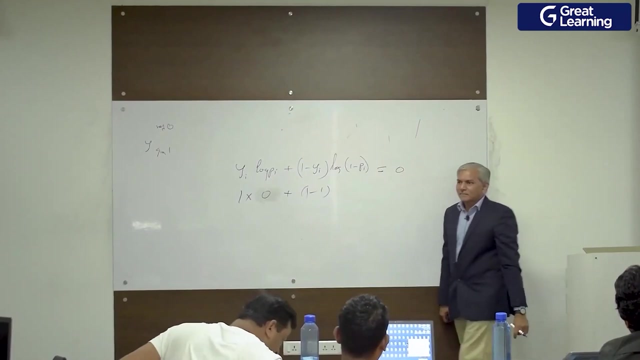 be zero. Come to this term, This becomes one minus one. we do not even need to evaluate, because this is zero. So when you do correct classification for the blue points, Your error is zero. Let's take the next case. The next case is this red point. 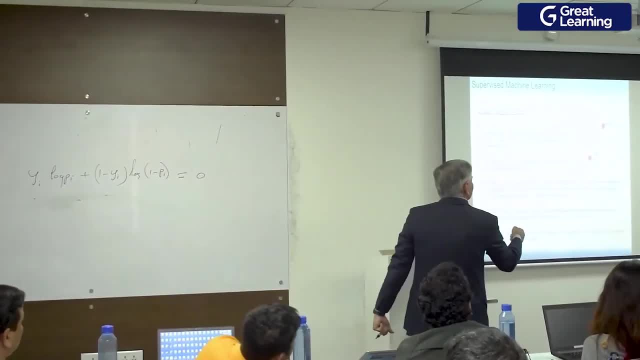 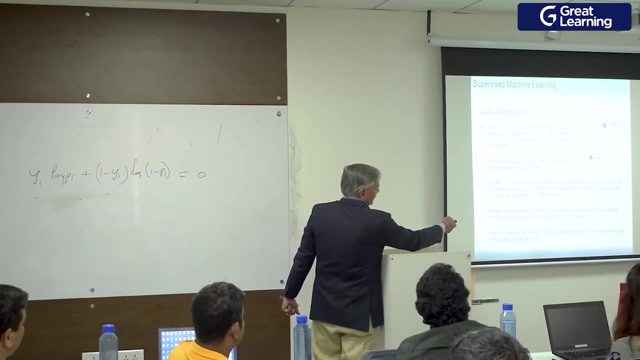 Let's take this red point, Let's take the case number three, or let's take case number two. the second case: ok, As per the model, given his income, this the probability of him belong to blue class is very low, which means model is predicting that he belongs to the red class. 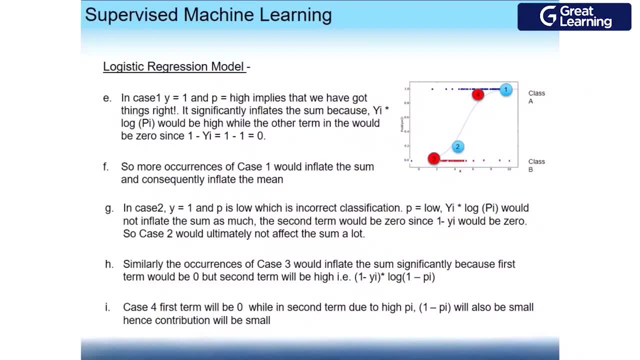 As per the income group of this person. the model. the model is a blue line. it's saying probability of him belonging to blue class is very low. Anything below point five is very low. So the model is predicting that this guy is going to be red. 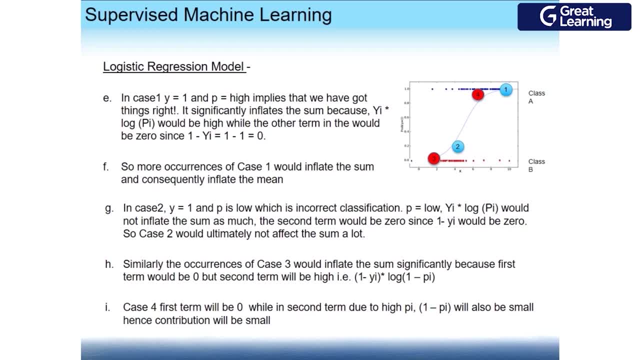 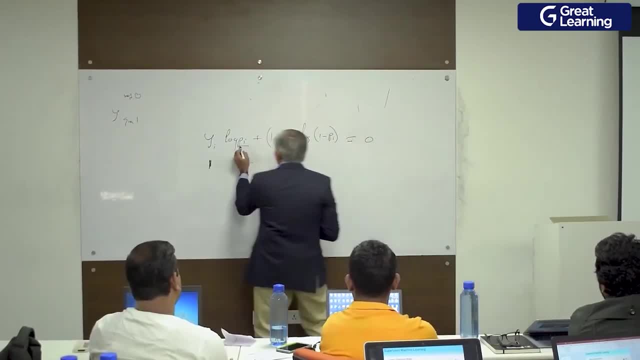 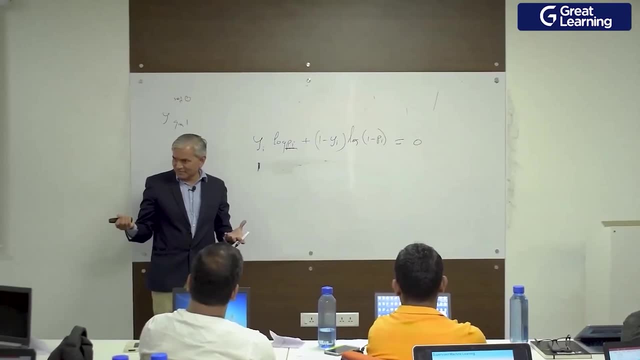 But actually he is blue. So let's see what the equation says. He is blue, value is one, Probability is very low. Probability belongs to blue class. The model is saying: probability is very low. Log of a very small number is a very large number. 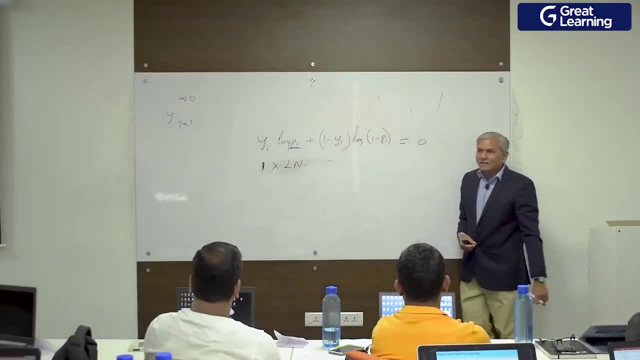 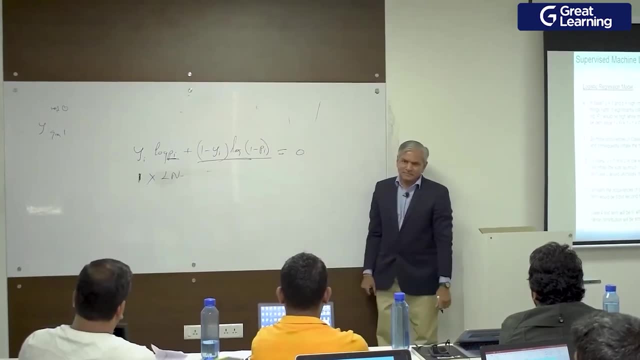 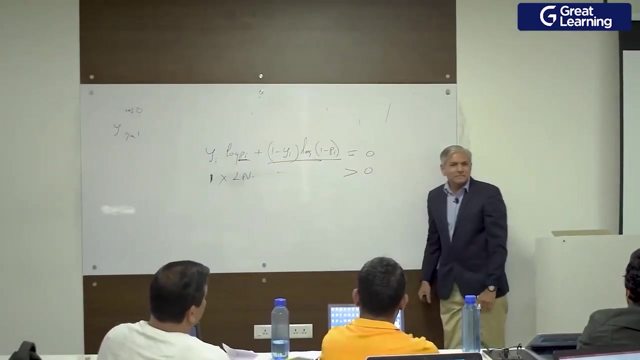 So this is into a large number. ok, Since he is a blue class, this expression we don't even need to evaluate. It will be zero. So whenever you do misclassification of the blue, you get a very large error. alright, 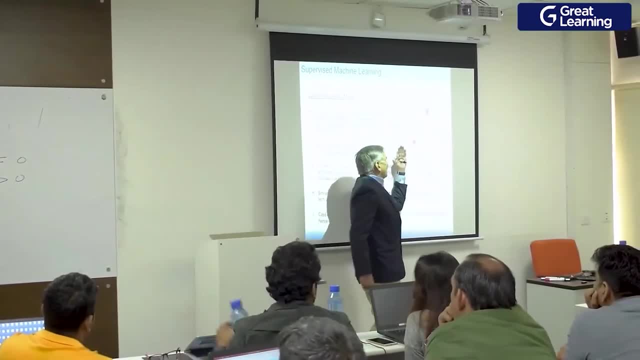 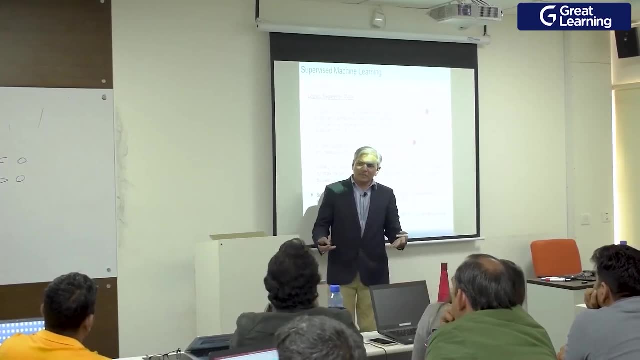 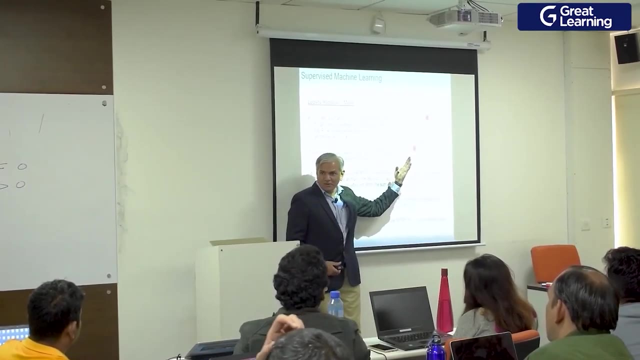 So the more the blue class is on this side, larger the error will become. So in technical parlance what we say is more confident. this algorithm is about a particular classification which we know is wrong. more the error it does Right. 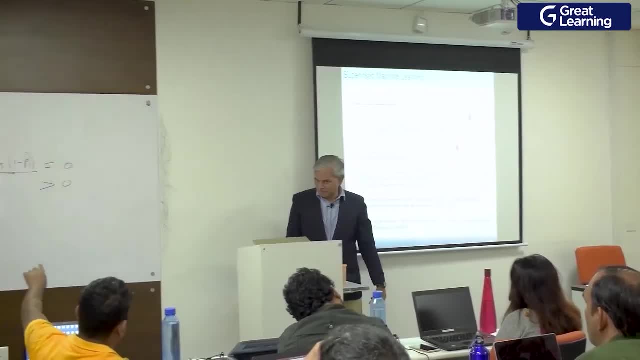 So the probability is less Because you just said t i will be. if it goes lesser, then the larger the error will become Right. So the probability is less Because you just said t i will be. if it goes lesser, then the larger the error will. 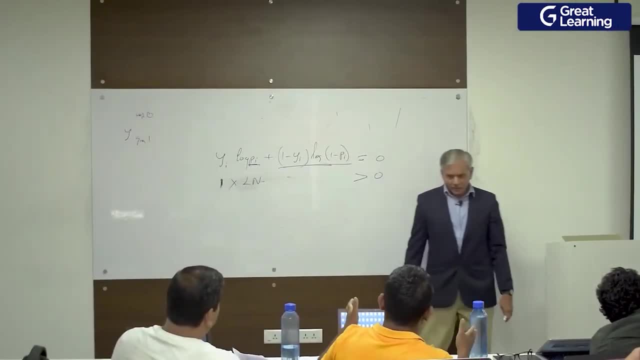 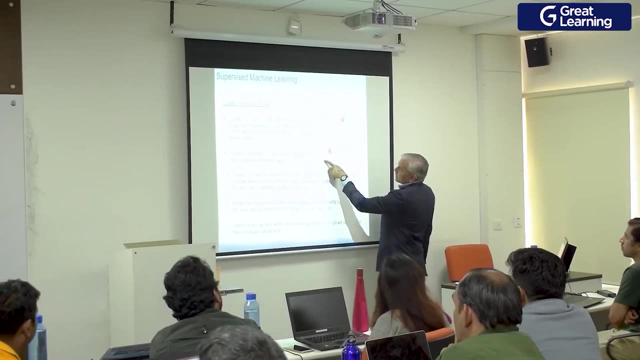 become Right, So the probability is less. The larger the error will become, the more the error will become Yes, correct, The error will go more. If you go down, this is still positive. So for this blue point, where the probability of him belonging to blue class is almost zero, 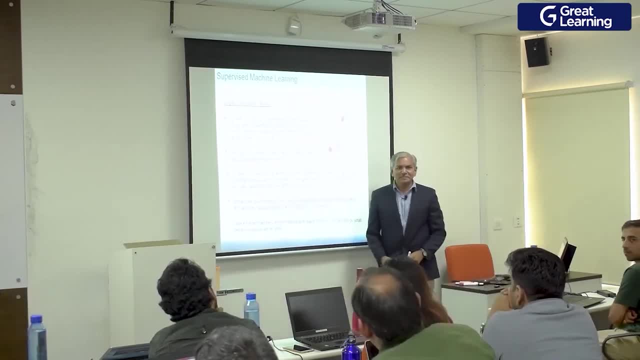 this error will be very high. So what we are saying is: more error we do on this side For blue class. For blue class, then loss is more. Yes, exactly, And upper side, even the error is there, but loss is less. 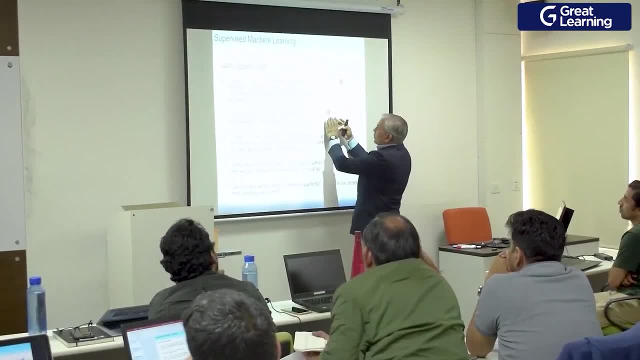 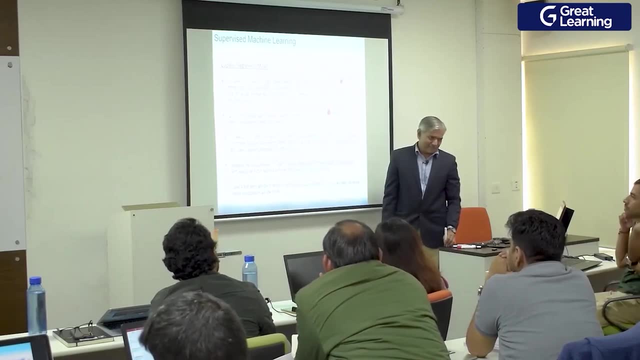 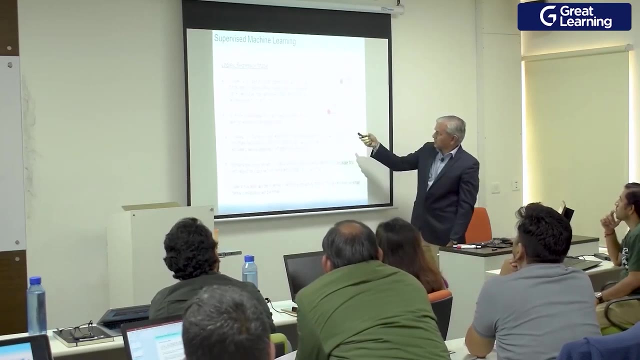 We will come to that. We will first discuss only the blue class. The more blue points are on this side In this case, the more the errors will come out, larger the error will be. Ok. Now look at this: the red one, the fourth one, or let us take the third one, sorry, third. 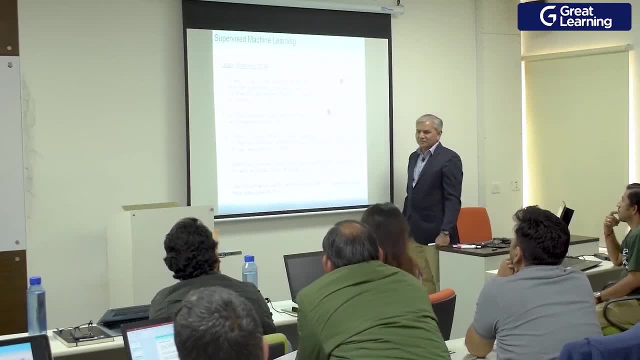 one. We know that this guy is a defaulter. The class is red, The model is given the income. the model is predicting he is going to be defaulter. Come to this equation: What is the label value for this guy? 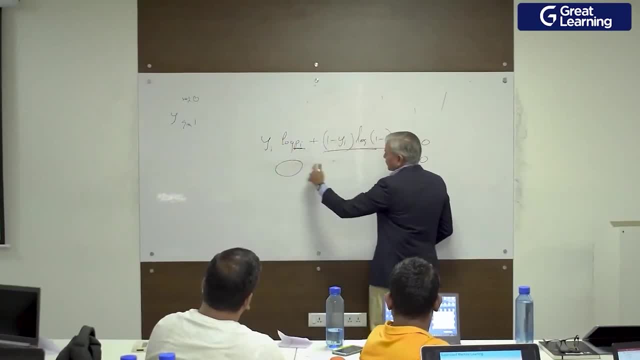 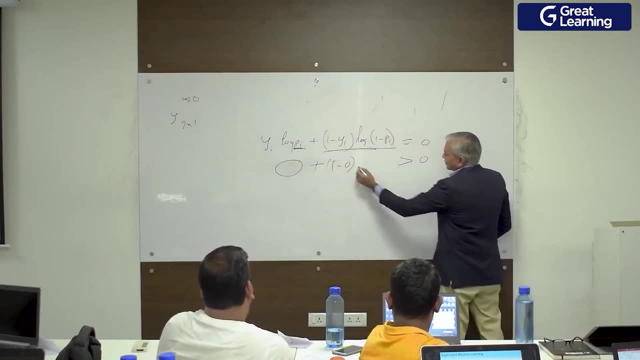 Class red: 0. So this expression becomes 0.. We do not even need to evaluate. Come to this guy: 1 minus 0 is 1 into log of a very small number, Very small number minus 1 becomes almost 1.. 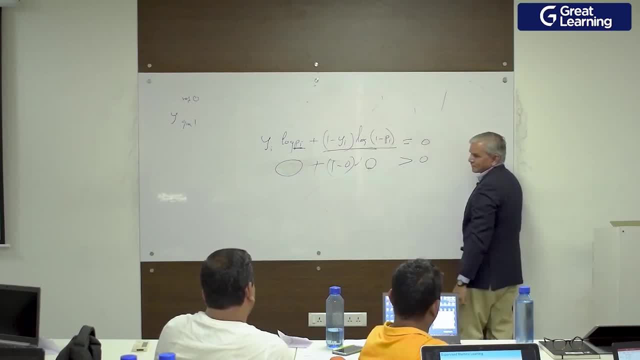 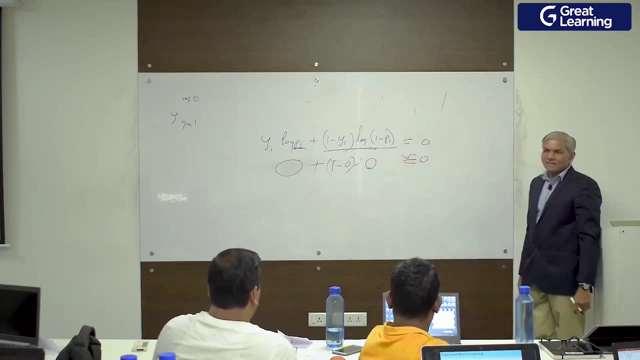 So this expression turns out to be 0.. Log of a very large number. It is 0. So this expression comes too close to 0.. Ok, So this is what we are going to do For red classification: we use this part of the equation. 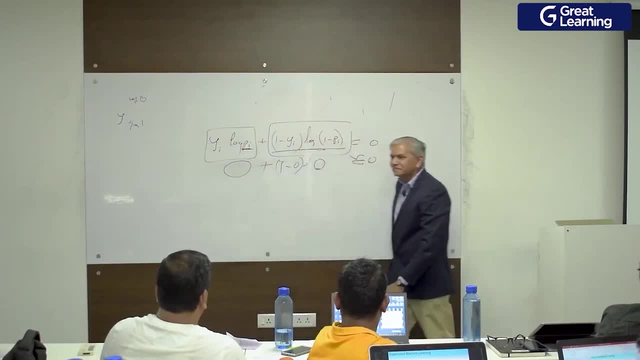 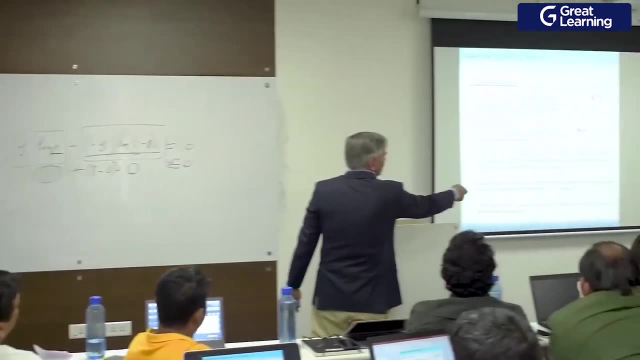 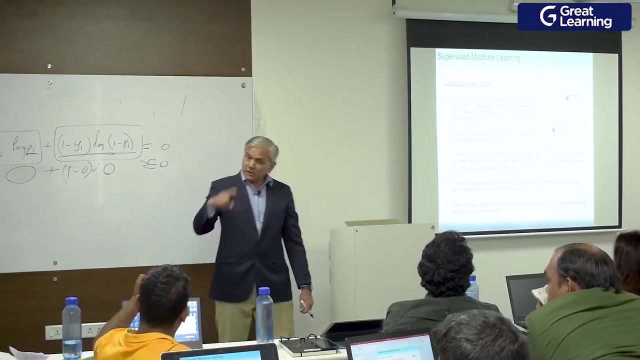 For blue classification. we use this part of the equation. Take the last case where the red class is misclassified. The model is saying he belongs to blue class. One question So here is the probability of belonging to blue class. Belonging to blue class. 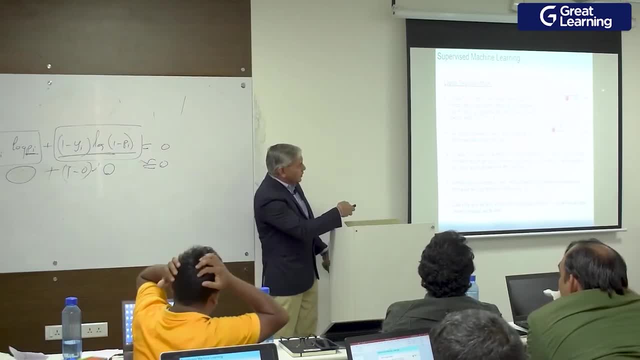 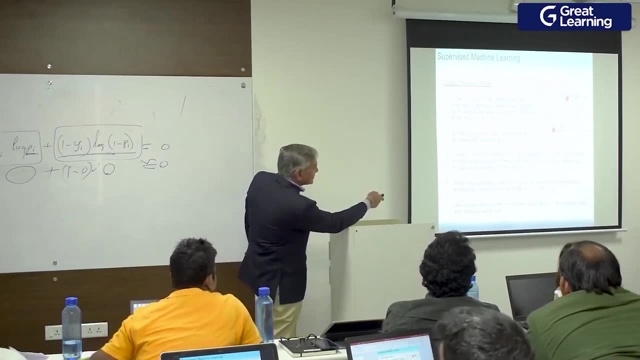 Yeah, See the model. the surface is probability of belonging to blue class. Yes, Belonging to blue class, Ok. That is why it is 0.. Exactly For the red. Exactly, Ok. Look at the last case. 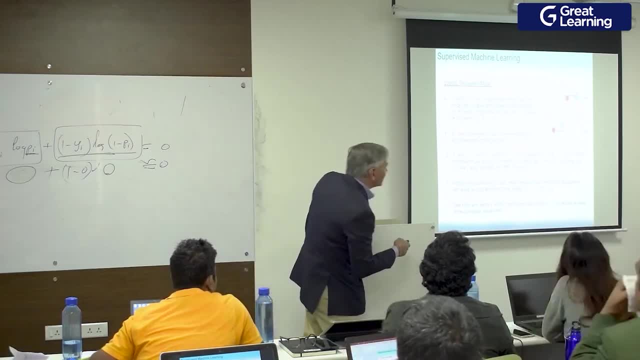 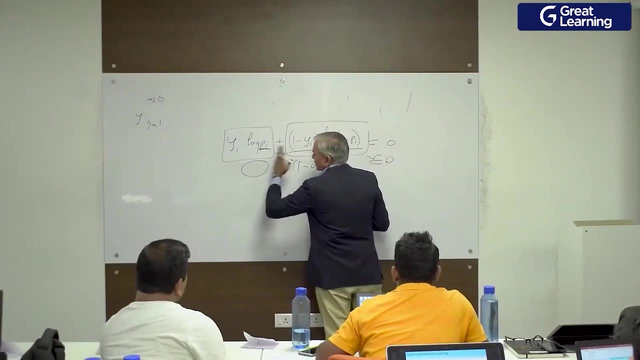 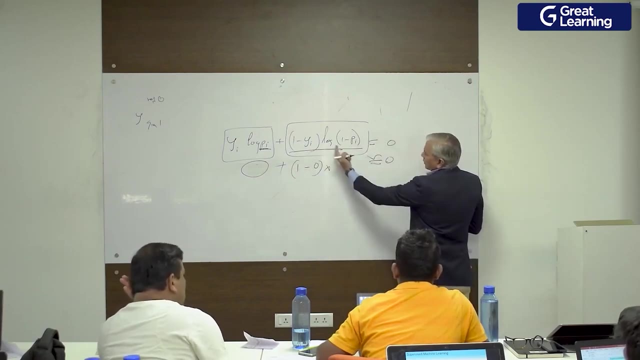 Last case is the fourth case, where the fourth case is misclassification of red. So when you do misclassification of red, this expression is not for red, So forget it. Come to this: This is 1 minus 0 into log to the base 2.. 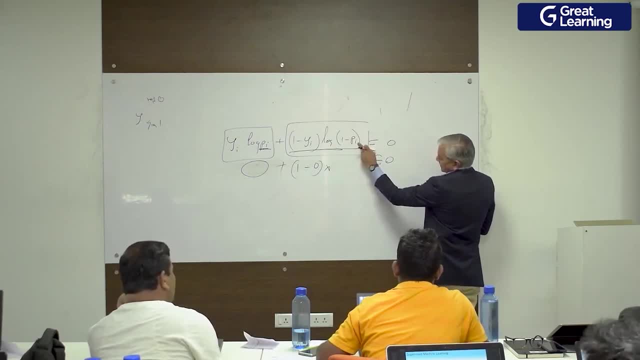 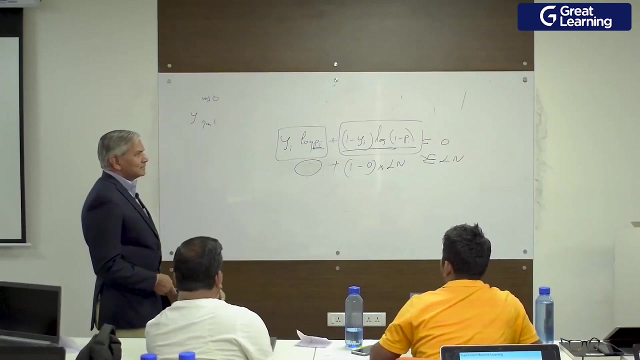 This is a very high probability, which your model is predicting. Ok, So this becomes a very small number. Log of a small number is a very large number, So error is very large. That is all this equation is. So you sum up the errors done across all the data points, those which are correctly classified. 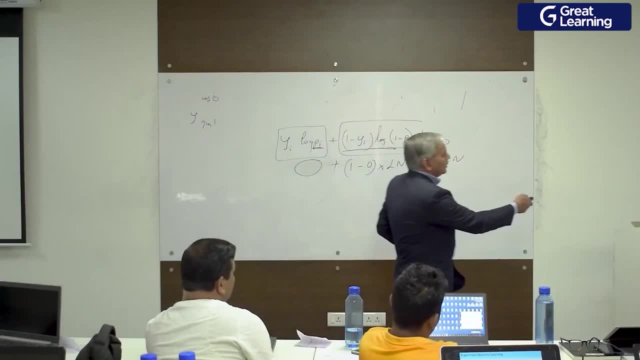 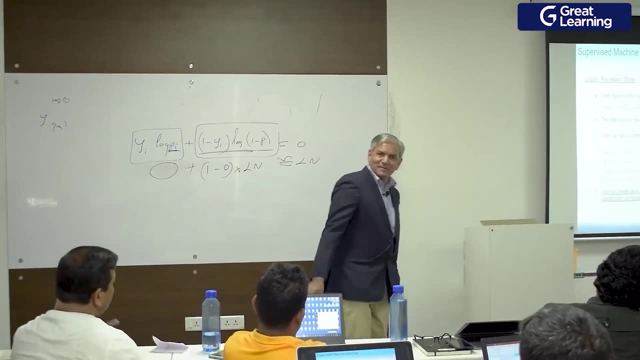 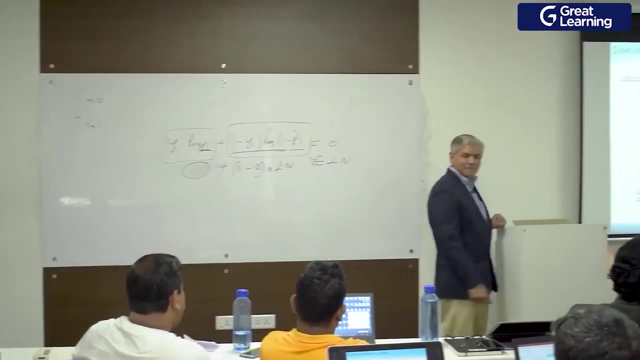 those which are not correctly classified. Sum it up, You will get the total error across the entire model. Sum of squared errors: Same way this. So the objective is to minimize the sum of squared errors by finding the right logistic surface, given the classes. 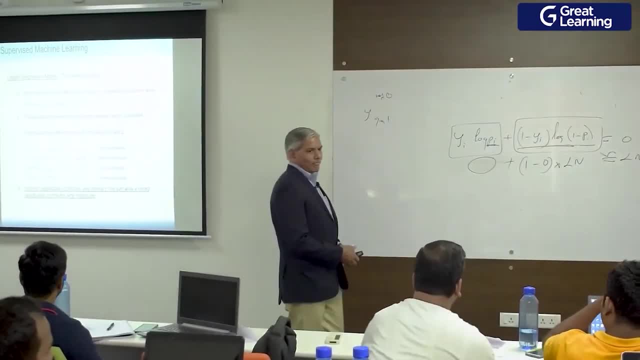 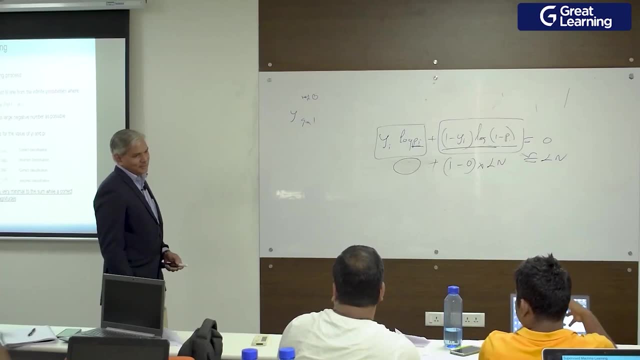 So the gradient descent will be the same. So suppose it is a high loss and it will go in a direction where it wants to reduce the total loss. Correct: Yesterday the sum of squared errors was driving the gradient descent. Here the gradient descent is the gradient descent. 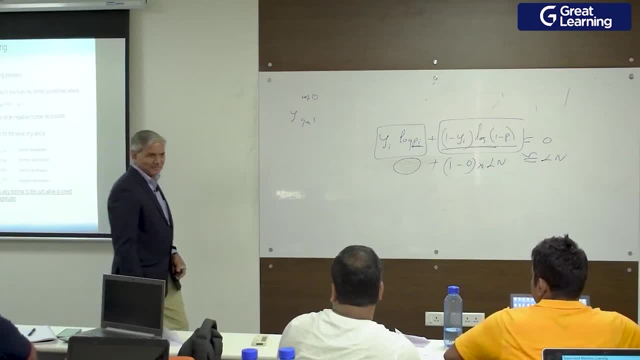 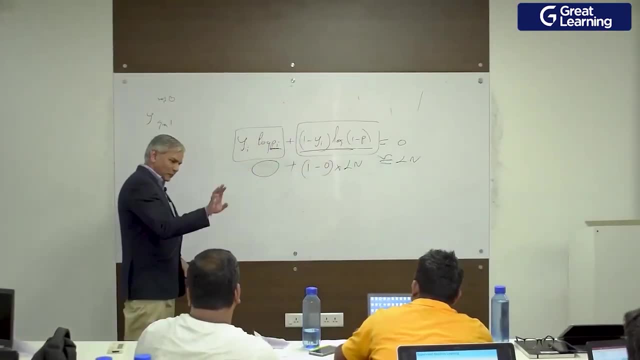 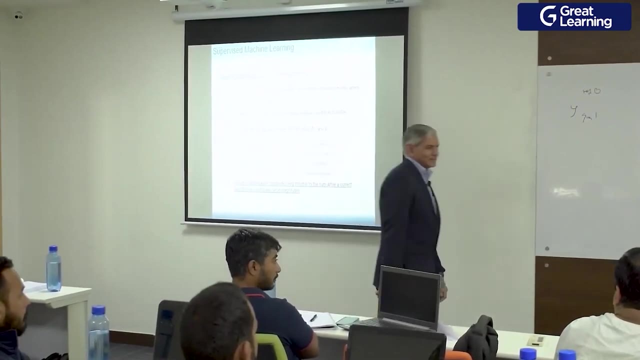 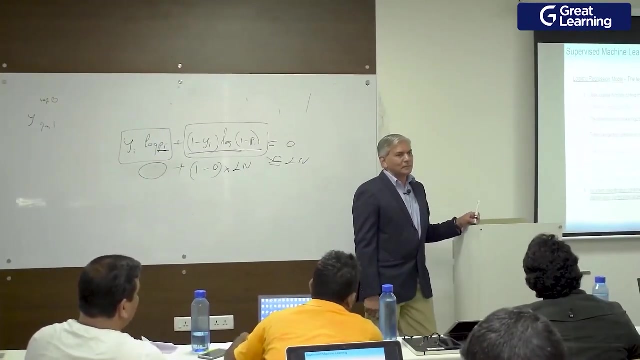 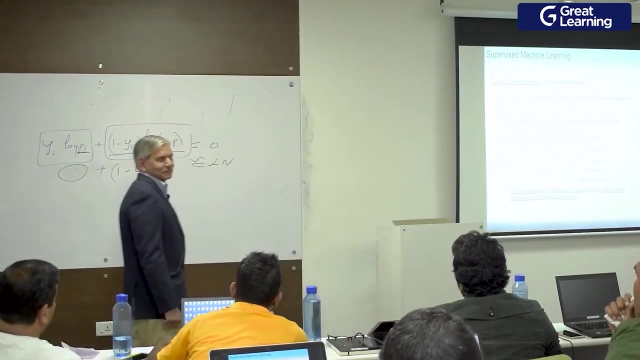 gradient descent here. this will drive the gradient descent Right sigmoid curve. Both happen together. actually both happen together. it is not one after the other, both happen together, sometimes 0 and 1, all 100% is your complete loss, Which will happen when you have all the reds. 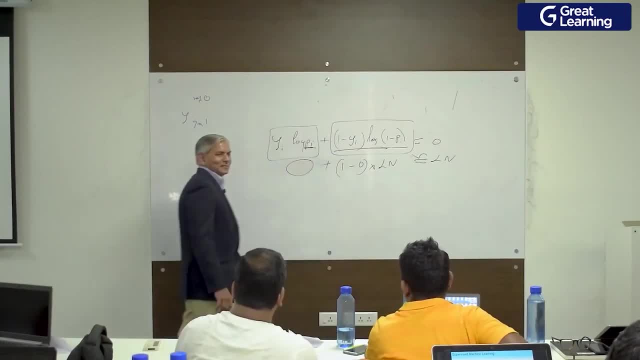 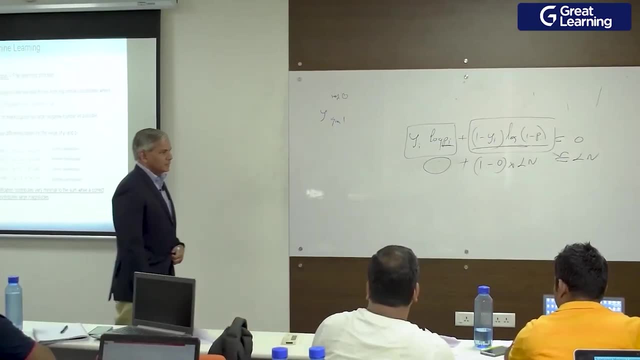 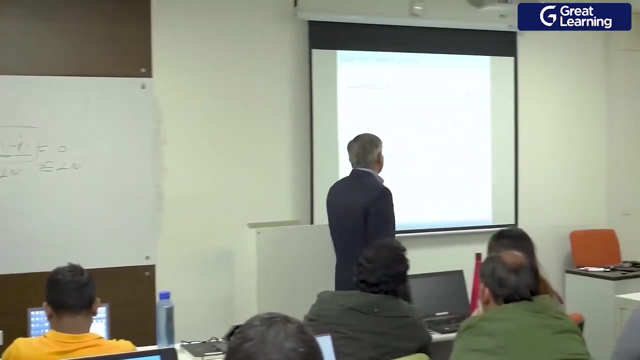 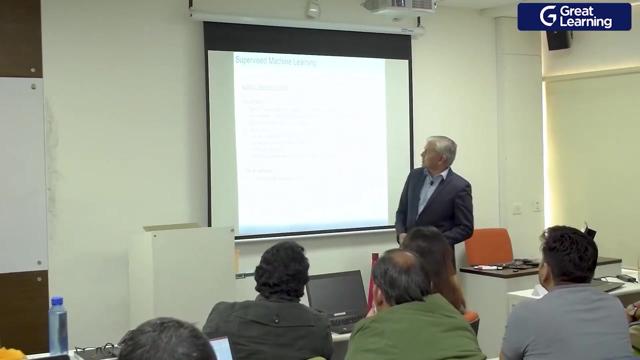 have been classified as blue and all the blues have been classified as red. Yeah for classification always 0.. All right, Shall move on. Extension of linear model that we saw yesterday. The beauty of logistic regression is it makes no assumption about the distribution of classes. 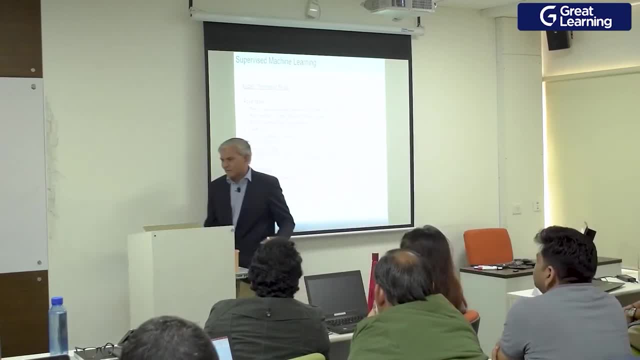 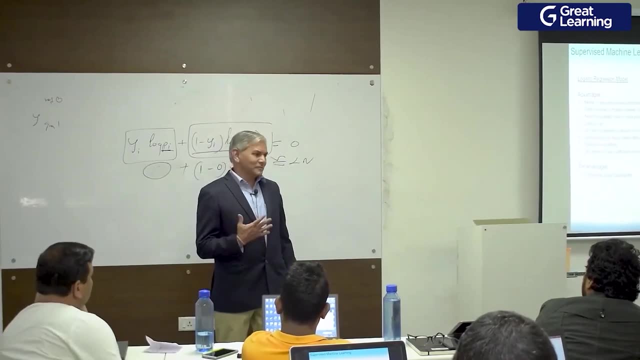 in the feature space. Many of these algorithms linear model, especially if you are building linear classifiers or linear regression. they expect Gaussian distributions. You understand the term Gaussian distribution, all of you? no, Okay, When you build any model, you will get the same distribution. 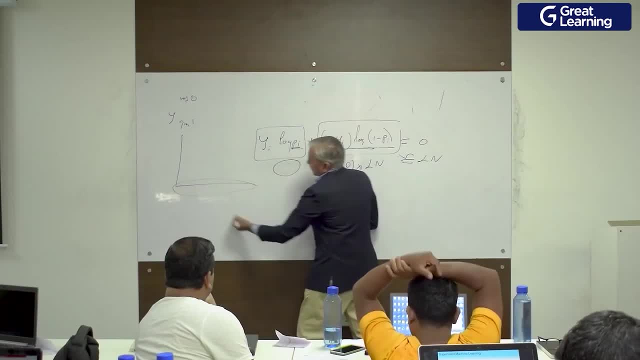 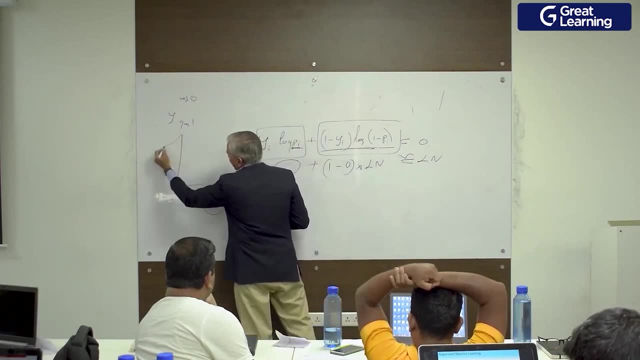 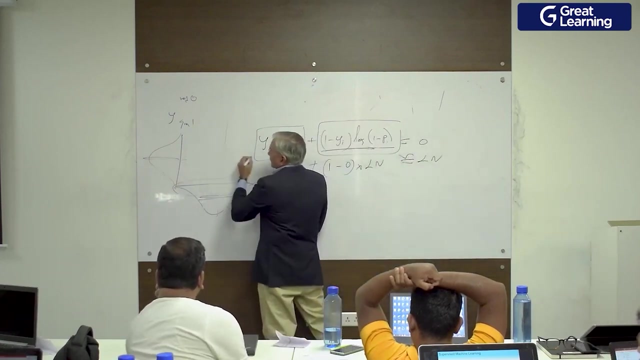 Okay. So the expectation is, if you take this attribute, the data will be spread around the central value of this attribute with some standard deviations. Same with this attribute, we will have a distribution with standard deviations. When you plot this together together in the 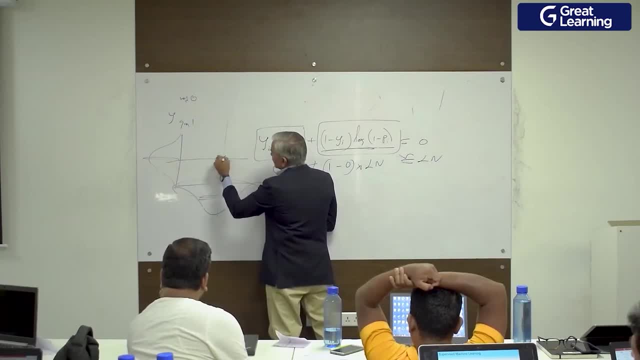 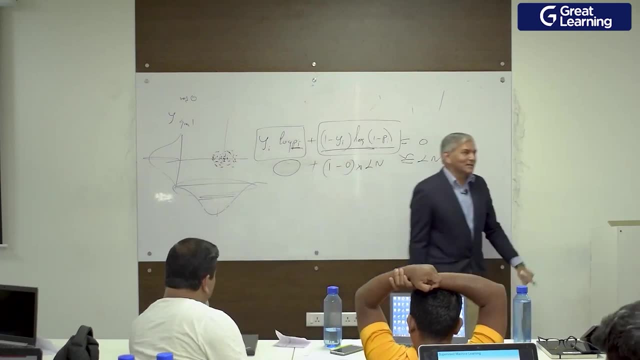 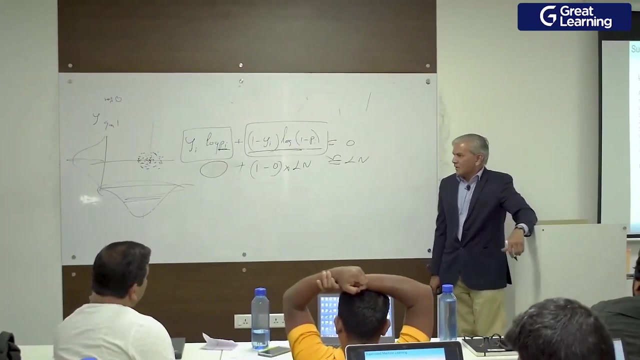 mathematical space they will look like if they are independent of each other. they will look like this. We have already discussed this. This kind of a distribution is called Gaussian. Okay, So in 3D it looks like a bell curve. All right, This algorithm does not make any 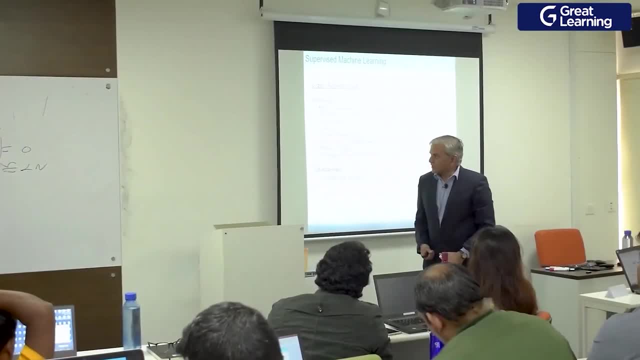 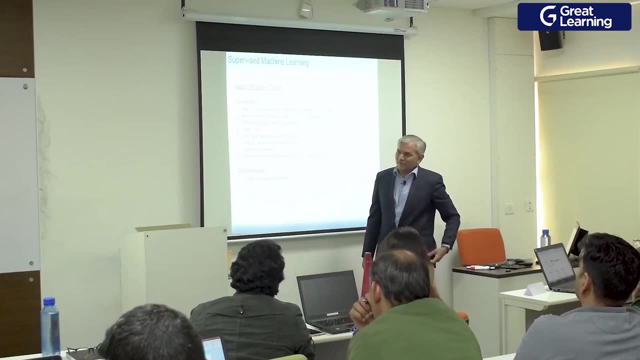 such assumptions. but keep in mind: if you have outliers in your data set, even this algorithm will fall on its face because it is based on linear model, So those outliers have to be addressed. What will happen if you have outliers? 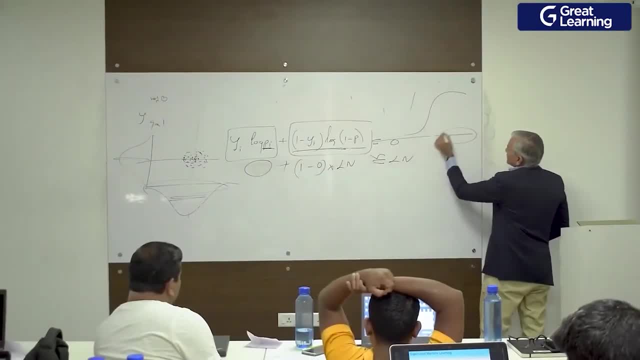 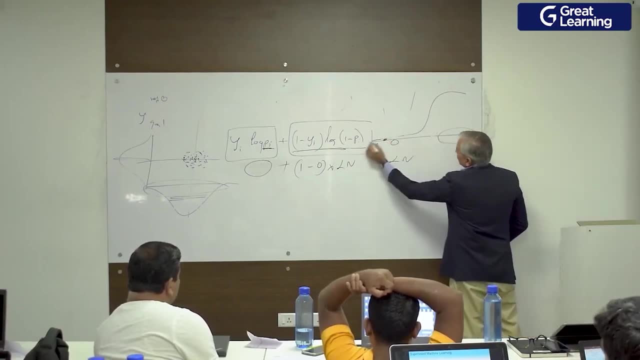 If you have outliers, you are likely to have outliers for, say, for example, what you call them the class 1. If you have an extreme outlier here, then you are in trouble. If you have outlier on this side, no problem. If you have outlier on this side, you have. 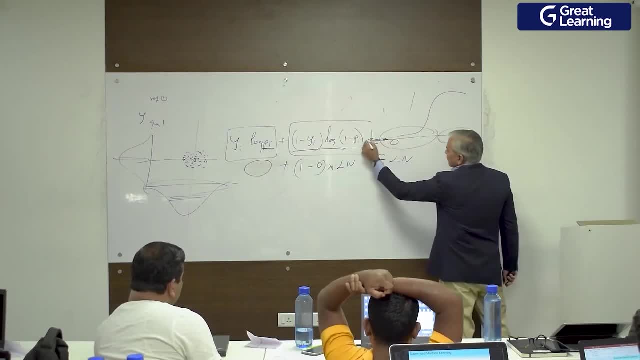 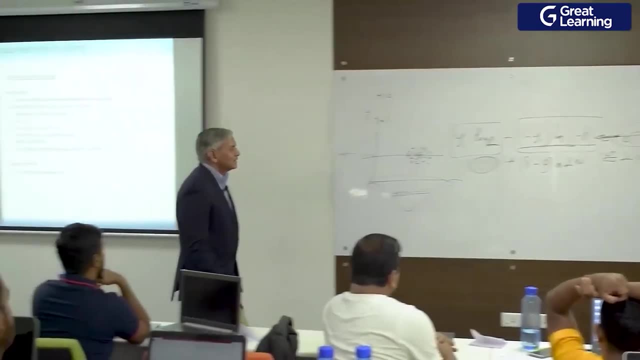 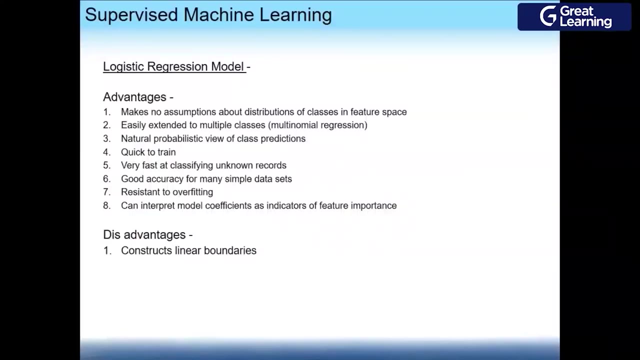 a problem. So more extreme it is, more severe the outliers is, more the errors will be Right. Okay, You can do multi-class classification, Yes, Yes, Yes, Using either binomial distribution in this case or multinomial distribution also is. 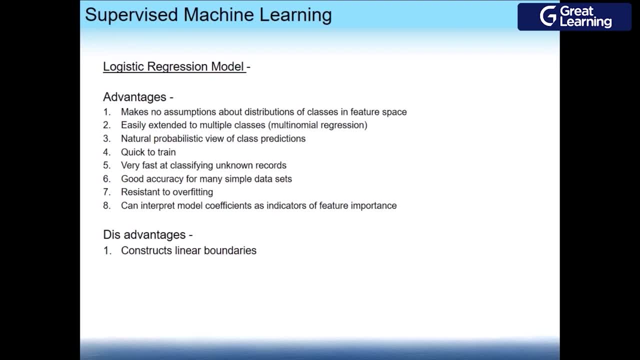 possible. You can also print out the probability values if you are not interested in the class, but I want the probability values. What is the probability? belongs to this class or that class? Quick to learn because it is based on linear model and you have gradient descent. 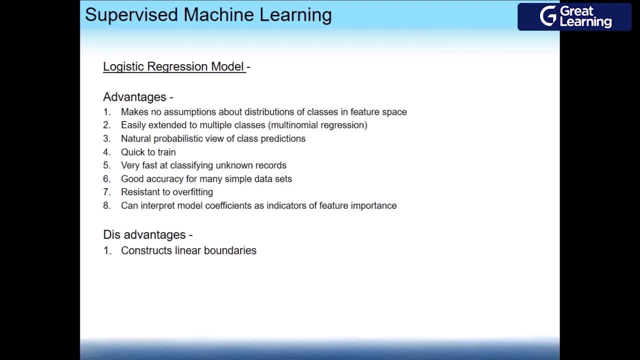 to help us out, to find the best fit line quickly, Fast in your test data also. Test data also. it is very fast. Yes, Yes, And as I said many times, I have personally seen logistic regression stands out among the top few in many of the situations. 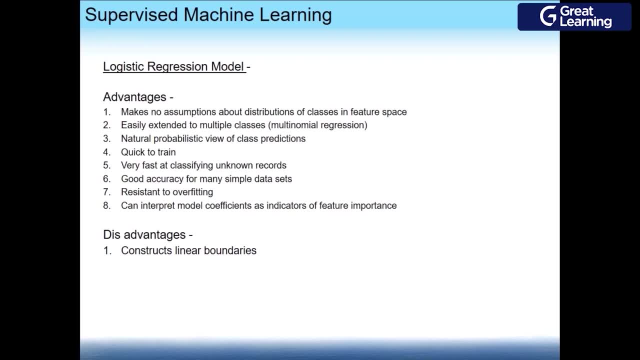 Resistance to overfitting because, as a simple linear model- linear models cannot be very complex shapes- it is resistant to overfitting. Okay, Resistant to overfitting does not mean resistant to bias errors. It may not be resistant to bias errors. It may not be resistant to 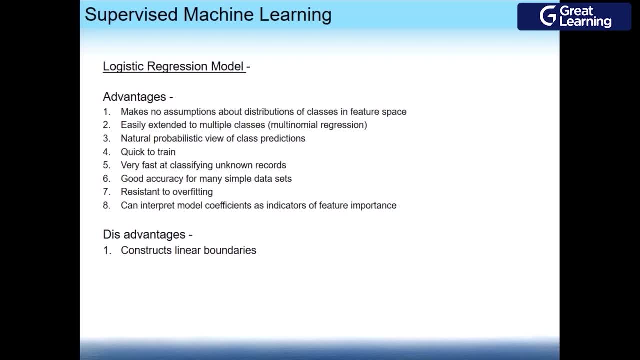 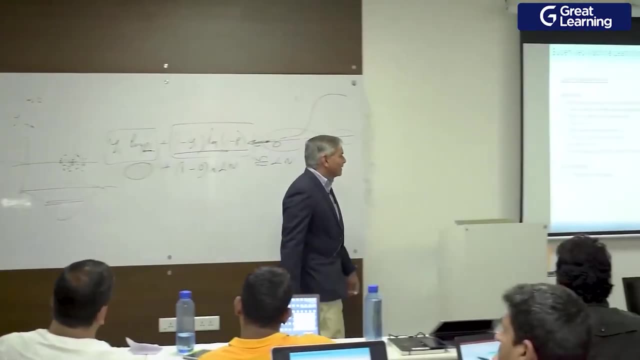 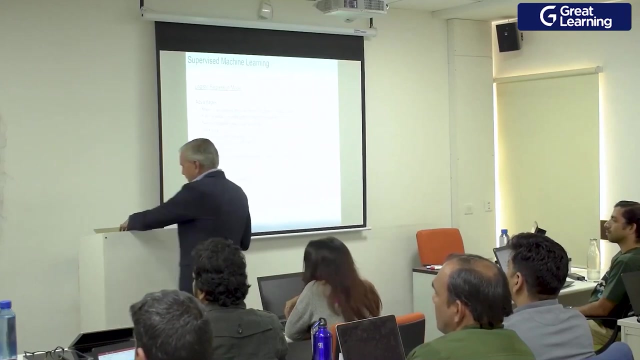 variance errors. It means resistant to variance errors. But we have another one to deal with And you can print out the coefficients, the probability values, and interpret the probability values. So the model is not a black box. Right Disadvantage in classifications is it uses linear boundaries. What it means is if the 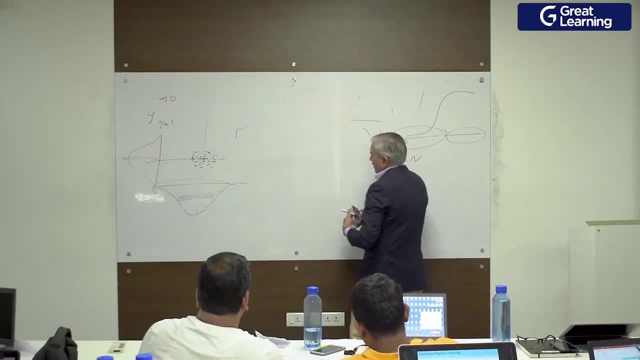 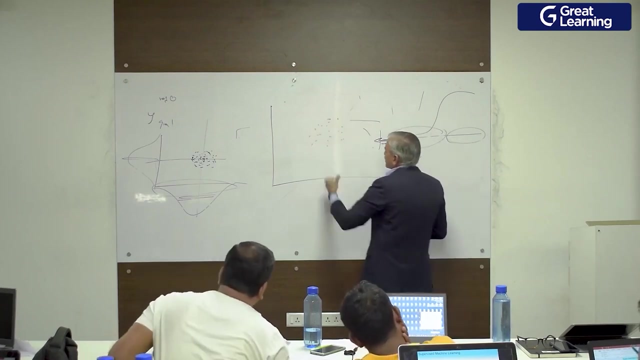 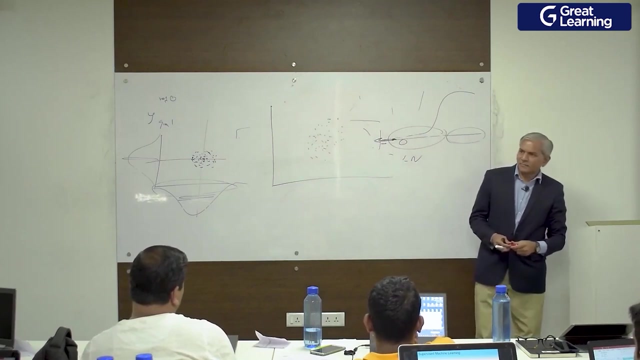 distribution of the classes. Yes, If the distribution of the classes is something like this, then the model will suffer. Right now we took a linearly separable this thing. but what if the distribution is not linearly separable? Then logistic regression will suffer. If the distribution was like this, with overlap, 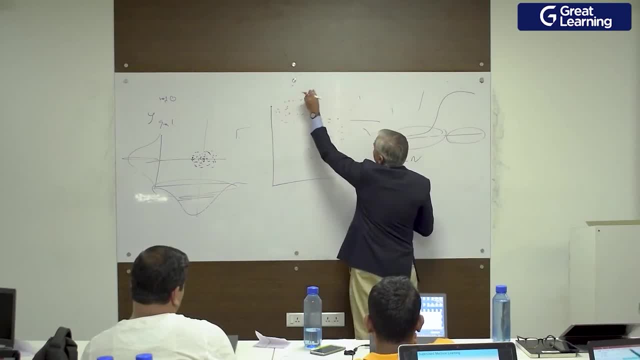 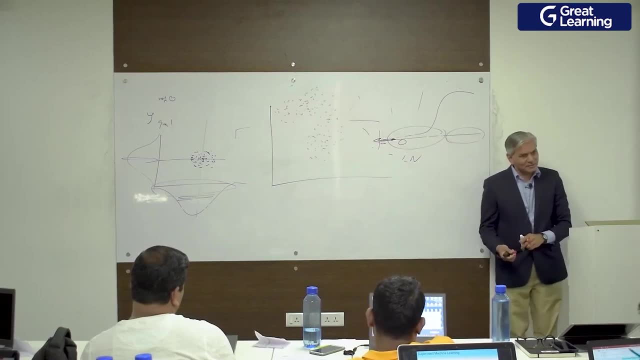 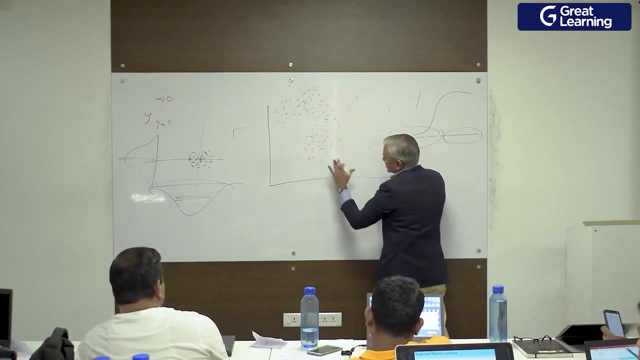 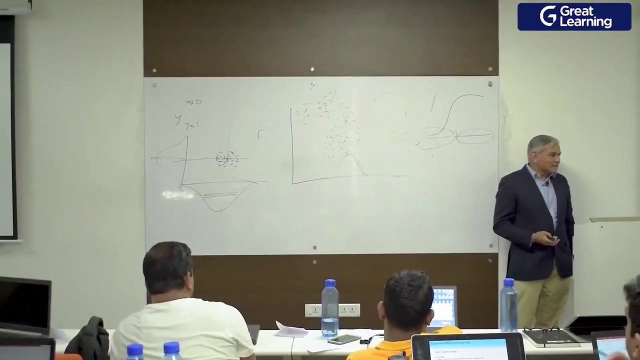 but it was like this, Then it will loop well. But if the distribution like this on the attribute you have decided, you see the difference. The difference is, if I plot the density graph, Okay, In this case the two density curves are overlapping Your t-test, analysis of variance and all these. 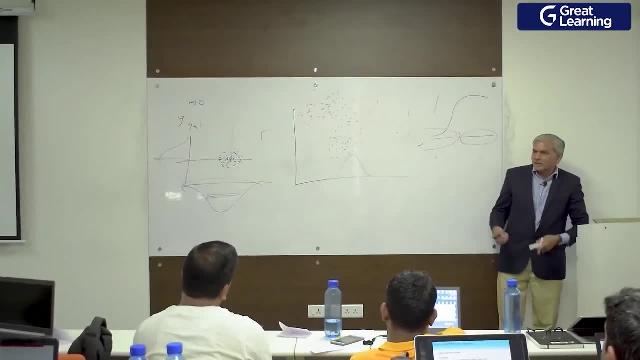 things will will tell you that these, this record belongs to this class, that class 50-50.. It will not be the same Right, It will not be the same. It will not be the same. You will not be able to classify. 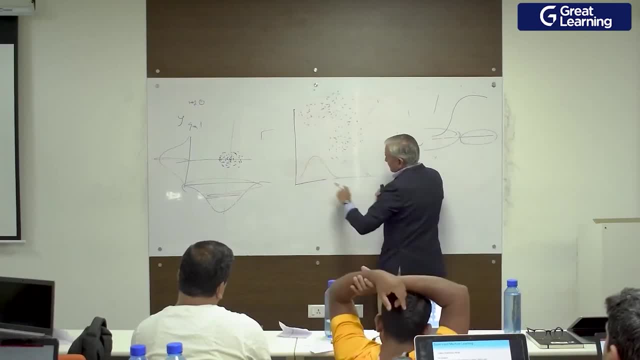 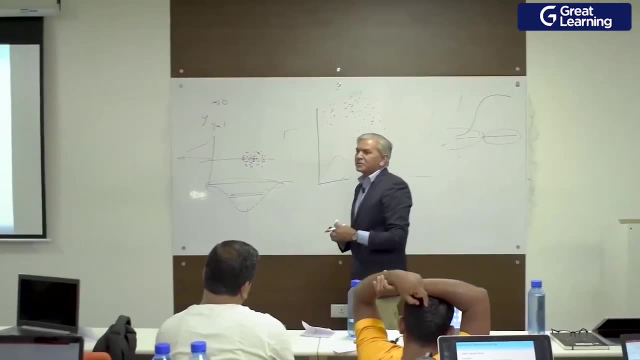 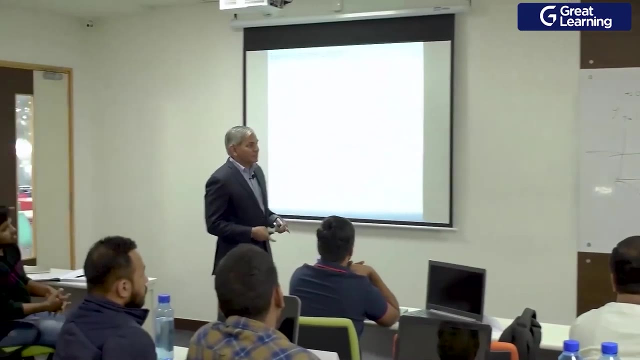 On the other hand, if I look at this situation, your overlap is there, but the central values are shifted apart. So when we have distributions which are linearly separable- may not be 100 percent- then logistic will do well, But you have distributions like this. I do not know. 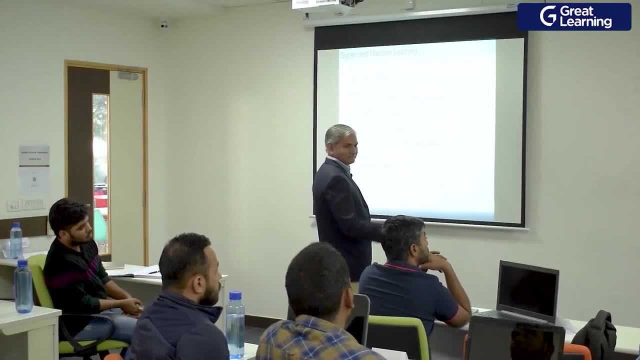 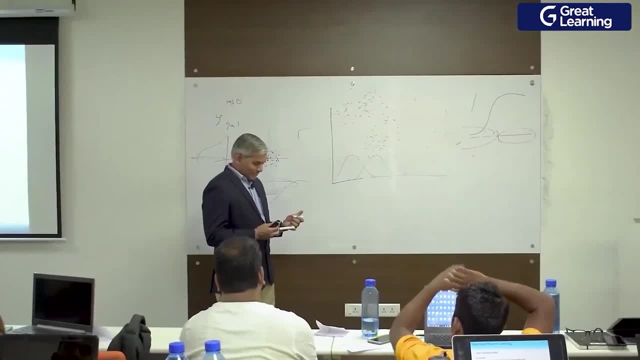 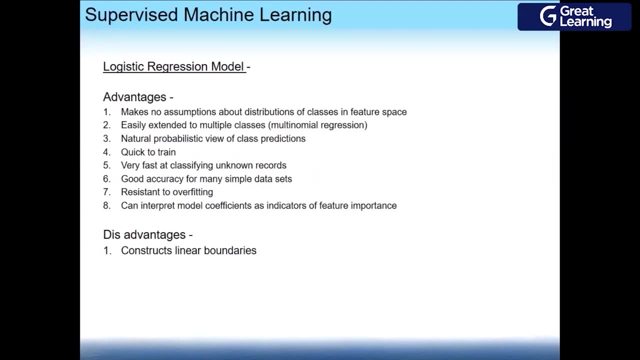 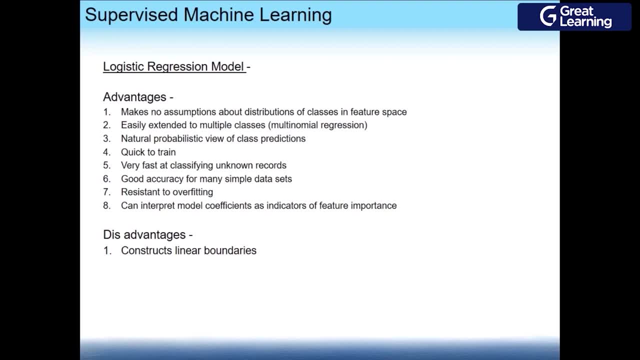 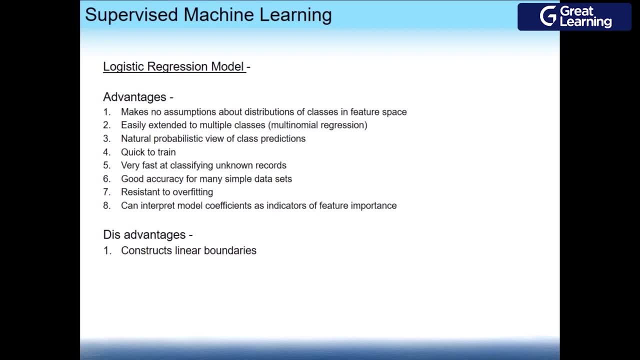 are distributed, which dimensions or which attributes are able to linearly separate the two classes? use only those for your classification models. You have some attributes where both the classes are significantly overlapping, including the central values. using such attributes for building model is useless and Pima Indians. 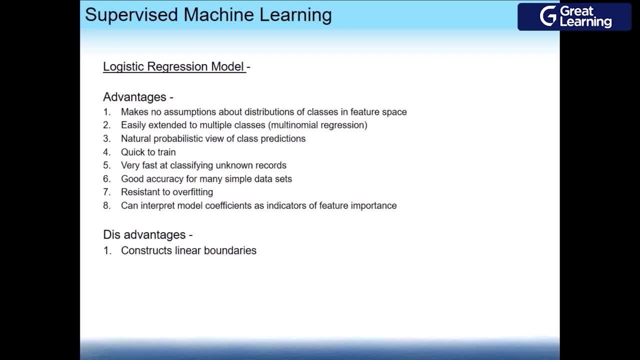 you will see, all the dimensions are like that. So then, what we can do? actually we can't do anything. no other algorithm can do this, No algorithm can do that. What human brain cannot do, an algorithm cannot do. So you have to have at least one attribute, as you will notice in another data set that 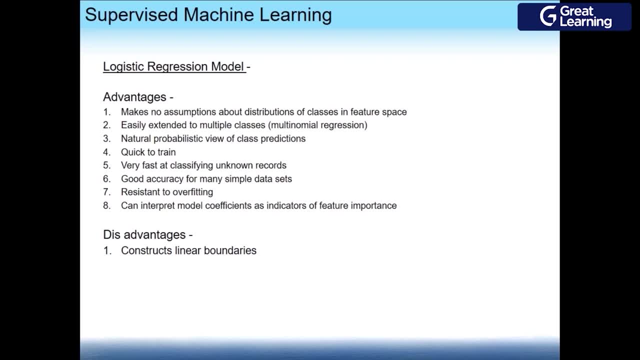 is called bankcsv. there also the data overlaps on all the dimensions between the two classes, but there are few dimensions 2 or 3 where the data central values are separated apart. Based on these three, it gives you 96% accuracy. 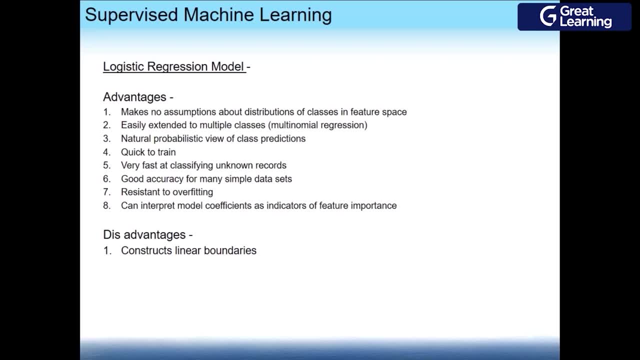 For our model. we should consider only those. Only those. yeah, correct, You don't need to include all of them. What is the name of that? Bankcsv? there are two attributes, Some attributes I am just randomly picking. What is that term called? 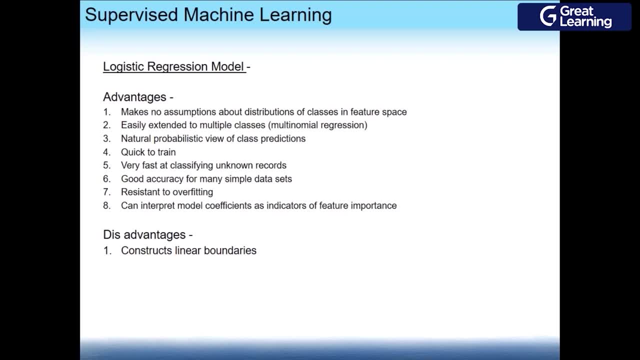 This is scatter plot. This is scatter plot. Now you find out how the density of the plot changes when you move from this direction to this direction. It is like a graph. It is like a graph. When you move from this direction to this direction, you will see that the density is very low. 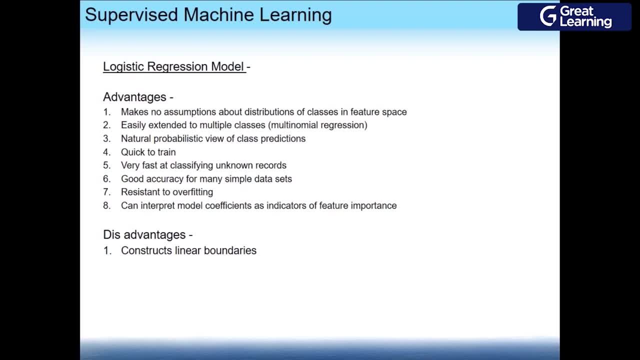 very low, very low increase is very high, highest. then it starts falling. So when you convert this into 3D it becomes a normal distribution In 3D. this becomes a normal. That is called density distribution in 3D. 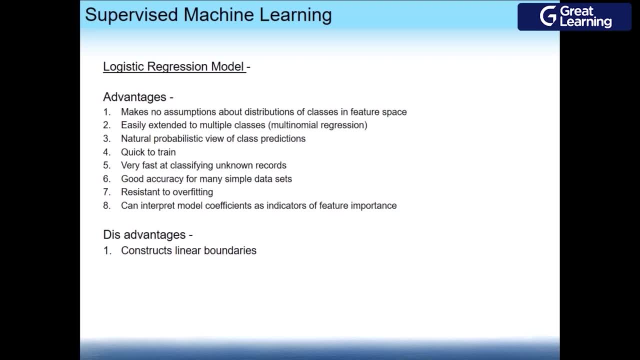 Sir, can we, can't we switch the axis for analysis in this case? Can we, Can't we switch the axis for analysis? Switch means, Say y axis becomes x axis, so that you are distributing. What you are basically saying is: 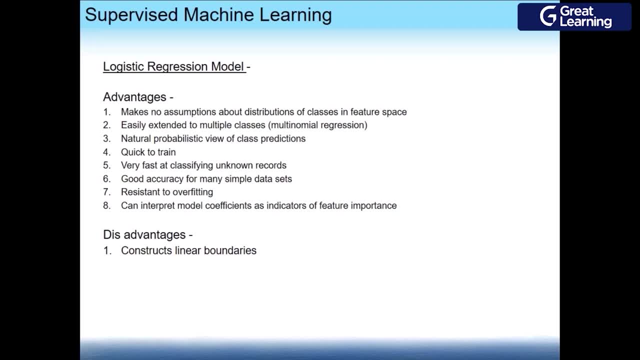 No, I am not. I am this way. I am comparing these two. with this over here, This axis is not there. I am just saying, if you have a distribution like this, your logistic will do well. If you have a distribution like this, your logistic will suffer. 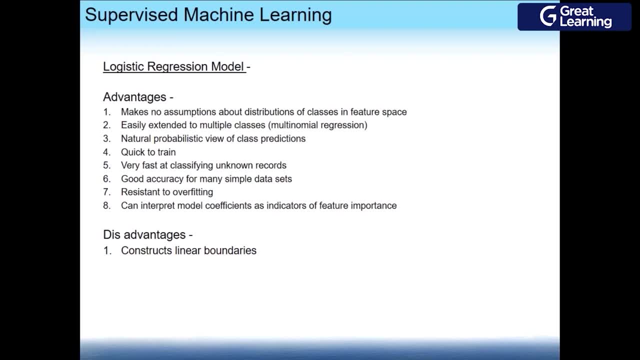 Any algorithm will suffer, Ok, But what you are saying is: can't we switch to this axis where the two classes are separated out? That is what you should be doing. So if you have two axis, two attributes on one attribute, they are not linearly separable. 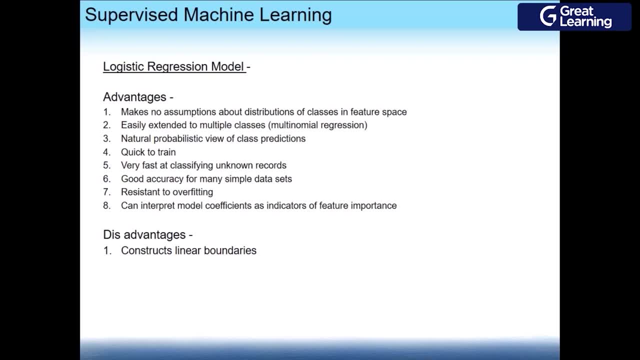 at all. But on the other attribute they are linearly separable. use the other one. That is what I am saying. Yeah, alright, Sir, in two dimensions let us say like this: we can change the three dimensions, we can. 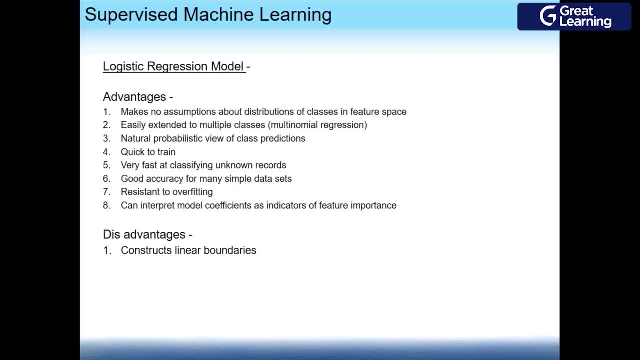 see some of the data are up. So use that dimension which is helping you to separate out two. do not use this dimension, Can we? can we apply one model on one attribute and then separate the attributes? That is a very complicated question. 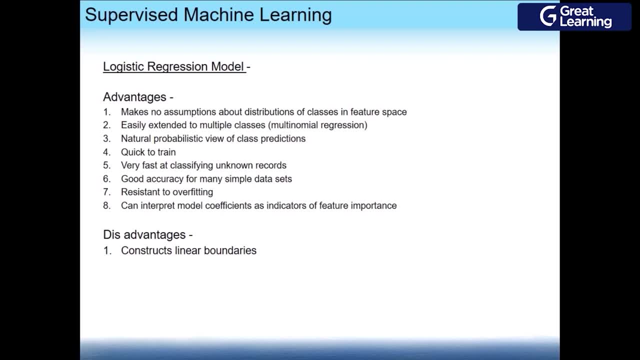 That is not a very important question. How do we solve this Random forest? every node of the forest is constructed using randomly selected features from the data set. Yeah, it has internally. it internally does that, But random forest is the only one which comes close to what you are asking. 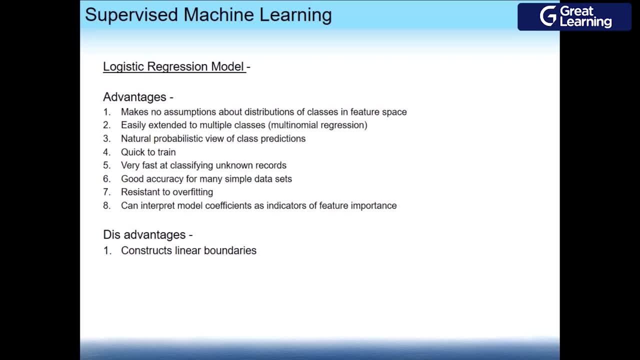 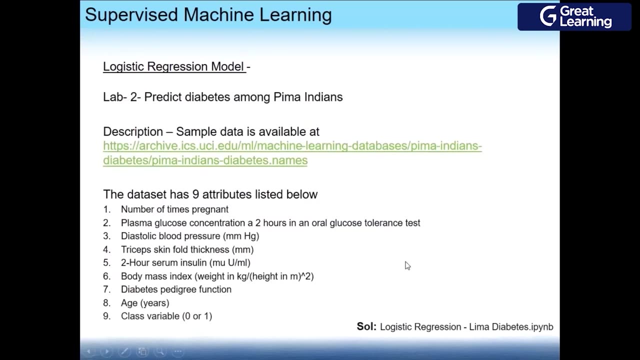 No, no, no, it does not do that. It randomly picks up. It does not see whether b is in this data set. Alright, Ok, Let us move. Let us do a hands on. Ah, this is the same data set. 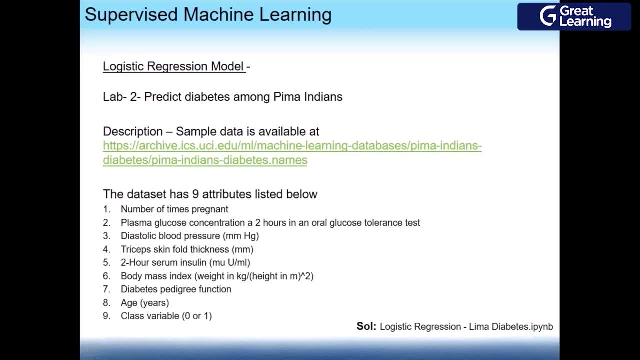 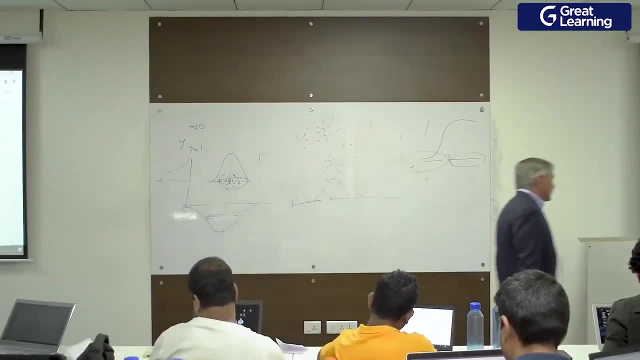 T-Mind Enceladus data set. Same data set. Shall we do a hands on on this? Ok, Alright, guys, Are you all ready? Yes, Ok, So if you have access to the code, the first line is matplotlib. 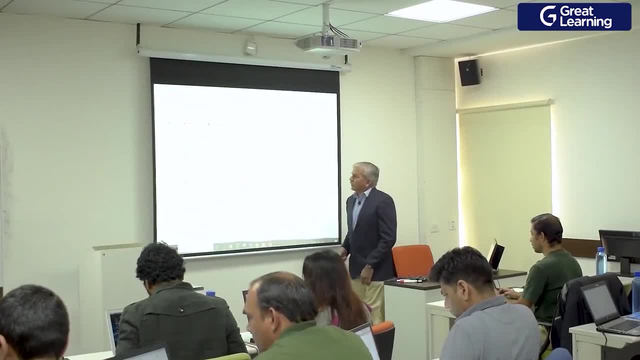 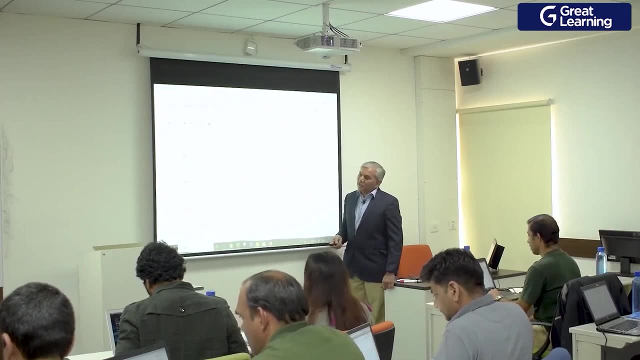 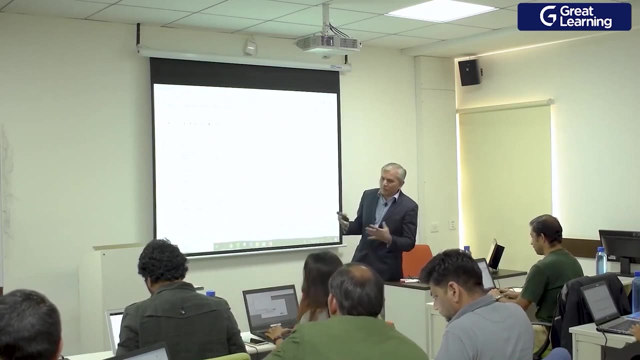 You already know what it means. I am importing from scikit-learn linear model logistic regression. Yesterday we had imported linear regression. Ok, Then I am importing matplot as plt seaborn. I use seaborn libraries for my plots. 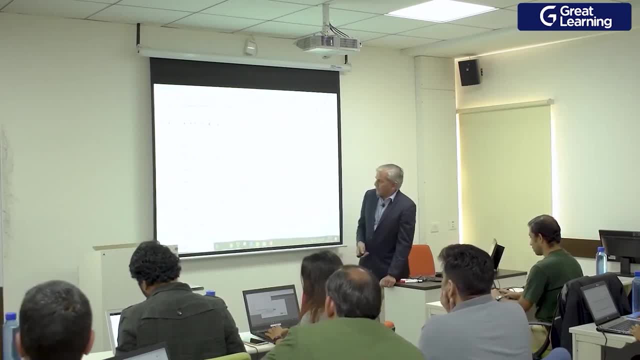 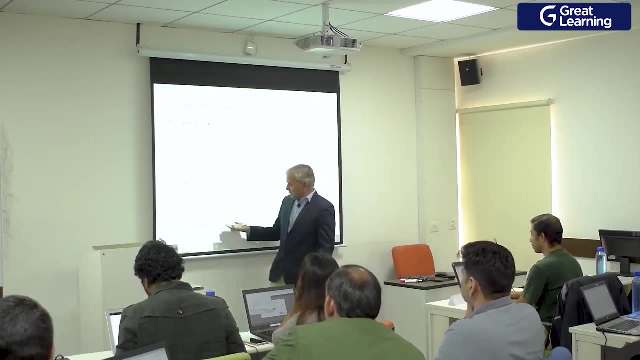 Especially, pairplot comes out very well in this. So I am going to use this Train testplot. you already know what it is- Numerical Python- And to measure the accuracy of the model I am going to use metrics. 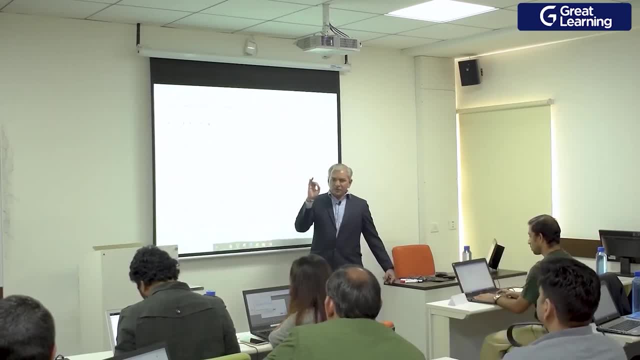 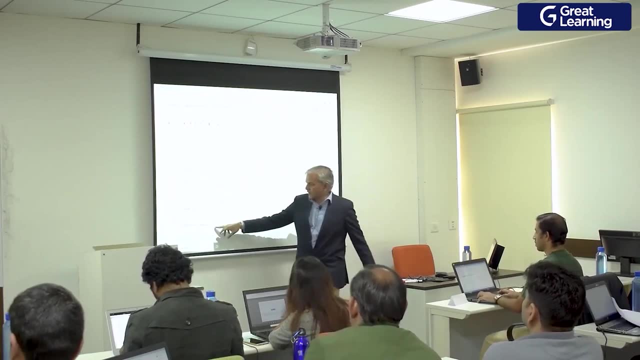 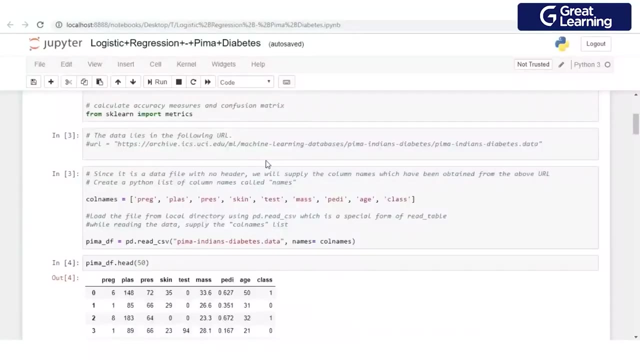 So whenever you are doing classification, one of the most important tools for evaluating a model is your confusion matrix, Confusion matrix. Ok, So that comes through this metrics library. We will see all these things down the line. Earlier this PMR diabetes used to be available in UCI dataset, but now I think it has been. 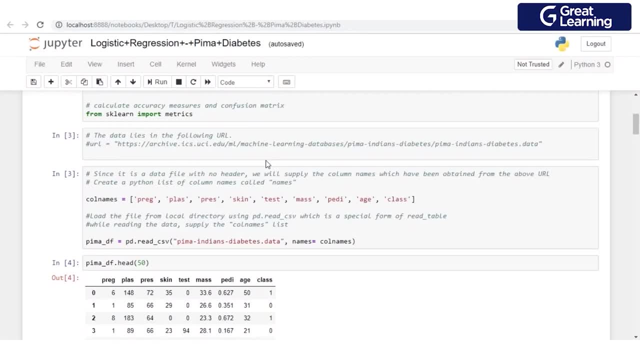 removed or archived So it is not available. But I downloaded it from caglcom, another site. I am loading the dataset over here. It is a data file, It is a text file. Why loading the dataset? While loading the data file, I am feeding the column names here, which I got from the 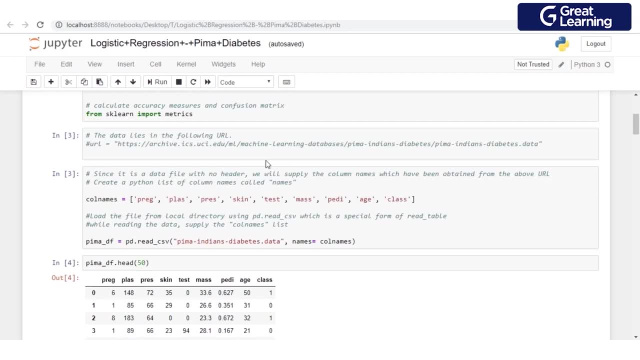 original source: the column names. So the column names are: the first column name is pregnancy. how many times? by the way, this particular test was done amongst Pima tribes, a tribe in South America where, apparently, the ladies are prone to type 2 diabetes very early in age. 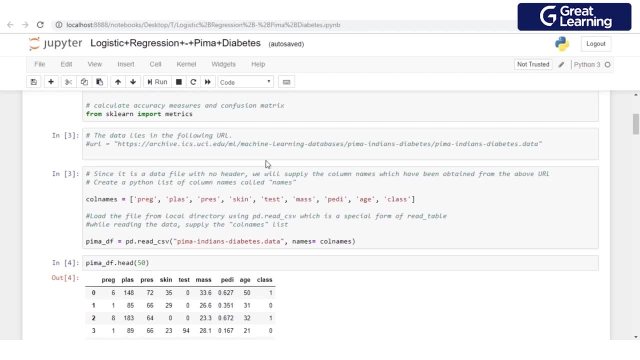 So this research was done by this university, where the objective was: can we build a model and predict who is going to have type 2 diabetes by the teen age? ok, For that. they did research on that community. some of them were diabetic, some of them were. 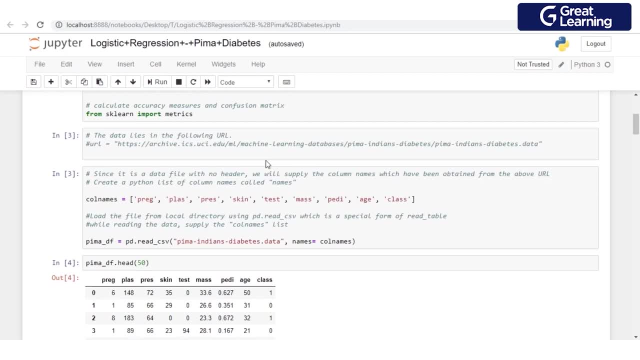 non-diabetic, and the characteristics that were captured are these: The first one is number of times pregnancy reported by the subject. next one is plasma level in your body. Plasma is a component of the blood. Then we have blood pressure. This is systolic, systolic, diastolic blood pressure. 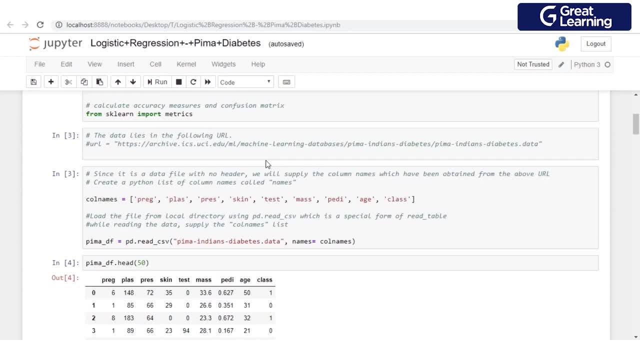 This one is diastolic- diastolic blood pressure. Then we have skin where apparently people suffering from type 2 diabetes in that tribe they have some kind of skin folds. This is measurement of that. Then they do some testing. this is called fasting sugar test or something that is this. 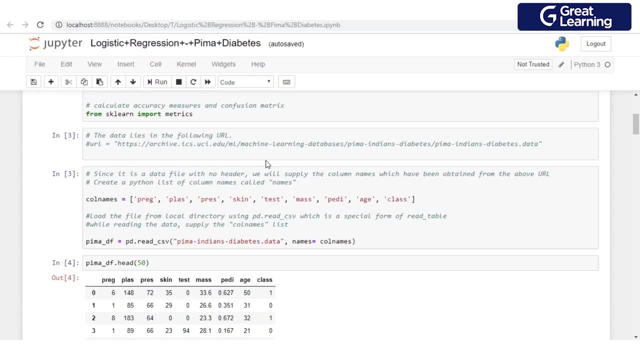 test. Body mass index, PEDI is another test. some pedigree test they do, I think. it is another test related to blood sugar, age. and the last one is your target column, whether this person was diabetic or non-diabetic. Diabetic means 1, non-diabetic is 0. 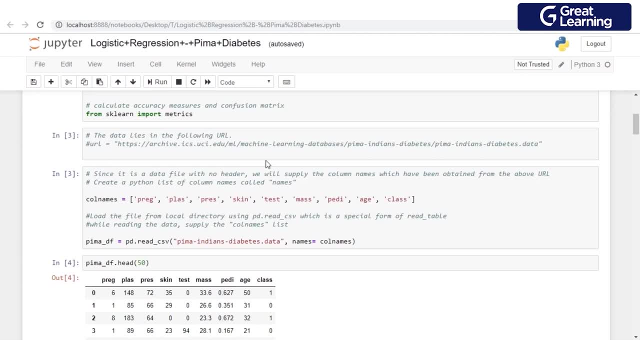 Now, the whole thing that the objective is, we are trying to find out: is there a relationship between the independent variables and the target variable? What is that relationship? We are trying to find out, That relationship we assume exists in the universe, in the real world. we are trying 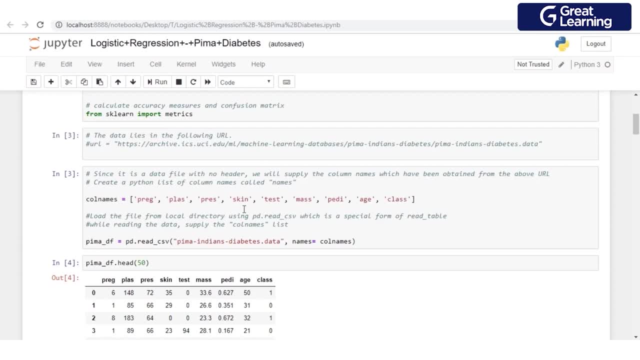 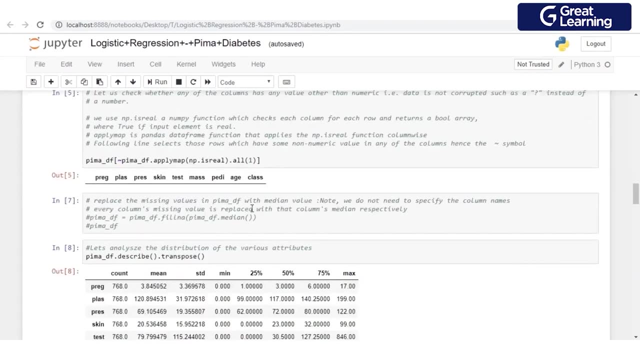 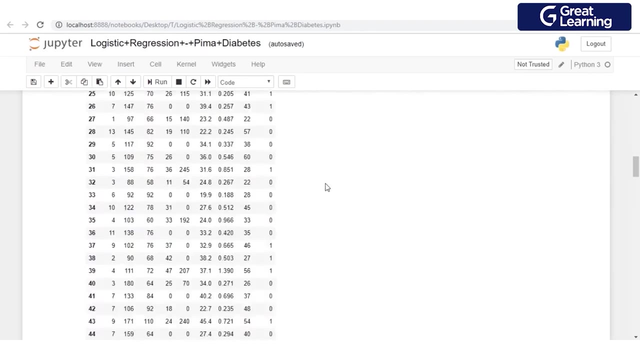 to find out whether we can discover that relationship. So for that we are building this model and I always do this based on the experience on CAR-MPG dataset. When you look for this head, ok, when you look for some sample records, you see all. 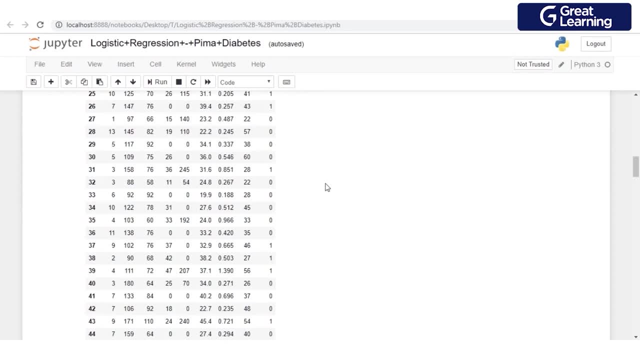 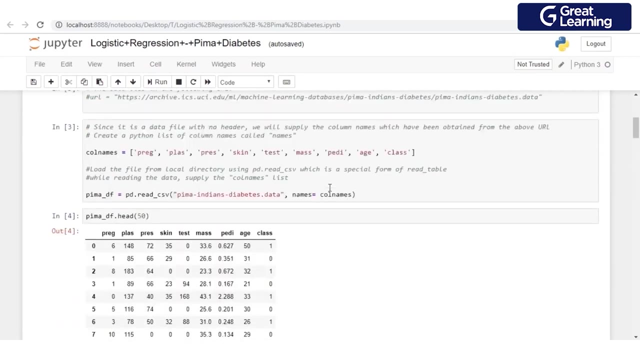 numerical values, But what is the guarantee that there is no record further down? There is no record further down, Ok, Which has some non-numerical values sitting in the numerical columns. What is the guarantee? How do you identify that? To identify that we can use, we can use this method. 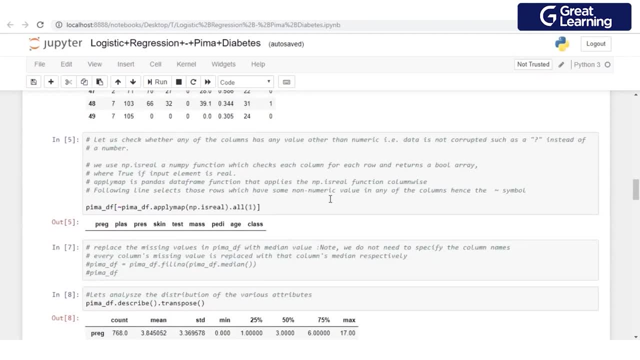 What I am doing is I am using a numerical python function, isReal. This function is a binary function, it is a Boolean function. It will give true or false. This function, I am applying it on to look at this apply. I am applying it on to all the rows, all the columns of this. 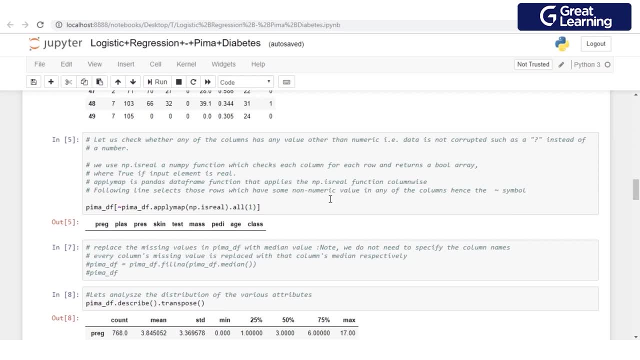 This is the beauty of python, where you have to do minimal coding. If you have to do this in java, you will probably write a for next within a for next over here. So all that thing is taken care of. So what is happening is I am going to apply this function isReal on all the rows, all. 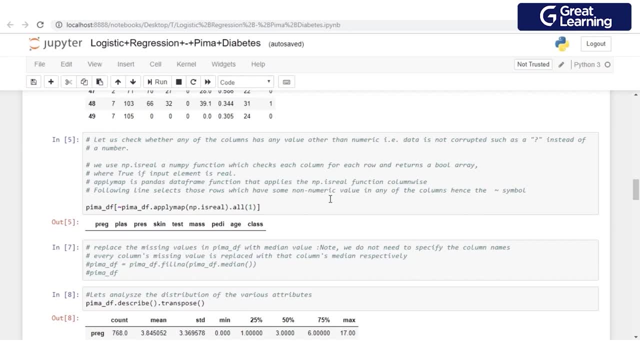 the columns of pYDF. Ok, And you see this tilde over here. this is a not operation. I want only those records where it returns a false. Ok. Fortunately there are no records where it returns a false, which means all records. 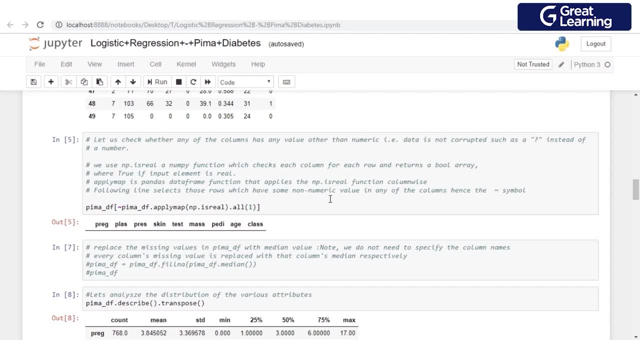 all columns are numericals. What is the other way of finding out whether any such non-numerical characters are coming to the data Data types? Df types, Df types- that's all Df types. when you do, it will return the data types of all the columns. 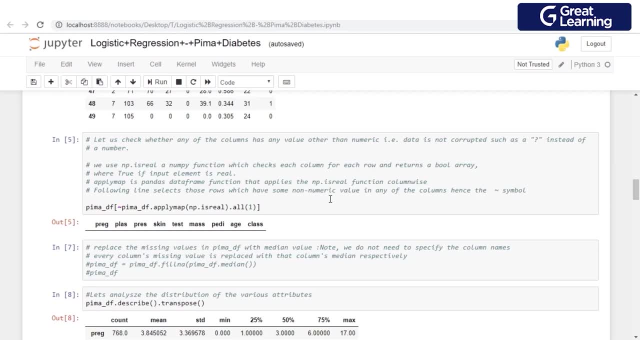 If there is any non-numerical value in any of these columns, it will return it as object. That is easier than this. df types. What we do if there is a, We have to go and identify the record, convert that into na na n numerical. 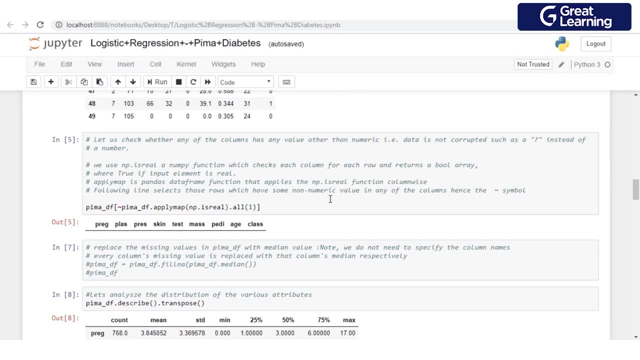 Then you can do the same thing, Ok. Ok, So you can replace with median mean, whatever replacement strategy you have. We don't have any such case right now. Ok, But we have nothing to be happy about because we are seeing lot of zeros. 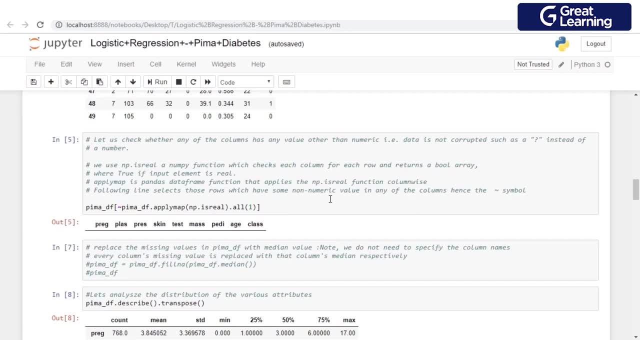 And zeros in blood pressure is surprising. it can't, be not possible. Zero in plasma is not possible, But you have zero values in blood pressure, you have zero values in plasma. So missing values are there. the missing values will cause problems. we need to address the 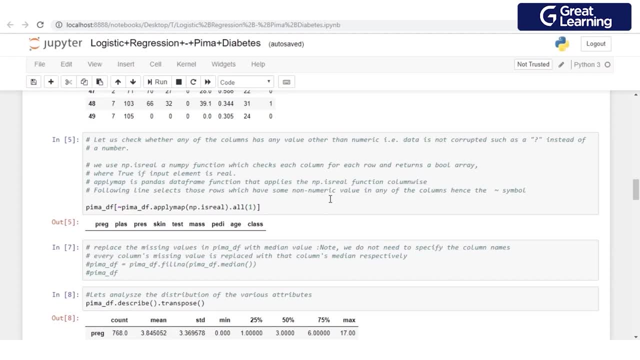 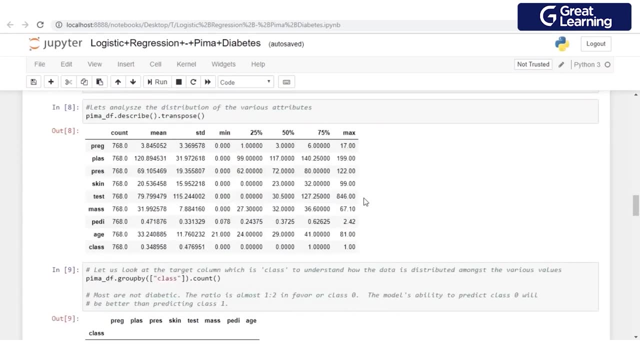 missing values. Ok, Let's move on. Do a df. describe how the data is distributed on the various dimensions. univariate analysis. If you don't like this, don't do it. do the pair plot. Pair plot also gives you visually the same univariate analysis. 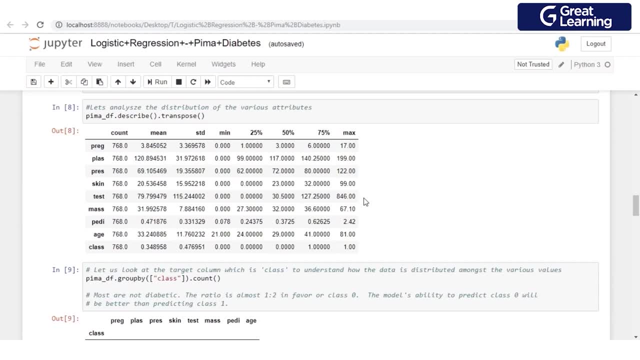 Ok, So I will quickly tell you one. look at the difference between: for the test data, sorry, the test attribute. Ok, Look at the difference between the mean 80,, almost 80, and the median 30. The mean is drastically shifted away from the median on the higher side, which means 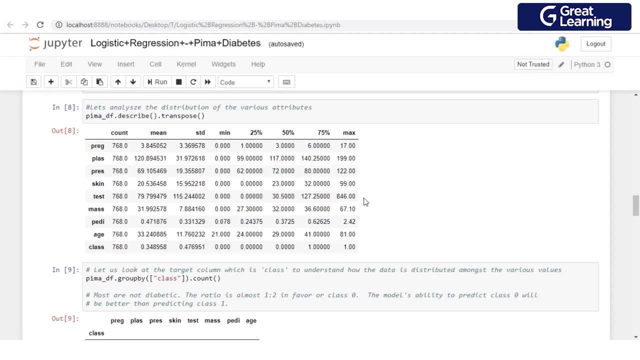 there is going to be some long tails on the right side. on the higher side, Mean gets easily impacted by outliers, So some outlier is pulling mean towards the right side. How do you confirm that? Look at the distance between the third quartile and this. 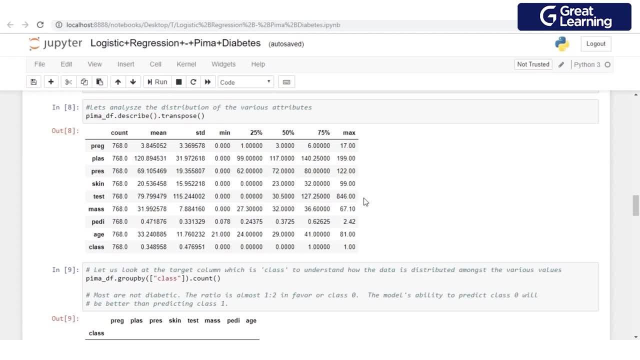 Look at this, Correct, Look at. you are like me. you don't want to calculate. Can you tell me how long is long The right side tail? look at the length and compare that to the left side tail. Left side: there is no tail. 719 units. 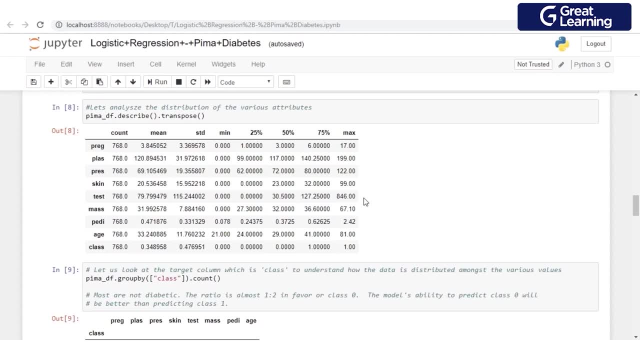 So is this possible or is this a typo? No, We need to go and check. Maybe this is a typo, We don't know. Ok, Right, I am going to move on. The next thing that you have to do is first understand how the data is distributed on. 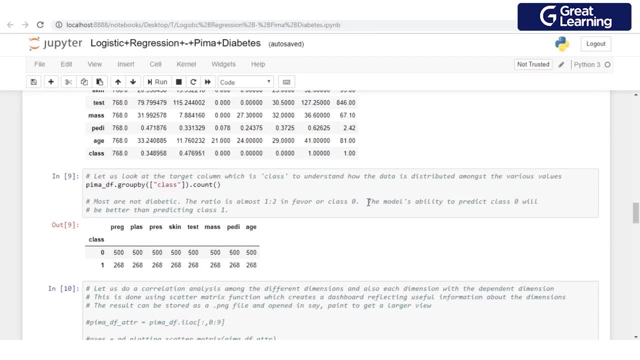 your various dimensions. If you think there are outliers, we need to address outliers. We already know we have missing values. we need to address missing values. The next thing you need to do is, since you are in classification, how many records are? 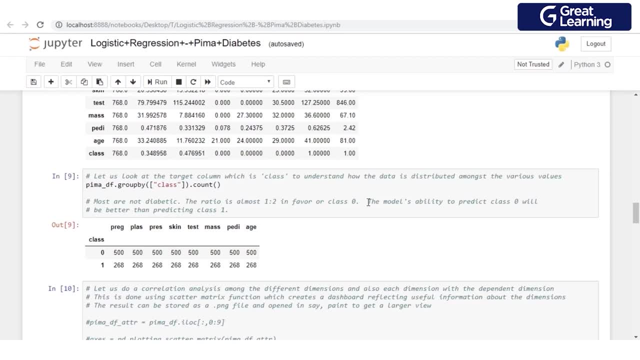 available for each class in the data set. Look at that. The number of cases for non-diabetic- 0, is 500, whereas the number of cases for diabetic is half of that, almost half. You are preparing for your board exams and most of the questions that you solve practice. 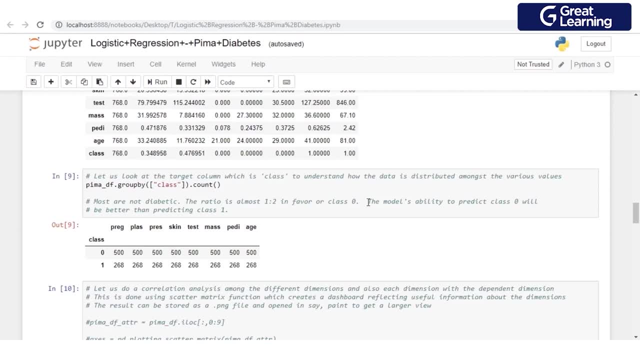 on is calculus A small part. you do it on trigonometry. Obviously, you are going to flunk in trigonometry. Ok, Right, Why? Because the pattern of questions that come to you in the exams in trigonometry may not. 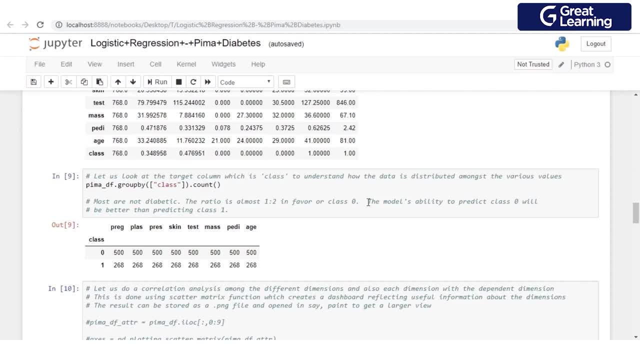 have been reflected by these patterns that you have used, Which means you have not gone through all the possible patterns in the trigonometry questions. Same thing will happen here To the model. I have given only 268 of the diabetic cases. Maybe this 268 does not reflect all possible permutations that lead to diabetes. 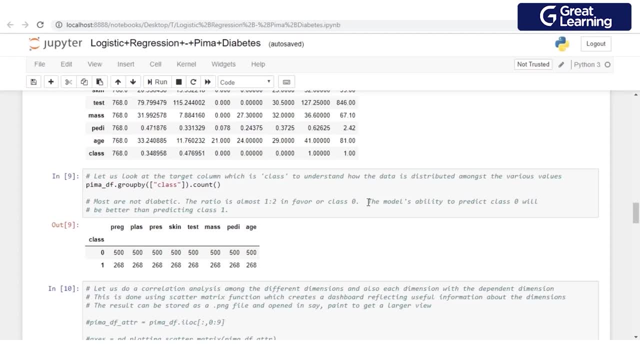 So the model will perform poorly in predicting the diabetic cases, will perform relatively well in predicting the non-diabetic cases, but I want the reverse. The objective is the reverse. Ok, And keep in mind whenever you are in classification and the classes are skewed like this all. 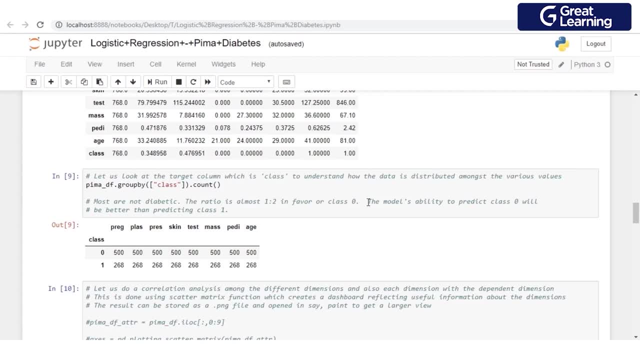 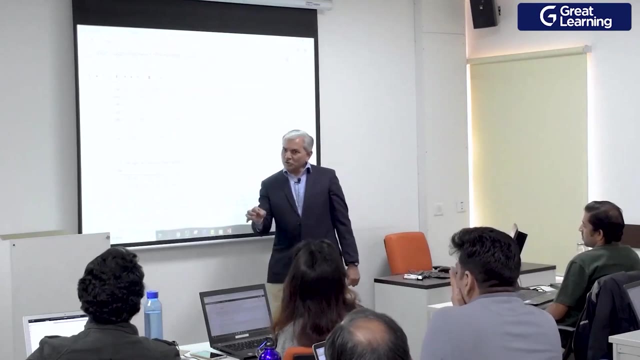 algorithms are biased towards the higher represented class. All models: the objective is to minimize the overall misclassification. Ok, So their focus will be on the higher class. So this is another source of bias which comes into the model, where the algorithms themselves 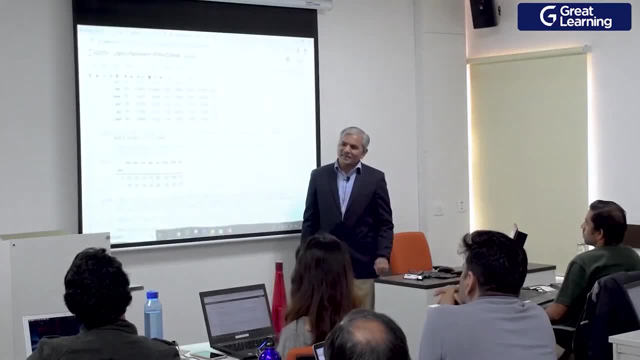 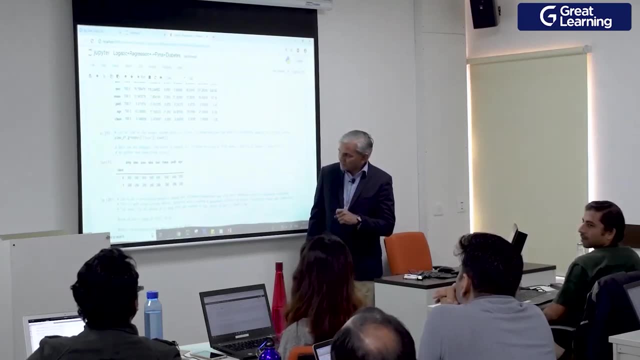 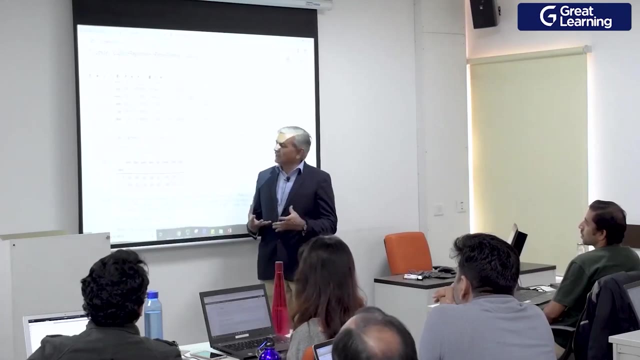 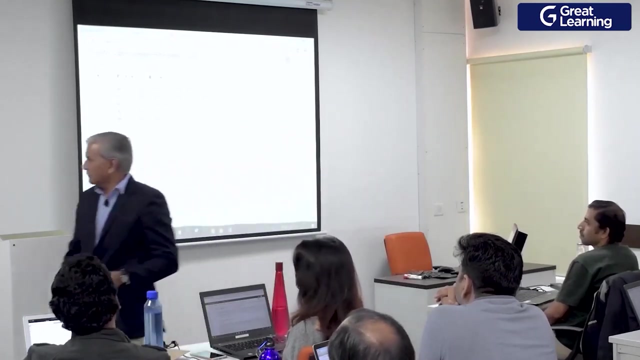 are biased. So how do you handle this? We find it to: yeah, We call this strategy upsampling, downsampling. ok, There is a strategy called upsampling downsampling thing which I will refer to, which I will take you through. when we do FMT model tuning, 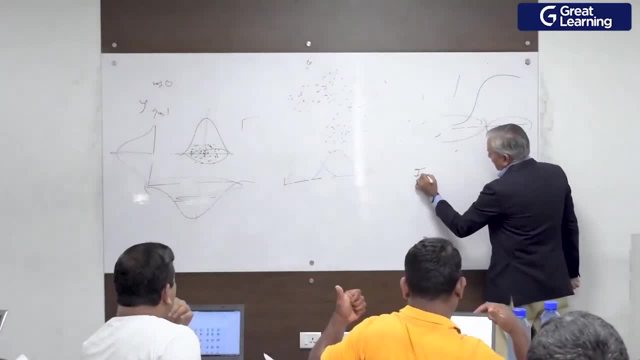 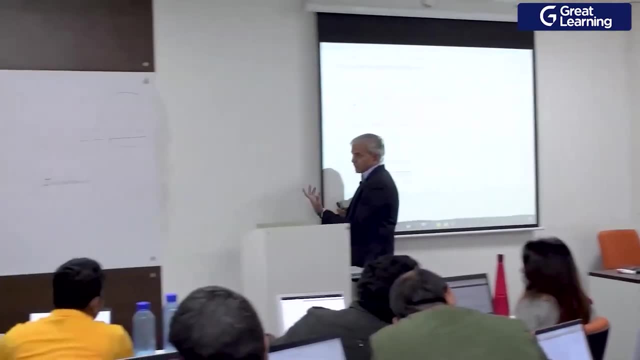 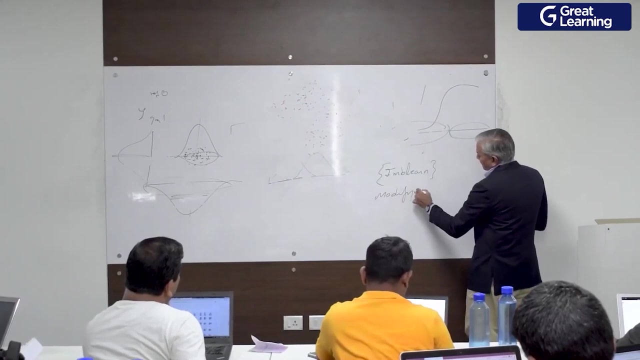 but right now we are not going to do that. There is a package available. it is called in learn, but right now we are going to live with this. There is another way of improving the this thing: the classification performing better in the underrepresented class. that is called modifying thresholds. thresholds In logistic. 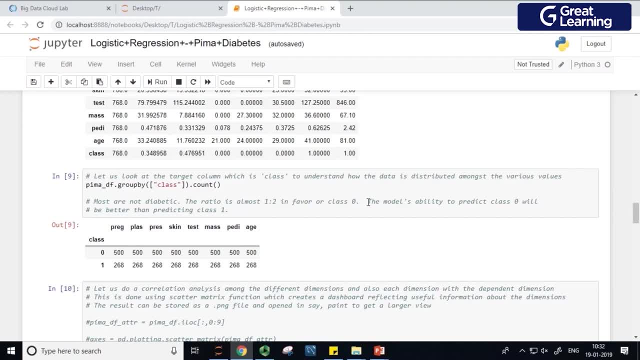 regression. Naive Bayes any other probability based model. the cutoff is 50 percent. If the probability of belonging to blue class is 51 percent, the data point will be classified as blue. If the probability of belonging to the blue class is 49 percent, the data point 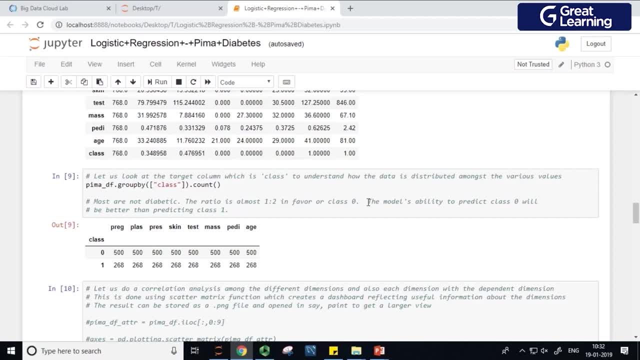 will be classified as red. So the boundary is at 50 percent. ok, I can modify the boundary. Now, none of the algorithms allow me to modify the boundary directly. I can build wrapper class. I build the model Around the model. I write my own class where I modify the threshold. 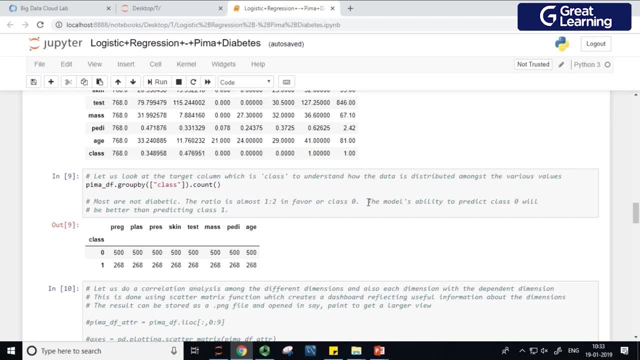 ok, Once again, I will cover this in FMT, not now, It will be too much. So we can play around with the threshold. modify the thresholds to improve the accuracy of the underrepresented class. We can do that. ok, How do we do that? We will take it later, But whenever you see. 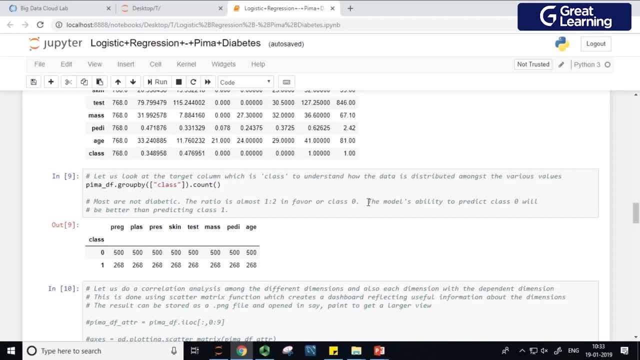 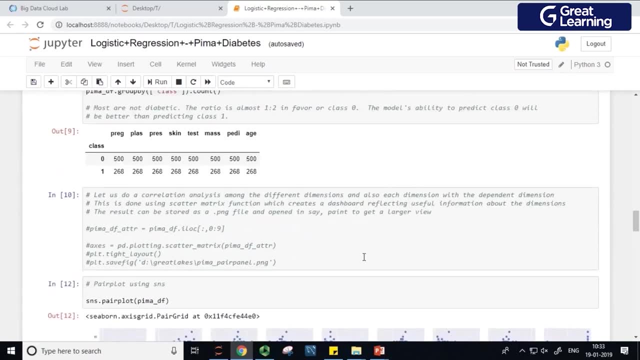 in classification scales, you will see that the thresholds are not the same as the thresholds and the distributions- Q distributions like this- be ready. There is no way you can achieve a very high accuracy for the underrepresented class unless you play around with these two. 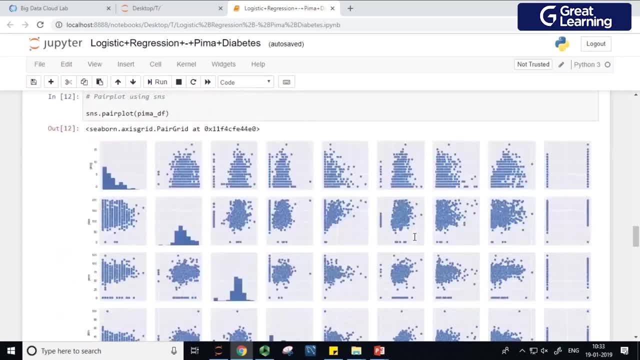 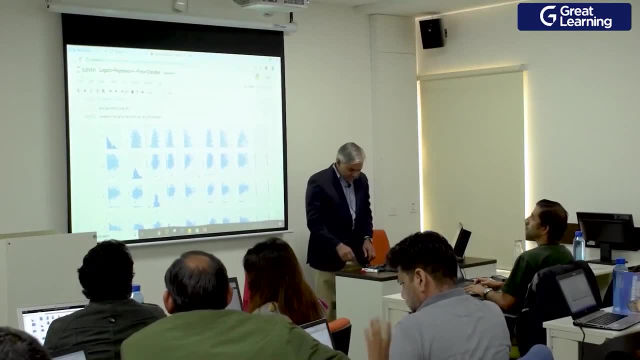 techniques. Let's move on. So this is my pair plot. Ok, I don't like this, So let me quickly redo this. Alright, I am going to come in to. I am not going to do all this, So it is just. 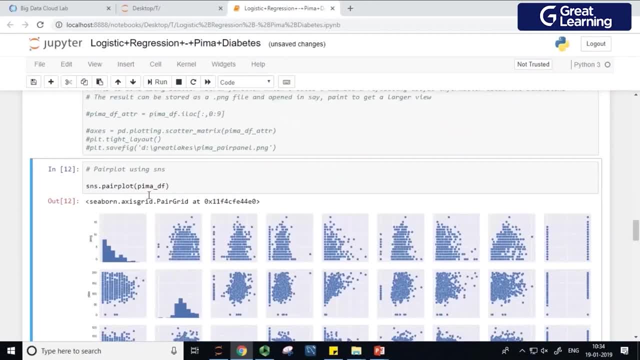 a few more minutes, But let me take a few more minutes, skip my time and we will be done with the class this. I am going to come straight to this, where I am going to say: SNS pair plot comma, dag, underscore. kind is equal to KDE kernel density estimate. Since these are numerical values, 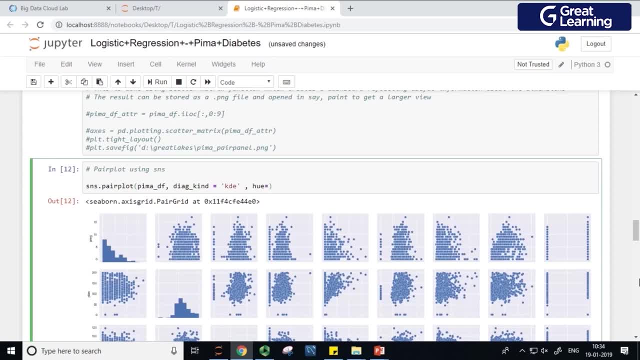 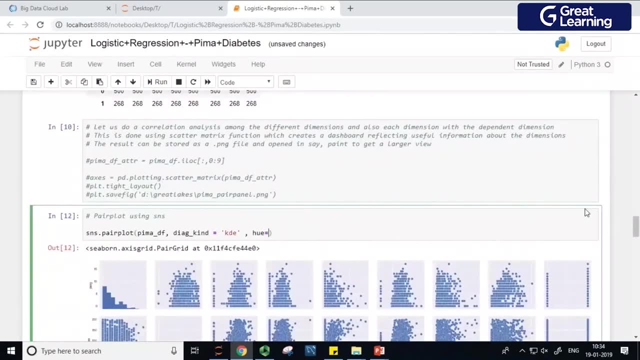 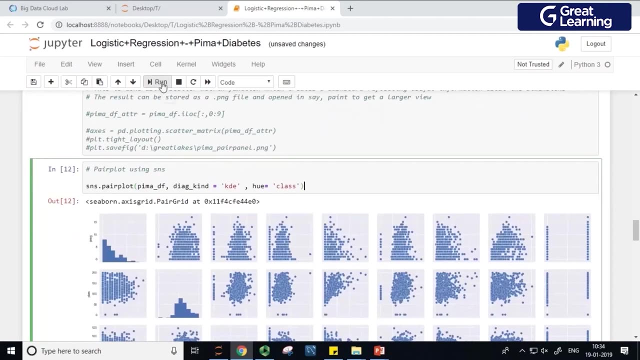 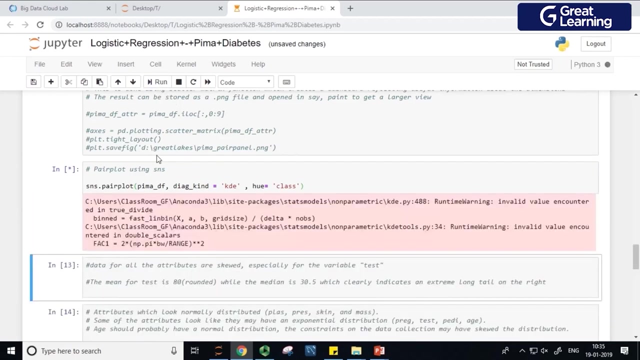 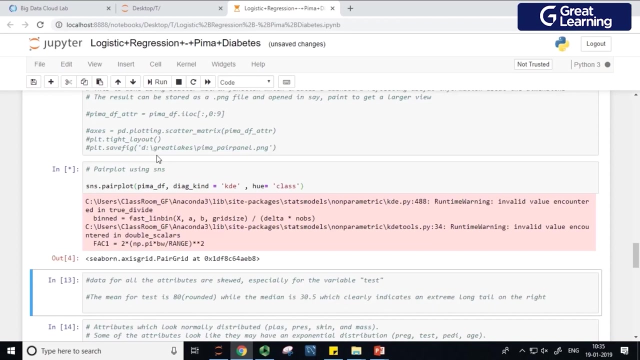 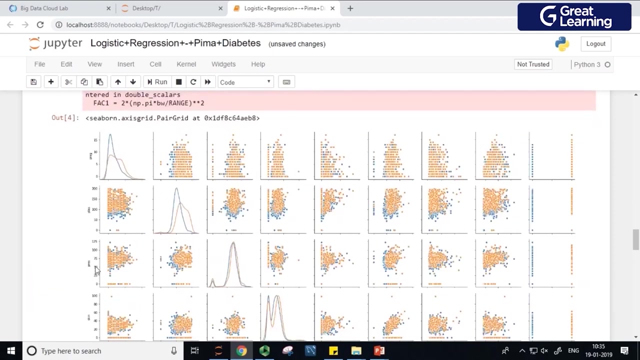 it makes sense to have this and hue- hue means color- is equal to the last one, what we call it target class. So hue is equal to class. yeah, on the raw data, it will take some time. let us fast actually. Yeah, there you go. Now let us understand this pair plot. All of you have it. Let us. 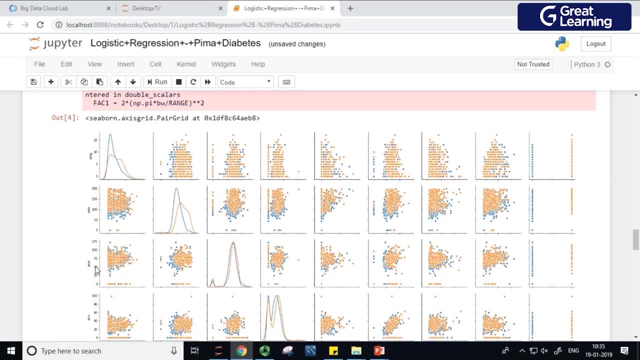 look at the very first dimension. The first dimension here is pregnancy reported. ok, The blue is non-diabetic class and the red one is the diabetic class. orange is the diabetic class. If you look at it, the two distributions are overlapping with the central values. They 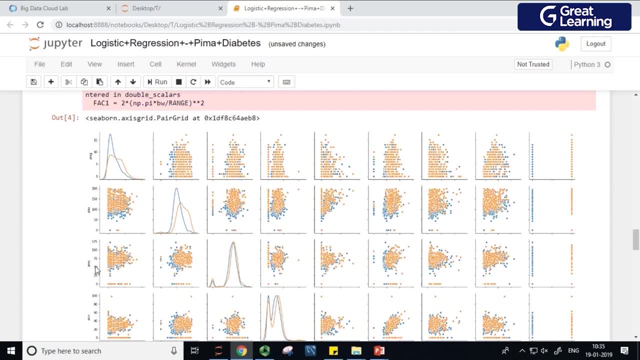 are overlapping Very small separation over here. Come to the next dimension. The next dimension is your plasma Plasma. you see long tails on the left side with a small bump. This is the route layers, the zero values, But otherwise the blue classes perfectly looks like almost like a normal curve, and the central values. 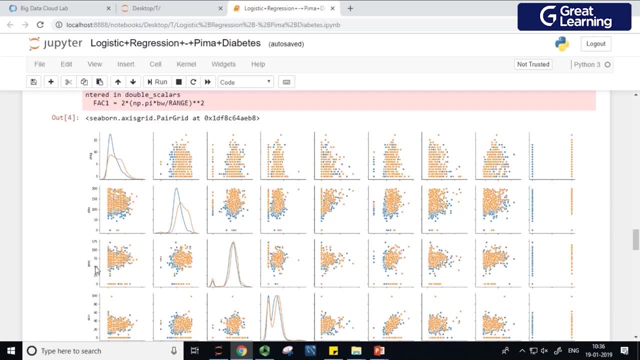 are overlapping. The central values are eclipsed. So once again, not a very good attribute, but at least we have some differentiator here. Look at this one: Even the outliers are overlapping. This is your blood pressure. These are the zero blood pressure cases. kanji for radiation: These are the zero blood pressure cases. The 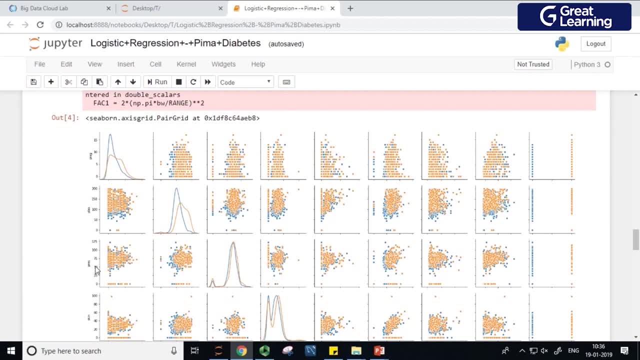 They are also overlapping. yeah, So there is no way your blood pressure will be able to separate out. based on blood pressure, you cannot distinguish diabetic versus non-diabetic. There is no way, you know. But if you correct those zero values, 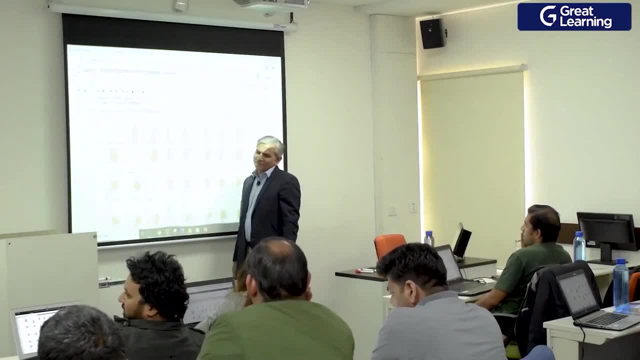 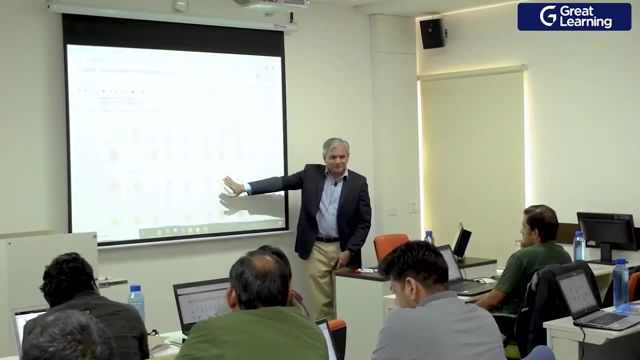 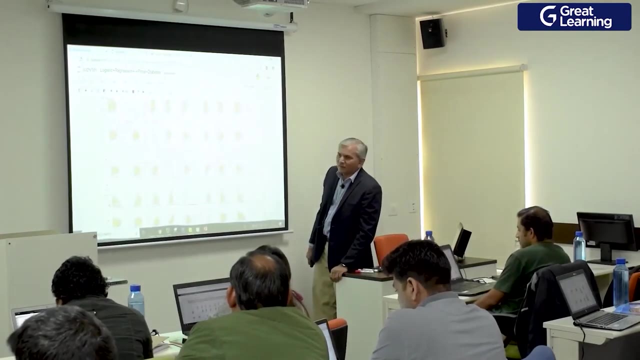 Still correct. Whatever technique you apply will be same technique, So both of them will shift together. right, So we have problem there. Look at the next one. This is even surprising: Almost gone. skin color, skin, not skin color. this is skin fold, yeah, You. 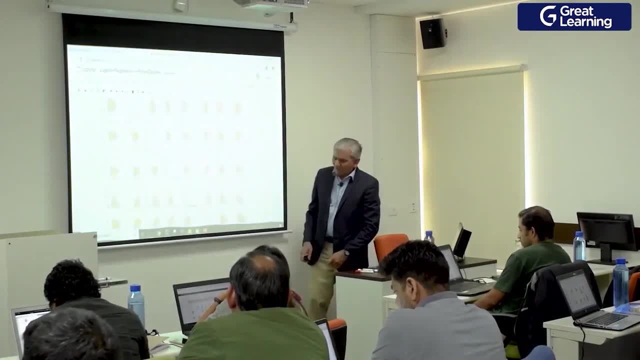 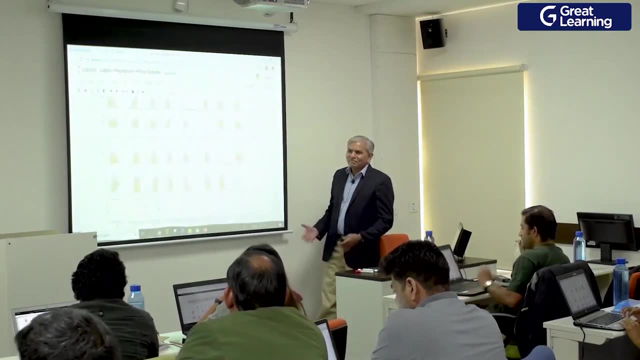 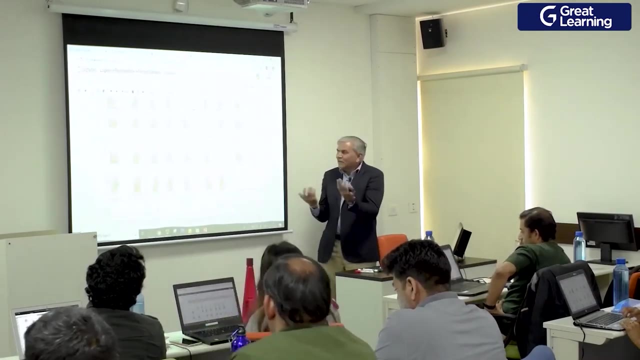 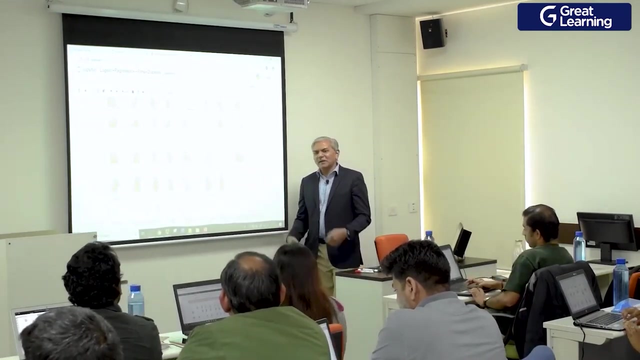 see the same problem here also. Every dimension, you look at it, every dimension- has this problem On none of the dimensions, except for a few dimensions where you see small difference in the two classes. none of the dimensions are separating the two classes. So even if you put all these dimensions together and build a model, you are not going. 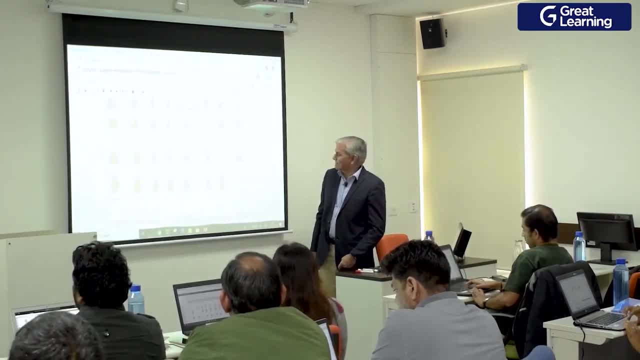 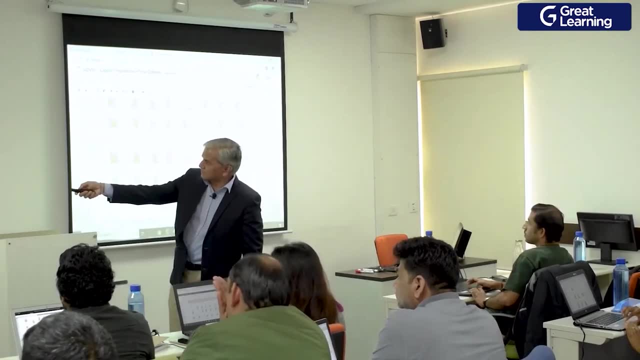 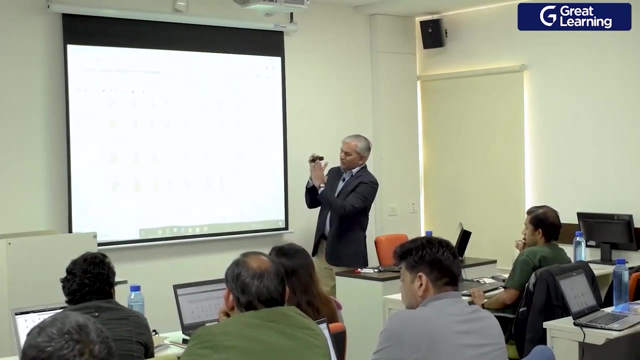 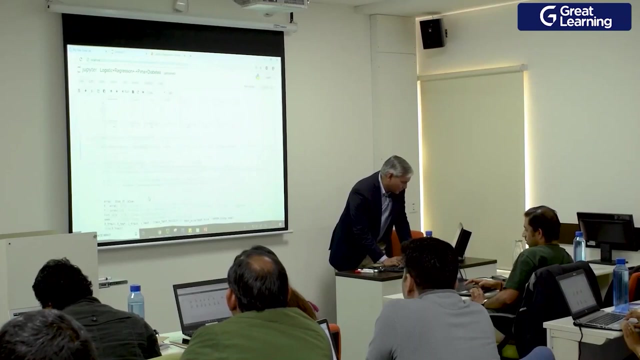 to have any problem. Yeah, it is overlap almost. this case, the previous case, this one, And that is what you are seeing here. The two classes are overlapping on every. they are not shifted like this. Let us go ahead and build a model. Let us not be very hopeful. 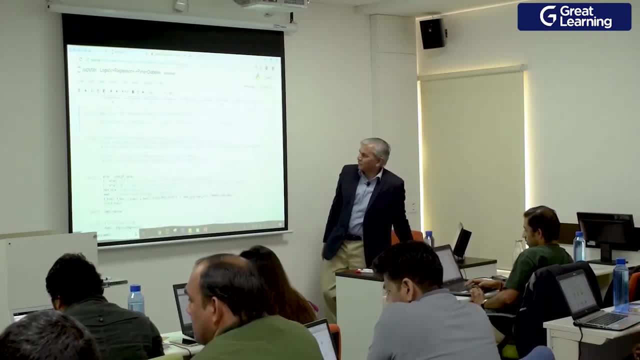 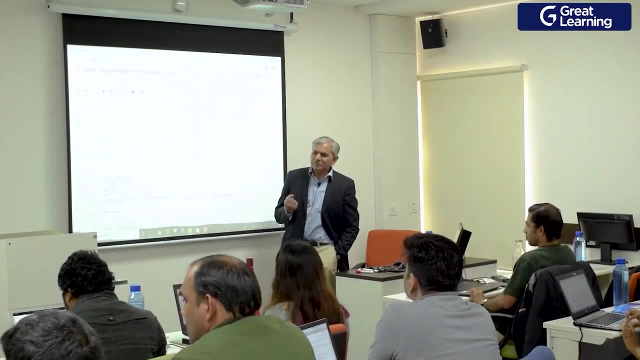 about this. Any model will give a problem here. So what I am doing here is: this is not required. it is not required to be done. All algorithms can take as input the data frame itself, But earlier I used to do this as a practice, where I am converting the data. 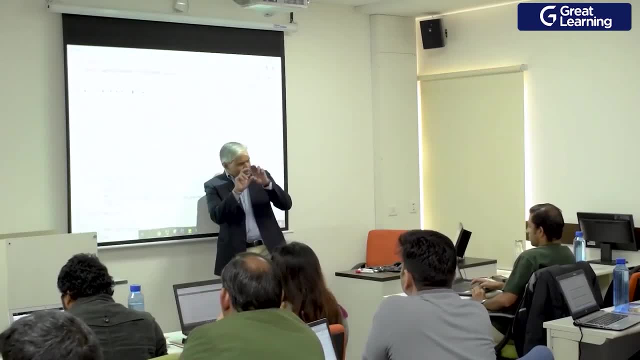 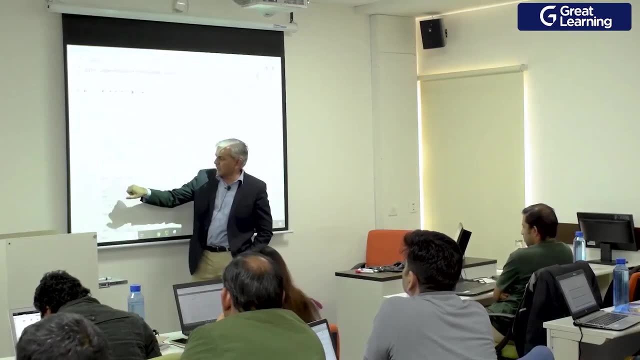 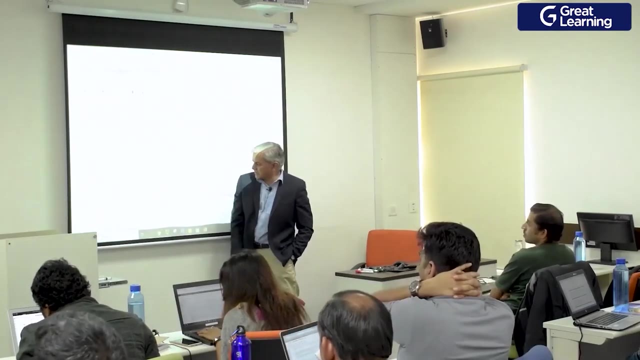 frame into an array. So data frame minus the column headers is called an array. ok, And that array. I am taking the independent attributes into x and dependent attribute in y. Ok, And then I am splitting this x and y into train set, test set. Is this part ok with? 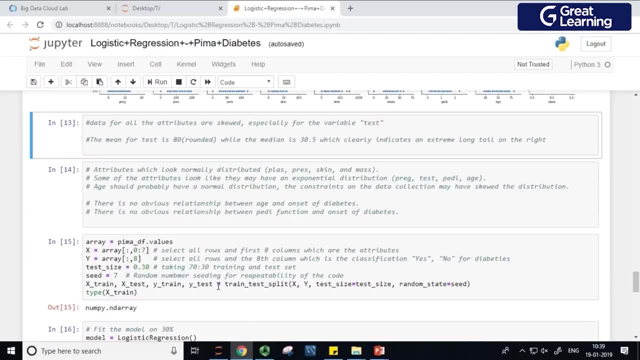 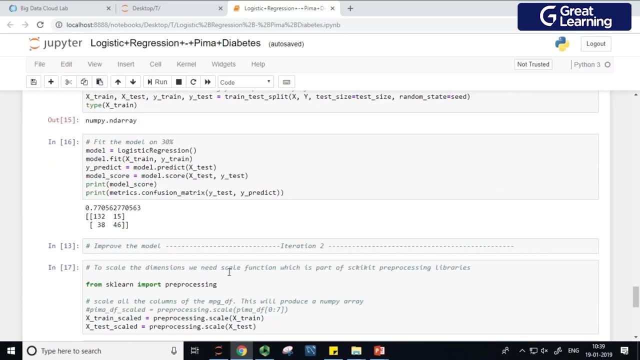 you people, All of you with me on this, All of you side arm, You are also on this. Great Now look at this. I am instantiating the logistic regression model. You can call it anything you like. I am calling it model. I am doing the fit. This is where the best fit line is. 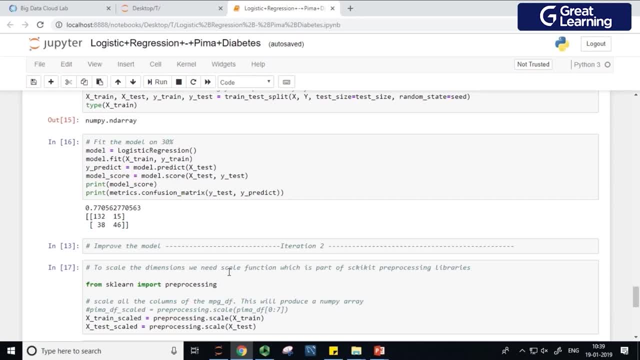 found and convert into your sigmoid curve The fit. Once the model has been found, then I make use of the predict function of that object on test. So these are my predicted labels: diabetic, non-diabetic. The actual labels are y tests. ok, There are some people get confused here, So I am going to stop. 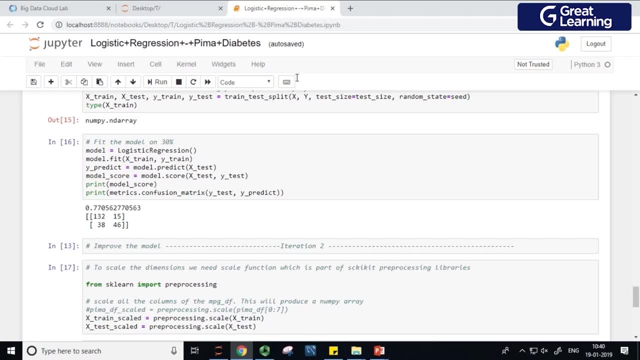 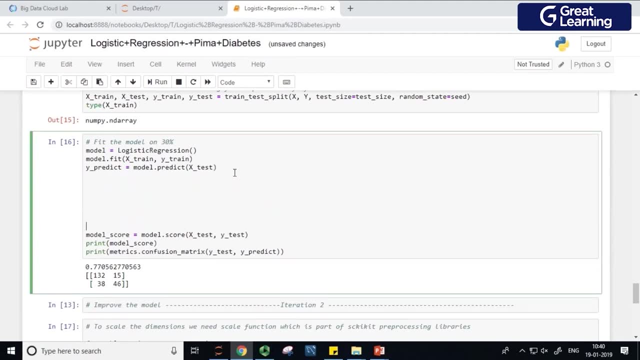 it. Do not look beyond this, Just stop it. I am asking you to just look at this. It is at this part, till this point, everything is fine. ok, Now, what I can do down is: I can. for the time being, I will remove this. ok, I will put a yeah. for the time being, just ignore. 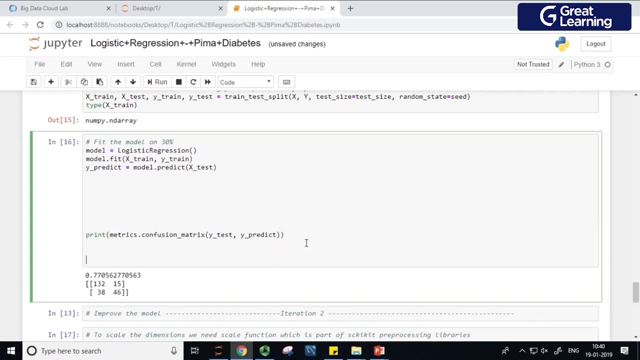 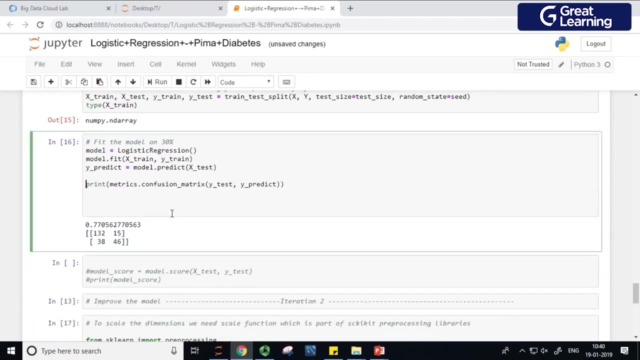 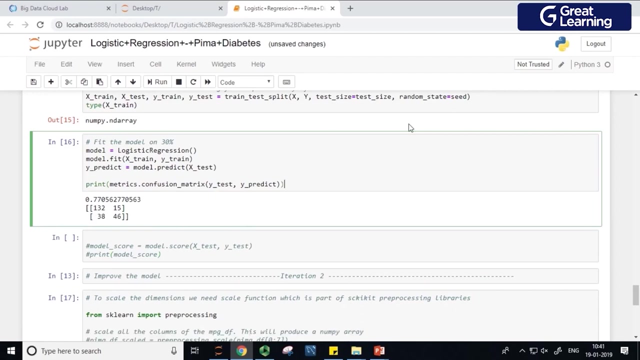 this control x. we will put it over here. insert cell below and we will put it here. alright, I will uncommit it later. I will do that. ok, Now look at this. have you seen confusion matrix before? Yeah, Yeah, All of you agree, it is exactly what it is called. It confuses people a lot, right? confusion? 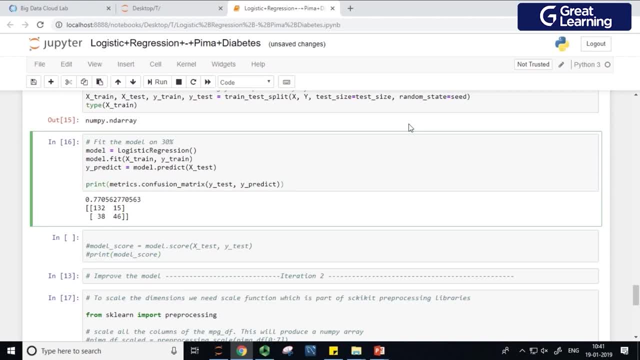 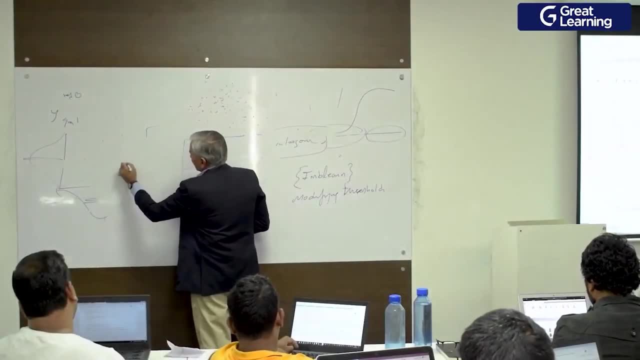 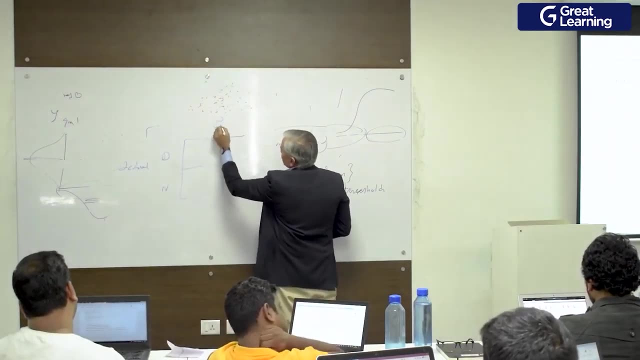 matrix. So what I do is, as a practice, when I make my confusion matrix, I always keep the actuals on this side- actual, diabetic, non-diabetic- and the predicted, the output of the model on this side- diabetic, non-diabetic. This is my practice. you can follow the other way, but 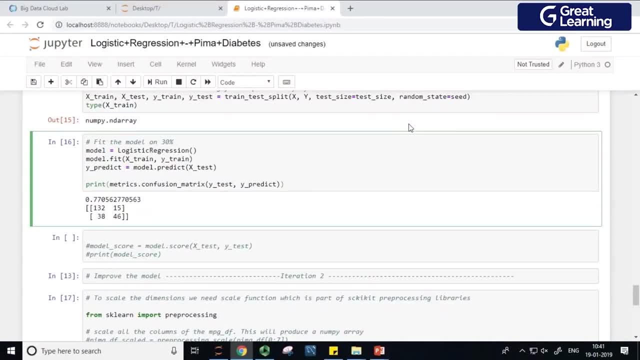 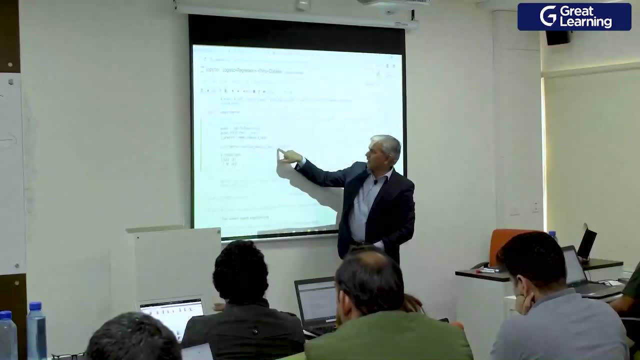 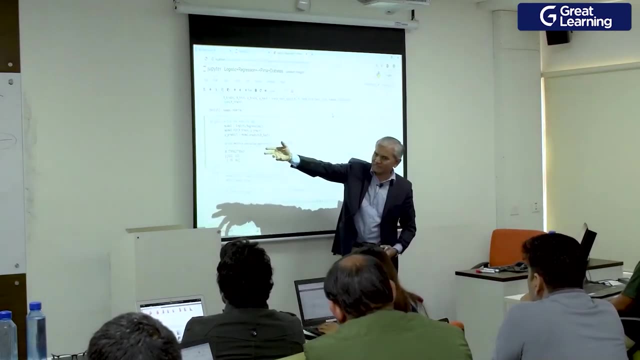 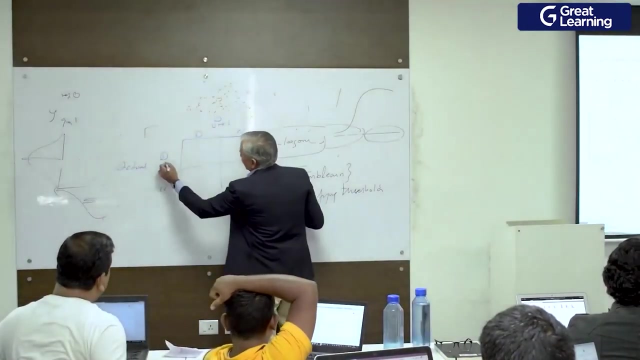 the way you follow, only one. How do you control this? Since, again, why test first? this is actual. it goes to the rose Y predict next. this is say the predicted values goes into the columns. If you flip this, you will flip that. Now what it is saying is, of the device, diabetic cases in your sorry, this. 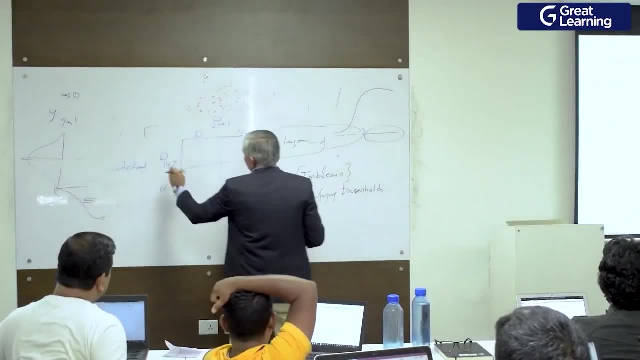 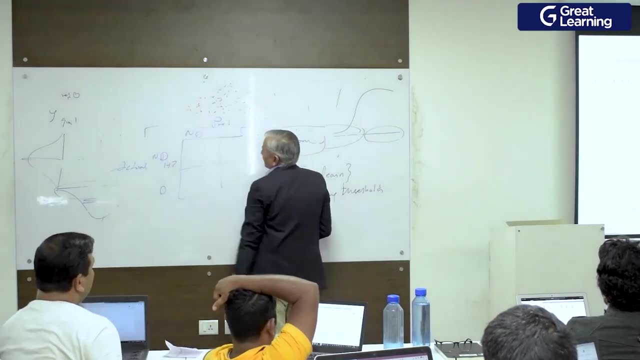 is non diabetic. non diabetic: this is ND. Yeah, Yeah, what are the definitions? They all give a lot of便用. Yeah, exactly, Oh, yeah, Ok, So we will analyze them, else is it grow further? Okay, non-diabetic: this is diabetic NDD. If you go and read the source of the data, they are: 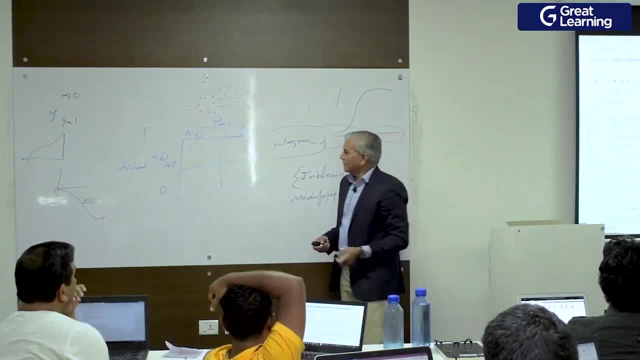 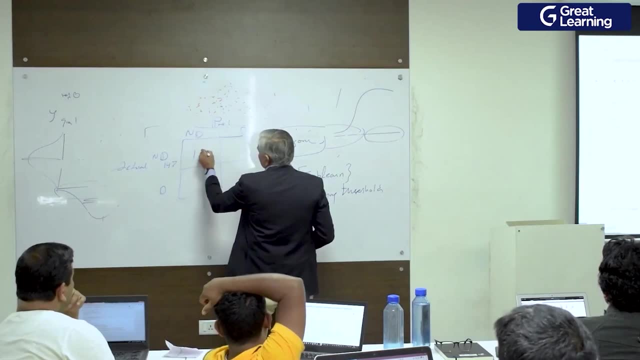 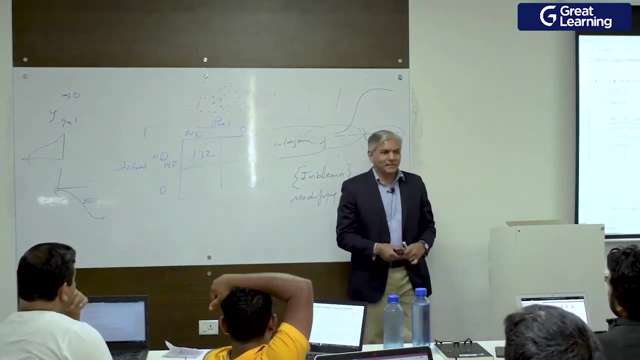 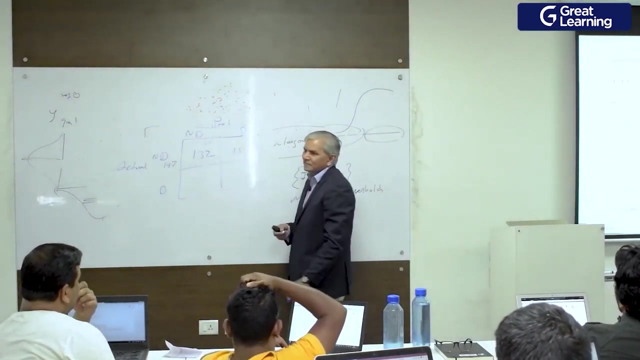 very clearly told: 0 is non-diabetic, 1 is diabetic. Of the 147 non-diabetic in your test data, 132 have been classified as non-diabetic. No mistakes For this. class 2 positives Of the 147, 15 have been identified as diabetic- Incorrect classification. These are those. 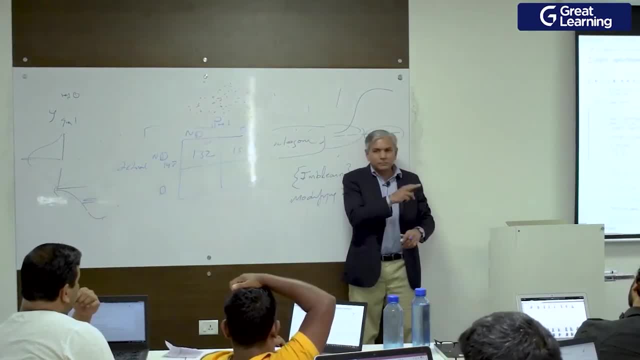 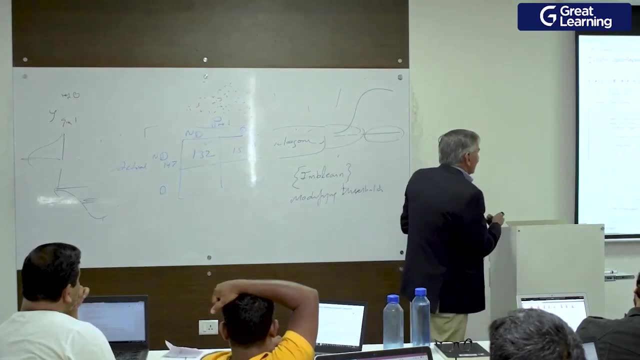 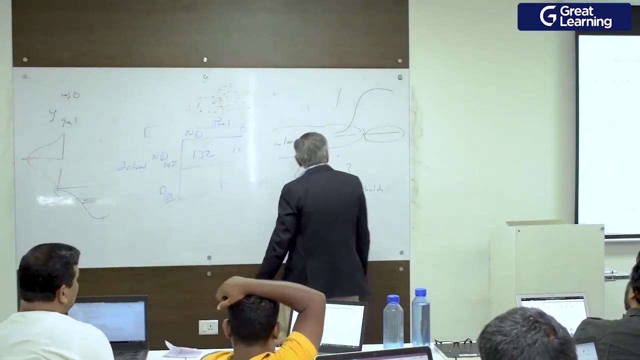 values of red lying on the extreme end, values of blue lying on the extreme end. Look at the diabetic class 84.. There are 84 diabetic cases in your test data. Of this 84, 46 have been correctly classified as diabetic. 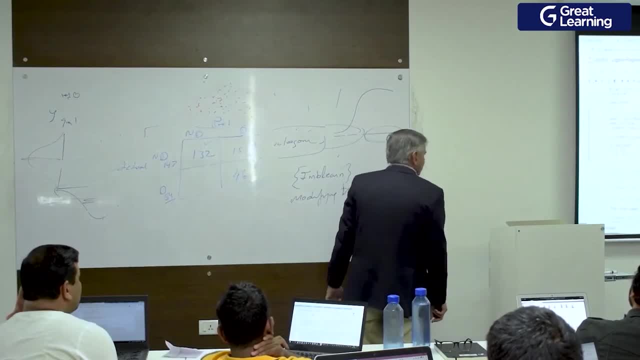 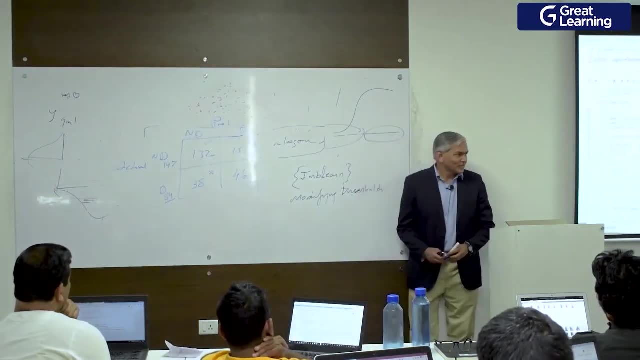 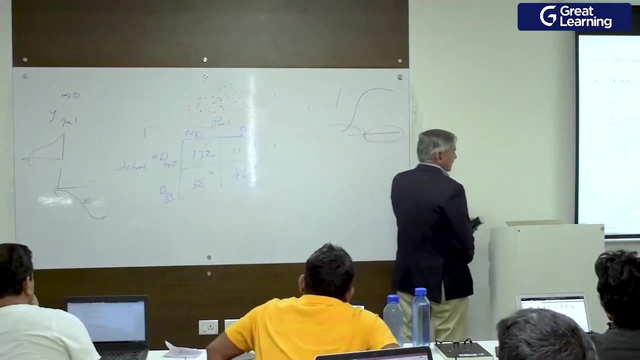 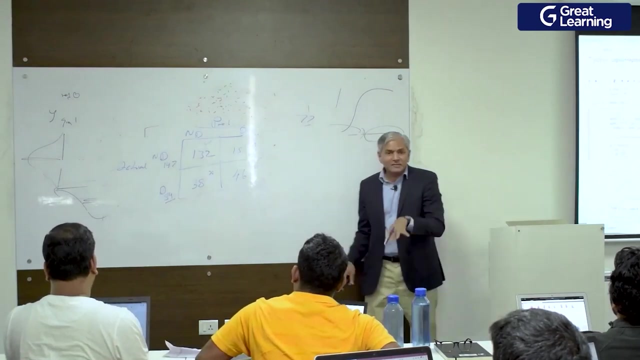 84 minus 46 is 38.. 38 have been misclassified. Now look at this. Now look at this. What is the overall accuracy? 77 percent Looks decent, But let us look at accuracy in diabetic class. We call it recall. 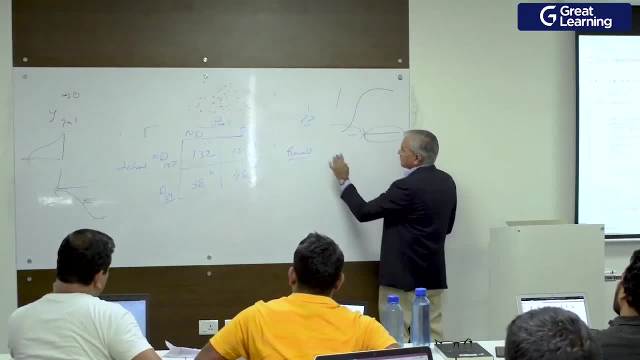 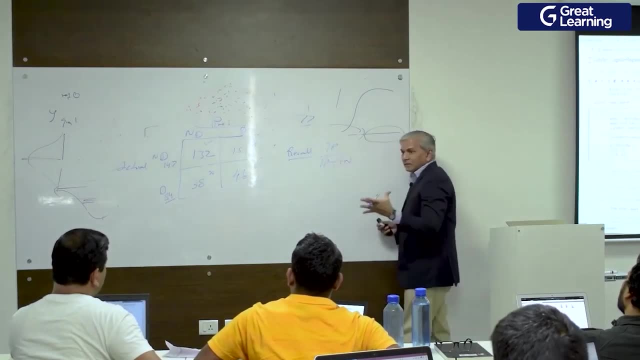 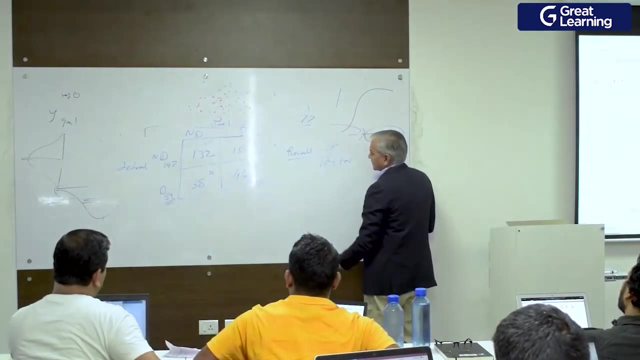 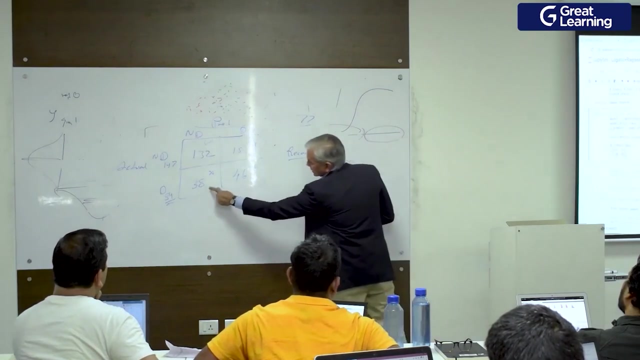 Recall is. the formula for recall is true positives by true positives plus false negatives. Looks very high-fied, But what it means is true positives divided by row total. So the recall is 46 divided by true positives plus false negatives. This is false negatives. 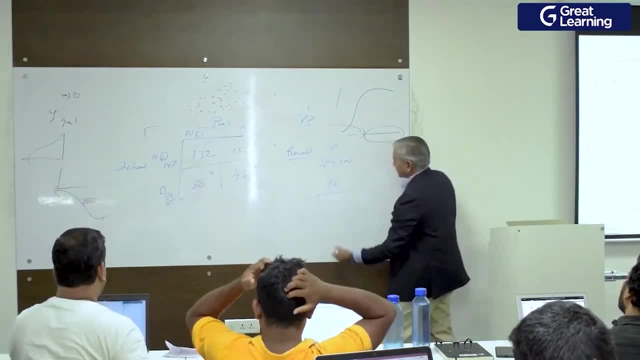 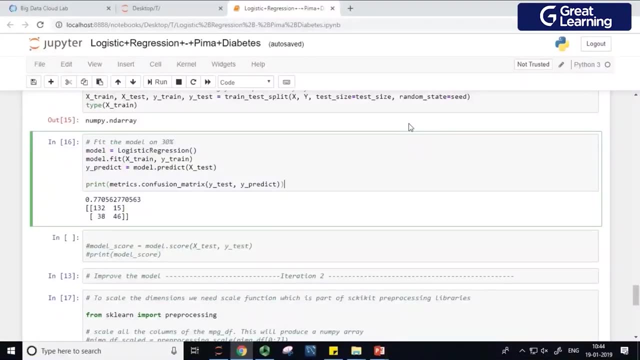 For this class. this is false, negative, Right? Ok, So yeah, So it is 46 plus 38 back to 84. That comes to around 55 percent, right? It is coming by 55, 54 percent, right? That is like tossing a coin heads or tails, You do. 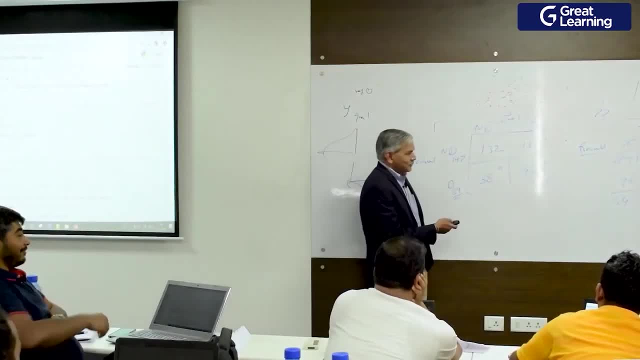 not need a model for this right. So to get this kind of accuracy, you do not need a model. You can just toss a coin and say diabetic, non-diabetic. That is what this is. So this is what this is. 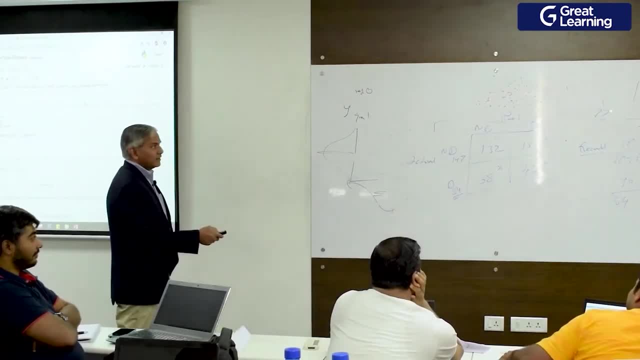 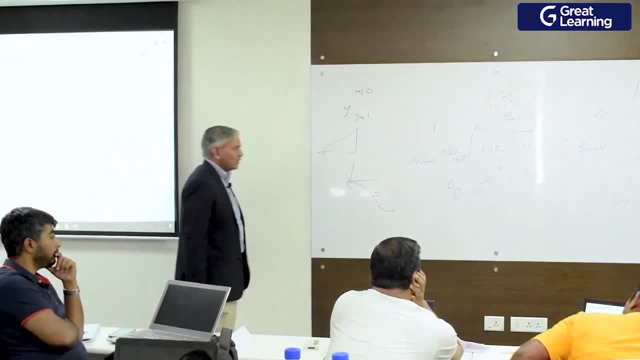 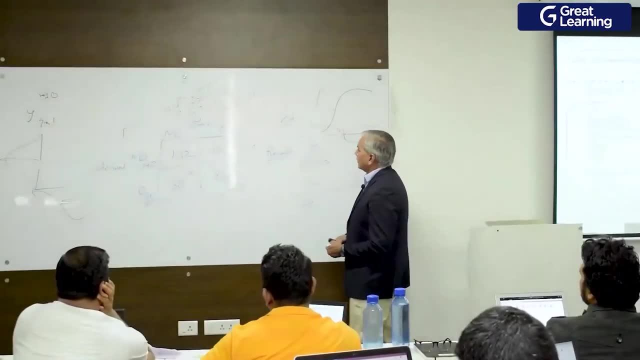 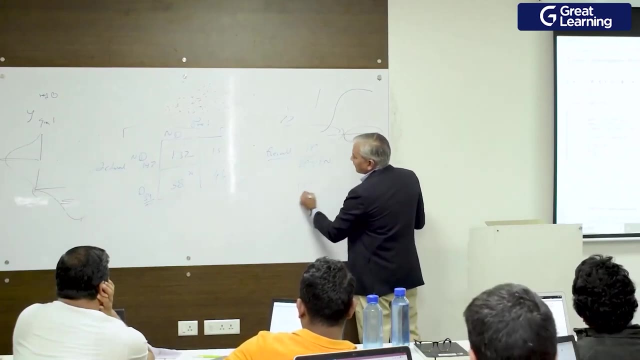 is what we expected, because this is represented very poorly. the diabetic class: This is important for us. Look at the recall for the non-diabetic class. Non-diabetic class: the recall is 132 by 147.. This will come very high: 90 percent, 80 percent, 90 percent roughly. 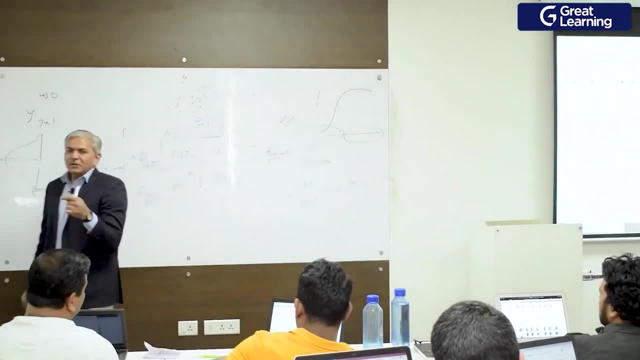 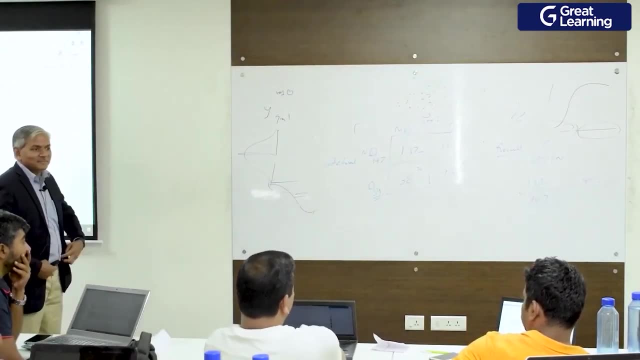 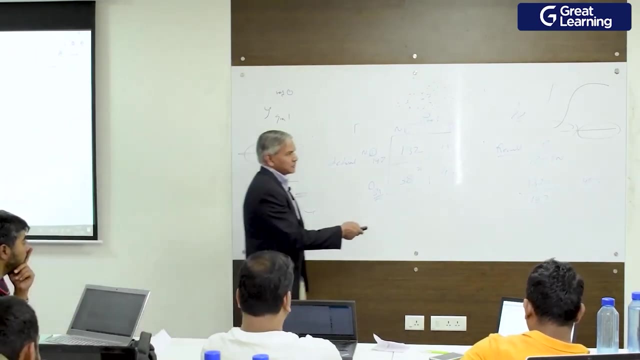 around. So the recall for the non-diabetic class is very high. Recall for the diabetic class is extremely poor. but that is what you should expect. We wanted the reverse, We wanted the reverse. So that is what will happen when you have situations like this. 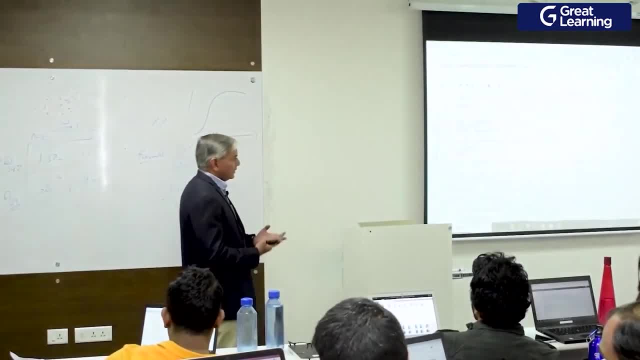 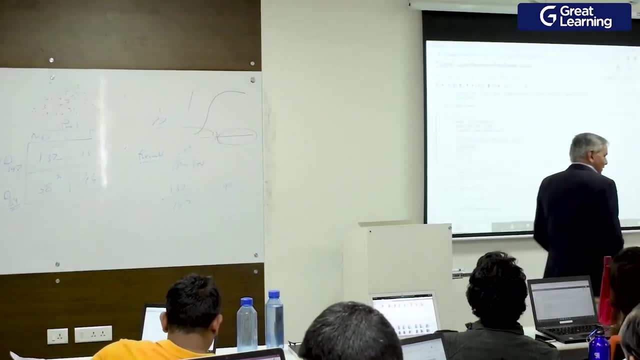 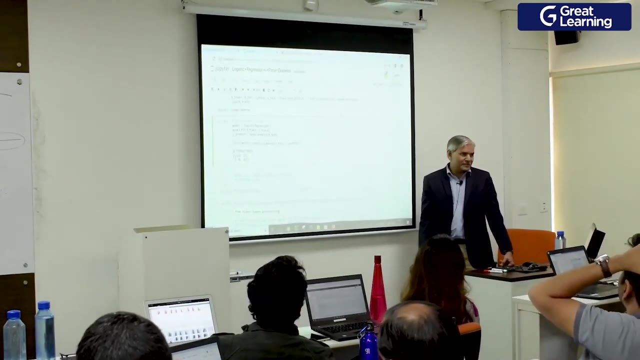 Ok. There is no way you can get a very good model when the individual attributes are poor attributes and the classes are underrepresented. You cannot do it. So the magic happens in the data. How do you prepare your data for analytics? That is where the magic is It. 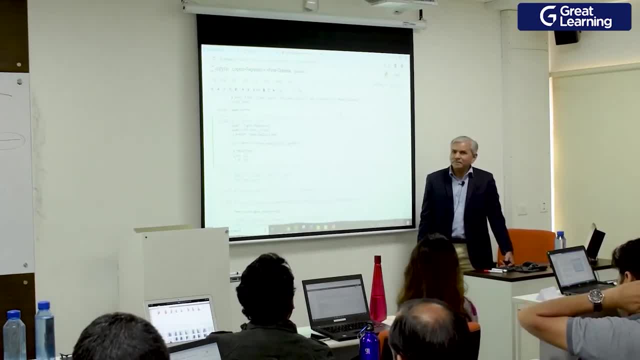 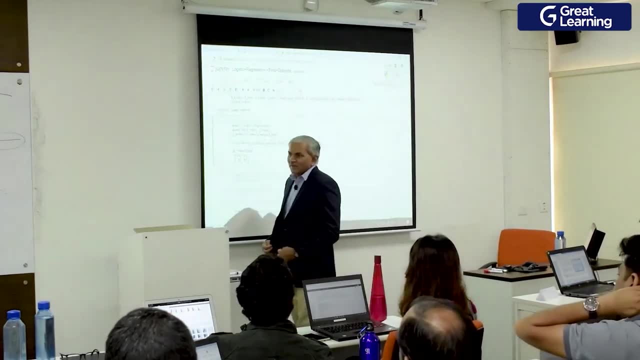 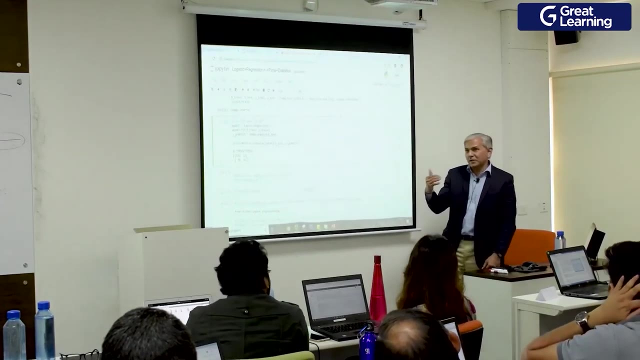 is not in the algorithms. Ok, It depends on data preparation. 80 percent of our project estimated effort in data science goes into preparing the data. Running the algorithm is not. then rest around 20,. 15 to 20 percent goes into fine tuning your model. It goes. 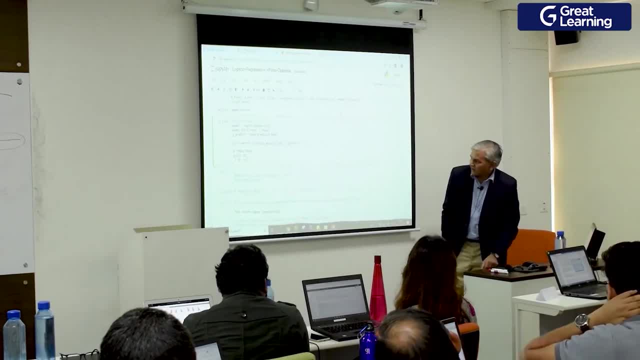 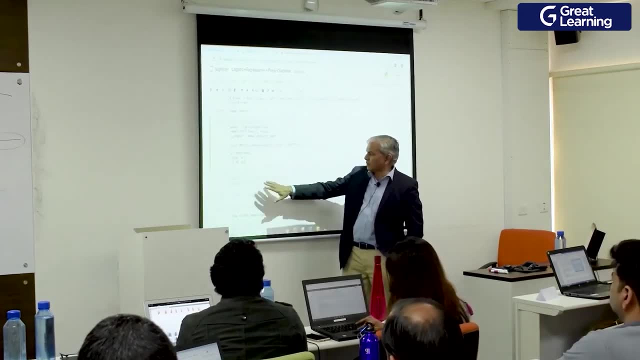 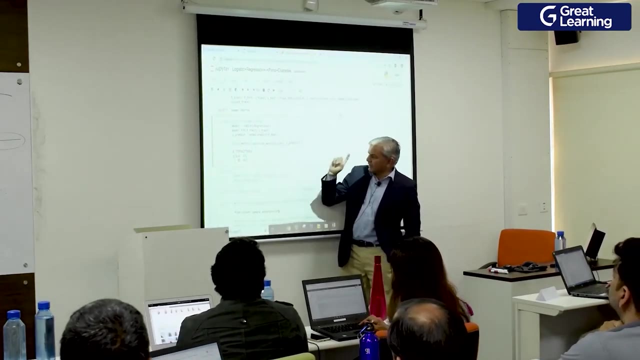 into that? All right, Let us do. there is a function called score. Instead of doing this, I can directly call score, but do not rely on this when you are doing classification. What this function does is it regenerates the model and then tests it on this test data. It regenerates. 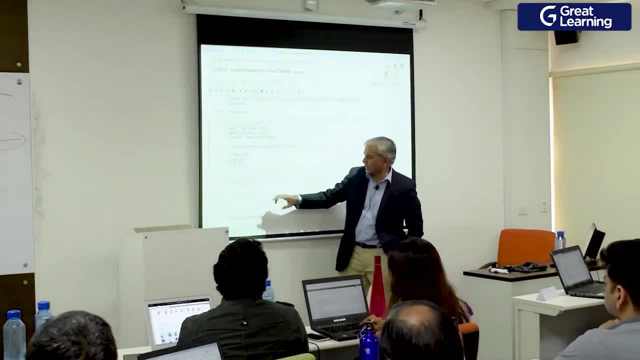 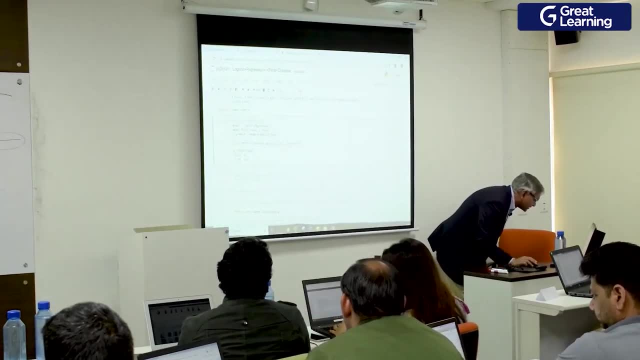 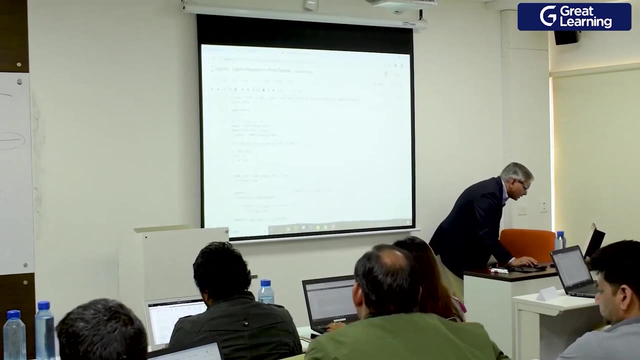 the model then compares the test data and this automatically and gives you the score Ok. So this has nothing to do with confusion. matrix, You can actually run this and say: remove the hash, run it, It will. it should give you. 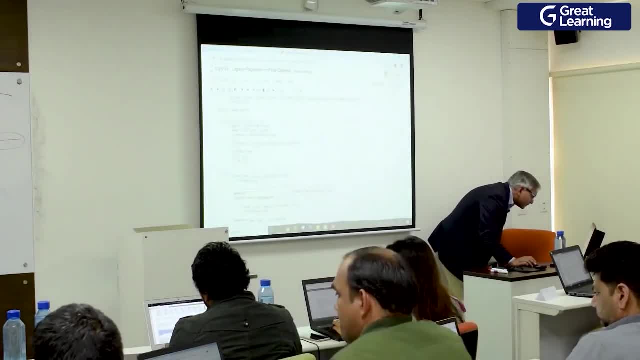 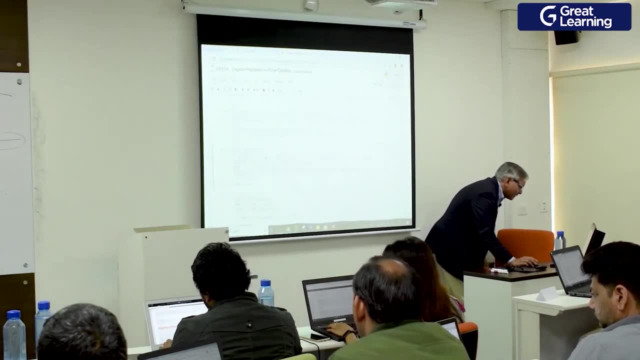 the score model is not defined. Why? What spelling mistake? Oh, I have not executed. I am just showing you this. Ok, I have not executed these lines. So it gives you overall score, but overall score is not defined. So this is the question. So you can actually. 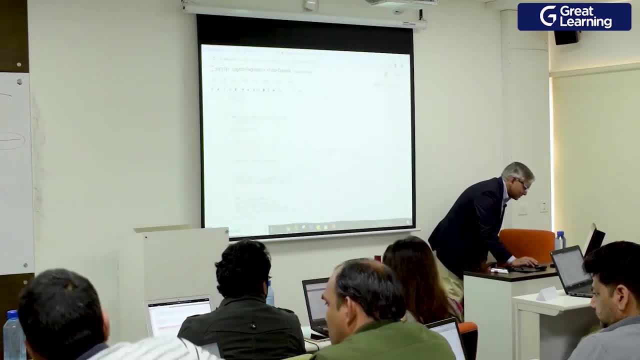 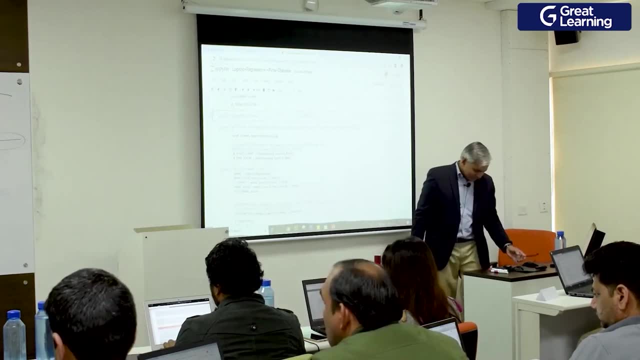 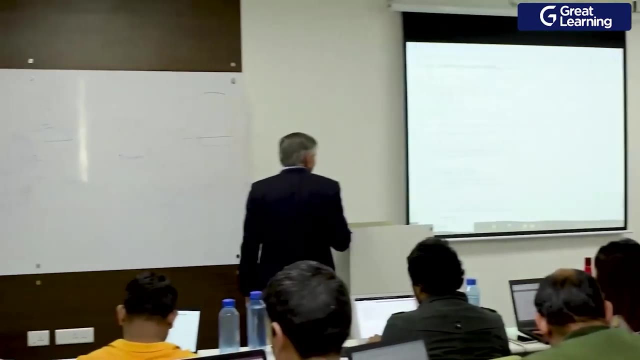 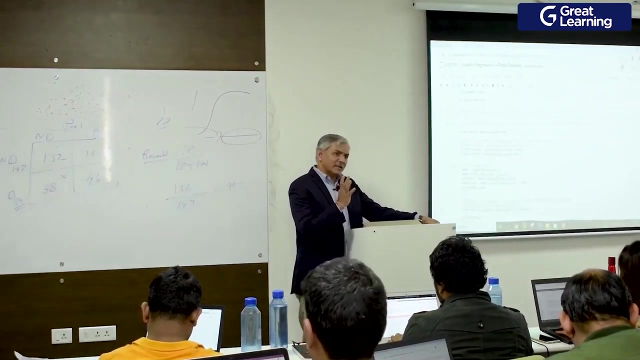 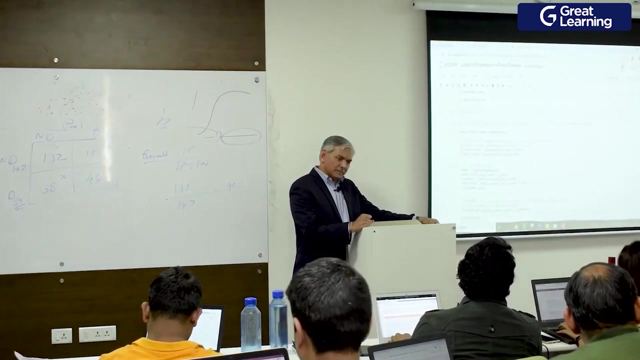 school is not reliable, so do not depend on this. Shall we move on. You need to learn the tricks of identifying good attributes, Feature engineering, feature selection, and that is where the core lies. 100 percent domain. If I want to predict the 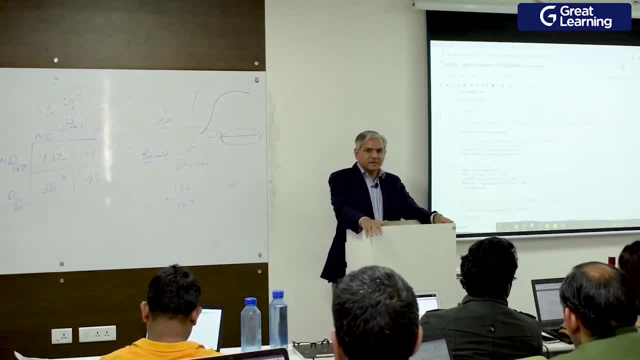 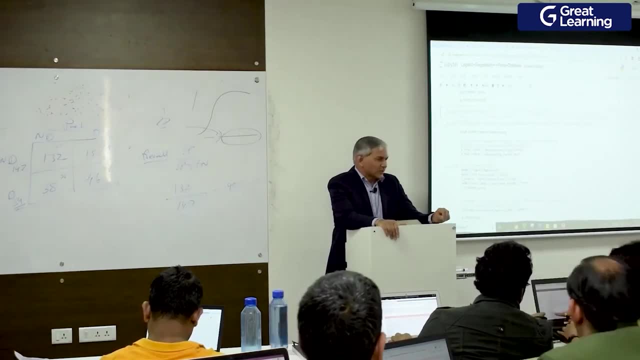 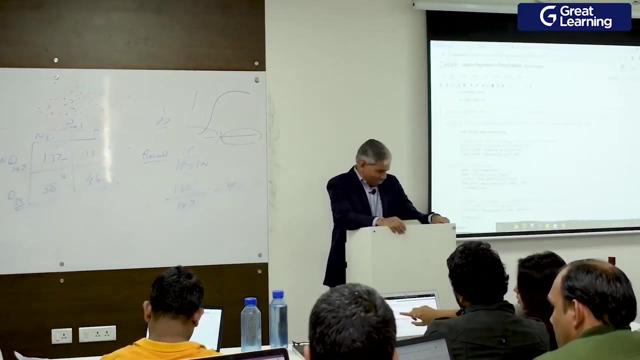 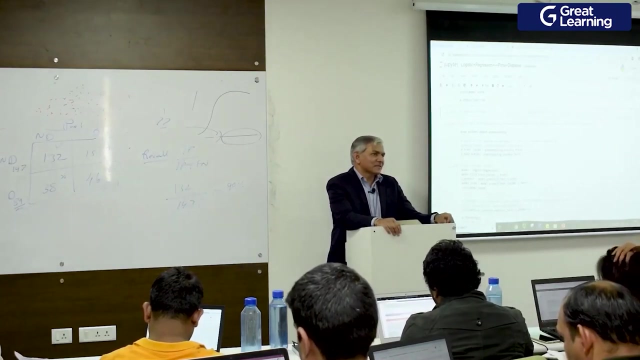 time taken to travel from A to B, then I should have the domain experience of what are the factors that can impact the time. That is what the attributes they collected are useless attributes. It is not good attribute. I do not know, I do not know, but the fact is it is not good data set for classification. 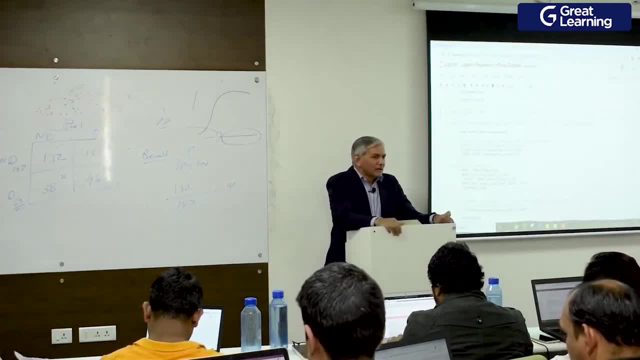 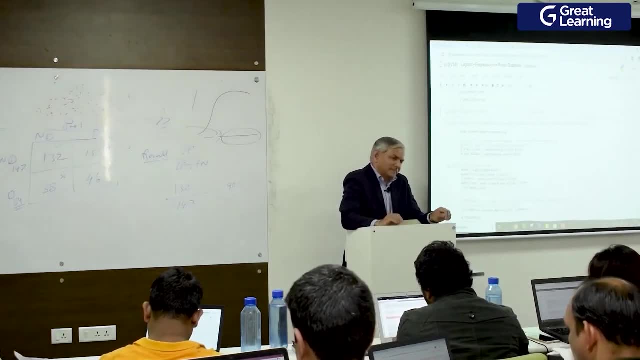 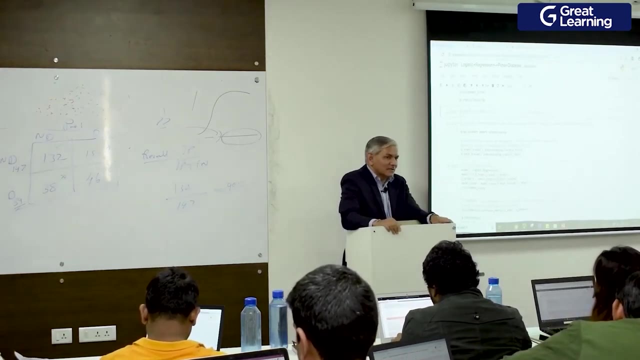 Non-data, Non-data. That is what this IMLN does: Upsampling. when you create upsampling, you create upsampling and you create upsampling. It actually creates synthetic data out of the underrepresented class. But is it acceptable to do that? 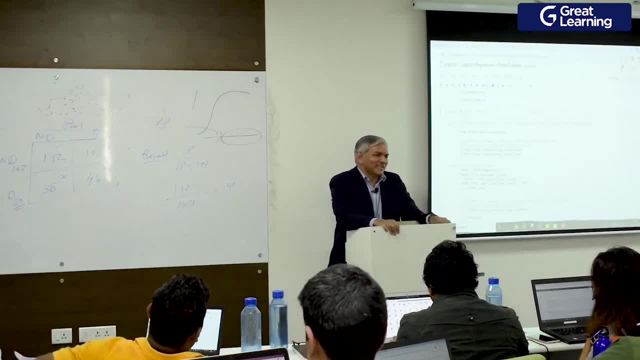 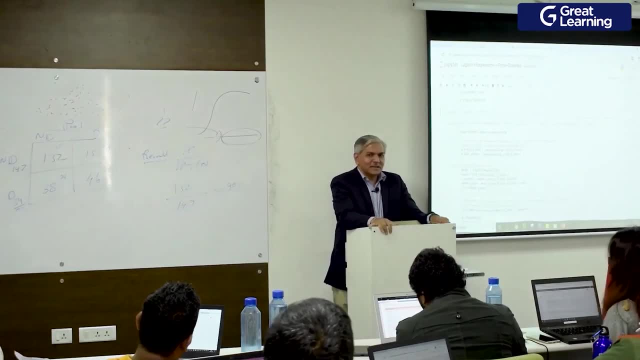 You have a choice. Are they acceptable? stay with us. No, no, I will tell you on a serious note, it is an acceptable practice. It is an acceptable practice. Finally, what is important to me is the models should generalize in production. That is important. 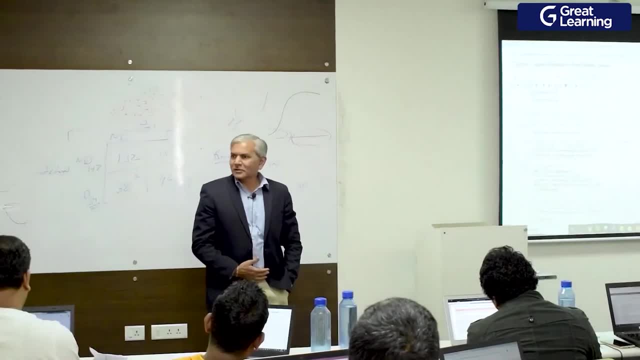 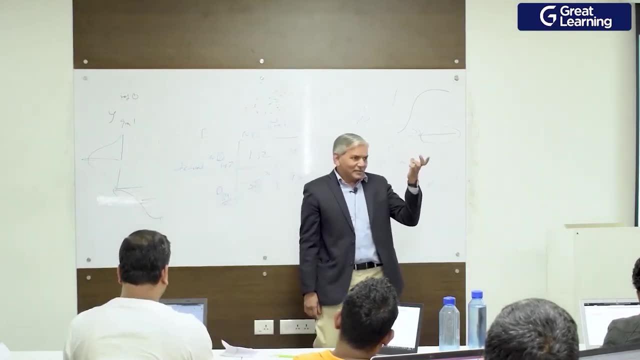 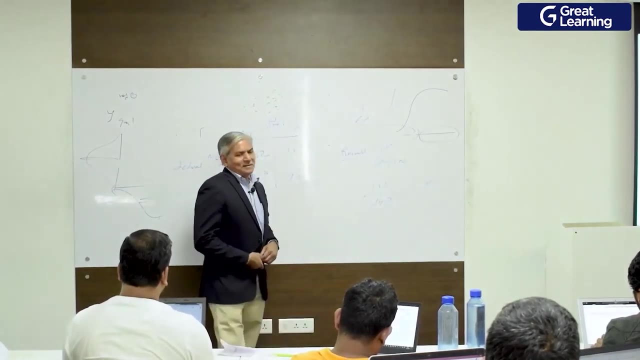 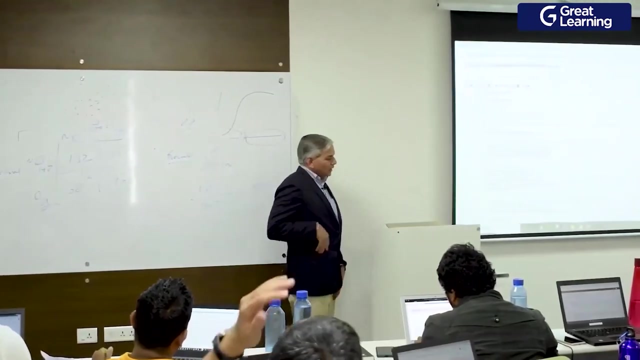 to me Ok into production. the models are not immediately used in production. they are put into alpha test, beta test. If, after jacking up the data, if the model is performing poorly in the alpha and beta, I will not release it. it is allowed. see, I will tell you quickly what happens in. 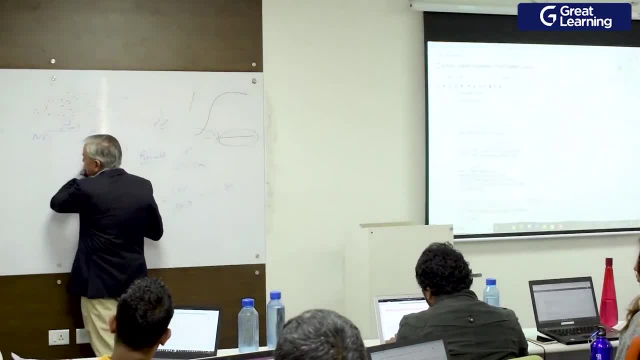 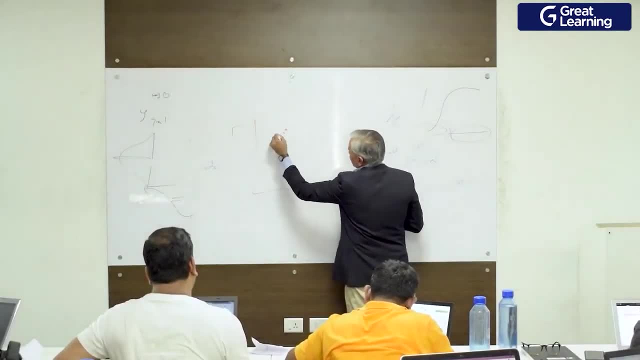 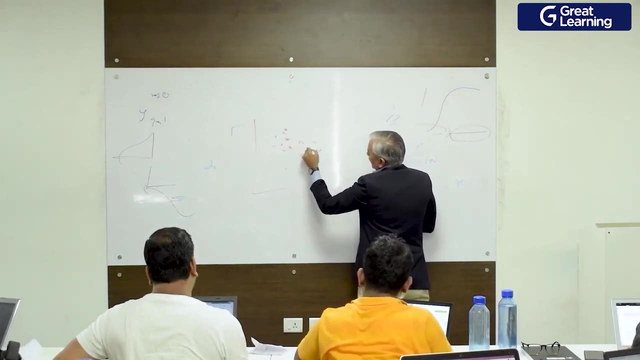 upsampling okay. Upsampling uses k nearest neighbors. So what upsampling does is, if you have two classes- this is underrepresented class- say diabetic class, triangles and non-diabetic. most of them will be non-diabetic. okay, And there is some overlap here. okay, most of. 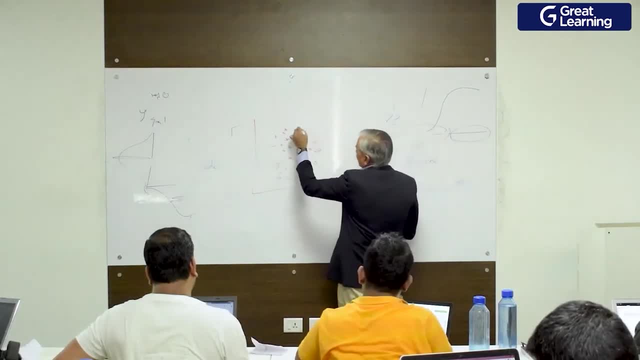 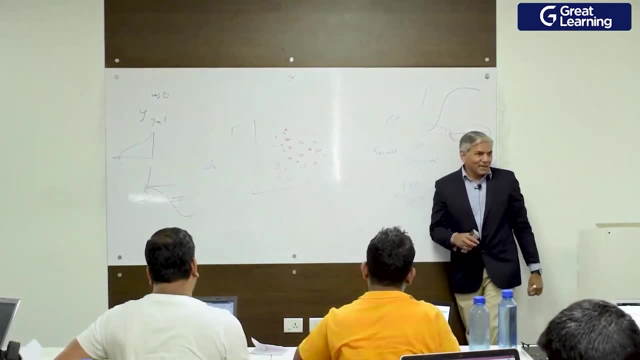 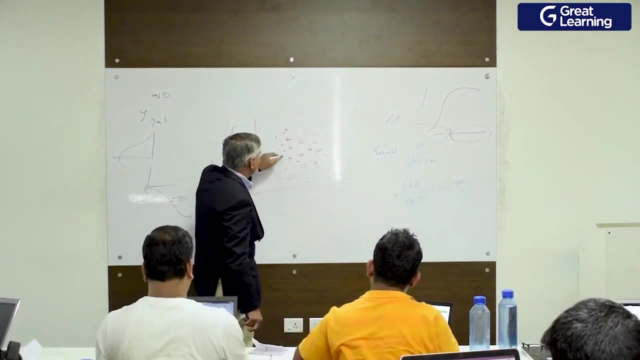 them are non-diabetic class. What this upsampling using Imblern does is it tries to generate synthetic data out of this. Just one thing, let me finish this. The synthetic data generated is such that it does not disturb this overlap region. It creates synthetic data in these regions. 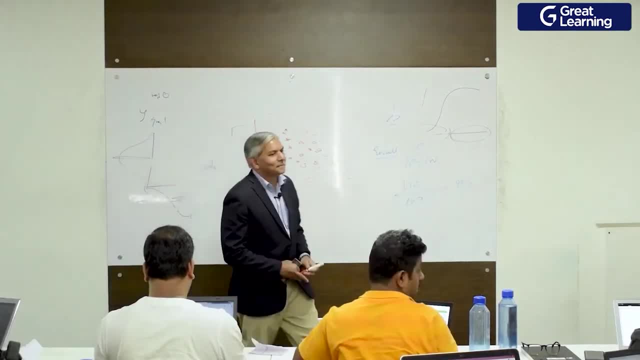 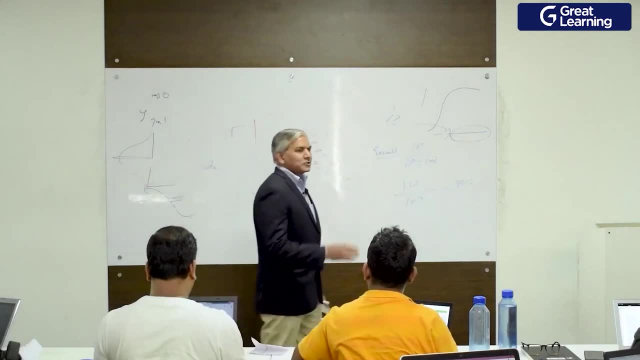 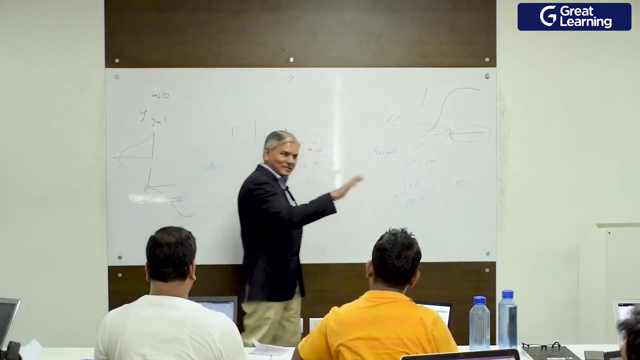 Yes, but by doing the upsampling are we not introducing the bias error? 100 percent guaranteed? So we are. by introducing the bias error, we are taking away the bias in the algorithm which is towards the higher class. We are trying to cancel that bias error. 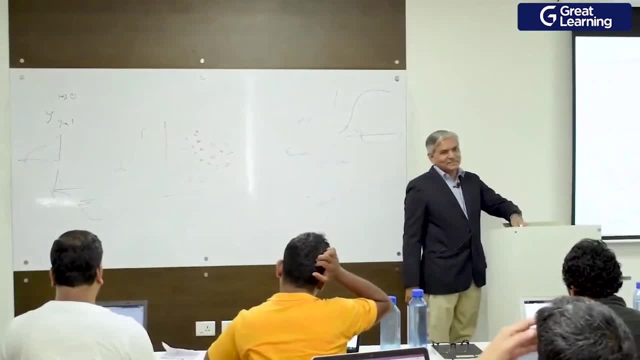 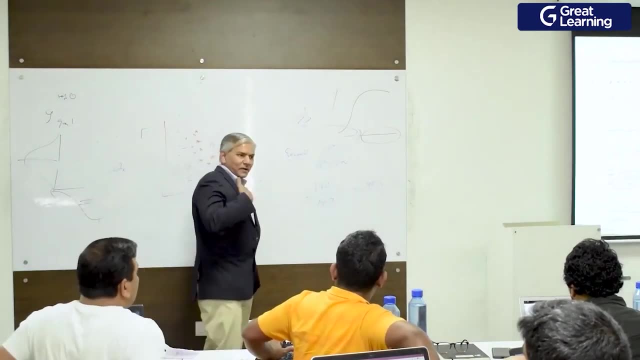 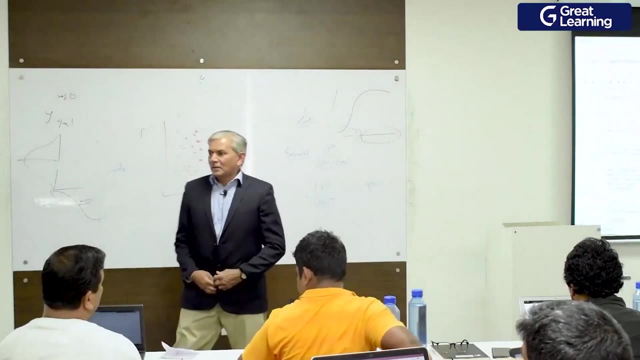 by upsampling. So actually upsampling and downsampling is adjusting the bias Correct? We are actually trading the bias. We are trading off the bias which exists naturally in the algorithm towards higher class. Sir, are they exact duplicates or No? no, they are not duplicates. That synthetic data generated using k nearest neighbors. so 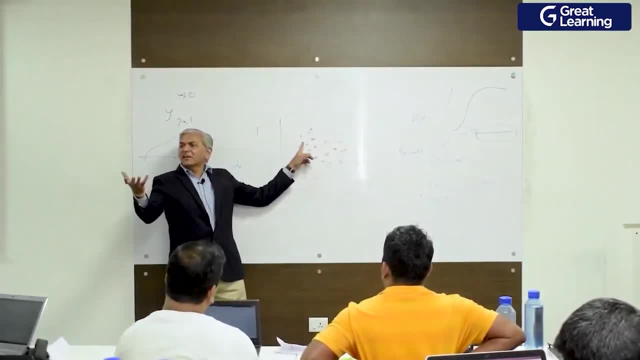 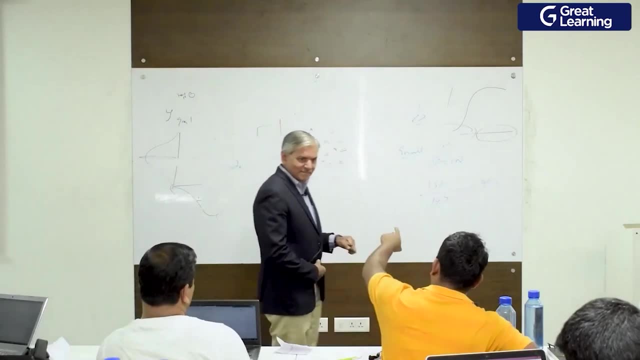 I take a random point here. then k nearest neighbors. if you use k nearest regressor, for example, it will sum up these three and give you the average. Okay, In this case, if you use k nearest to all the stars, will it not surface? 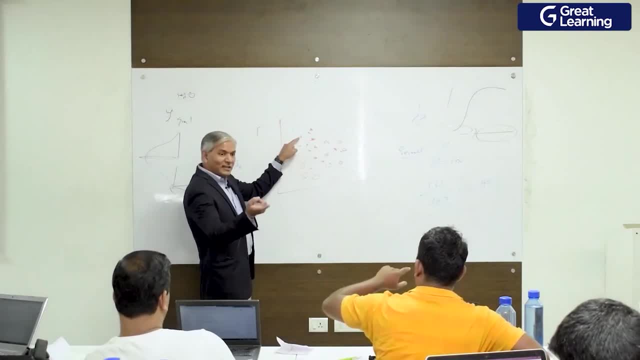 No, all the stars. but what it will do is it is k nearest regressor. Okay, So it is going to take the blood pressure of all three, find out the average, give the average to this new point. Okay, So that can be surface. 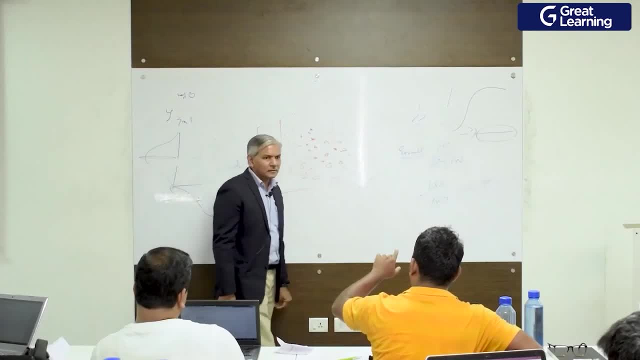 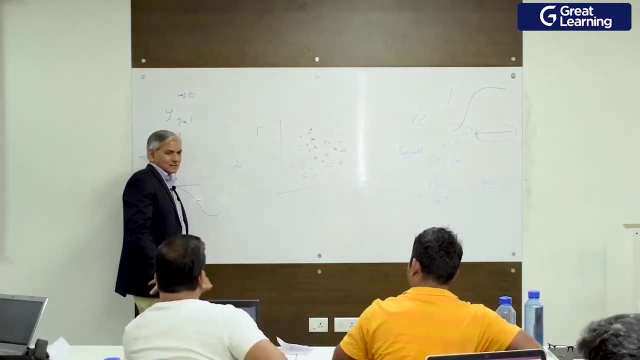 That can be, That can be. So there are two class words, star and circle. So you know It works only on the underrepresented class. It generates synthetic data only for the lower case. So in this case it will generate synthetic data only for the diabetic class. 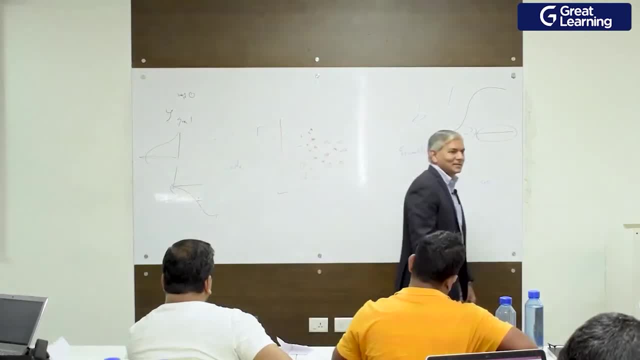 Sir, in this case, if you sample our data at what point we should stop like it will bring both the samples to the same level: 50-50.. 50-50.. It will bring it to 50-50.. 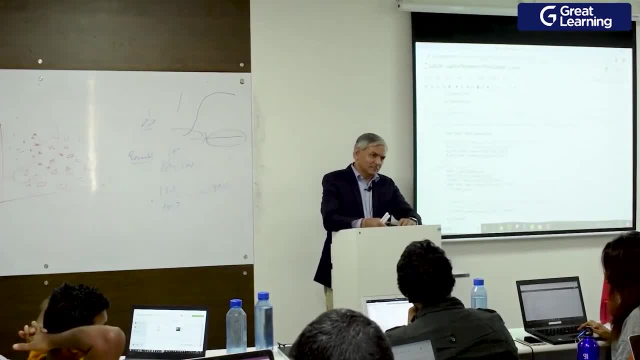 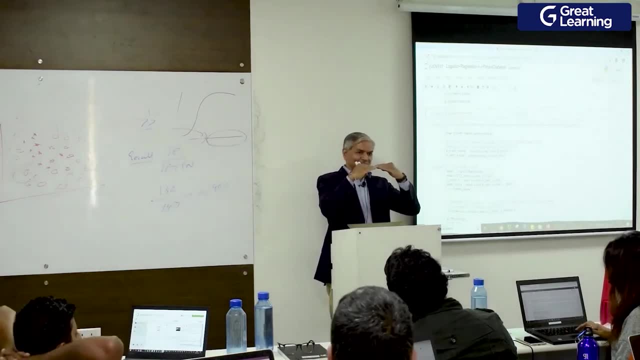 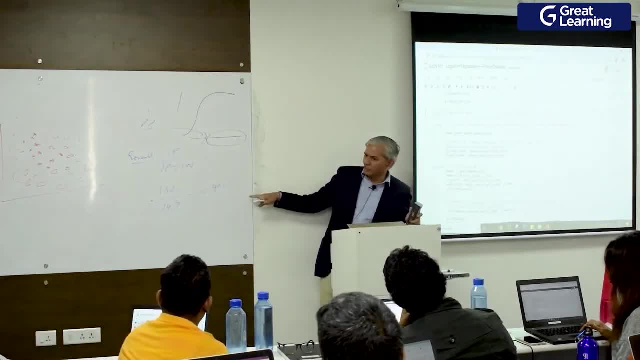 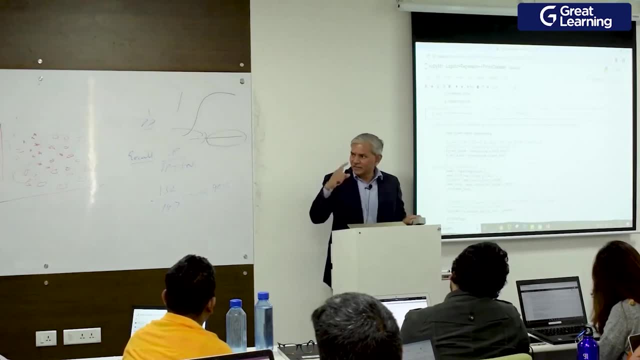 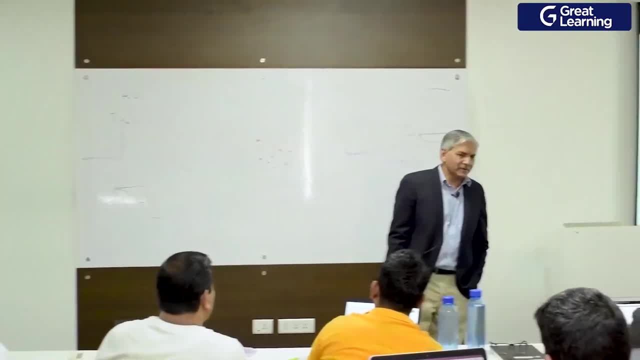 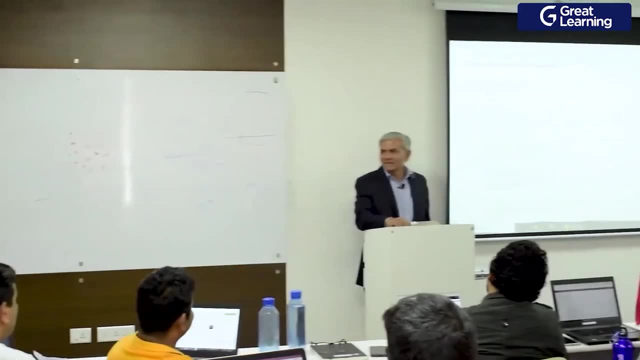 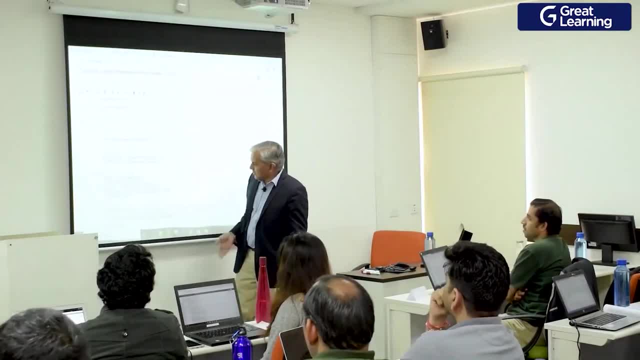 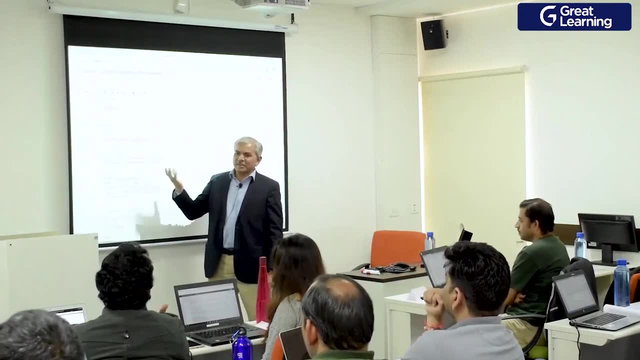 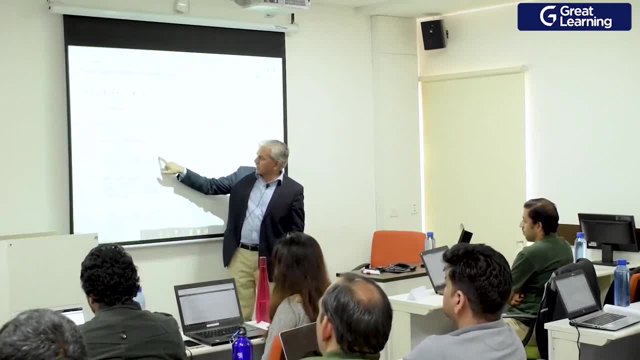 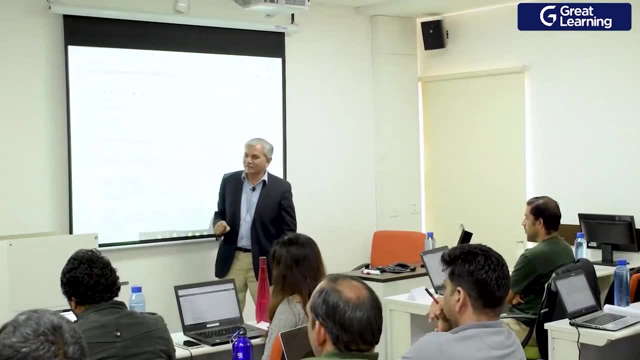 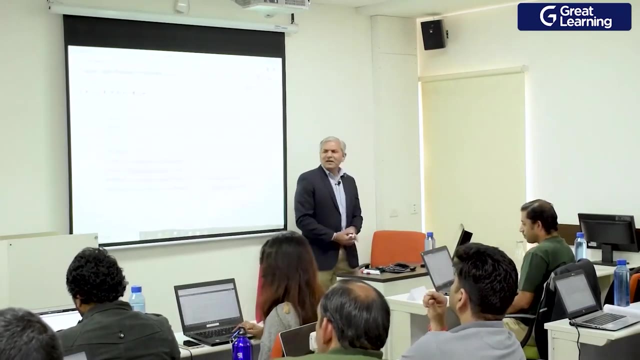 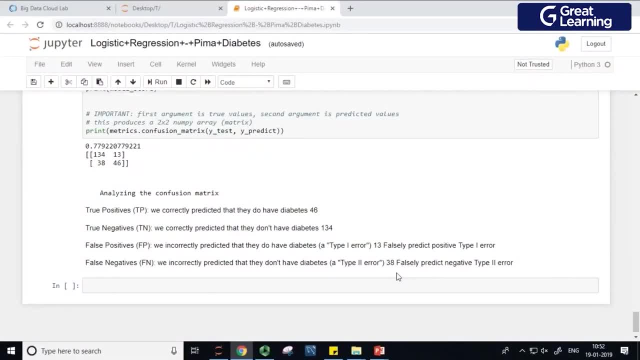 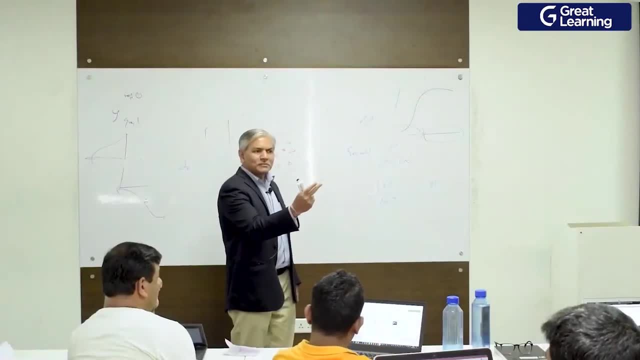 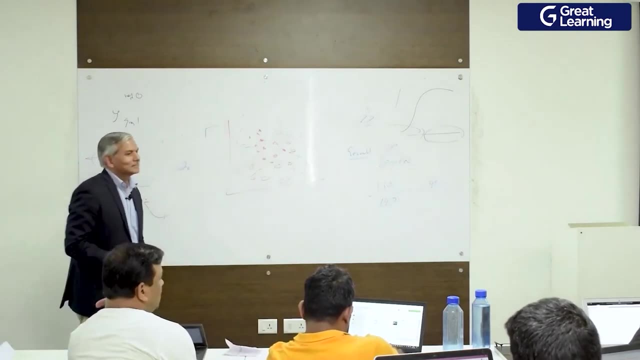 to happen. it never happens. Which type of scaling does it use? Have you told Which type of scaling does it use? This is z-scores- Z-scores- Central variables. La Yesterday I told you scaling does not impact linear models, so you won't see any impact. 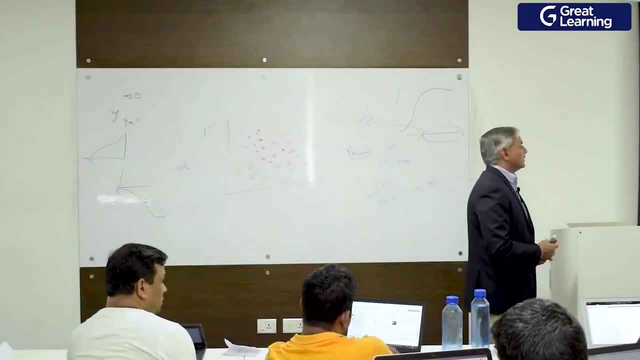 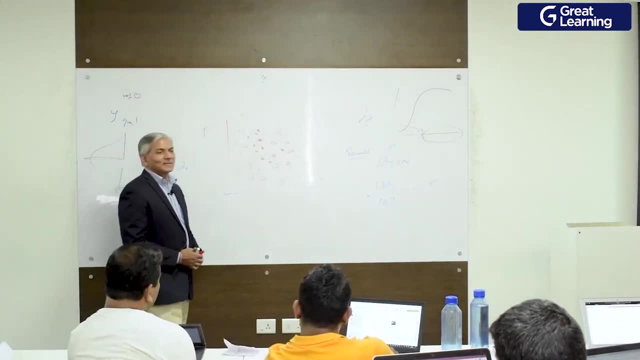 There is nothing else we are going to do, Converting z-scores, x-minus x-bar by standard deviation for every column. centralize the data to zero. So we have a few ways: either we do some dappling or down-dappling. but I thought we don't know. 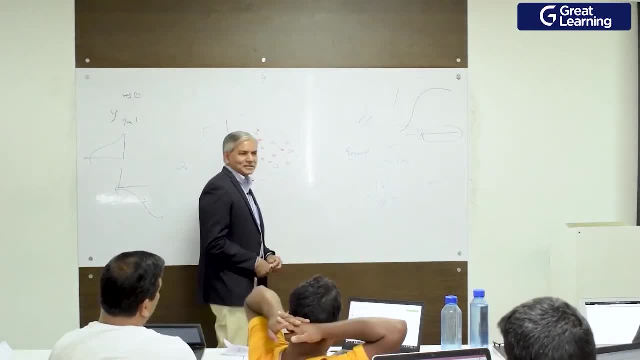 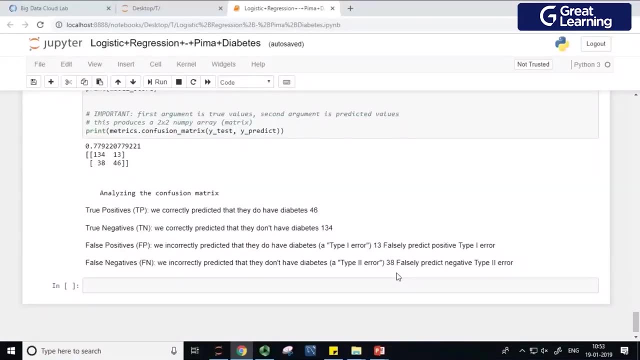 which is okay, Correct. We need to try this more and see, Exactly, Exactly. Will that really affect if we do another one, 100 percent? It will affect the accuracy of the recall for the dappling class 100 percent. 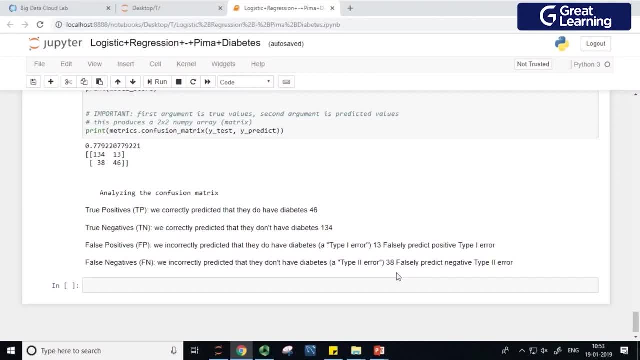 No, no, I mean It is not like doing it half-survey. I mean I just need to go for either one. That depends on how your data is distributed. It depends on that. It depends on that. It is a very subtle relationship with the data distribution in the way it is done. 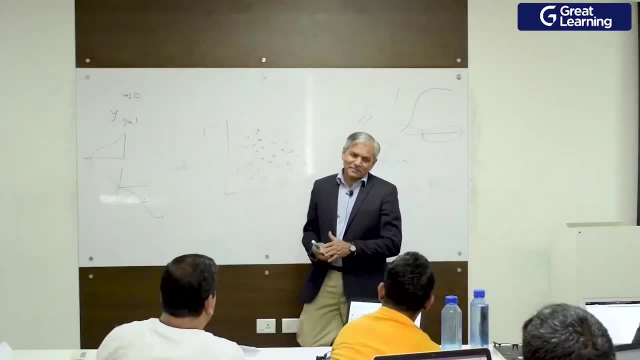 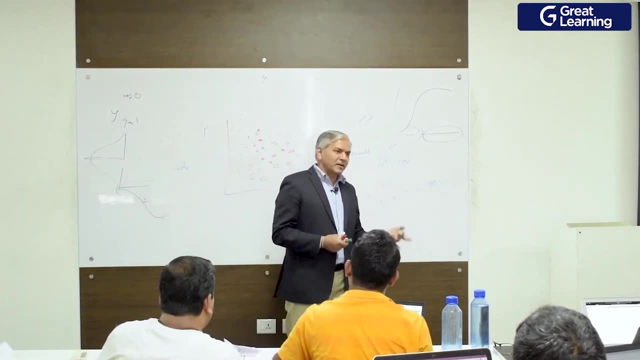 And the threshold management. Changing the thresholds: Yes, Thank you very much. 50 percent is the threshold. no, So I can say: whenever probability is less than 30 percent, it belongs to red class, above 30 percent, it belongs to blue class. 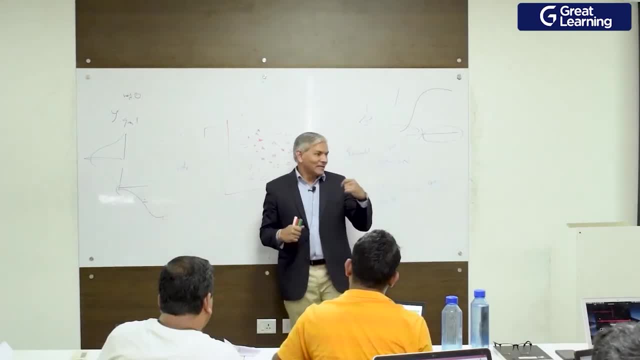 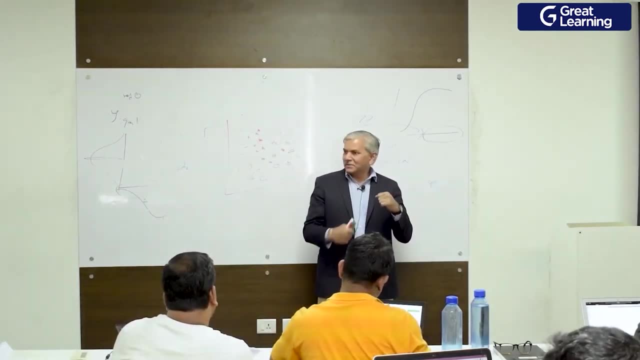 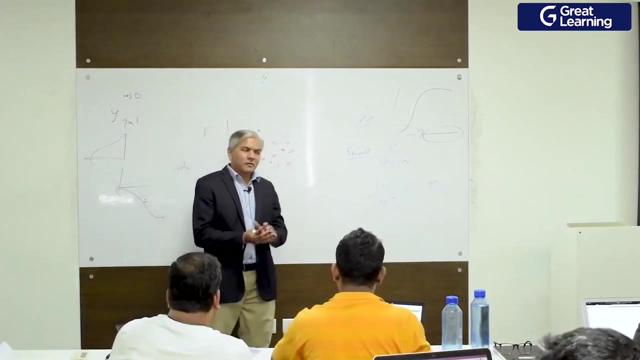 I can change the threshold. right now, by default, it is 50 percent. If probability of belonging to red class is less than 50 percent, that means he belongs to blue class. right now it is that So that 50 percent can be changed to 30 percent by building wrappers around this model. 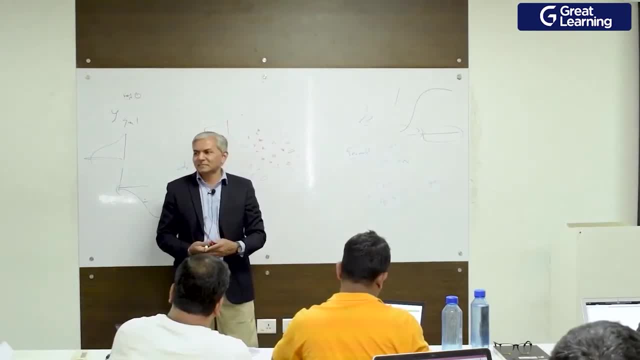 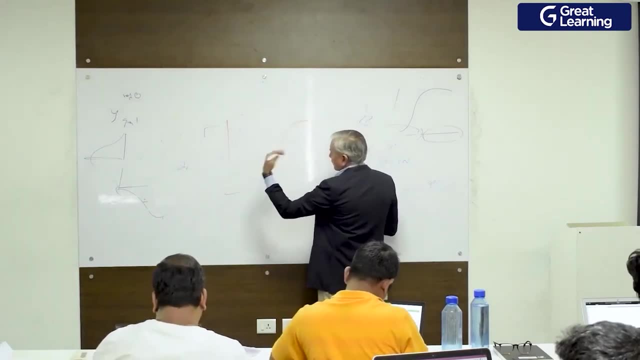 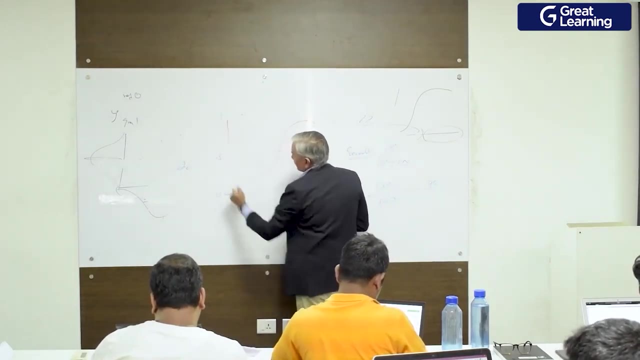 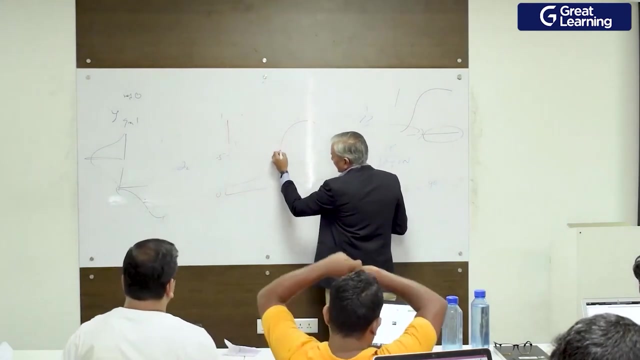 Number of records is what you have in your data Threshold, is in your sigmoid curves. okay, sigmoid or any probability based algorithm. this is my probability dimension: 0 to 1, 0.5,. whenever function this sigmoid function says the probability is greater than 0.5, 0.55, 0.56, then it will automatically say that. 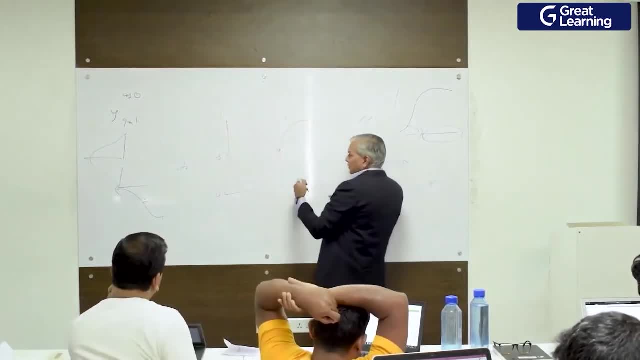 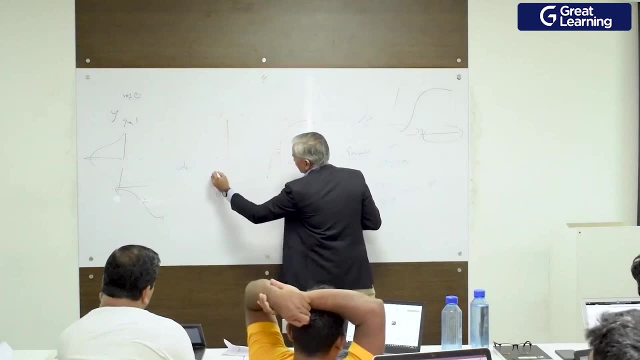 this record is less than 30 percent. If it is below 0.5, it will say it belongs to the red. So I can bring down this threshold and I can put it over here: 0.3.. Anything over 0.3 belongs to blue. anything below 0.3 belongs to red. 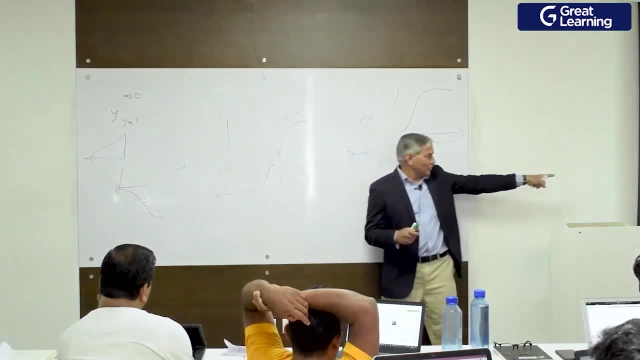 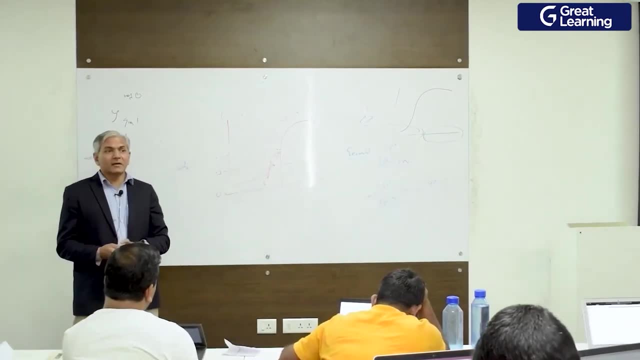 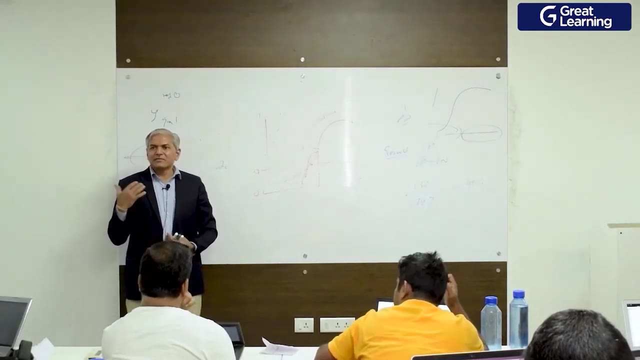 So by changing the threshold I can control the misclassification of the diabetic cases? No, no, it is not a parameter. you have to build a wrapper around your model. There is no automatic way of doing this, So I will use a function in scikit learn. 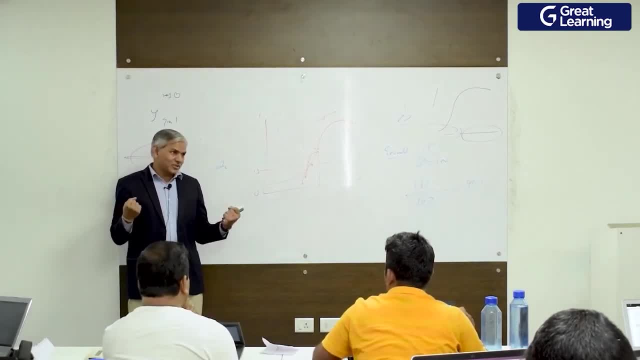 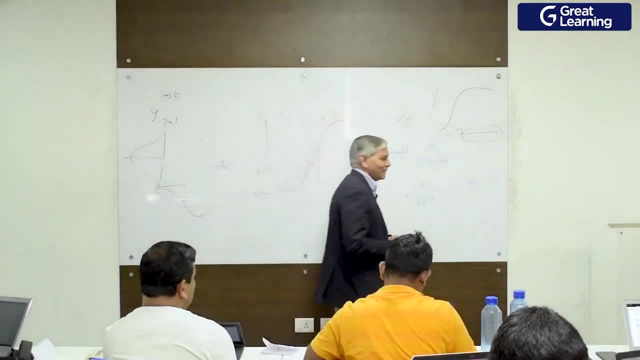 It is called binarize. In case you are very impatient and you want to know what it is, please go and explore this function: binarize- B-I-N-A-R-I-Z-E- How, using binarize, we can control the threshold. explore that. 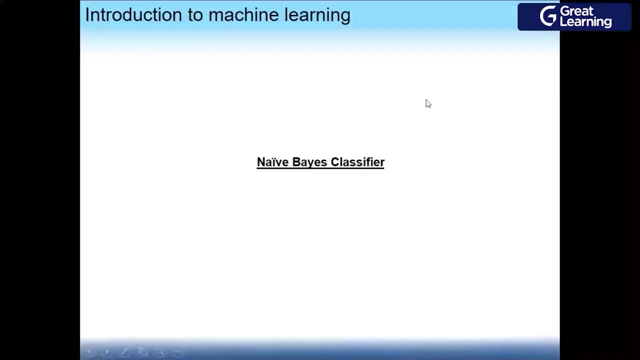 If you are not able to find, I will tell you how to do that in FMT. How do you find the threshold? Which models are suitable for time series? When you talk about time series, automatically only one model comes to the mind: ARIMA ARIMA. 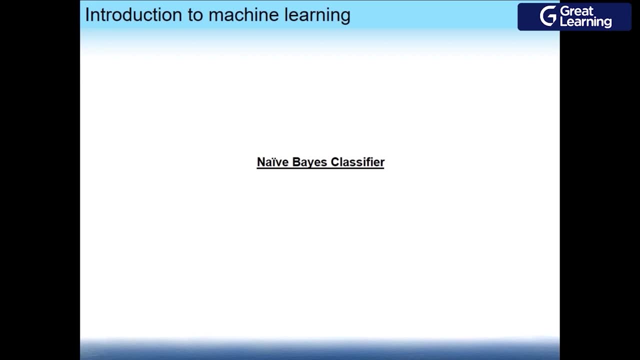 A R I M? A. it is a time series based modeling which is basically linear regression applied on a time dimension. right, So you will explore that. Do you have anything on time series to be done? ARIMA is linear regression for time dimension. 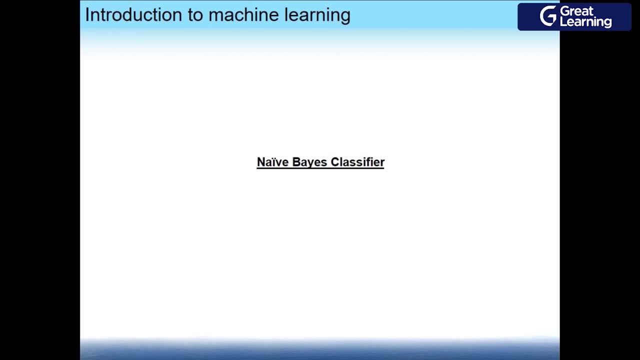 Suppose I want to optimize Tobi. what is that Tobi, Tobi? What is that Tobi, Tobi, Tobi? That is basically to look for intrusions and all these things, kind of things. So at what point of time I want to do network discovery? 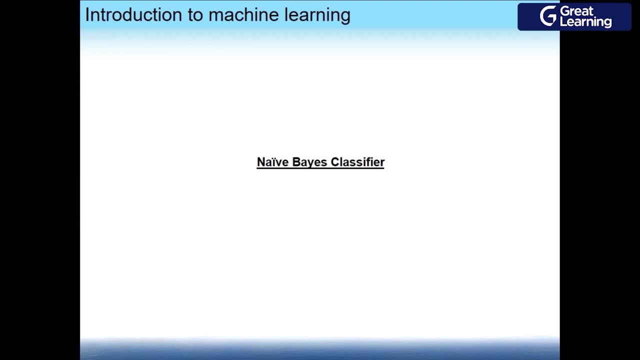 Network discovery. I am not able to put any particular algorithm there. probably we will discuss this further and design You bring it up, we will take it up. Alright, let us quickly start and summarize what we did. okay, We started yesterday by discussing about linear model, linear regression. okay, 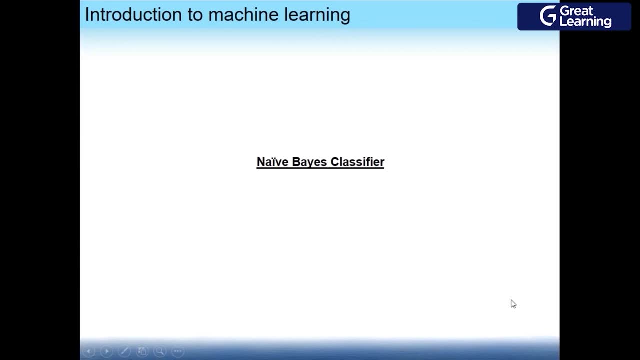 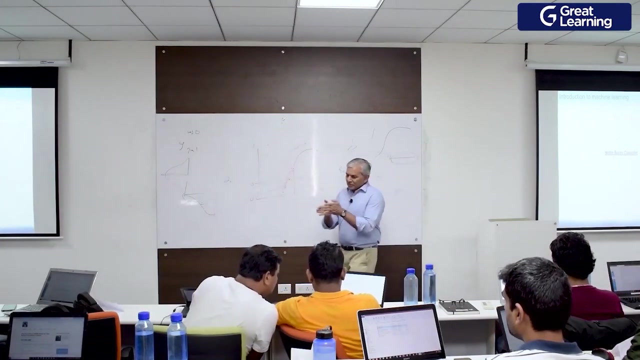 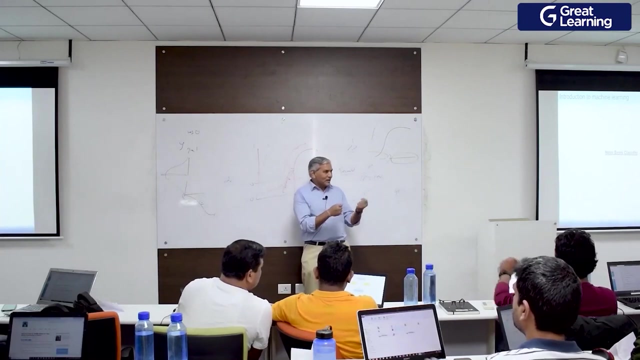 In linear regression, we, the algorithm was used to predict the values. the output is, the target is values, running numbers. okay, And for that we discussed how it is important for you to first analyze your data and check which attributes are strongly related to the target attribute. select only those. 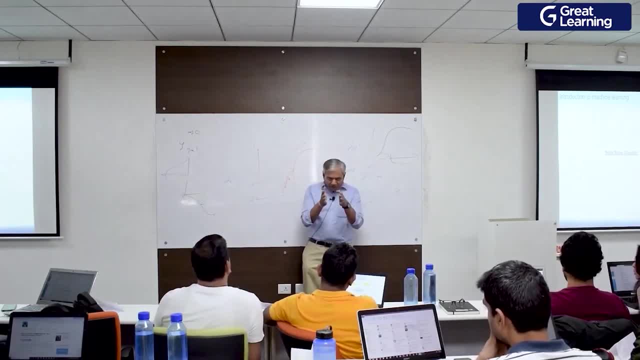 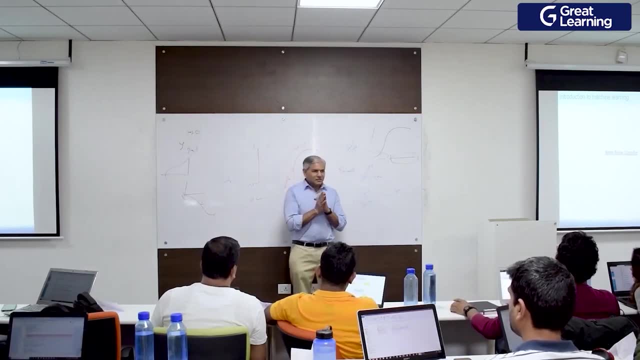 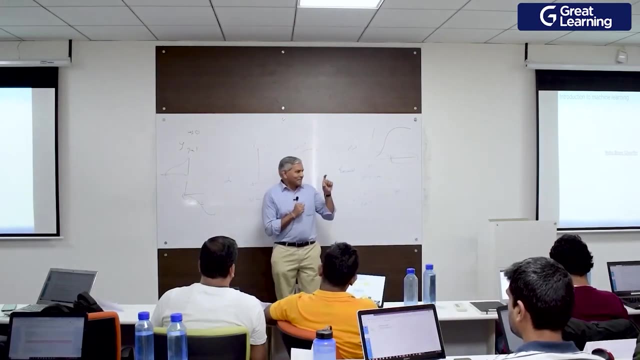 Amongst those, those attributes. drop the attributes which are redundant. That is, they correlate with each other. Remember this discussion we had yesterday. Same discussion continues today also, But before I come to today's topic, we also discussed yesterday that in linear regression. 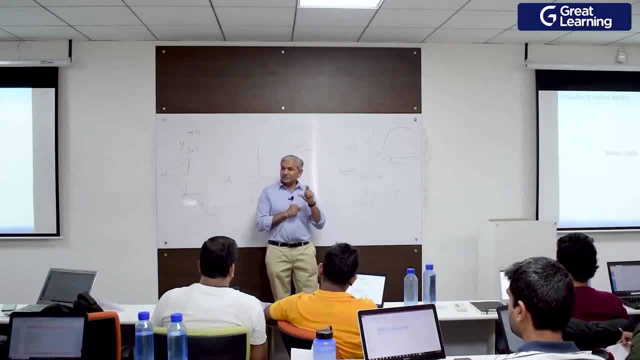 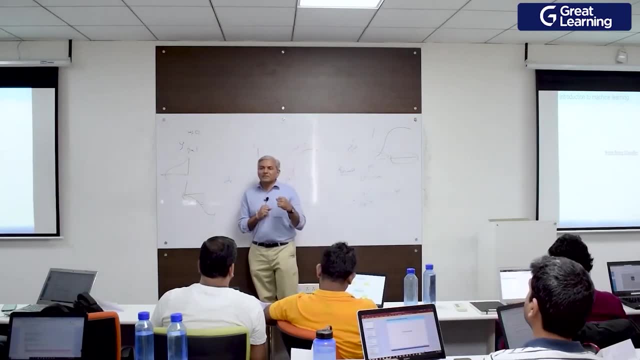 the algorithm finds out for you a needle in the haystack, the best fit line from infinite number of lines, using the gradient descent concept. okay, So the objective is find the right kind of M and the C which will minimize the sum of squared errors. 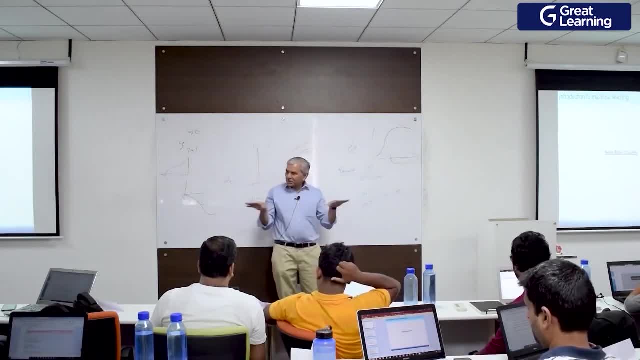 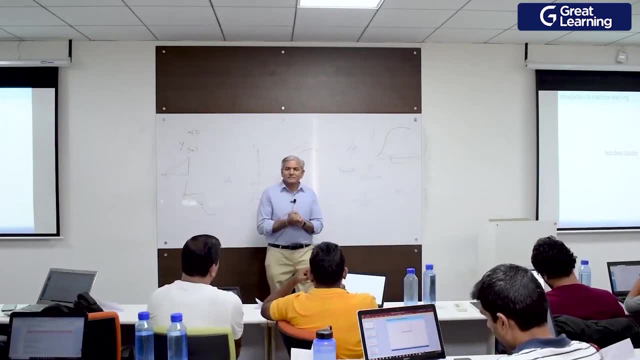 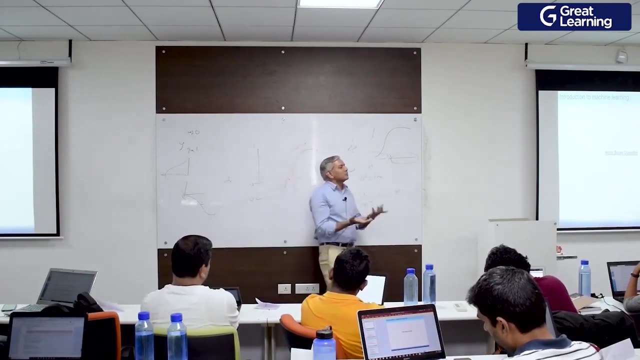 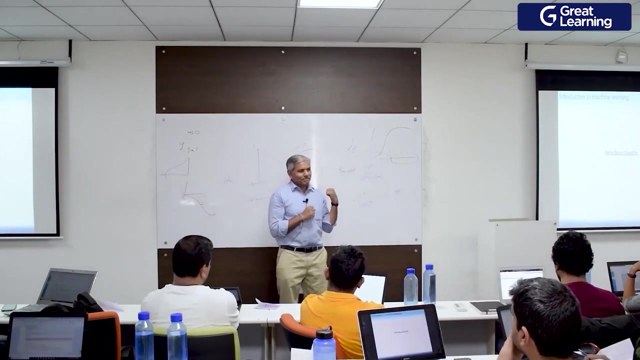 All algorithms have some objective to achieve. In mathematical terminology, we say that all these algorithms are optimization functions. Optimization means minimize something or maximize something. okay, By using this optimization functions, it identifies for you the best fit line, and the methodology is called gradient descent right. 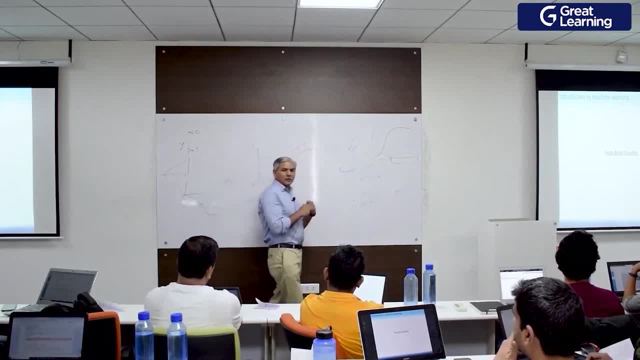 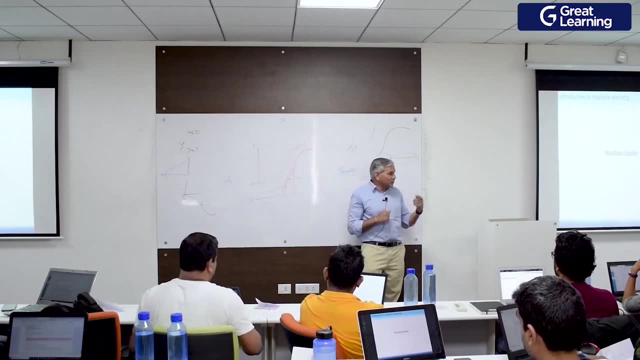 Then the linear regression. Today we saw how linear regression works. So let us start with linear regression. We saw how it is used in classification. This is not the only way. there are various other ways in which linear model can be used. 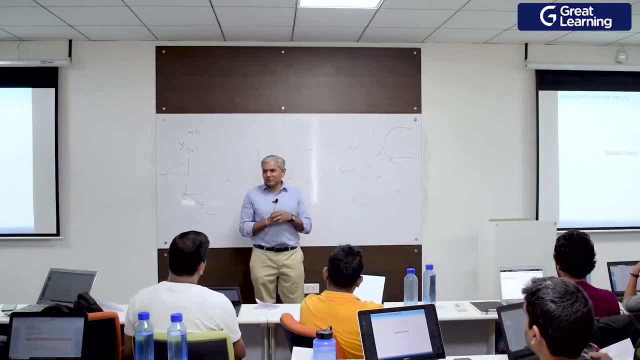 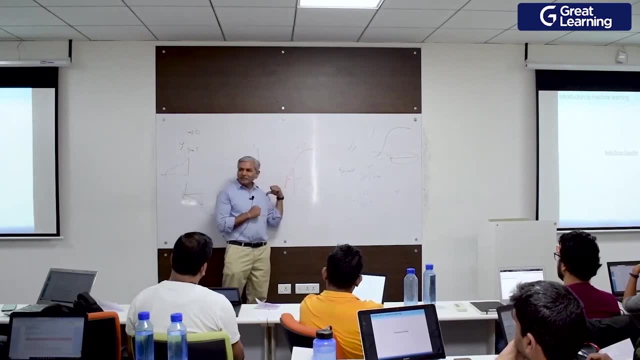 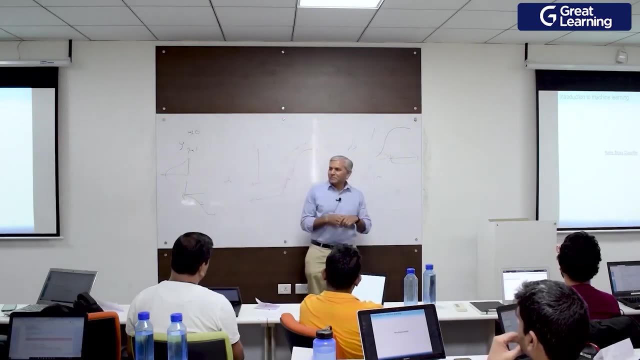 for classification. When we come to support vector machines, we will talk about that also- Support vector classifiers Using linear model for classification based on probability values. you have a challenge. The challenge is linear models extend to infinity and it makes no sense to have values beyond. 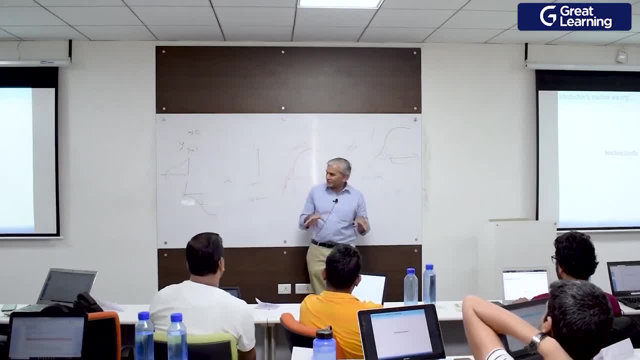 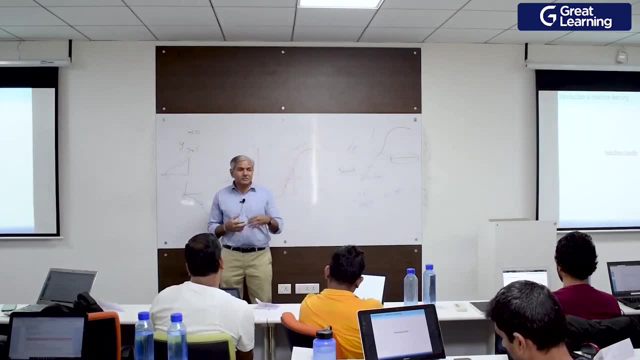 0 and 1.. So we convert the linear models into sigma 1.. All right into sigmoid surfaces. ok, The sigmoid surface will come to you again and again, many times, in many different algorithms, especially those who are going to do neural networks. You will 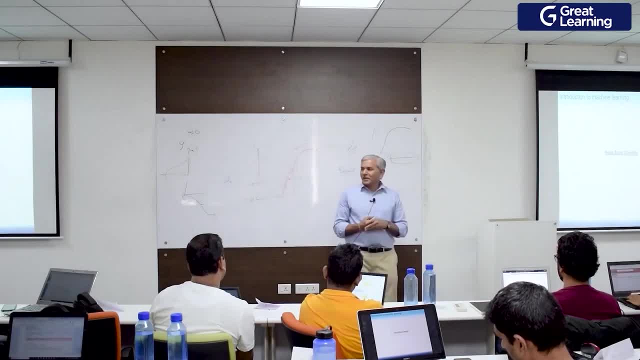 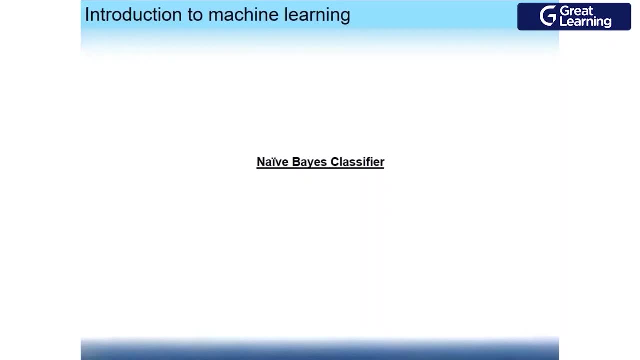 find that neural network uses by default sigmoid to bring in what we call non-linearity. We will talk about those things later. So linear model is used for classification in logistic regression, where it is convert, transformed into an S curve, a sigmoid curve, right. But 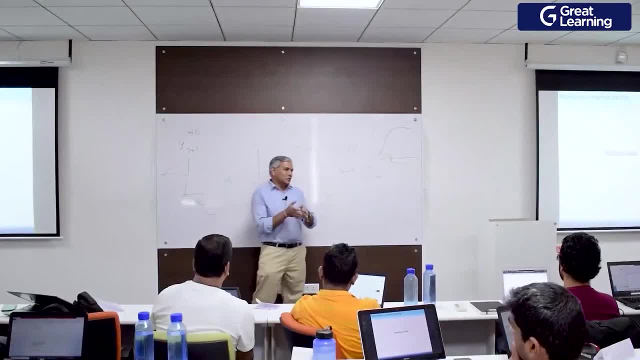 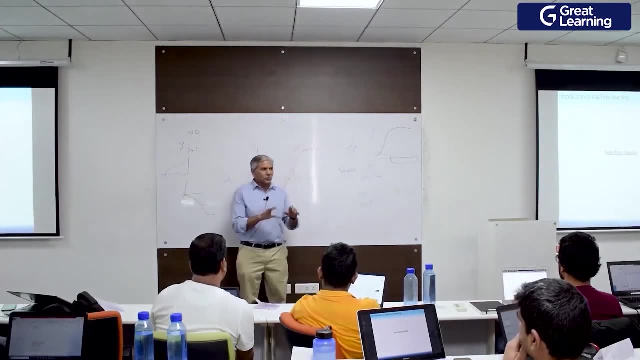 all the rules of data analysis, use only the right attributes. Within those right attributes, there should be no collinearity between them. All those things continues to hold here also. ok, Now I am going to introduce you to one more model called Naive Bayes. 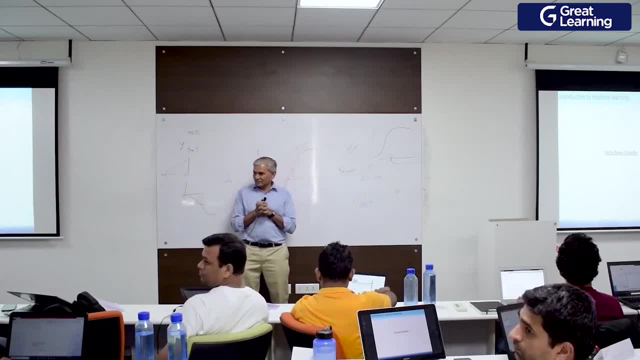 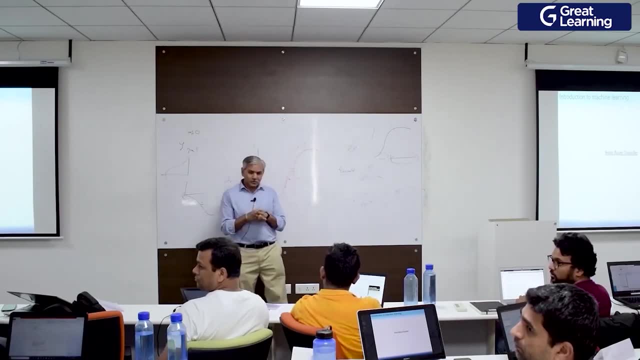 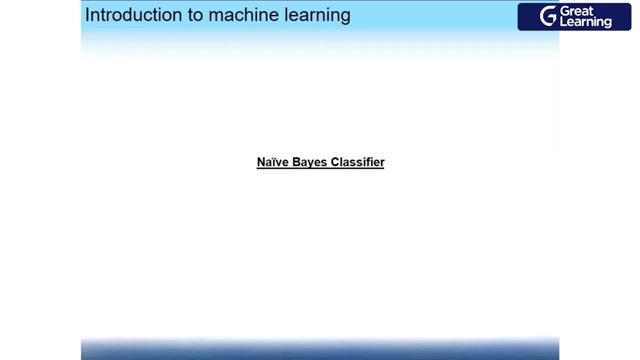 Before we go there, can you just give me a brief? So you have a distinction between covariance, collinearity and correlation. There is no difference. Covariance divided by standard deviation, measured in terms of standard deviation, is called correlation. ok, So if you have x, i minus x bar into sorry. 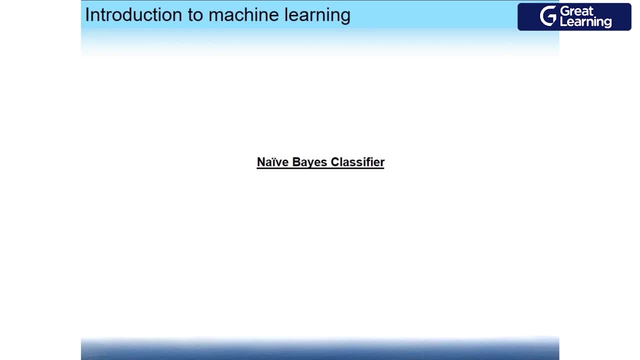 into y, i minus y bar. ok, When you divide this by standard deviation of x and standard deviation of y, we measure it in terms of standard deviation units, We measure it by standard deviation. But if you have interest of this, which we are, 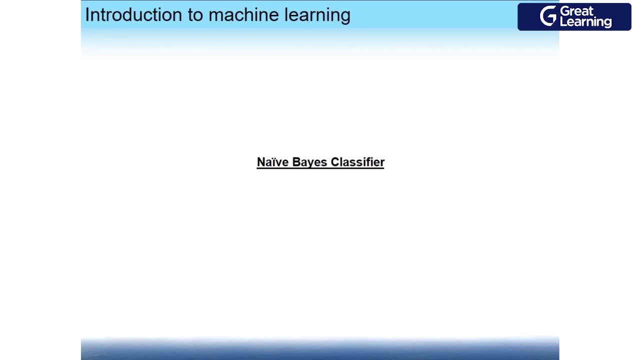 talking about. we can tell them this much: It is called correlation. If you don't use this, it is called covariance, And whenever I have two dimensions have very strong covariance or correlation, they are called collinears. That is called collinearity. ok, So same thing. 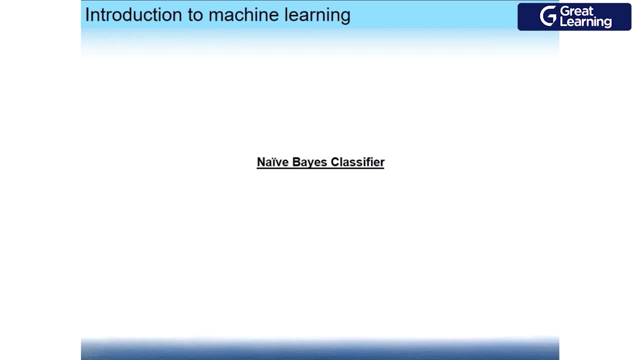 coming in three different ways. Alright, linearly separable, is that distribution okay, whose data points in the feature space have some kind of a gap between their distributions? So I can represent this gap using a linear model. So when I use a linear model for classification, the model is trying to not represent the data. 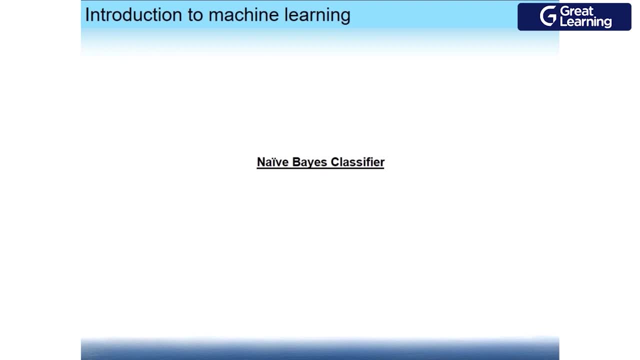 points, but its trying to represent this gap and trying to model this gap between the two. Such distributions are called linearly separable distributions. They may not be linearly separable on one single dimension. there might be overlap. Even on this dimension there is an overlap. 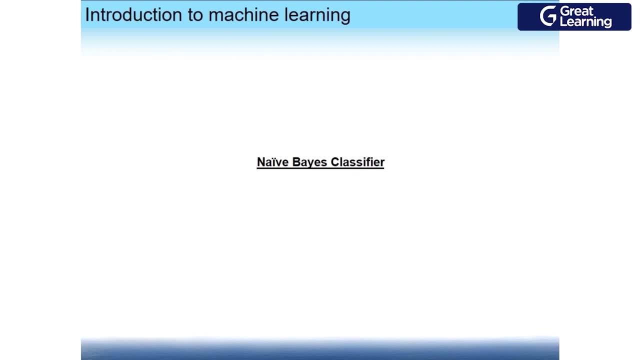 but put together they might become linearly separable. Question: Shall we move on? Yeah, So I will extend this discussion a bit further. Here we see the red ones. okay, this is the distribution of the triangle. this is the distribution of the circles. same way distribution. 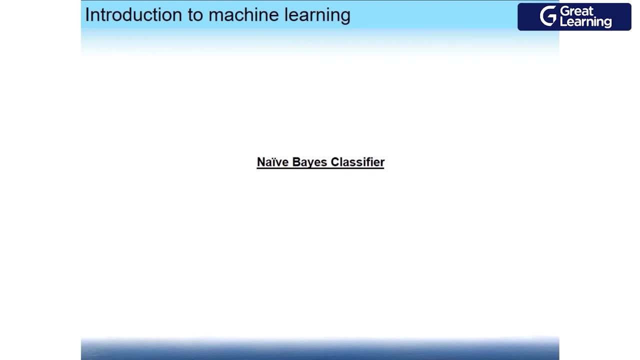 of the circles. distribution of the triangles. okay, The two distributions are overlapping on individual dimensions, univariate analysis. But when you put them together, the two dimensions together, the two distributions get separated out. They become linearly separable. yeah, So even. 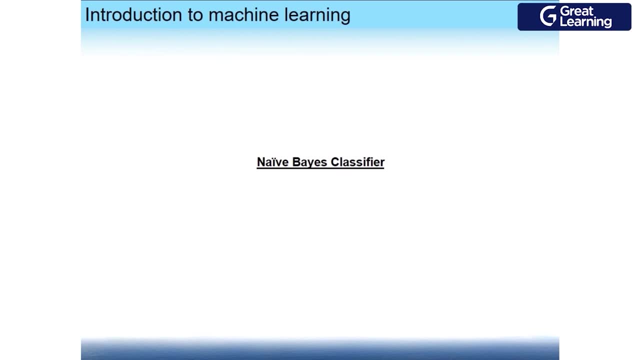 if I have weak dimensions. in the pair plot I see very weak dimensions. They are very significantly overlapping but the central values are slightly away from each other. Maybe combination of these weak dimensions put together will give me this, But unfortunately in Pima diabetes none of the dimensions give me this. 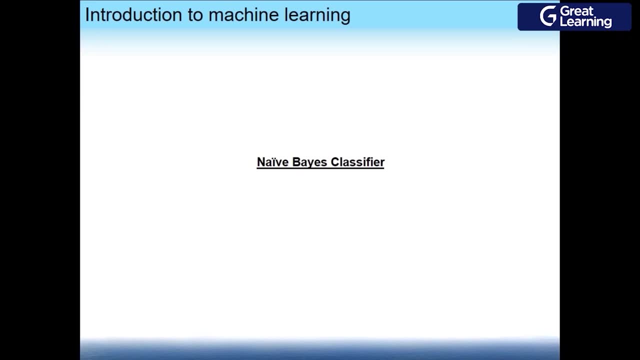 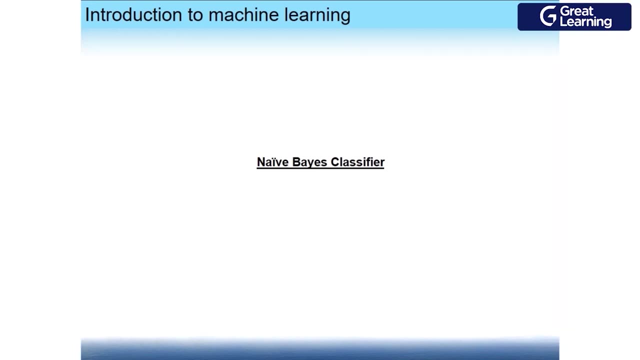 I understand the point. You told that two dimensions are overlapping each other. In two dimensions the classes are overlapping each other. So in Pima diabetes, if you see the diagonals, the diagonal, all the classes or central values are significantly overlapping. 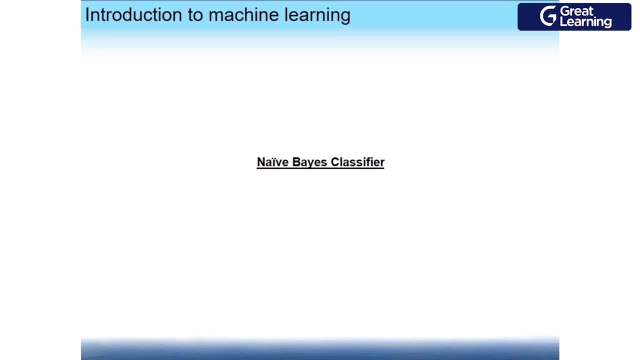 If you have even a single one, which is central values are shifted away, Ok, Maybe another single one where the central values are shifted away, not significantly shifted away. Maybe these two together will be able to give me linearly separable classes. 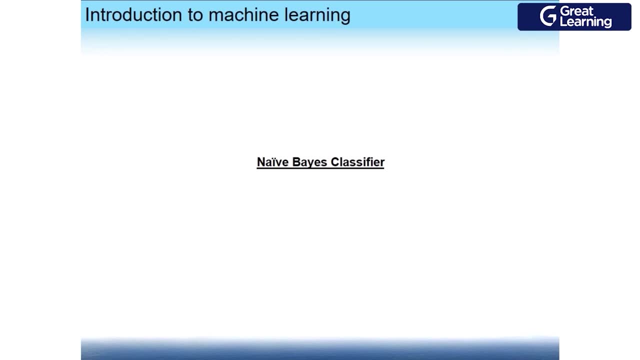 But unfortunately Pima diabetes all the dimensions. if you observe carefully, the central values are sitting on top of each other. Analysis of variance uses the difference between central values to tell you what is the probability that these two belong to different class. So as long as the central values are sitting on top of each other, you will be able to. 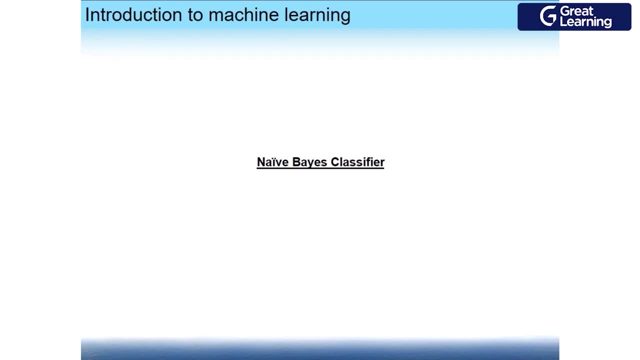 find out what is the probability that these two belong to different class. So if the central values are overlapping, there is not much you can do. The body of the distribution overlapping is still tolerable, but central values are overlapping. that is the problem. 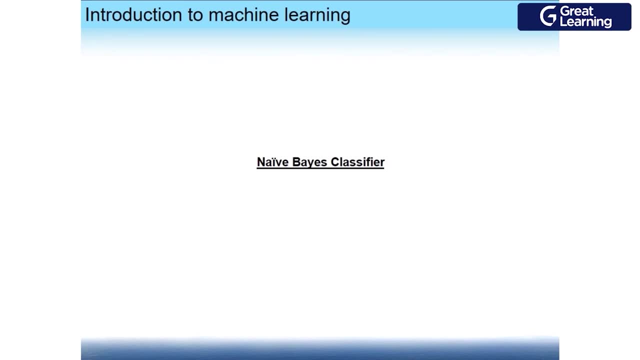 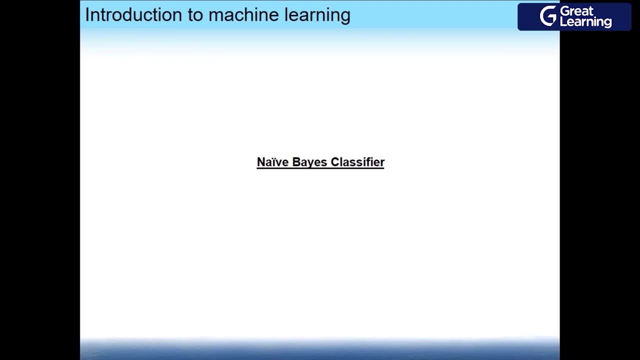 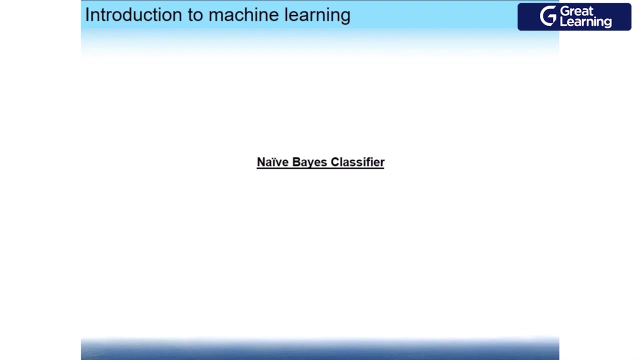 All of you. ok, Shall we move on. But what we analyze is just from one. so we did not have to different variables to be known. We did not. We saw in diagonal, We saw just diagonal, Diagonal, Diagonal. Look at this: scatterplot also, Scatterplot also. they are all sitting. 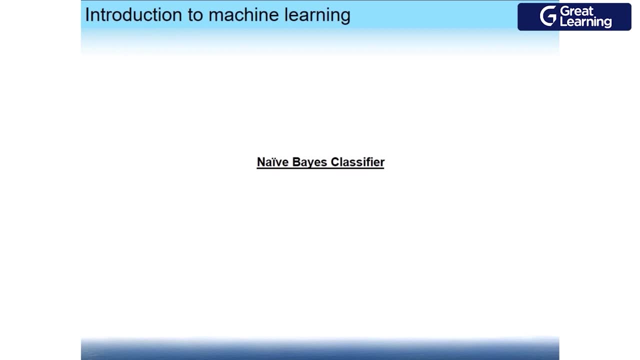 on top of each other. they are eclipsing each other. Scatterplot also: the blues and the yellows are eclipsing each other. So the centroid of the blue cluster and centroid of the yellow cluster. they should not be eclipsing each other. 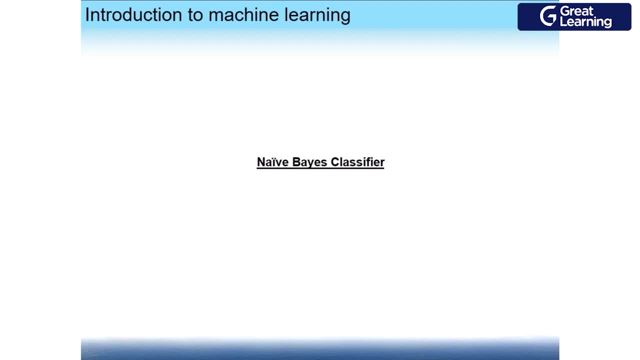 All right, Let us go on to this new one, Naive Bayes. This is purely statistical model. It is based on the Bayes theorem, which I presume you people have already covered in the statistics class. Do not say no, Right. 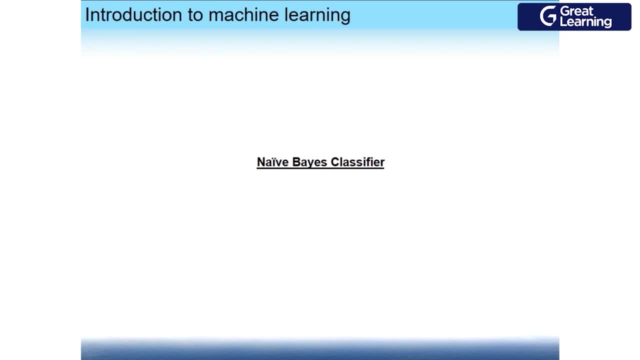 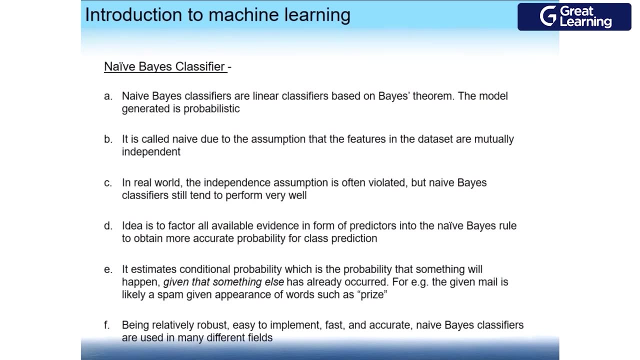 Ok, So let us see. what is this Bayes theorem? how is it used in modeling This model? this algorithm is based on the Bayes theorem. It is used for classification. Again, it uses probability values to decide which class a test point belongs to. 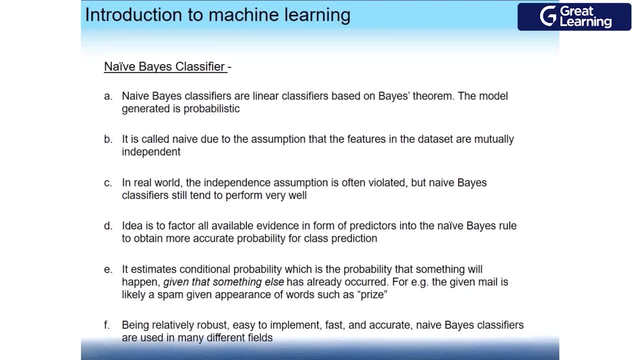 This is the only algorithm which gets this term associated with it, called naive. The term naive is not a very good thing to be associated with, Ok, But this algorithm is the only one which gets associated with that. very unfortunate, because all algorithms are. 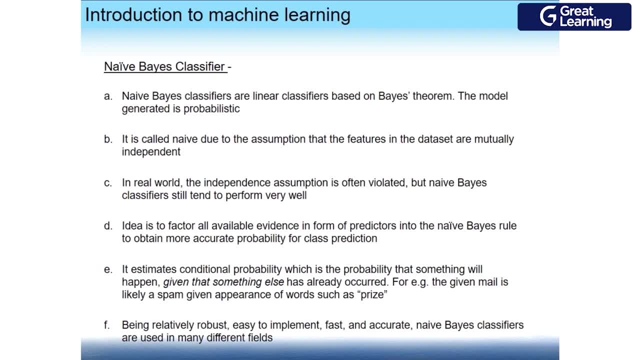 naive, as per this definition. The reason why it is called naive is: this algorithm assumes that all the variables that you are going to use to build the models, Those variables, are independent of one another. The independence assumption is often violated- We already discussed this, But then this is true for all the algorithms It is called. 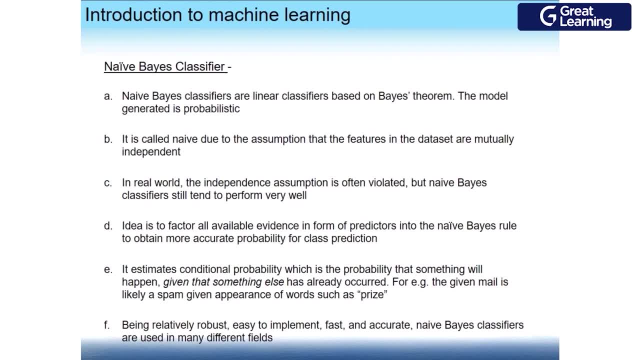 naive due to the assumption that the features in the data set are mutually independent. They do not interact with each other. But that is what every algorithm does, So this is the only one which gets the cap, the hat, whatever you call it. But the beauty of this. 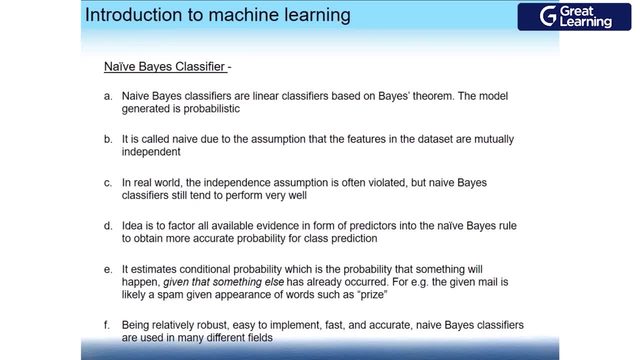 algorithm is what this algorithm says is: howsoever weak predictors your features may be, do not drop them. Consider them, Take into account the information given by each feature and build your model based on probabilities. So it does not advocate you from dropping 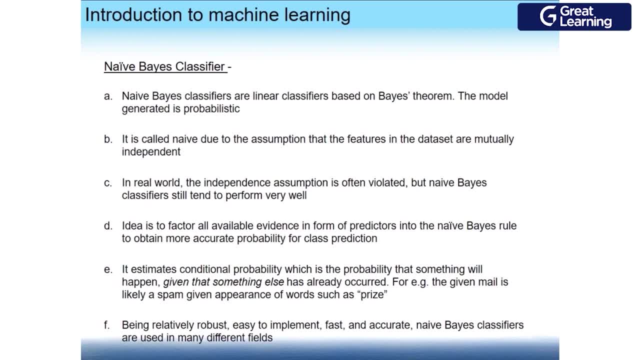 any of the features, Howsoever significant the overlap might be, use them. That is what this algorithm says. To understand this algorithm, we have to understand what is probability, we have to understand what is joint probability and we have to understand what is conditional probability. 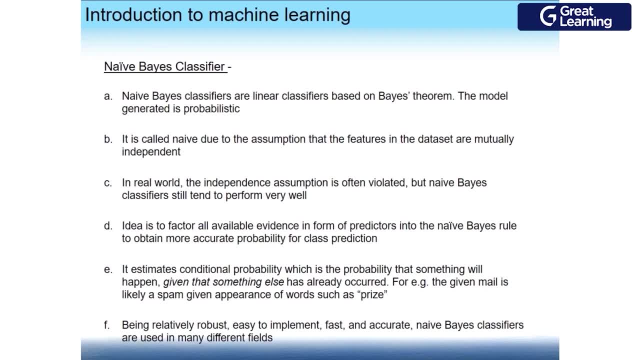 three of them. So let us quickly start. What is a probability? How do you define probabilities? Ok, Chances of some event occurring. So in the definition you have an event and then you have something called chances. What is the chances? How do you find it out? How do? 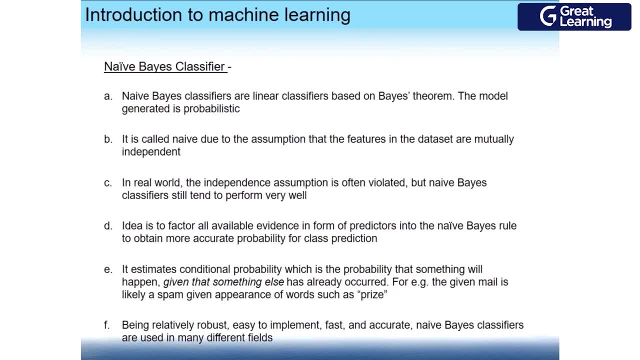 you find a chances, Right. Ok, How do you find the chances? How do you find the chances of something happening? so, what involves the experiment? what is there in the experiment? Trials and proportion, right. so if I ask you, what is the probability that today it will? 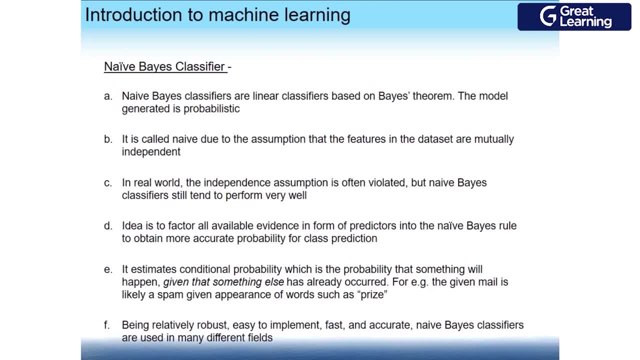 rain and you might be surprised. just a week ago, week or 10 days ago, there was news in the web where in Kerala there was snow fall. have you seen that In Kerala there is a hilly- what do you call- hill spot, Munnar? right there they had snow. 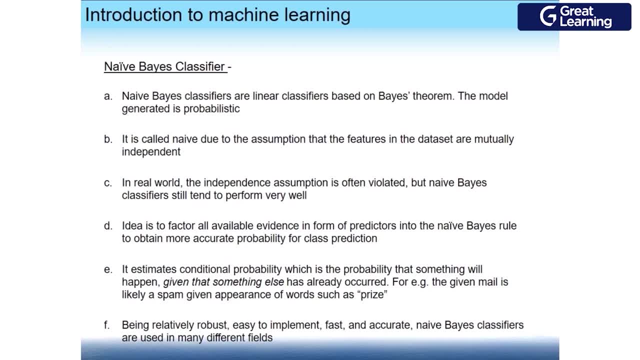 fall and the temperature was minus 3, right, so such events can happen. So if I ask you, what is the probability that today it is going to rain at 5 o'clock? Why did you say 0?? Who said 0?? Why did you say 0?? 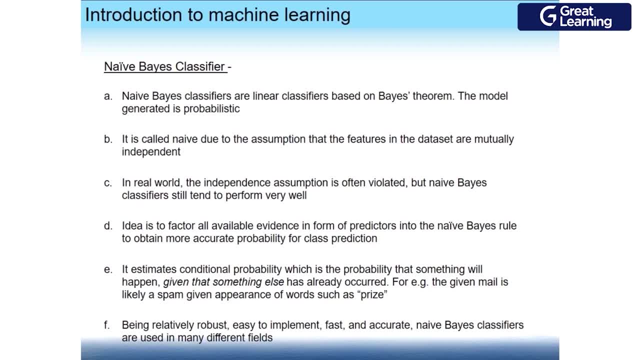 Son, Son, I don't say any thoughts, Son Never had much to say: Get much, Get much. Don't check the weather, just talk. So what you have done is you have taken your past experience into account on this particular. 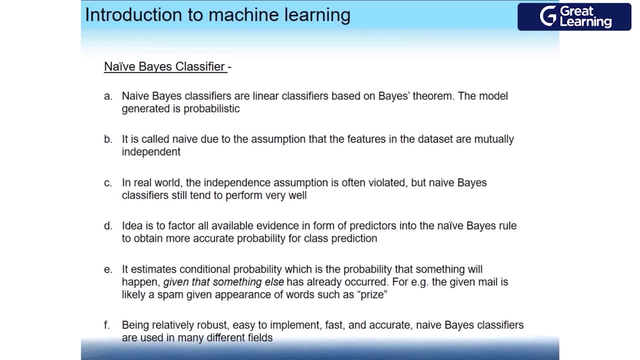 date: January, month of January, almost middle of January. how many times in the past did I see rain? That ratio, how many times you saw this event of interest versus your past record, the number of trials. this ratio is called frequencies approach to probability. 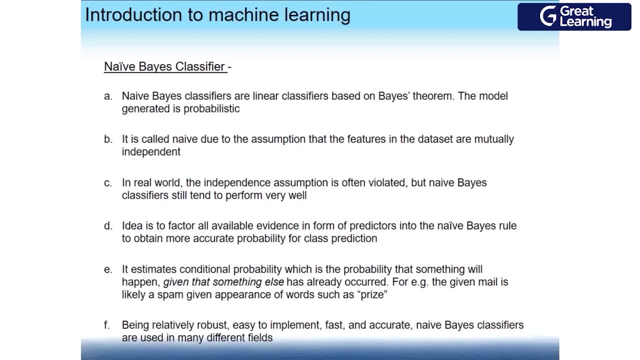 So the probability is a ratio. Well, it is a ratio of the events of interest to you, how many times they have occurred out of the total number of trials, how many times the event could have occurred. That is the ratio called probability values. 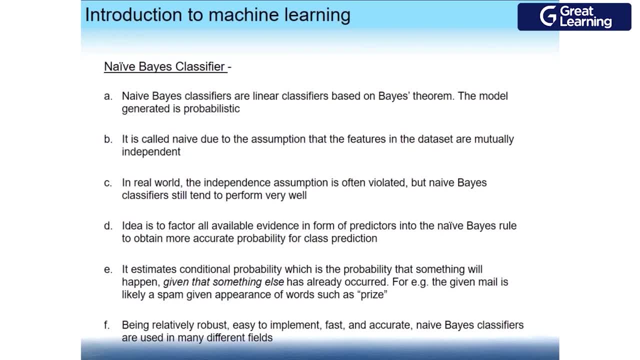 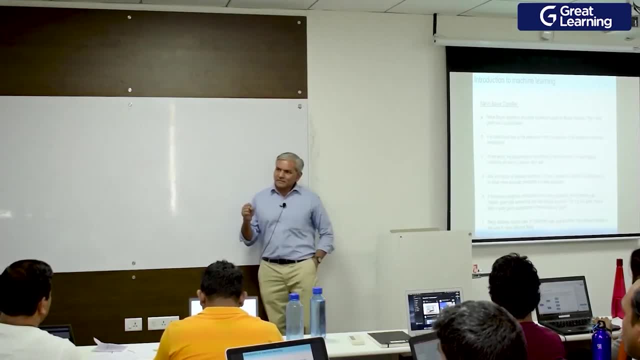 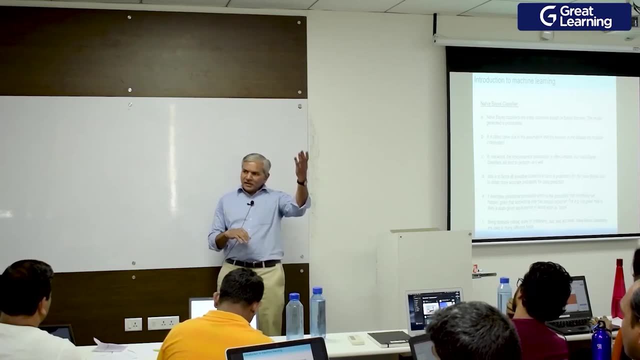 Did you know that probability values can be calculated in another way? Have you done Poisson distribution in statistics? Poisson distribution: very convoluted formula there. If, given the state I am in, Yes, What is the probability that I will be in a different state? the next state? 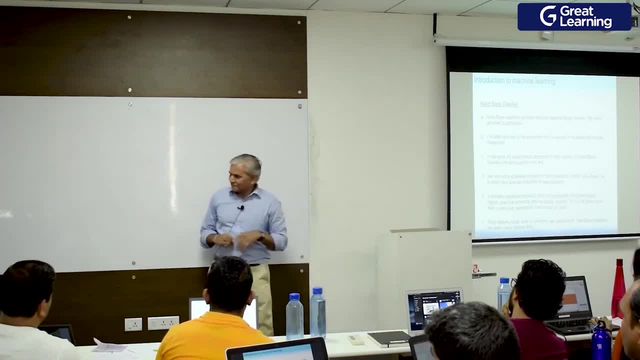 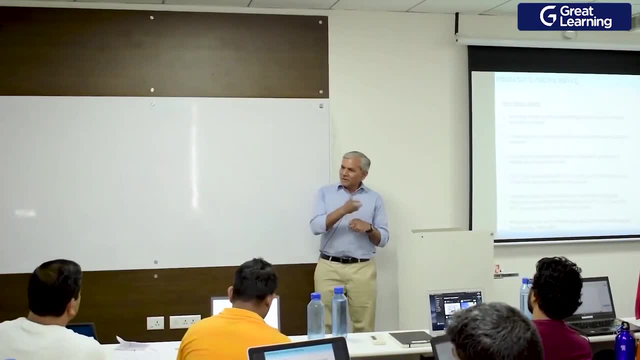 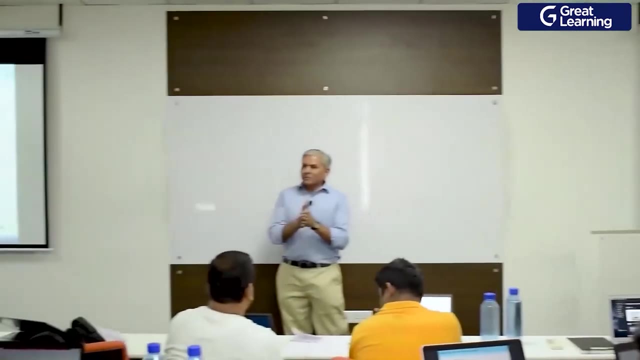 That is a function of how many ways you can reach that state. ok, So that is another way of finding probability. We are going to use the previous definition of probability, which is based on frequencies ratios. ok, Now that you know what is probability, the next thing you need to know is what is joint. 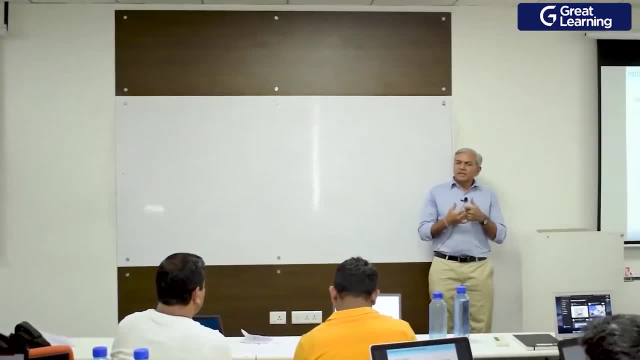 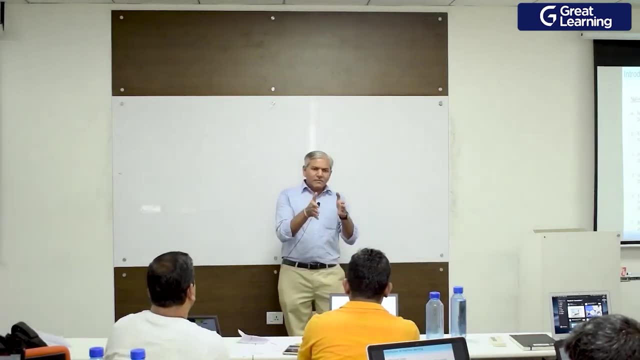 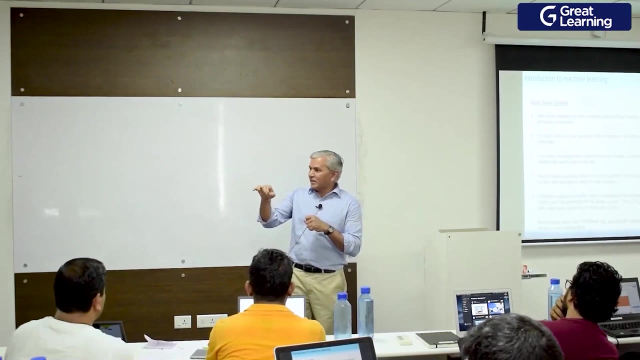 probability. Joint probability is probability of multiple events occurring together. Ok, So what is the probability of if I give you a deck of cards and ask you to pull a card out of it and I ask you what is the probability that this card is going to be a red king? 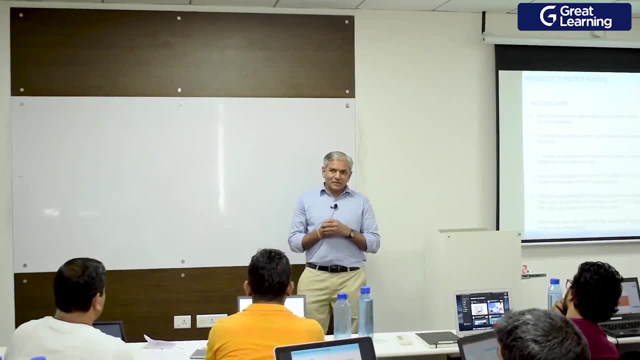 1 by 52.. 1 by 52 is red. No, you have red cards, 2 by 52.. 2 by 52.. Red king: 2 by 52.. Red king, Red king, Red king. 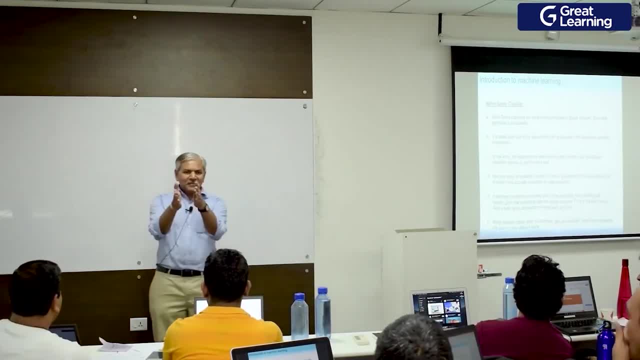 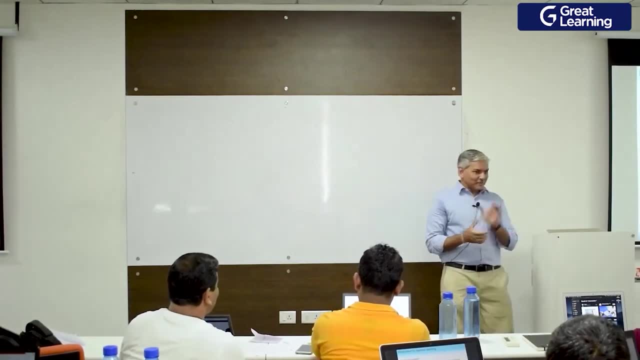 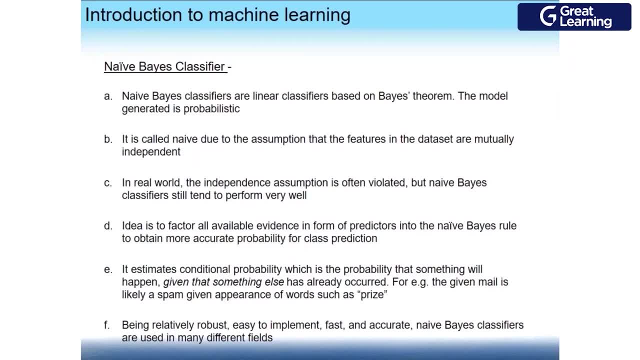 There are 2 colours: red and black, 52 cards. So 52 cards. you have 2 red kings: hearts and diamonds. So the probability of this joint event of red king is red is 1, king is 1 the probability. 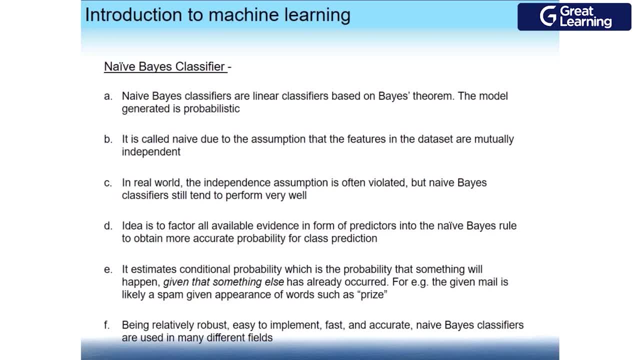 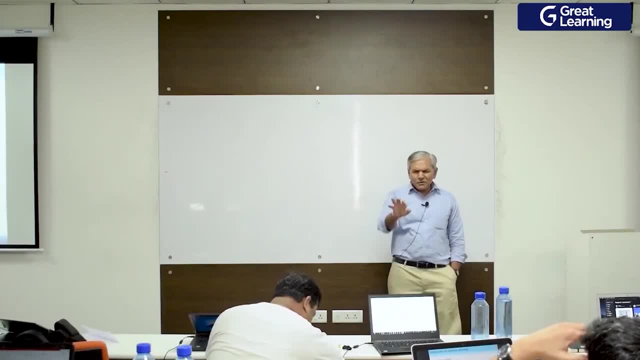 is 2 by 52, all right. Now, when you are pulling out the card, somehow you come to know that it is a red card. Let us look at this way: Red King is 2, red is 42. Somehow you come to know it is a red card. 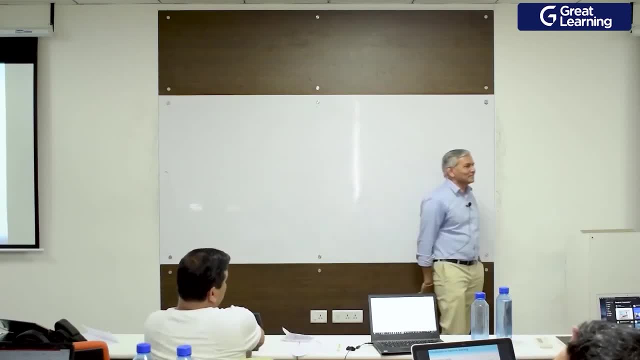 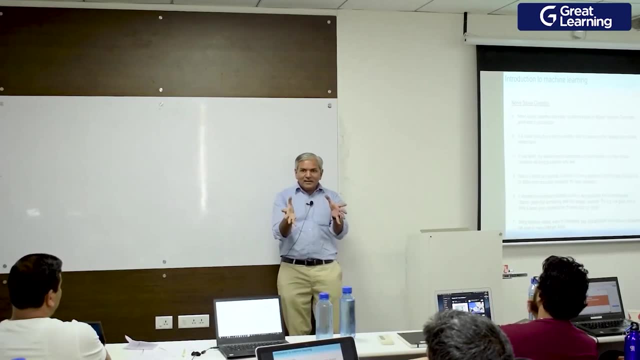 Now, what is the probability? this is a red king. Now you know it is a red card. So your scope is now limited to only red cards. 2 by 26,. 2 by 26 is 1 by 13.. So you have taken into account and evidence and information that you captured, that it 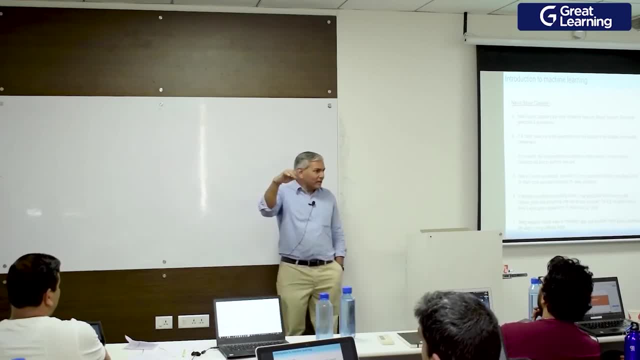 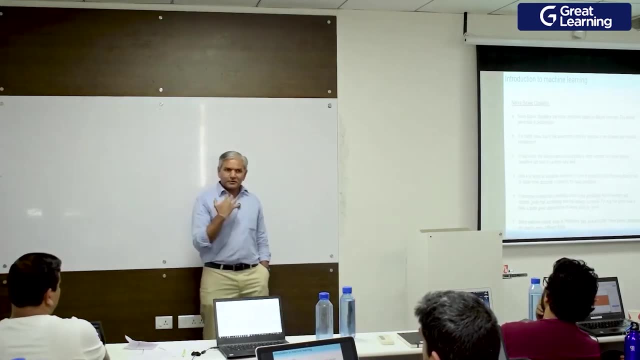 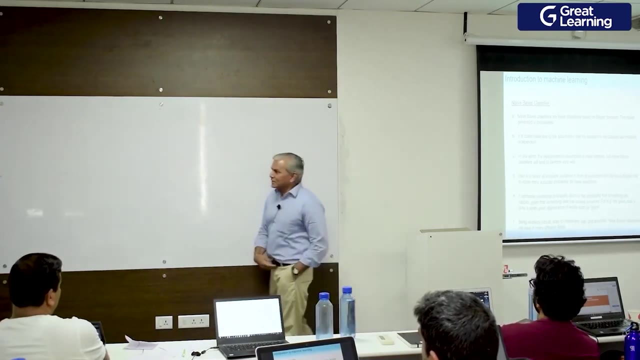 is a red card. The moment you get that information you recalibrate your probability of red king. That concept of recalibrating your probabilities based on the information that you are gathering, that concept is called Bayes' theorem. So what Mr Bayesian said is start with some probability, the default probability values. 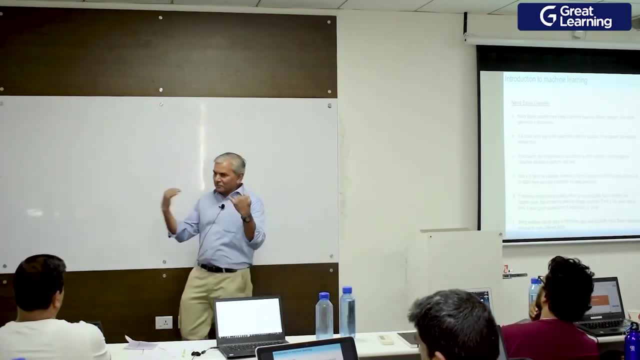 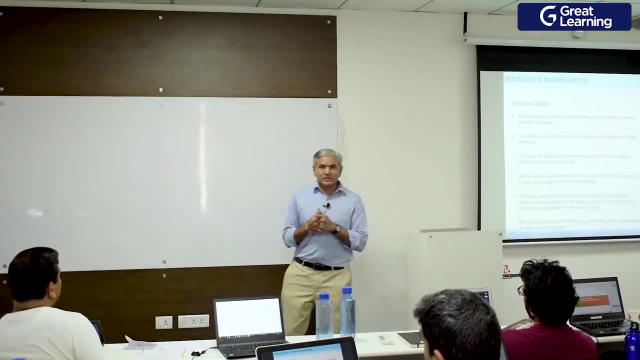 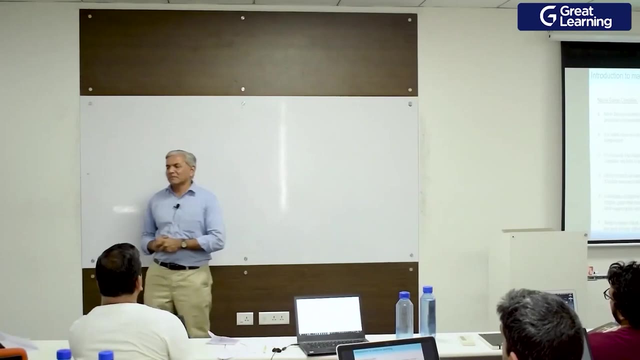 But keep on recalibrating those probabilities. the moment more and more information comes to you, Howsoever the information may be, howsoever weak the information may be, Don't ignore any information and recalibrate your probabilities. That is the philosophy or reasoning behind this Bayesian theorem. Bayesian models. 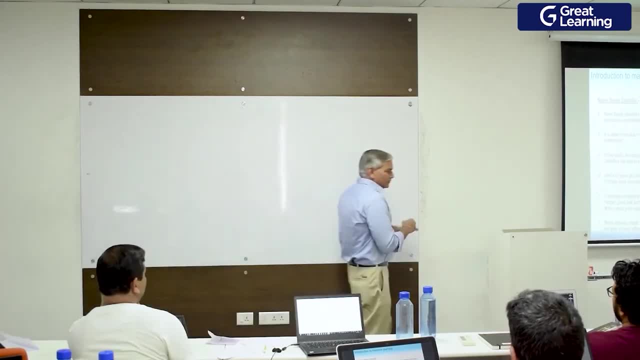 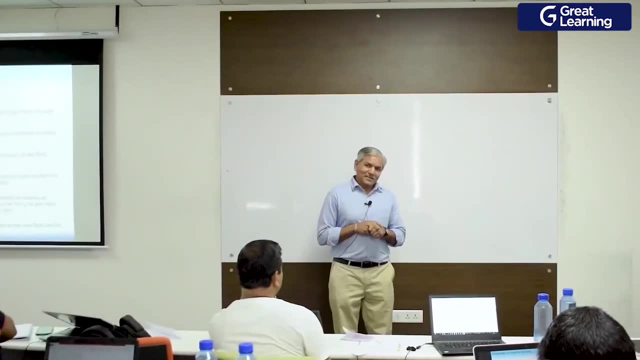 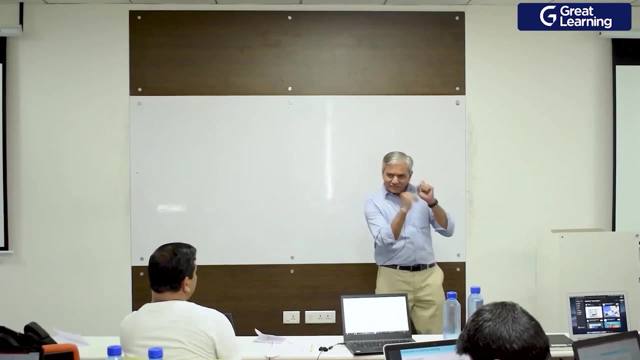 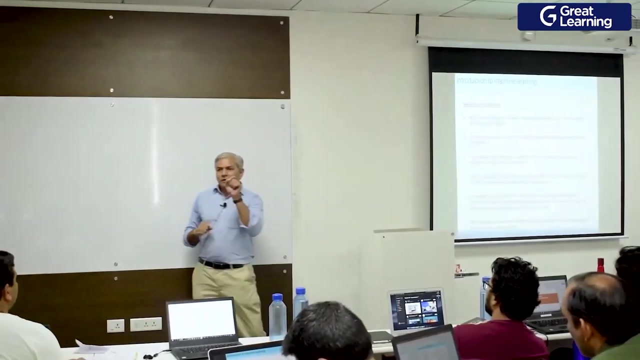 Are you all okay? So for this, to understand this, we need to know probability, joint probability and your. what is conditional probabilities? Conditional probabilities: what is the probability of king, given it is red? We know it is already red card, So now only the event left to happen is king. 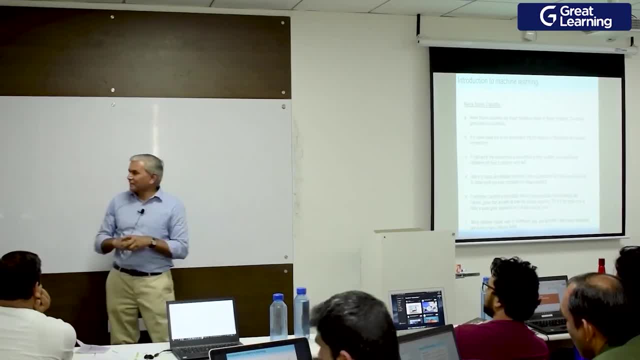 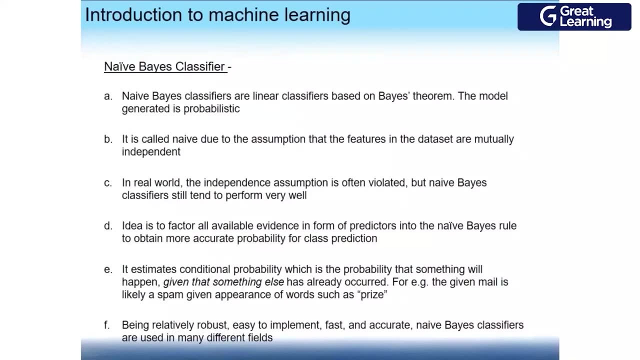 So what is the probability that this card will be a king, given it is red? That concept which you call 2 by 26,. that concept is called conditional probability. So we started by joint probability. what is the probability it is a red king? 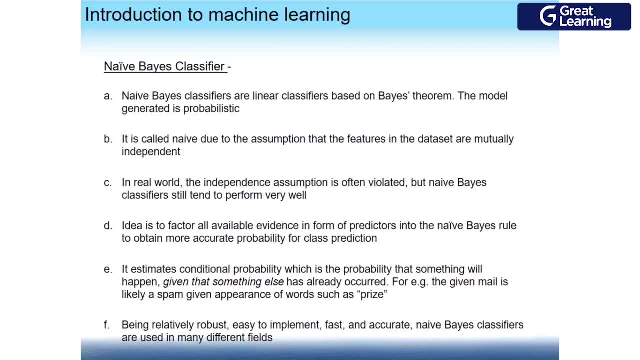 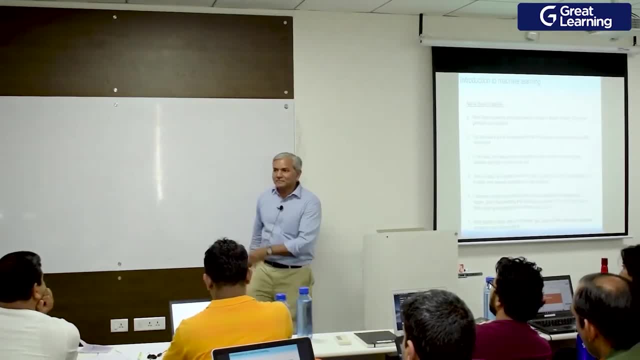 Because we didn't have any information. It was 2 by 52. The moment we came to know it is a red, Then we switched to conditional probability, Then we switched to conditional probability, Then we switched to conditional probability. What is the probability of king, given it is red? right? 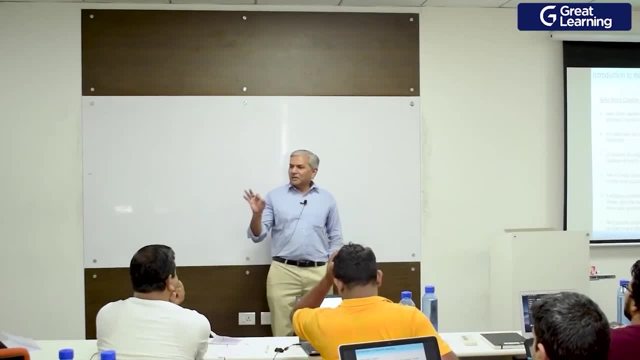 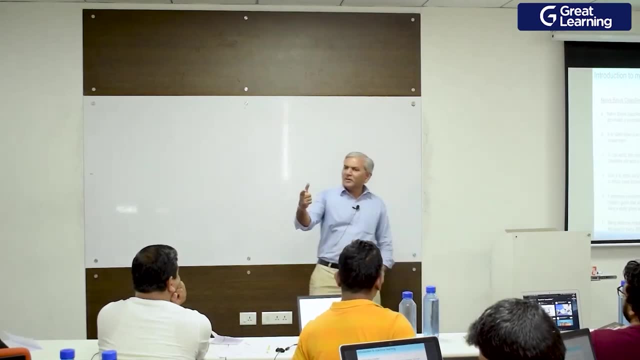 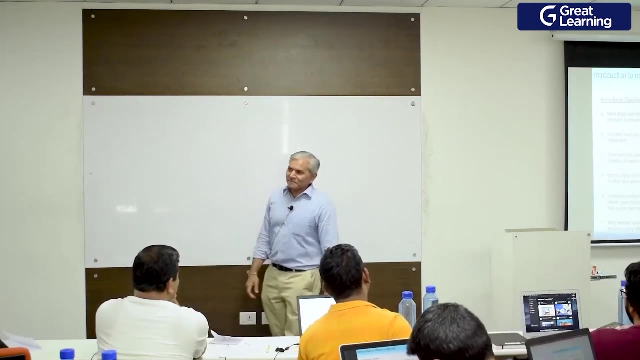 Conditional probability is invalid if joint probability is 0.. If probability of 2 events occurring together is 0, we don't talk about conditional probability. What is the probability of drawing a green king? There is no green king possibility, So don't even talk about conditional probabilities. 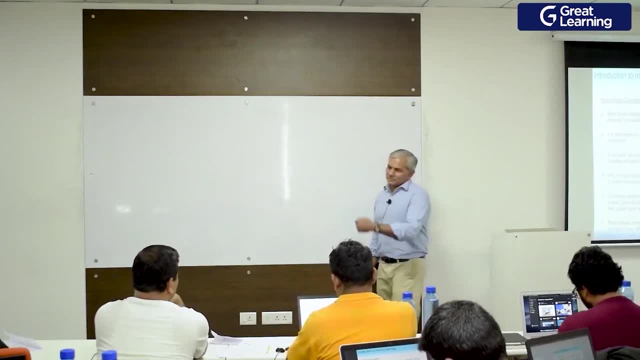 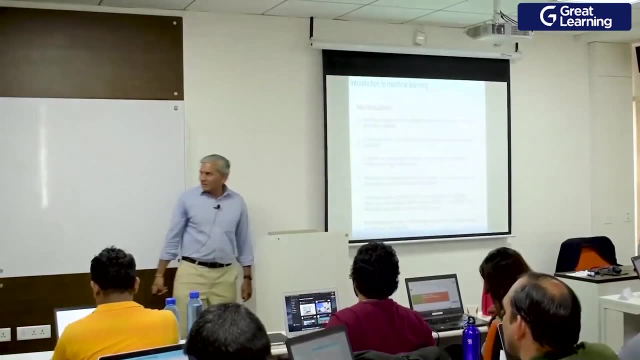 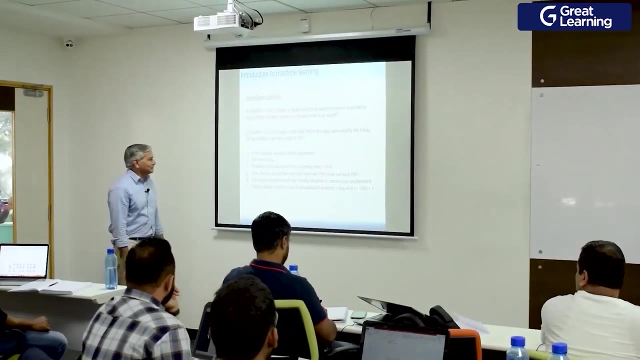 So we talk about conditional probability only when we have joint probability greater than 0.. Alright, So let's see how all this was put into build a model. We already discussed this: What is probability, What is joint probability and what is conditional probability? 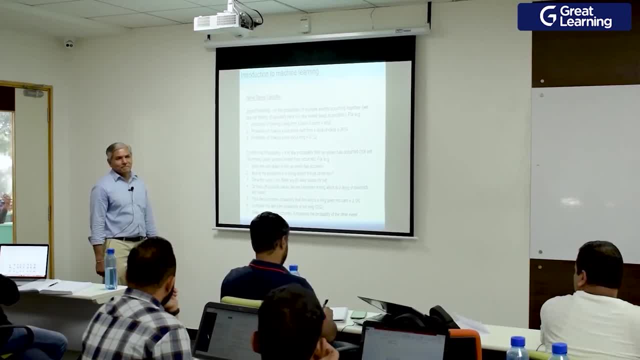 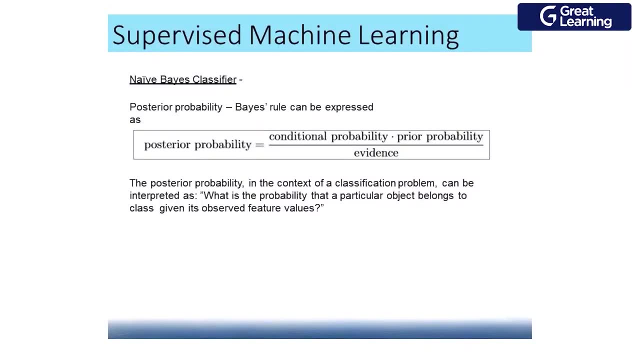 We already discussed this, So I am going to jump these slides. This is the model. I am sure you would have seen this formulas Looks very similar. Right, It is familiar. Wow, Wow. You should put it on some kind of board and put it on. looks like you are going to launch. 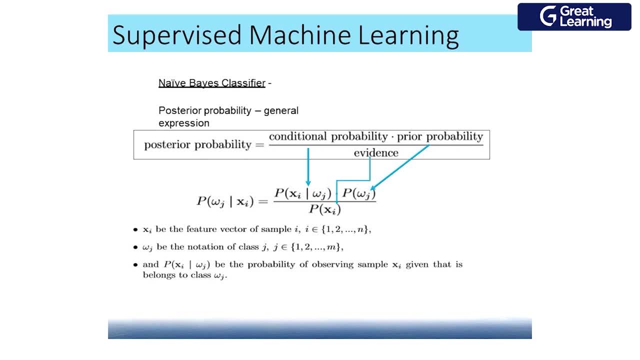 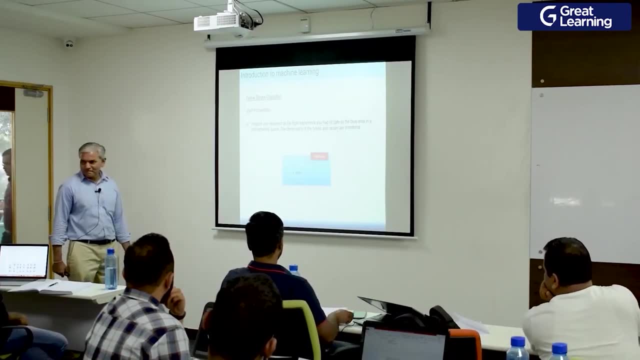 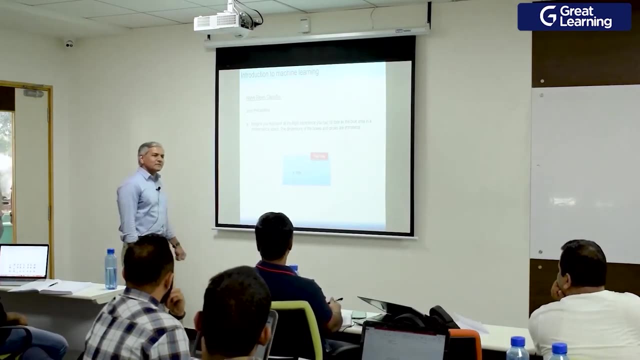 some rocket. It is very easy, Ok. So what I am going to do is I am going to jump all these slides back. I am going to explain with some animations. This blue box represents all the flight information I have captured from my experience. 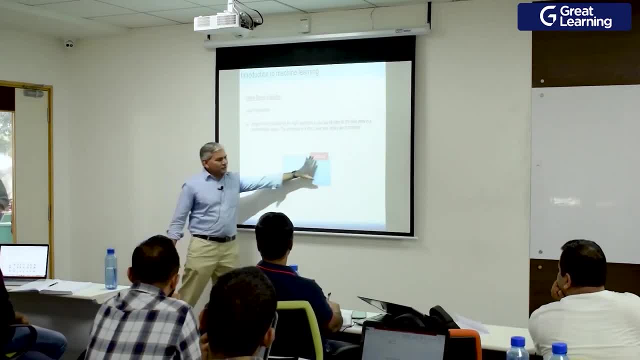 All the 100% flights which I have taken. I am representing it by blue box. The dimensions of the box are inconsequential, they don't matter. When I look at my past data about the flights which I have taken, I notice that 20% of the 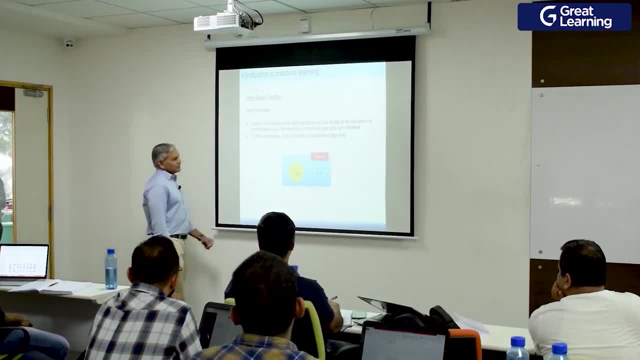 time there was flight delay, 80% of the time the flight was on schedule. In mathematics in school, you would have done this as Venn diagrams. Ok, Ok, Ok. So this is the information, past data- that 5% of the time there was fog at the airport. 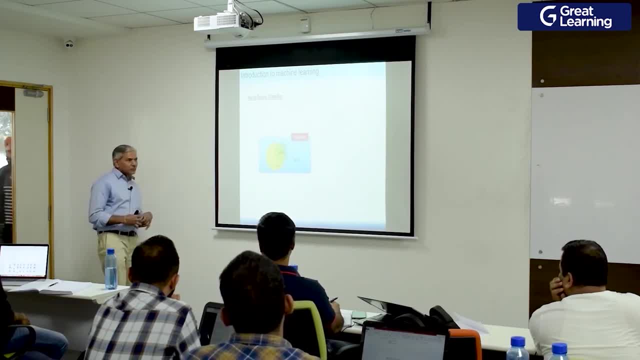 Now it will be. it is natural for us to quickly link fog with the flight delay. Don't do that. We are not here to say that the flight delay was because of fog or fog was because of flight delay. We are not here to establish that link. 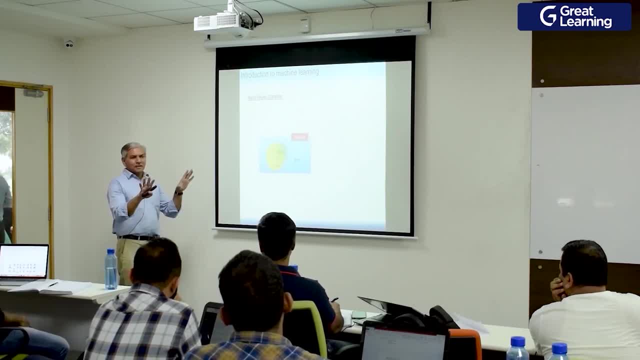 Naive Bayes algorithm assumes that these two events are independent of each other. Whatever the reality may be, the algorithm assumes these two independent events are independent. Ok, They have nothing to do with each other, Ok, But we know through our experience that they are not really independent. 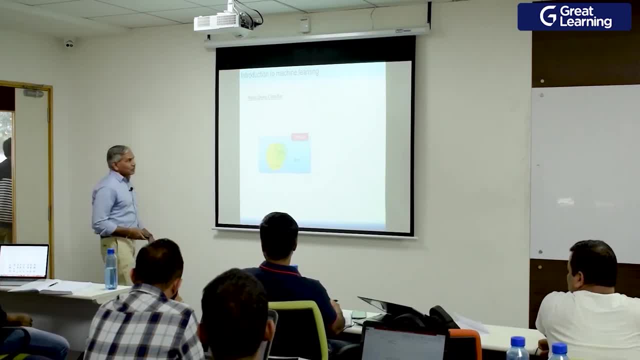 But the algorithm assumes they are independent. Ok, And we know that if I mark this as flight delay- no fog, this is fog, but no flight delay this crescent. This is the case where flight delay and fog occurred together. That does not mean flight delay led to fog or fog led to fog. 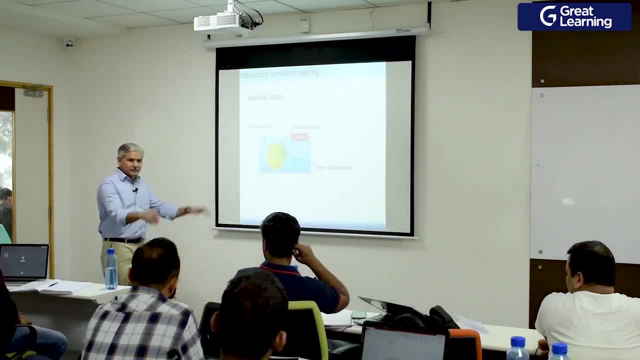 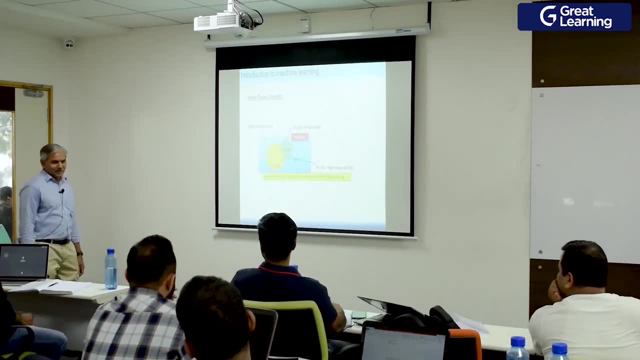 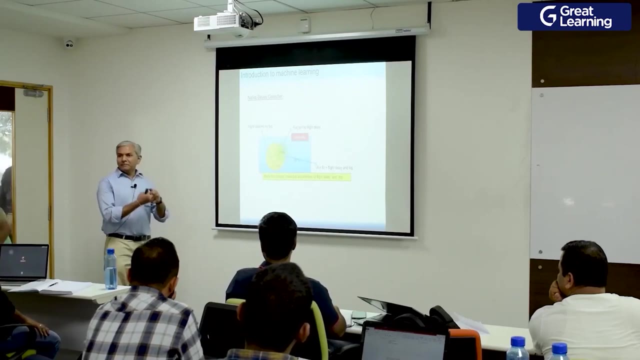 We don't know. We are assuming that they are independent. What is going to happen is: the lesser the overlap, more unlikely they are linked, The more the overlap, more likely the two events are linked, they influence each other. But I repeat, we are not here to establish any causal relationships. 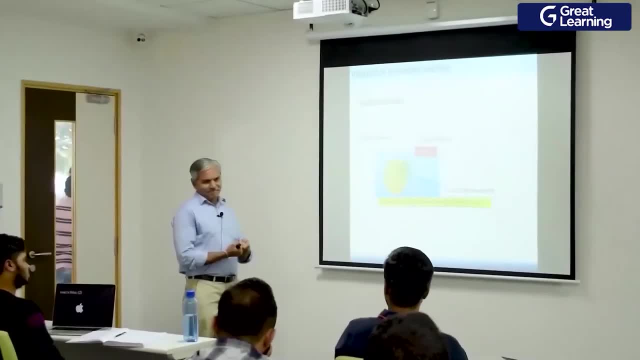 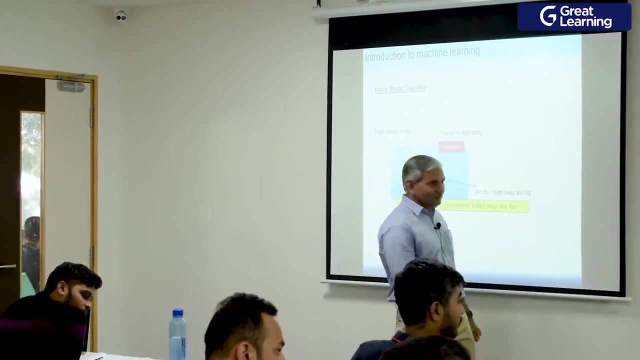 We are assuming that the two are independent, Sir you mean to say Suppose this, Suppose there is a strong relationship from our intuition that for a particular use case we found that there could be a strong relationship, then we should not use Naive Bayes in that. 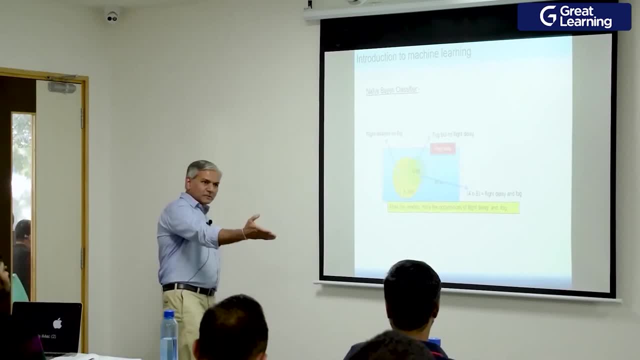 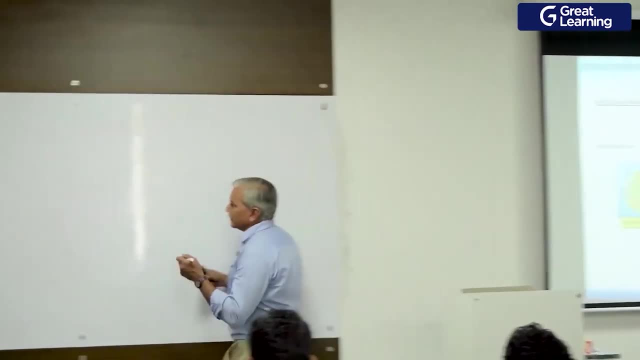 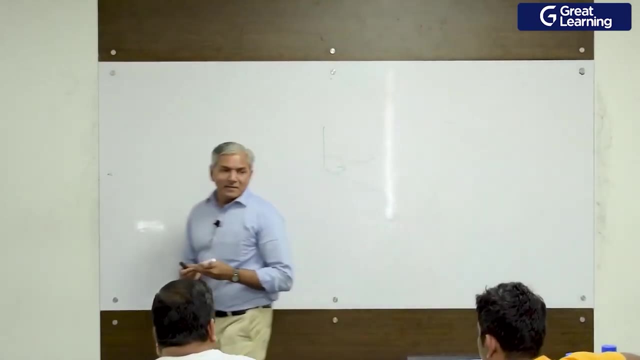 case Correct. We should not use Naive Bayes. All algorithms are like that. All algorithms show you the independent variables orthogonal to each other. That means they are independent of each other. Mathematically, when two things are independent of each other, they are shown at 90 degrees. 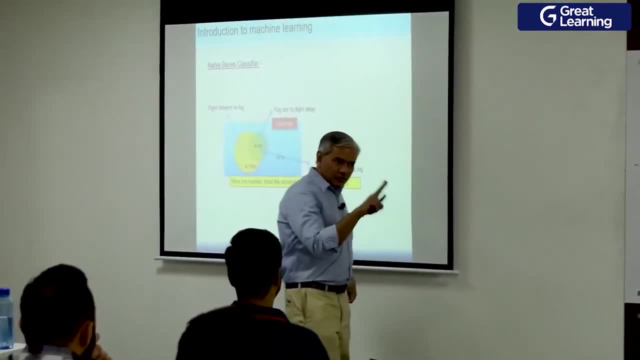 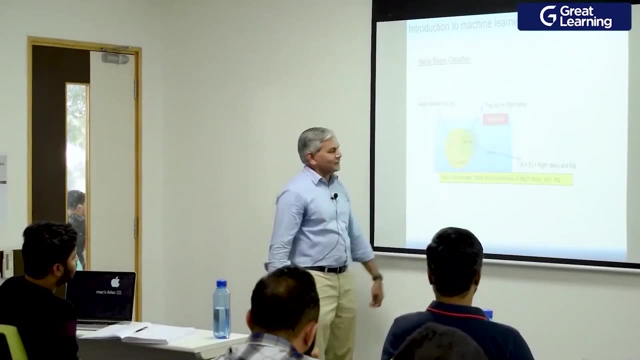 Ok, Ok, Ok, So the two values are very strongly influencing each other. You have to replace them with one synthetic dimension, PCA, or drop one. You have to do that. Same thing applies here also. Shall we move on, Ok. 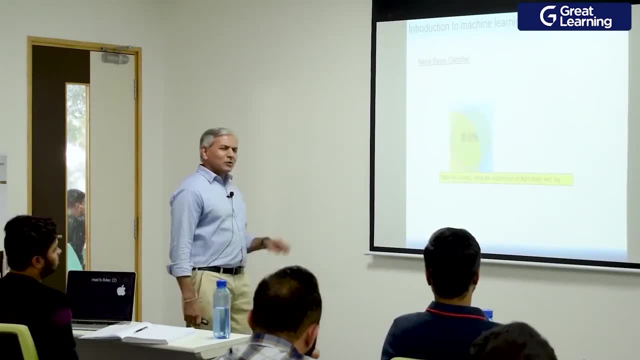 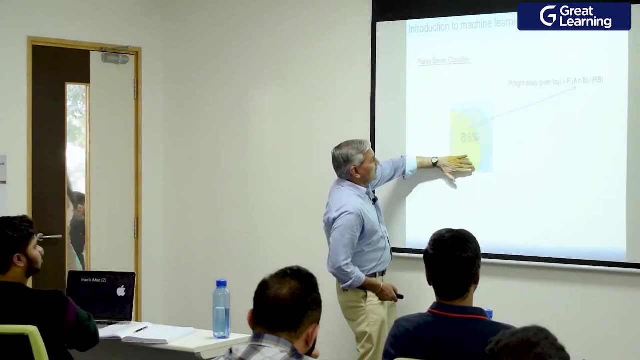 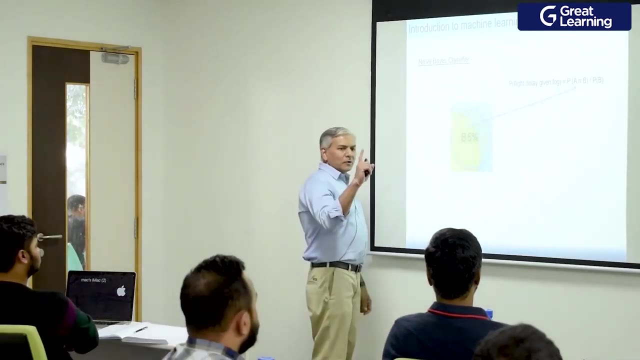 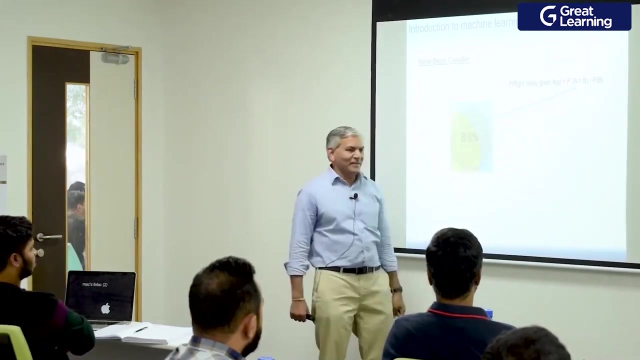 Now look at this. Let us look at this region closely. This region is the intersection region. Ok, Probability of flight delay and fog, the two events, the joint probability- Ok. Now I told you I want conditional probability. Now that I am seeing fog at the airport, now that the card is a red card, what is the probability? 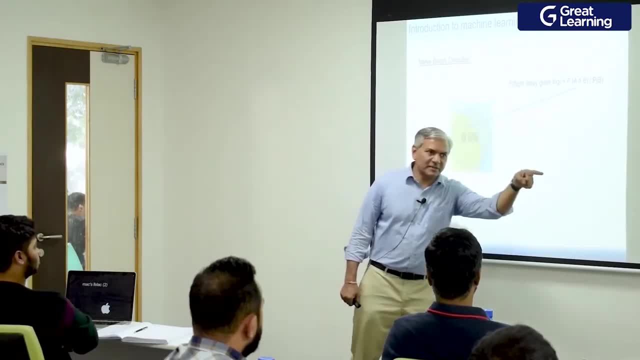 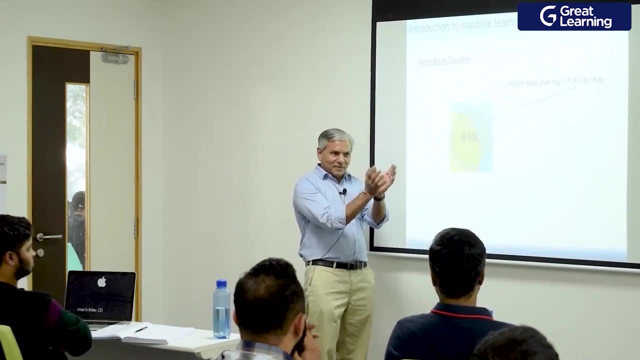 there will be flight delay. Now that it is a red card, what is the probability? it is a king. So what happened? Your Bayes, which was earlier 52, it shrank to 26.. Same way here. Now that I am seeing fog at the airport, what is the probability? the flight will get delayed. 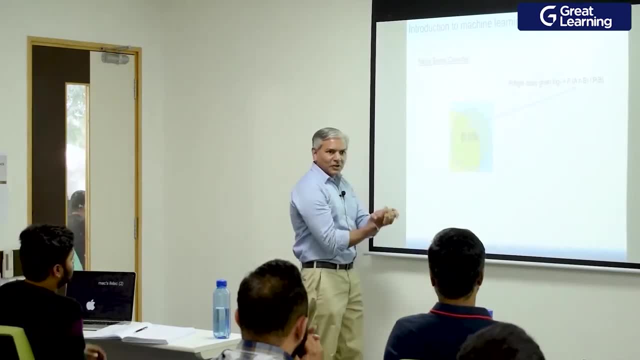 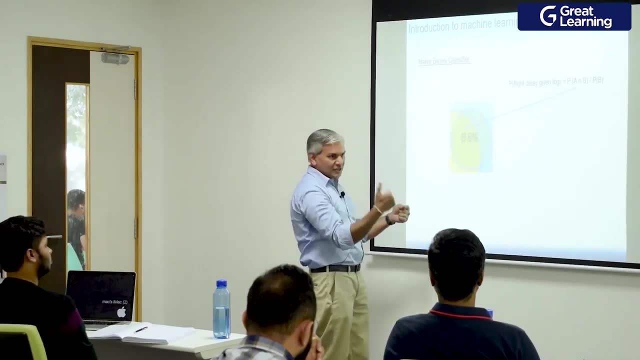 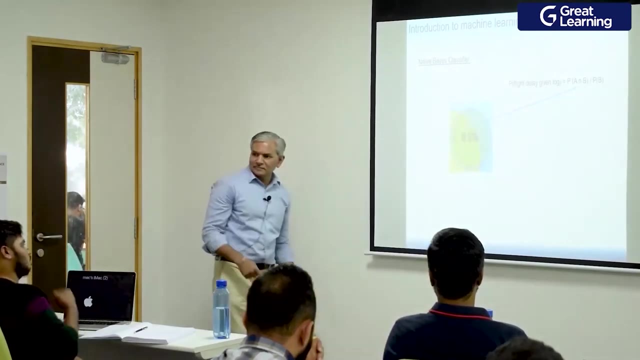 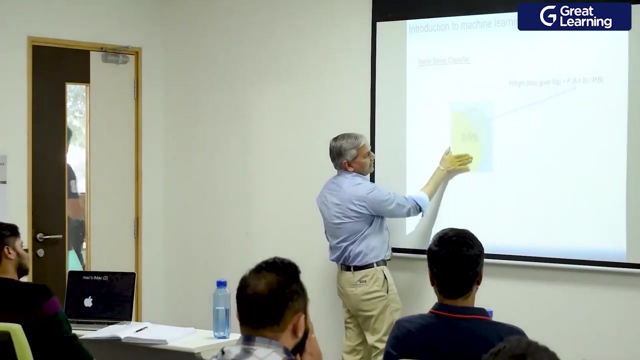 So the Bayes becomes fog, Ok, And the numerator is this area. So probability of flight delay given fog, the conditional probability is this intersection area divided by the blue. So if this is red cards, this is red king. these are the other cards. 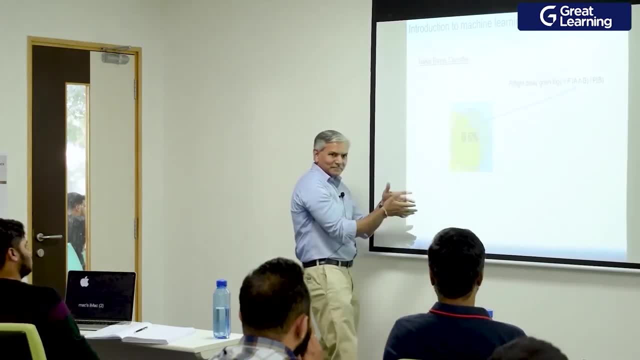 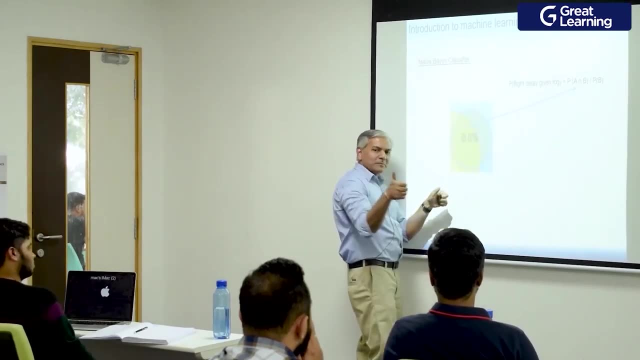 So what is the probability of red king? It was 2 by 52.. Ok, Now that I know it is a red card, that means this is not my Bayes, this is my Bayes. What is the probability it is a king? 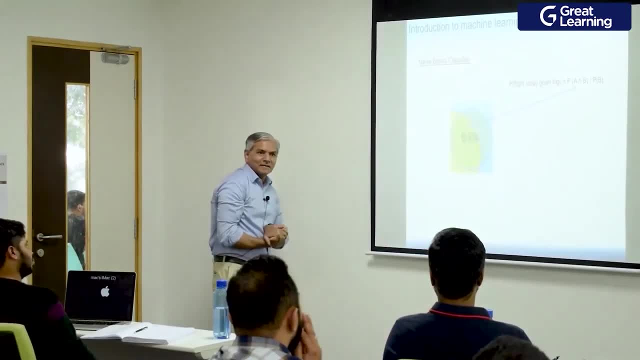 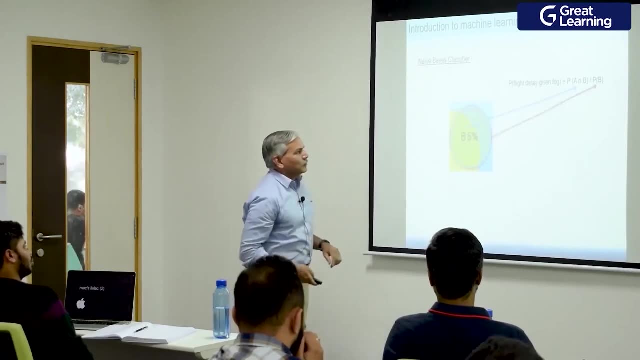 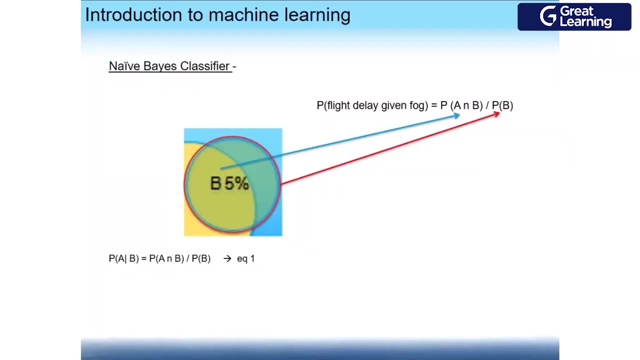 Numerator by denominator. All right, All of you, ok? Ok, Let us move further. I am going to write this equation on one side and play around with this equation a bit. Caution, Ok, Caution, Be ready to slip. 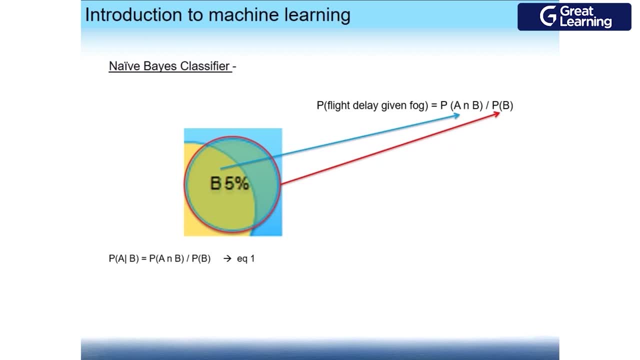 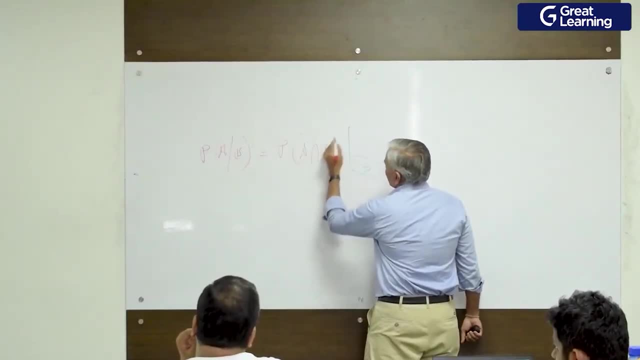 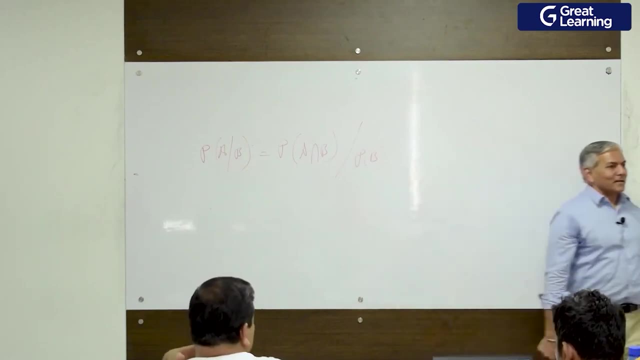 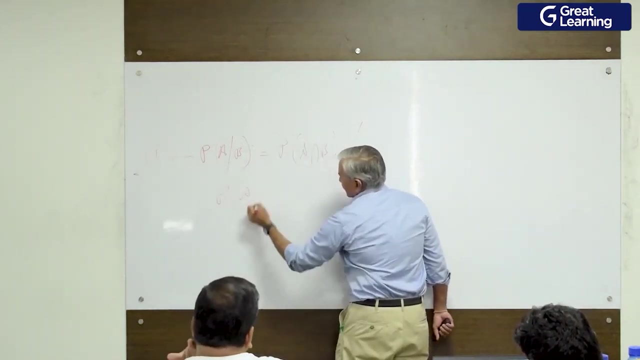 So P A, condition B. this I am showing it here as P A intersection P by P V, A intersection B by P V, All of you? ok, Can I rewrite this equation? and rewrite this equation one as P A, condition B, intersection B by P V? Ok, 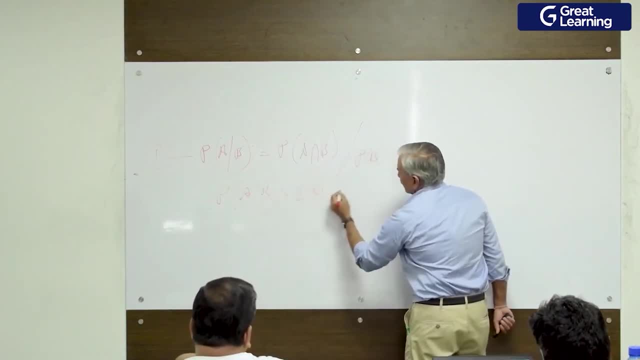 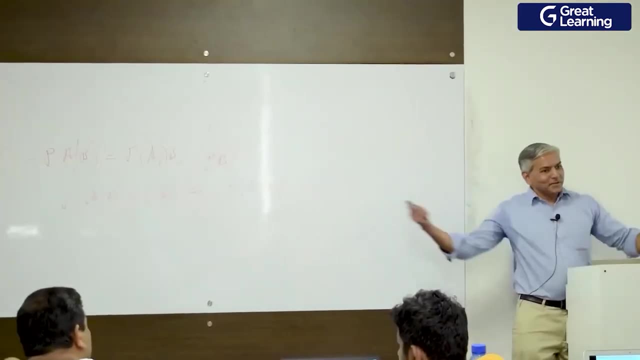 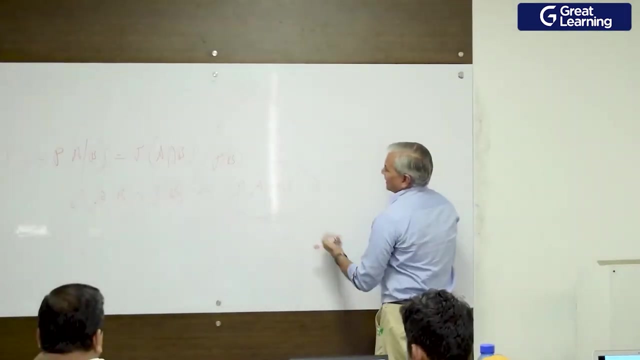 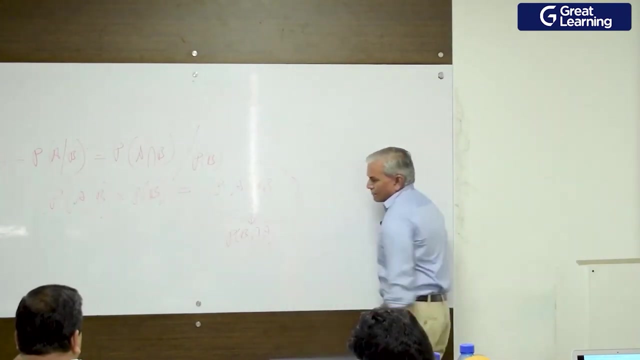 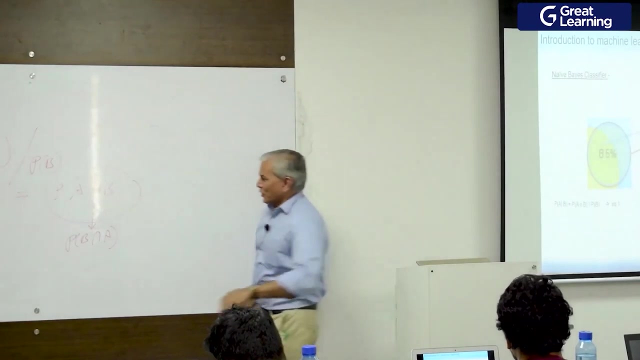 P B into P B is equal to P A intersection B. Can I do this? Can I do this? All of you? okay? Okay, Look at this: P A intersection B. Does it make any difference whether I write this as P A intersection B or P B intersection A? Does it make any difference? Okay, If P? 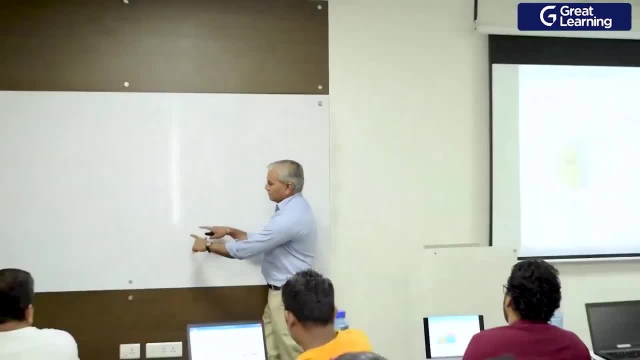 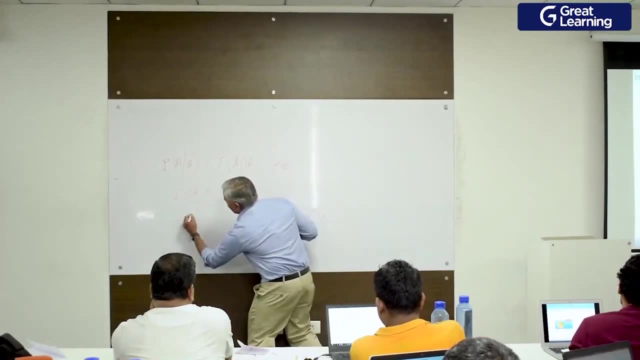 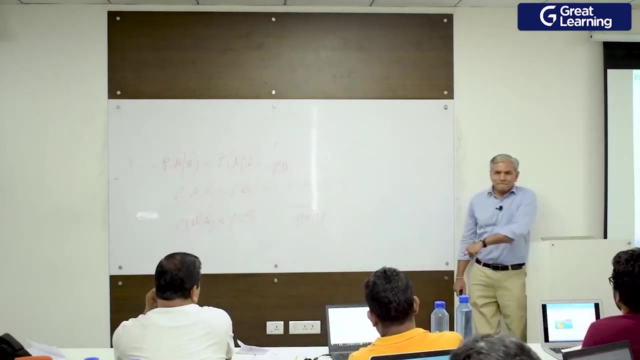 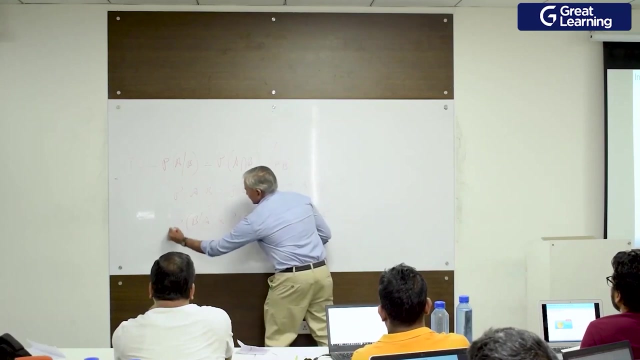 intersection B. is this then P B? intersection A, where the denominator, the numerator is changed and denominator is changed, it becomes P B given A into P A. Okay, I take this expression and I put it over here. So this conditional probability, 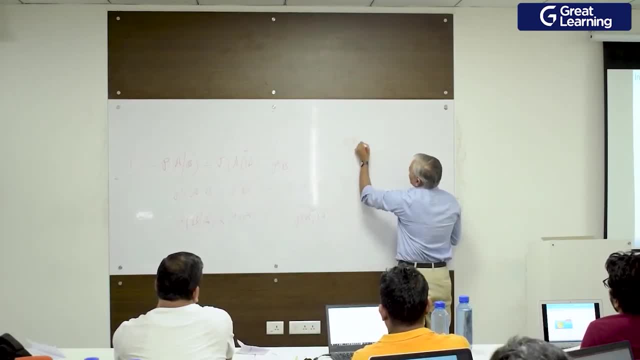 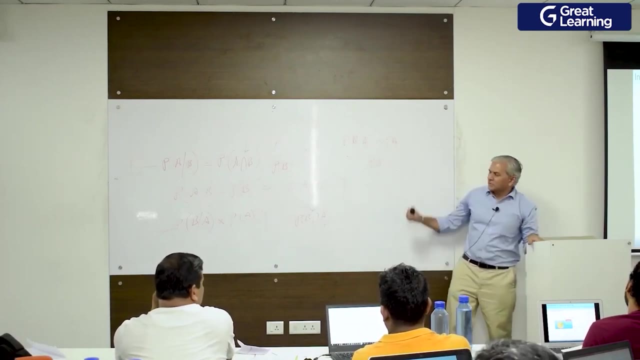 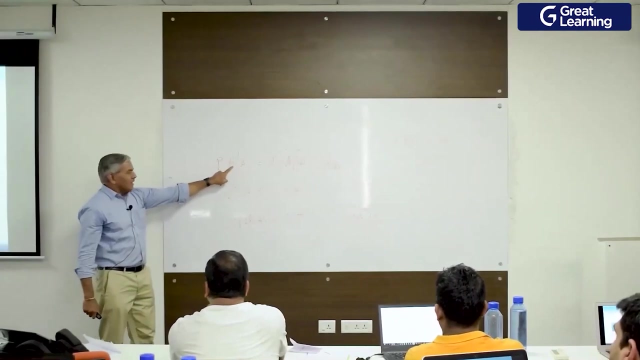 becomes P A. intersection B is P B given A into P A divided by P B. This is your Bayesian model. I will tell you what it means. This is all algebra, but let us understand what it means. What is the probability of a person being diabetic given the conditions? So this is the class: diabetic: non-diabetic. 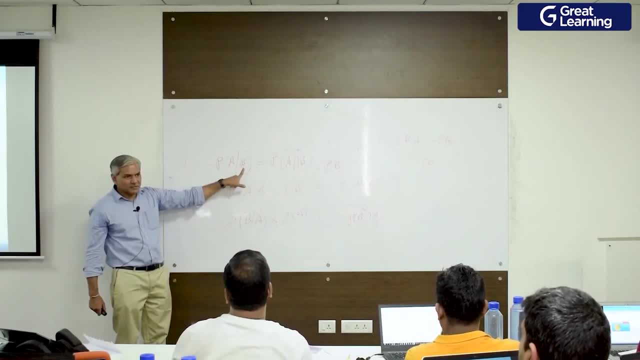 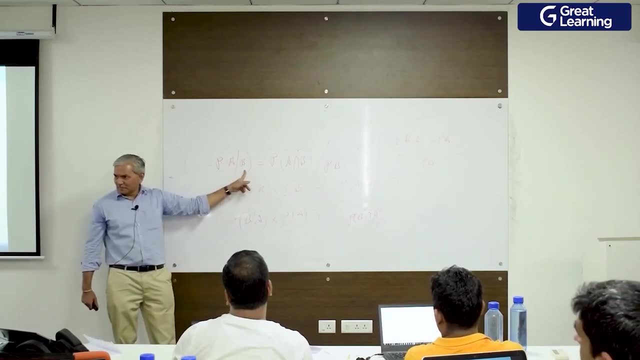 These are the independent variables: the BP, the plasma and all these things. So what is the probability a person is diabetic, given the conditions? What Mr Bayesian said is, instead of building models, go back to your data. From your data, pull out all those records. 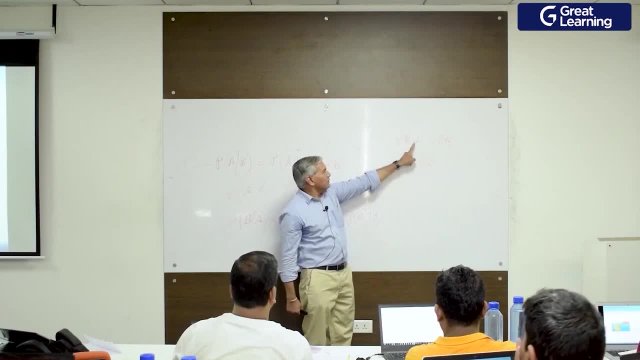 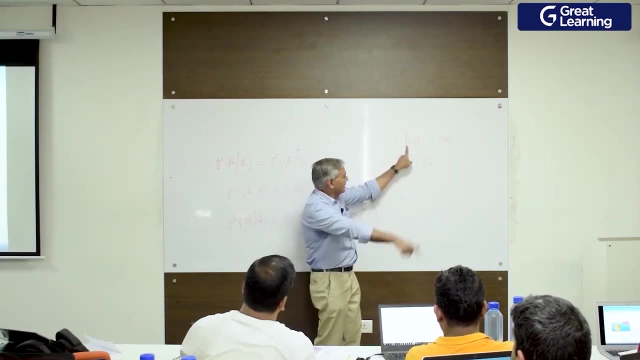 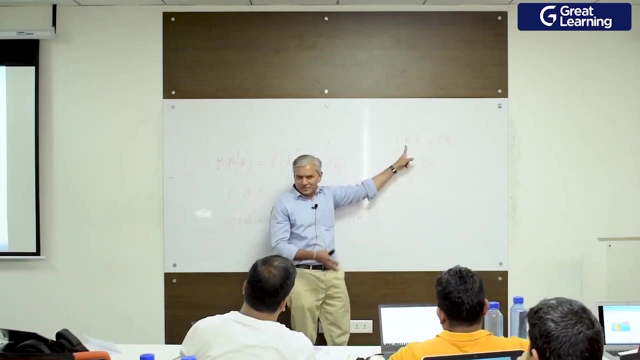 where people were diabetic. How many of them had these conditions. This is called likelihood ratio. Go back to your data. From the data, pull out all the diabetic cases. How many of them had this condition? So, instead of building models, do this Likelihood ratio. 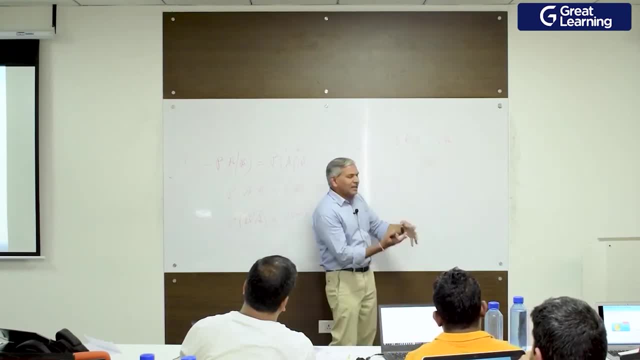 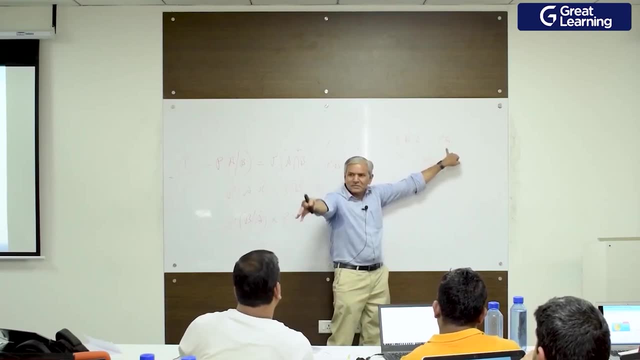 Multiply that with what is the probability of anybody in the population having diabetes. So this is the base probability. What is the probability it is rain today? 3.5.. 3.5.. is the probability of rain today? 0 percent based on past experience. and this is that. 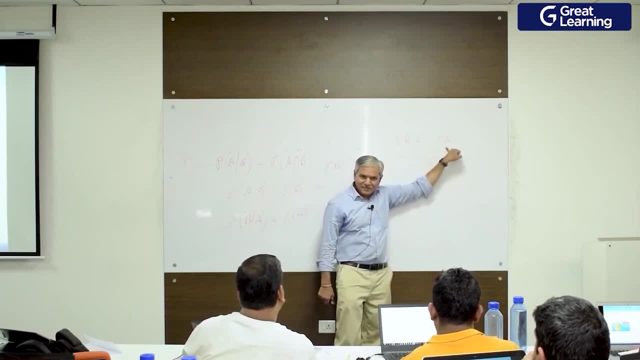 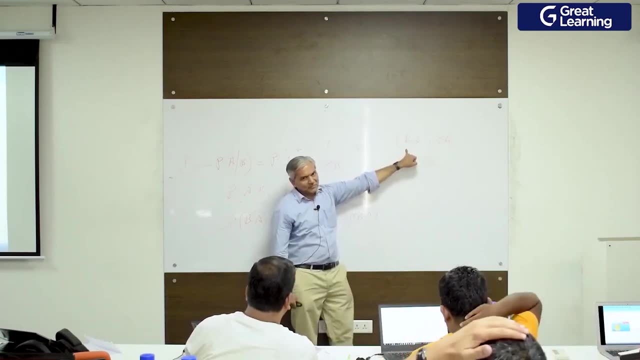 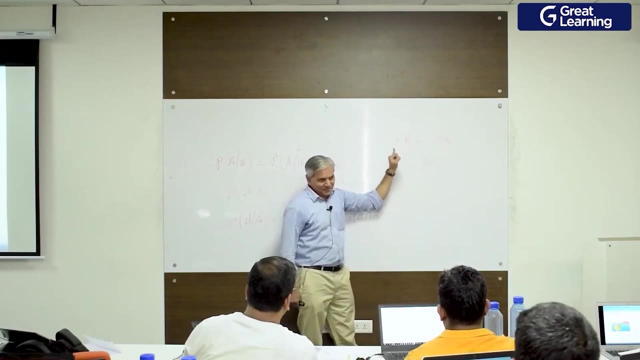 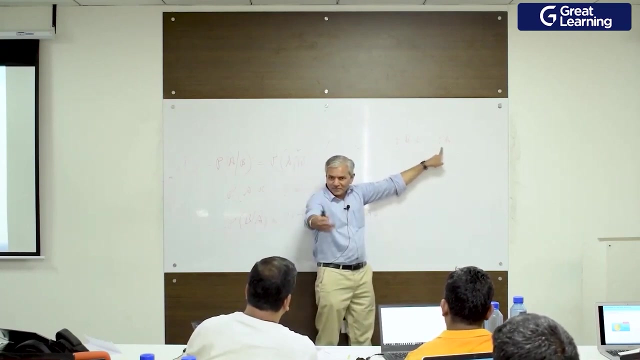 probability. Recalibrate this using this likelihood ratio. What is the probability of red king? 2 by 52. We modified that into 1 by 13. that is recalibration. that is what this numerator is doing. So this is called likelihood ratio. Prior knowledge: you already have knowledge. 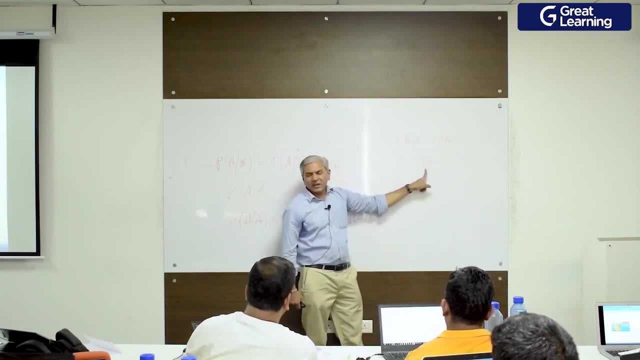 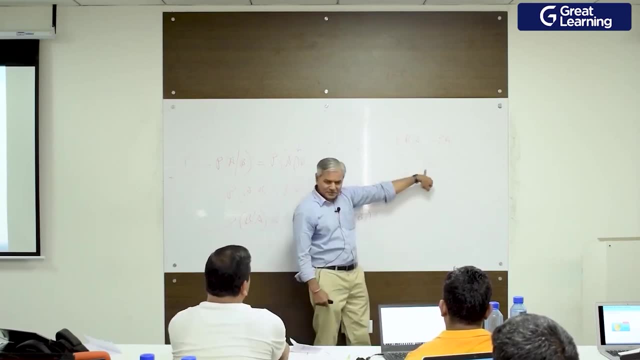 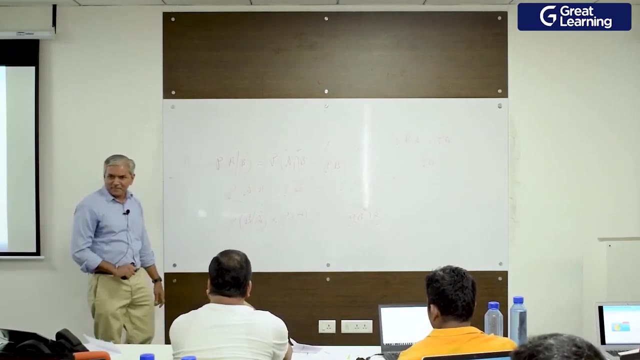 about this ratio in the universe, and this is called evidence. I am seeing this occurring. Given that it is a red, I am seeing that occurring. This is evidence. So the argument which Mr Bayes put is very simple. He did this 200 years ago. He said that instead of trying, 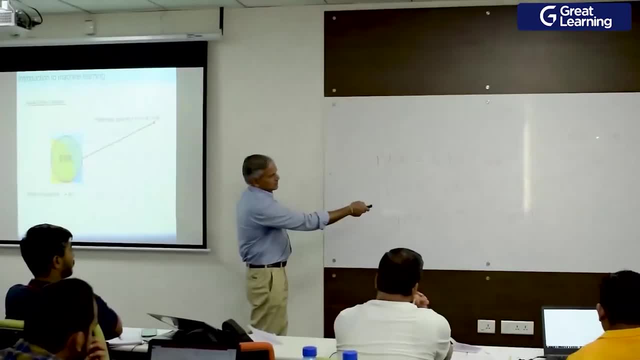 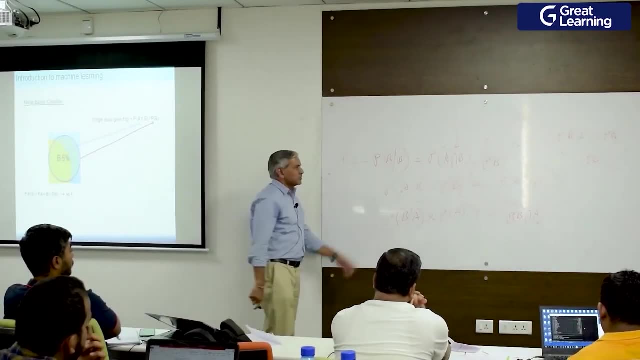 to build a model for this. go back into data. pull out all the cases which satisfy the condition, which are diabetic, belonging to that class. How many of them had this? 20. Conditions which you are seeing today. That is all to this model. So this model, this, 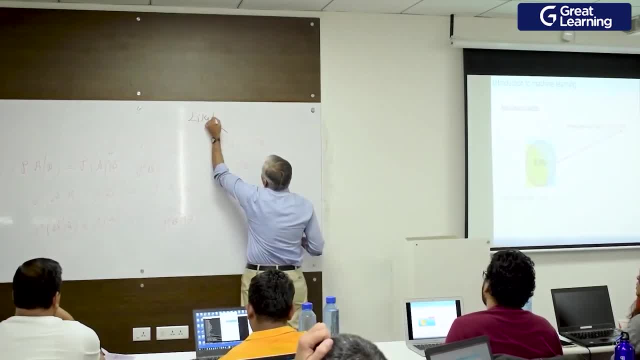 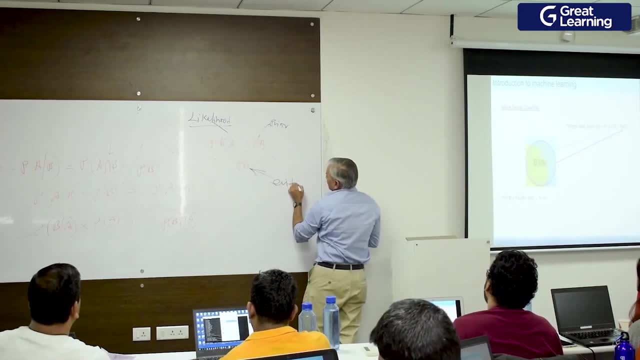 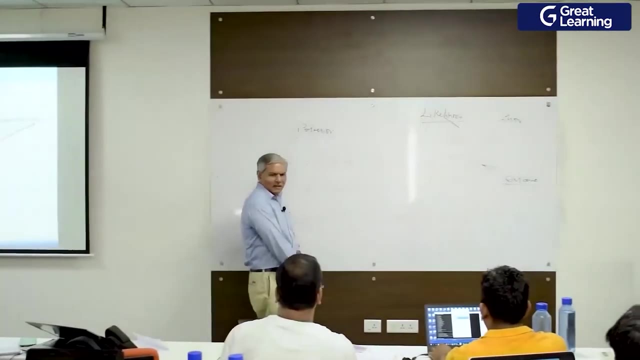 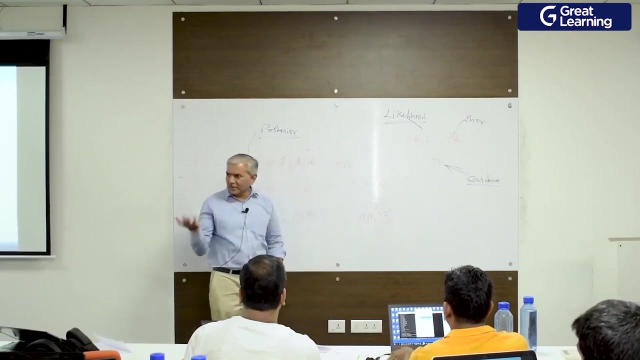 is called likelihood, This is called prior, This is called evidence and whatever you come out with this is called posterior, and we do this in common sense. I will give an experiment to you. Are you all ready? Yes, We actually use Naive Bayes in our day-to-day life. Lakshmi, is it going to be male or female? 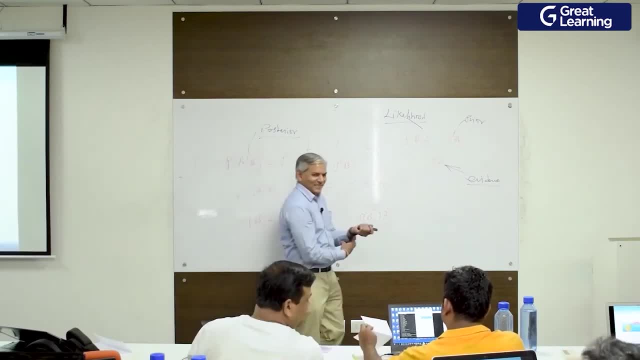 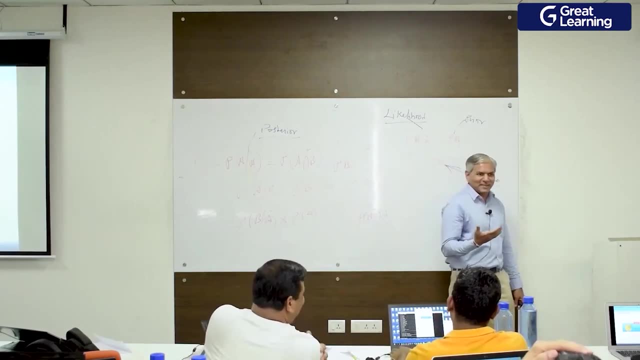 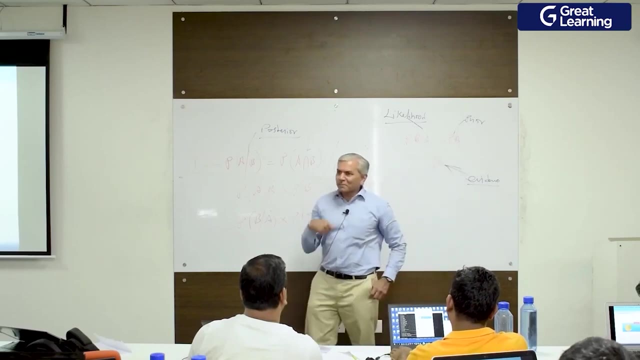 Male or female. Lakshmi is the evidence. now, Is it going to be male or female? Male or female. So what you are doing is you are going back to the past. how many times you have come across this name where it was a female versus where it was a male? 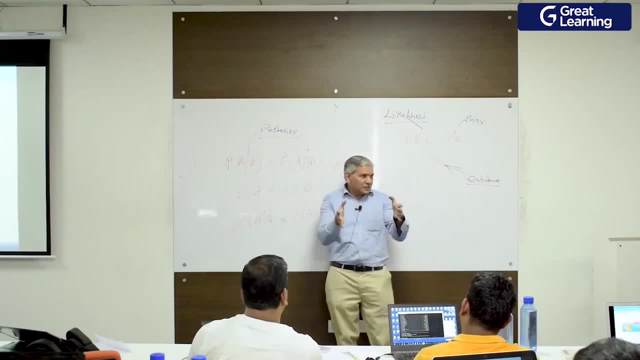 So you are pulling out all the past Lakshmis that you have in your mind. How many of them were males, females? That is Bayesian probability. I have a friend called Lakshmi Narayan Babu, and this one particular name I will not forget, because there was one class which I was supposed. 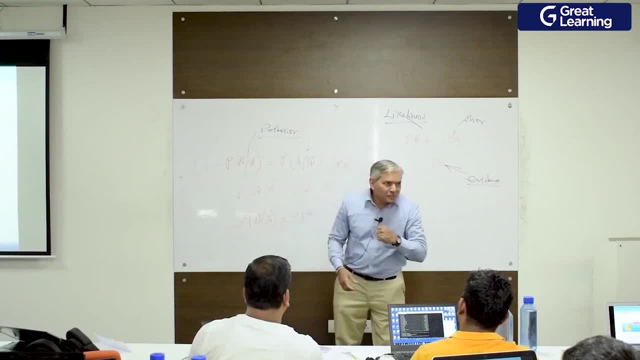 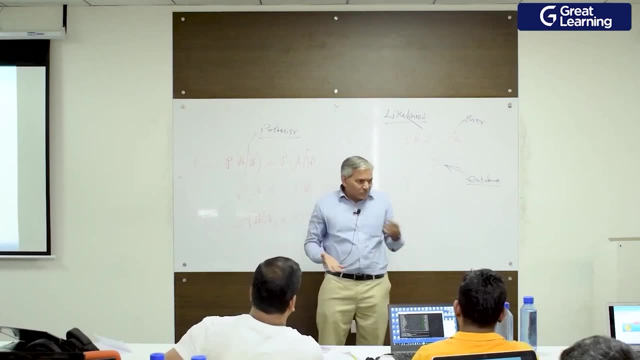 to attend and the class was being taken by Lakshmi. Every door I opened, there was a male standing there. Every door I opened, there was a male standing there. So it took me some time to understand that this guy's name was Lakshmi. 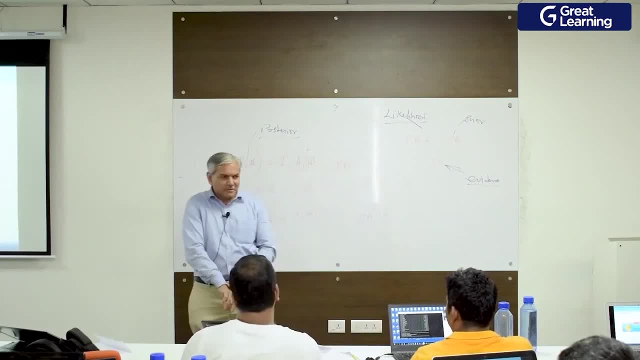 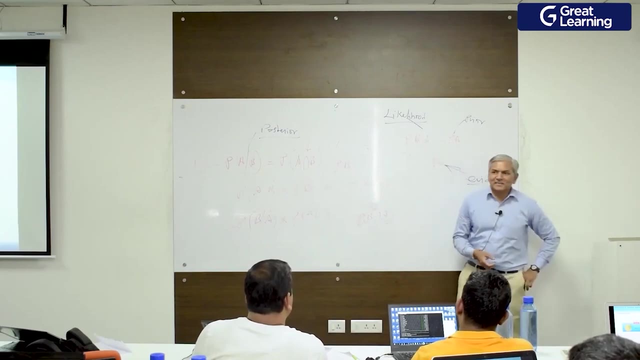 So I did a wrong interpretation. Lakshmi means female, but there are people, males, with name of Lakshmi. So what you have done to answer this question is Bayesian probability. So it all looks strange, but we all use it in day-to-day life. 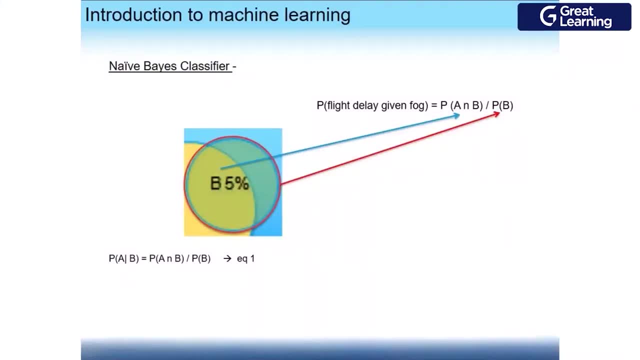 Shall we move on? Any questions on this? That is basically the first thing to do while you are in Texas. Yeah, This one, this one will give you that. That reminds me. Ok, So before I move on, when you read about these algorithms in books and articles you need 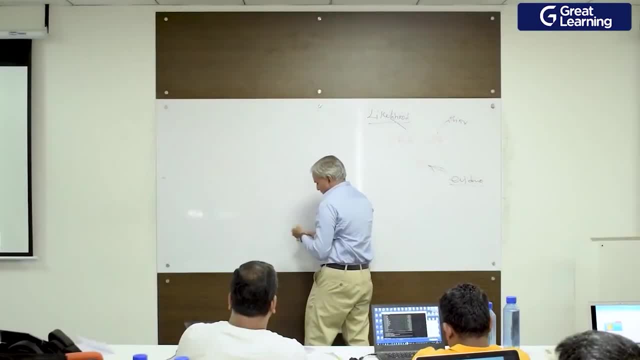 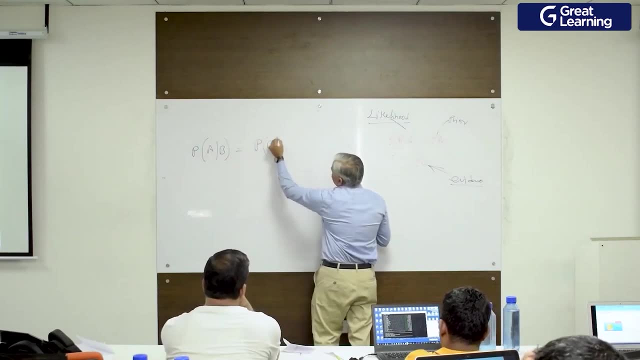 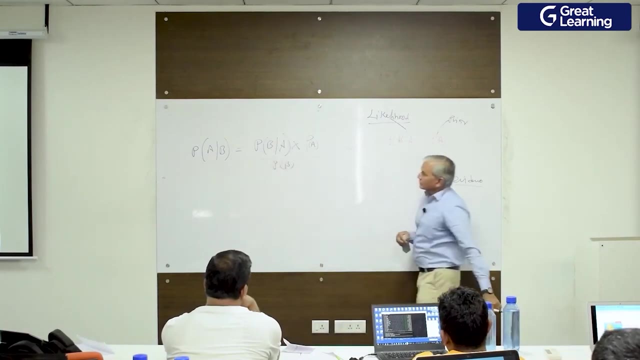 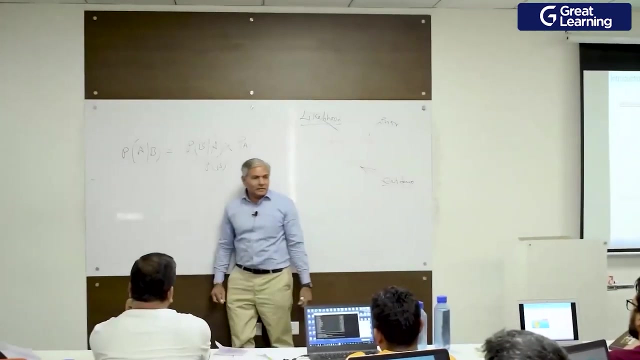 to be slightly careful, So let me explain what the problem is. So what happens is: what is the probability of A given B? is equal to probability of B given A into P A by P B- alright, Many of the authors. So what is the probability of not A given B? 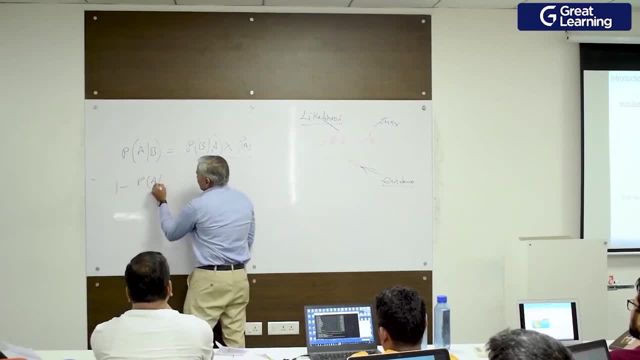 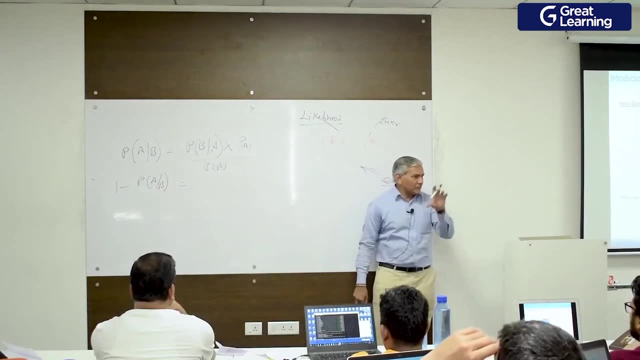 So what are these probabilities? 1 minus P, A given B. ok, So this I can write it as all of you understand what I am doing: Probability of A given B. probability of king given red. What is the probability of not king given red? 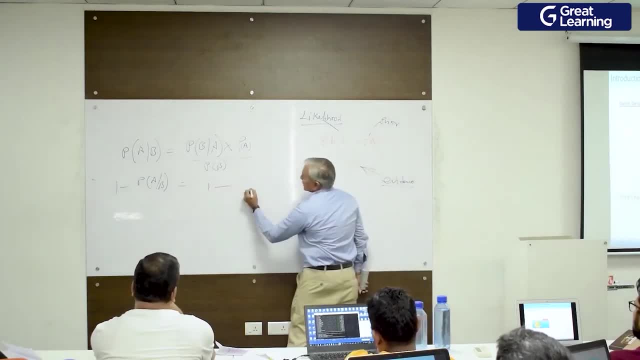 That is what we are doing here. So this: I can write it as P B, given A into P A. Ok, Ok, Ok, P A by P B, which can be further written as P B by P B. Agreed, All of you, okay. So whether? 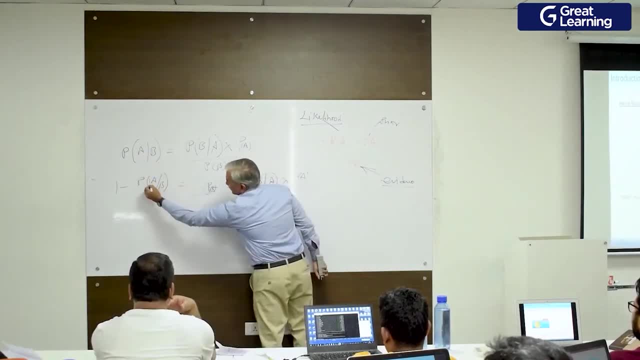 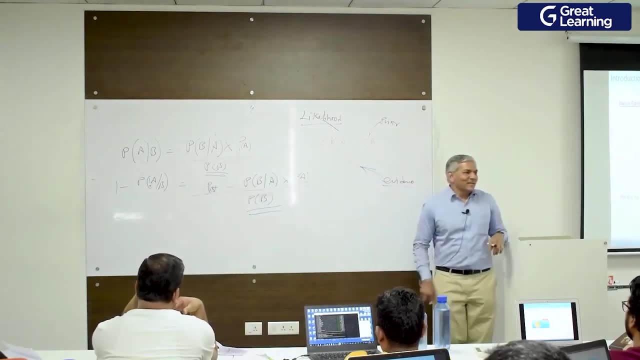 you are finding probability of A given B or not A. I will put it as like this: not A given B. both of them have in the denominator P B. So it is not P B which is going to decide whether this is going to be class A or class B. What is going to decide whether it is going 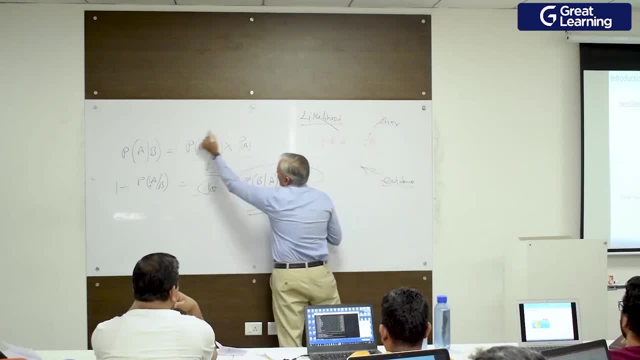 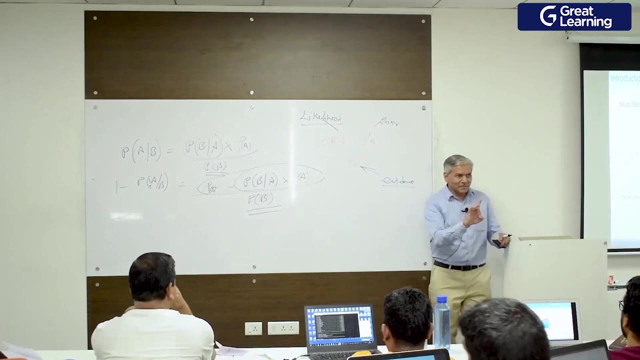 to be class A or class B is the numerator, sorry the numerator. If this crosses 0.5, he is going to belong to class A. If this crosses 0.5, he is going to belong to, not class A. Get my point? So what decides your class is the numerator, not the denominator. 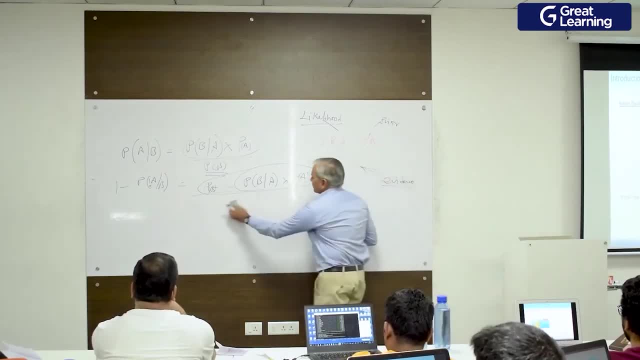 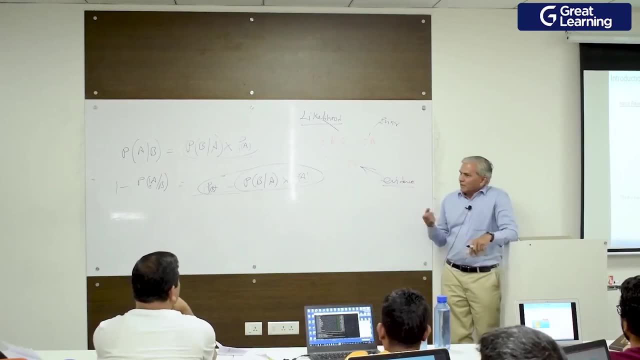 Denominator is same in both. So many of the authors. they do not reflect this. They say that this is the Bayesian model And you will keep wondering: where did the P B go? So the reason why they do not show P B is it is the numerator which decide the class. However, in case you want not the classes, 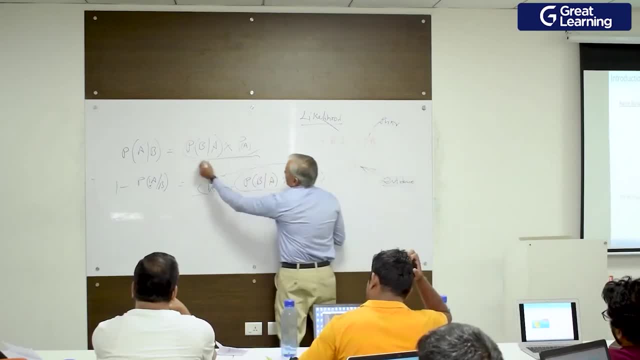 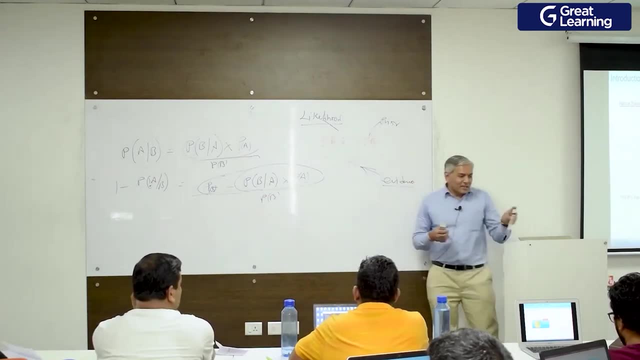 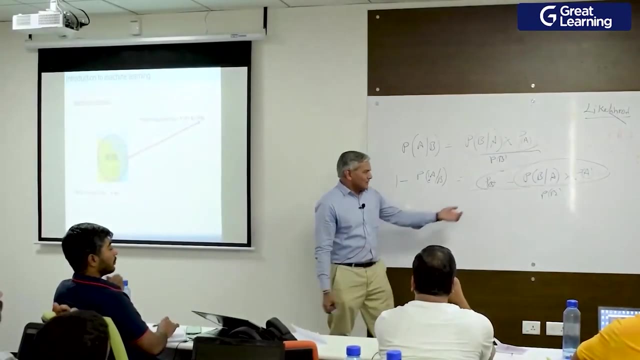 but the probability values. then you will have to divide the P B, All right, And the reason why they do not show P B. they often say that P B is a constant. What the hell? what do you mean by P B is a constant? P B is a constant. some people say that since 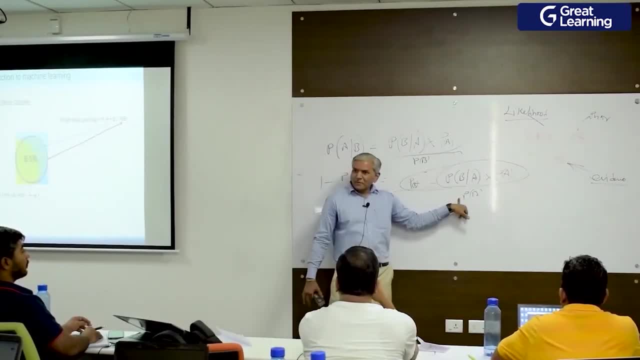 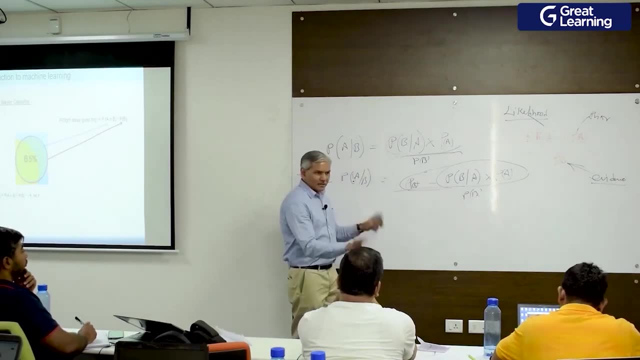 this is an evidence. evidence has already occurred. this is one. Probability of event which has already occurred is one. So there was that argument also. But the argument is mathematically for classification P, B is not important, So it is not shown All of 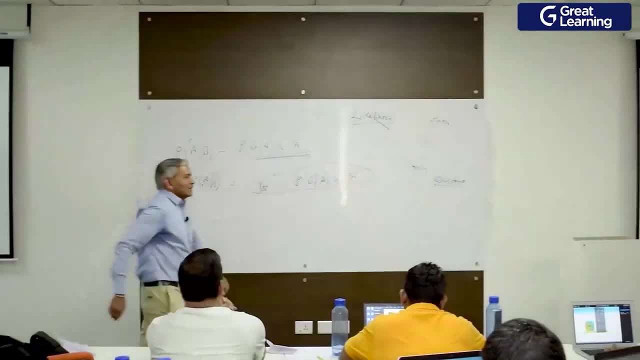 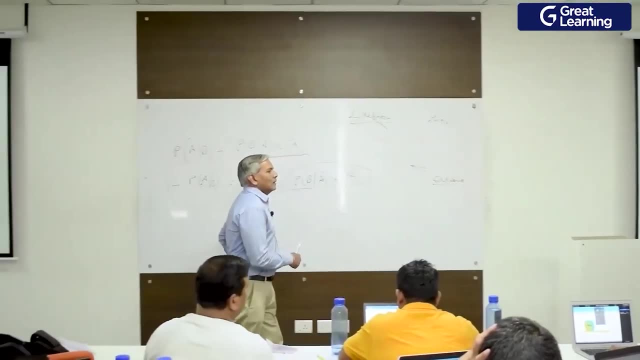 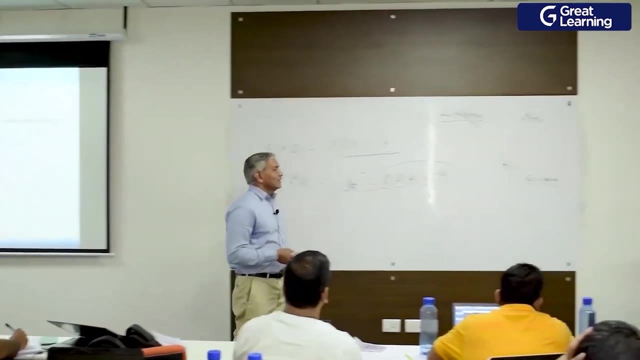 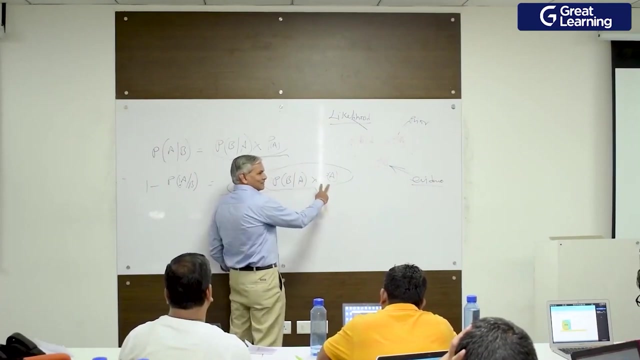 you okay, Okay, Thank you, Given evidence, given what you are saying, This is anyway. how many people in the population are diabetic? Yes, No, no, diabetic, Which symptoms we do not know In the population, how many are diabetic? 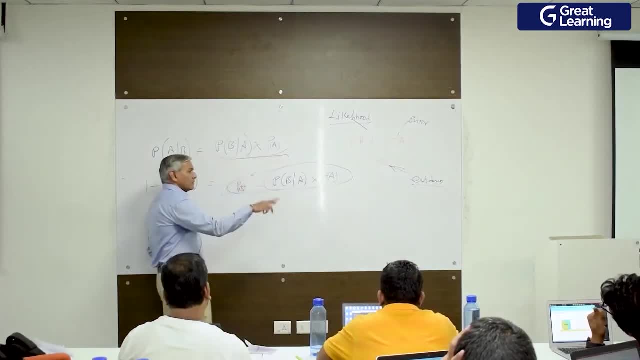 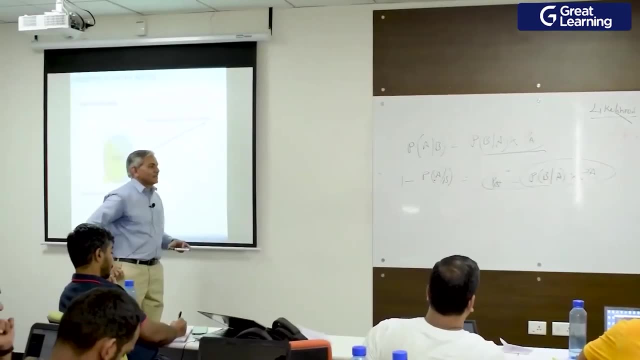 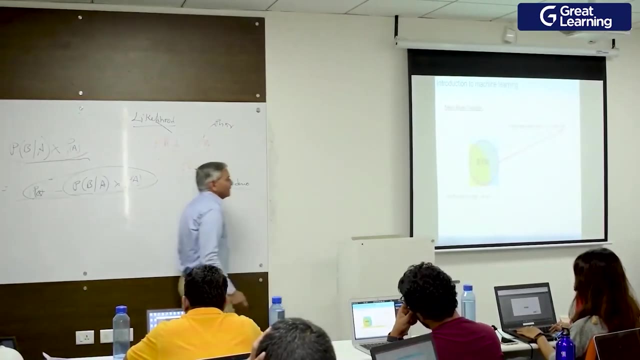 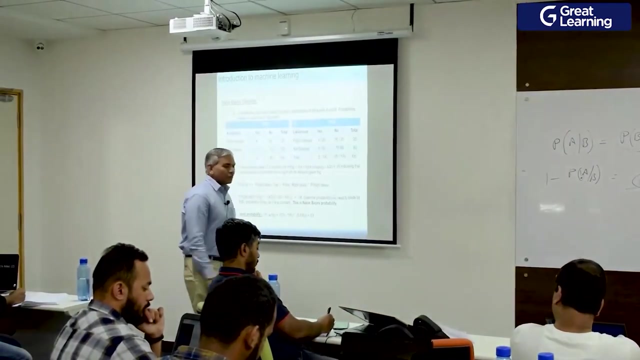 What percentage? That is this: How many are diabetic with this symptoms? Likelihood ratios. Okay, Now I will go back to the slides which I jumped, or should I go forward just one second? let me check. Yeah, I will go forward and then go backward. So I have my data set. This data set is 100 records. 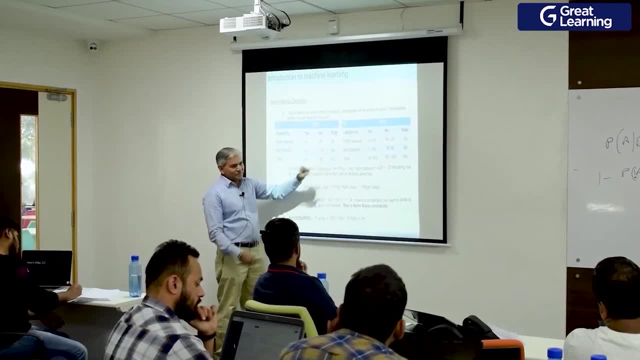 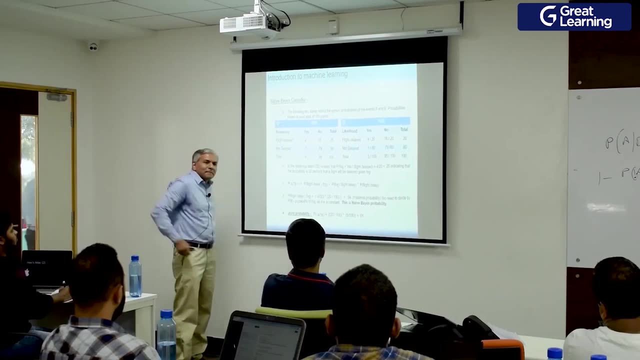 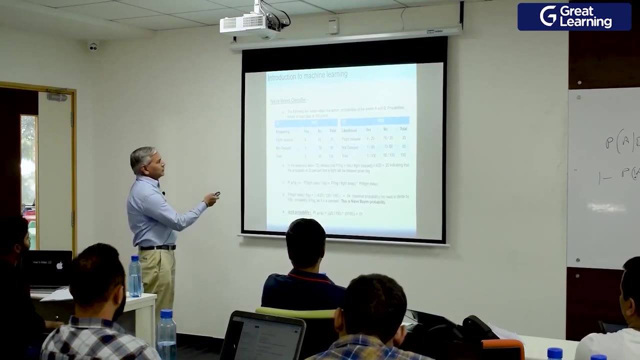 You see 100 in the bottom right. Total number of records is 100. Of this, 100 records 80 records no flight delay, 20 records flight delay. That is what I showed you in the Venn diagram. Okay, 20 times when there was flight delay I noticed 4 times there was fog at. 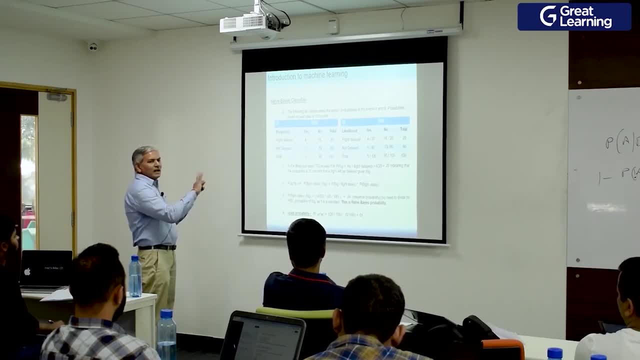 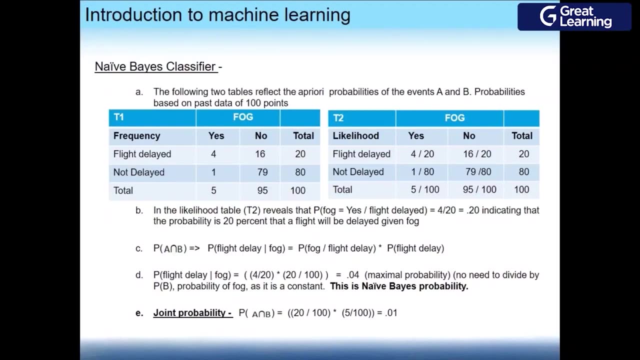 the airport. 16 times no fog at the airport. This is that overlap between fog and flight. I also noticed that 80 times when there was no flight delay, 79 times there was no fog and 1 time there was fog. This is the same Venn diagram which you saw earlier. Okay, 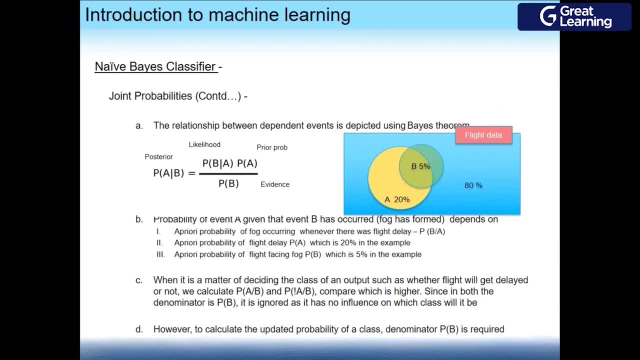 So, if you are getting confused, this area is no flight delay, no fog. This area is fog, no flight delay. This is 1 time which is occurring in my case. Yeah, This blue, the blue left out region, is no flight delay, No flight delay and fog. 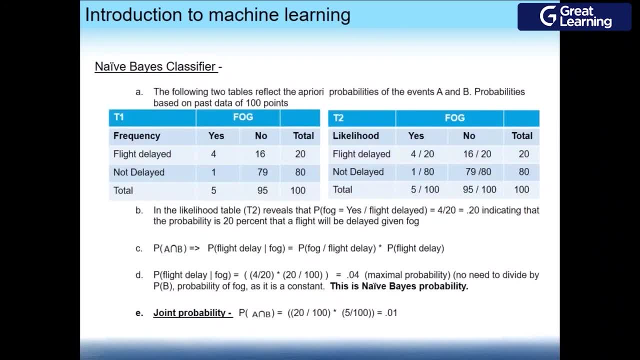 This crescent which you see here is this one: No flight delay and fog. is this? This is the crescent. Okay, We convert this into ratios: 4 by 20,, 16 by 20,, 1 by 80,, 79 by. 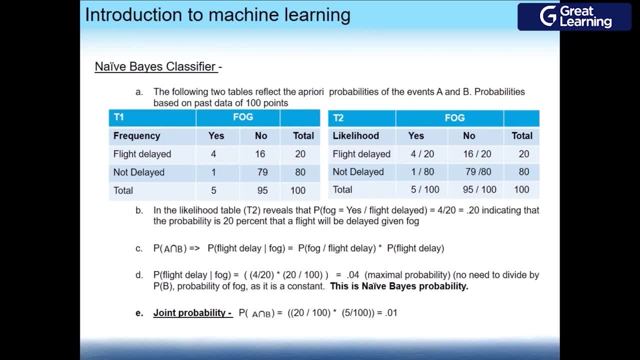 80. We convert into ratios the likelihood ratios. Now, once you convert into ratios, you can use any permutation combination to find the probability. This is what we have seen earlier. Okay, You can. you can put those ratios over here and 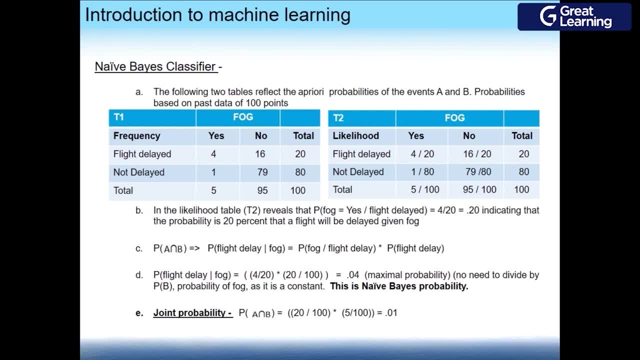 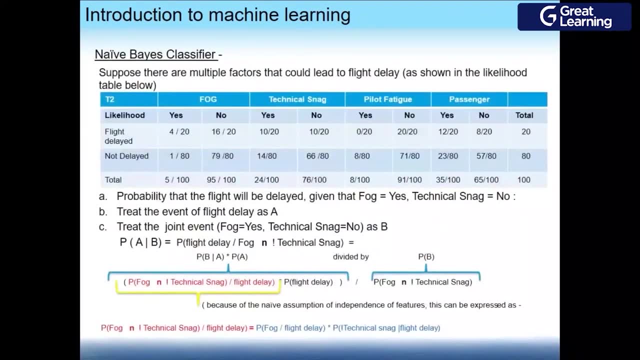 you see the calculations. Okay, What I want to show you is: I can extend this argument. I can extend this argument to include multiple parameters. Once again, I have only 100 records: 80 times no flight delay, 20 times flight delay. Okay, And these are the various events. 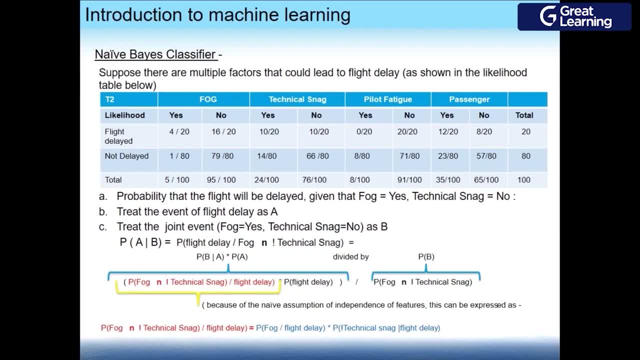 which I have captured. Okay, So I can extend this argument to include multiple parameters From the past. These are my attributes. So, 20 times when there was flight delay, 4 times there was fog at the airport, 10 times there was technical snag. Oh, what is this? Oh, 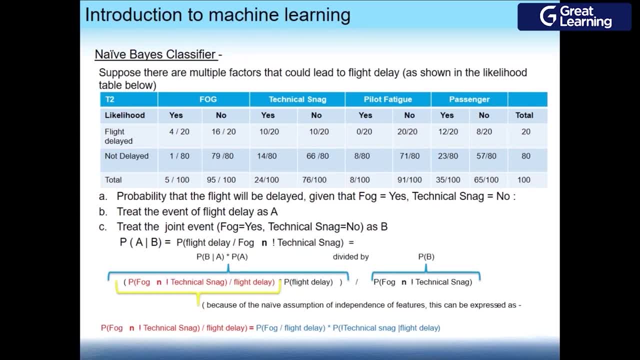 this: Okay. Yeah, 0 times there was pilot fatigue. Okay. So these are all my observations, which I convert into likelihood ratios. Keep in mind these don't have to total up to 20. They can be overlapping regions in the Venn diagrams. They don't have to total up to. 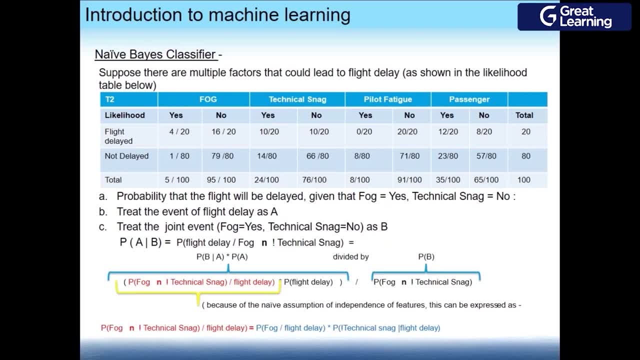 20. What I mean is, in the Venn diagrams these regions might be overlapping each other. Okay, So I convert everything into likelihood ratios. Now look at this Probability that flight will be delayed, given that I am observing fog at the airport, but no technical snag reported. 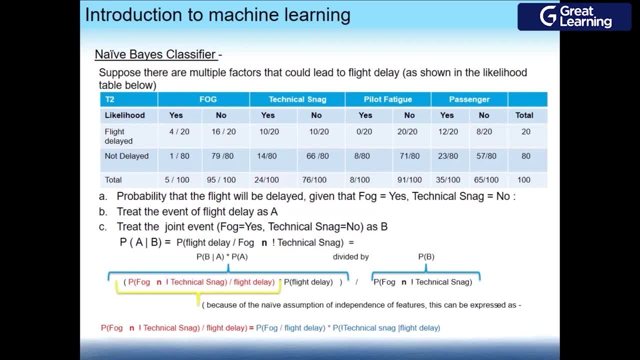 How do you find the probability that when I see these two events occurring, Use the formula: Treat the event of flight delay as A and the combined event as B. So it is again probability of A given B. Okay, P, A given B, It is nothing but probability of flight. 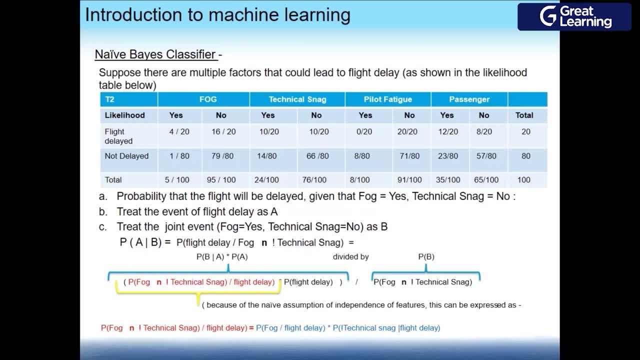 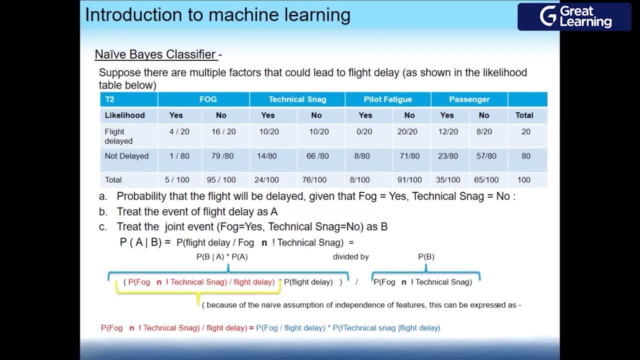 It becomes P B given A into P A. You are going back into your records and seeing how many times flight delay happen, how many times these two events occurred together in that records. That is what this expression is. The likelihood is B given A right. 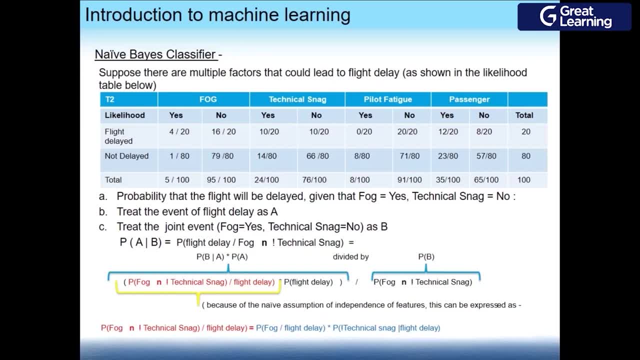 Ya, likelihood ratio correct. Yeah, likelihood ratio Correct. A- B is a compound event right now. So P given A is this: P A continues to be P A. That is nice. Who did that? Okay, Divided by probability of B, So you can form any. 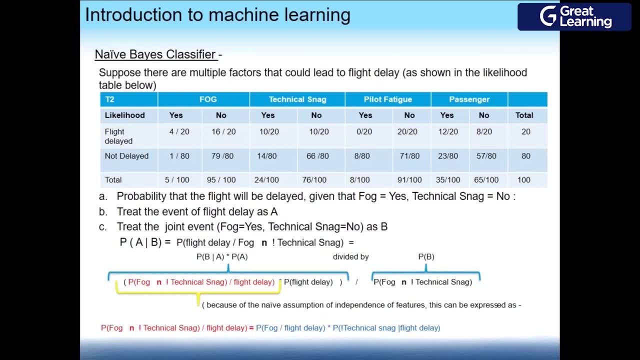 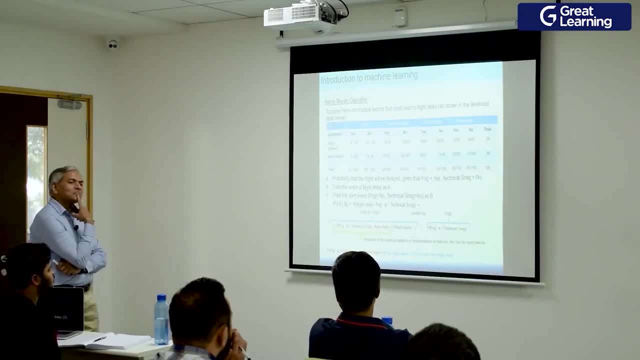 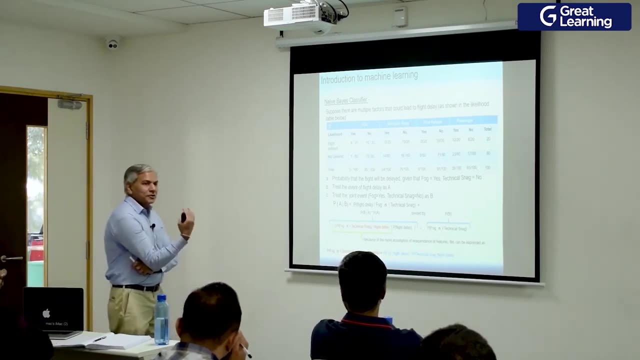 permutation, combination of these events and substitute into this equation of events and substitute into this equation over here the likelihood ratios and I will tell you the probability. What is the probability of flight delay? now that you are observing these events, So you can keep on recalibrating your probabilities? Forget flight delay. What is the probability? 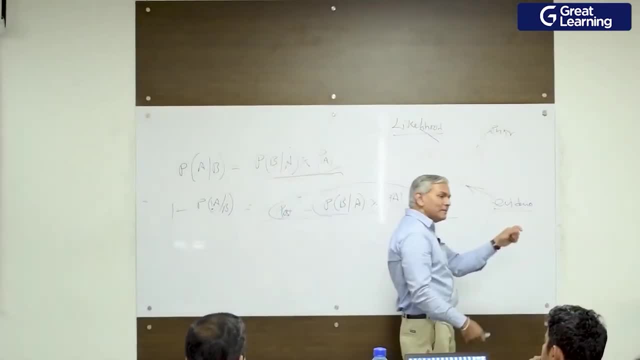 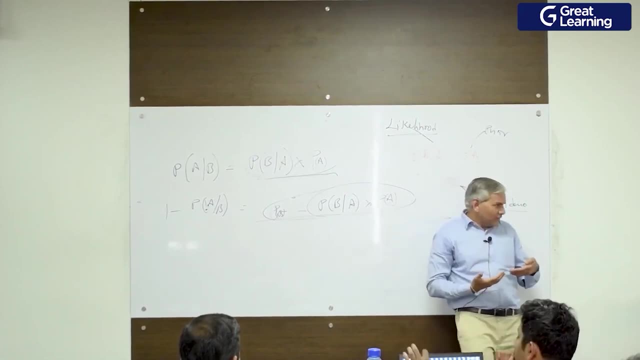 of an intrusion, network intrusion, given that I am seeing this IP, I am seeing this login ID from this particular geographical location, So you keep on recalibrating your probability values. So when you see such events in the log files, the more the probability value crosses the 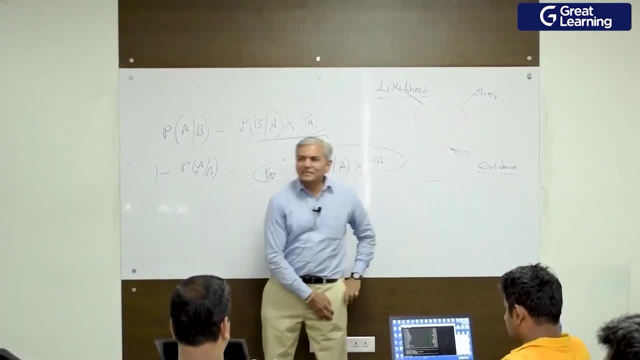 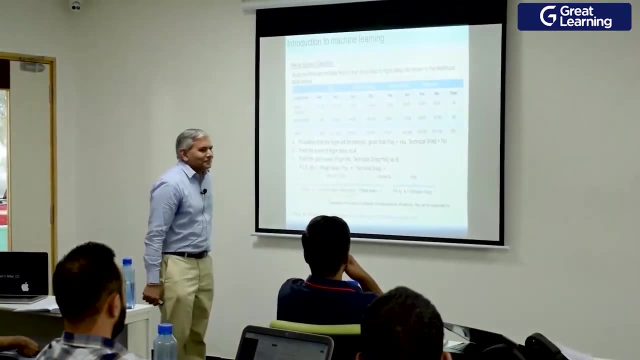 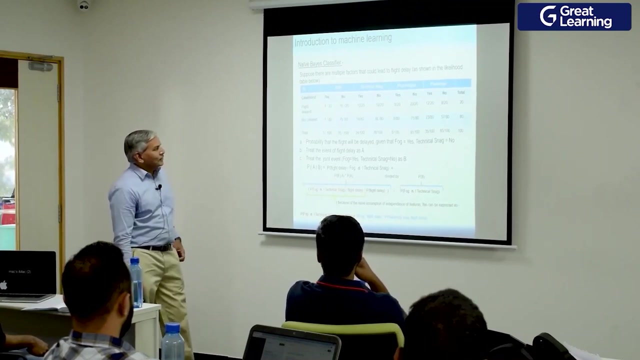 threshold. you send your alarm right, But there is a problem. We have time, So we will discuss the problem. What is the probability of flight delay, given fog at the airport and, say, buffaloes grazing on the runway? I do not have any data about buffaloes grazing on the runway, So this algorithm will give. 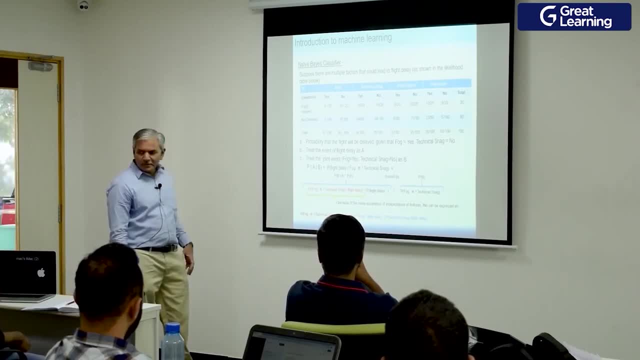 you. the probability is 0.. Okay, This comes from experience. Earlier in Delhi we used to have Palam airport. Palam airport had no boundary, So you can see lot of buffaloes coming from the villages and grazing there on the sitting on the on the runway right. 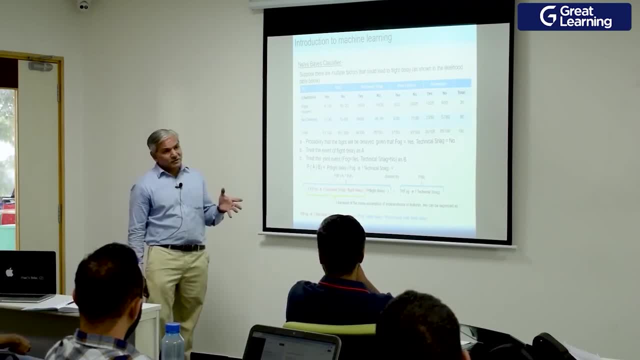 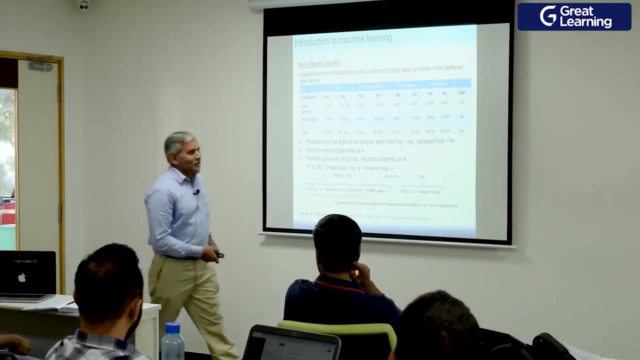 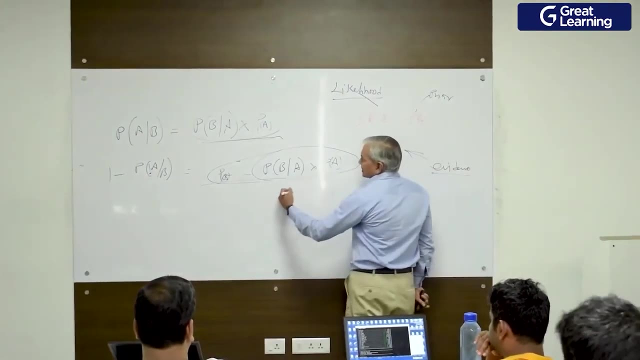 So what is the probability of flight delay, given fog and buffalo at the runway? The algorithm will give you 0, because you do not have any such information with you. So for that we use something called Laplace smoothing factor, So Laplace smoothing factor. 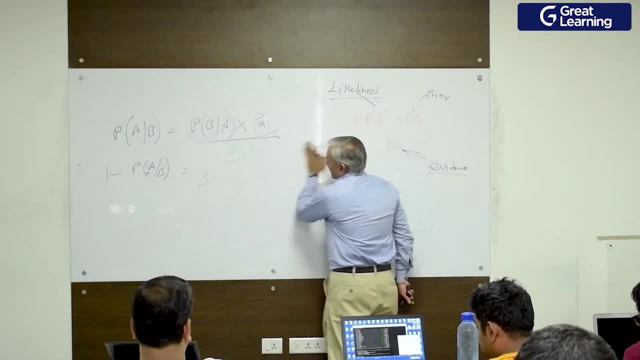 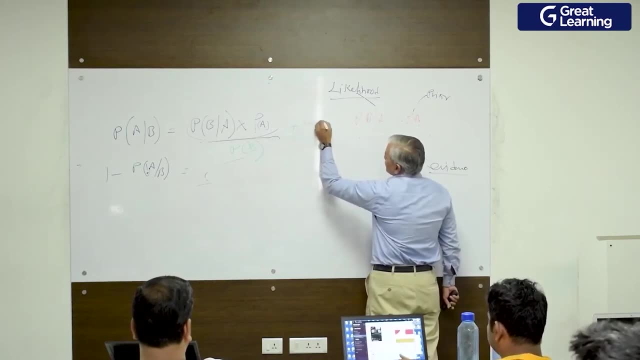 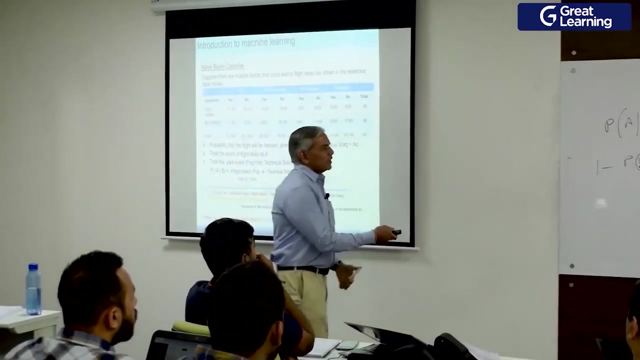 sounds very hi-fi, but it is actually adding one small to the numerator. adding one small, 0.0005, a very small number. You are free to add any number you like. This very small number prevents the numerator from becoming 0.. 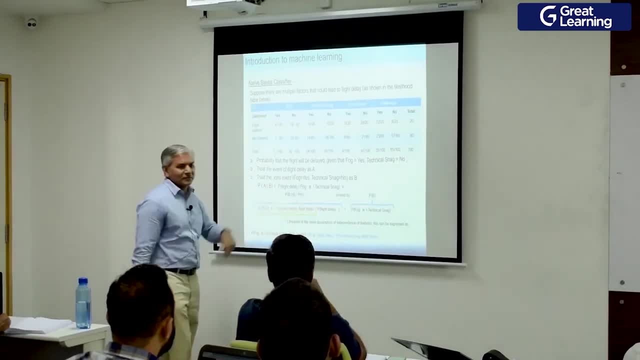 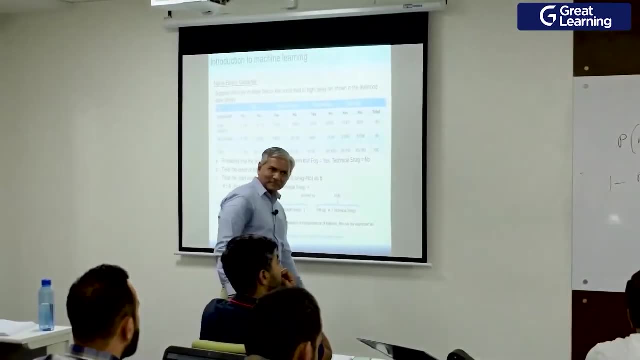 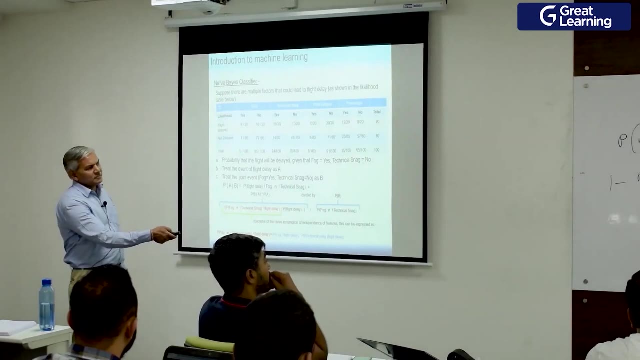 When those rare events occur for which you do not have data. Okay, Since the event is very rare, we give it a very low value. This is. there is lot of technical discussions behind this, but this is called Laplace smoothing factor. By default, it is a very small value. 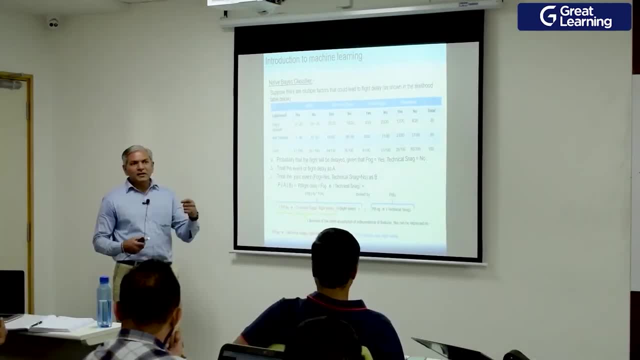 of 0.00005.. Any outlier, any event, comes in in the test record, which you have never seen before, it will be 0.. So at that time the probability should not become 0.. So probability is very. 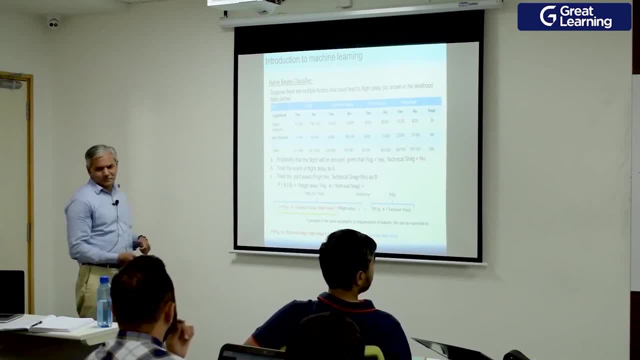 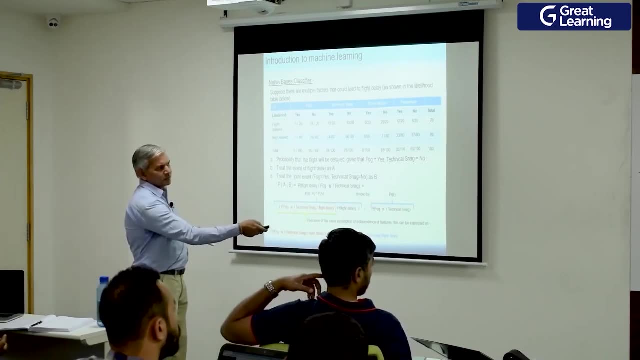 low value. That low value comes because numerator is very low, So any rare event for which you do not have any training data. when it occurs, this expression will become 0. But this will prevent it from the numerator from becoming 0. So the probability value will. 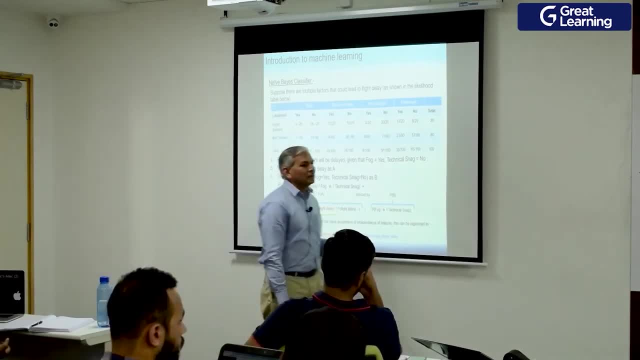 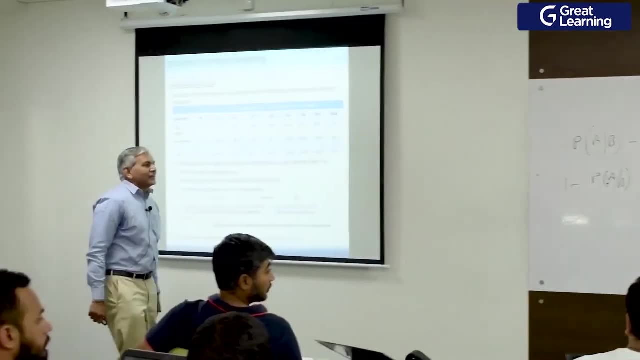 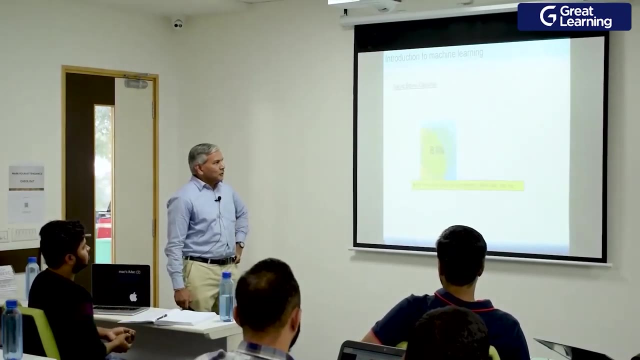 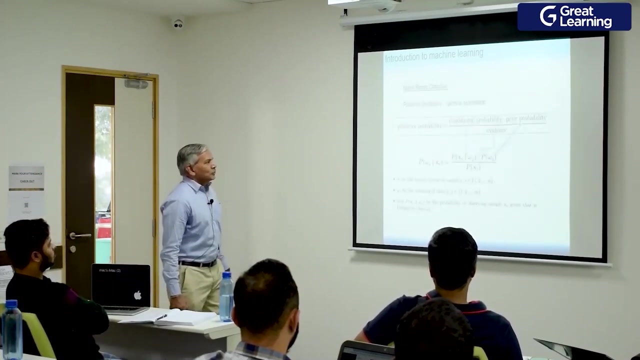 be very conditional. probability will be very low. Generally it is a prefixed constant but you can change it if you like. Any other question on this? Shall I go back to the slides which we jumped Now? those slides which earlier looked like hieroglyphics, now will make sense to you. 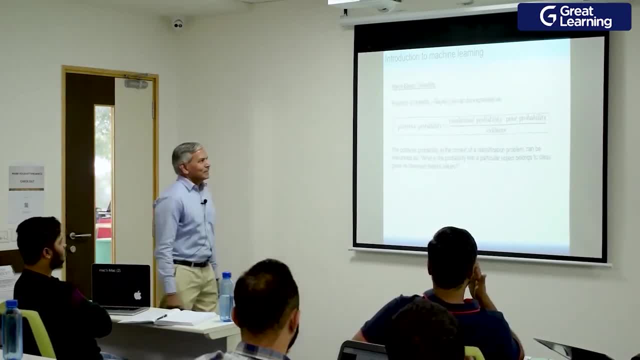 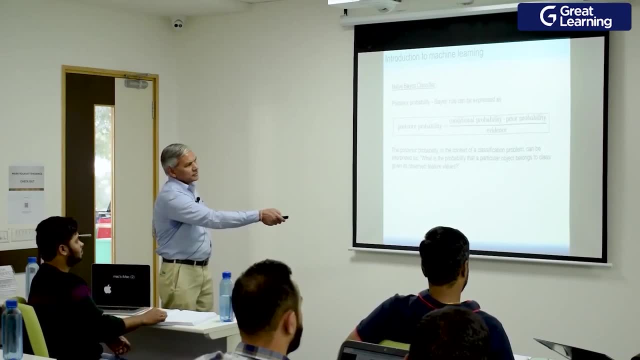 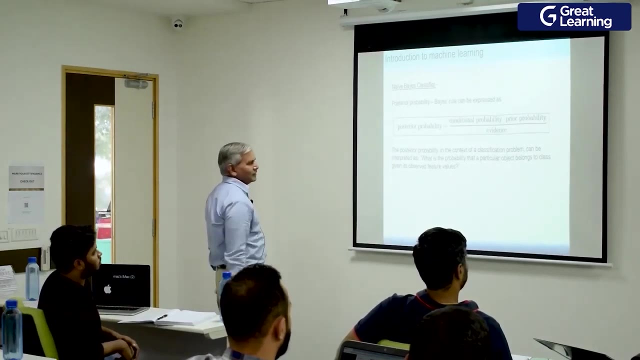 So this is where we jumped, Is it okay? So posterior probability is this which you are trying to find out. This is my likelihood ratios. it is also called conditional probability and this can also be called conditional probability, but this is posterior, this is likelihood, this is. 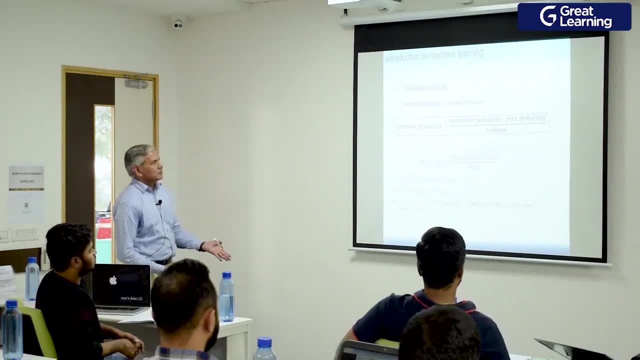 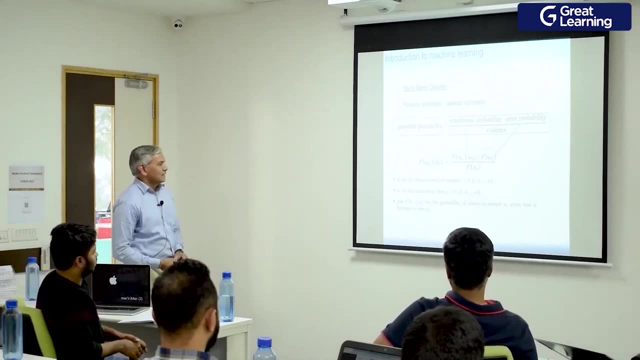 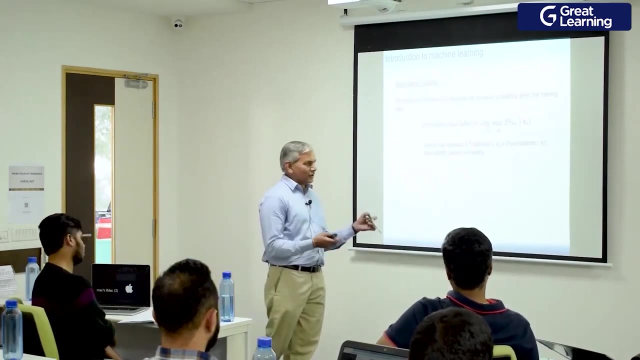 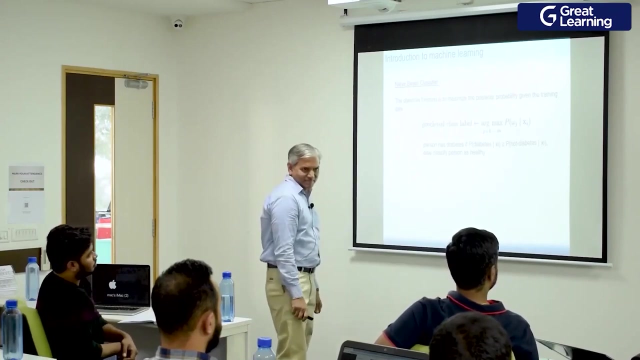 prior. this is my evidence. Some books, some authors will reflect it like this, but it means the same thing. So the class that will be assigned to a test record will be whether this numerator is greater or this numerator is greater than 0.5, that is called argmax, okay. 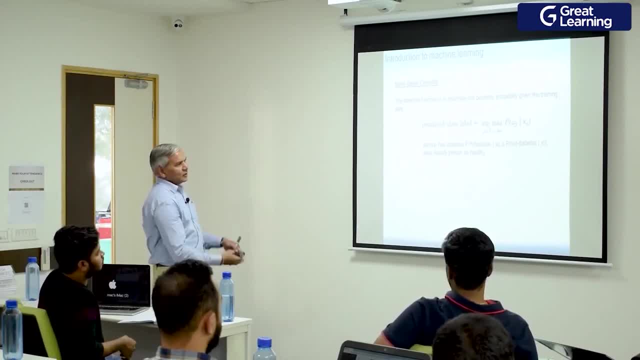 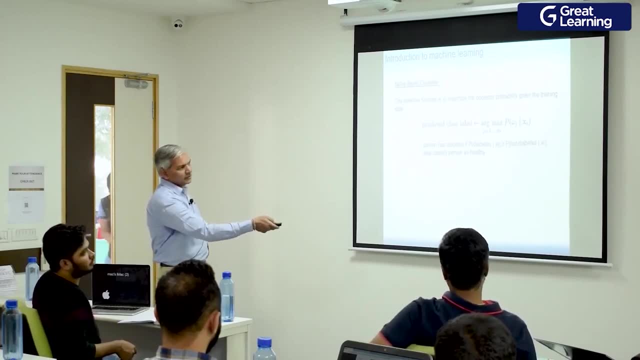 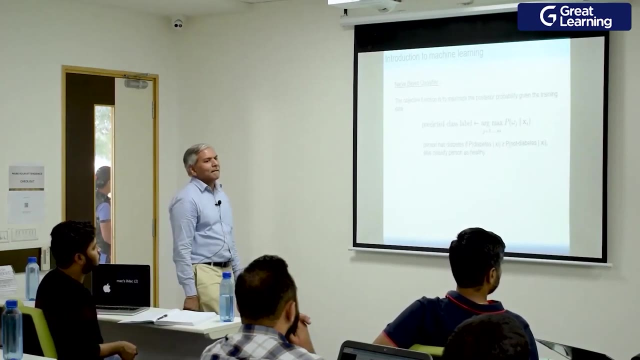 So whichever numerator is higher, the accordingly the class will be assigned to the test label. So that is indicated by this, The technical name that we use for comparing the numerators, argmax. which one is maximum higher? You mean? Yes, 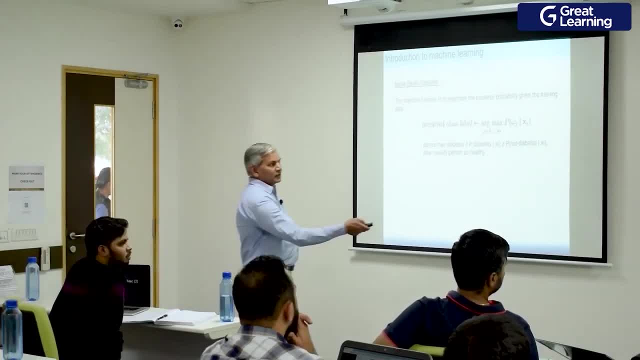 So it is equal to what is that number? yes, At the bottom, At the bottom, whether pB is greater or pA is greater. Yes, Now, whether this numerator- and there was one more numerator here- right? 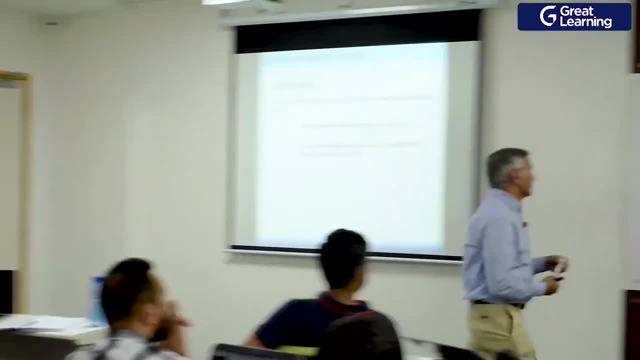 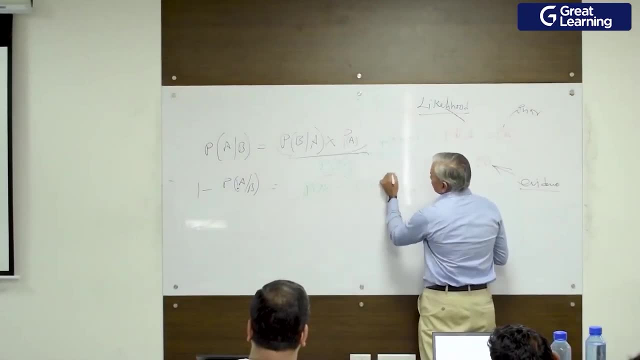 One minus Okay, at the bottom. So let me rewrite the numerator here. So this is pB minus pA given B No, pB given B, So v given and v given. Correct, correct, it is opposite. One minus no. 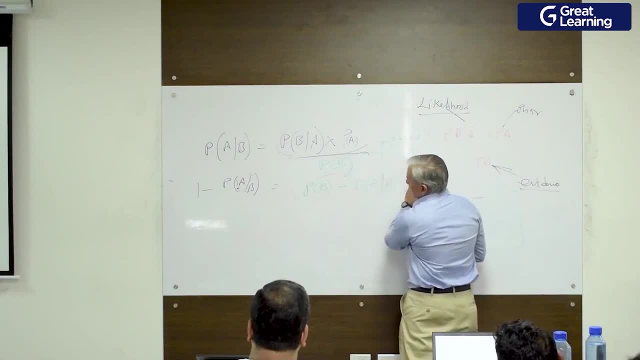 So this will be one minus pA given B, is this? I will again add this thing here: what is the total number More or less equal to 1 minus 1 minus? no, So this will be 1 minus pA given B, is this: 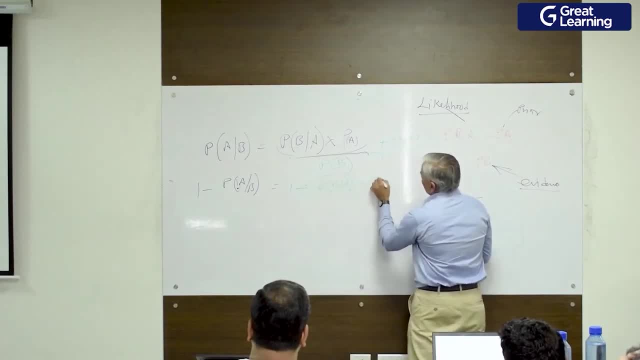 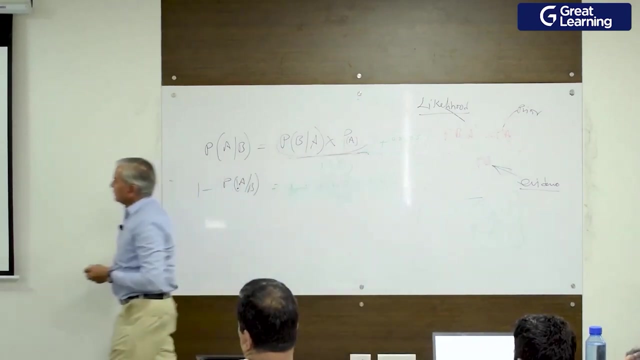 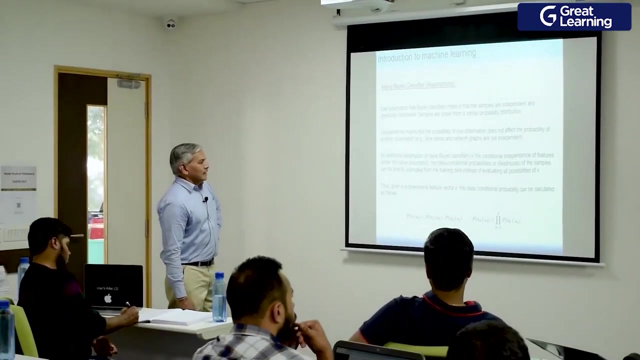 1 minus no, given A into P A by P B. So what? this will become P B and this whole thing will become P B. So now argmax compares this with this: whichever is greater than 0.5, that class will be assigned to the test label. Then, important thing, too much of words, but 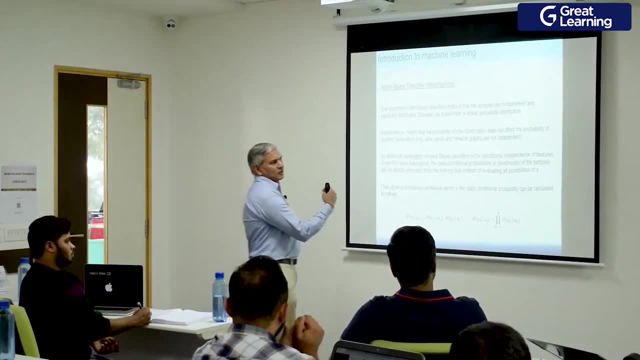 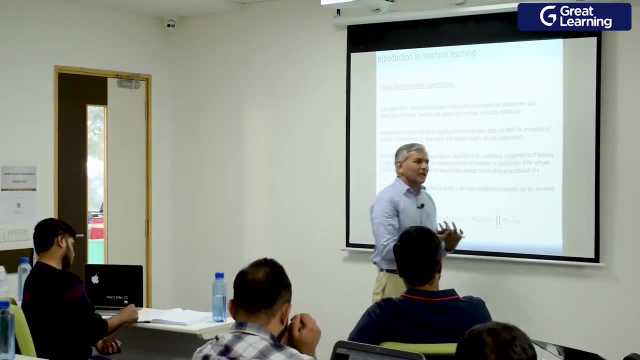 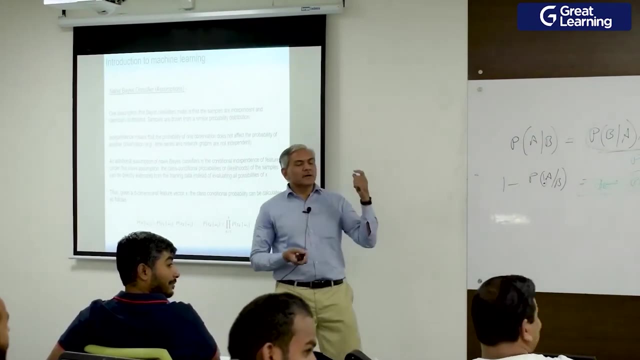 let me tell you in a brief way, because this algorithm assumes all these different events to be independent of each other. They do not influence each other. In probability theory, you would have seen, when events are independent of each other, we multiply their probabilities. See, I told you So. when events are independent of each other, we multiply this events, remember. 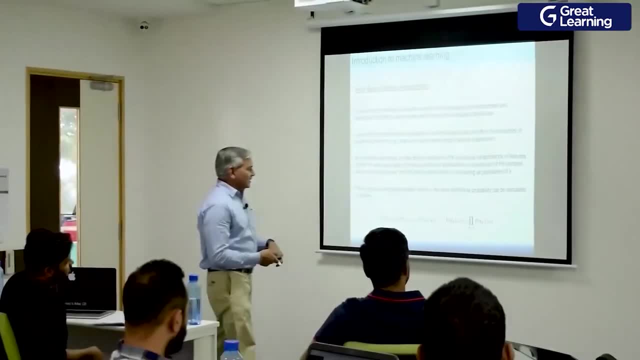 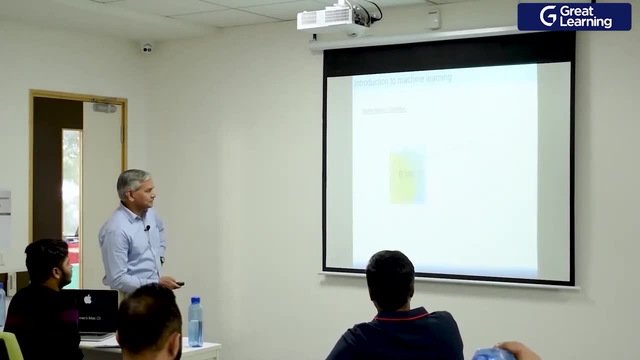 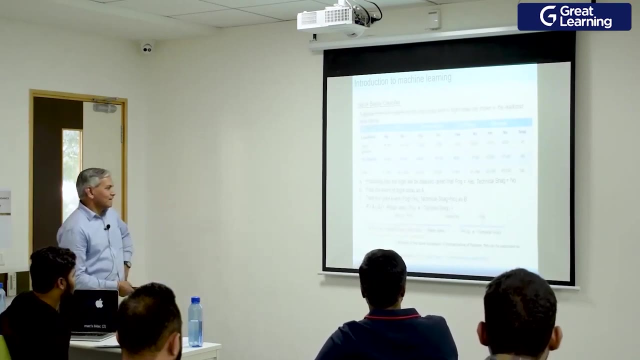 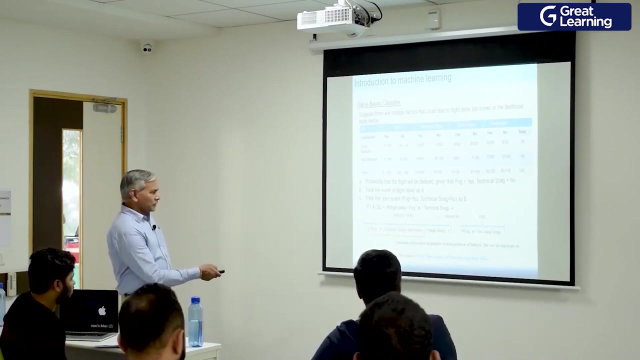 that in probability theory, So in the base, since the events are independent of each other, we multiply these events. What I mean this by this is: Look at this example. Look at this example. This is my numerator, this is my denominator. Probability of flog: no technical snag. probability of flog: no flight: no, what you call pilot fatigue. 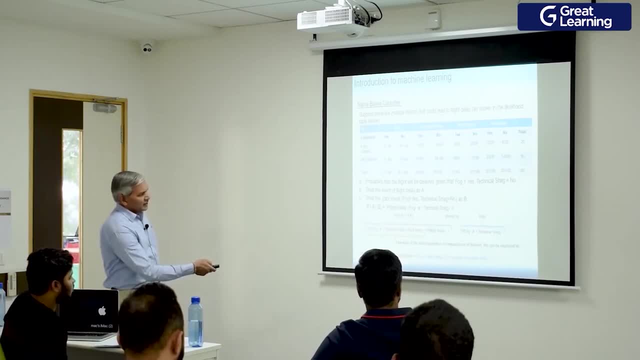 no passenger delay. If you want to find all these things out, just take individual probabilities and multiply each other out. right, I am not showing multiple things over here, but you can just multiply the individual probabilities over here to find the PV. B is the condition. So in diabetic case it was. this represents: 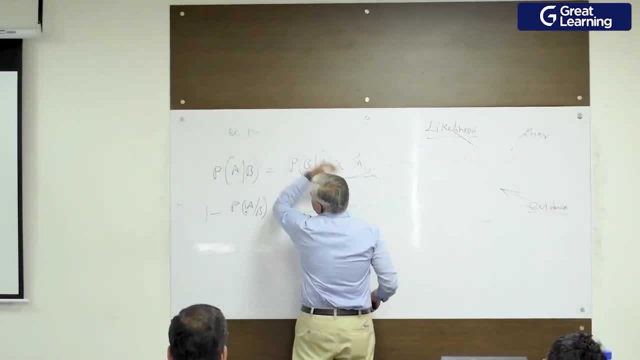 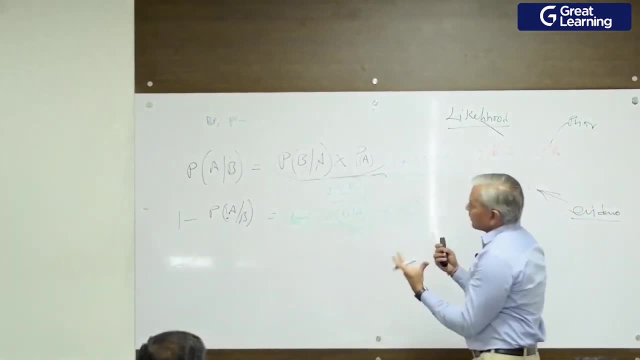 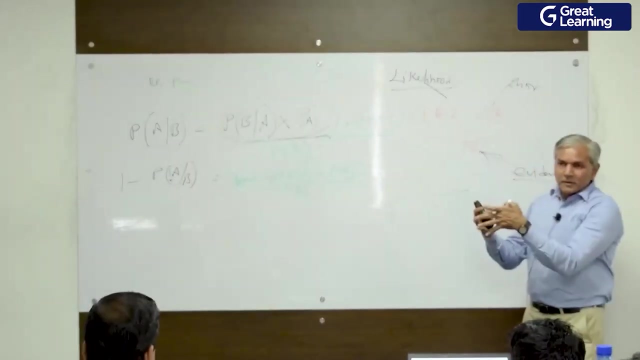 blood pressure. it represents plasma. it represents something else. So I can say numerator where I am using it. what is the probability of your what you call it, diabetes, given blood pressure? what is the probability of diabetes given plasma into? what is the probability of diabetes? 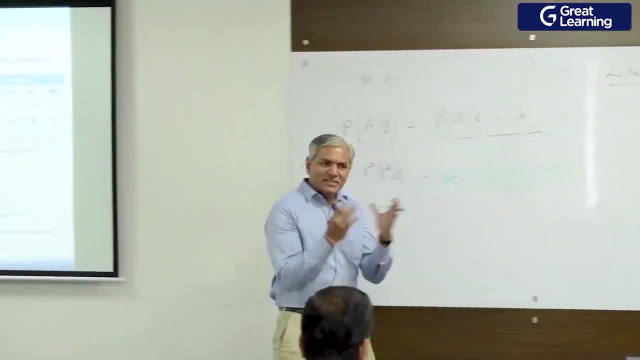 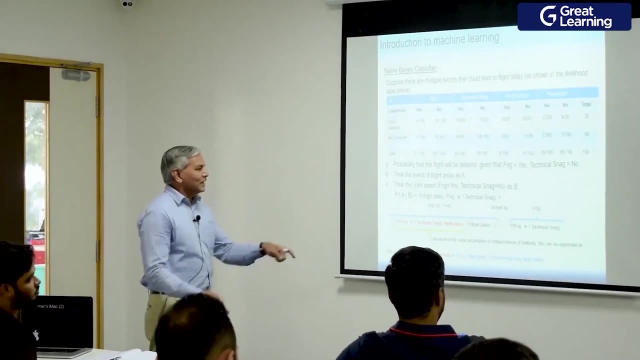 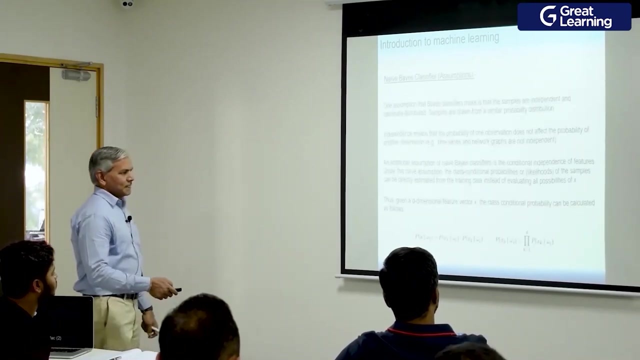 given this that. So just multiply those events, because they are independent events. That is what the numerator will become right. Same thing is shown. You will come across this expression. Do not get scared with this. This is what it means. The same equation will be repeated for each other. 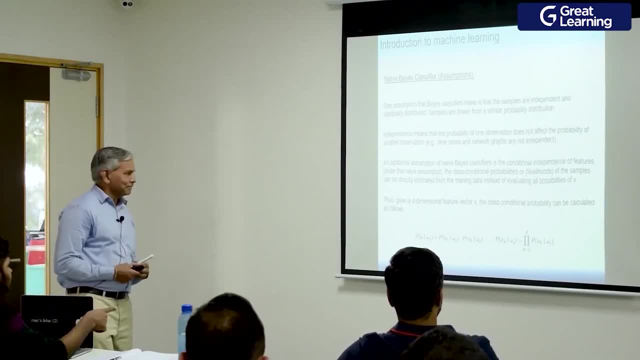 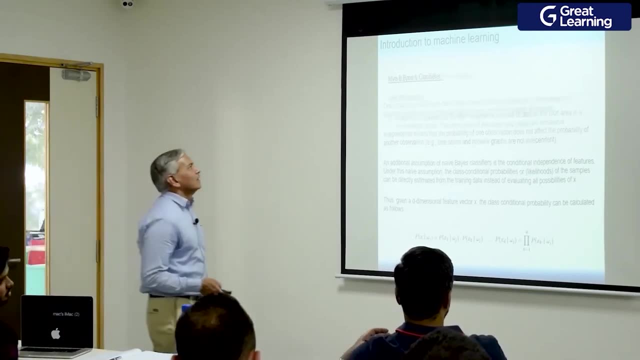 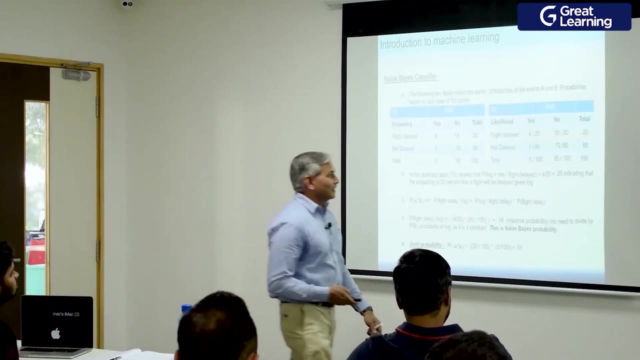 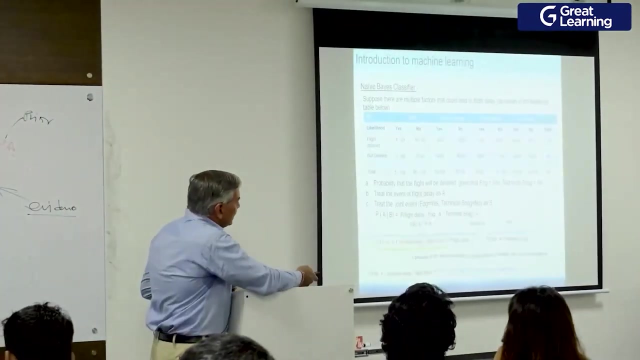 Yeah, each other, each other attributes. It is the multiplication. Which class? Yeah, W is a class. Which class is the last? All right, There is actually lot of depth and discussions on this Bayesian probabilities, which I am assuming you have done in statistics. I am going to move to the hands-on Before. 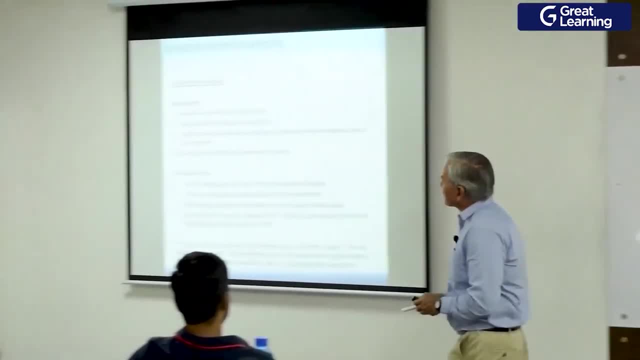 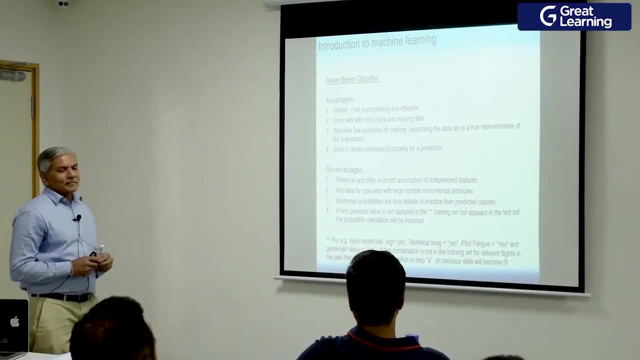 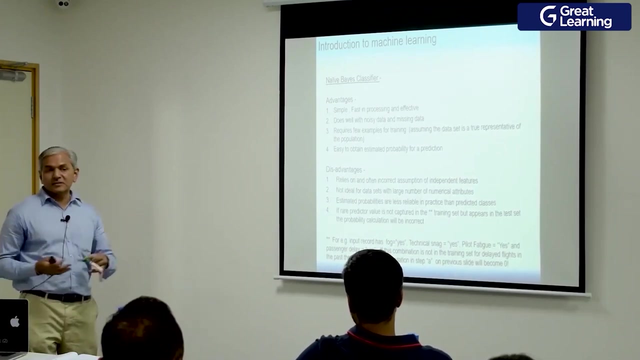 we go into hands-on advantages, disadvantages, Yeah Yeah, Just like your logistic. it is very fast both in training and testing. K nearest neighbor is very fast in training but very slow in testing because it has to find so many distances to find. the K nearest neighbors Does well with noisy data is what you will see in many. 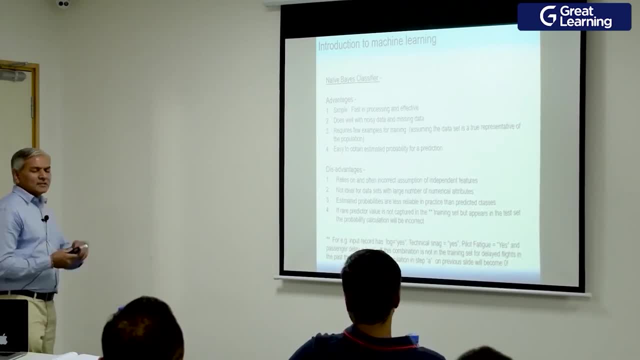 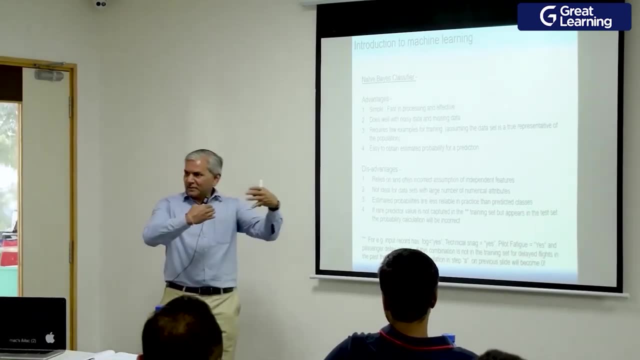 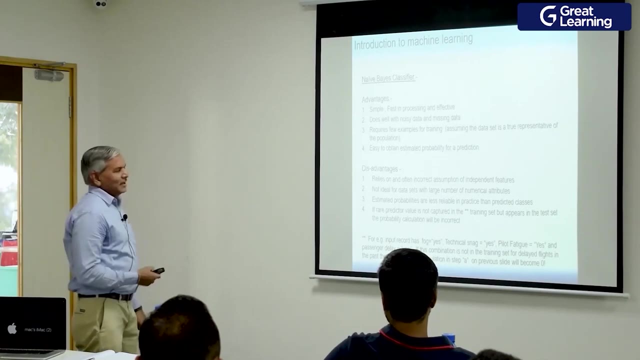 of these books and articles. But noisy data means there is a lot of jiggle in the universe from where you are taking the snapshots, Which means two consecutive snapshots will have different distributions. Okay, So I you have to take this with a pinch of salt. Any, 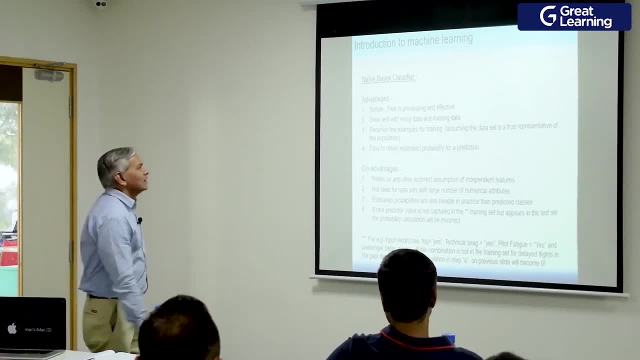 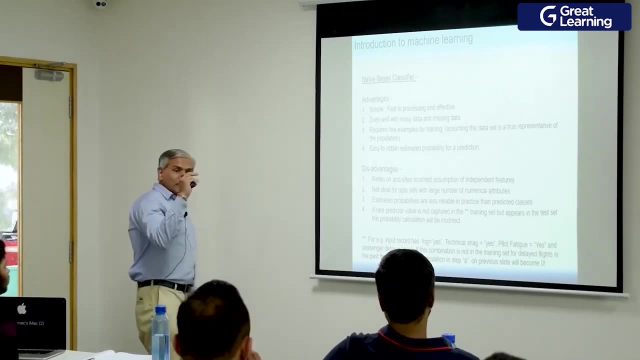 algorithm will find it difficult with noisy data sets. Requires few examples for training, Again something which we need to actually take up the pinch of salt, As long as the few examples are good representation of the universe, But otherwise no. We can convert our class into probabilities. Sometimes probability is useful. 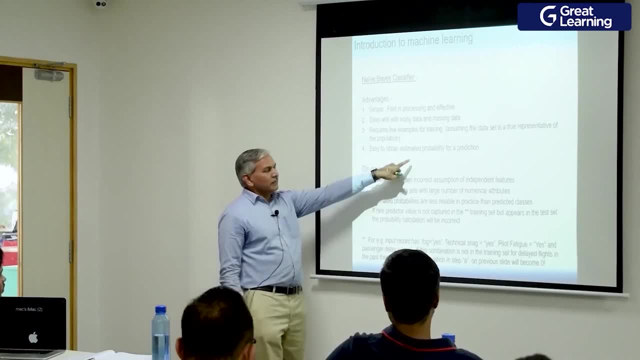 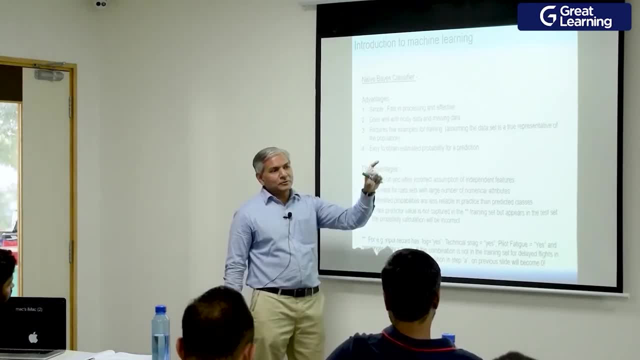 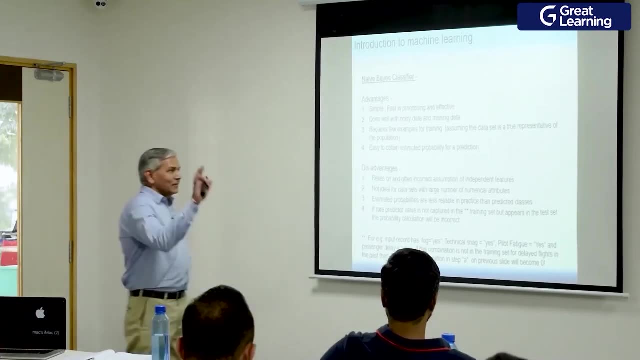 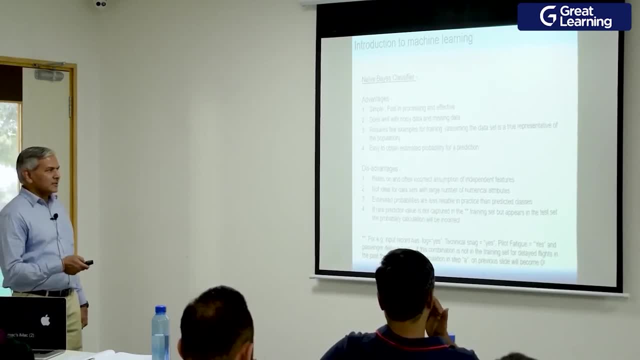 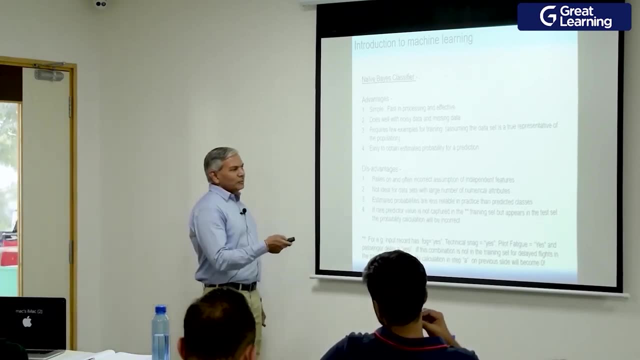 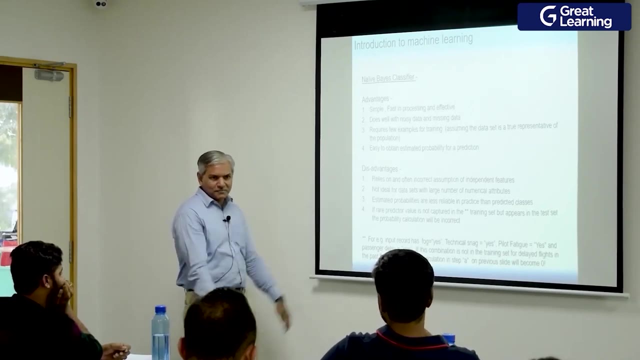 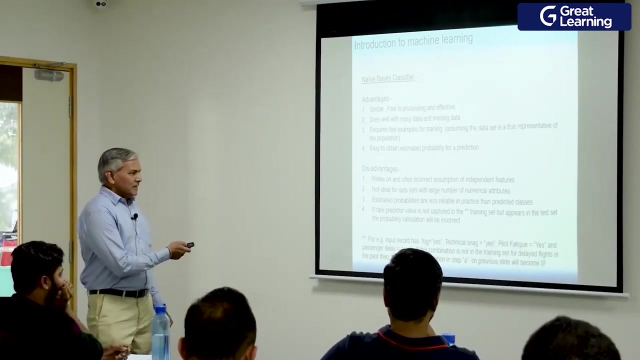 Biggest disadvantage is the assumption it makes, but then that is the assumption made by all the algorithms. When you have too many numerical variables, first it will convert this numerical variables into bins boxes. ok, It will categorize them, create bins and then calculate the probabilities. People have said that the estimated probabilities conditional. 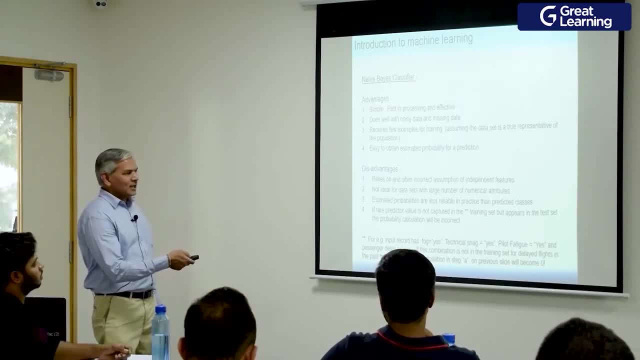 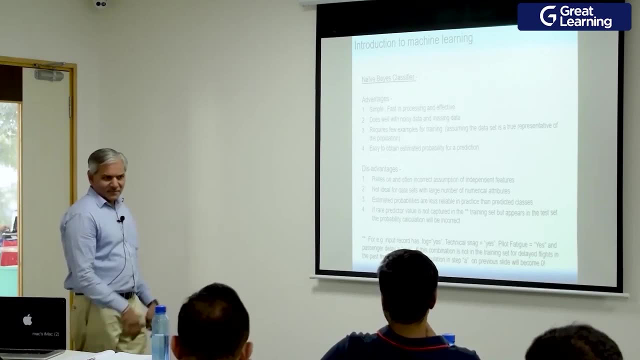 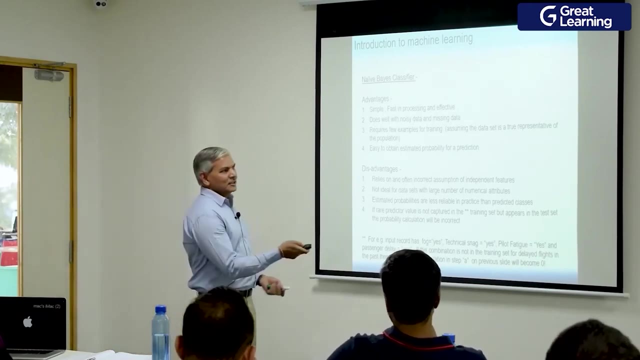 probability is usually less reliable. it is not reliable, That is true because these probabilities- assumptions is the attributes- are independent of each other. But because attributes are not independent, these probabilities have to be further jacked up. That is the same problem that you saw in p values between mpg and horse power. if 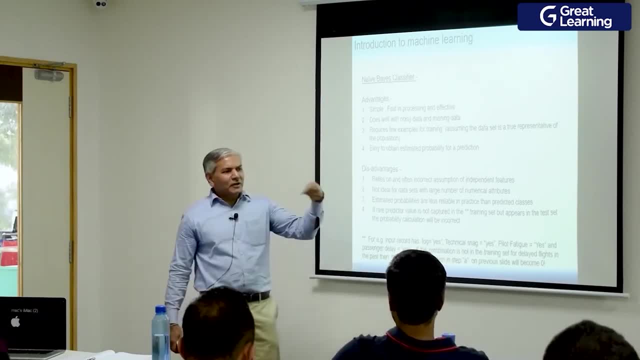 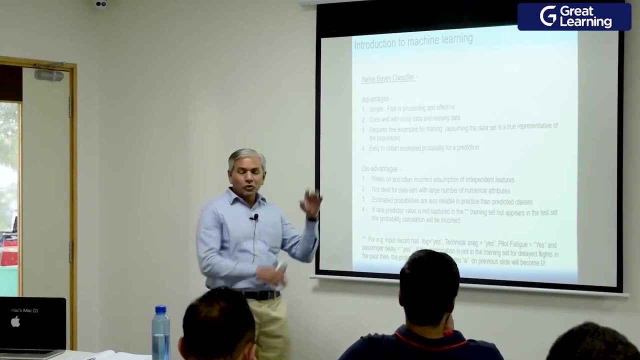 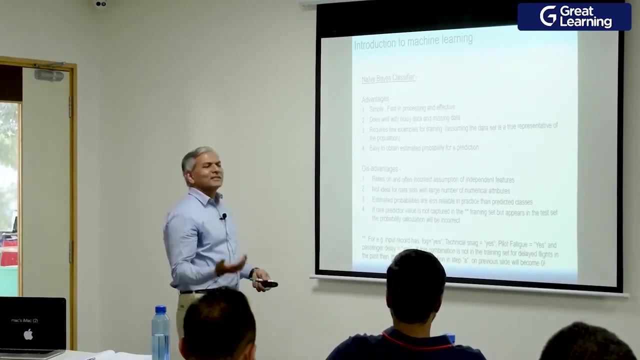 there is a relationship and there is a p value. why should that p value change when you use, along with horse power, the weight of the car, also coefficients and the p-values for the horse power change when you add some more dimensions to your analysis? that happens because of the collinearity between horse power and the 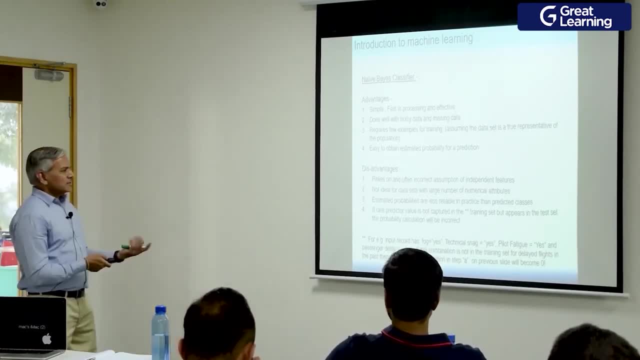 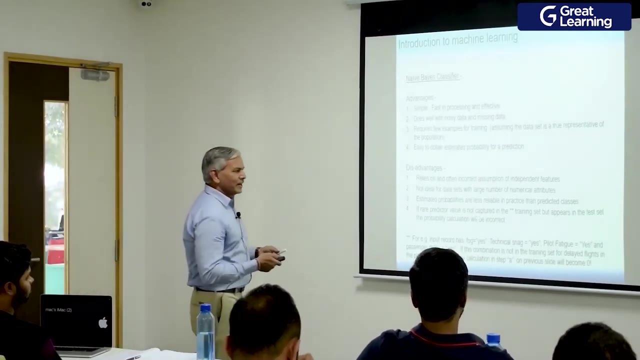 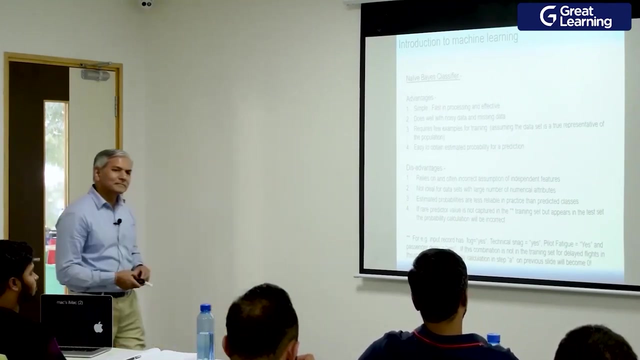 weight column. So this is true for all the cases. Estimated probabilities are, so estimated coefficients are usually different from the coefficients in practice. If you come across a rare event, then the numerator can become 0, but we can handle this using that Laplace factor. So what about descent regarding this? 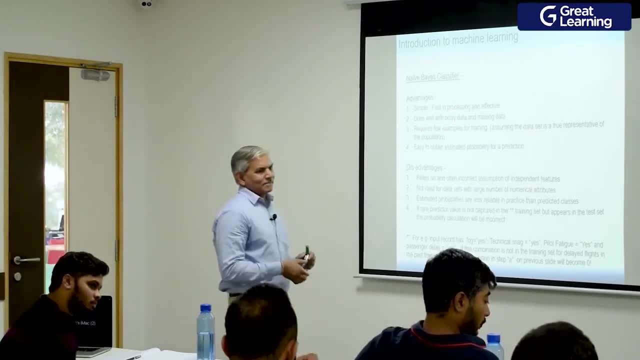 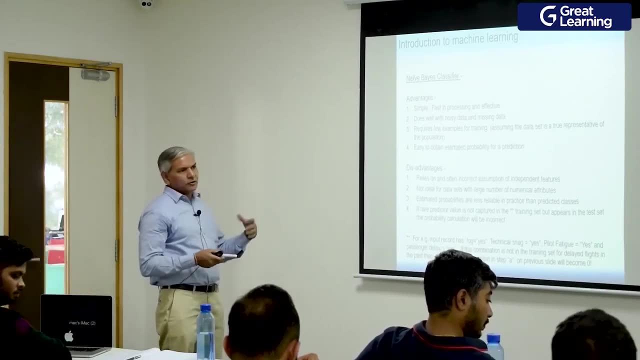 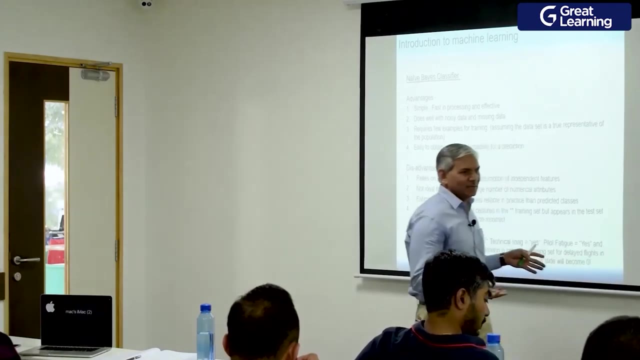 attribute. See, you are considering all the attributes. say, you have huge number of attributes, So will it be slightly slower because you are considering It will be relatively slower to less number of attributes? yes, it will be, But in the case of this it will not be visible to you. it will not be significantly different, However. 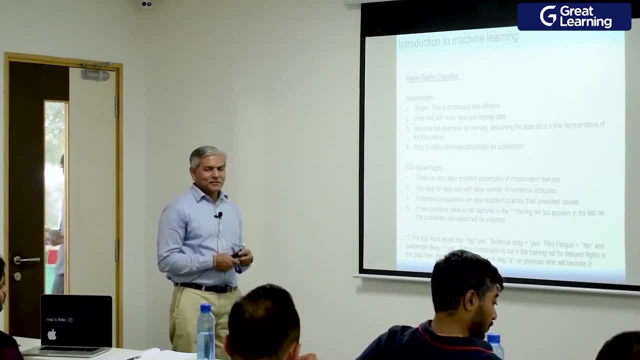 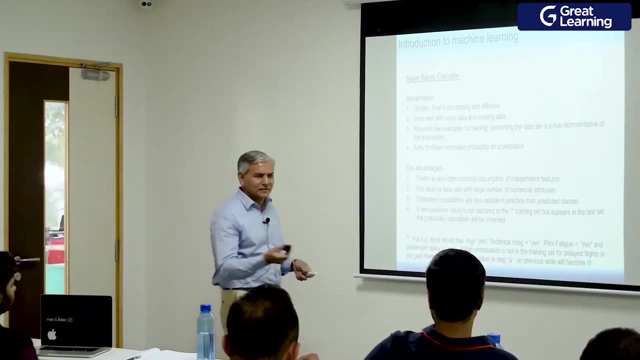 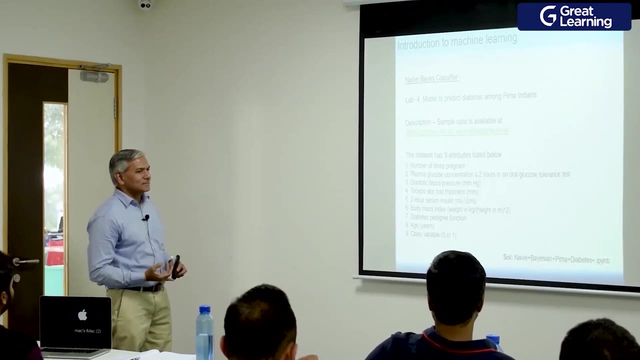 you need to be aware of curse of dimensionality. You should be aware of curse of too many dimensions, too less records. any algorithm can end up in curse of dimensionality. Shall you try this on the Pima Indians dataset? Ok, before I proceed in the UCI dataset. 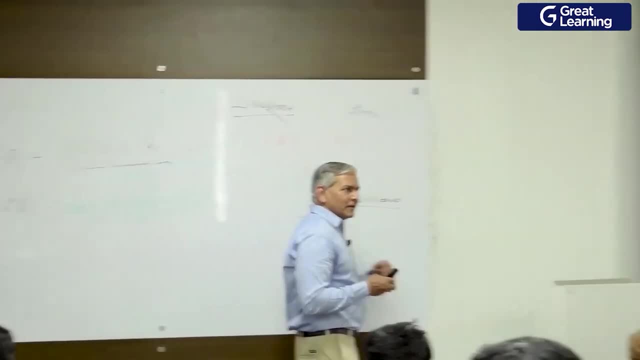 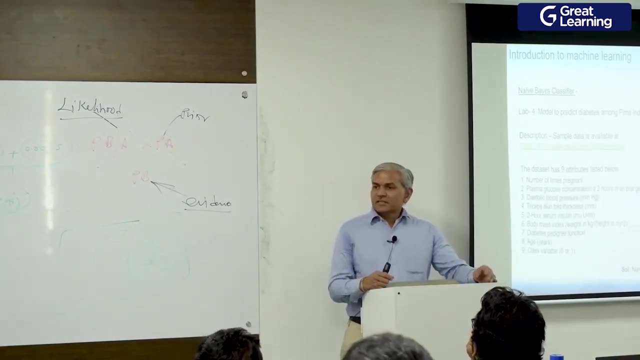 you seen the UCI repository That to my knowledge there are 512 datasets- pretty rich source of data. I might cover in the class Pima- diabetes datasets. but nothing prevents you from going and building these models. on the bankdatacsv, We have to predict defaulters versus non-defaulters. 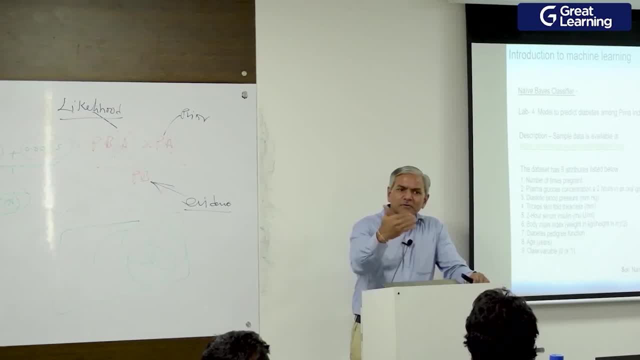 Just go ahead and practice this. Don't worry about the accuracy and all. How do you tweak the accuracy to a further, higher up level? That will deal in feature engine model tuning. But first thing that you should do is get used to the libraries that you need to call. 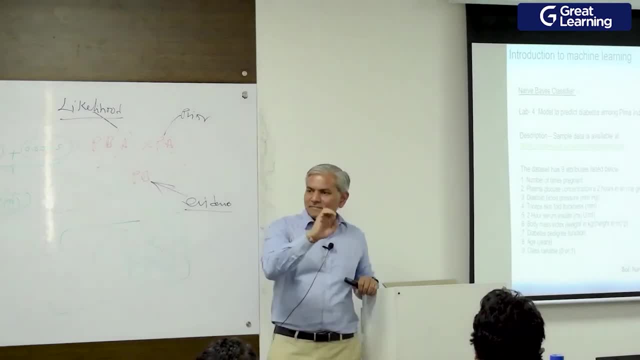 Second thing you need to learn is the basic syntax of scikit-learn. Third thing: by the time you become comfortable with all these things, then we can go into model tuning. So that will bring in continuity in your- I know many of you are on jobs you will find. 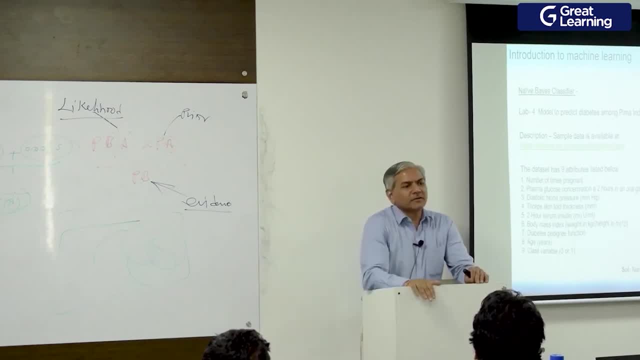 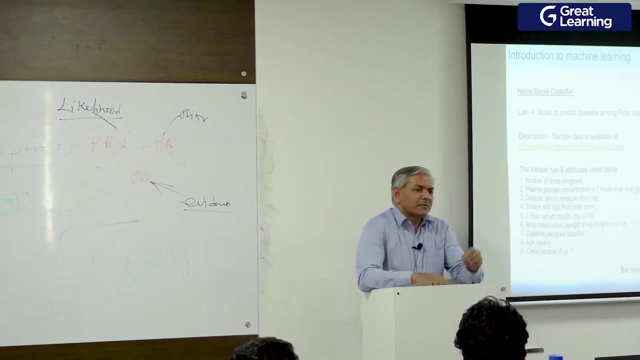 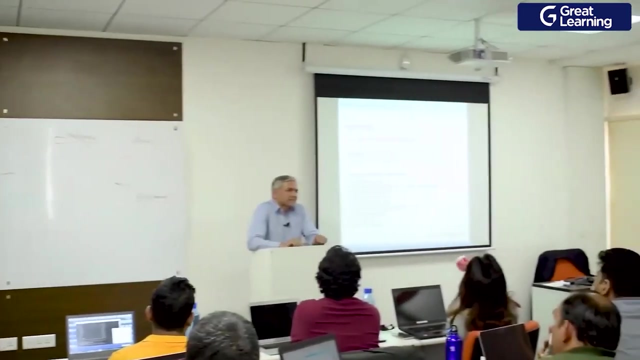 it difficult for the continuity to be there. This is one way of ensuring continuity. Yes sir, Yes sir, It is a ratio, so the ratios will have to be first. it will have to bind. Do you know that even decision tree does that When you use it for classification? it has to bind. 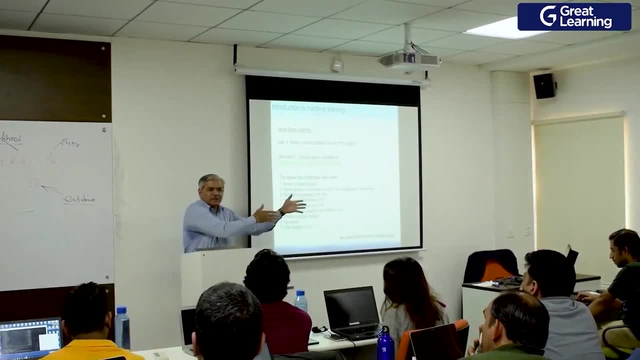 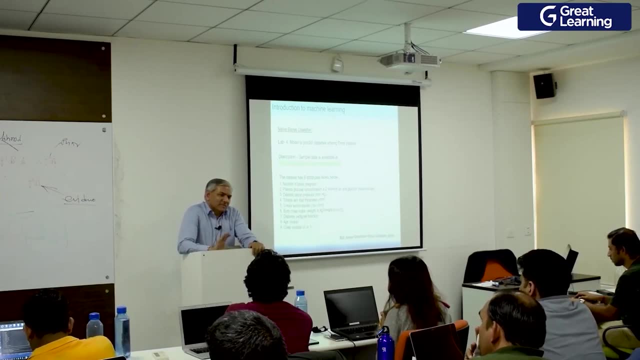 So if I have a attribute called plasma, it will bind first. equidistant binds will be created. So if you have too many numerical variables, it will take time to do that. So I have too many learning assignments, it will take time to do that. 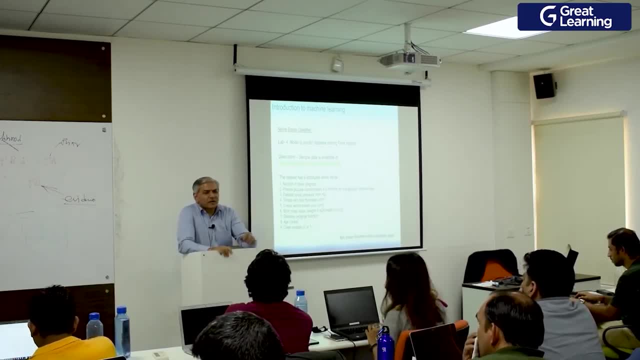 And there also we can. I will not be able to do all the things and there also, you cannot change the result. the result will not change, But what you have to do is you have to judge it by the data. But, however, we will not see all these things because we 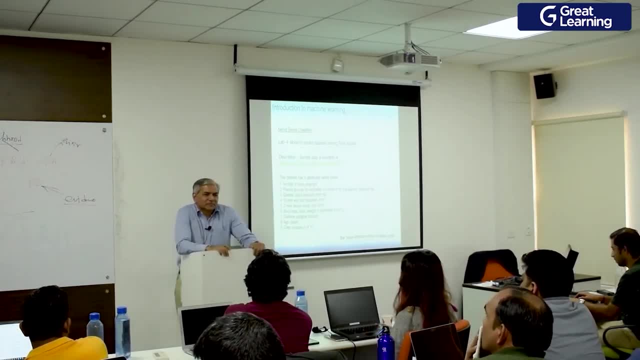 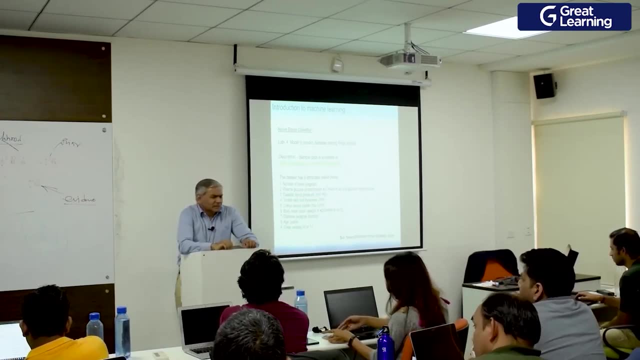 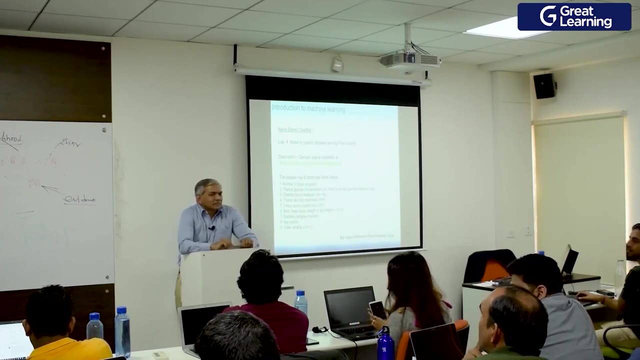 have today modern computers which are very fast. This was this algorithm was two hundred years ago, But that the problem was in slowness, not in the accurate, No Performance Performance. We are all under under the hood. they are all related. Decision tree also creates based. 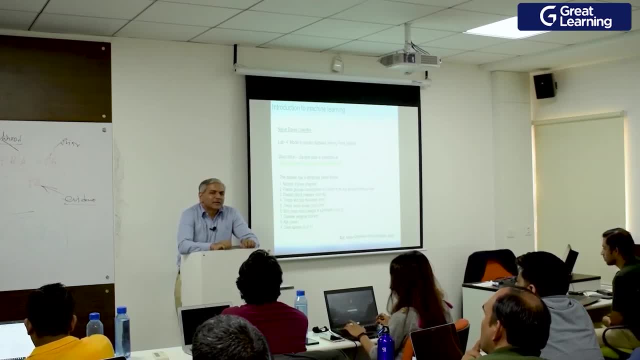 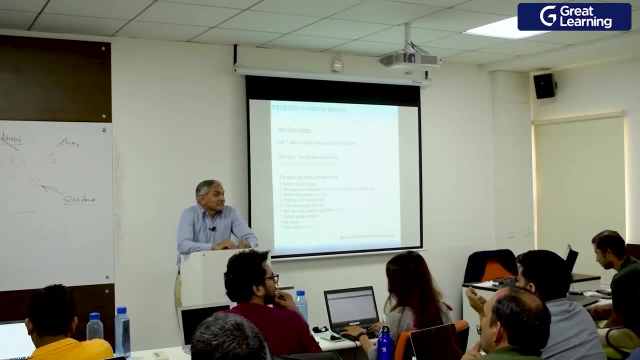 on interpretation but not on the data, Because …. the data is not. it is not the one thing creates based on entropy and Gini. That is another way of maximizing basic probabilities. Sir, the question was, what you are suggesting is the conditional division division rate. 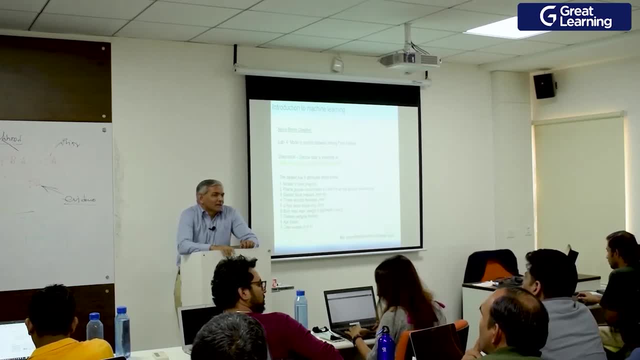 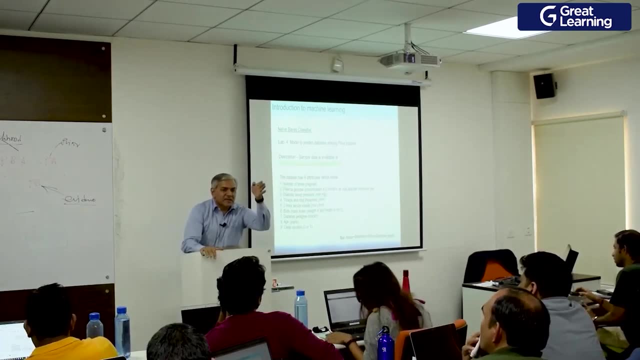 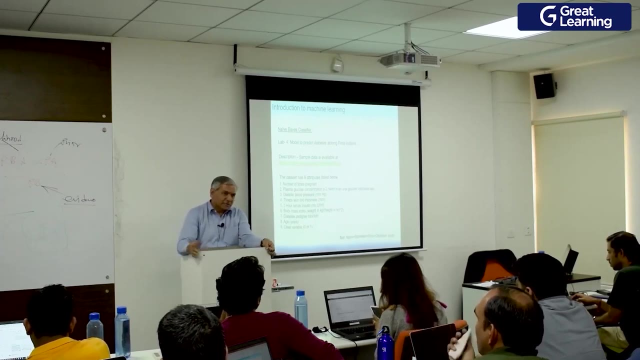 Yeah, This also may give us conditional probabilities. They are conditional probabilities, absolutely. What is the probability of class A given income? is this age, is this and this is that? that is what the path is, Sir. they are using a different loss function. Yeah, they are using a different loss function. 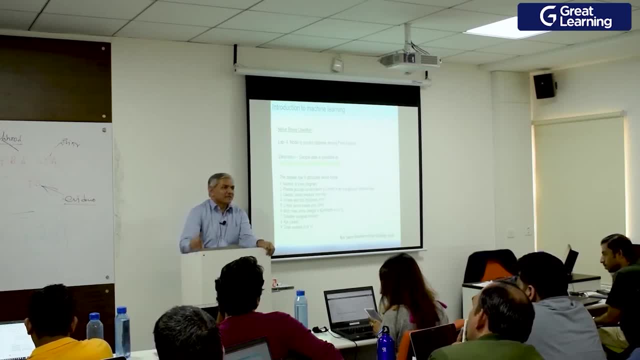 So all algorithms do the same thing in different ways. If you understand this, you will not have problem in learning any algorithms. So decision tree is all the conditional probability. The path is the condition based on the condition. what is the probability of finding this class? 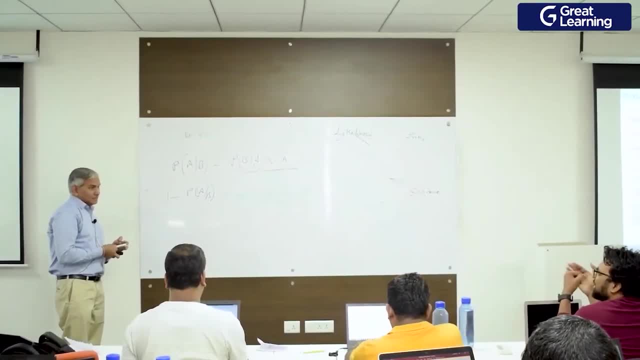 I do not know whether it is 0 or not. Can we do like that? let us say 0, 1, 0, 1 and a half. can we predict whether the next question will be 0 or not? Yes, Can we predict whether the next question 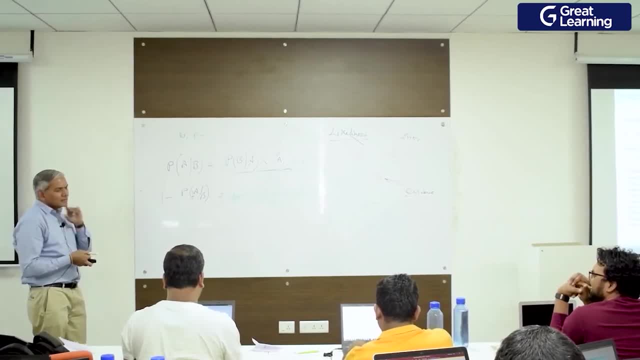 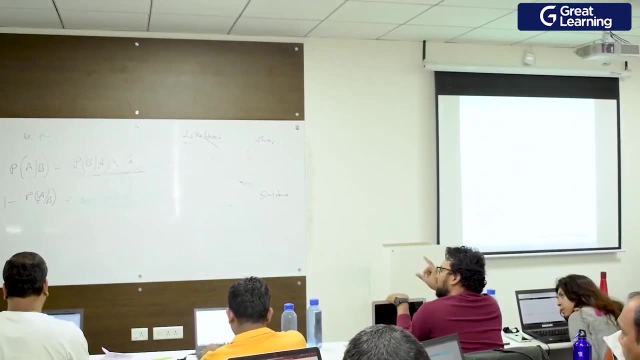 will be 0 or the next question will be 1? What do you mean by that? And this is the sequence. we just follow the sequence. what is the pattern of the data? Yeah, In that way it is. let us say the next value will be. there might be a possibility. 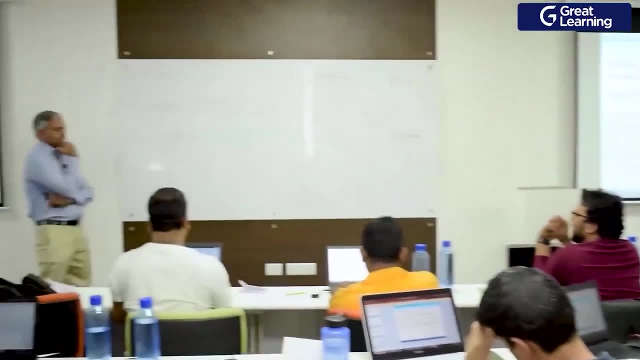 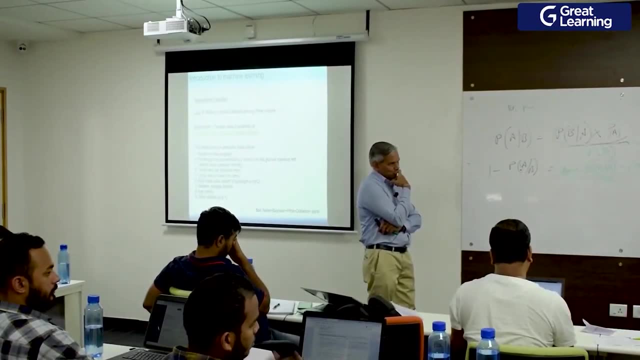 that the next value will be something whatever. Can we do it that way? Let us say: we see 1 0 0, 1 0 0, 1,. this is the pattern we want in some data And this is not the prediction. 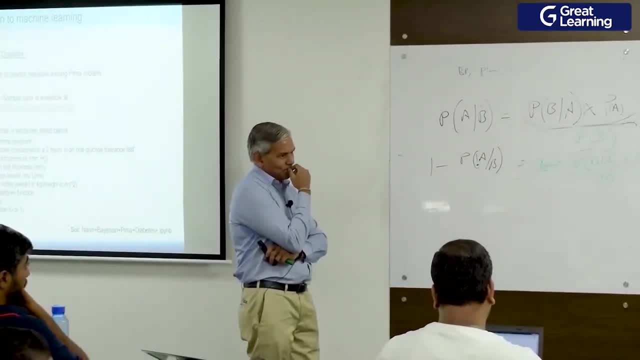 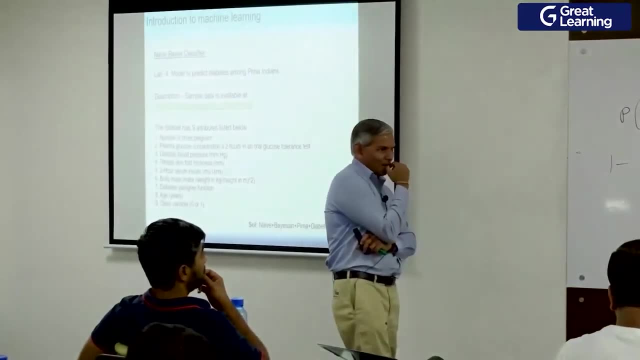 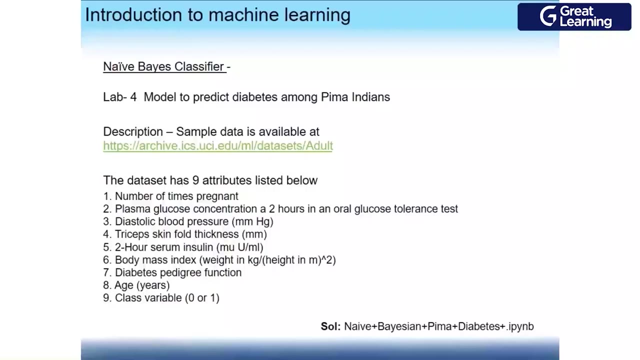 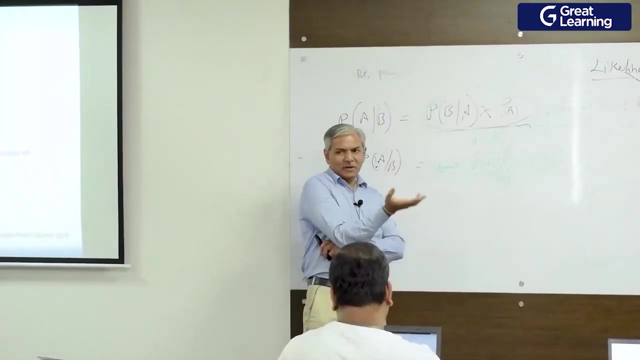 model. Can we predict the next value? Predict what is the next value going to be? seeing the pattern of the curve. there is a pattern inside. that is it. only if you have see a pattern you can build models. if you don't see any patterns, you can't build models. 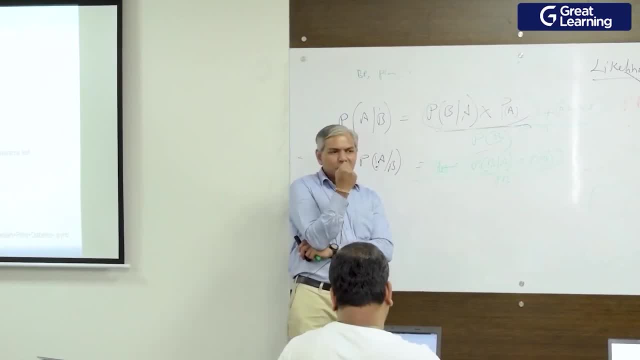 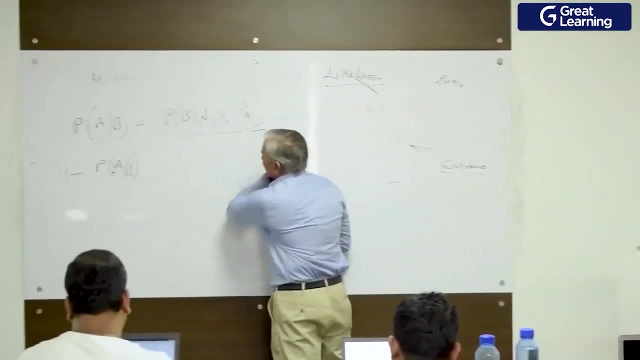 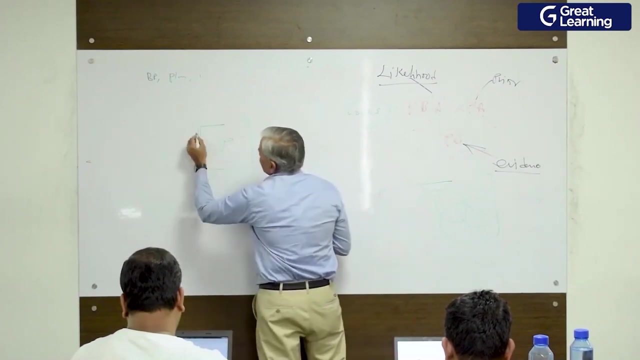 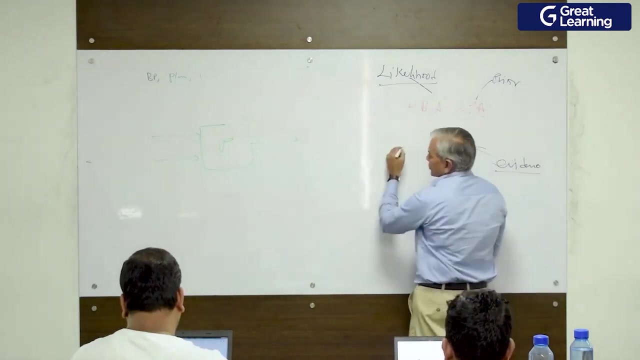 He brings me back to one more very core issue, very core point that you need to be aware of. we build models only when, ok, this process, P, it takes as input something and output, ok, this output that it generates. this output should be: usually, it is say, if it is a numerical, 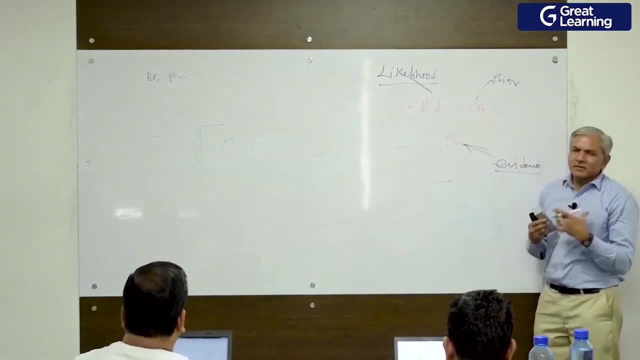 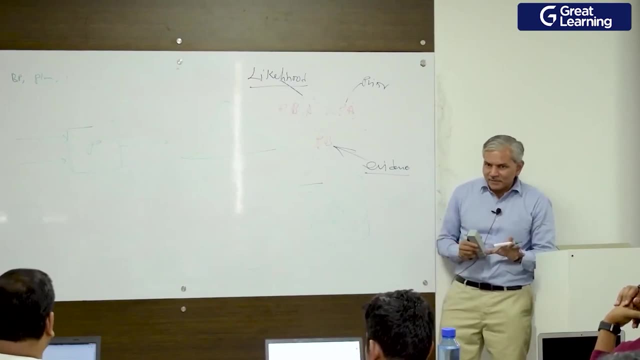 value you should. it should have some kind of a distribution. The distribution will have a central value and some spread, and so on, so forth. the characteristics of distribution: ok, only when you have well-beweaved, well-defined processes like this, whose outputs 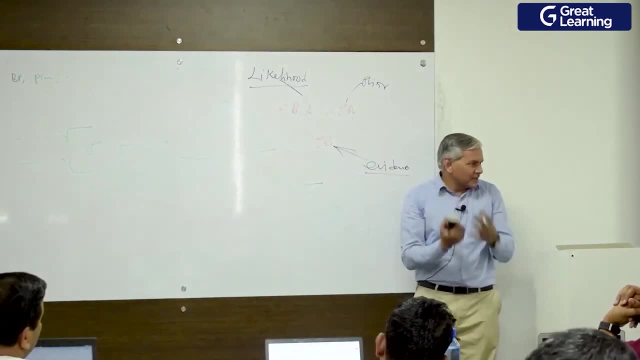 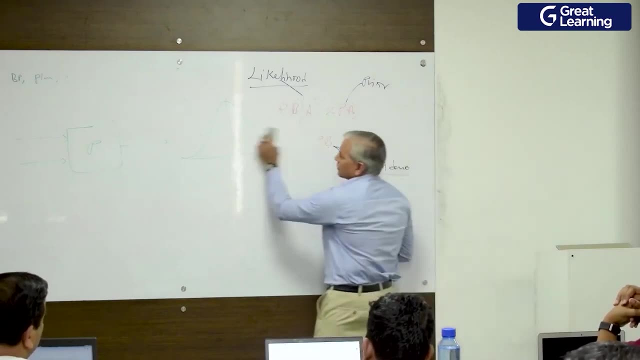 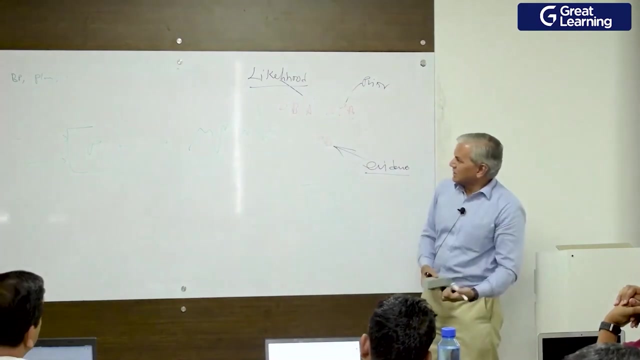 have some well-defined shape in terms of the central values and the spread. only then we can build models for to represent this process. If the output of this process is going to be random in nature, we don't know what, what, what it is going to be- sometimes it is 10, sometimes it is 10, sometimes it is 10, sometimes. 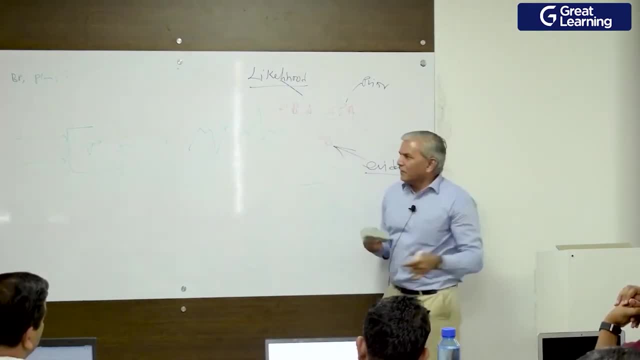 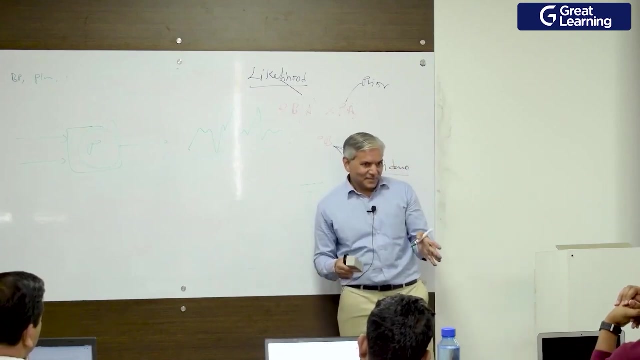 it is 40, sometimes 9, random outputs. we cannot build a model to represent this. We can build models only when, only for those processes which are well-defined processes. So, coming to your requirement, if the output the 1, 0, 0, 1, 0, whatever you are seeing it is. 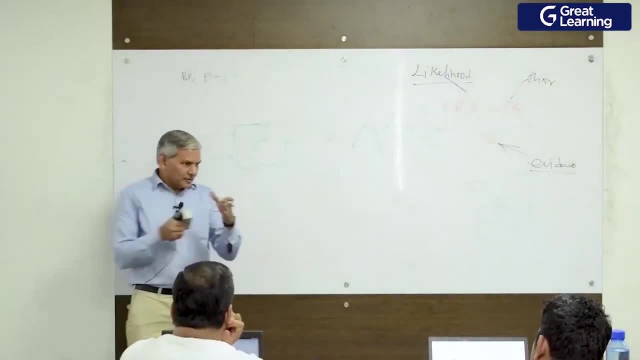 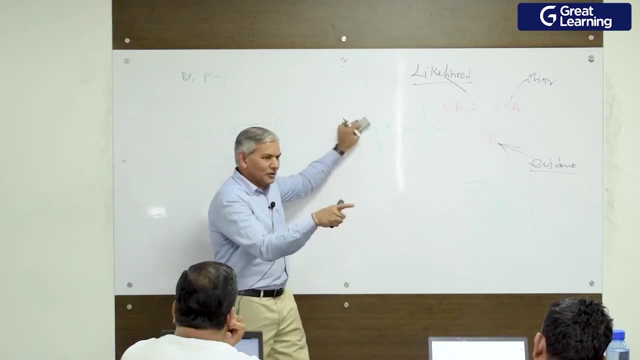 an output of some process. If the process is outputting this in some patterns, the pattern could be in form of Gaussian distribution, so on, so forth. only then you can build a model to represent that process and predict what's next value going to be with some 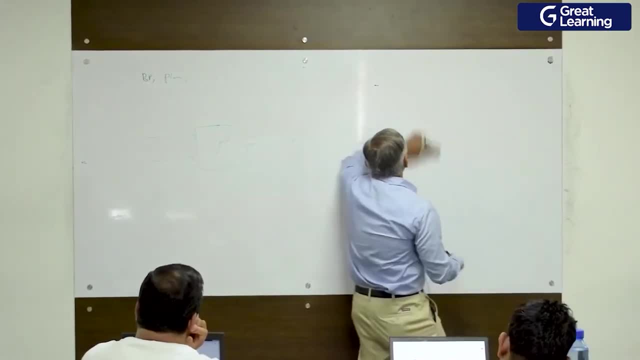 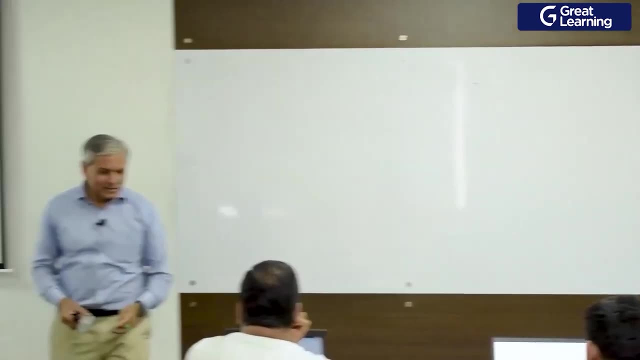 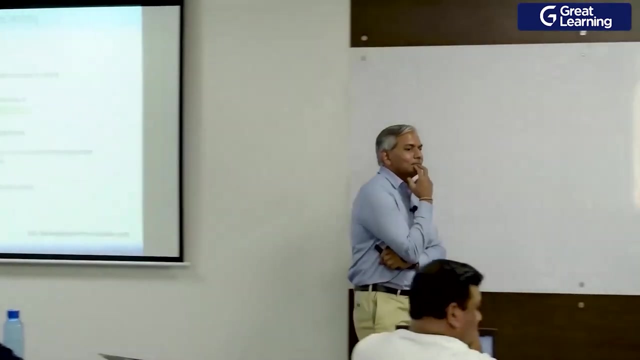 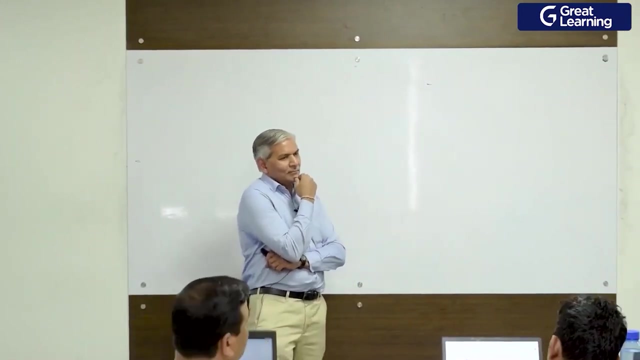 confidence levels. You can't model a random process. If that 1, 0, 0, 1 and all is coming out randomly, then you can't build any model. Yes, I understand what is the b? a with condition, a right. So now we are actually calculating. 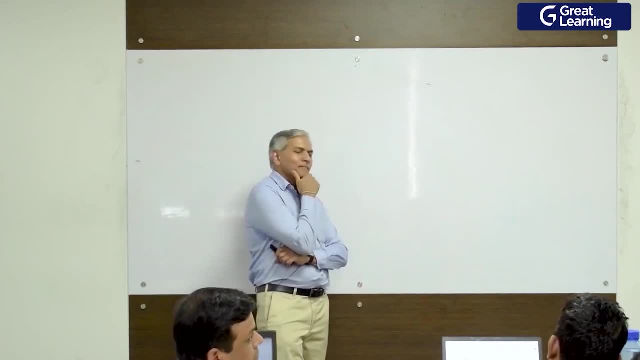 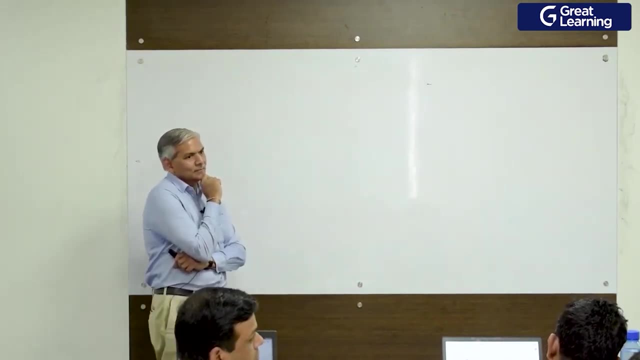 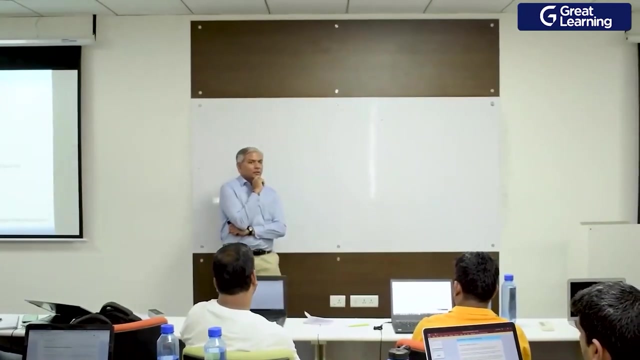 b, a b by putting b b a condition. So, yeah, we can, we are getting an output. but what is the need of doing that? Is it that previous denominator values d, Yes, No? you are depending on the past data. what is the probability of now a patient walking? 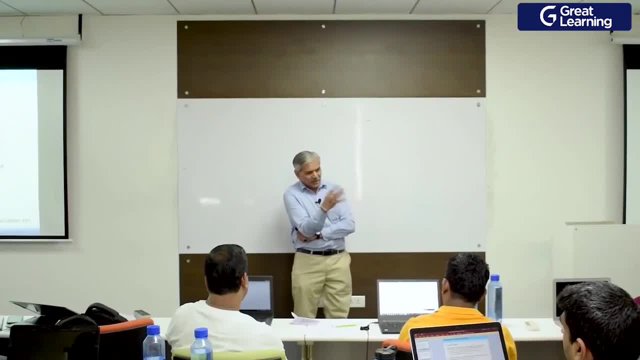 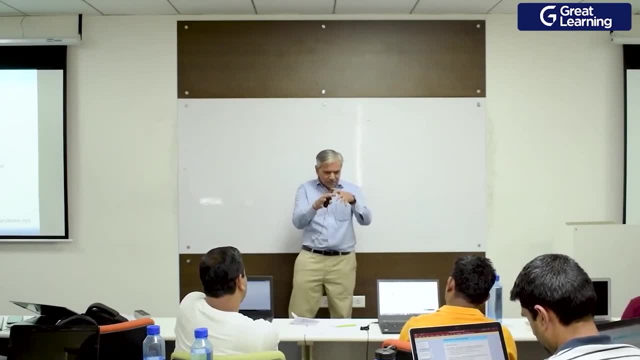 into my dispensary. I want to classify him as: does he have? benign or malignant, cancerous or non-cancerous, Instead of building a model which is where input is the attributes of the patient, and building a model to predict that go back into your data set of the past. 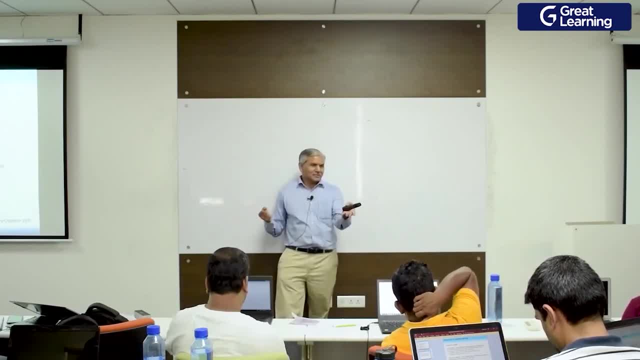 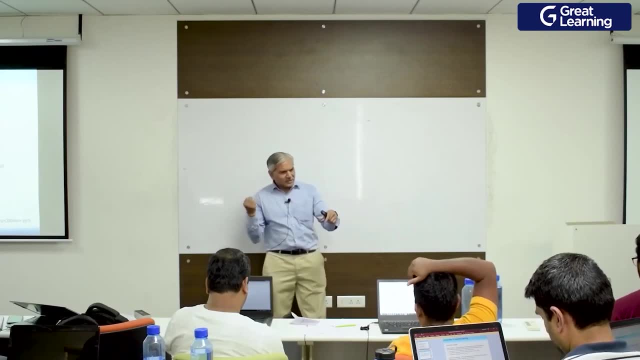 patients, those who are cancerous. how many of them had these conditions? If majority of them had these conditions, how many of them had these conditions? By these conditions, then likely this guy is going to be cancerous. If, if the past. 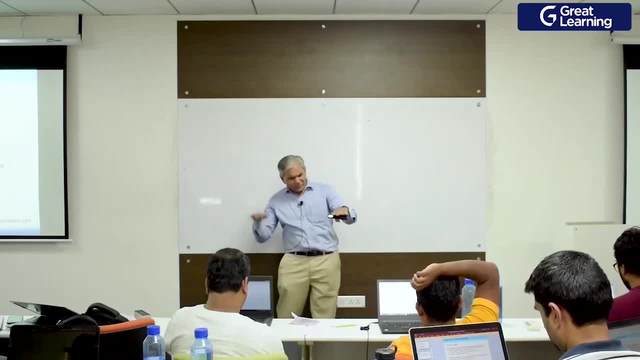 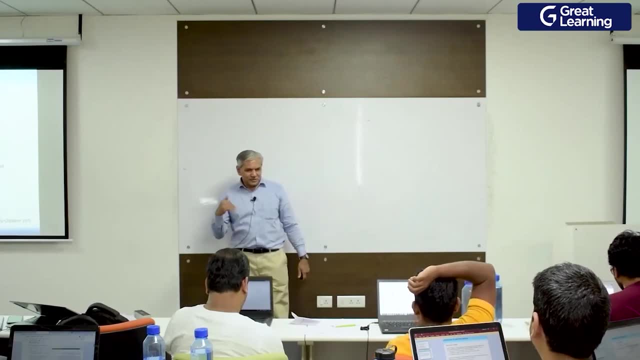 data shows that amongst cancerous patient this kind of attributes are very low, then maybe he will not be a cancer. So I flipped the argument and go back to my past data and see what is the likelihood ratio given the past. You can do same thing in this river case, because we have also. 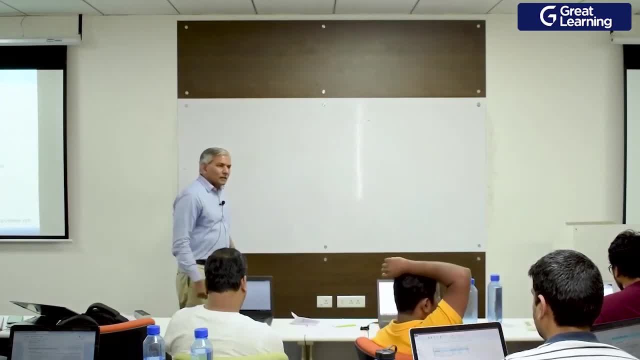 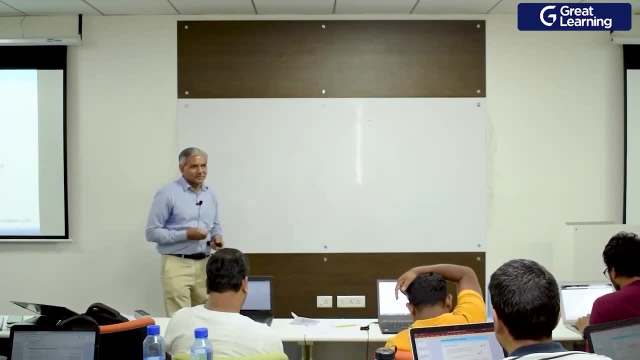 That is what I am going to do, correct? That is what you are doing here. That is what you are going, So shall I get in the handwriting? which way? Yes, yes, yes, please Correct. Ok, good. 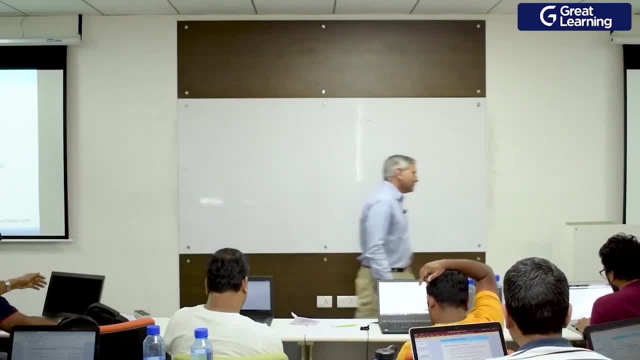 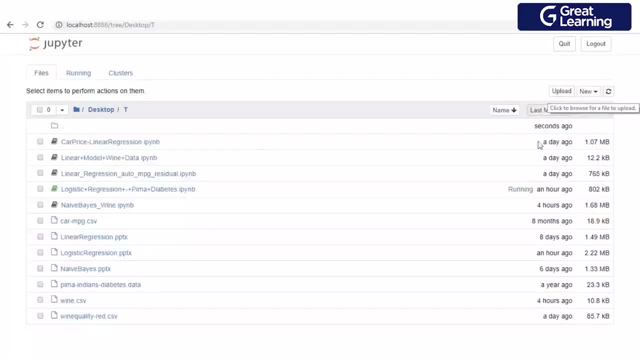 So shall we get in the hands on? It's the same data set, so all of you know what the problem is. We have the wine data sets, this thing, but we can do this on. would you like to take this as a homework? 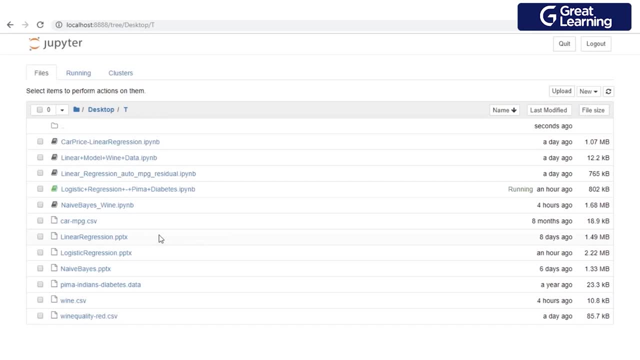 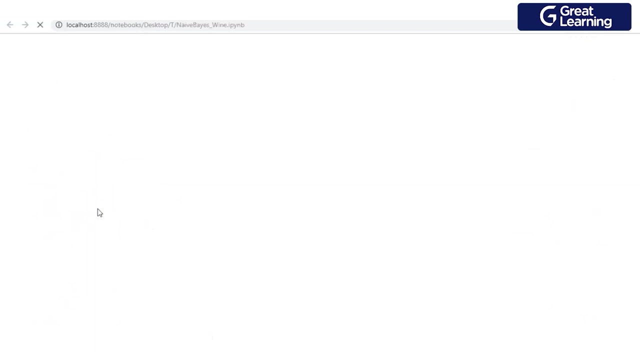 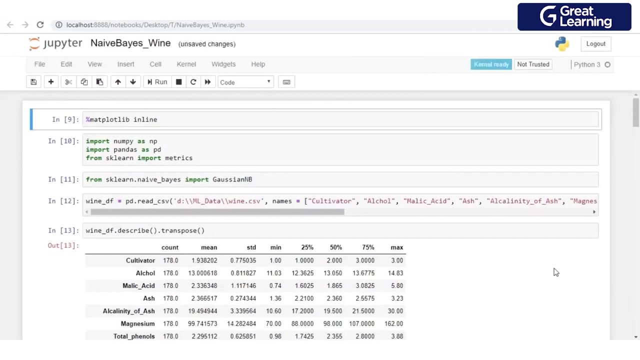 Apply this Naive Bayes algorithm on Pima data sets and see what is the result. You have to give me overall accuracy and class level accuracy, All of you. okay, Would you like to give it a shot? Then let us go through this wine data set: Naive Bayes wine. 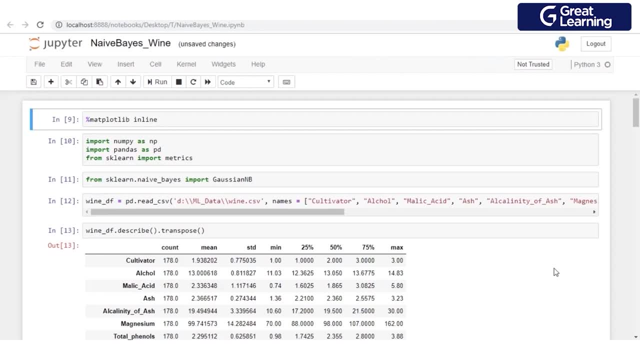 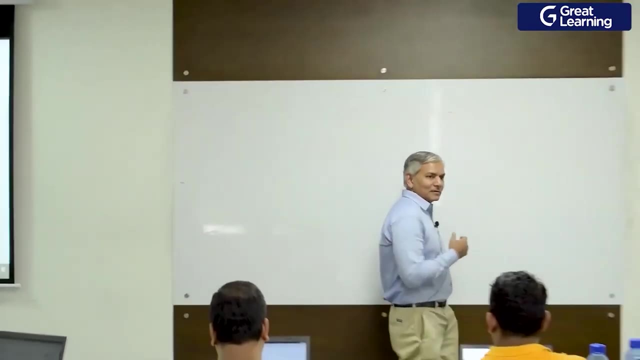 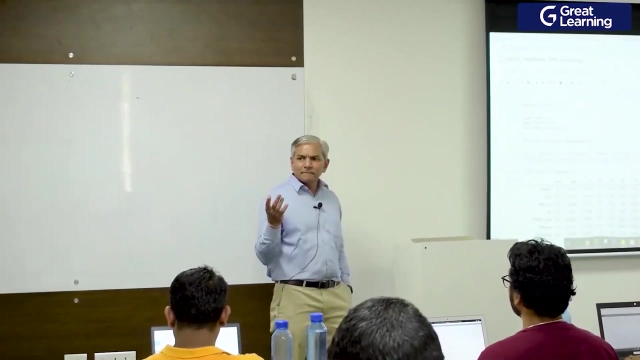 This data set has come from Italian wine brewery wine farm. This is the real data set. Apparently, there are three different data sets: Wine data set: we do not have. We do not have wine data set. that winecsv: We do not have data set. 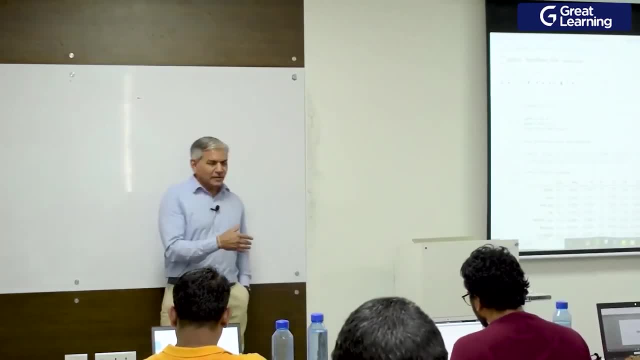 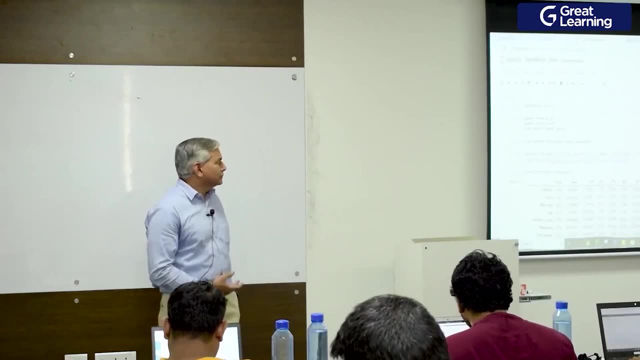 I will pass it on to you. It is there on pen range. I will pass it on to you. This is winecsv, not red, But you can try it on red also. it does not matter, They are the same, this thing. 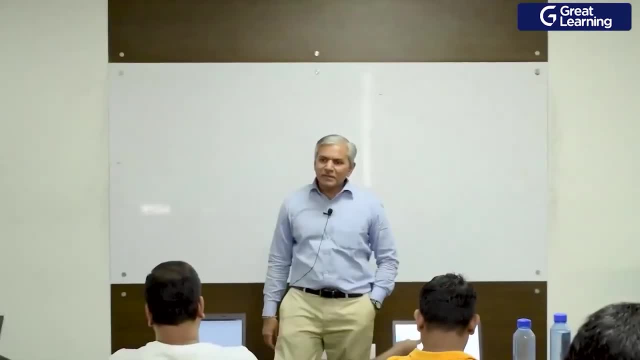 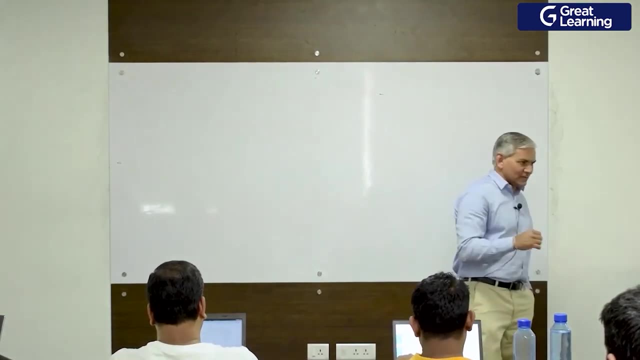 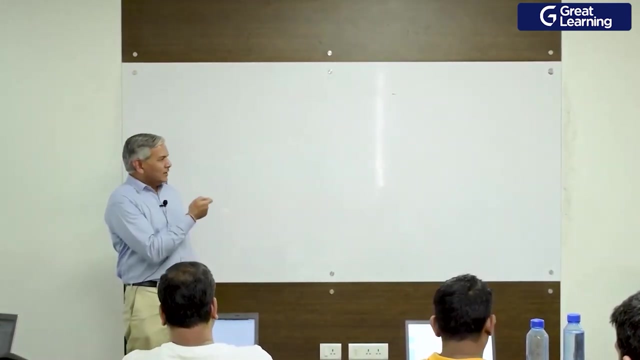 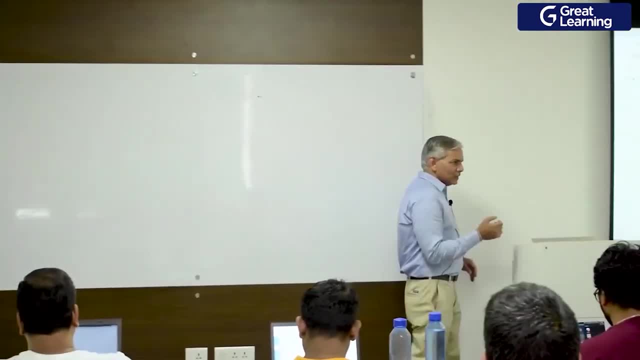 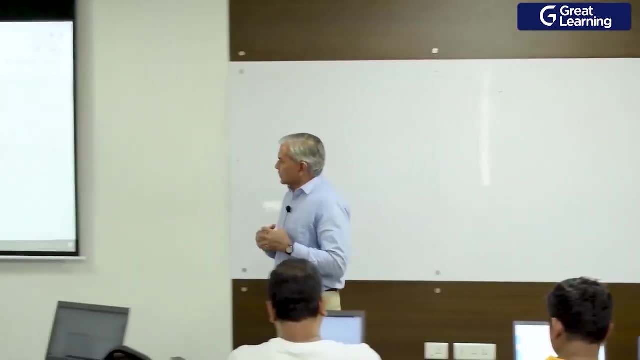 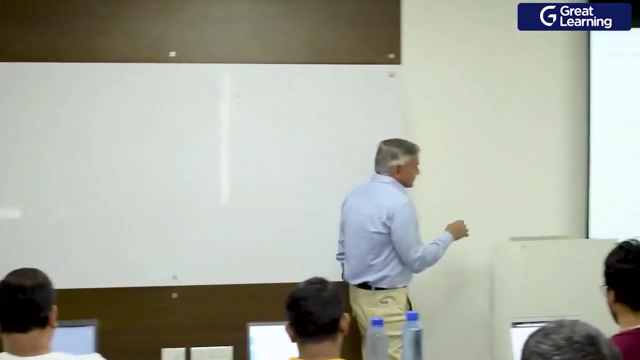 it is classified. You have specialized, skilled people who actually taste the wine and they give the classification the quality of the wine. Yeah, So this is one of the most unenviable jobs, or rather enviable jobs, where you get paid for drinking on the job, right. 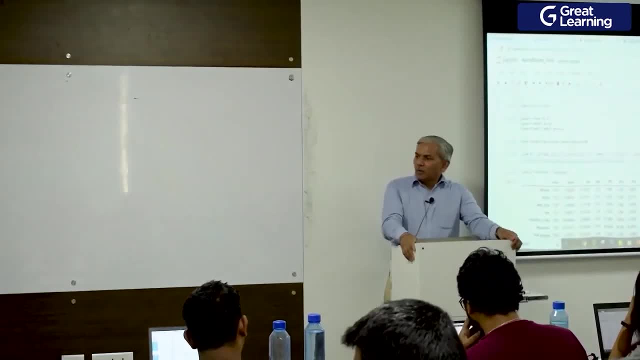 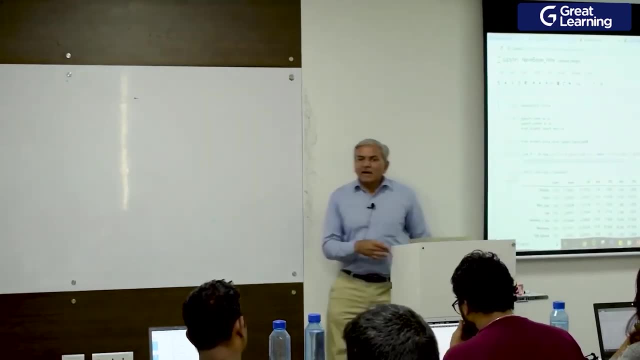 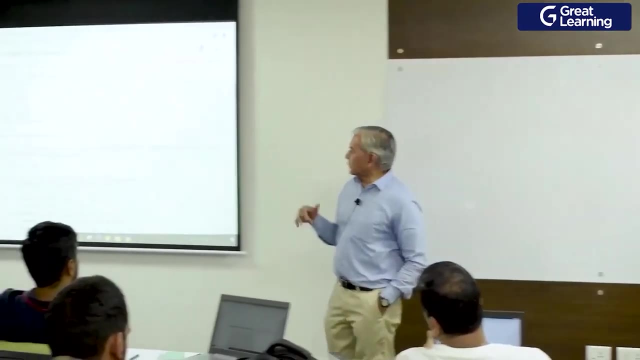 So the requirement is: can you build, using data science, a model which takes as input the various parameters of the wine and it tells you what the class of the wine is going to be? So I can replace these people with automated systems? That is the objective. 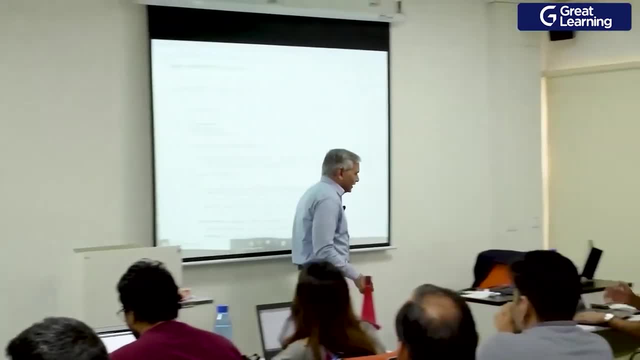 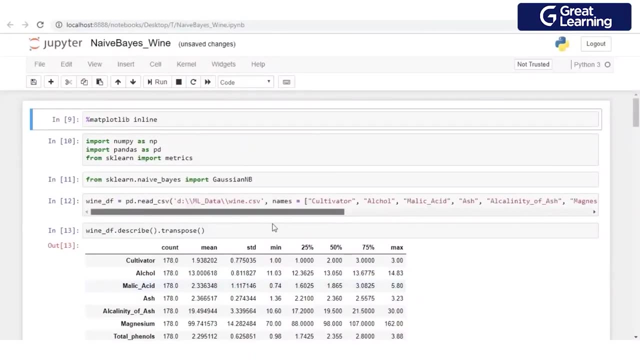 So, if you look at the data set, these are the columns available in the data which I have noted from that UCI data set: The cultivator: alcohol levels, malic acid, ash, alkinate. honestly, I have no idea about these things, but these are the various parameters available. 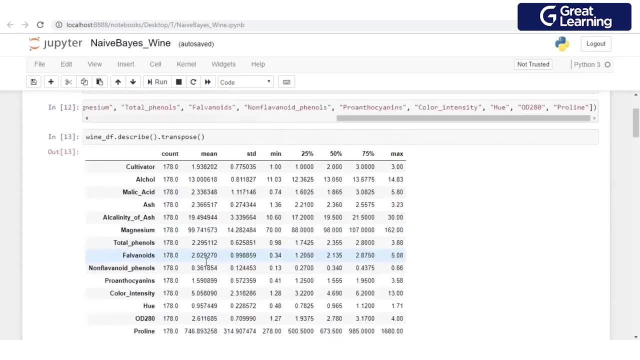 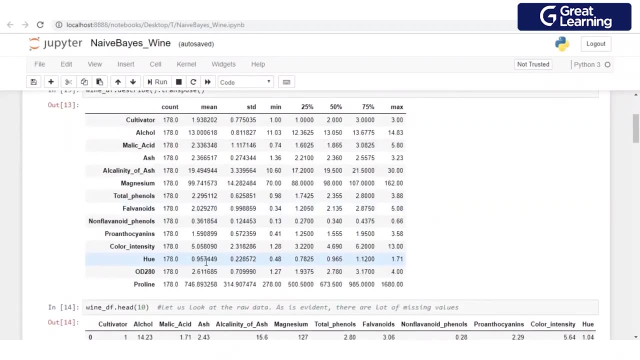 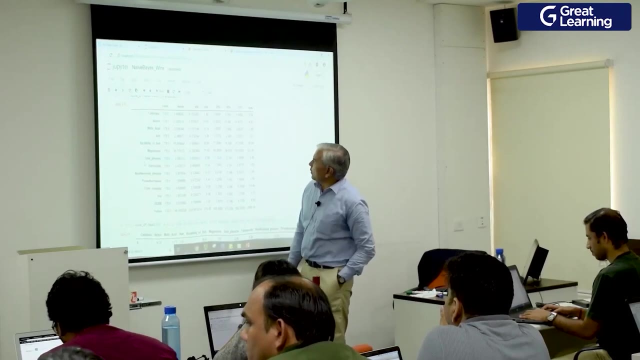 So when I load this data set and do a df describe, df, describe, df, describe once again- is used to identify the tails. Look at any of these columns. we will just look at one. Take your ok. look at this interesting. 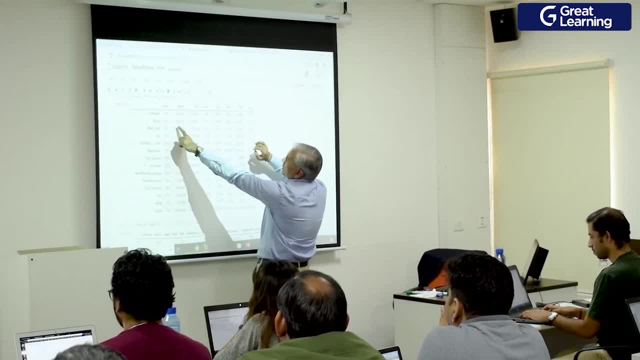 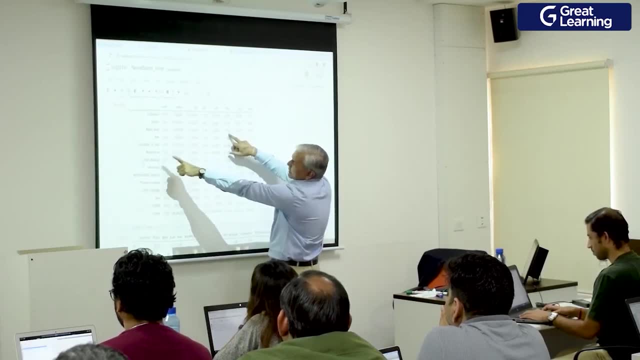 Look at: the cultivator is a categorical variable, so do not look at that. Look at: alcohol mean is 13,. median is 13. Malic acid mean is 2.3,. it is almost 2.3. Ok. 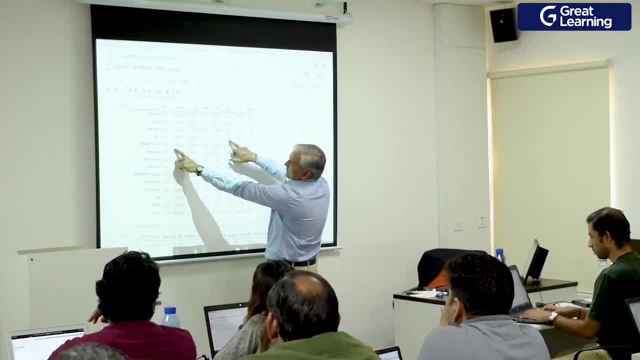 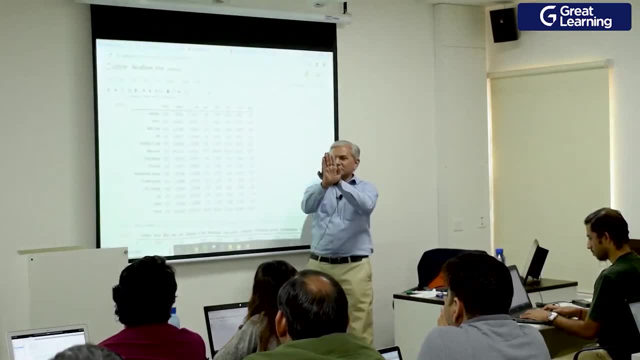 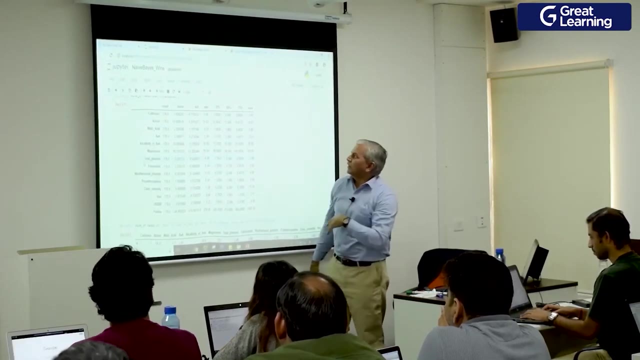 Ash: 2.3, 2.3, alkalinity: 19.49, 19.5, almost same. So every attribute, the mean and median are almost coinciding. So there is, to that extent, we are safe. Look at the tails. 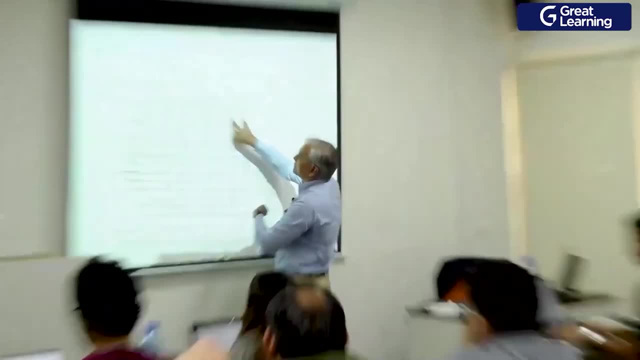 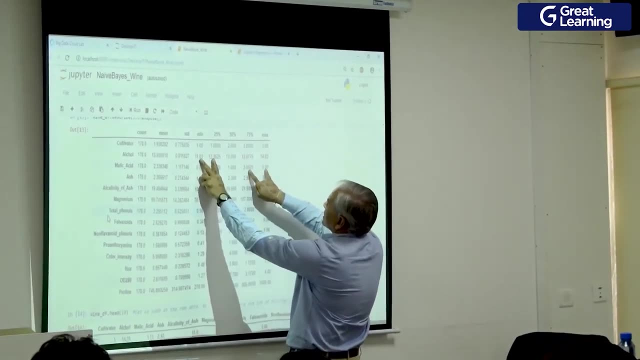 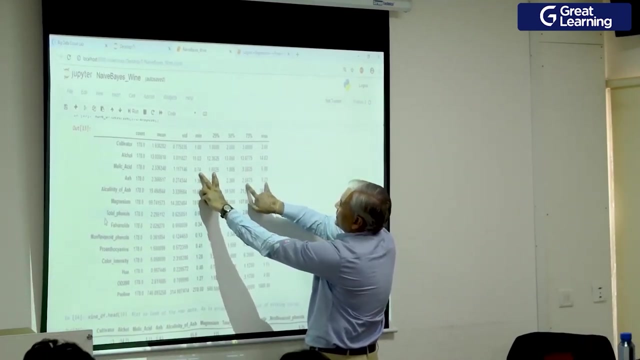 This tail is sorry, start with this. this is one, almost one unit. yeah, it is one unit. and the right left hand side tail is also one unit. This is two units. This is almost two units. This is 2.5 to 3.5 units. 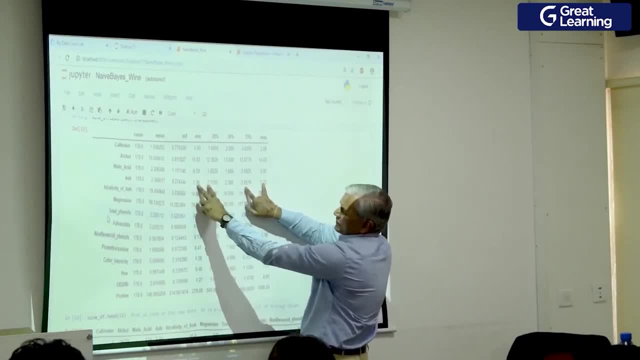 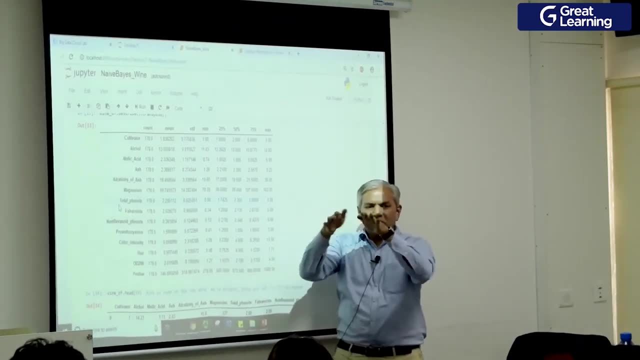 This is 1.3 to 2.2, almost 5 plus units, 0.7 units. Every dimension, mean and median are coinciding and the tails on the both sides are almost equal size, So looks like most of the dimensions. there is not much long tails. 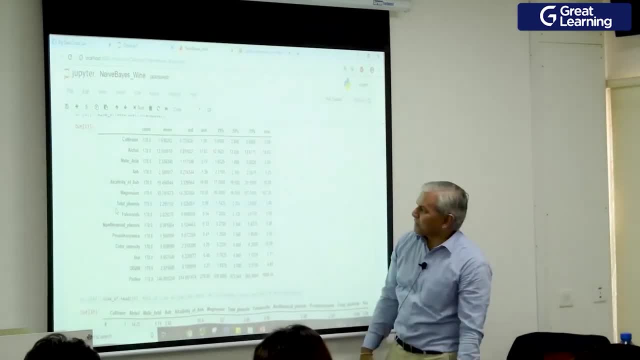 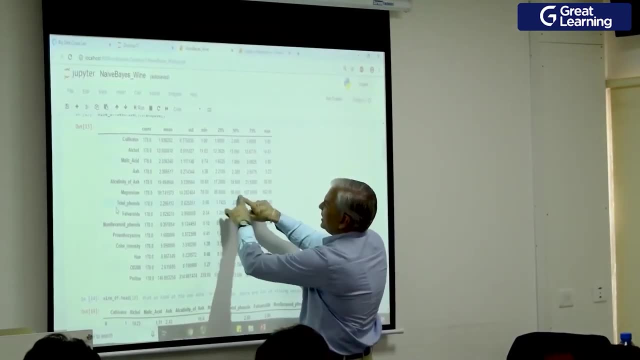 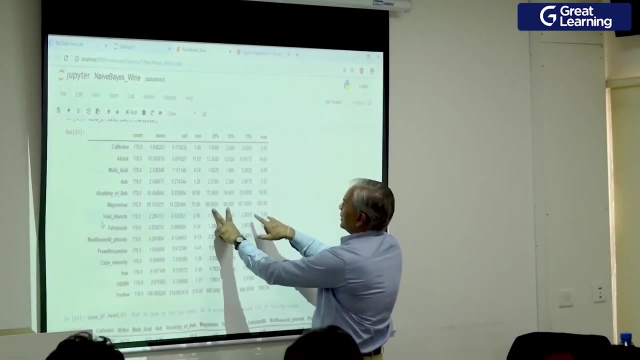 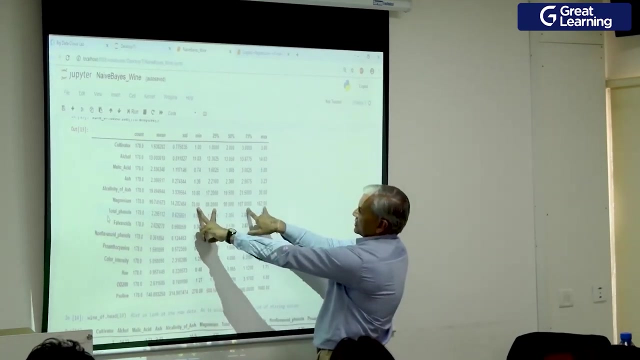 Ok. Ok, So the tails are skews. Only one dimension you will see, which is magnesium. Mean is 99,. this is 98, a difference of only one unit. Central value is no problem. Look at the tails: 10 units. sorry, this is 18 units. 18 units versus 55,, 54 units. 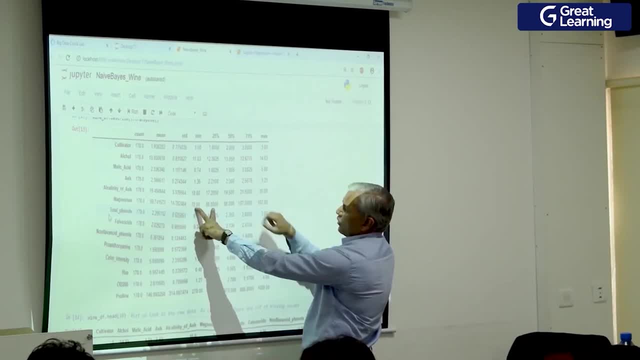 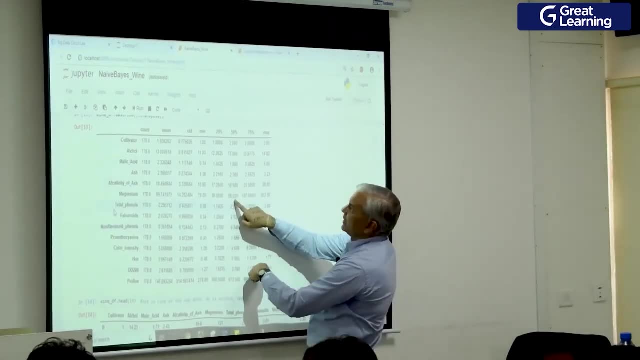 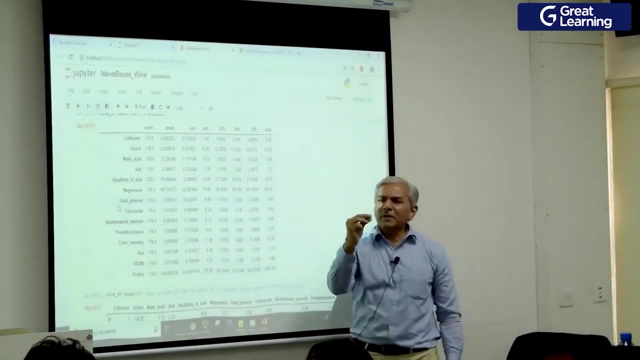 Yeah, So this tail is very long compared to the left hand side tail. So this is when when your central values are overlapping 98 versus your 99.. Central values are overlapping very small shift. That means you have only a few outliers, very few outliers on the right side. 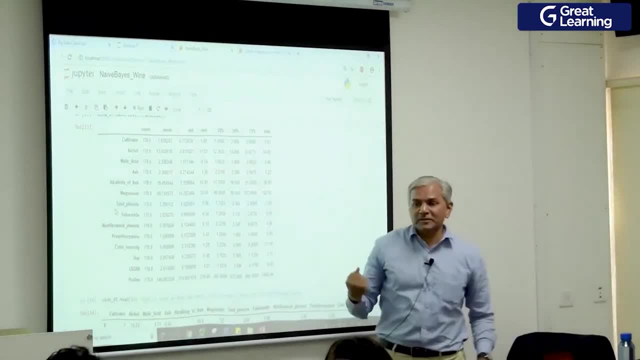 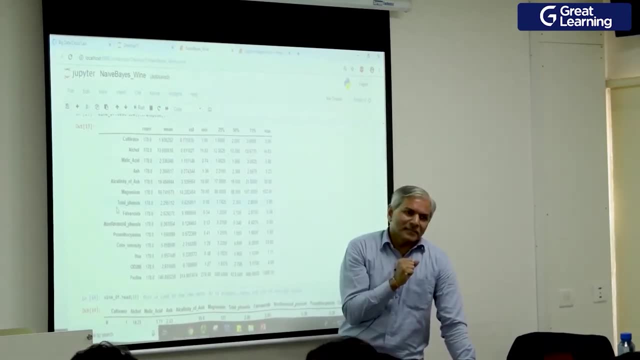 Otherwise the mean would have been drastically pulled to the right side. So one or two records seem to have outliers on that one particular dimension. So should we go ahead and do all outliers have to be handled and then replace them with some different values? dropping records is the last option. 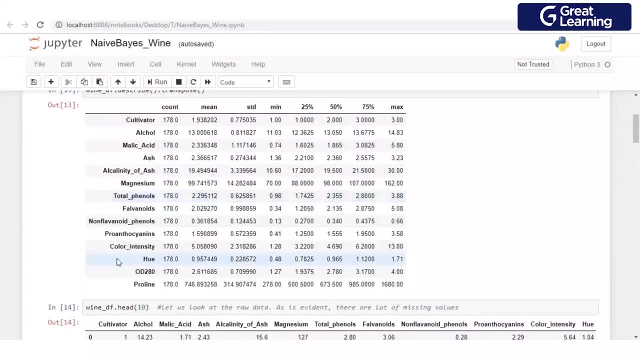 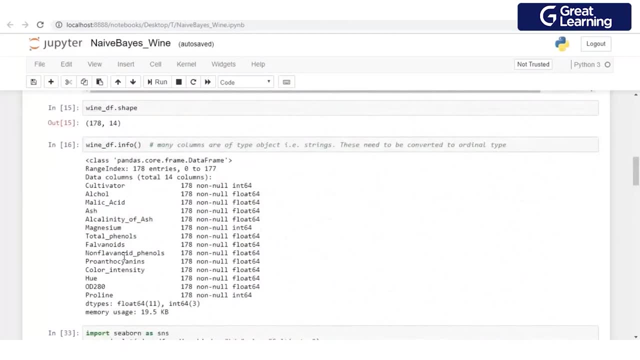 You may have to, but it is the last option. The visual way of seeing this is pair panel and this is the pair panel. I will come back to this code. I am looking at the data types here, but I will come back to the code. 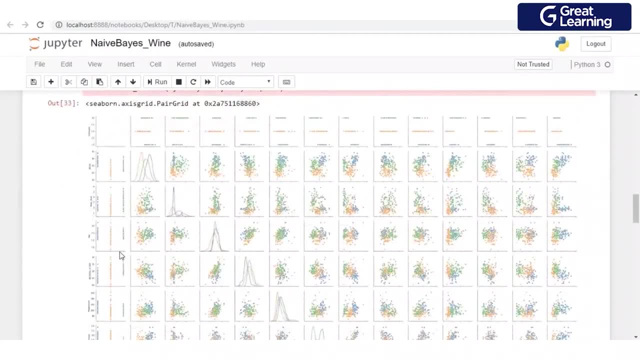 Look at the distributions And I want you to compare This distribution with Pima distribution. So let us compare this with Pima. okay, There are three classes and hence three curves. And look at these curves: They are overlapping. They are overlapping, but you see the difference. 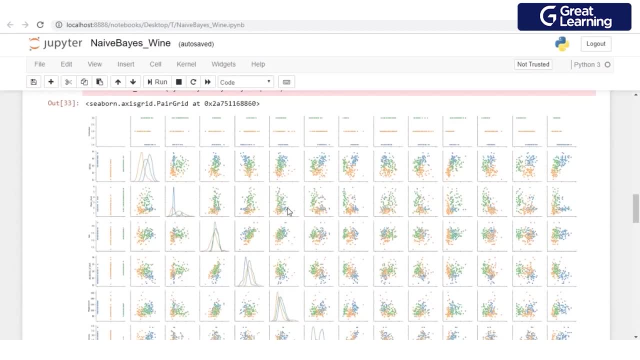 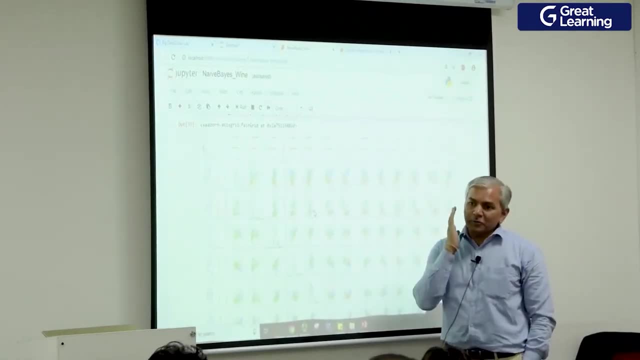 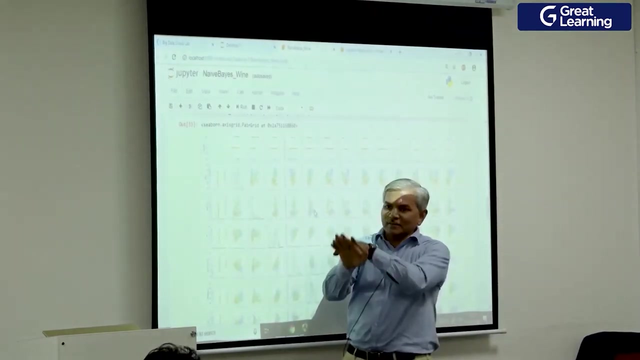 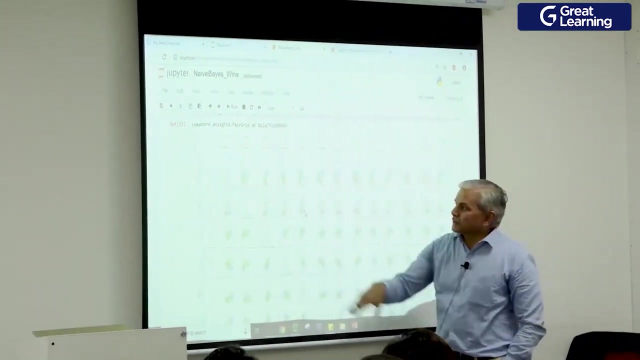 What is the difference? Central values are separated apart. The means are not overlapping, Okay, And that makes a huge difference in your ability to distinguish the classes. In Pima, the problem was even the central values are sitting on each other, So the body is significantly overlapping, but central values are separate. 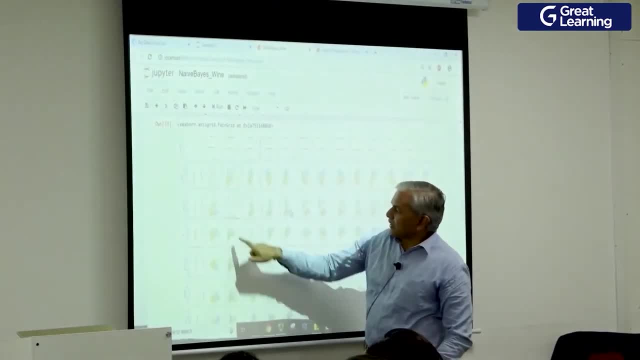 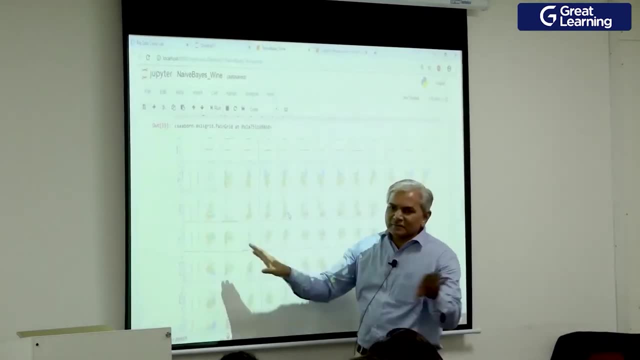 So we are in a better condition than we were in Pima. Look at this column: The blue and the orange are overlapping. even the central values are overlapping, But at least the green is away. Okay, So all the columns? this is. I think this is the worst column we have. 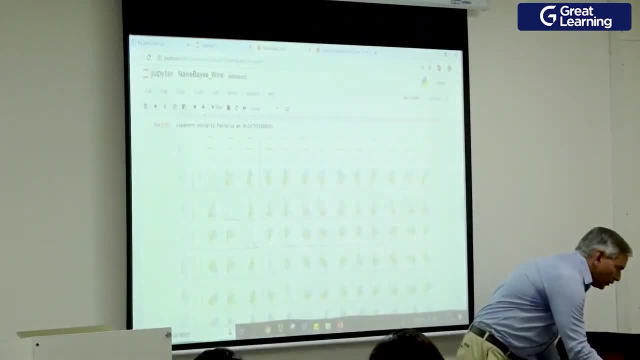 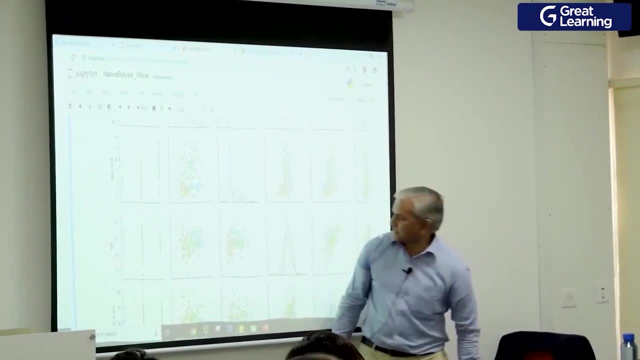 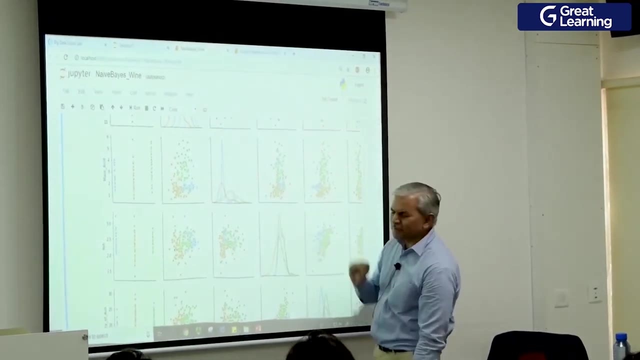 This is in your data sets, where all the three columns are absolutely sitting on top of each other: This one And this is Ash, Okay, Ash. all the columns, all the classes are sitting on top of each other, including the central values. 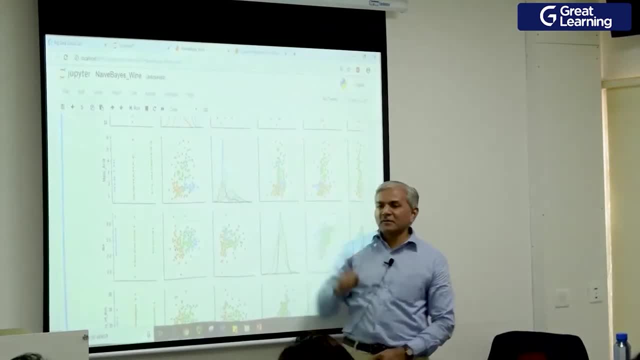 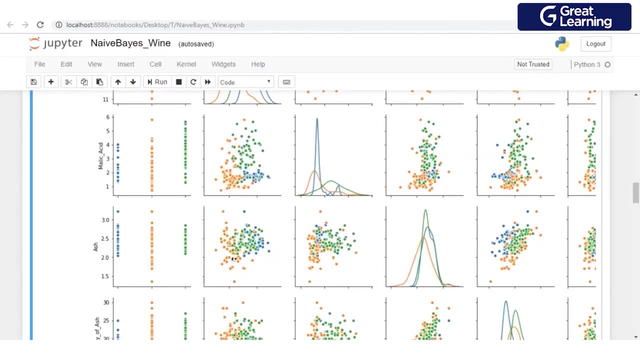 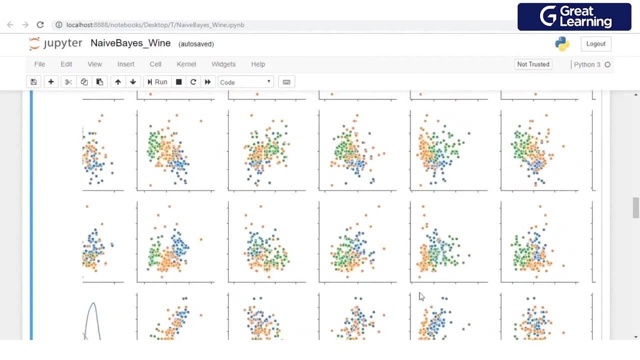 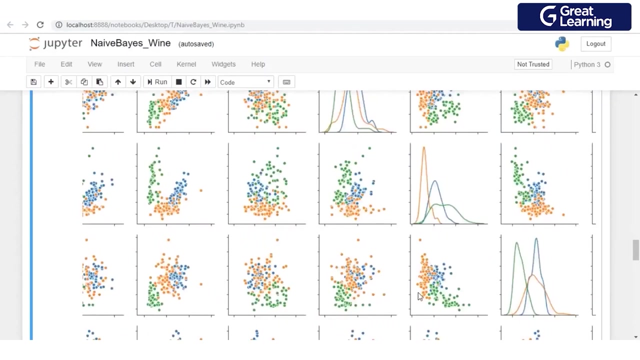 However, because I have other attributes which can help me segregate. Okay, I can ignore this Right. There you go. So in many of the dimensions, two classes are overlapping, but as long as the third one is away. So this is what I was saying. 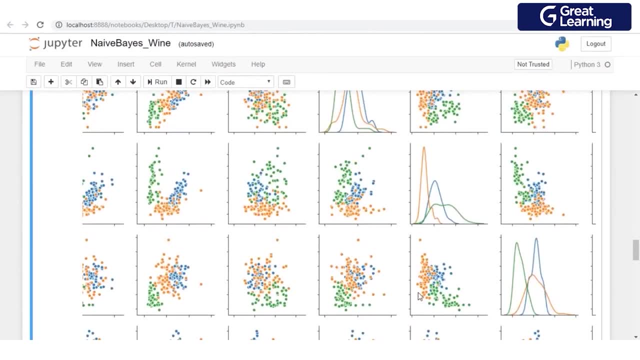 If you have a dimension in which the two classes are significantly overlapping, small change in shift. But when I combine this with another dimension, The two gaussians, they become linearly separable. So I am seeing this, I am seeing this distribution this way. 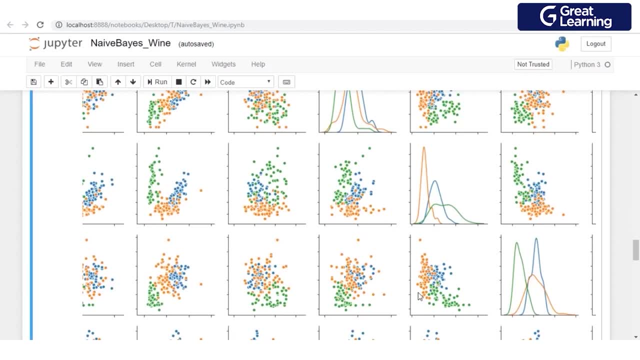 I am seeing this kind of overlap. I will redo this. I am seeing this kind of overlap. I am when I use another dimension in the other dimension also I am seeing an overlap. But when I put them together in that mathematical space, the two gaussians become linearly separable. 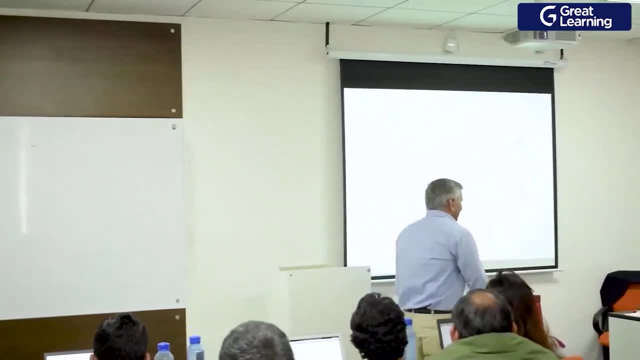 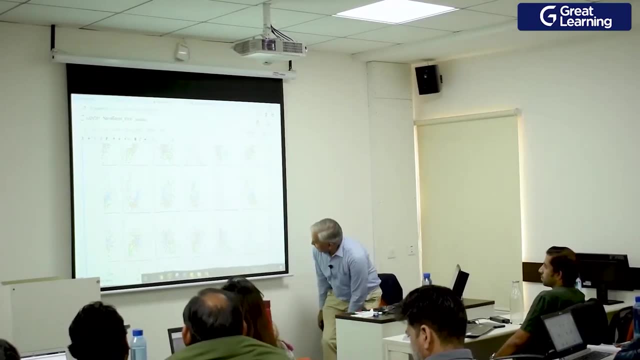 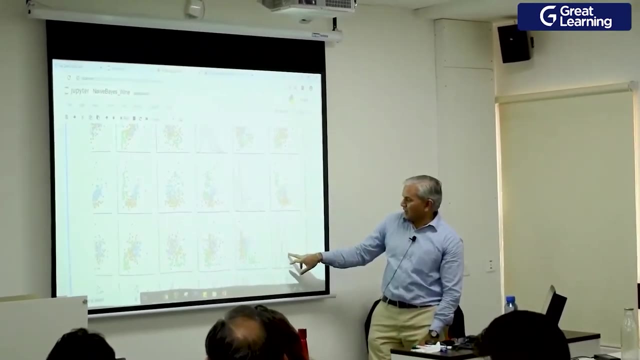 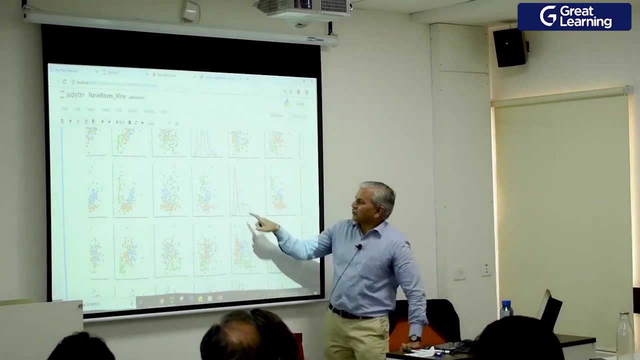 Because of that linear separability now possible amongst the classes. on the dimensions, Look at this dimension, This one- I do not know which one is this. This one is not going to help you separate the orange from the blue. Does not matter, as long as I have this dimension with me which separates orange from the blues. 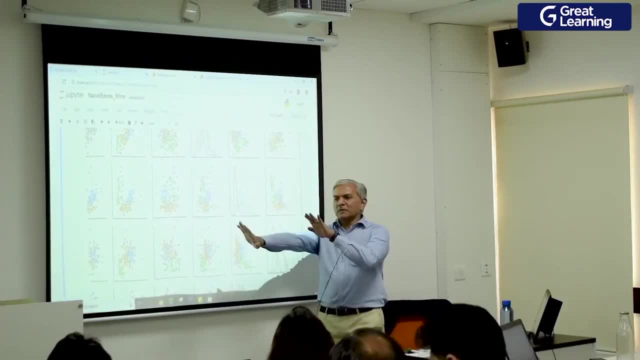 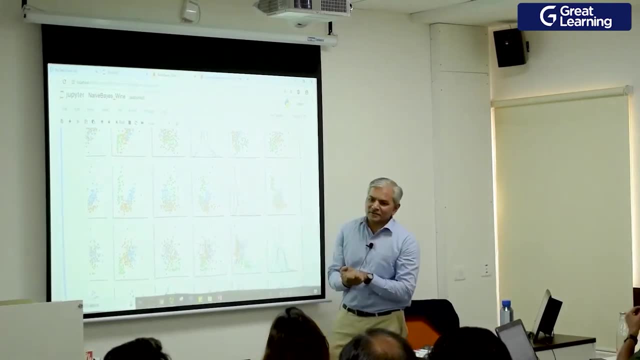 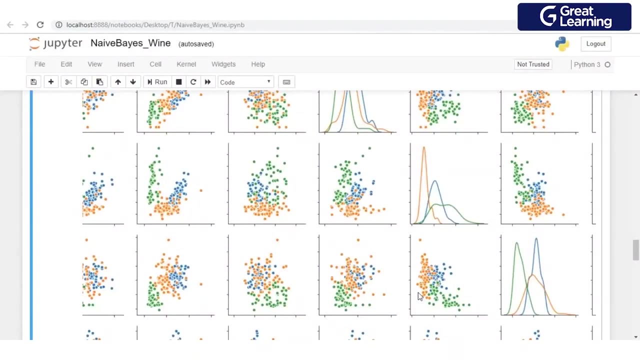 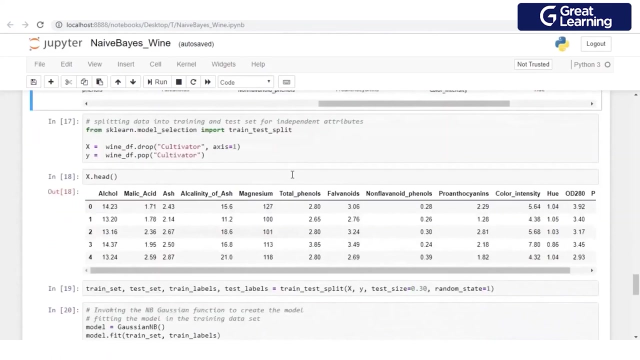 So one dimension will compensate for the other dimension. So, overall, these weak predictors put together become strong predictors. Exactly, Overall, these weak predictors put together become strong predictors And, as you will notice when you go down the line, Look at, let us look at- the data types. 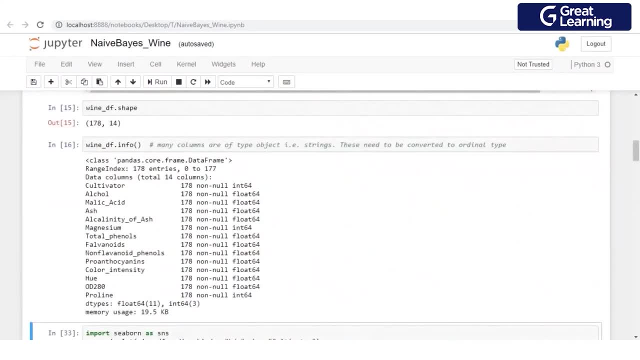 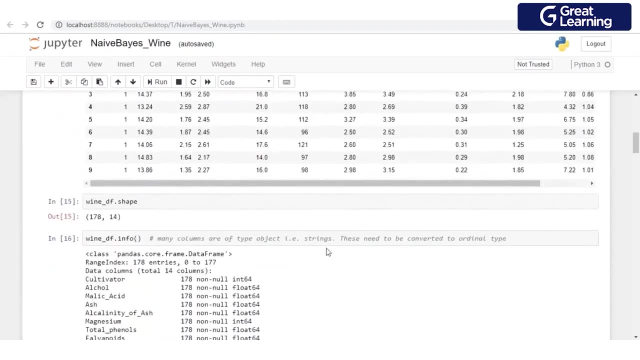 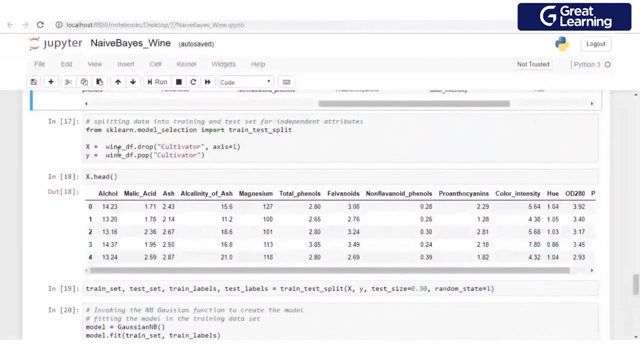 We do not have any non-numerical columns here. Everything is numerical. Keep in mind: all algorithms need numerical columns. only Numerical columns could be categorical or real numbers Come down. So I am separating out the x variables independent variables. 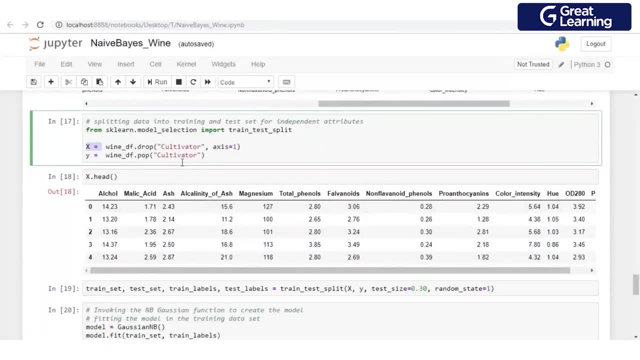 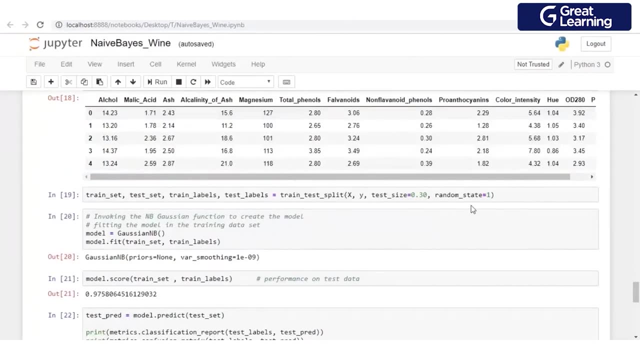 The target is the cultivator. I am splitting my data into training set test set. I am splitting my data into training set test set. Are all of you with me on this? You can actually download the data set from UCI if you wish to. 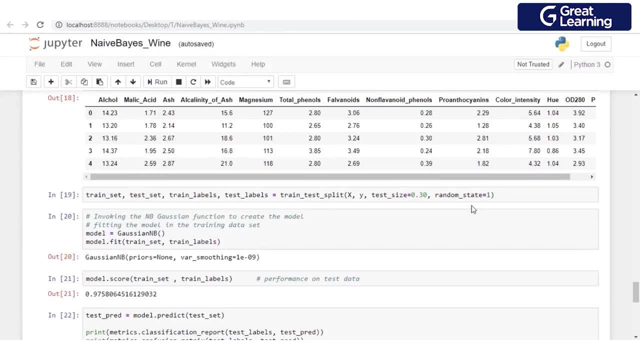 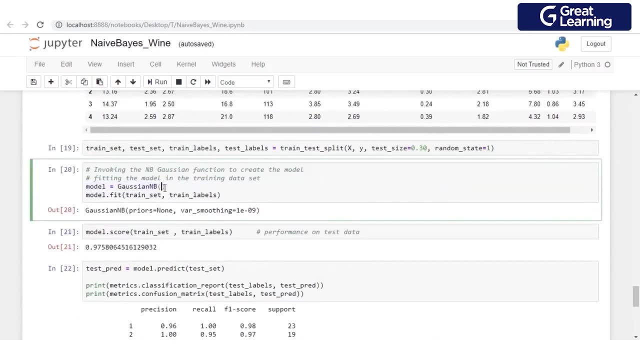 This data set you can download from UCI and run the code. Very good, I am instantiating the Gaussian Naive Bayes here. There are different variants of Naive Bayes. This Naive Bayes assumes that the dimensions, The dimensions, are Gaussian. on each one of these, 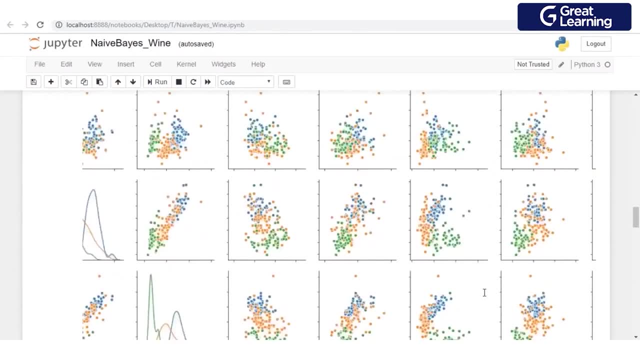 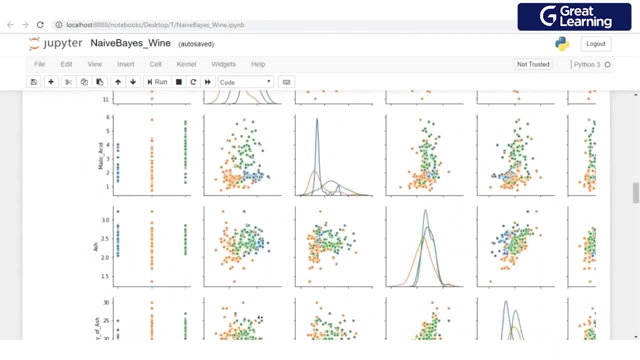 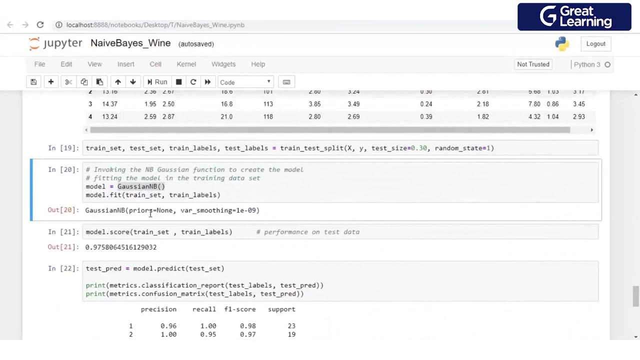 The distributions are Gaussian on each one of the dimension and we meet that requirement very well. On all the dimensions the classes are distributed in almost Gaussian ways. Gaussian means looks like normal distribution, So perfect case for Gaussian Naive Bayes. So I am calling Gaussian Naive Bayes here. 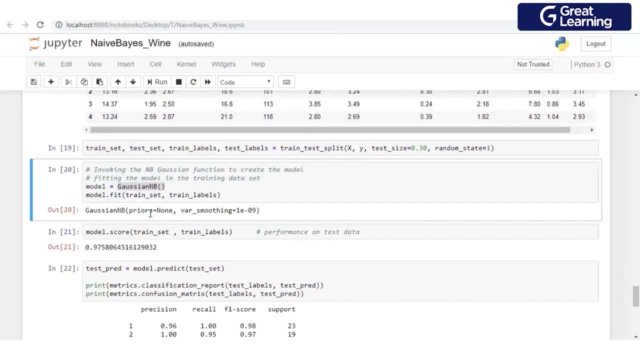 There are other variants, like Multinomial Naive Bayes and other Naive Bayes which you can make use of. So I am instantiating the model here. I am gaussing, I am going to do the model fit here. This is where our this Naive Bayes likelihood ratios will be calculated. 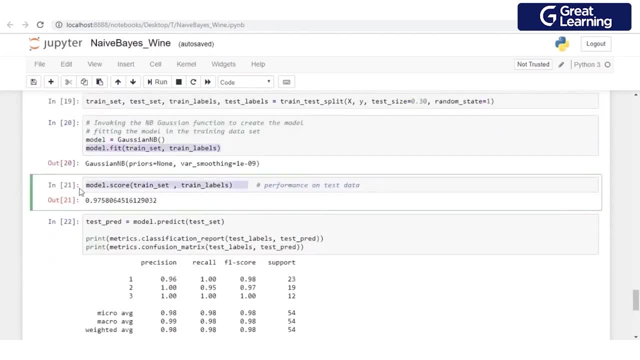 And then I look at this On the training set itself, I am doing a testing. It is giving me 97% accuracy. Why am I doing this? I will tell you in a minute, While I can also do this model on the test data. 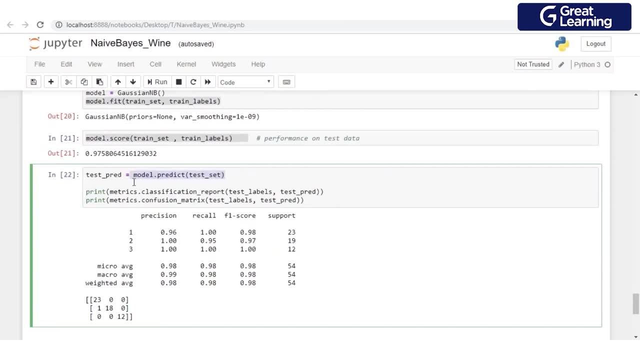 Here I am running the model on the test data. Ok, And in matrix there is a function called classification report which gives me this: all this matrix, recall, precision, everything in one shot. If you are interested, you can separately print the matrix also, confusion matrix. 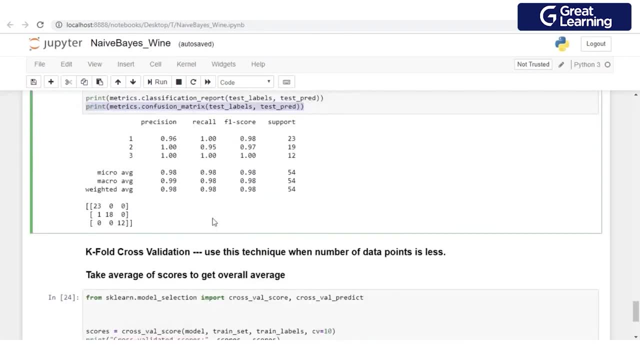 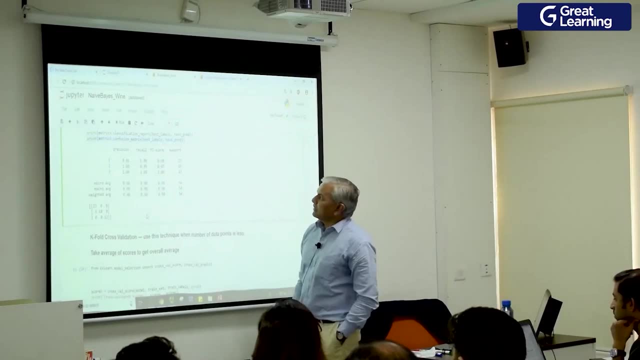 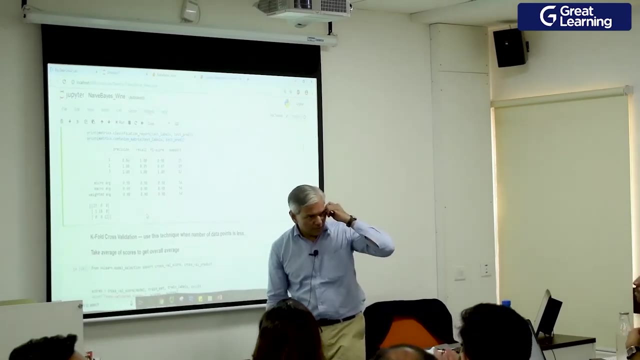 Now look at this confusion matrix. Look at this. Look at the class level recall. Look at the class level recall. Any problems? Hey, Mohit, Mohit, any problems from SQL and import gaussing? Ok, Alright, Now look at this. 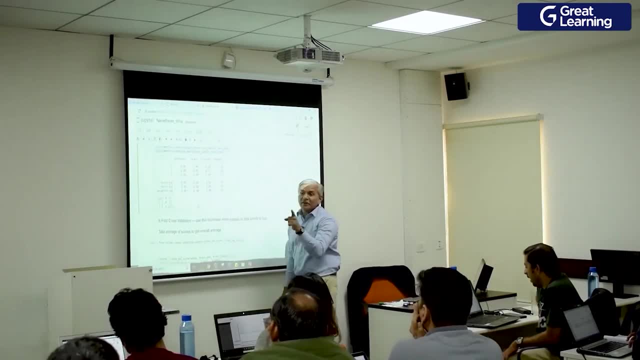 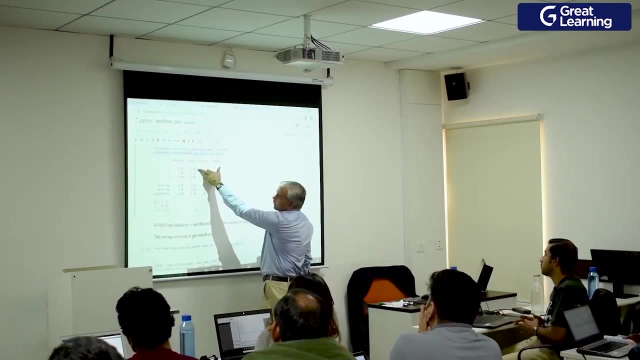 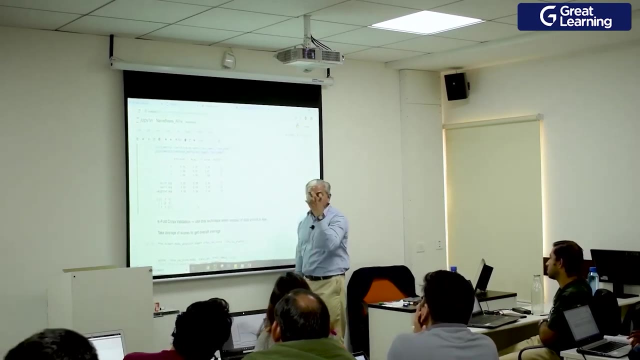 There are three classes here, 1 to 3. And look at the class level recall. What is class level recall? Accuracy at class levels: almost 100%. One means 100, 95%, 100%. So each one of the classes it is able to accurately classify with precision. 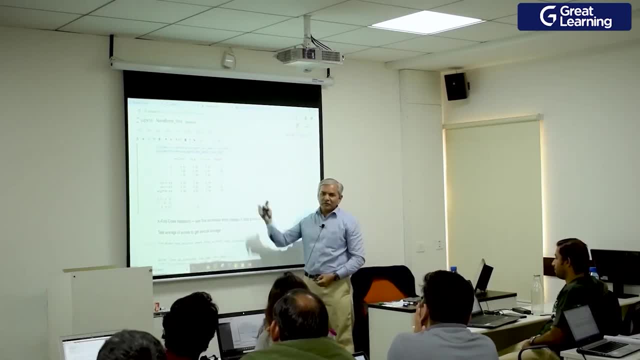 Ok, This is the degree of. this is what we wanted in Pima Diabetes. It is giving us accuracy in wine data set. Ok, I will talk about this micro average and all these things down the line. We will talk about this later. 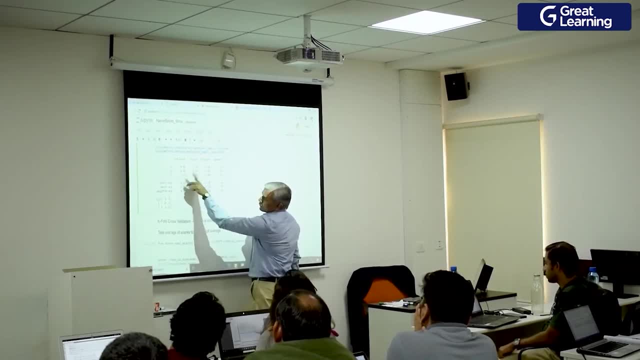 Right now. just look at this recall matrix- I have not told you what precision is- And look at the confusion matrix. Actual number of class A in your test record is 23.. All of them have been classified as class A. Actual number of class A in your test record is 23.. 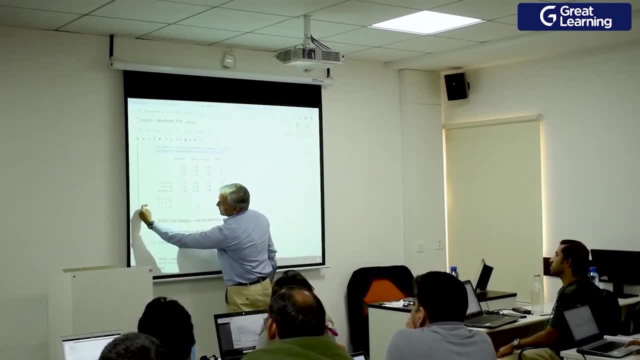 All of them have been classified as class A. Actual number of class A in your test record is 23.. And score is 33.. So each volume is recorded as B. The number of records for class B in your test data is 19.. 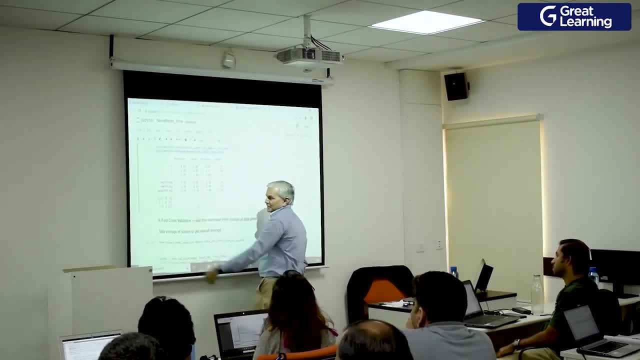 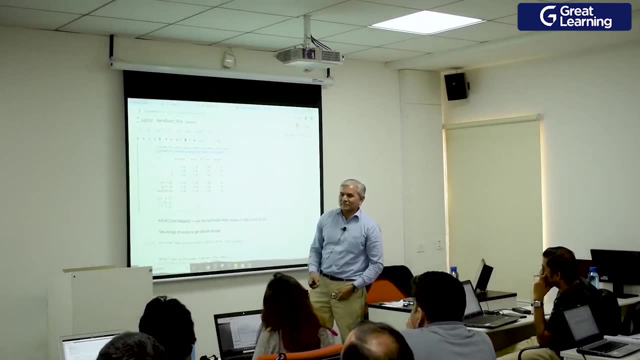 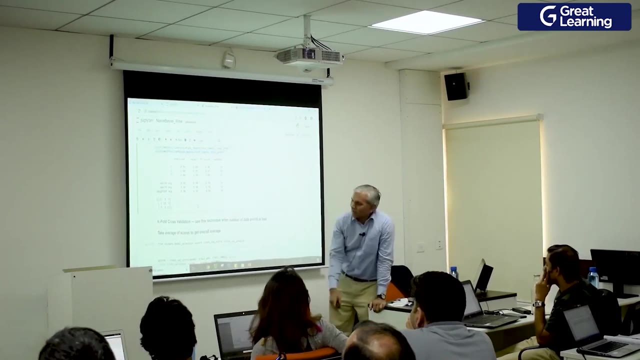 It has correctly classified 18.. 12,. it has correctly classified 12.. You are able to achieve this kind of a score in this model even though the dimensions are overlapping. the classes are overlapping in all the dimensions because of some dimensions which come together to make strong predictors. 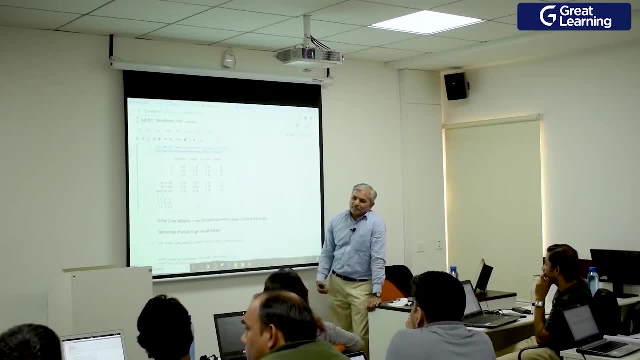 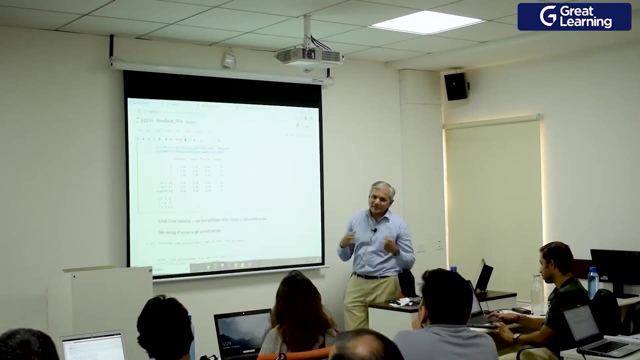 Right. Ok, So you should understand the difference between PMI diabetes and this. in both the cases, the classes are overlapping, but there is one very important critical difference and it is that difference which is making this right. So you can run the same algorithm- Naive Bayes- on PMI diabetes and see what is the score. 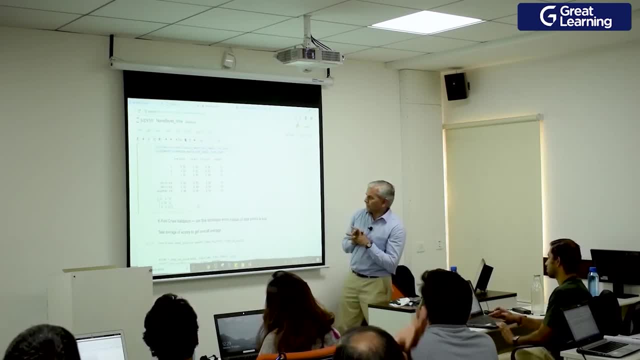 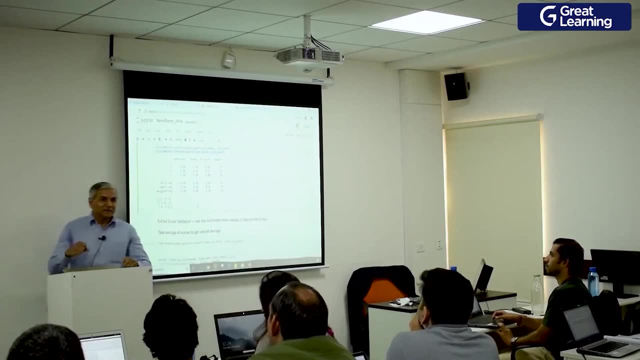 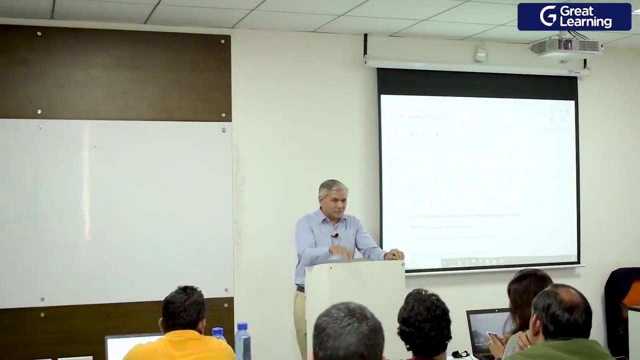 you get there. Your job here is to select the right attributes, but this is: you will never get data on a plate when you are doing real life projects. This is only a classroom, but when you do sit down and do real life projects, the customer 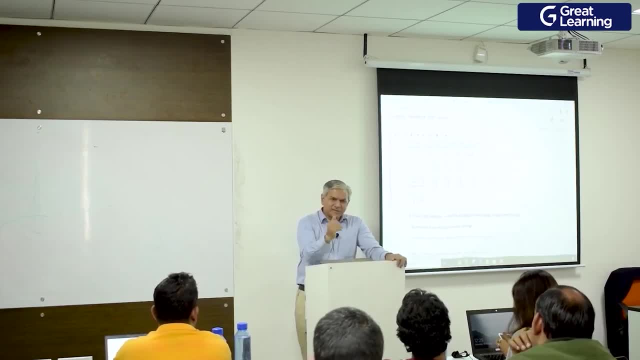 says like: suppose a simple example: Can you use data science to image: Can you improve my customer CSAT rating from the current 3.5 to 4.5 out of 5?? Can you do something using data science to help me improve my customer rating in my technical? 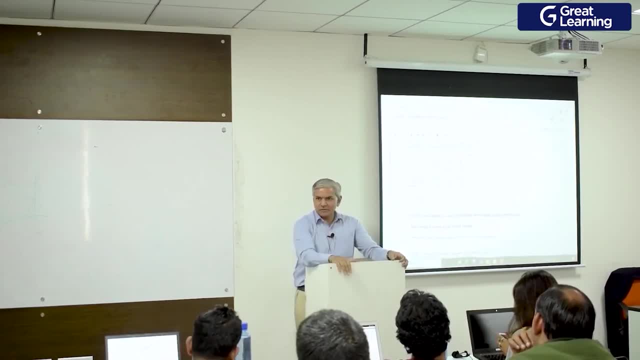 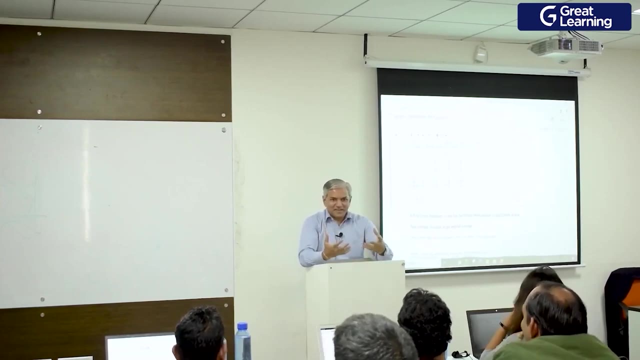 support. These are the kind of requirements which will come to you. data will never come to you. So now your job is CSAT rating, customer rating for technical support. What kind of data you need, Not desired. You have to first guess. 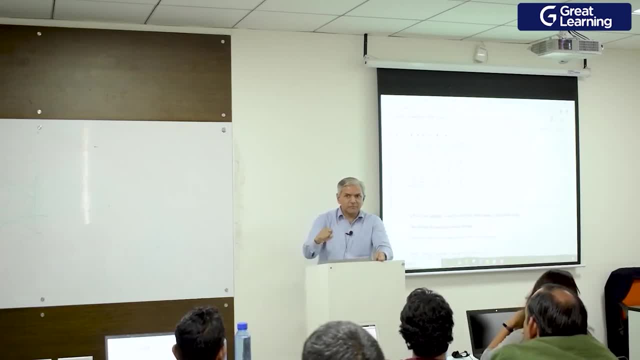 What kind of data I need. Your domain expertise will help you. If you don't have it, you need to have domain expertise. So for CSAT rating in customer tech support, what kind of data I need? can somebody give? Go back to the past tickets, ok. 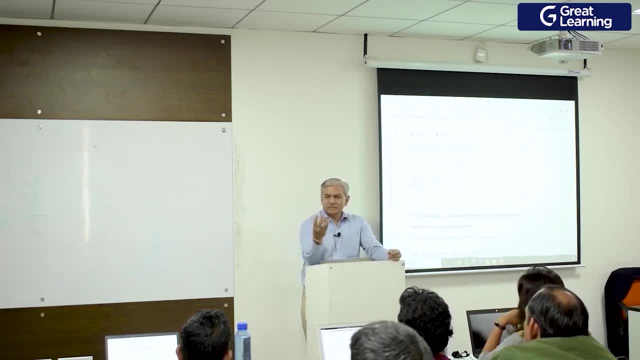 Go back to the past ticket. What kind of data you need? Go back to the past tickets. From the past tickets you collect. what kind of ticket- P1,, P2, P3 tickets. I need to find ticket classes then, whether the ticket belong to hardware, software or. 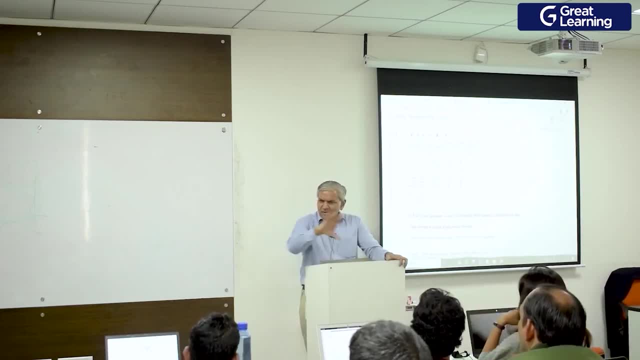 something else. I need those things and various other. you will decide what kind of data you need. The next challenge will be: where will you get the data from? Some data will be available within the organization. Some data will be available outside the organization. 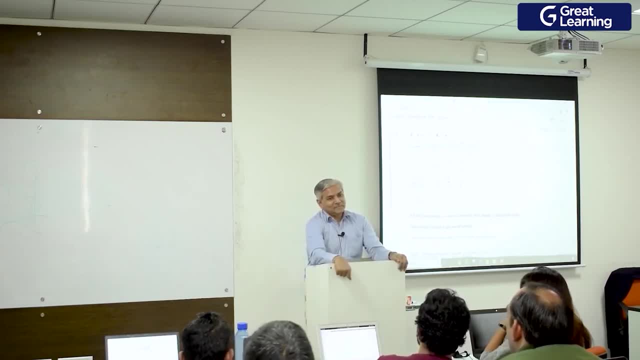 Some data will be available with the customer, So getting these stakeholders to give the data to us will be such a challenge. So all your soft skills will come into play right. So once the data comes in, you have to first establish the roadmap. 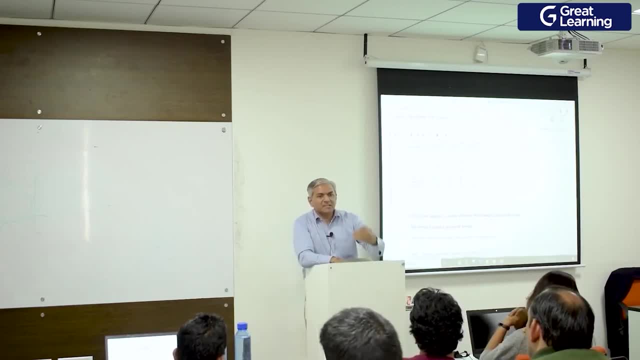 Ok, Establish the reliability of the data. What if the tech support department has given you data where customer is very happy? They have not shared with you the dirty data. Your model will go for a toss. Those are the challenges which you will face as a data scientist. 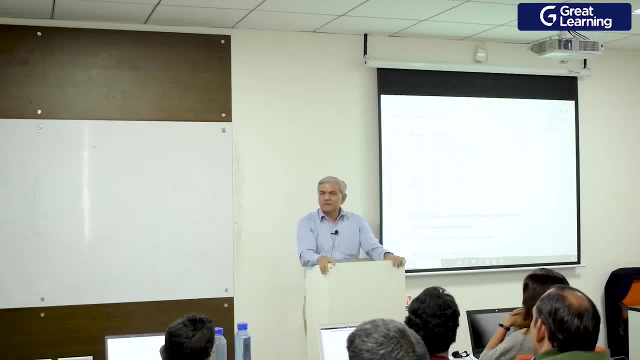 Once the data comes to you on this various attributes that you have, you will do this analysis using pair plot and other techniques. Is this column good or that column good? Which column should I use? Which column should I use to define customer satisfaction? 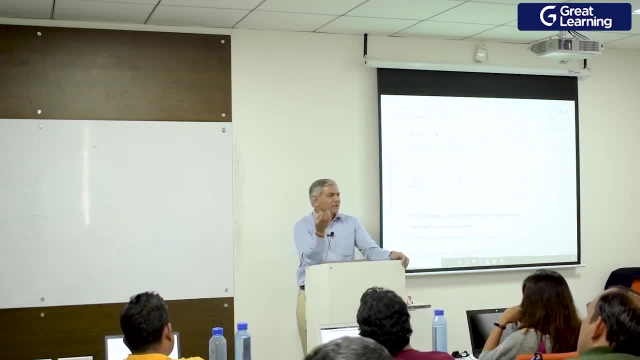 I come from the IT world, just like you do, Many of you do. We people have done lot of projects in Java and C and all these things. The project starts with customer requirements which we turn into technical requirements, That we turn into design requirements. 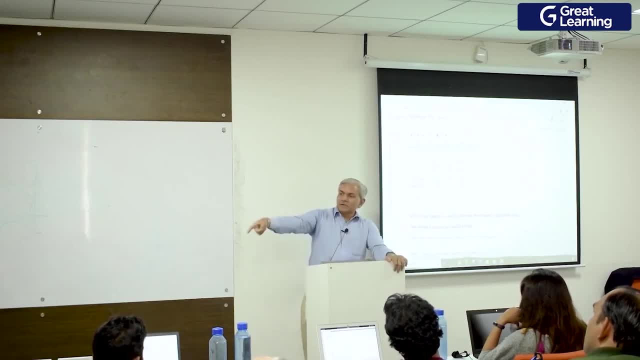 That turns into code specs, coding requirements. That turns into unit testing, integration testing and finally some. then we go for acceptance testing. Ok, Acceptance testing. usually it bombs, right. The reason why it bombs is we look at data only in the last stage, where we come to acceptance. 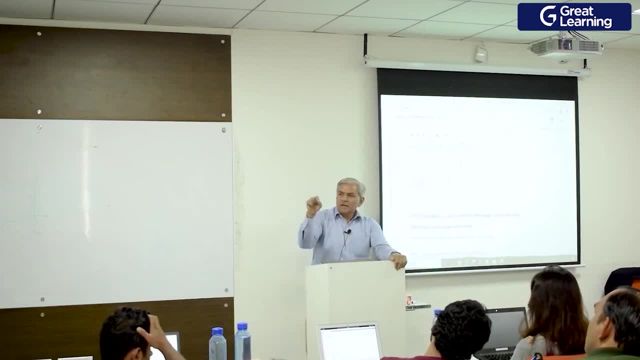 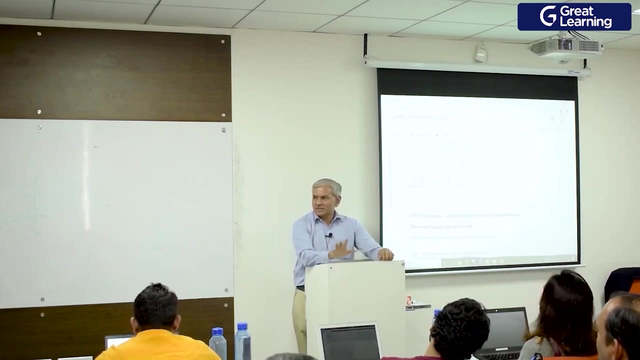 testing. We ask customer to give us some data. In data science projects your project will start with data. the project will end with data. Data is the core. You will be revolving around the data sets. So 80 percent of your effort, estimated effort, in data science project. you will see that. 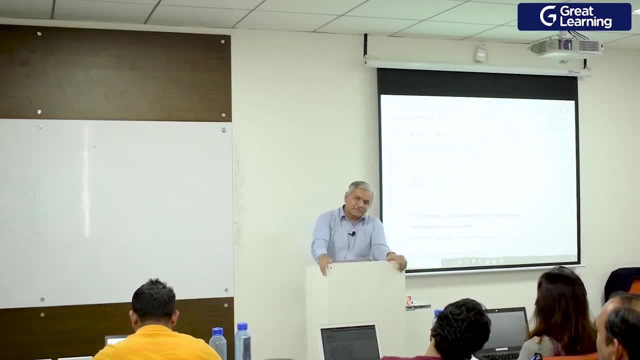 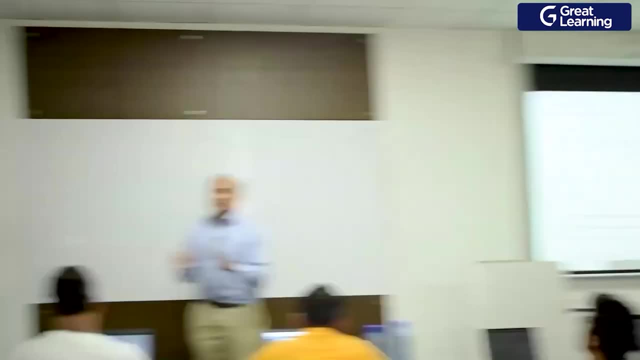 when you do the capstone project You will go in getting the data. So it is usually start with data given approach and the end with data telling- Hundred percent And end with data telling story- Yes, hundred percent Visualization and the story telling from the data. 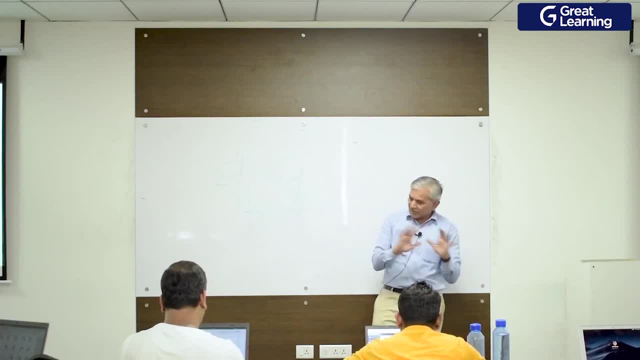 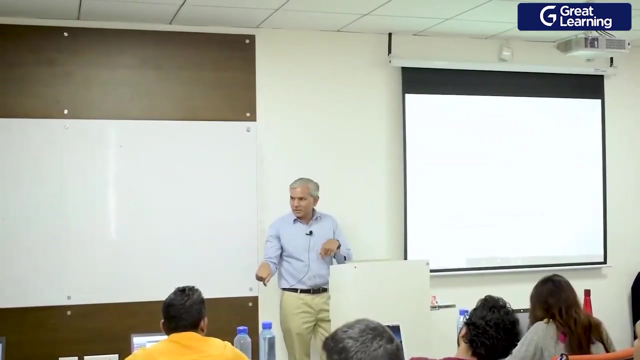 That is what data science is. So, in between the data analysis, In between the data analysis, feature engineering, feature selections, model tuning, all these things come in between, Ok, Ok, Ok, don't make this assumption in this hands on exercise we are doing in the class you. 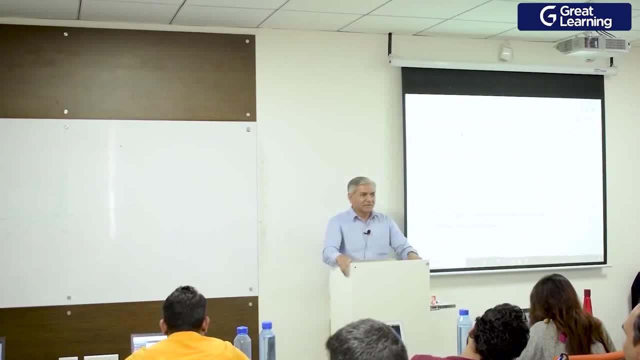 are getting all the data from right. this will not happen in real world. That's why, when people come and do capstone projects, many of them want to do self-driving cars, so we have to take them out separately and tell them: was hold on at least a decade. 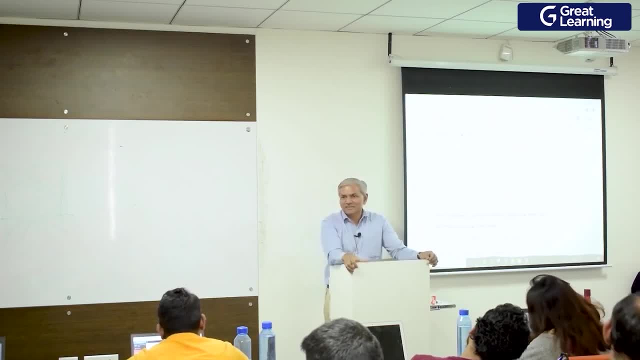 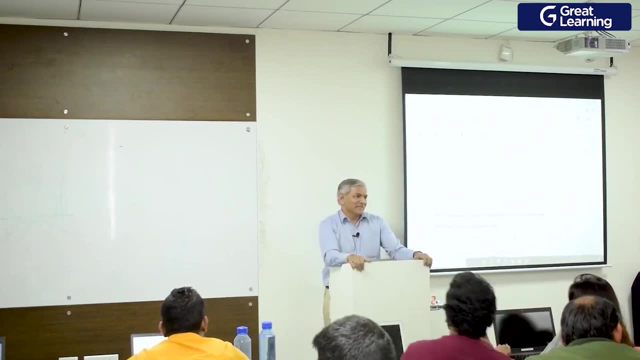 of research has gone into building those self-driving cars. you can't do it in 4 months, So when you come to capstone project stage, you are very far away from that. please sell it to capstone projects with care, right, guys? ok. 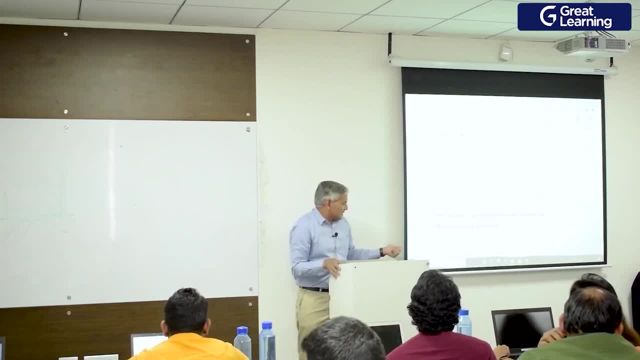 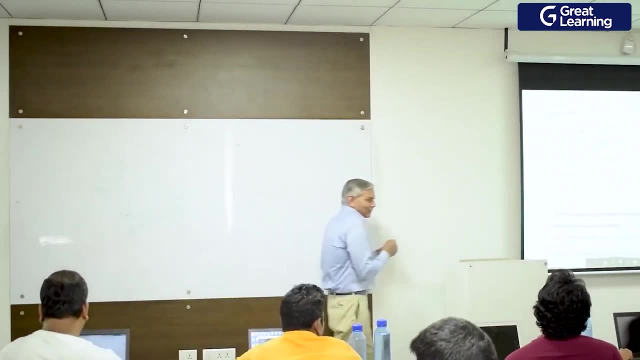 What I am going to show you is one more thing. ok, though this is kind of a doing very too early in this for you, but still let me do it. when you build these models, ok, we need to understand how the model is likely to perform in production, because I am going to put the 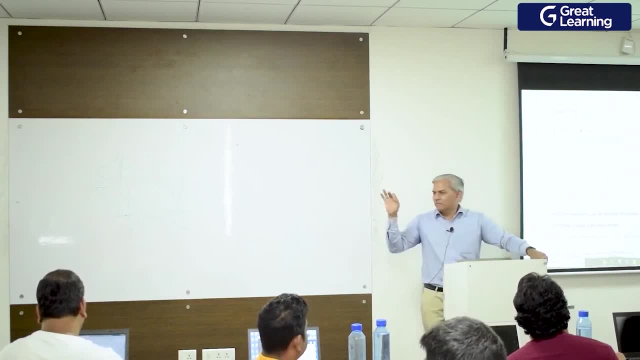 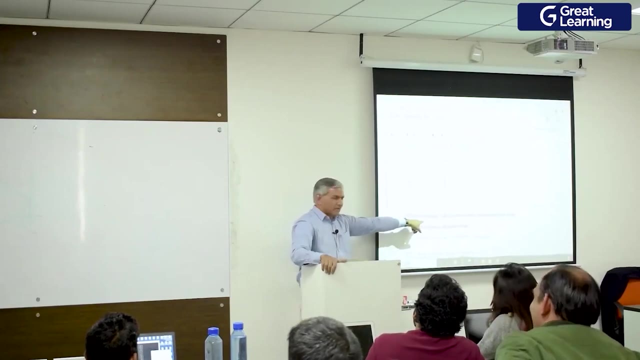 model into production, Which means I am going to disrupt many of the processes in production. So the stakeholders in production are going to ask me: what is the performance you expect from this model in production? Suppose somebody asks you this question, what is your answer? ok, it completely match with. 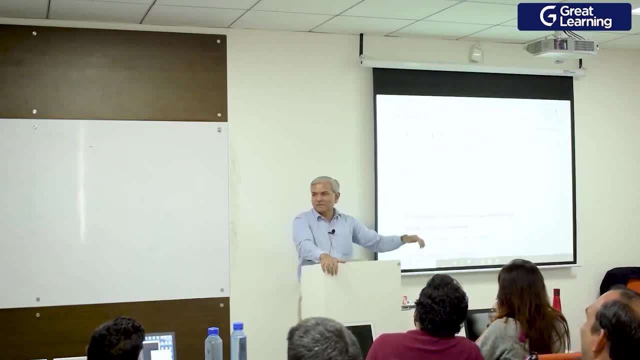 this what I am going to cover, because how do you prevent this from happening in production? So when somebody asks you this question, what is the performance you are likely to have in production? we never give point estimates. we never say: my model is going to give 78%. 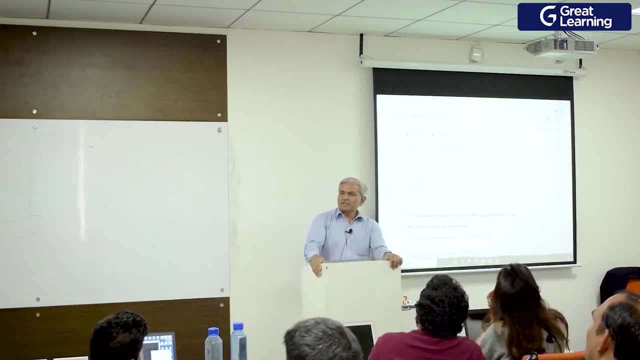 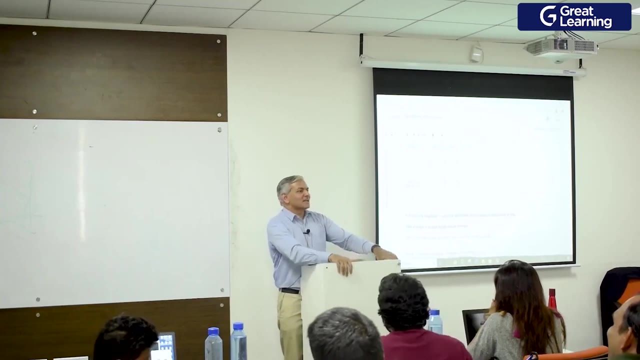 or 80%. we always give a range estimate. My model is likely to give me accuracy between 80% to 95%. The moment you give range, that means you are not 100% sure. The moment you are not 100% sure, statistically, you are supposed to associate with a confidence. 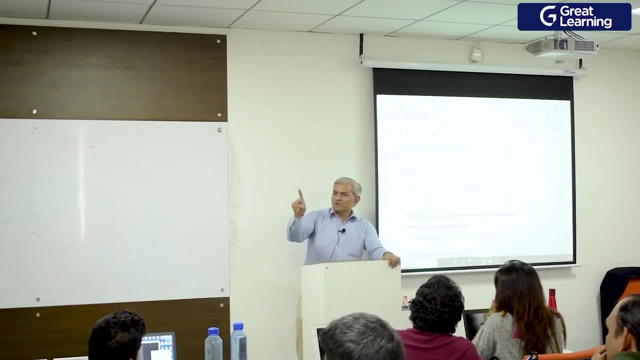 level. How confident are you in this range? So usually the confidence level is measured at 95%. So we give a confidence level of 95%. Ok, 95%, confident that my model is going to give me accuracy between X and Y. 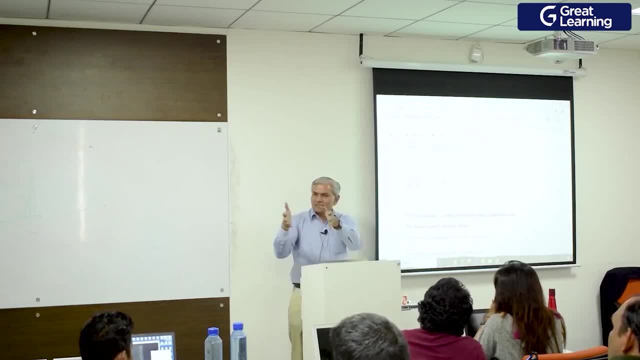 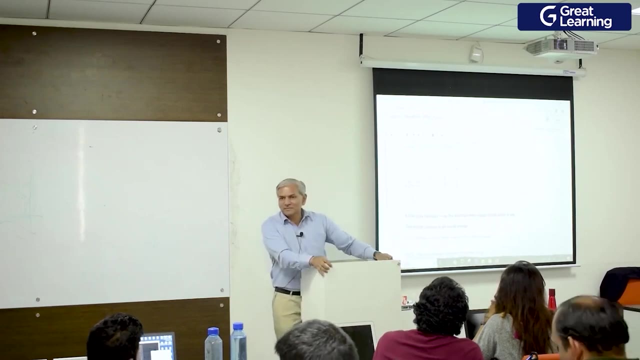 But to be able to do those things, find the 95% confidence level for your estimates, we use a technique called bootstrap sampling- In statistics it is known as sampling with replacements, ok. And we also use a technique called k-fold cross validations. 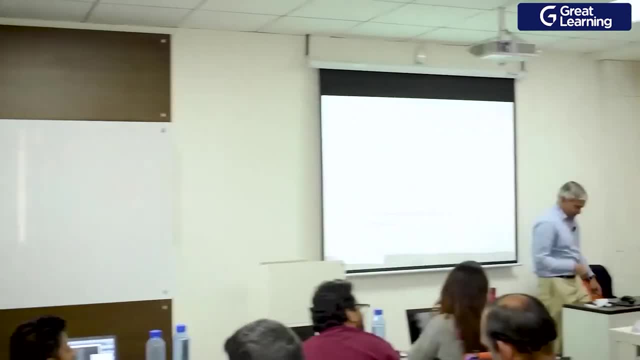 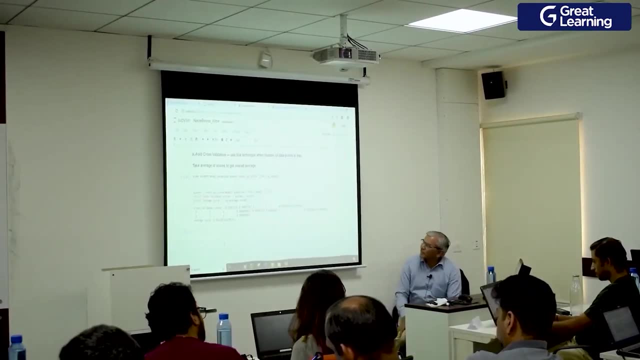 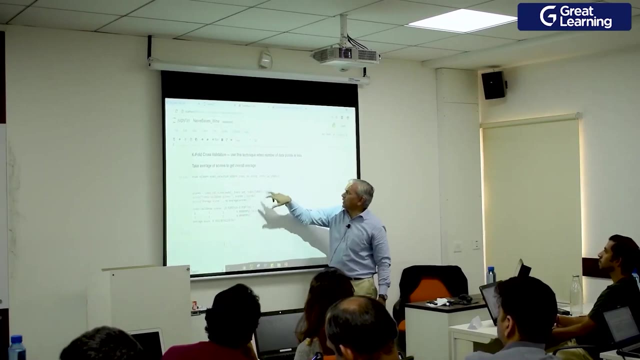 So I am showing you this k-fold cross validation what it means, But we will do this in detail down the line. Look at this From scikit-learn: import cross validation score and cross validation predict. These two functions are available already. 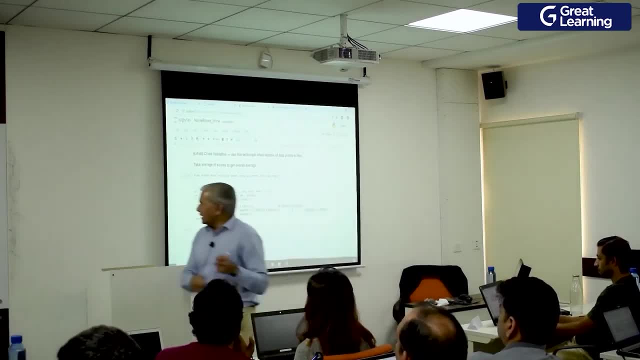 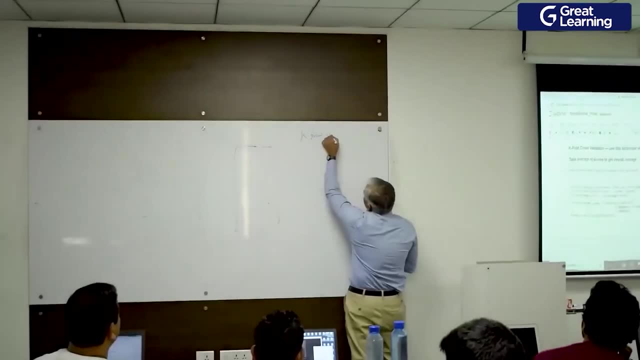 Let me explain to you first what is cross validation. I have this data set with me. Ok, Suppose, k-fold CV, Ok, Ok, I have this data set with me. That which I am going to use, k stands for an integer number, just like k. nearest neighbors. 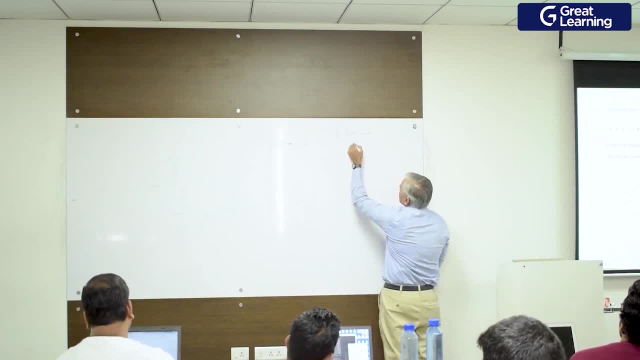 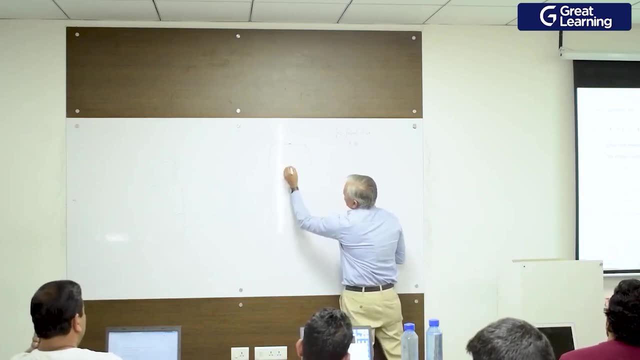 an integer number- Suppose I see k is equal to 10, usually we take 10 as a reliable. What it is going to do is it is going to break your data into 10 pieces: 1,2,3,4,5,6,7,8,9. 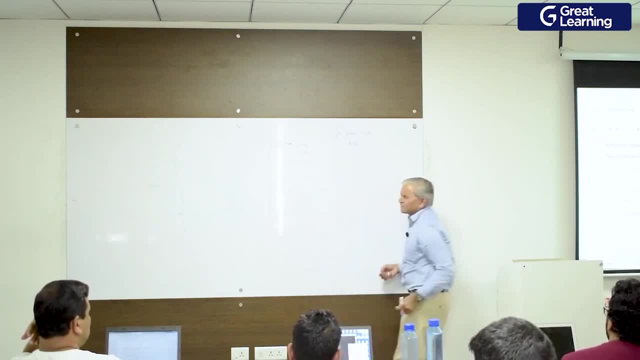 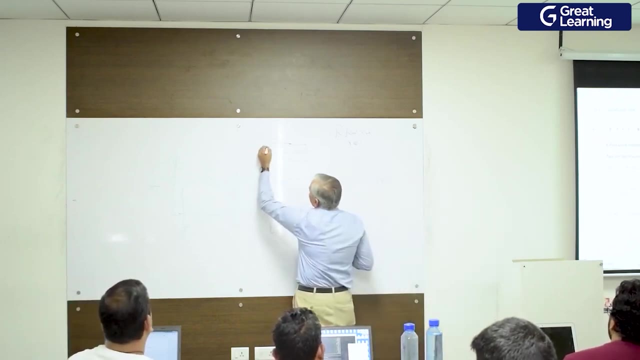 and 10.. It is going to break your data into 10 equal pieces. Then what it is going to do is For i, equal to 1 to 10, where i is an index, i equal to 1,2,3,4,10.. 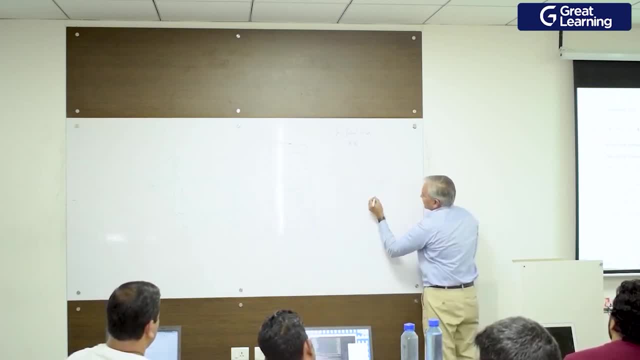 For i is equal to 1 to 10, fit using 9,. test or predict using the left out: left out. So first time when i is 1,, 2,3,4,5,6,7,8,9.. 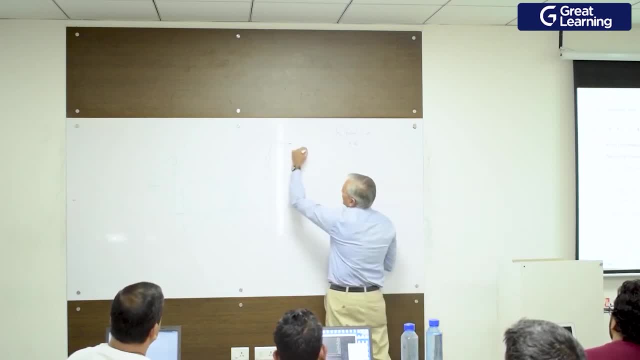 Ok, When i is 1, it will take some 9 data sets, do the fit and it will test on the left out. Then, when i becomes 2, it takes some other 9, may be this 9,- do the fit and do the left. 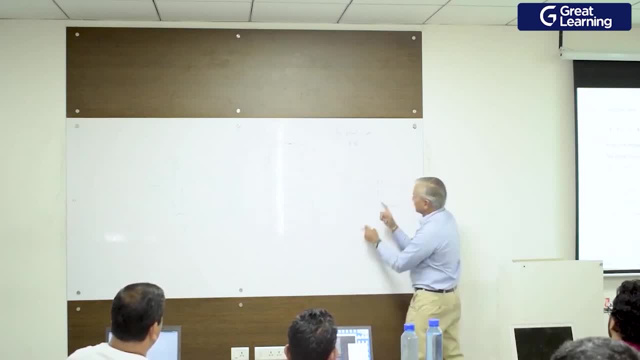 out. Then it will take some other 9, do the fit left out. It will do this 10 times because you have taken 10.. k is equal to 10.. Ok, Ok, Because you have taken. k is equal to 10,. it is going to break your data into 10 pieces. 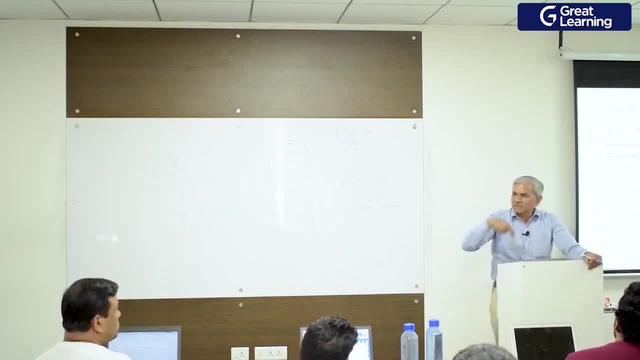 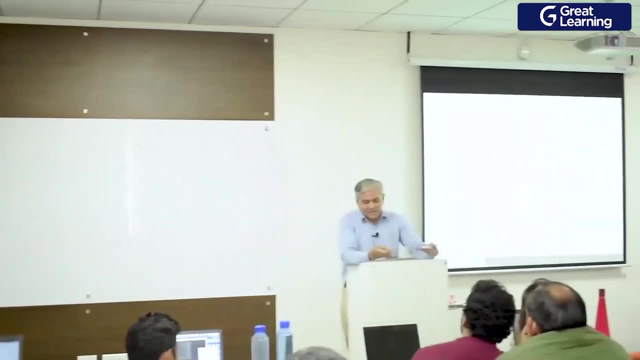 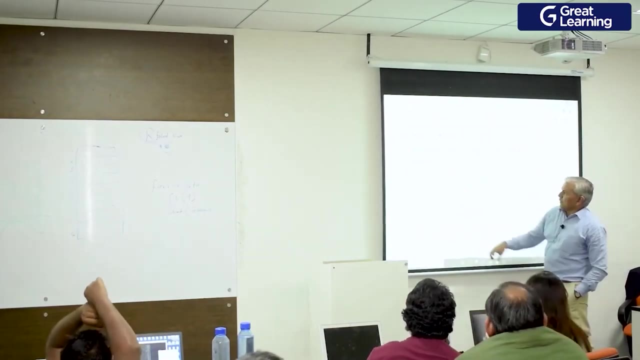 Train on 9, test on 1. and it will do this 10 times. Train on different 9s each time. test on a different. left out each time When you do this on this particular data set. so i have imported these two cross one. 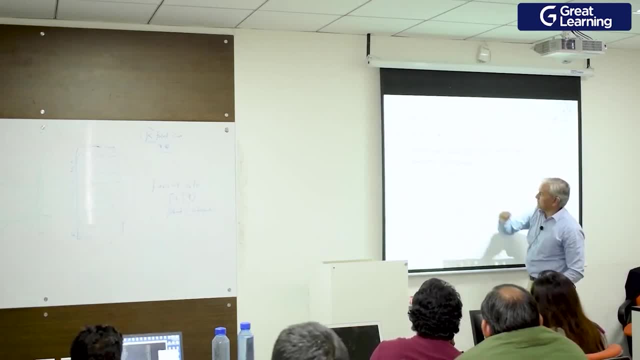 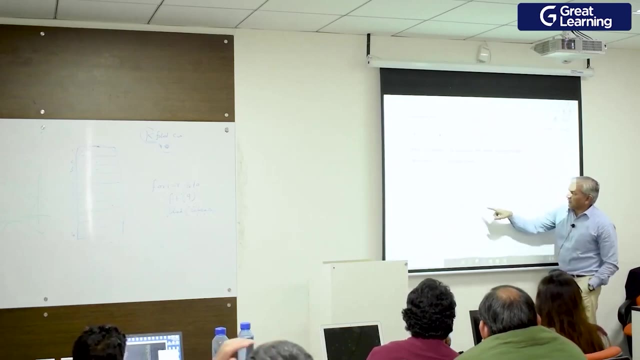 score. i have supplied the model to it, the model which i have built up, the training set, test label And CV is 10.. When i do this, look at the scores i am getting. First run, it gave me overall score of 92.8,. second run gave me 92.8,. third run it gave. 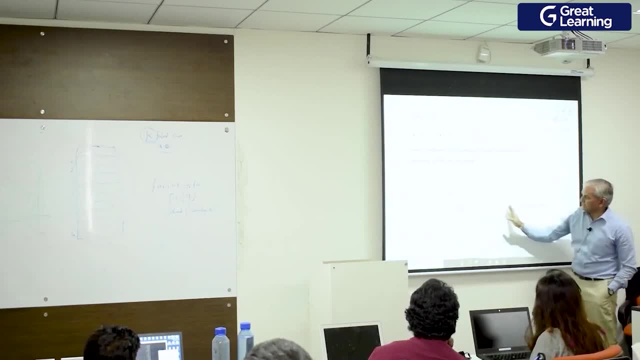 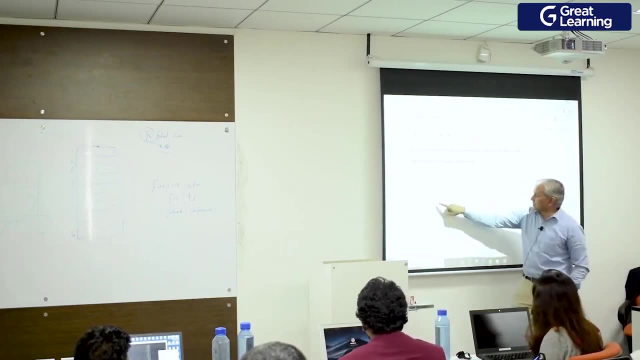 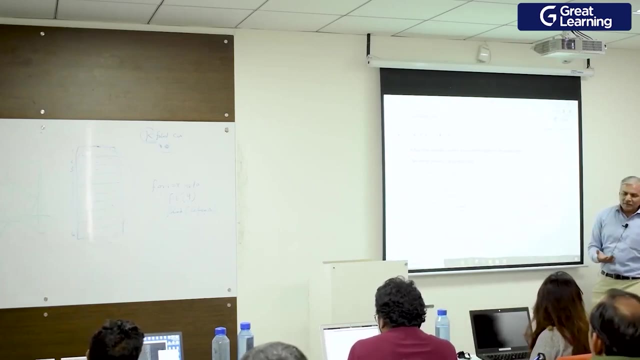 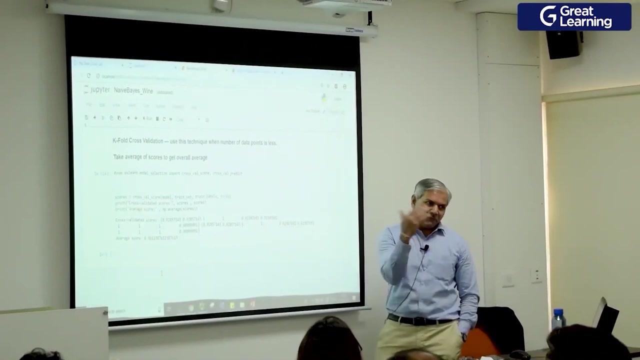 me 1,, 1,, 92.3, this is all the scores you have got. Average of all these scores: average of all these scores is 96.12.. So you can expect your model In production, on average, to give you 96% accuracy. however, we want to give a range. 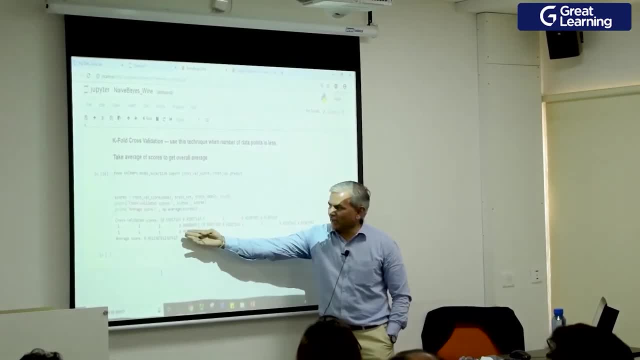 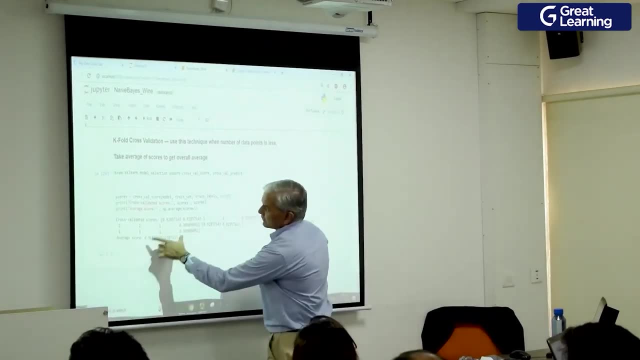 To get the range you can find out this distribution, 95% confidence level of this distribution- or resort to bootstrap sampling. We will talk about that later in detail, right, So we make use of this technique to find out overall how the performance is going to be. 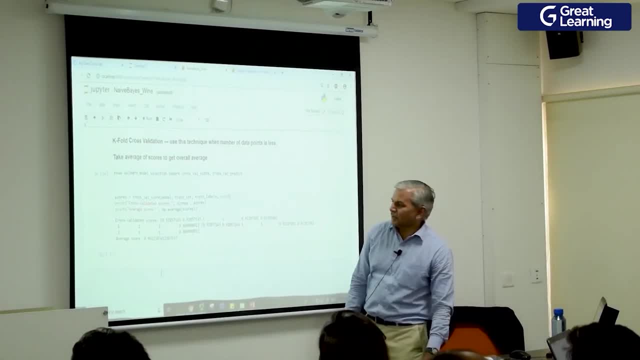 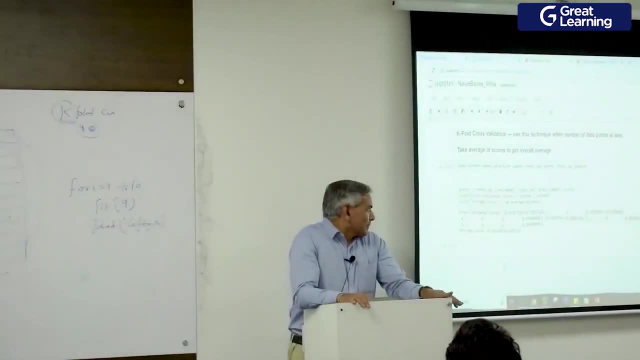 in production: 96% average accuracy score. I can expect from this model On this data set: No, no, I will tell you why. why we did that. No, we did subsequently testing. also, we did Look at the line. 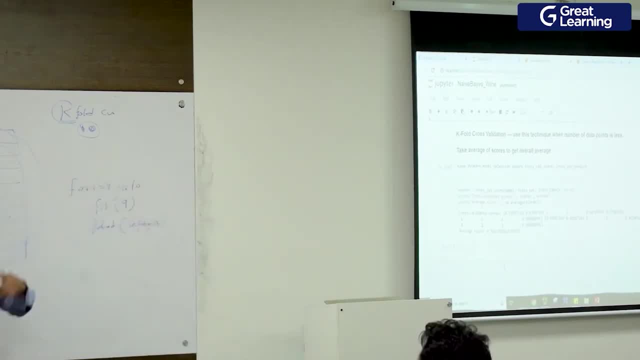 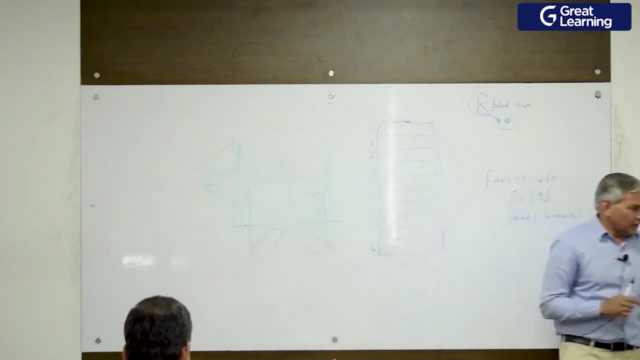 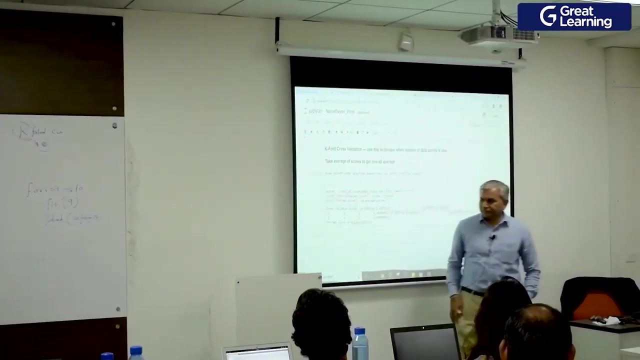 We have done on testing. on testing also: Okay, why did I do the evaluation? on training and testing, let me tell you this: okay, with that we will wind up. This is very important point and you should learn this trick now itself, and if you reflect all these things in your projects, it will be good, Oh. 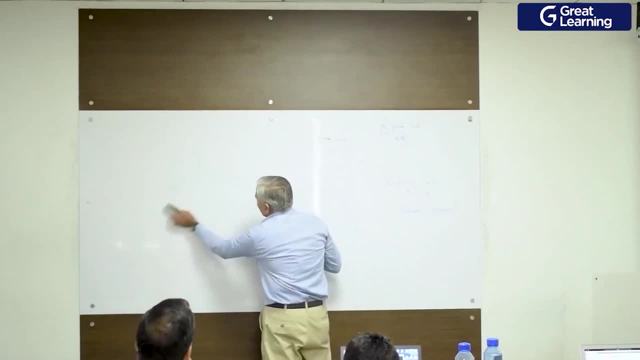 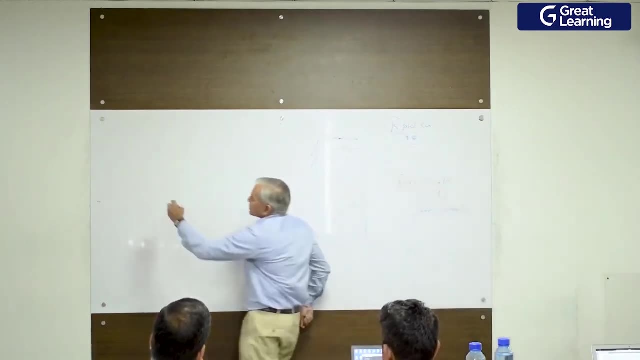 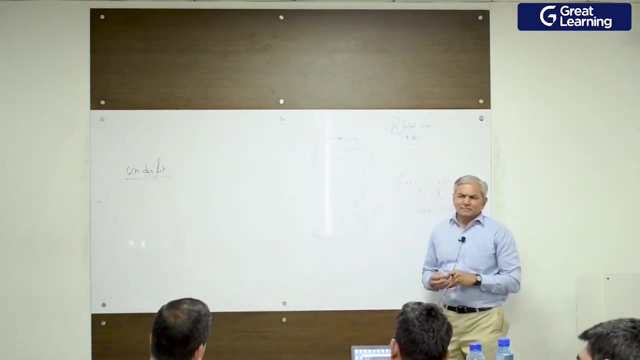 there, it is okay. Remember we talked about over fit, under fit. okay, what is under fit? How do you define under fit? Sorry, Loosely coupled with less dimension. Straight line, Straight line, curve line- what the Straight line? Straight line, curve line- what the? 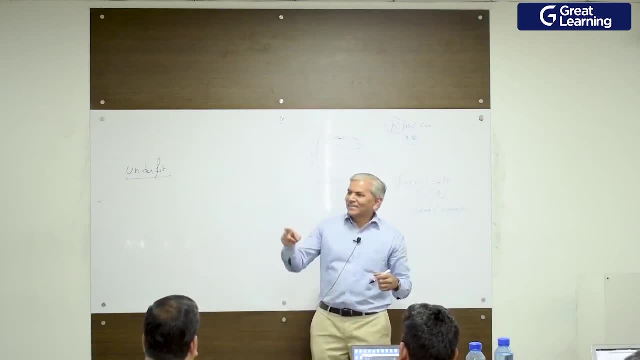 What is going on Using what I want to reach? the sweet spot on the left side is low. this thing under fit on the right side is over fit. but how will it know whether a model is under fit or over fit? Ok, ok, ok, ok, guys, let us, let us, let us. very good. thank you, enough, enough, enough enough. 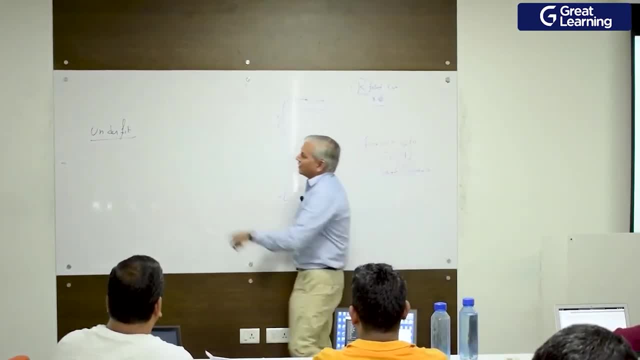 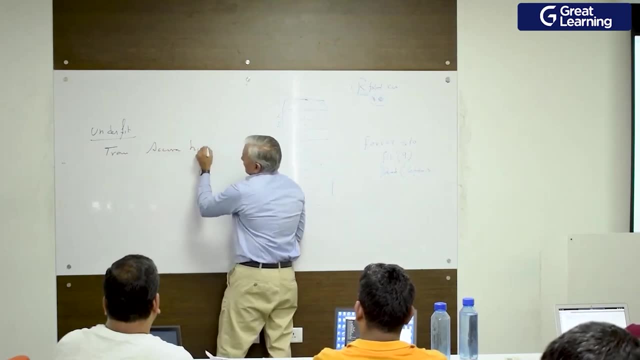 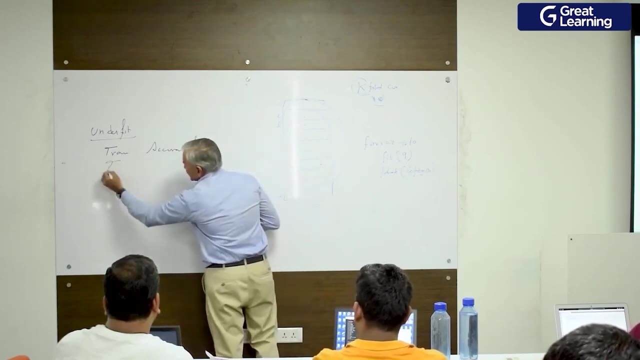 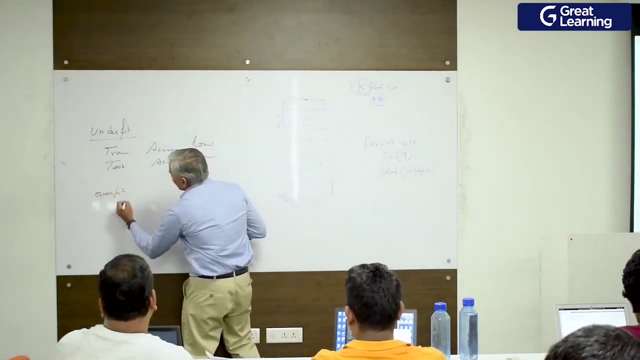 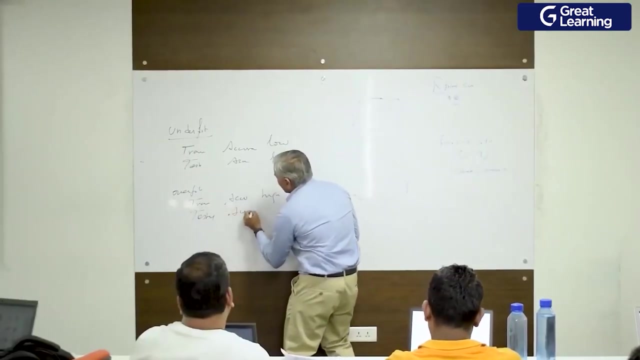 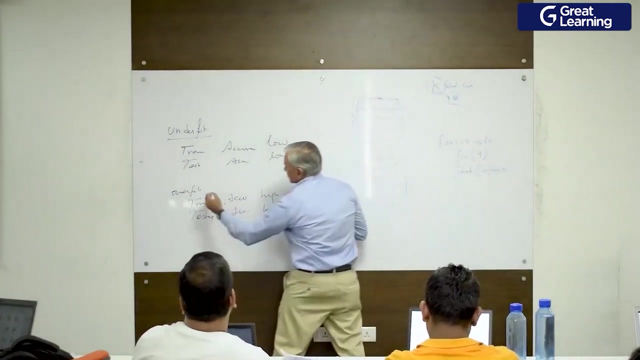 under fit. is that case where in training set accuracy is very high- ok, I am sorry, accuracy is very low, low and in test set also, accuracy is very low, over fit. is that case where in training accuracy is very high and testing Accuracy is very low? alright, right fit. this is over fit, right fit. is that case where 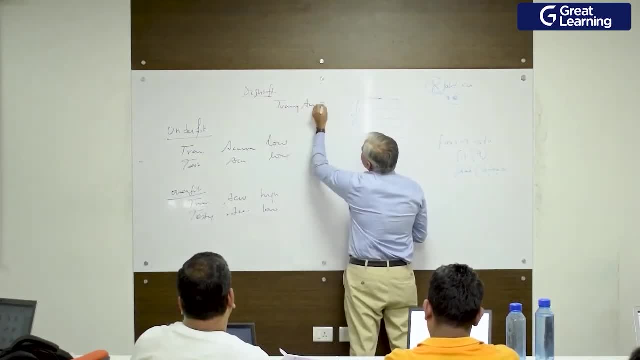 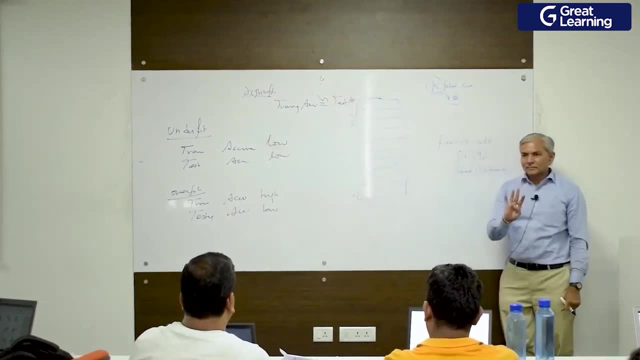 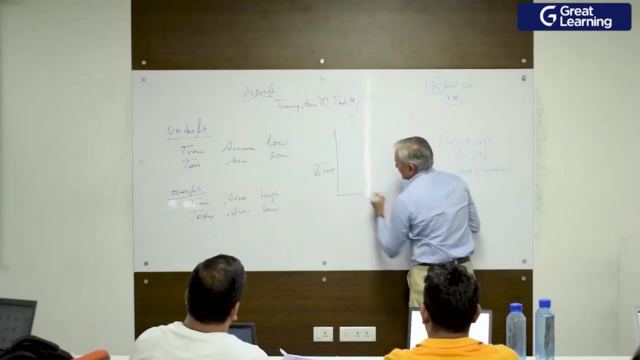 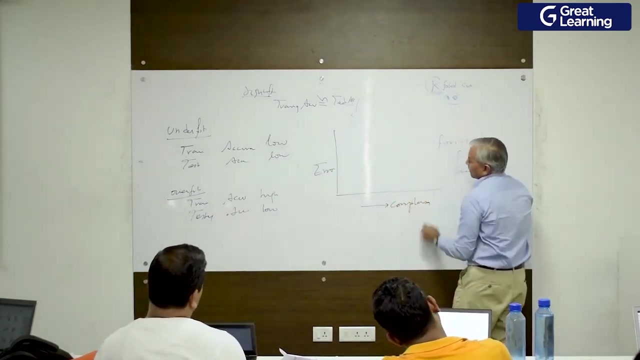 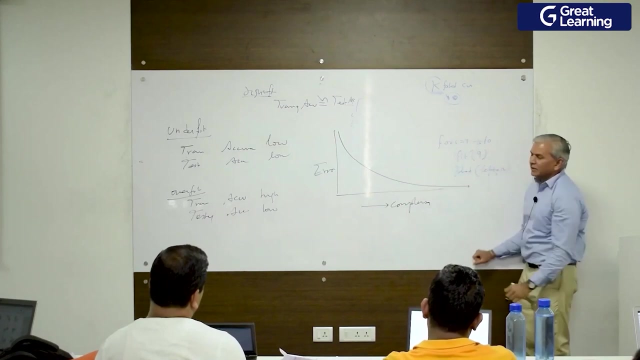 training error. training accuracy is equal to more or less equal to test accuracy. alright, so if I plot a graph of Ok, Errors, ok- and this I is my complexity, complexity- then you will see that my training error comes to 0, especially decision tree will give you training error 0, but this is my training. 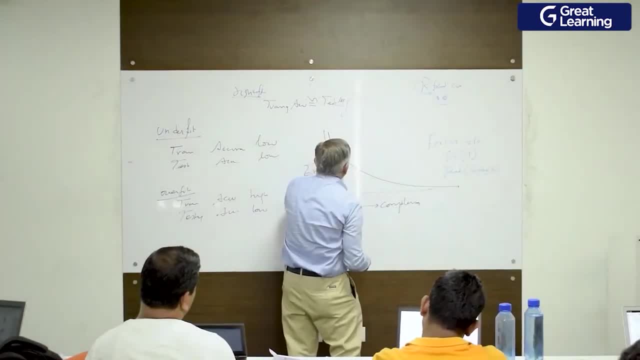 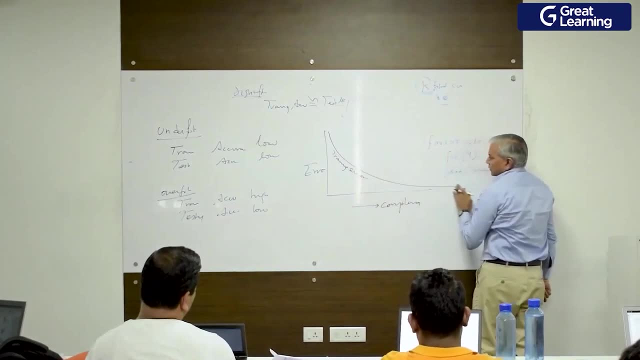 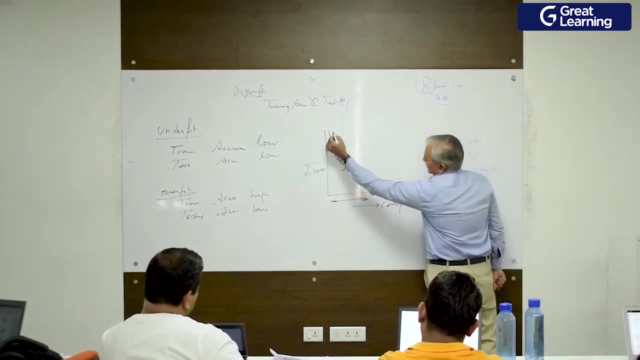 error. I call it training error, t r a i n i n g error. As my complexity increases, training error comes to 0, but you will see that this is my complexity. ok, I am increasing complexity in this direction. you will see that the test 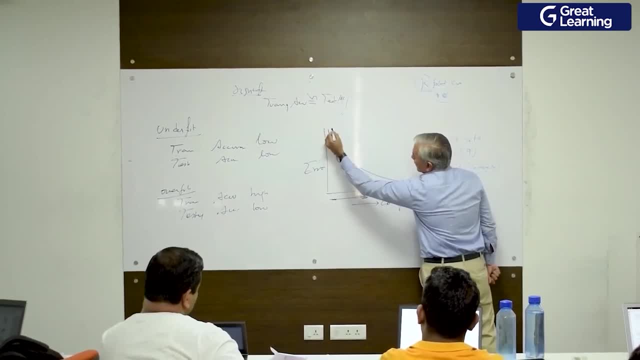 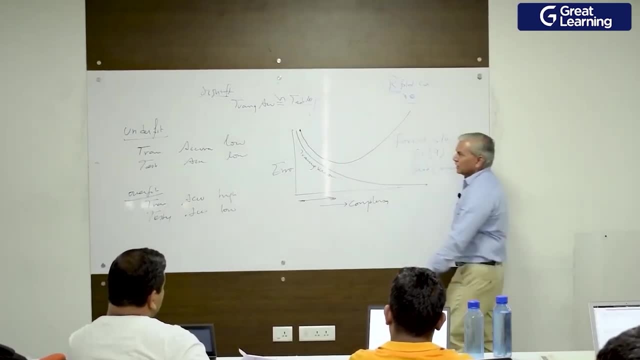 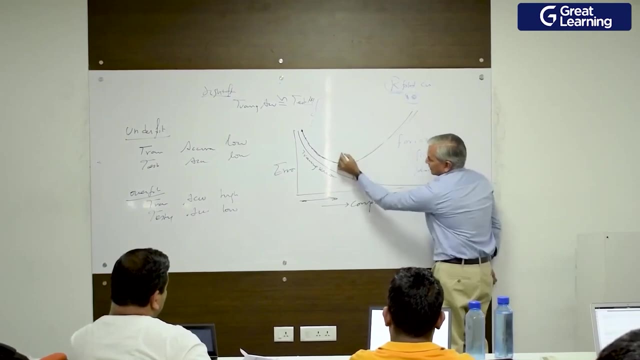 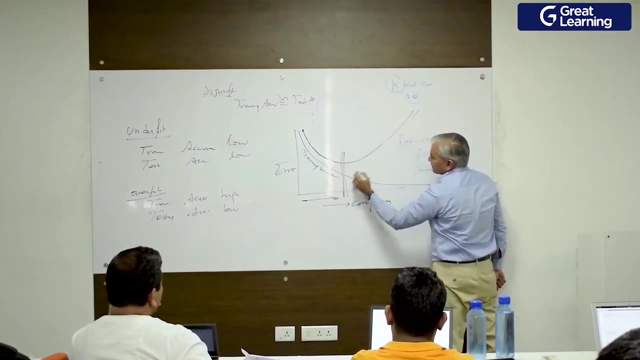 error is usually higher than the training error. it also comes down, but after some time it deviates back up. you will notice that the test error also comes down to some point. after that it backs up, it peaks up. Ok, This difference, ok, this difference where the training error starts deviating back up. 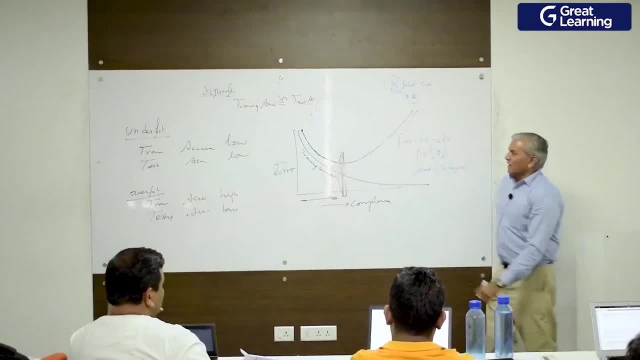 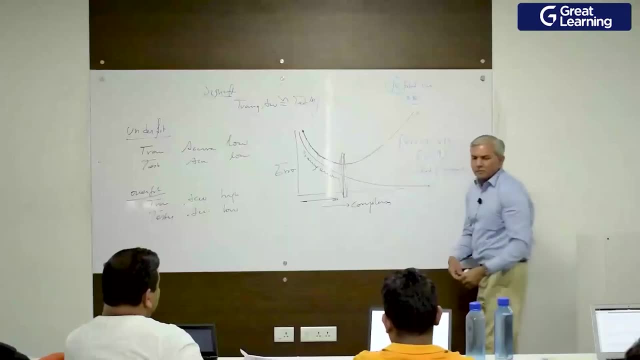 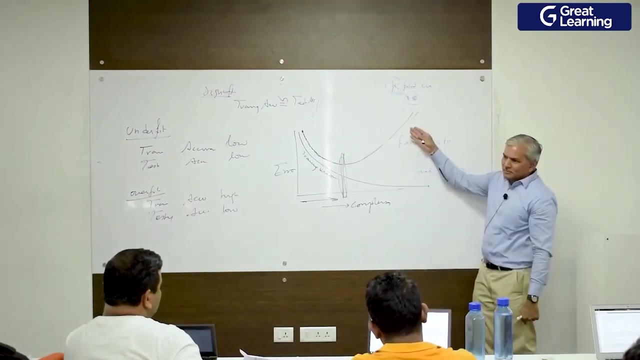 you should stop here. below this it is under fit. above this is over fit. In this situation your model is absorbed, all the noise in the training set and become very complex and when you take that model on the test data, on test data, it bumps. error is. 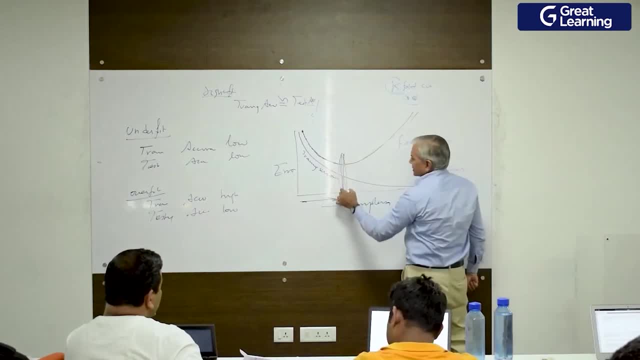 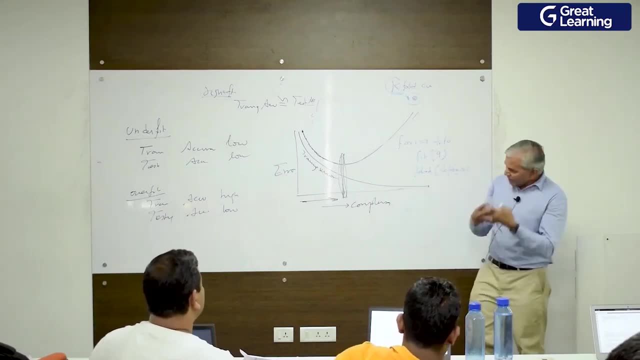 very high on test data. ok, So this point is what you want to check. so whenever you build model, run the model both on training set and test set. If on training set and test set, training is 80 percent accuracy, test set is 60 percent. 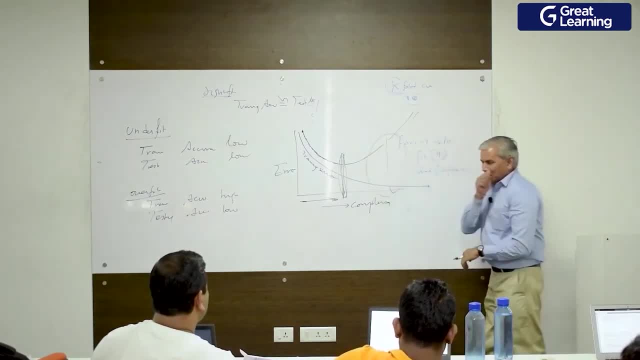 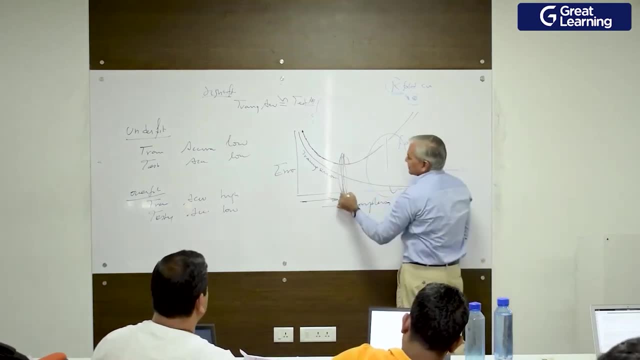 accuracy. you are in this region. If training set and test set- both of them- are similar to each other, with very few difference here and there, then you are probably in this region. training is also poor. testing is also poor. you are in this region. 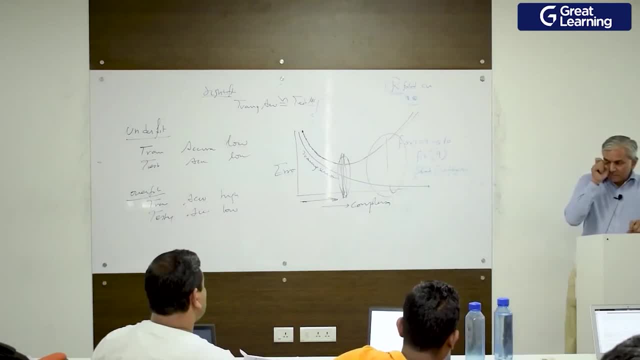 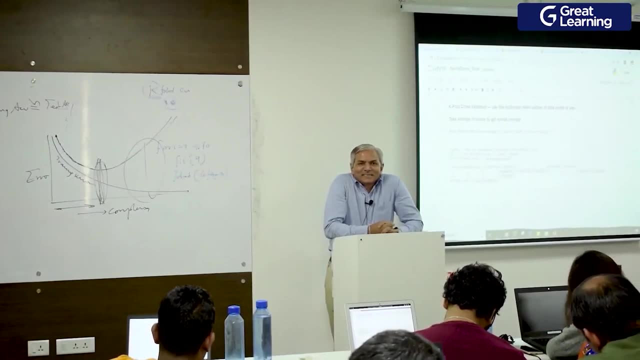 Ok, This is under fit region. so much to discuss. I know it becomes a bit of a overwhelming with so much of information coming in such a short span of time. you will take time. do not worry about it. take time, take your. 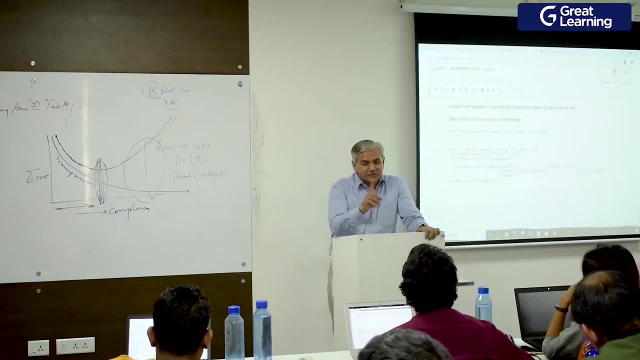 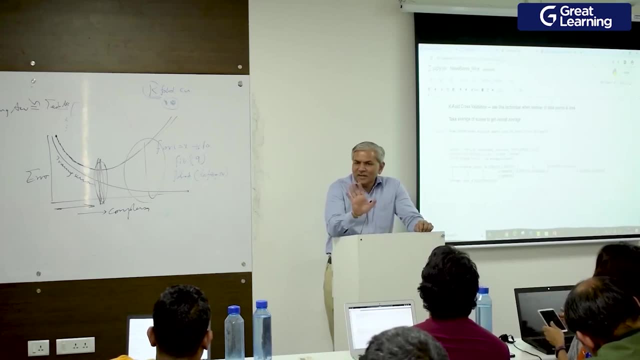 own time to sync all this in and keep practicing on the UCI data sets, but do not get miscarried by the UCI data sets. as Biryant pointed out, in the reality you will never get such data sets readily available, never. 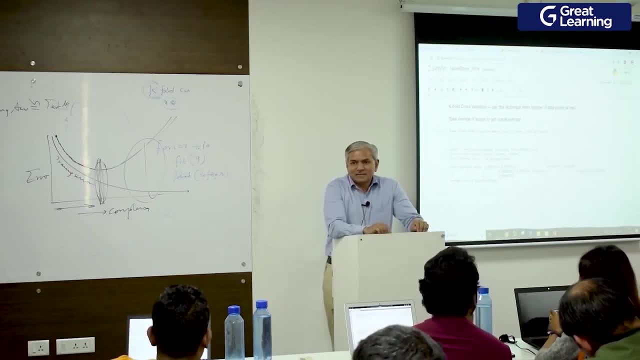 If you get, you have to suspect it. ok, That reality will hit you when you do the capstone project itself. the idea is to teach you that reality. alright, So I am going to stop here. I am done for the day. any questions, feel free to shoot. 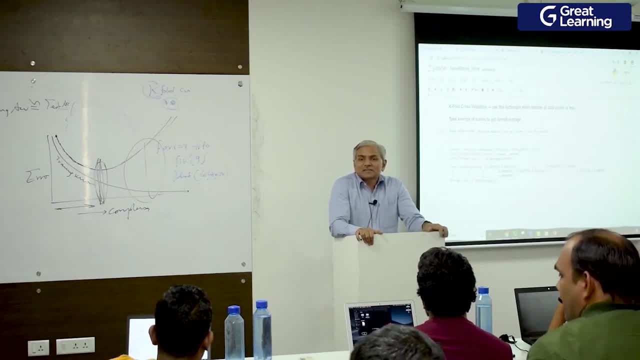 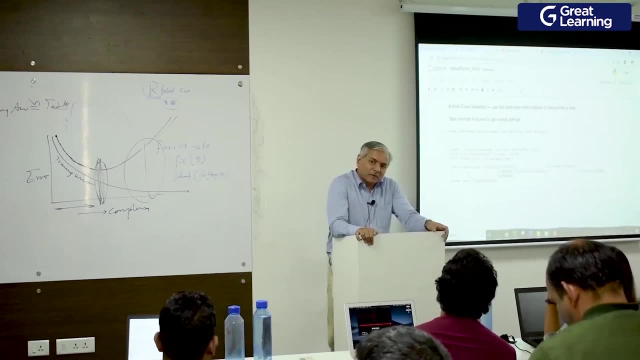 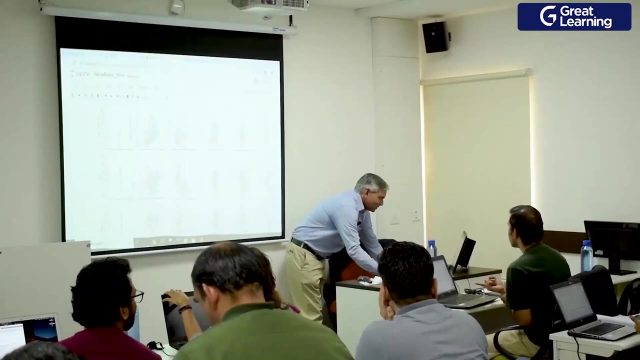 we are stopping a bit early today. But yeah, Can you explain the back plot and what are the inferences of the back plot? Back plot: Yeah, sure, why not? we can do that For this data set. Ok, Actually, I have done this on the data set. 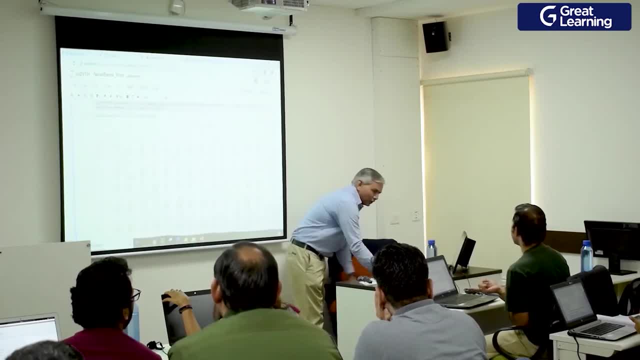 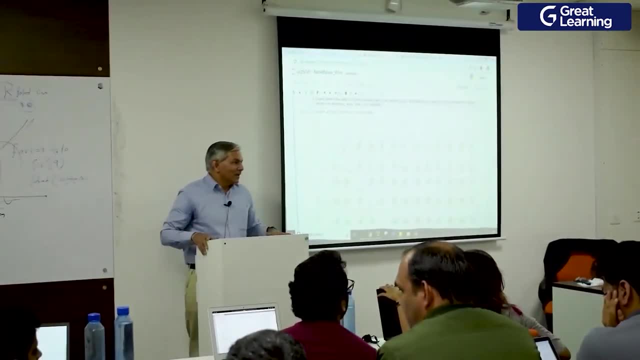 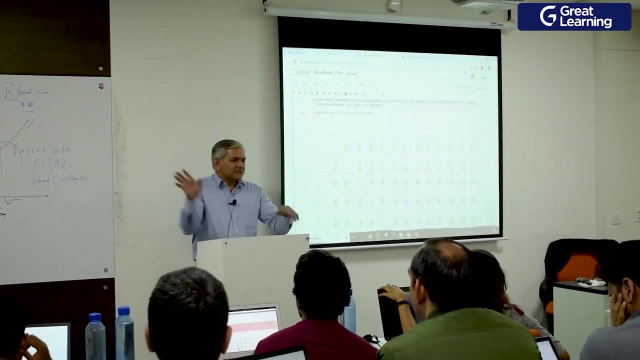 Scores have gone down right Overall. what is accuracy? 76. Overall accuracy, Overall accuracy. Yeah, that is what is accuracy. Total accuracy, Total accuracy, Total accuracy. Yes, 74, 76. that means it is an under fit region. both of them are very close to each other. 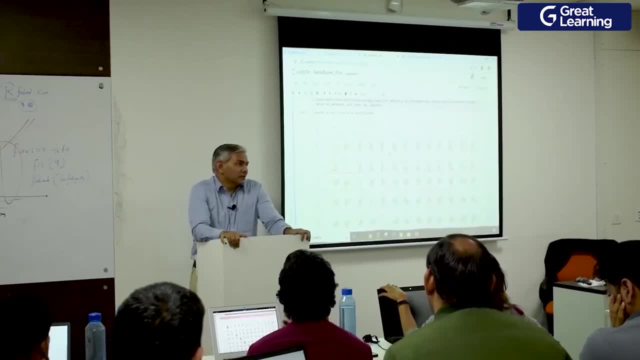 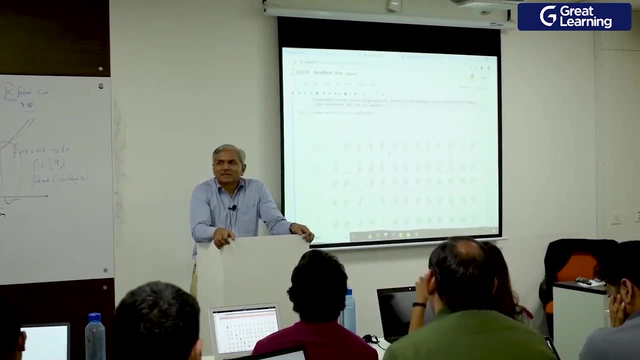 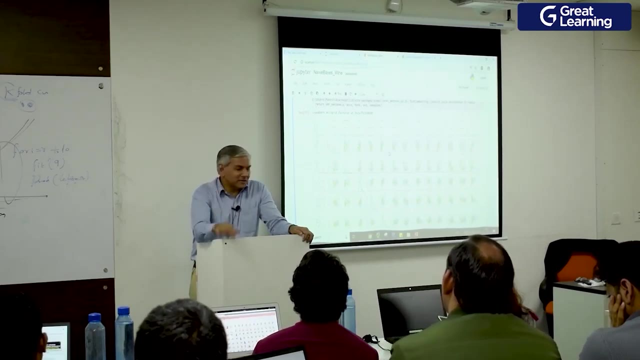 and class level accuracy: diabetes class recall. what is the recall? a diabetics class 88,, 62. for diabetics class is 62,, 55% and 62% is a big jump. actually it is a big jump. 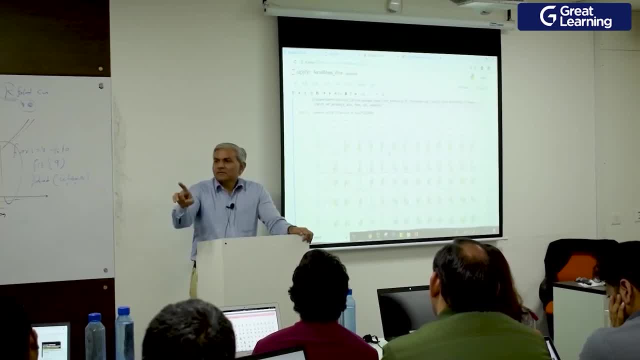 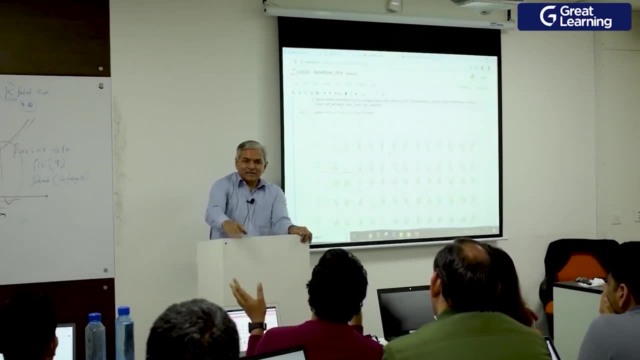 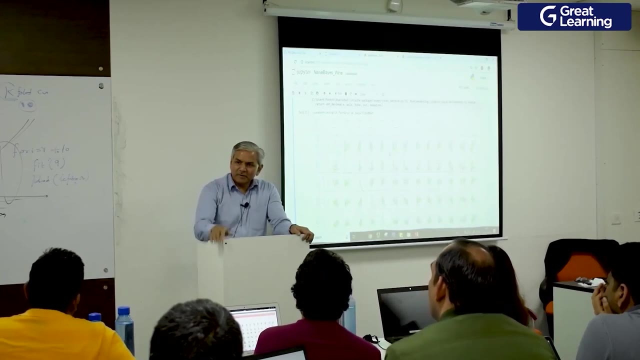 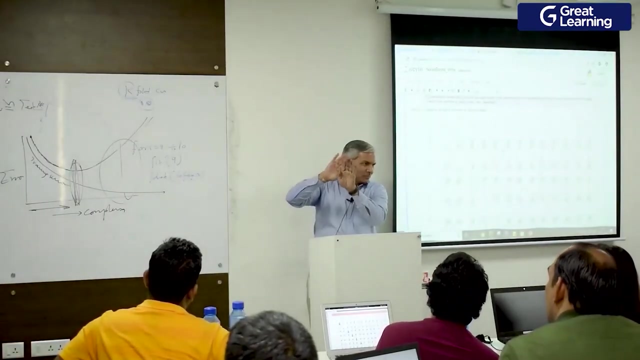 so for diabetics class this NiBase is doing well. because can you tell me why NiBase is doing well for the diabetics class In diabetics class in Pima diabetes data, as you notice that there are three attributes on which there is a very small separation between orange and the blue on the three dimensions. 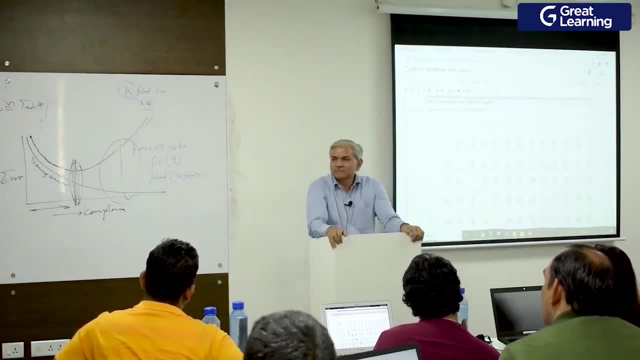 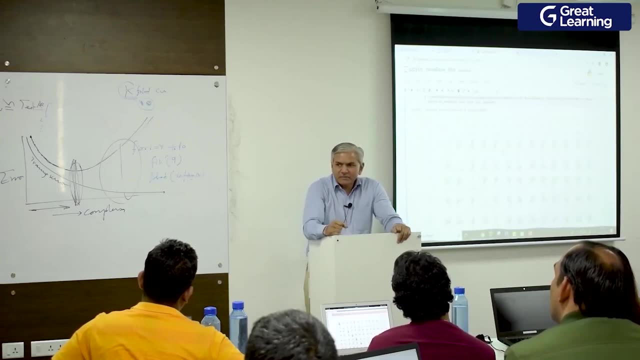 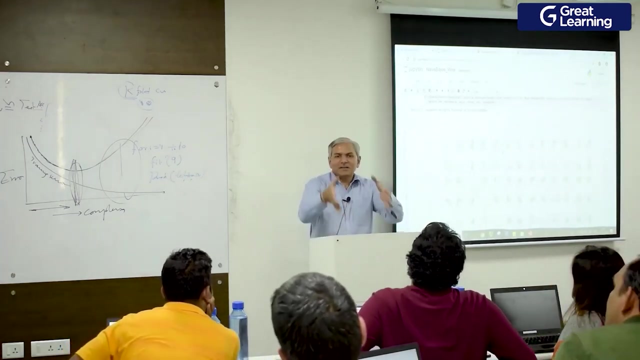 Those weak predictors are helping the NiBase approach. So the lesson that we have from this is- which we will revisit tomorrow anyway, given data set and given problem statement, we never rely on one single algorithm. we always build multiple models. each model might be different algorithm, and then we average out that concept. 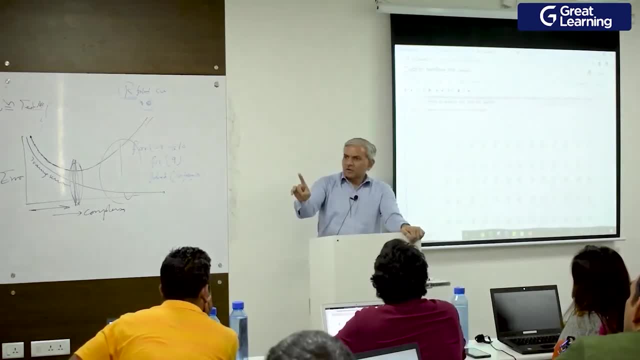 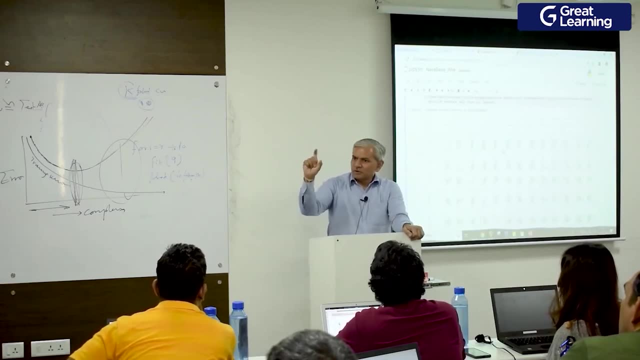 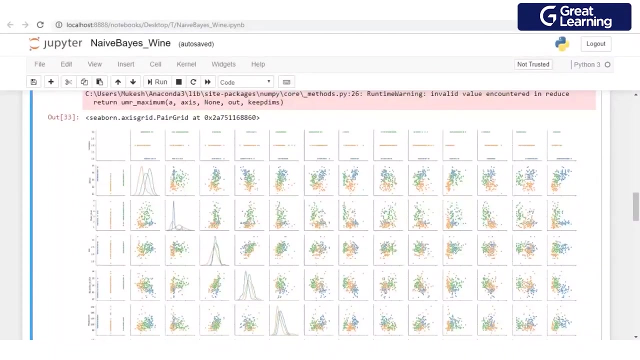 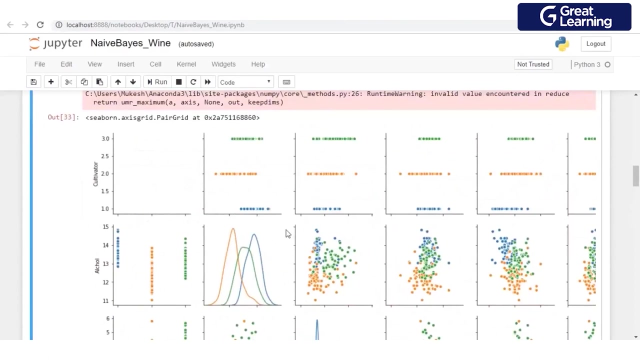 is called stacking If you use the same algorithm, multiple instances that we call ensemble. So in production we always put an ensemble or a stack, and the ensemble or a stack will give you much more reliable result than individual instances will. Let us move on. so let us see this pair plot. there you go always. first look at the diagonals. 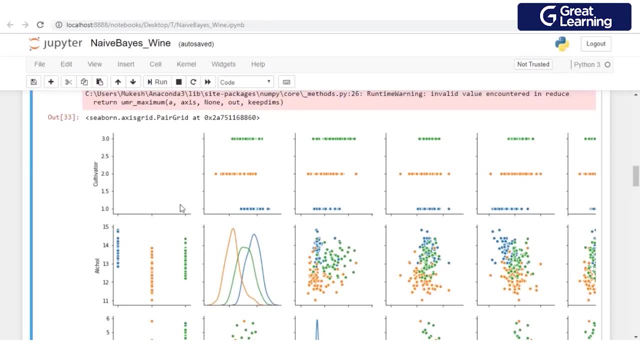 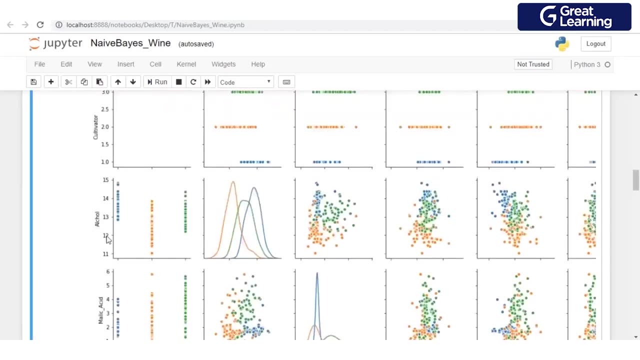 in the diagonals. the first column is the category, the target column. So you, we can ignore this. this is category of the three cultivators, people who cultivate. The next column is the alcohol. look at the diagonals. this is alcohol versus alcohol. 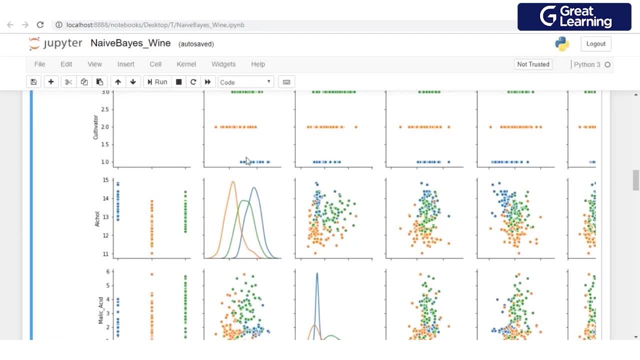 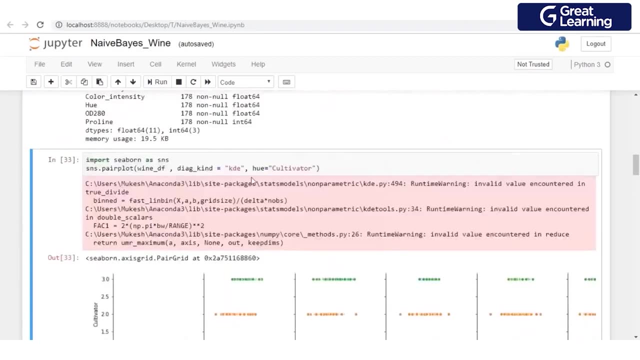 So it makes no sense to give you scatter plot here. So instead they have given you density distribution on the alcohol dimension, Since we have used this hue color, which means give me separate colors for separate classes. it showing you the three classes. 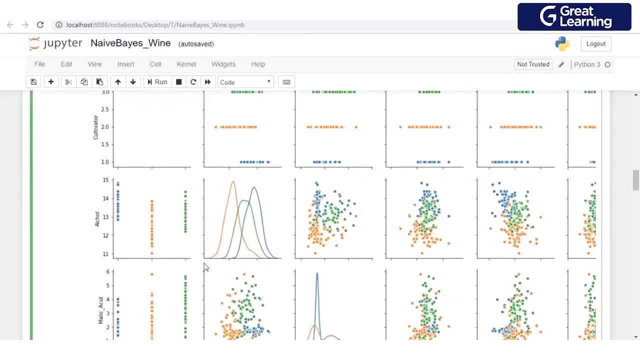 And what is coming out of this is between classes there is overlap, but fortunately the central values of these classes they are not overlapping. No, this alcohol versus alcohol. this is just distribution of the classes on alcohol univariate. This analysis is univariate analysis. it is not comparing the dimensions. 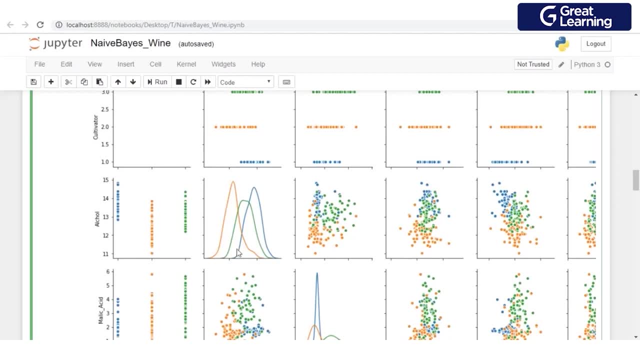 So it is giving you distribution of cultivators from class 1, class 2, class 3 on this dimension, How the values of alcohol for class 1 is distributed, how it is for class 2, how it is for class. 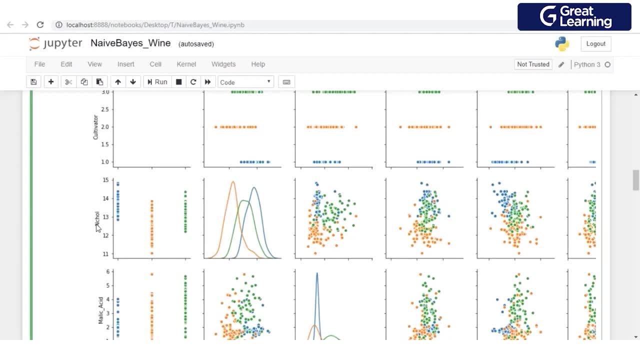 3.. So what this is telling us is the alcohol dimension can be used to separate out the three classes. Go to the next one. if you observe carefully, malic acid- what it is saying is the class of alcohol can be used to separate out the three classes. 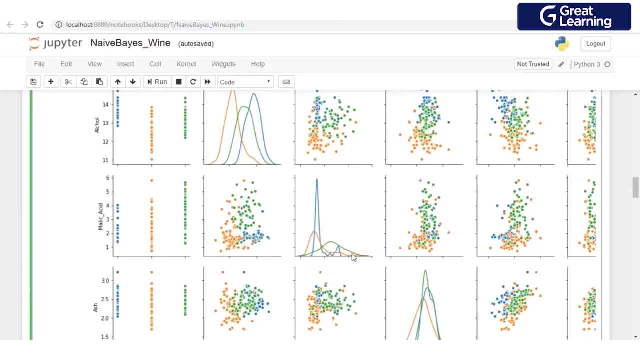 Go to the next one. if you observe carefully, malic acid- what it is saying is: the class 1 is distributed like this. the class 1 malic acids are distributed like this. class 2 malic acids are distributed like this: and class 3 is the green one. 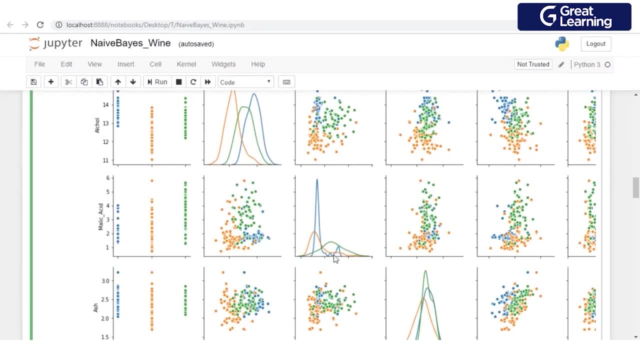 What we are seeing is outliers here For the blue class. on this particular dimension, there seem to be outliers. You see the small bulge over here. similarly for orange. similarly for orange also, we are seeing bulge. The problem we are seeing for the green one, there seems to be huge range on both sides. 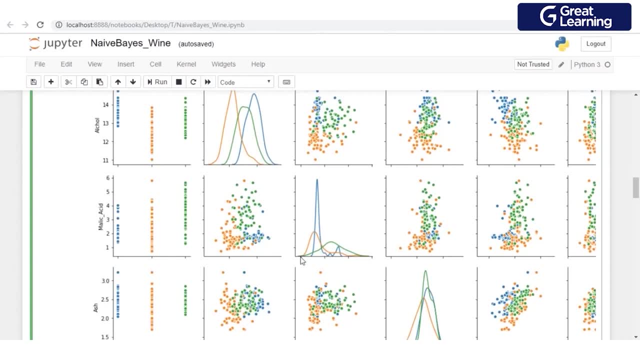 So green one also seems to be having some extreme values on both sides. that is why the distribution itself is stretched out. So I have to go back to the records and see on this malic acid for each class. what is the problem, what are these outliers and we need to deal with it. 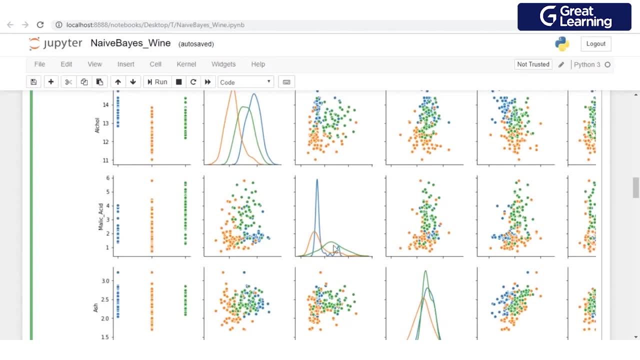 But right now, in the raw form, In the raw form, the green stands out separately from the orange and the blue, But the orange and the blue class are overlapping. So this dimension may be very useful in separating out greens, but may not be very good in separating. 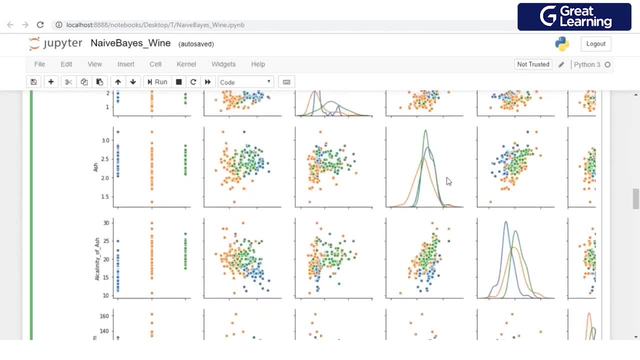 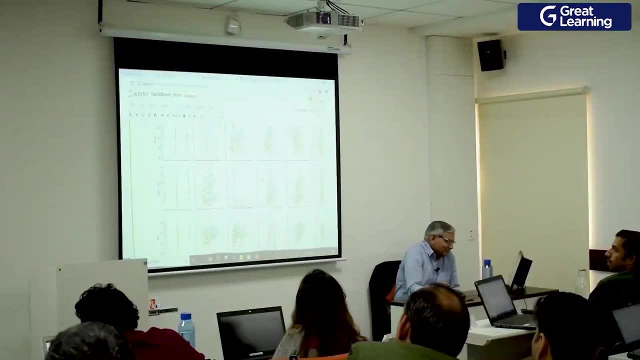 out orange and blues. This dimension is your ash. it is relatively the most useless dimension in this set. Malic acid: it still has the outliers. suppose if you take the outliers it will still have the outliers? It will still have the outliers. 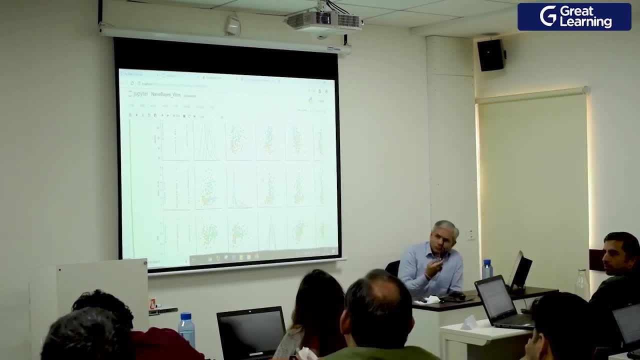 It will still have the outliers, So you have very less predictability. So you mean that it is a very good predictor for the blues to this data? No, The predictive power base is. the predictive power is a function of how cleanly these separate. 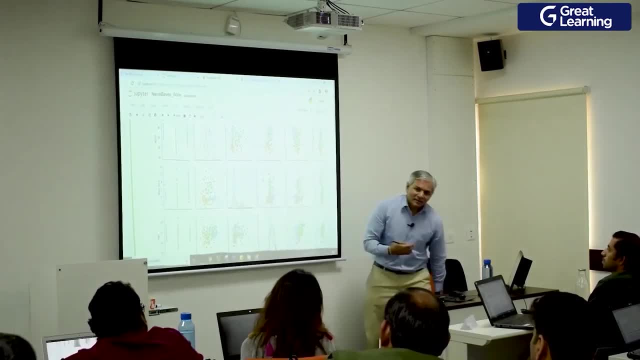 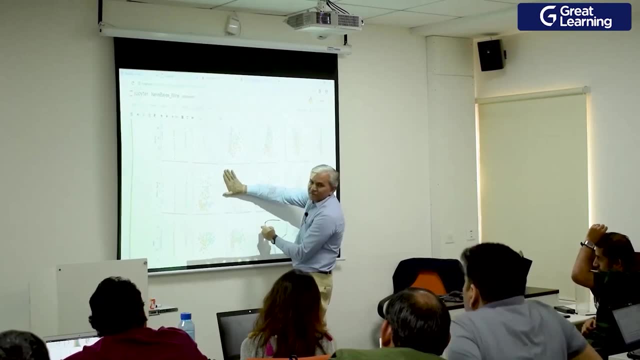 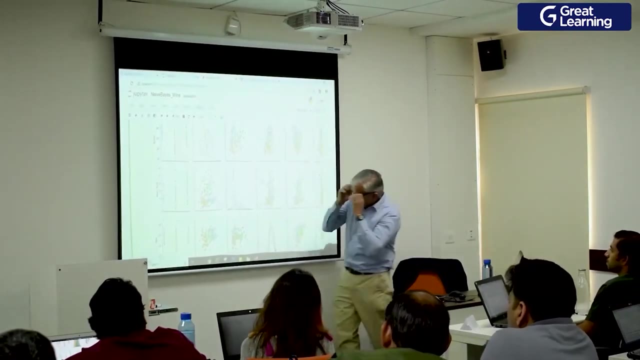 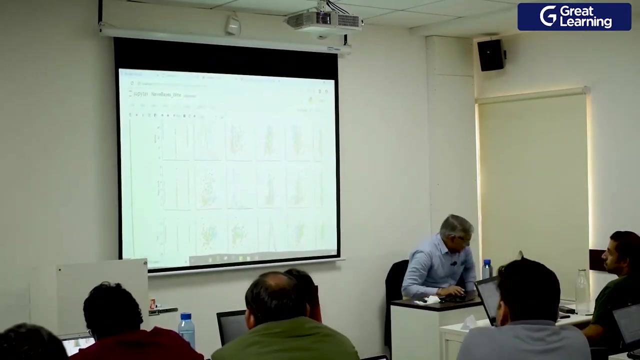 out the distributions. The predictive power of a dimension is a function of how cleanly these distributions are separate out. Suppose there was no blue class, this is a very good dimension to separate orange from the green. If suppose there was no green class, this is a weak predictor for orange and blue. 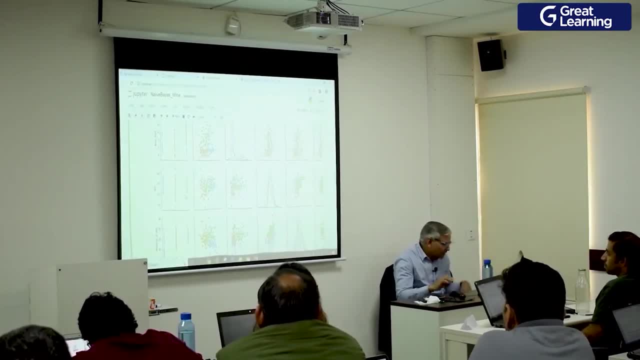 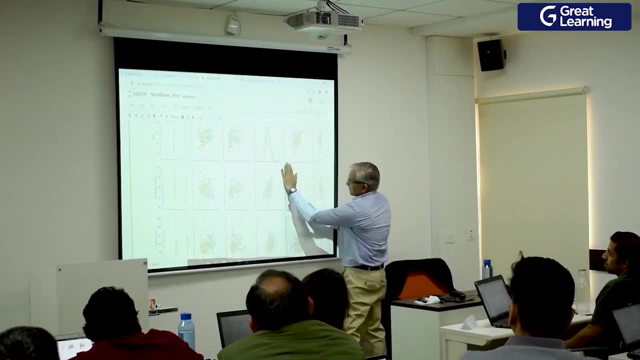 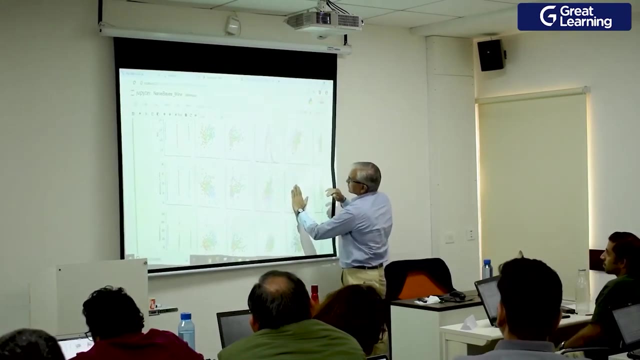 This ash. it is a very weak predictor for all three of them. This alkalinity, if you see, if you look at, if suppose the blue class was not there, then we are in Pima diabetes case. But at least it is a good separator for green and blue. 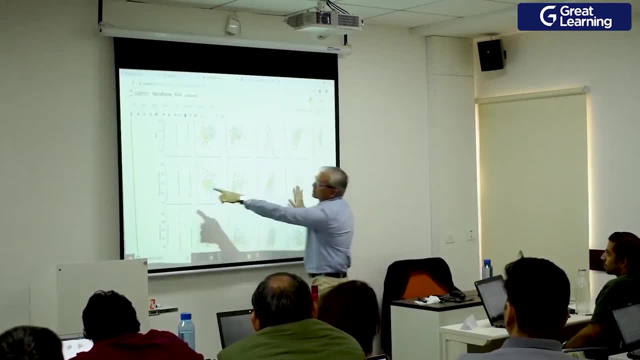 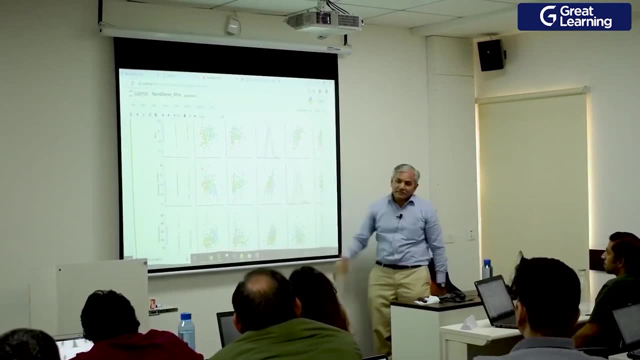 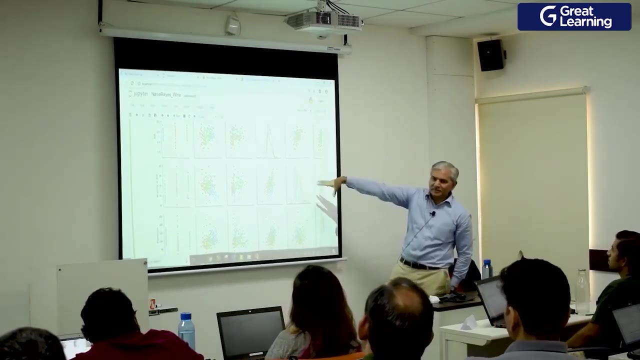 Right. So individual dimensions may be weak predictors, but when I put them together, they might be able to segregate the three classes properly, And that is what is happening in the dataset. You asked the question right: How to interpret this. 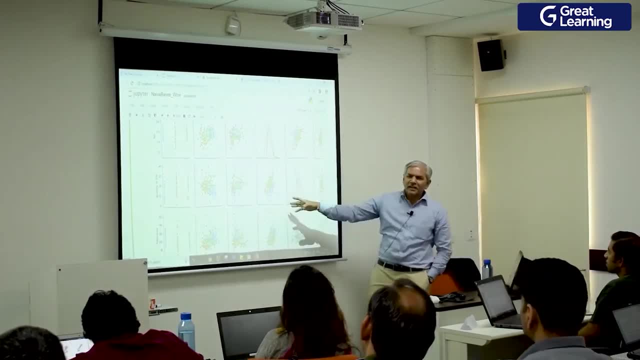 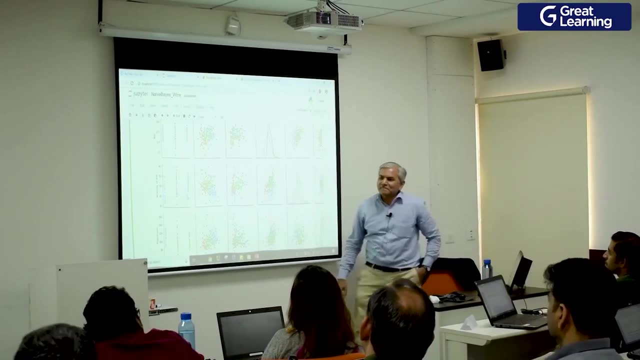 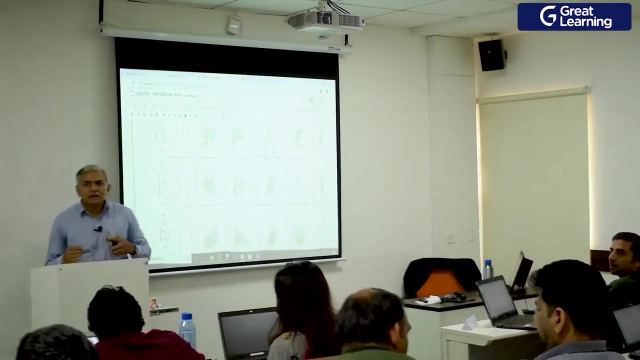 That is what we are doing. The scatter plot makes no sense because we are not building any linear models here. Ok, So scatter plot- I am not referring So diagonals- is important for us. Any other question Based on this. we can drop the variables which are less important, right? 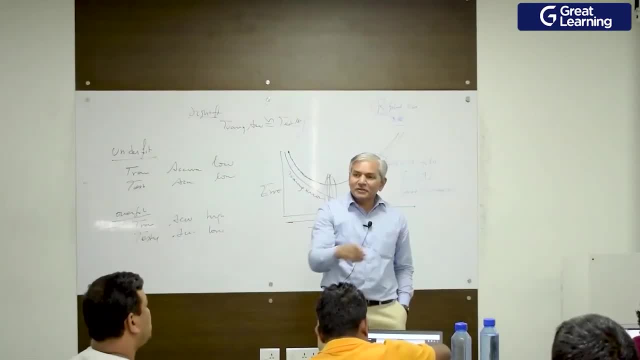 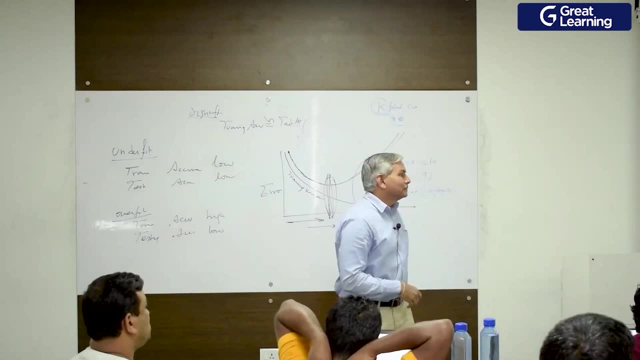 100 percent. So, but Maybe by dropping that ash dimension and reducing the curse of dimensionality, I might be able to get more than 96 percent. Ok, So if you drop the ash, and again, what is the? what is the? 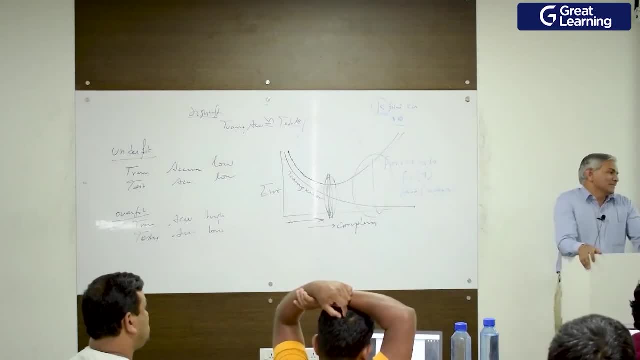 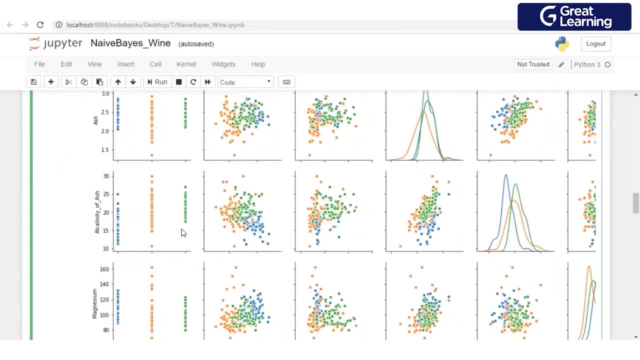 I do not know, I do not. I have never done that, but you should try. Maybe you will get Handling. the outliers might help you in classifying, Because outliers, Hey guys, all of you this side, please, All of you this side. 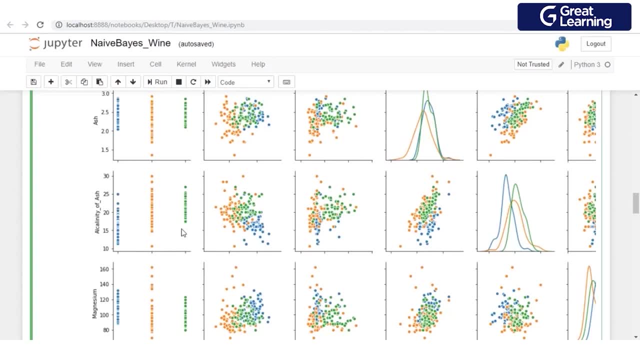 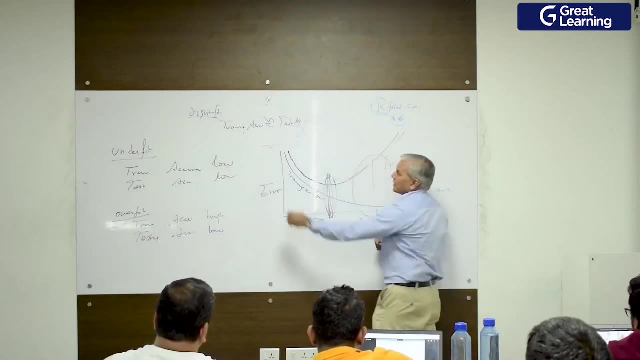 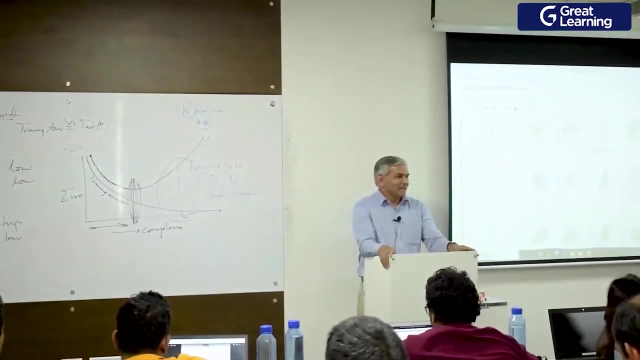 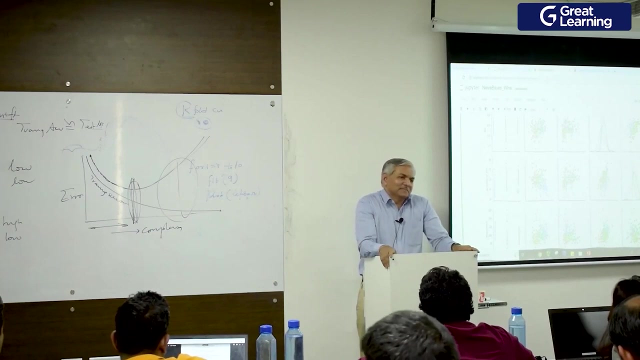 This is a Gaussian Naive Bayes. Gaussian Naive Bayes expects your data to be distributed like this, But wherever your data is distributed like this, if you handle these outliers, you might get better results Right. So if you handle the outliers, both logistic and Naive Bayes will give you better results. Because outliers increase log loss in your logistic. So if you handle outliers, both logistic and Naive Bayes will give you good results. Treat: it means You are talking about outliers. Ok, Do not remove the outliers. Do not remove the outliers. 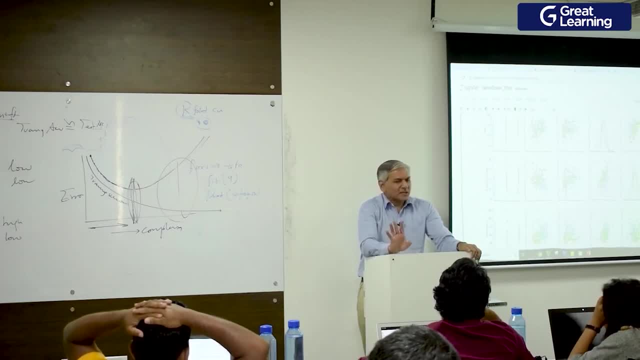 Ok, Do not remove the outliers. Do not remove the outliers. Do not drop the records as much as possible. Unless you are lucky guy, you are given terabytes of data Right, So usually you will find yourself in a situation where we do not have the luxury of dropping. 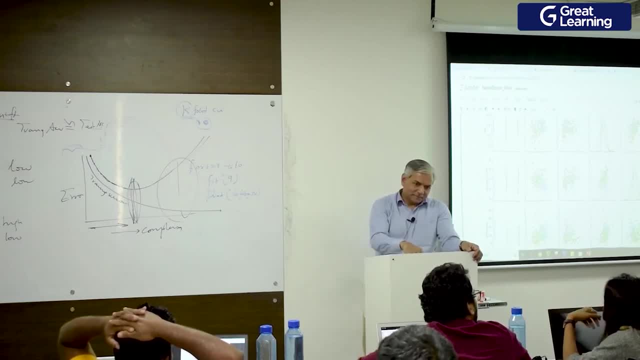 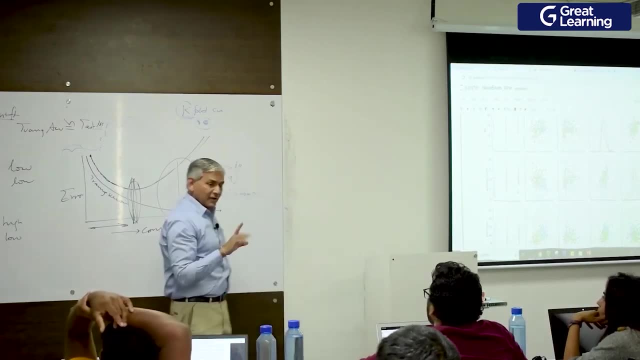 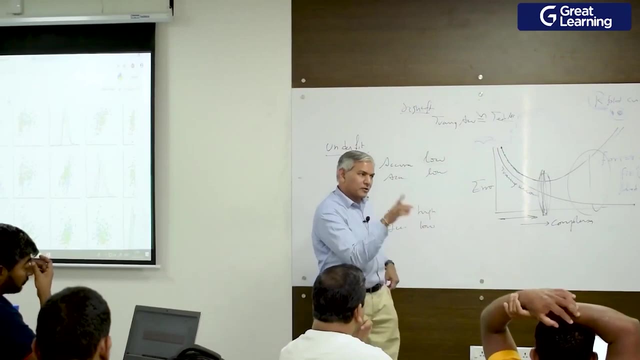 the records You have to take. yes, good point, You have to have the domain expert with you to tell you, the domain expert with you to tell you whether calculating the radius is prone to error or the perimeter is prone to error. right, because there there is a strong relationship between 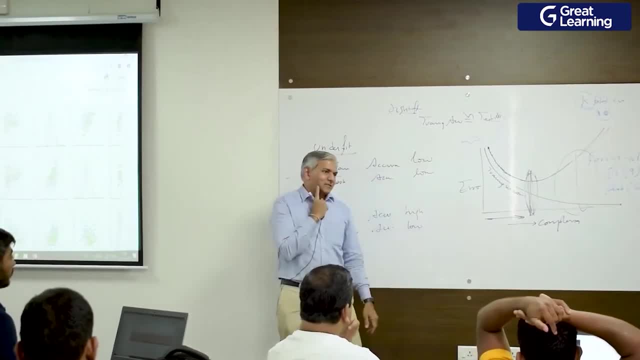 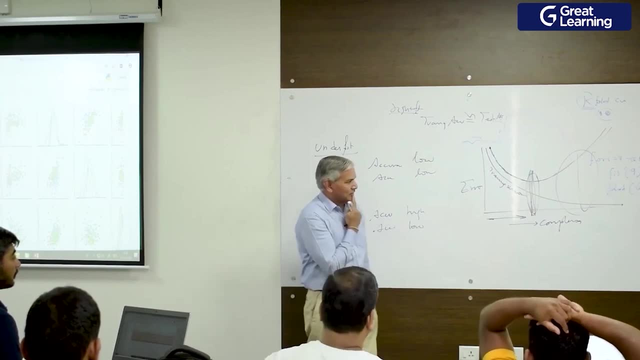 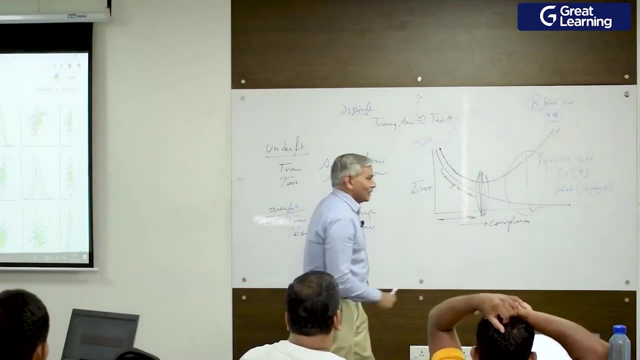 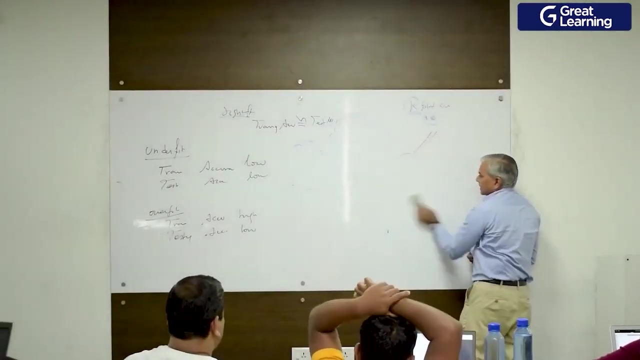 perimeter and radius. that is why you are saying that. So it depends on the domain expertise you have. Alright, okay, this one point which I wanted to say. okay, this is called data leaks and, guys, with this I am going to stop. I will not go beyond this. Be careful about. 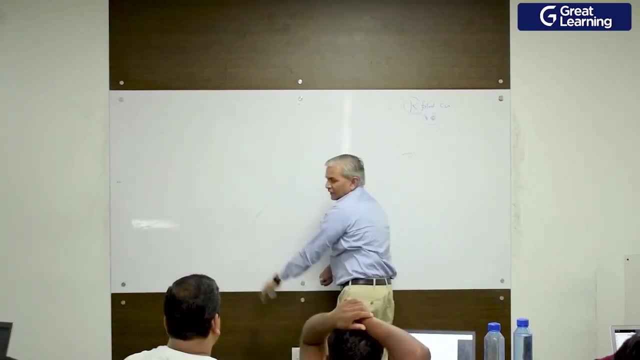 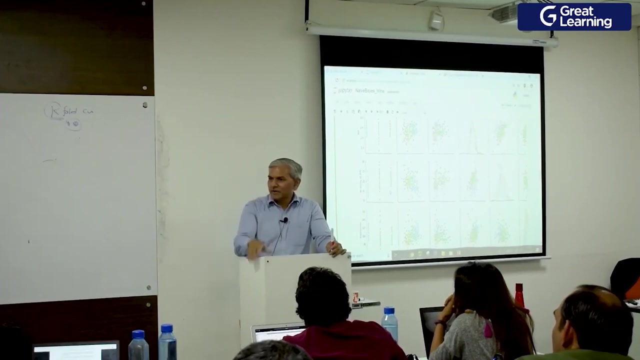 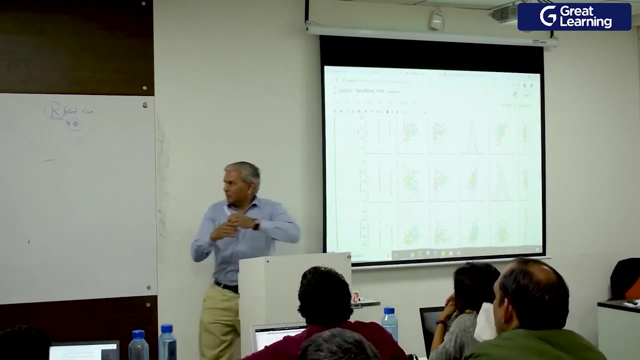 data leaks. I will tell you what data leaks is In your exams. if the question paper gets leaked out, obviously we will score very high. obviously we will score very high, right, but we might not have the real knowledge with us. Same thing can happen in modeling. So in modeling we break our data into training, set test. 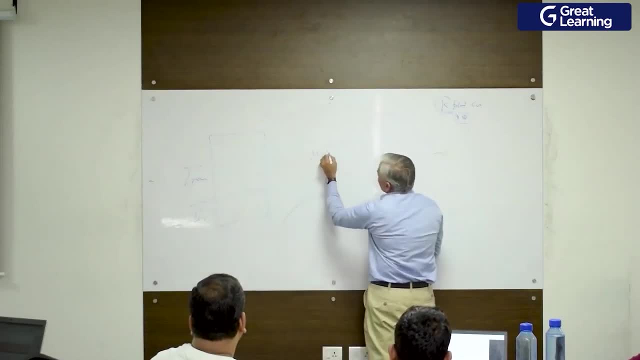 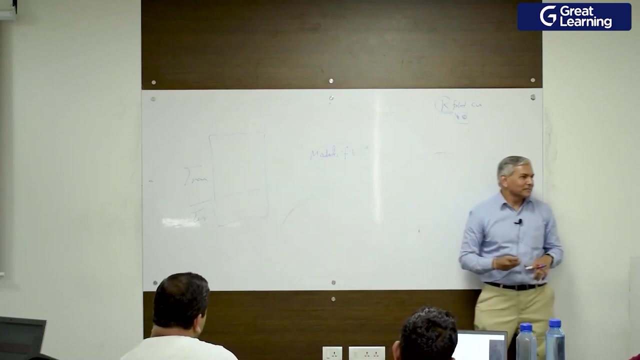 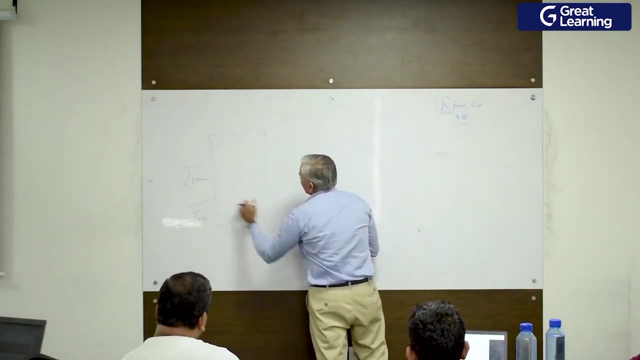 set right and we build our model MODEL FIT. we do this using training data. There are various ways in which the test data can leak into the FIT function. One of the simplest way you can do this mistake is where you first take the data, you convert this data into z score and then you split this data into 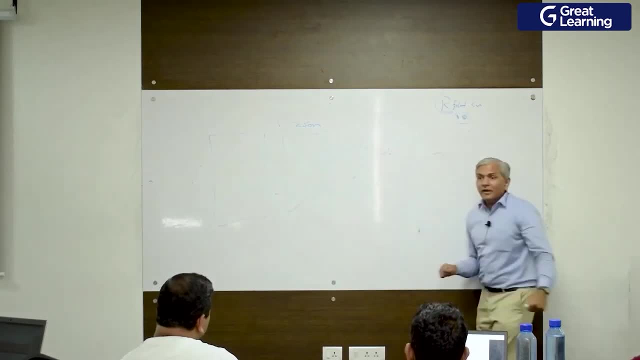 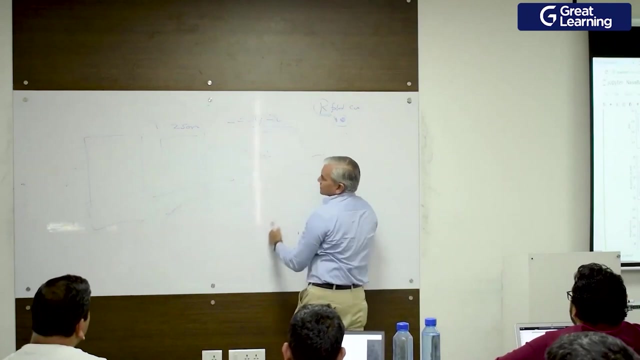 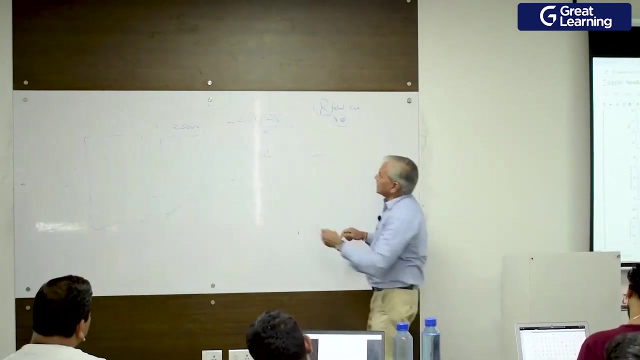 training set test set. build your model on this. Why? Because z score is xi minus x bar by standard deviation. X, i minus x bar by standard deviation is a z score. This standard deviation is a result of all the records put together. right Now, when I break this data- z score data- into this, 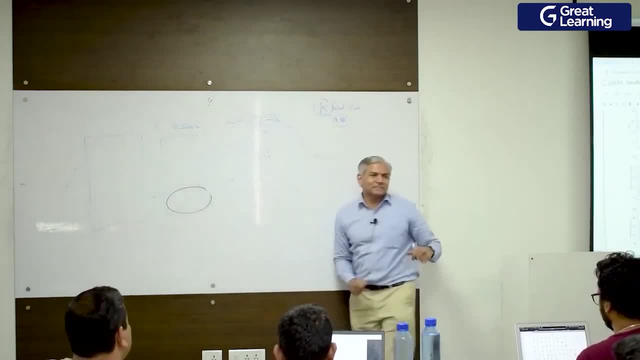 the test data is already been influenced by the training set, HONORrás. But the test data innovation because this test data, we have all the training set. everything has been influenced by the training set And we can't much understand the datasound. but 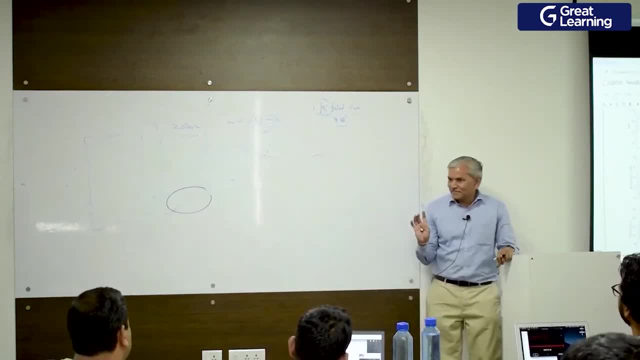 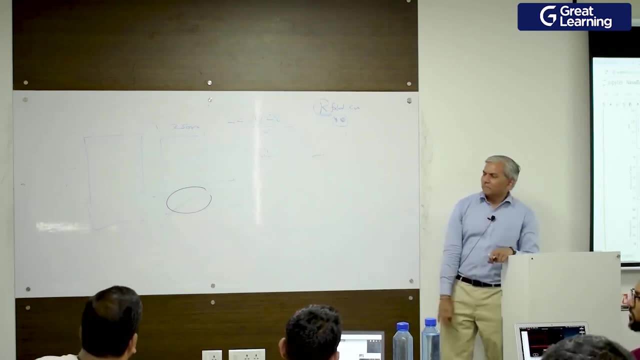 we can't downgrade any reference inside a learned ricc Er. No, we could not understand. the data should have been influenced by the training set. They are not independent of each other. This is a very common source of data leaks In the classroom. it is ok, but you cannot. 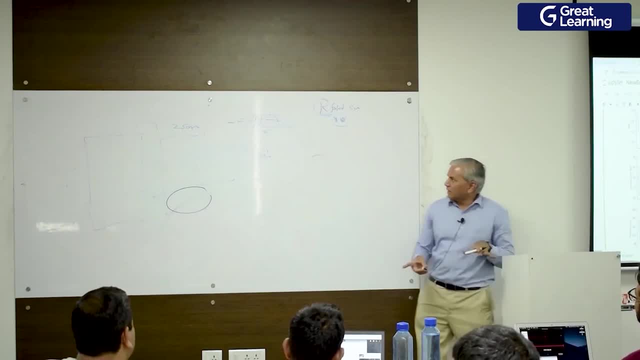 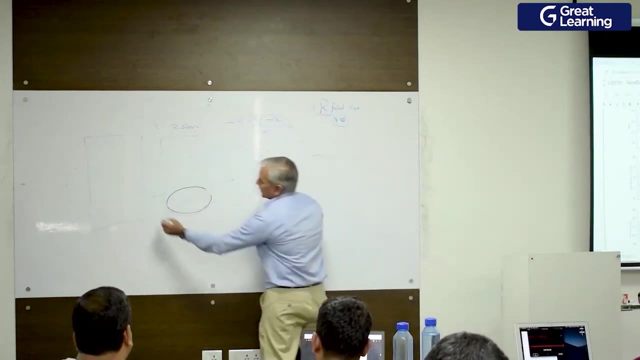 do this in your projects, Then what will happen is your model will perform well on test but will bomb in production. That is one very common way of data leaks. So whenever you do transformation of your data from raw to this, if the transformation involves all records- 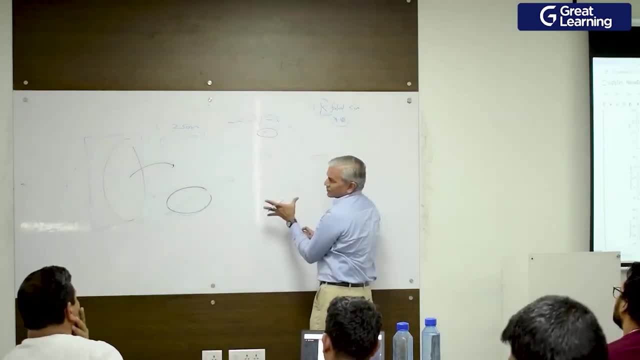 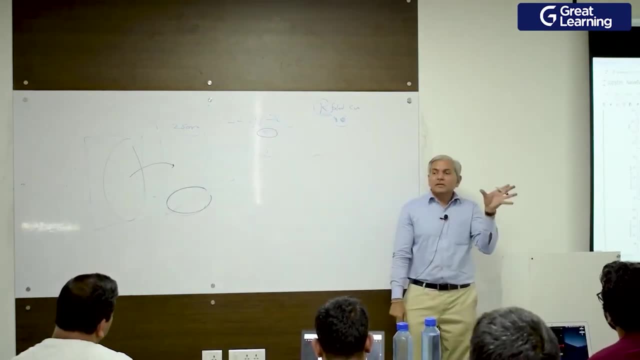 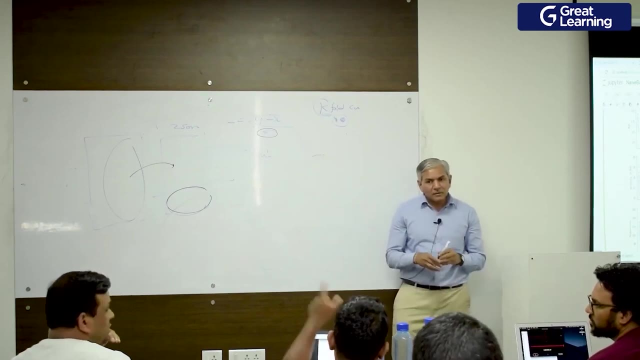 put together to find your standard deviation, something of that sort. don't do that Always. break your data into training set, test set first, then do the transformations. I think we did this for the data. First Python node to complete the data. We are doing. we will do this mistake in entire all the Python nodes. Ok, I think we did this for the data First Python node to complete the data We are doing. we will do this mistake in entire all the Python nodes. 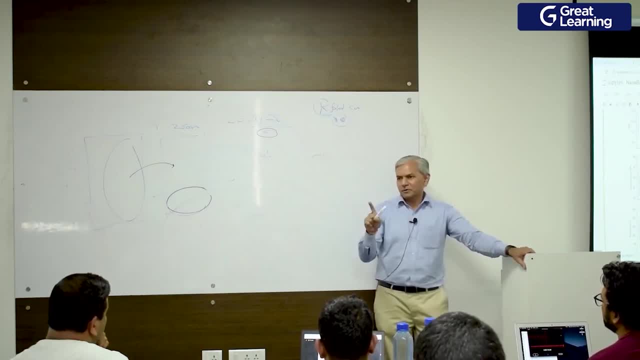 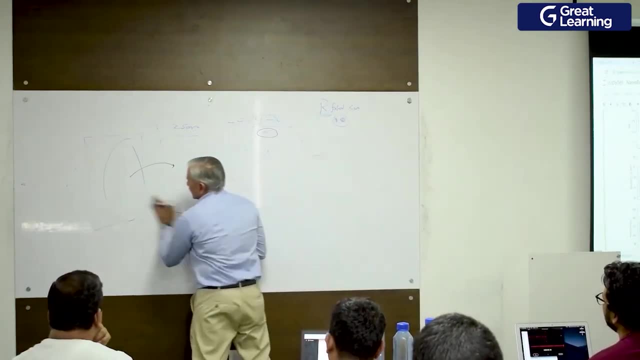 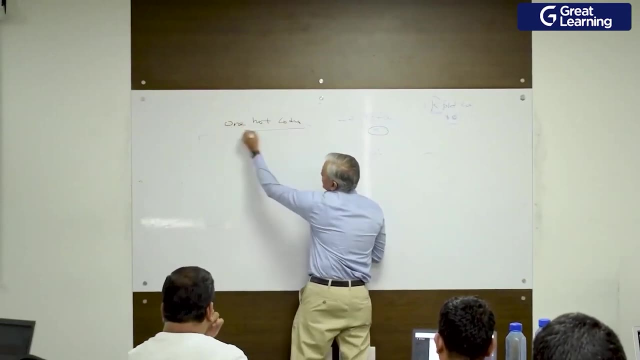 But you please be aware of this, don't do this in your projects. The second thing I will tell, Second problem statement, is: we talked about 1-0 coding. We talked about 1-0 coding right. Look at this. You have in your data set a gender column. 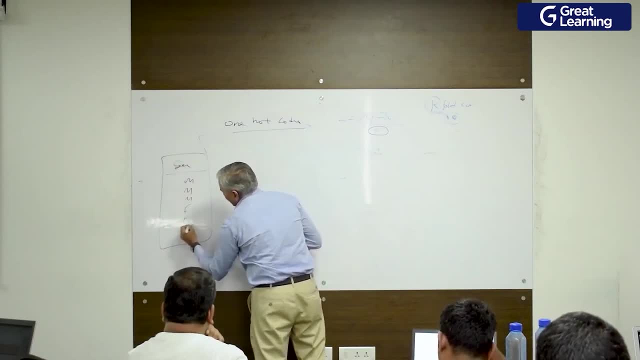 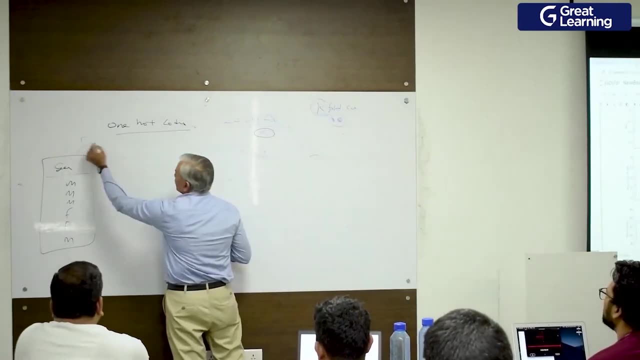 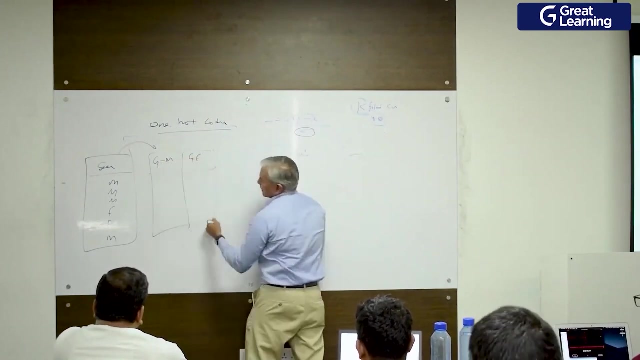 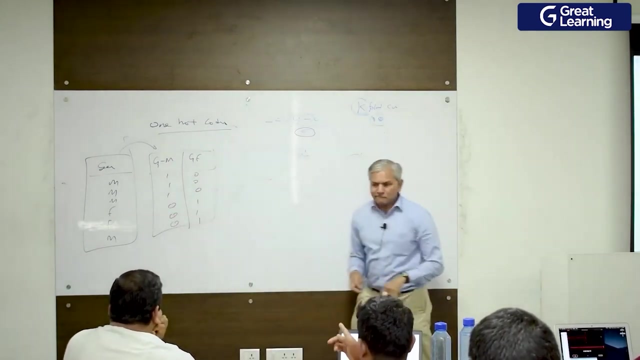 which has male, male, male, females, females. ok, males, Always convert the one-hot coding first so that it becomes gender male, gender female. This will become 1-0, 1-0, 1-0, 0, 1-0, 1-0, 1, 1-0, 1, 1-0, 1-0, 1-0, 1-0, 1-0, 1-0, ok. 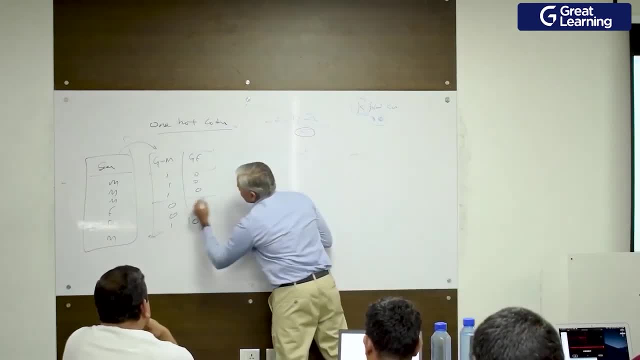 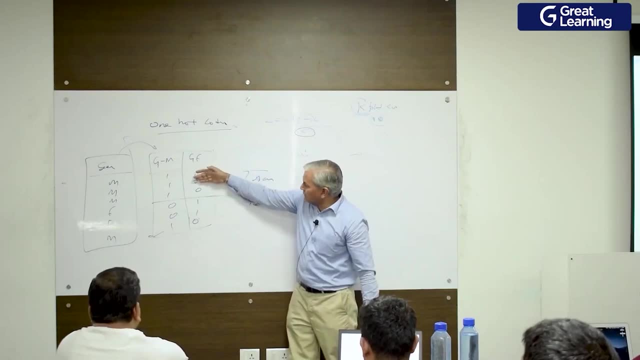 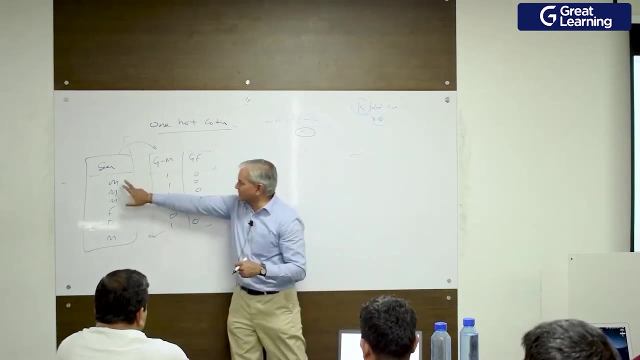 All of you got it. Then you break your data into training set: test set. This is ok: Training test. The reason why this is ok is this record has not been influenced by any other records. The records don't influence each other. The transformation of records from. 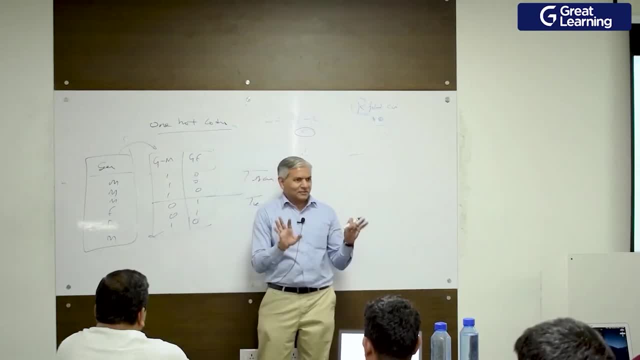 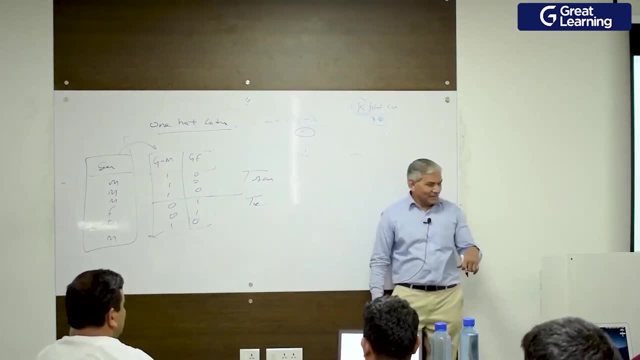 here to here is independent of other records, So this is ok. ok, If you do this transformation after breaking your data into training set test set. I told you in z-score you first break your data into train set test set. ok, Then first do. 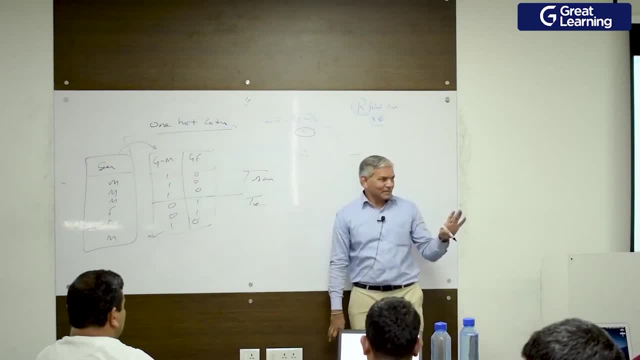 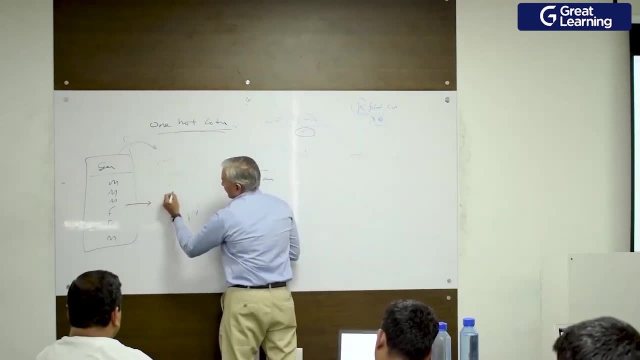 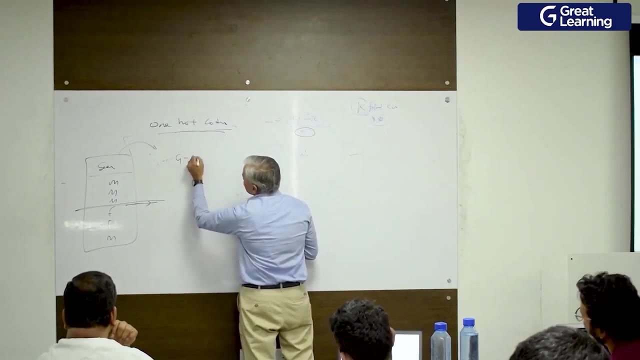 z-score on training, Then do z-score on testing separately. If you do this one-hot coding after breaking your data into training set test set- Now I break this into training set test set- What is going to happen is, in your training set you are going to have only one column. 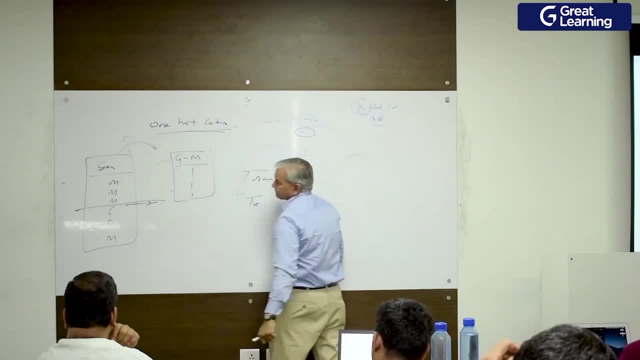 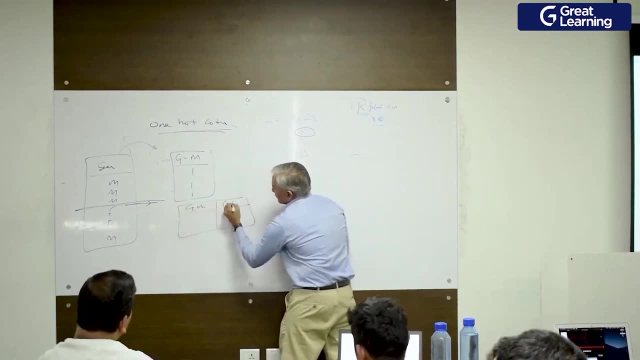 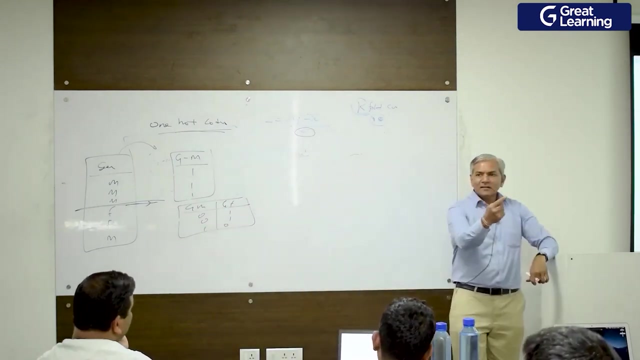 gm: 1, 1, 1.. In your test data you are going to have two columns, gm and gf. This will be 0, 1, 0, 1, 0. So your training data and your test data will not match in terms of the attributes. 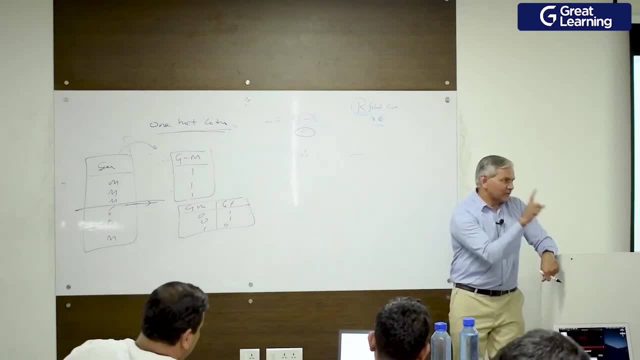 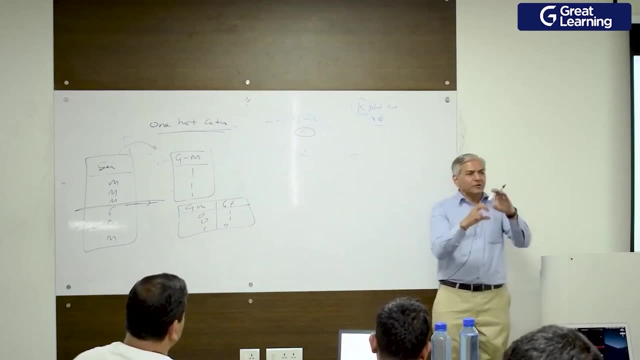 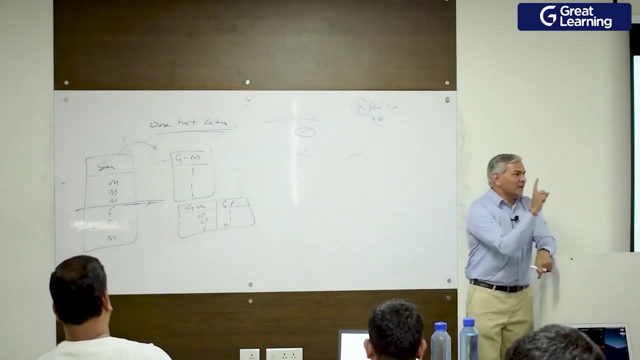 So whenever you are doing transformation, if the transformation is something which is done record-wise, do it first. then break your data into training set, test set, Especially one-hot coding, Otherwise you will end up in run time problems If you are doing any. 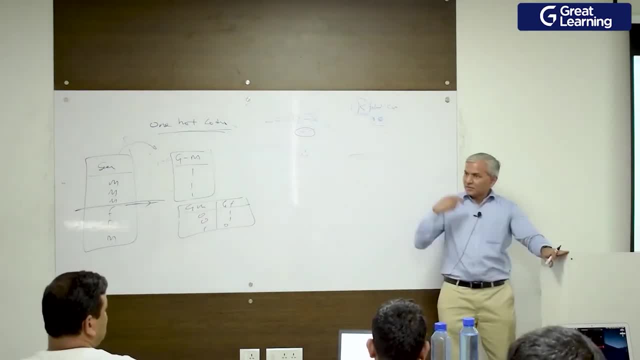 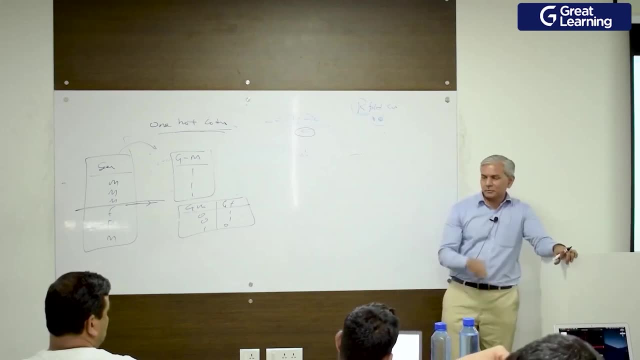 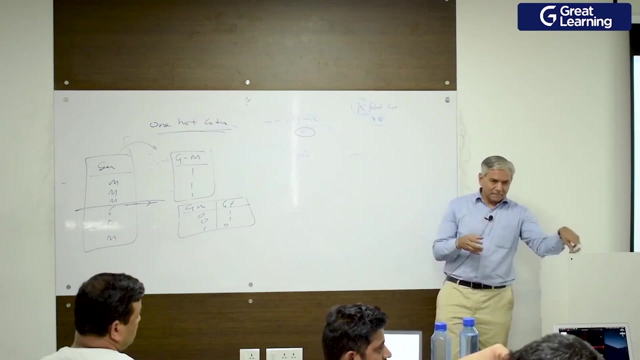 transformation which involves all the training data test set, then you are not going to break your data into training set test set. If you are doing any transformation which involves all the records put together, like calculating standard deviations, then first split it, then transform it, otherwise your data will leak. 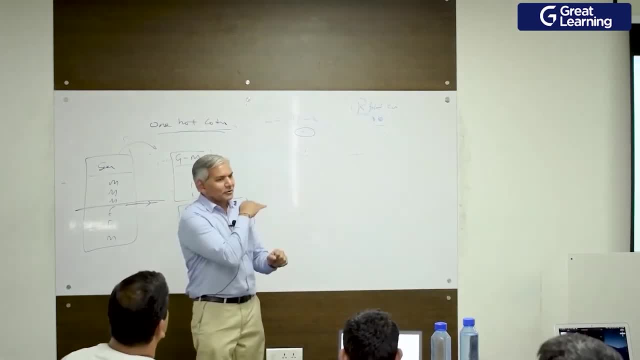 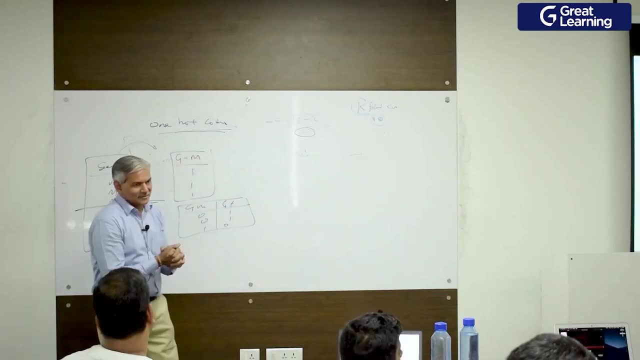 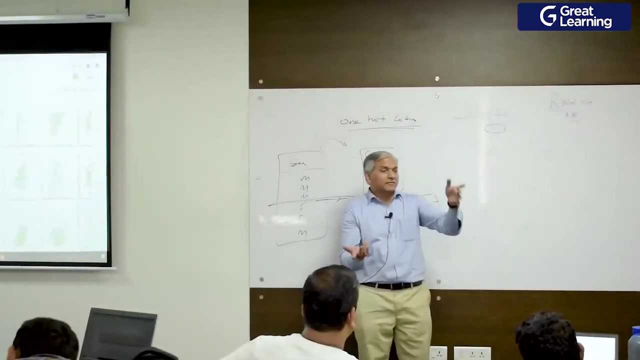 Yes, you are. the moment you add dimensions, you are going towards higher complexity of your models, so you are decreasing the bias error but increasing variance errors. So if you create one odd coding out of a column where the cardinal values, the distinct values, is 50, you are going to end up with 50 new columns. 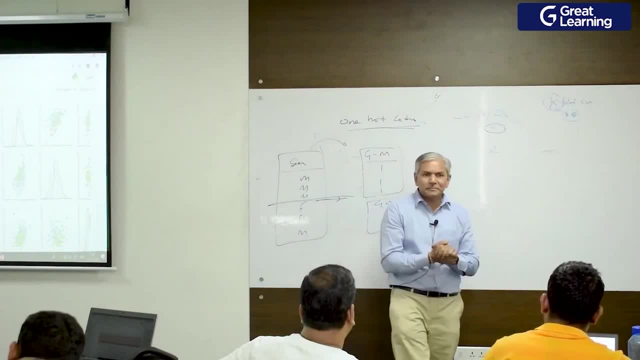 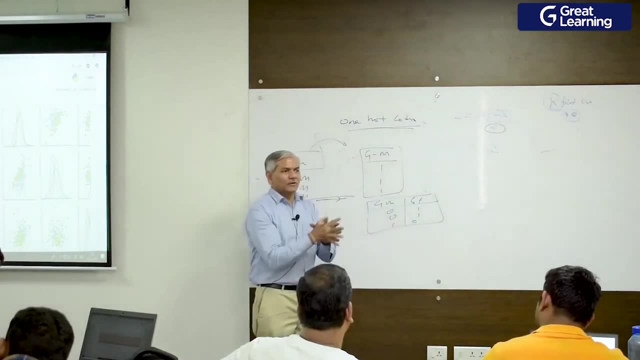 So imagine, from lower dimensional space you are going to such a high dimensional space and your data points is also not very high. you will end up with a very complex model. so you will end up in over fit zone variance errors. So why we need to do that? we can still do 0, 1 as the value for. 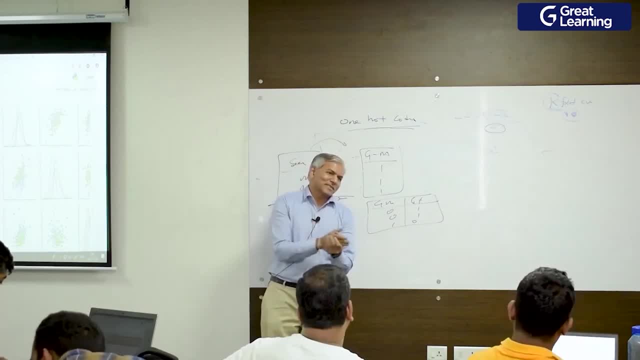 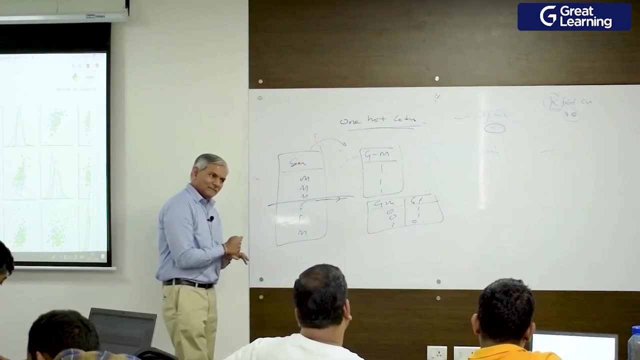 Algorithm will think that 1 is greater than 0.. Here if we have three categories- A, B, C, D, C- and we do a little encoding first, so it will come up to 1,, 2, 3, in this case it might think that C is the higher value. 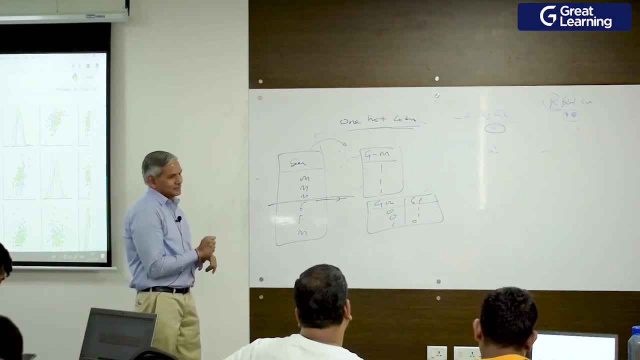 It will, it will. So what we will do? we will do one more time, One more time. So it will come up to 2, 0, 0, 1, 0, 1, 0, as per the sequence. 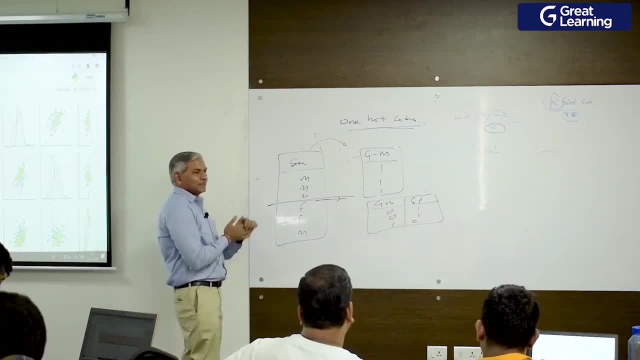 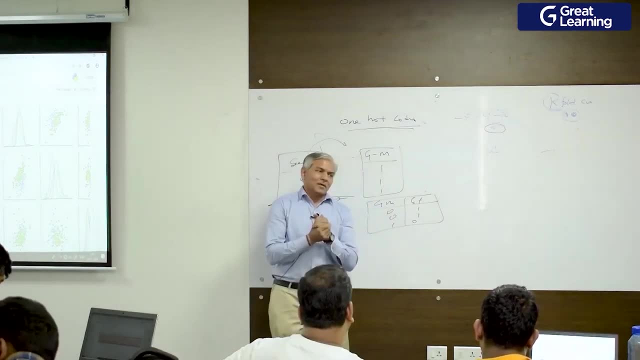 Correct. So in this case, if we drop one of the variables, the variance will also decrease and we can predict that if it is 0, 0, then maybe that variable will be 1.. So we can do that. Yeah, okay, one one, sorry. one last point, last test point. 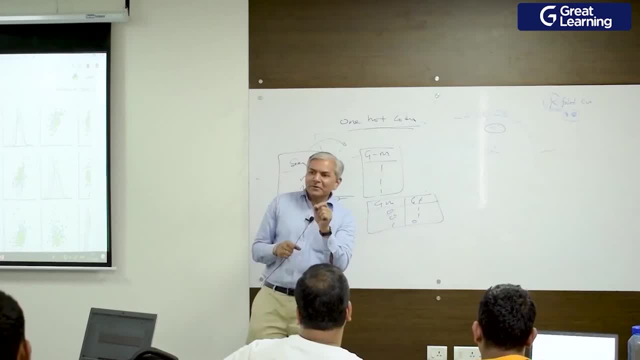 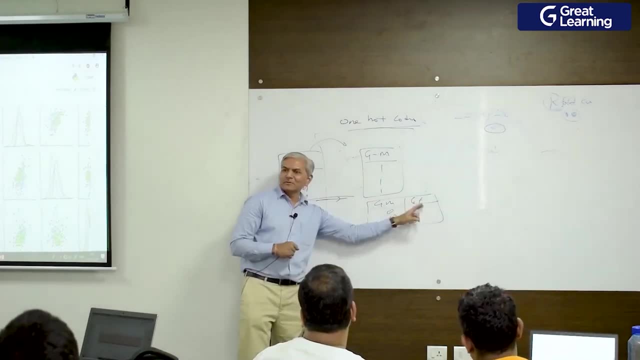 This we have been saying since last three points: Whenever you create one odd coding, for example- in this case, you are creating collinear columns, columns which influence each other- The presence of 0 here tells me that this column will be 1.. 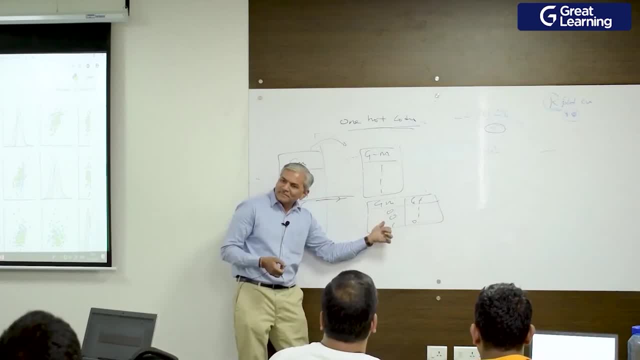 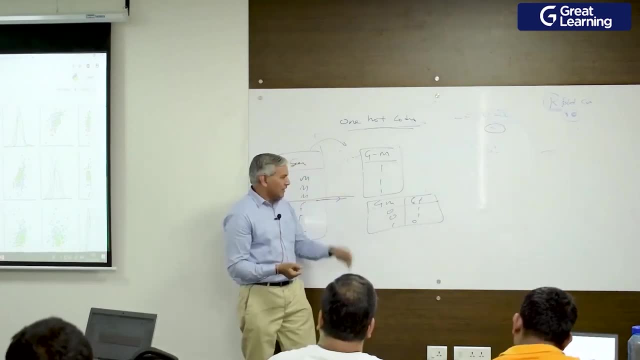 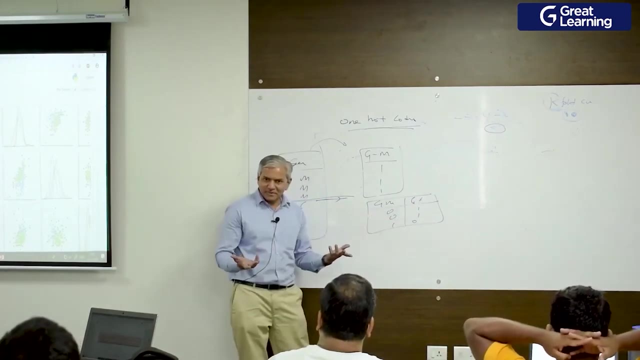 So I am able to predict the value of the other column based on this column. So you are introducing collinearity over here To address this collinearity problem. when you create one odd coding we might drop one of the columns. So 0 means male, 1 means female. 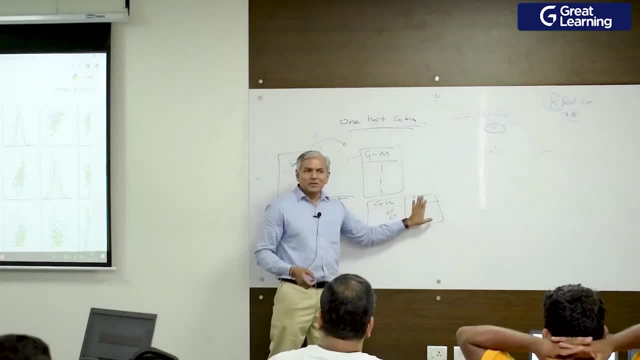 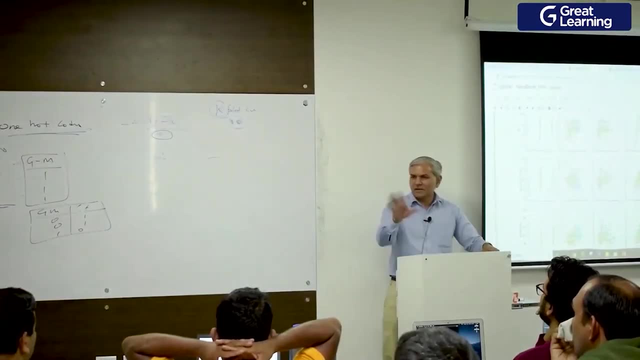 So I get that information from here itself. I do not need this. So when you do one odd coding, you are introducing multi-collinearity. When you bring multi-collinearity, you know what problems exist, what problems happen. 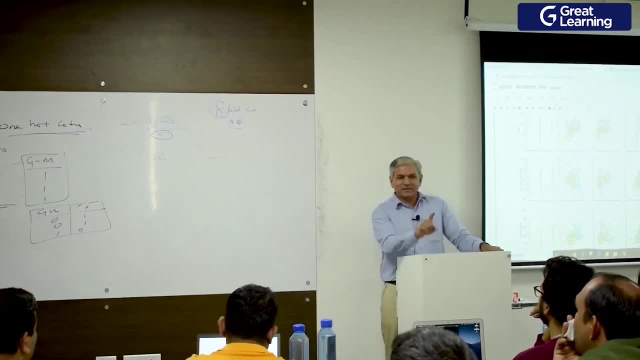 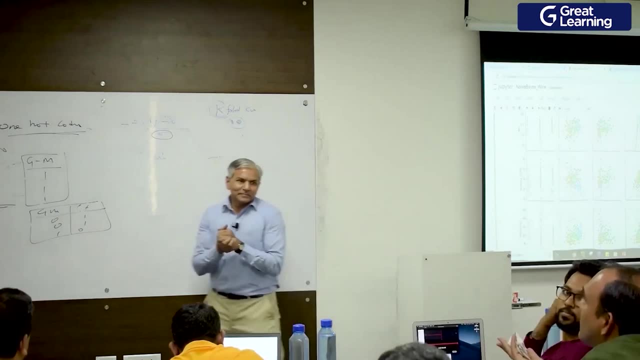 you know that. So we might have to drop some of these one odd coding columns to remove the multi-collinearity. We do that Again. we have 0, 1.. Again, same issue 1 is. But the purpose of one odd coding is: 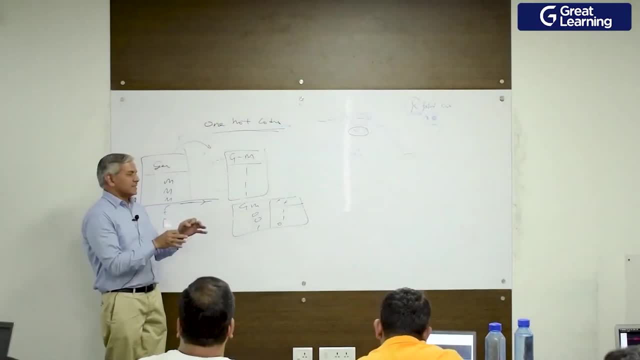 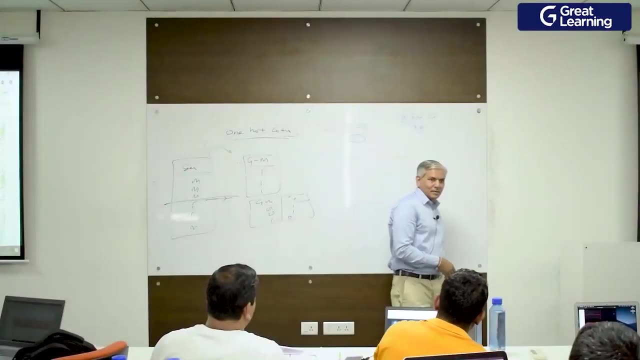 One odd coding does not introduce any order. It just stores it as a label: 0 and 1. So we can also convert the variables. Unfortunately, when you do that, when you use Pandas DataFrame categorical function, it actually says that it is ordinal values.